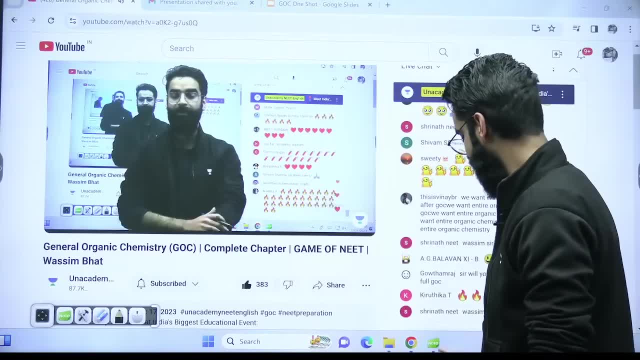 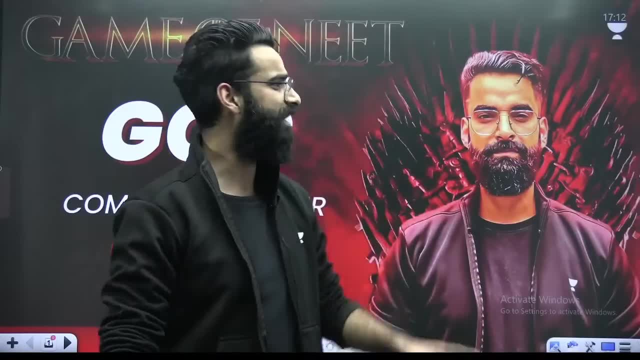 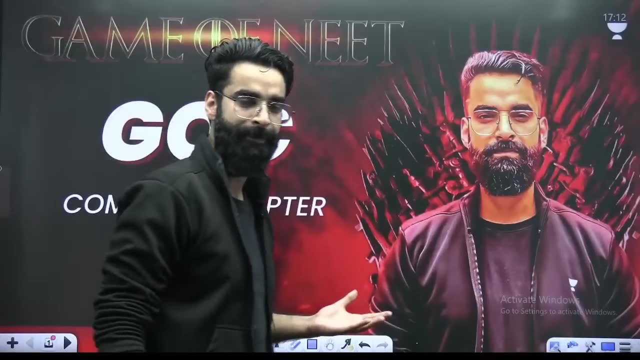 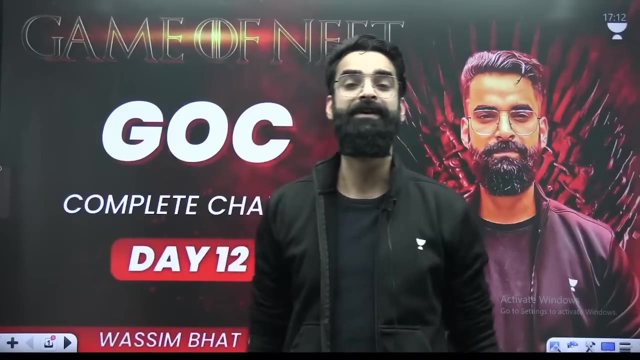 It's not day 12,, it's day 13, right? So, people, today we shall be doing the general organic chemistry, GOC, right? One of the high-weighted chapters of your chemistry, Perfect, And this particular chapter is involved. almost, I won't say almost, I would say- this particular chapter. 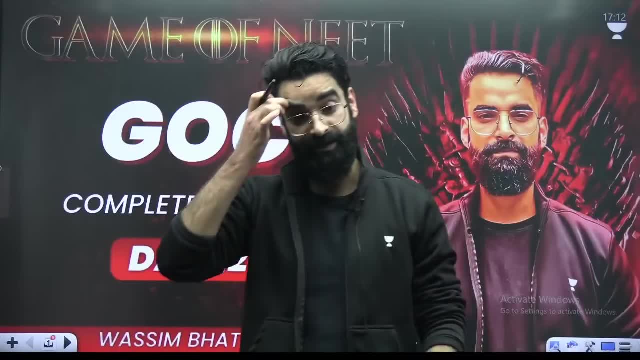 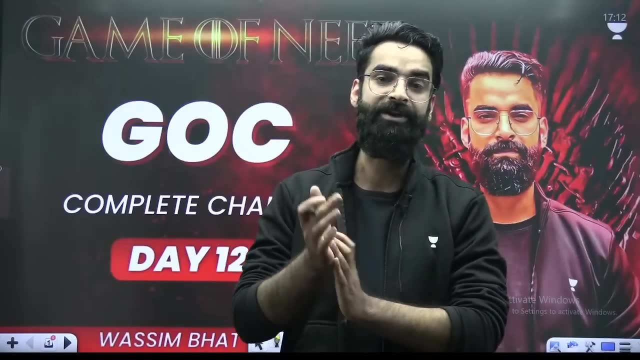 it's involved everywhere when it comes to your organic chemistry, right? So if this particular chapter is stronger, that means your entire organic chemistry is automatically going to be strong. If there are doubts in this particular chapter, that means there will be doubts in the entire organic chemistry. 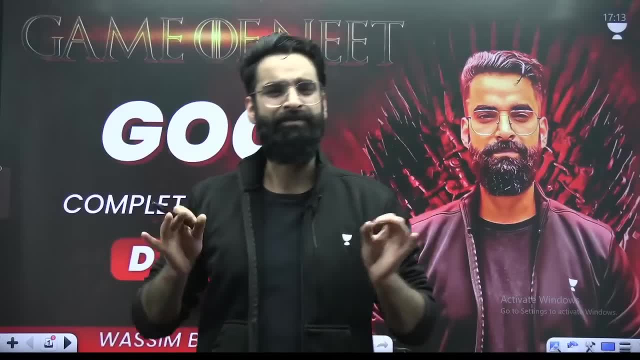 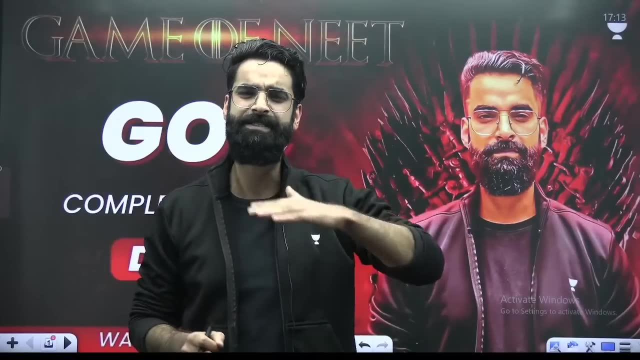 So I've decided to start exactly from the basics, from the scratch, as if you have never studied this particular chapter before. Okay, We'll be starting from the scratch, from the basics, and slowly, slowly, slowly, we'll be scaling up the things as well. 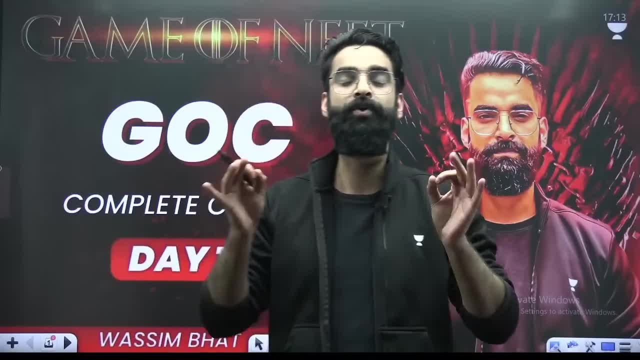 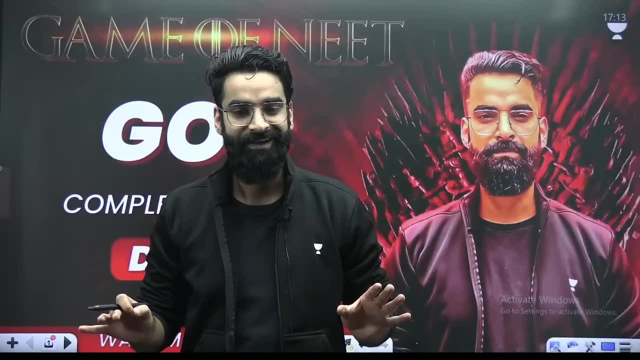 It is just, I would want you guys to call up everyone, Everyone Whosoever is preparing for NEET 2024 or even 2025, I would want you guys to call up everyone. right, Let everyone taste. GOC by Vasim sir, this time, yeah. 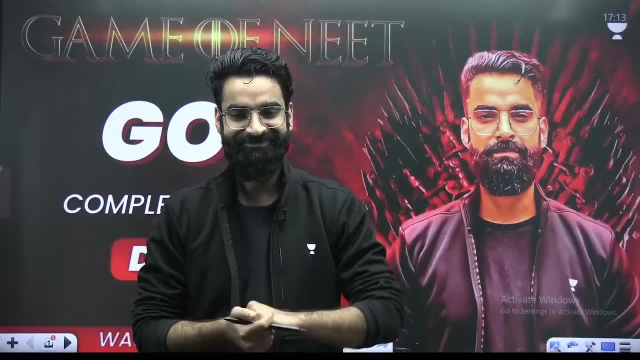 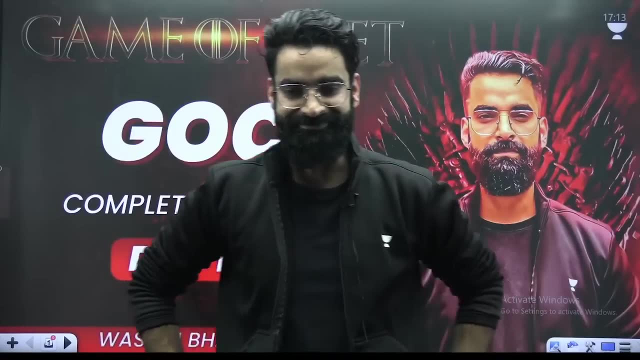 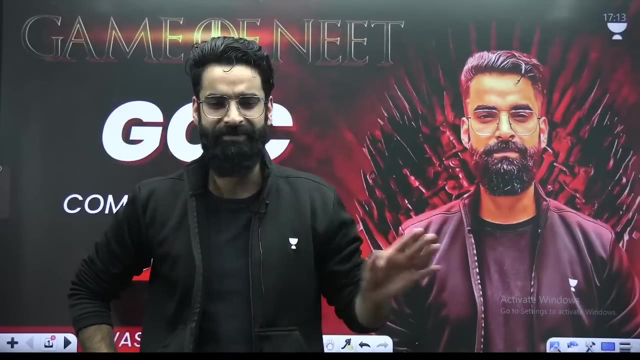 All ready, All ready, people, All ready? yes, Guys, I want the chats to run continuously. Yes, NEET students, JE Students, everyone, Everyone is welcome. Right, This is for everyone. This is for everyone. 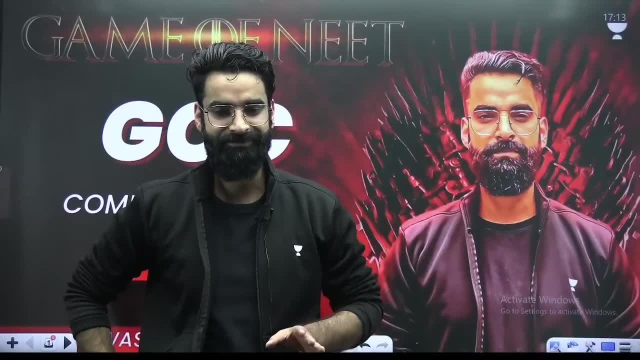 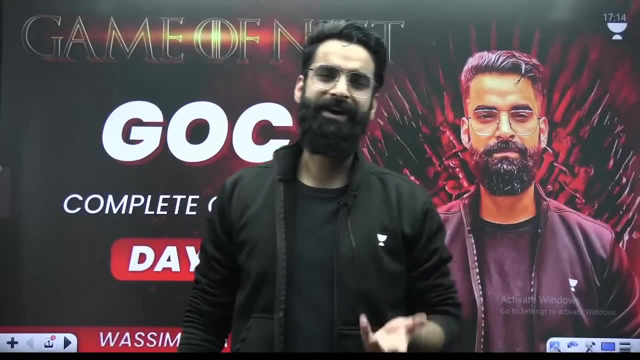 This is for everyone. I don't want the chats to stop at all. I do not want the chats to stop at all, And a lot of people are asking how long will it take to complete the general organic chemistry Ideas? students have no idea. 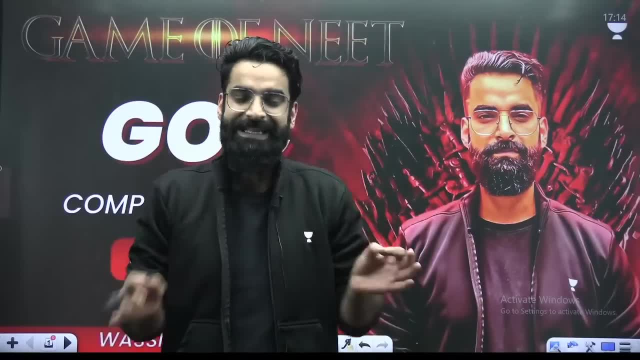 It can take 8 hours, It can take 10 hours, It can take 12 hours, Till the chapter is over. I'll be with you and you will have to be with me as well. So are you ready to be with me till the end? 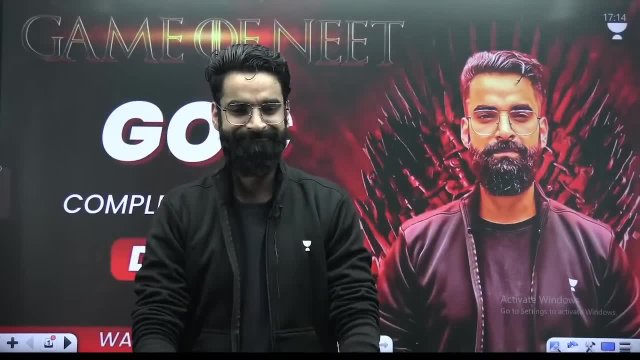 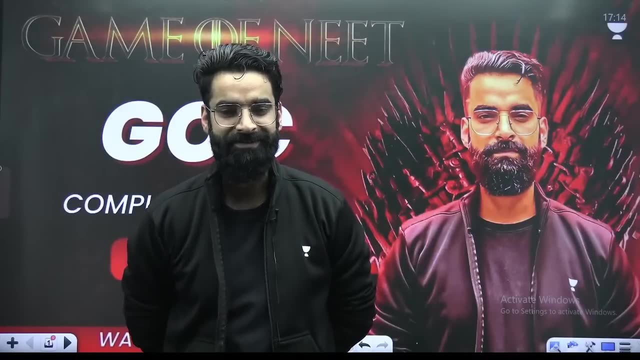 Are you ready to be with me till the end? Quickly, Quickly, then only I'll be starting. Are you ready to be with me till the end? Perfect, guys, Perfect. This is something which I wanted from you. Yeah, this is something which I wanted from you. 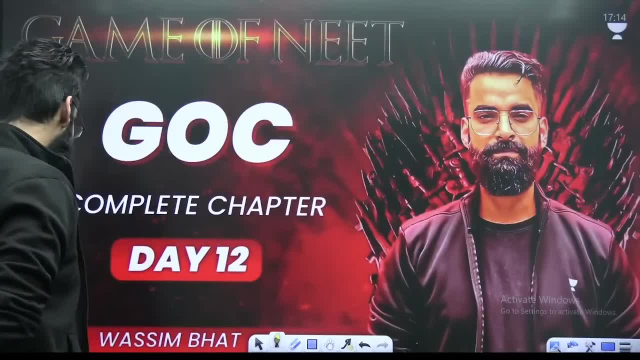 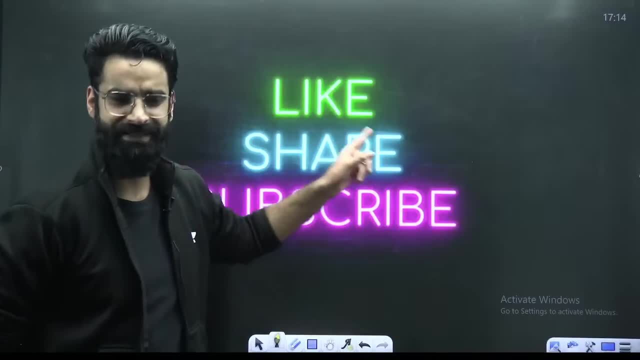 So, people, before starting this particular chapter, before starting this particular chapter, the ones who have not liked the session yet. I can see not everyone has liked the session yet. I would want every one of you to like the session right now. 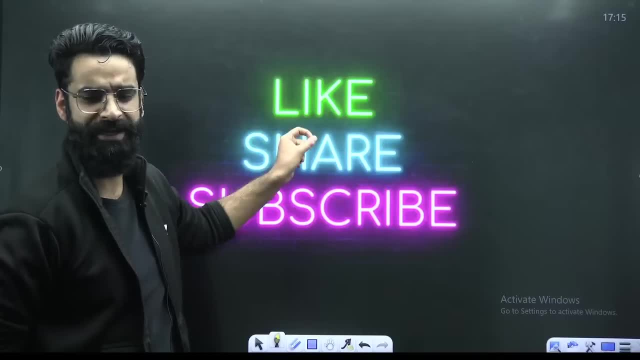 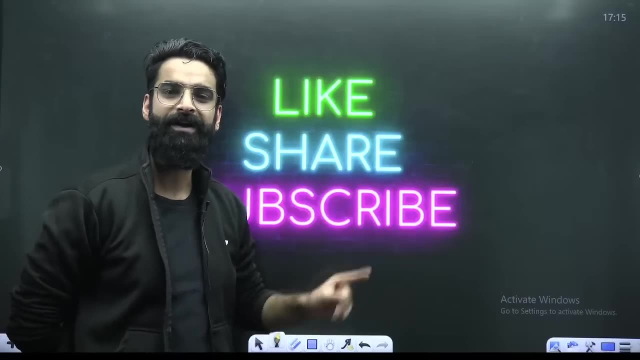 If you have not shared this particular video with everyone, I would want you to share this with everyone Who's server is preparing for NEET, 2024,, 2025 or even GE. share this particular video with everyone And the ones who have not subscribed the channel yet. 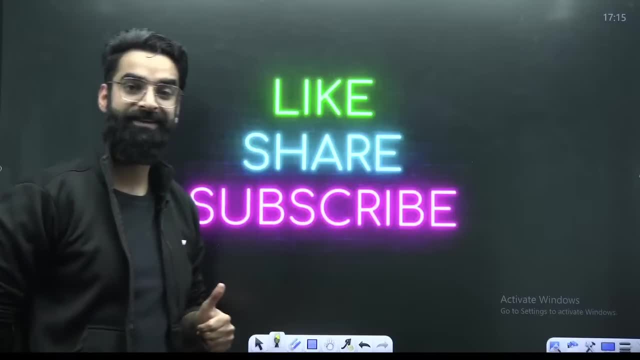 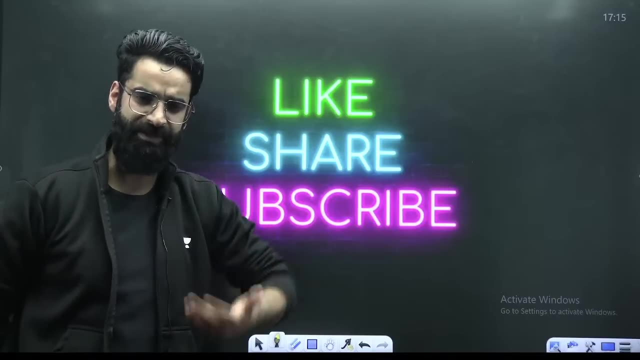 I would want you guys to subscribe to the channel as well. Right, Perfect, Okay. so, before starting this chapter, few announcements I need to make over here, and then we shall be starting. Yeah, So, dear students, as you all must be knowing, 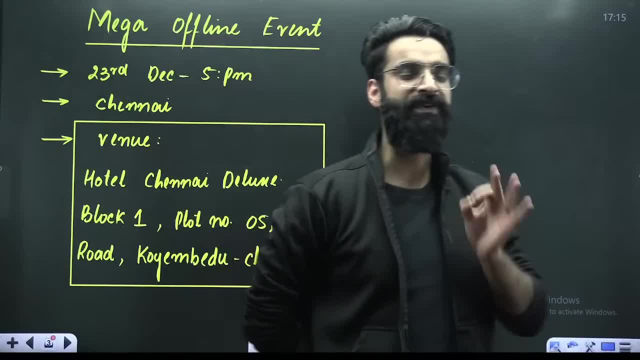 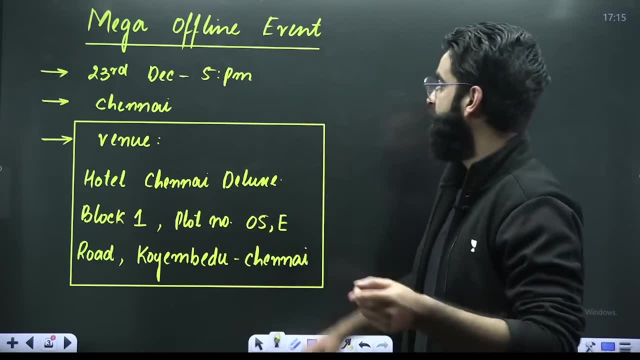 there is one mega event, mega offline event, which is going to happen in Chennai on 23rd of December. That means coming Saturday, Right? So this mega event is going to start exactly at 5 pm, Right? The venue of this particular event you can see over here. 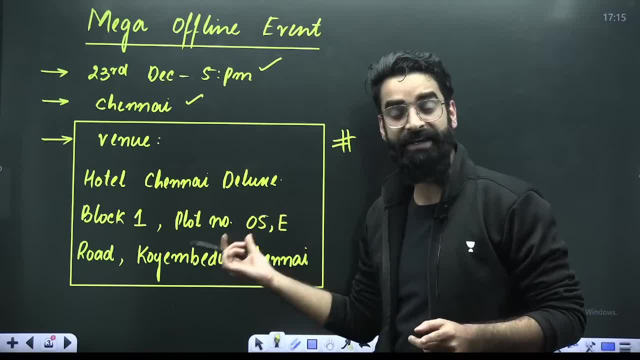 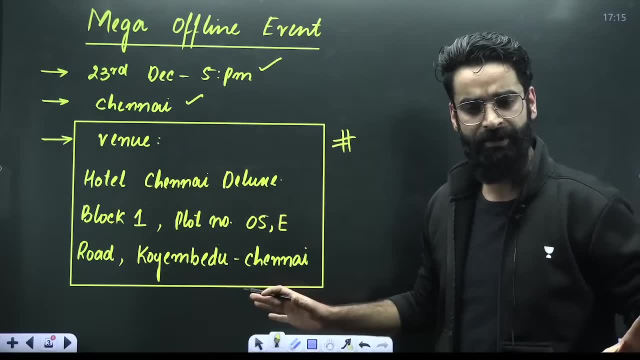 Right, I have mentioned the exact address, where exactly you guys are supposed to come. You guys can come with your friends. you can come with your family members, your parents, whosoever you want to be with. Everyone is most welcome in this particular event. 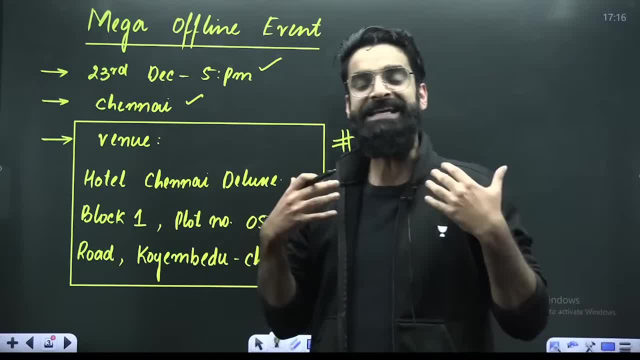 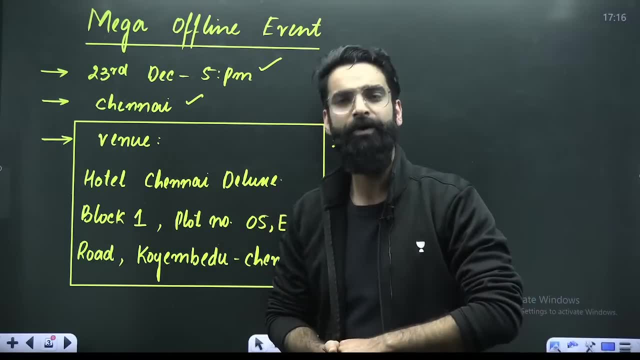 And in this event there will be- I mean, we NEET English team, complete NEET English team, will be there in the event. We'll be addressing you in person. Right, There'll be a lot of NEET toppers as well. 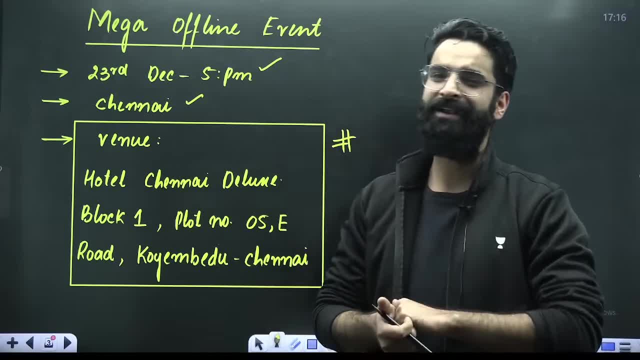 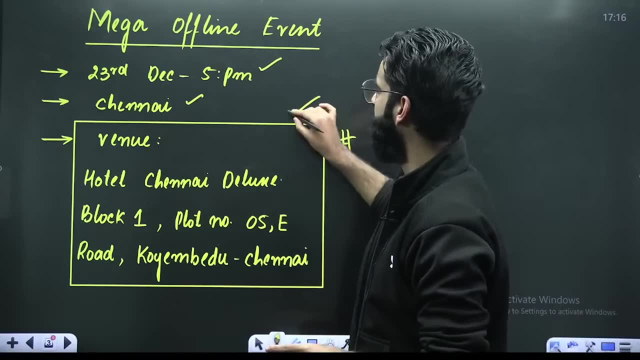 who have qualified this particular NEET examination with amazing scores, and they'll be addressing you at the same time. So if you are preparing for NEET 2024 or even 2025, right, You guys are most welcome in this particular event. 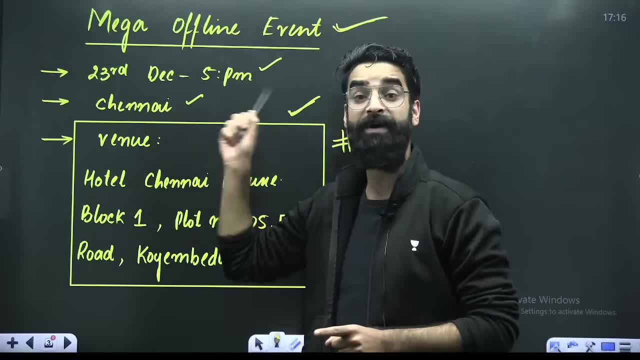 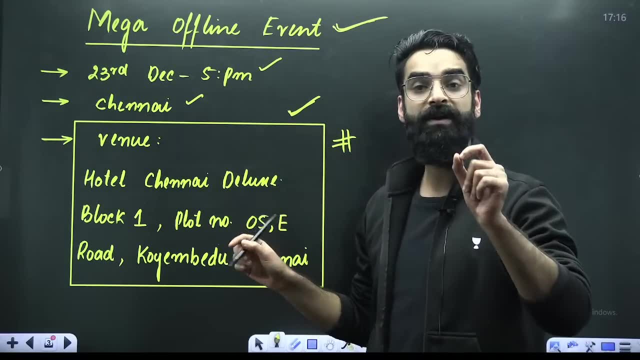 Right, The Chennai event which is going to happen on 23rd of December sharp at 5 pm. Okay, And and, and, and, My dear students, in order to attend this particular event, you just have to. 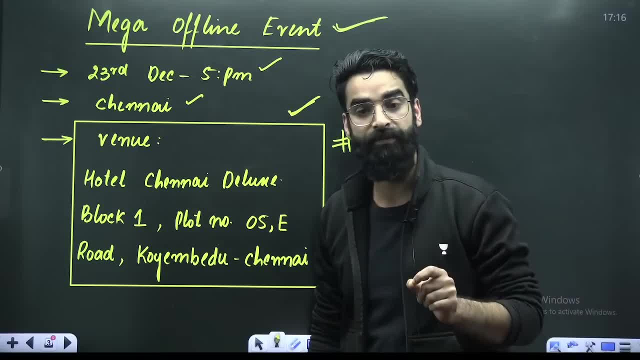 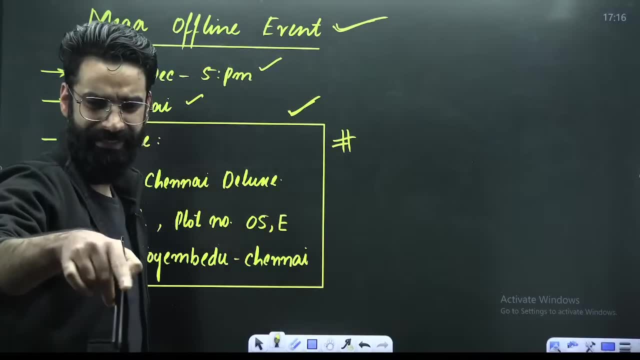 fill one Google form. Right, You just have to fill one Google form. That Google form you can find in the description of this particular video, or you can see the chats. basically, Right, You can see the chats. In the chats there's a link which is pinned. 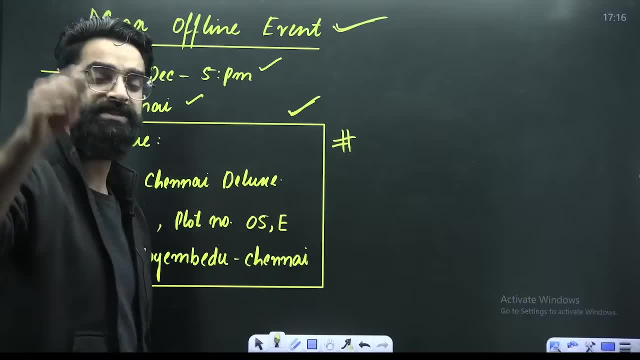 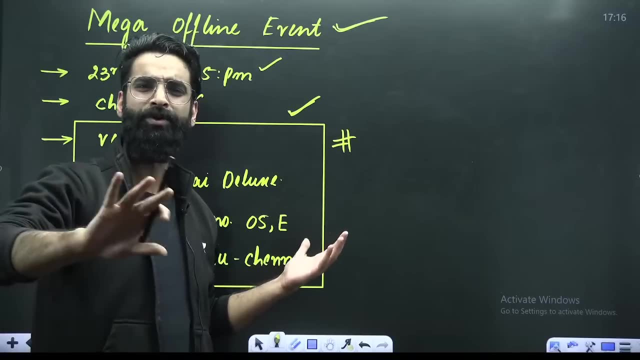 You just have to click on that link and after that, right after that, you just have to fill the Google form. if you are really willing to join this particular event, Okay, And it's not going to take you more than 5 to 10 seconds to fill that form as well. 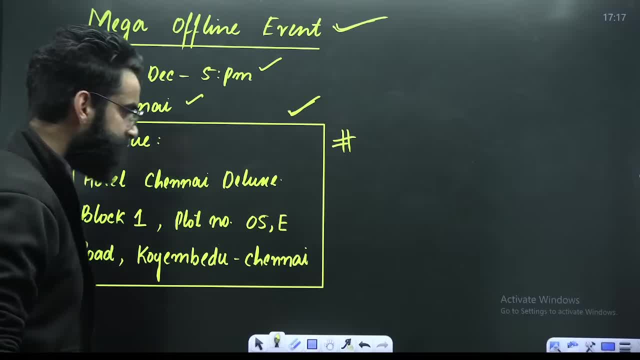 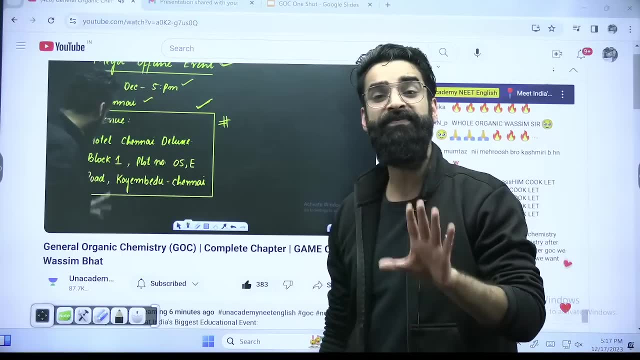 Yeah, So do that right now. Number one, Number two, Number two, my dear students, So today we are completing the chapter General Organic Chemistry, GOC. Okay, And as you all must be familiar with the fact, 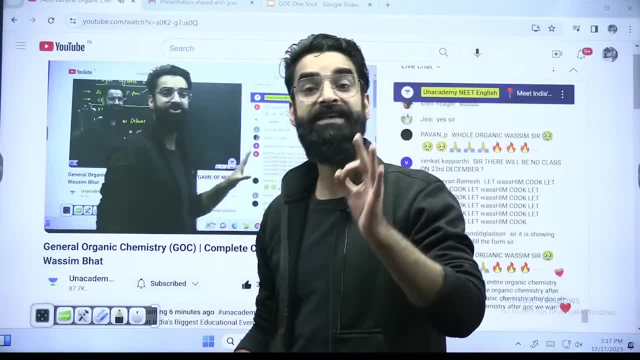 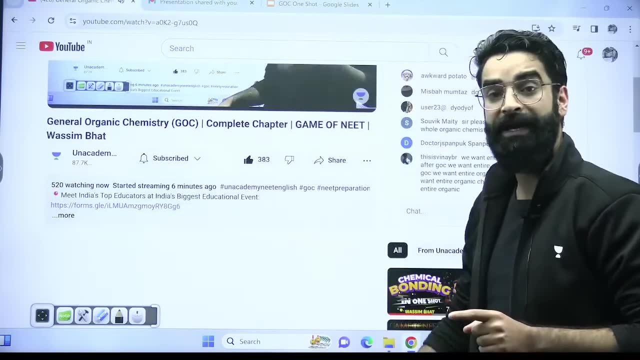 after completing a chapter here on YouTube, what do we do? We do extra problem practice. We do extra problem practice And extra problem practice. how exactly you are going to attend that? See, this is the video. Click on more. After clicking on more, here you'll find a link. 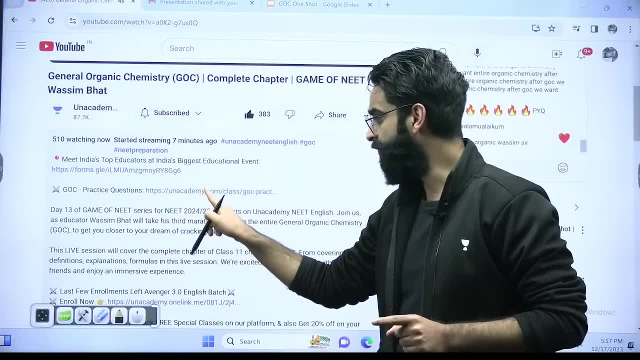 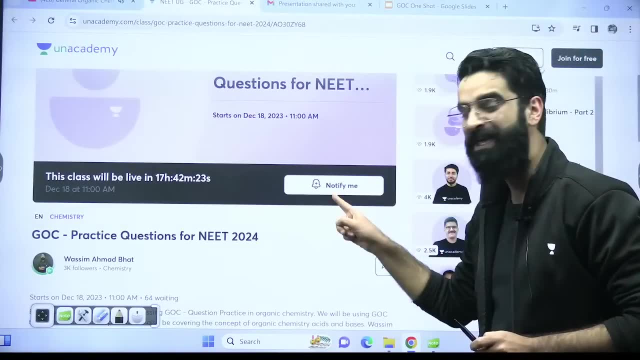 GOC Practice Questions. GOC Practice Questions. there's a link. You just have to click on this particular link. Once you click on this particular link, my dear students here you have to click on, Notify Me. And tomorrow at sharp 11 am. 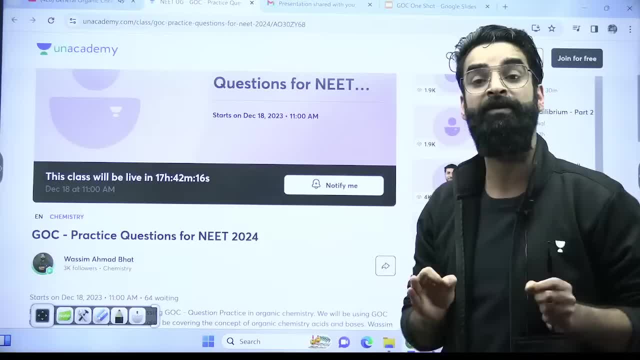 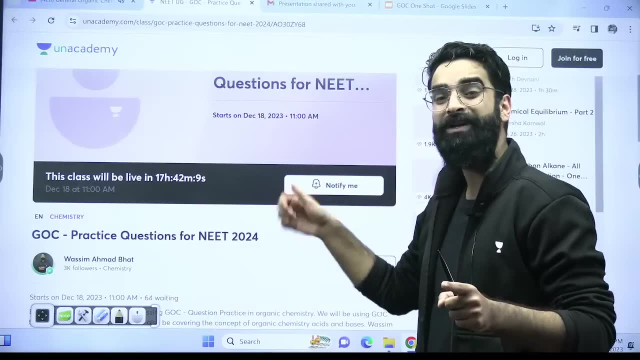 Tomorrow at sharp 11 am we are going to have extra problem practice for the chapter General Organic Chemistry. Are you ready for it? The ones who have not clicked on the link yet. I would want you guys to do it right now. 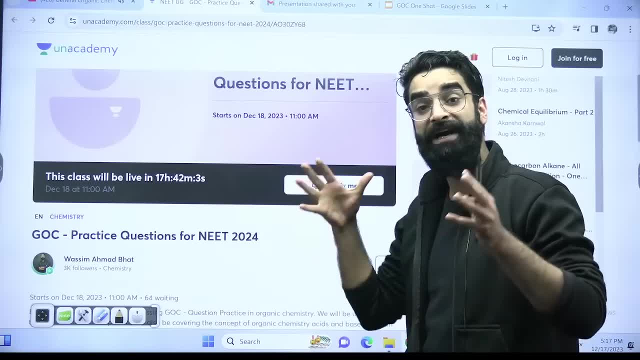 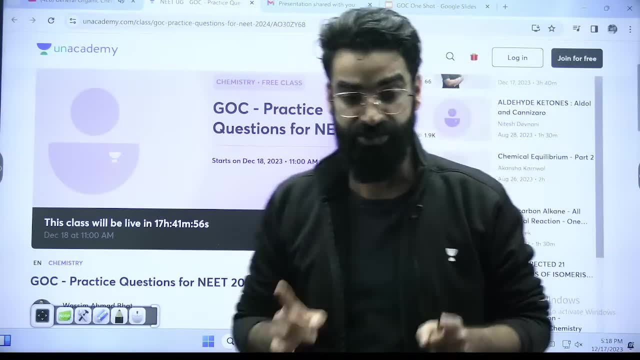 Right now with me. right And click on this. Notify Me so that you will remain updated about this particular extra problem practice session, which is going to happen tomorrow at 11 am sharp on the Unacademy platform. Yes, Are you all done with this? 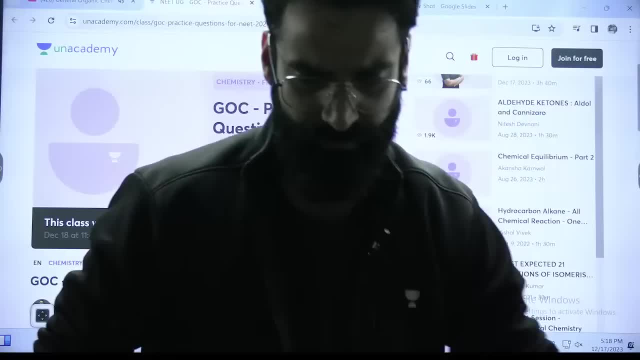 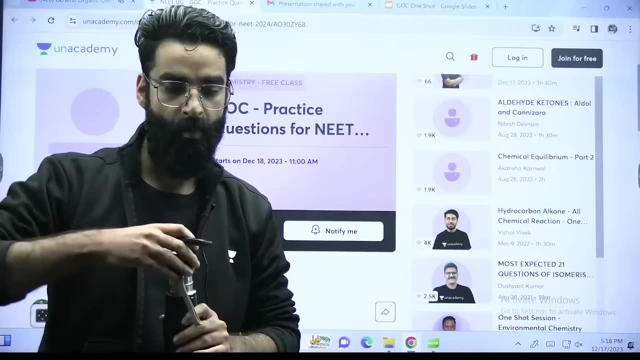 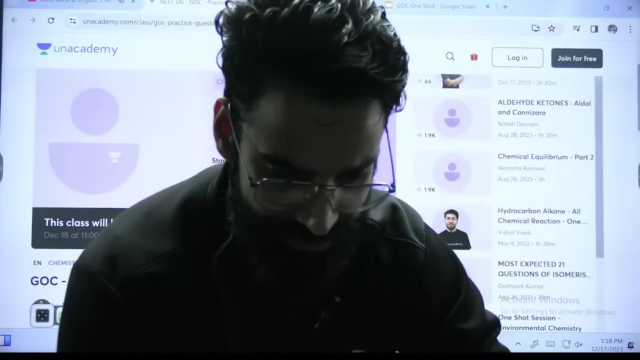 Are you all done with this? people, Quickly, Are you all done with this? Are you all done with this? Yes, Are you all done with this? Yes, Are you all done with this? Yes, Yes, So should we start now? 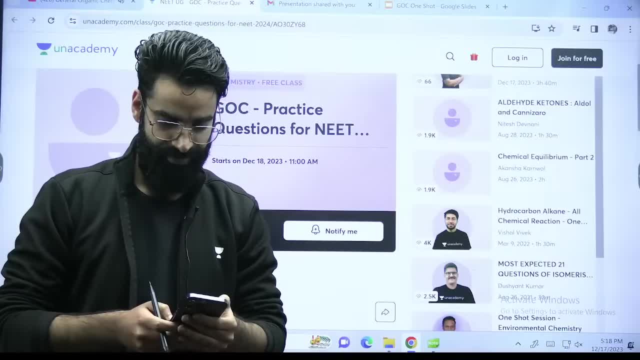 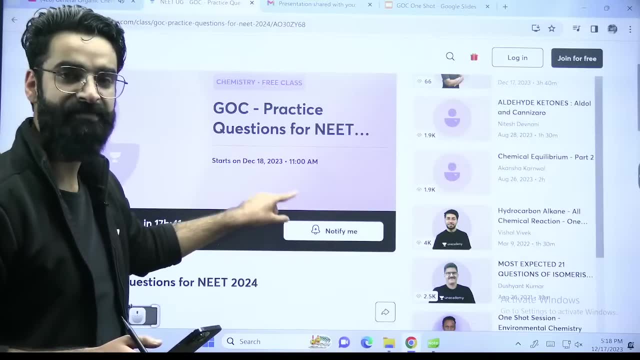 Should we start now? I think a lot of people have gone to attend this particular session. Yeah, My dear students, everyone, I would want everyone to click on this. Notify Me here so that you can remain updated about the extra problem practice session. 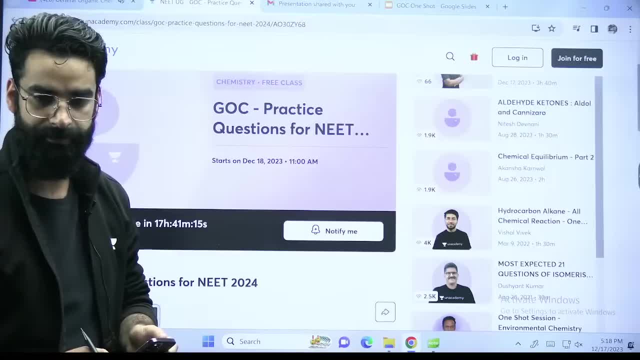 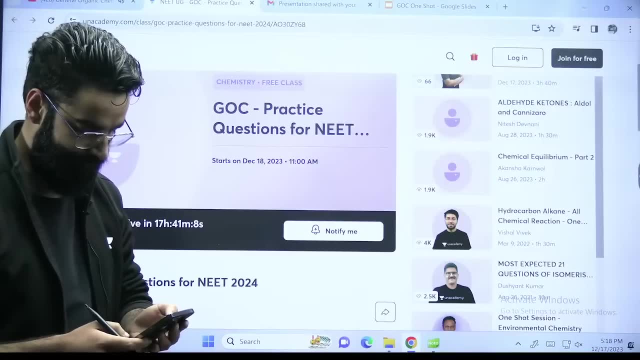 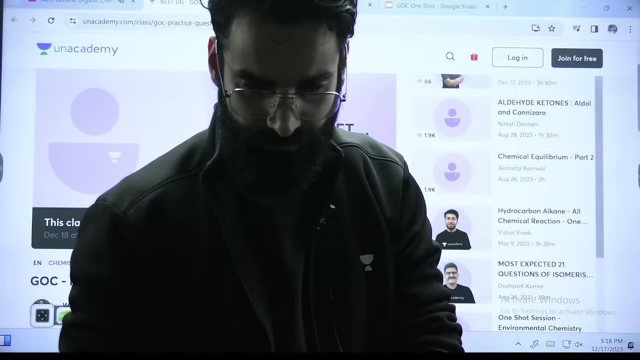 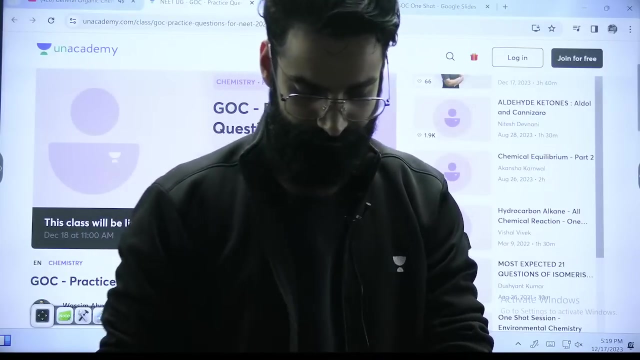 which we are going to do tomorrow at 11 am sharp. Thank you, I think we need to start the session now. Just give me a second. Just give me a second. We are going to start. Just give me a second, people. 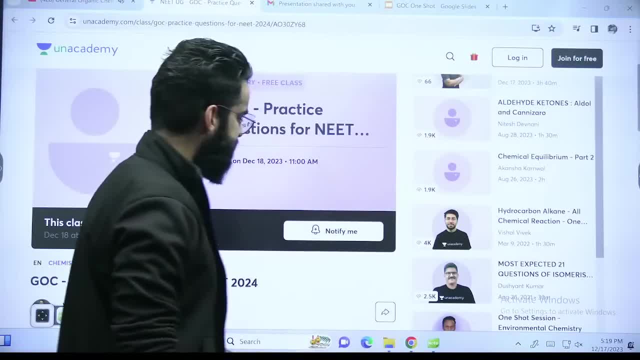 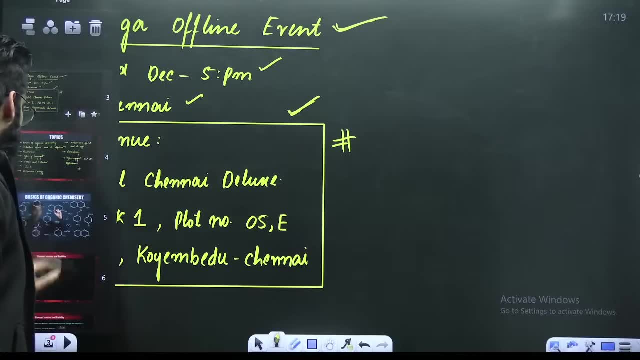 OK, So let's get going. then Let's get started with the chapter General Organic Chemistry. Let me exactly show you the session flow. first of all, Session flow from where exactly we are going to start and where exactly we are going to end the session. 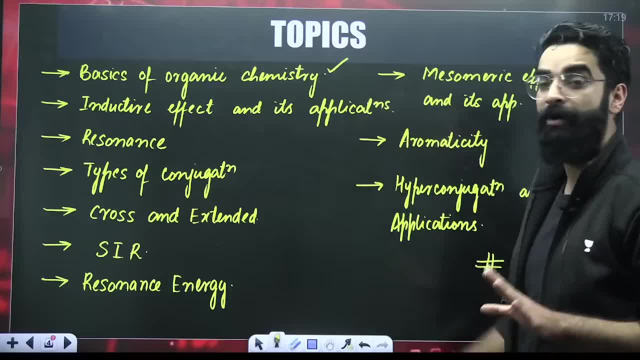 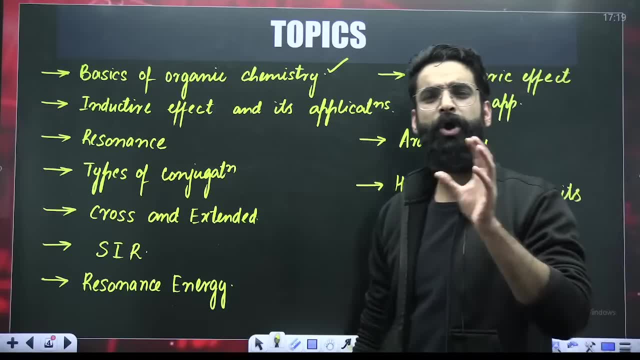 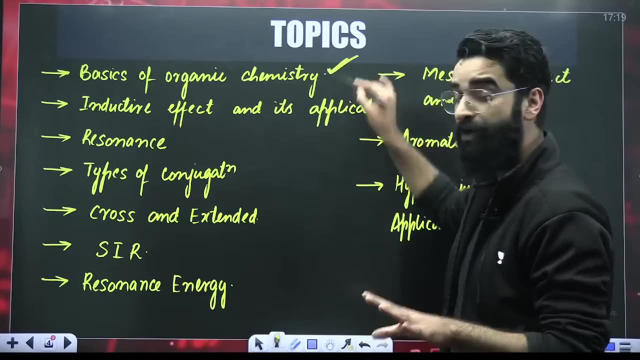 So, my dear students, we are going to start from the basics of the organic chemistry, Since, you know, in your organic chemistry a lot of concepts from chemical bonding are involved, right? So I'll be covering those concepts, perfect, which are from the chapter chemical bonding. 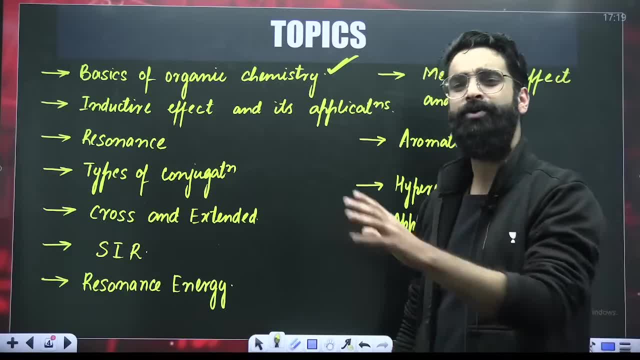 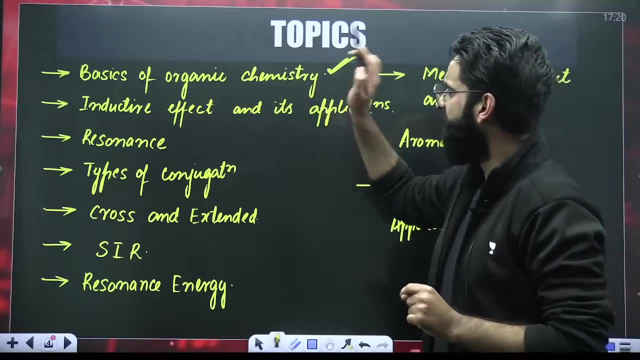 Perfect, I'll be covering those concepts first, so that you'll be fit to attend this particular session, so that you'll be fit to cover the entire organic chemistry with us. Point number one: Right after this, we'll go to inductive effect and its applications. right, 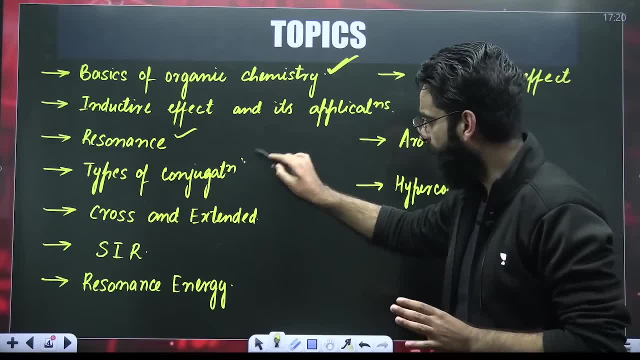 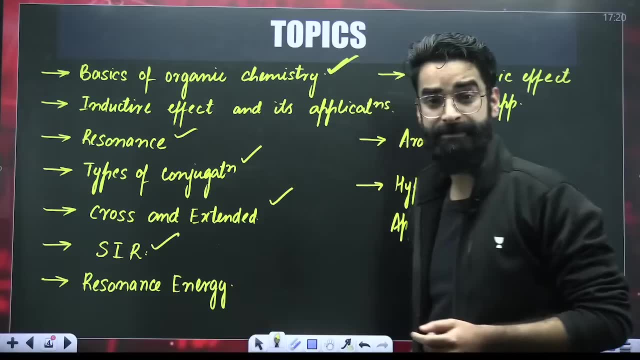 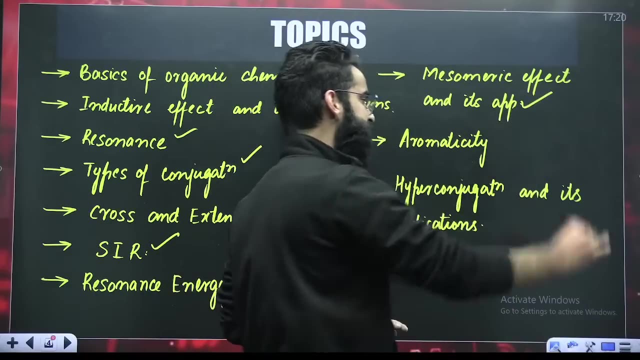 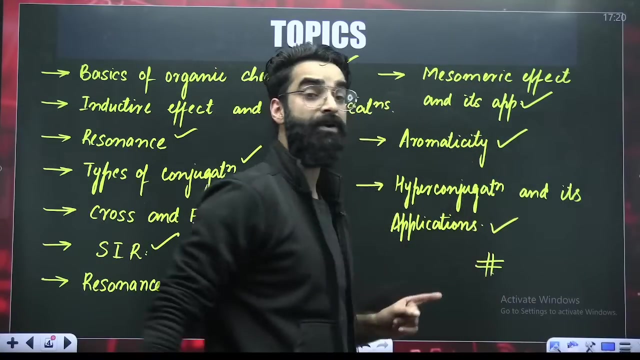 Then we'll be talking about the resonance types of conjugation, cross and extended conjugation, steric inhabitants of resonance, resonance energy- OK- mesomeric effect and its applications. Then we shall be covering the topic aromaticity And at the end of the session we shall be covering the hyper conjugation and its applications as well. 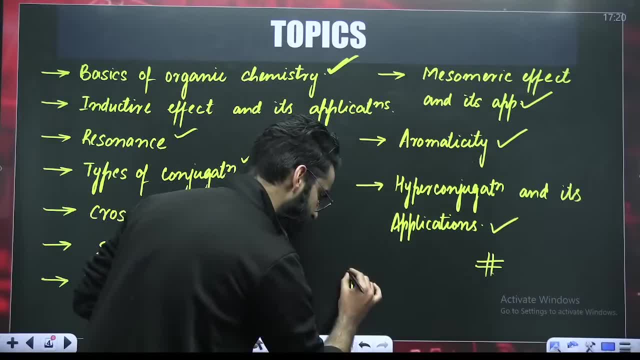 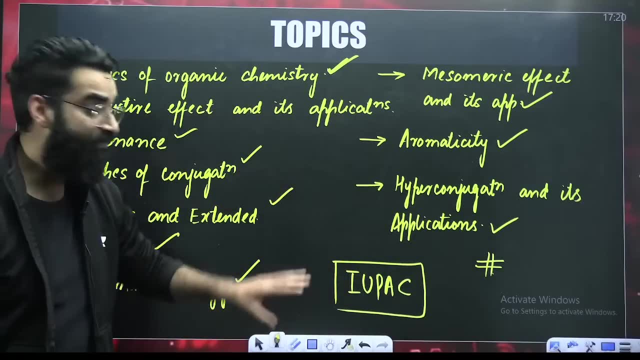 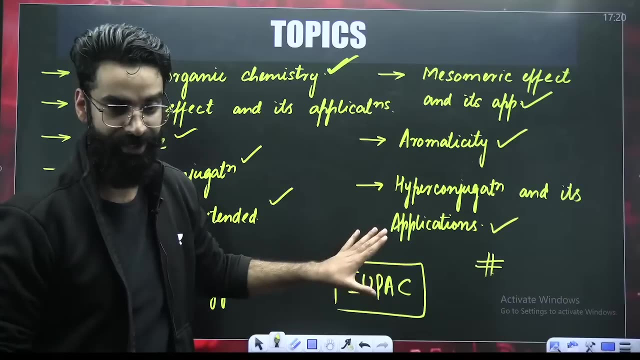 Now a lot of students must be thinking: what about IUPAC nomenclature? What about IUPAC? My dear students, if, if, if, if. if I teach IUPAC also in this particular session, then it's going to exceed 14 hours for sure. 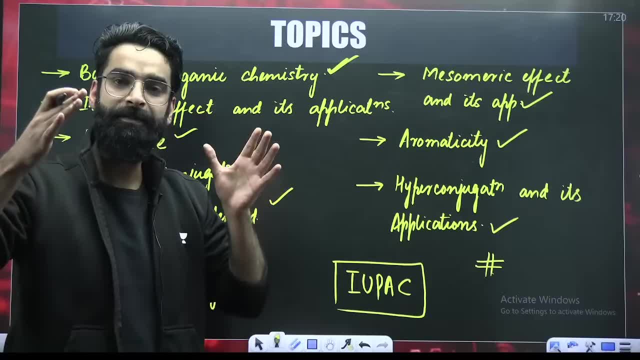 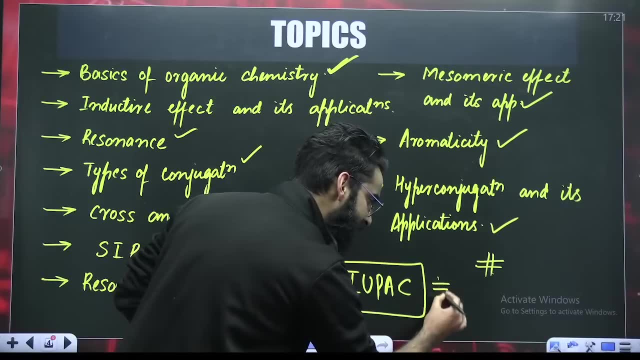 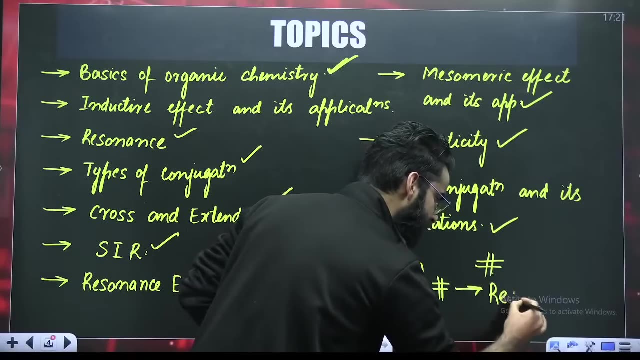 Right, And one YouTube stream, can I mean one YouTube stream can be there for maximum 12 hours, Perfect. So, related to your IUPAC: IUPAC tomorrow in the afternoon. tomorrow in the afternoon, you'll be getting one recording and be providing one recording. 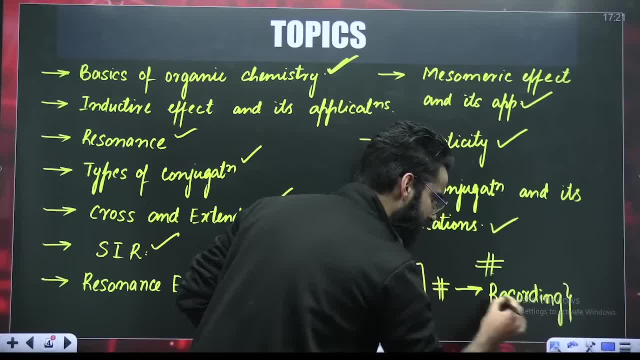 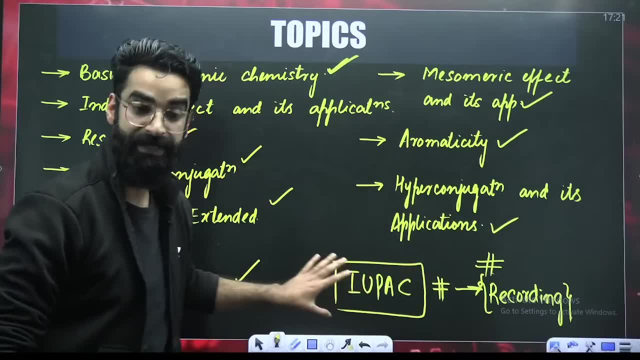 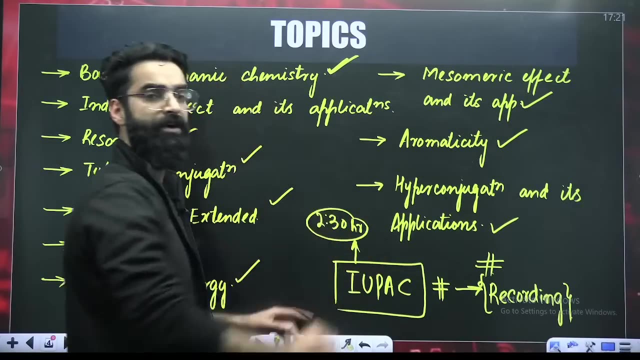 in the afternoon, tomorrow, Right Tomorrow in the afternoon, I'll be providing you one recording in which you shall be covering your complete IUPAC as well, And that recording will be maximum for two and a half hours. That is a two and a half hour recording which you'll be getting tomorrow right on IUPAC. 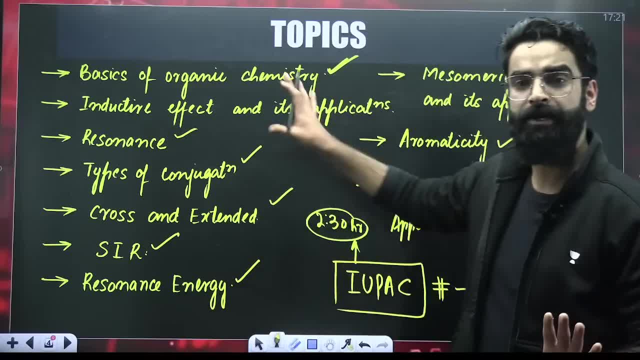 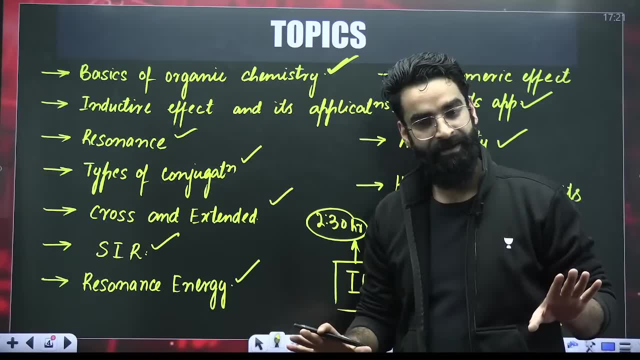 Perfect, All ready Isomerism does not include air. Isomerism needs another 10 to 12 hours. Right, That's again a vast topic. Perfect Isomerism, we'll do. we'll do isomerism as well. but 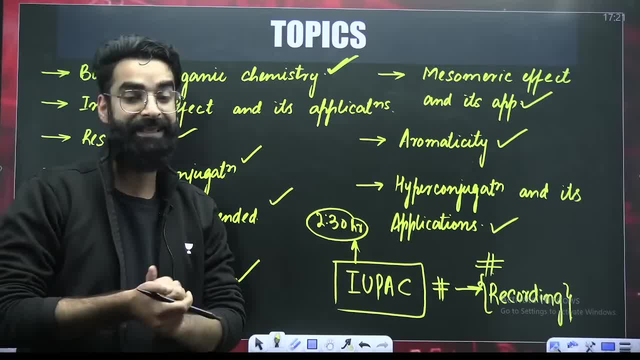 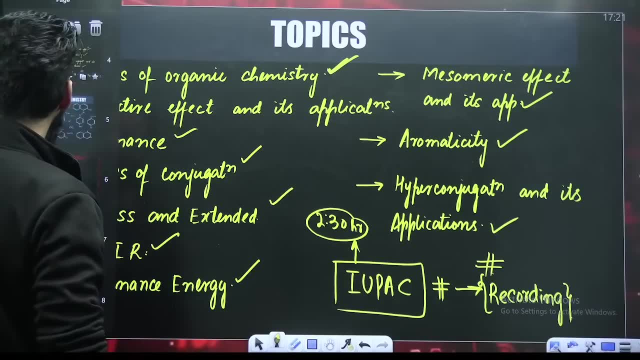 not in this particular session. that also needs some like eight to 10 hours minimum. So let me know once in the chats if you all are ready with your pen and paper. Let me know in the chats quickly if you all are ready with your pen and paper. 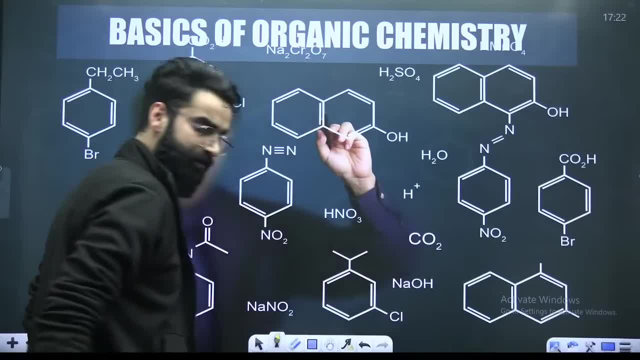 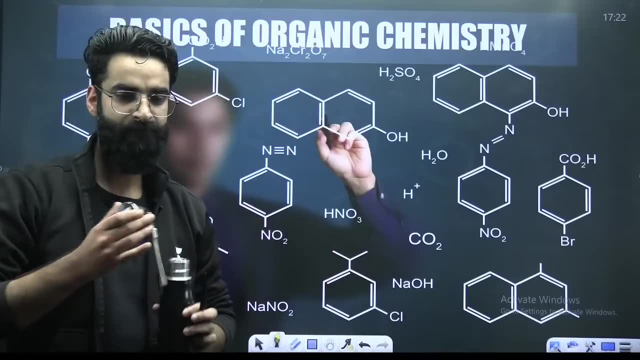 Let me know people quickly If you all are ready with your pen and paper. everyone, everyone, everyone. let me have some water first, because the session is going to be long. Quickly, Guys. everything will be done. Relax. Everything will be done. Yes. 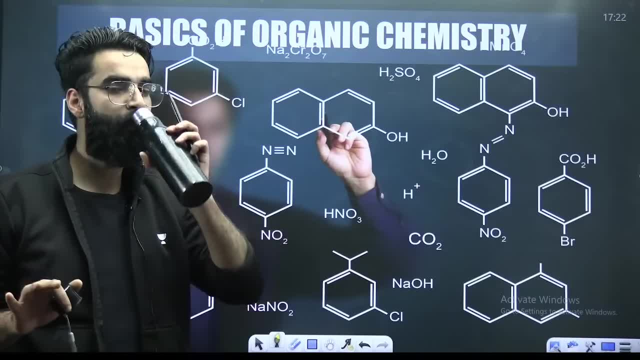 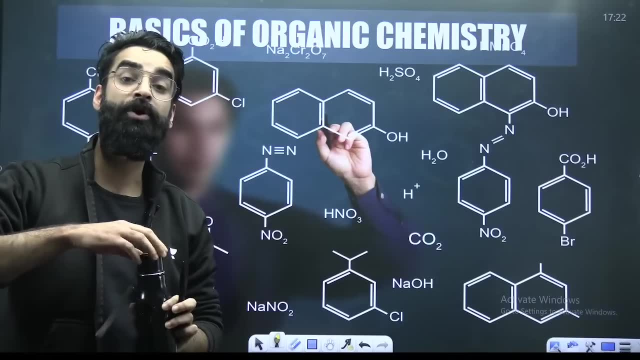 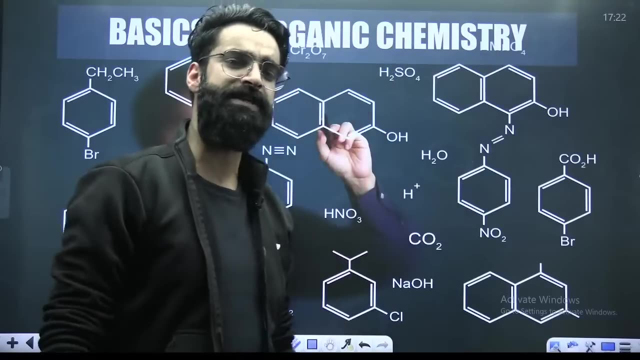 Just remember and follow whatever I'm saying. That's more than sufficient for you After attending today's session and after attending tomorrow's 11 am extra problem practice session as well. Whatever module, whatever book you want to solve on GOC, you can do that. 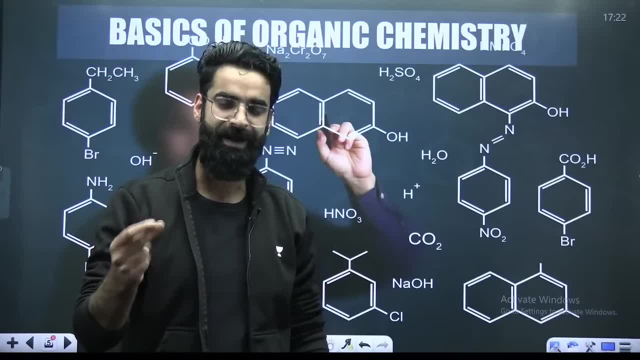 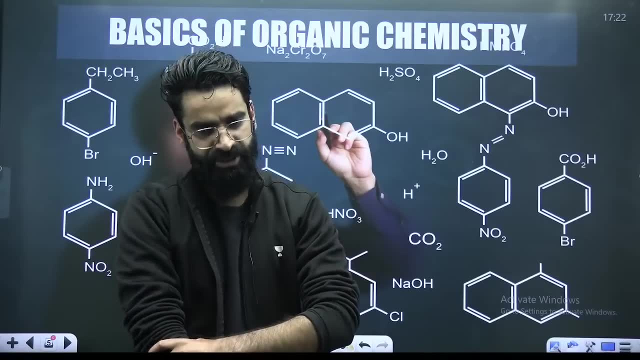 You can do that And you'll be solving those questions like this. I'm telling you that, Yeah, Perfect guys, Purification will be also done. Purification will be also done. I told you already: I'm not going to skip a single thing. 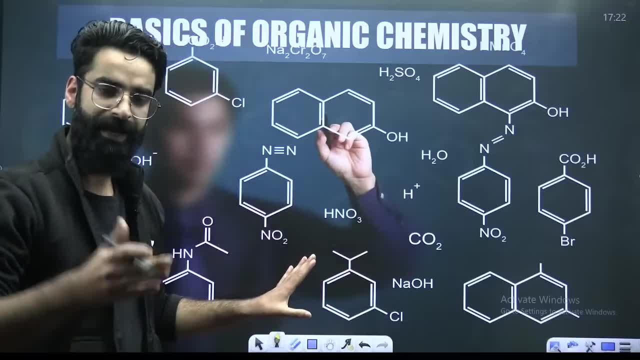 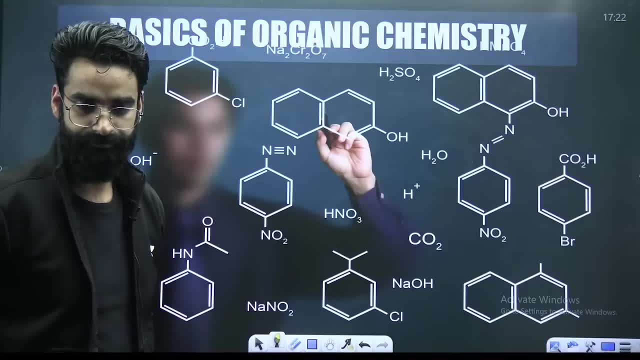 Session duration: I have no idea. OK, I'm starting the session and let's see Till the chapter ends. I'll be here with you, and you are going to be with me too. Perfect guys. So let's get going. then Let's get started. 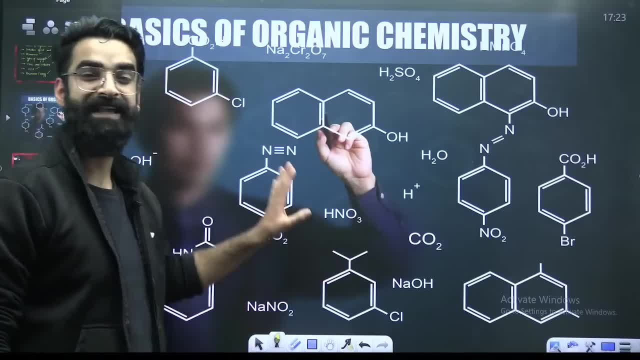 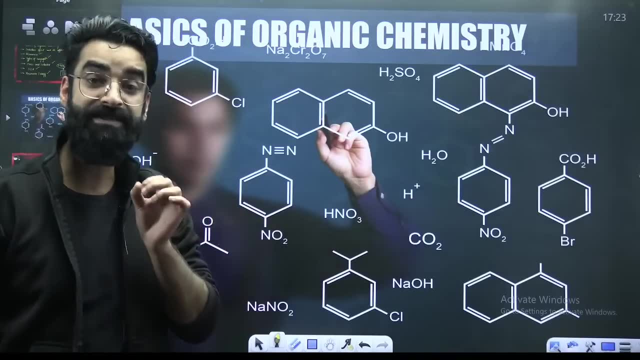 I hope you all are ready with your pen and paper And please, and please, whatever points I'll be noting on the screen, whatever points I'll be writing on the screen, I would want you all to take a note of every single point, because every single 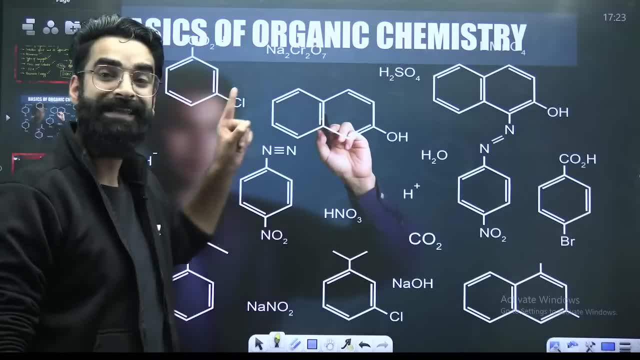 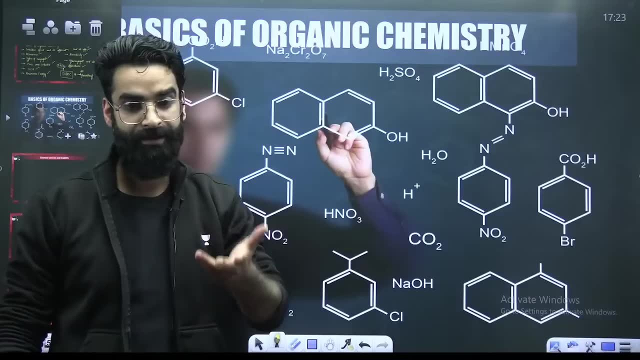 point is going to be equally important by your students, And at the same time, at the end of the session, I'll be providing you the hand written PDF of this particular session, also in my Telegram group. I am pretty much sure you already are there in the Telegram group. 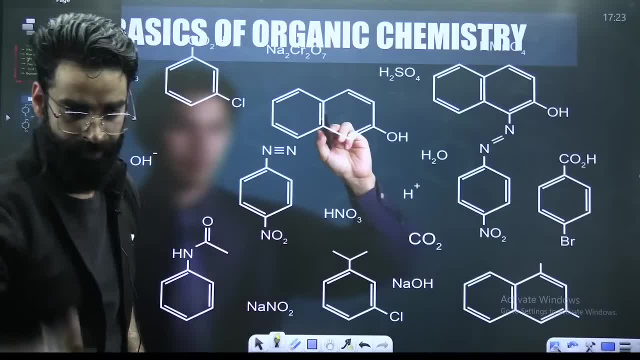 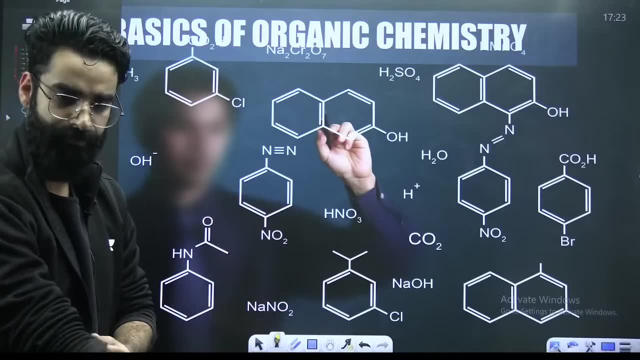 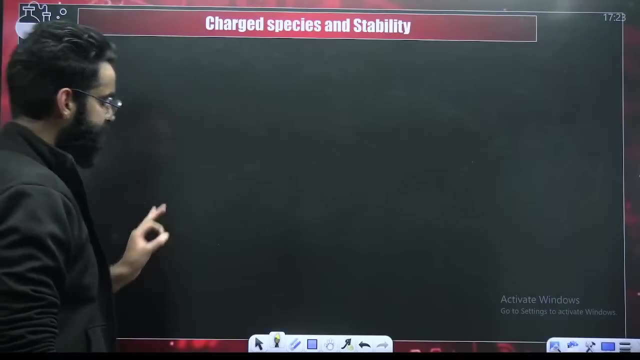 Yeah, If not, then do join it right now. OK, Perfect guys, Perfect. Yes, GE students can also watch this session, No issues, You can watch this session. So, people, let's get going then. So I'm starting this session from a term. 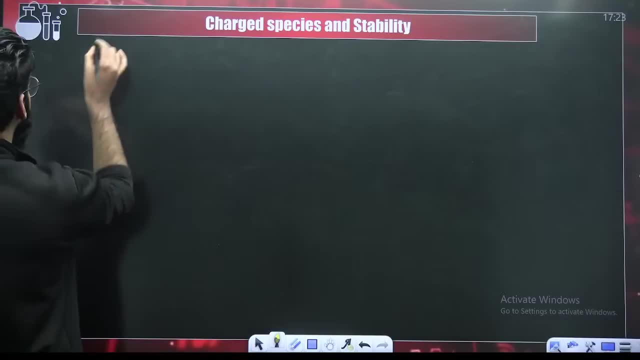 I'm starting this session from a term that is Charged Spatial. This particular session, I'm starting from the term that is Charged Spatial. First of all, if you ask me, what is a Charged Spatial, What is a Charged Spatial? 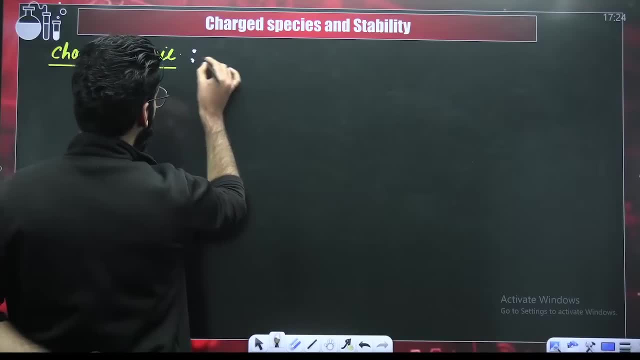 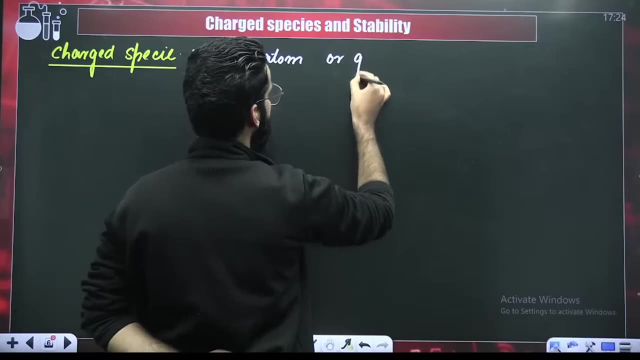 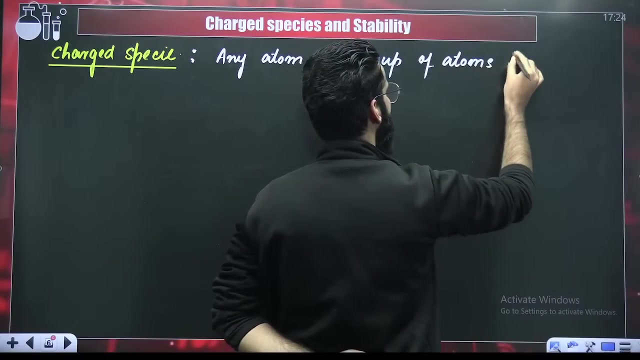 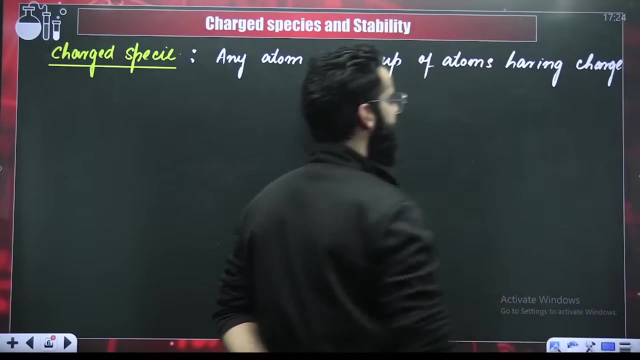 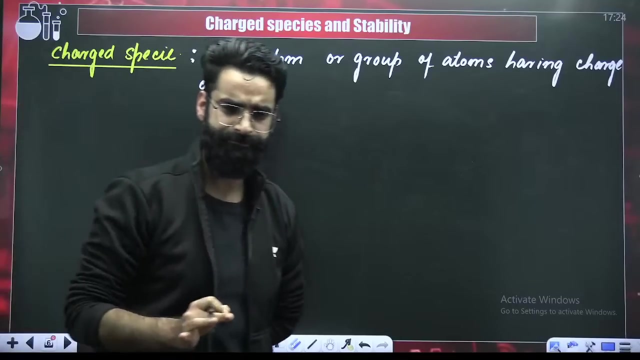 My dear students, any atom, any atom or group of atoms, any atom or group of atoms having charge on it, any atom or group of atoms having charge on it. Having charge on it is something which you call as the Charged Spatial. 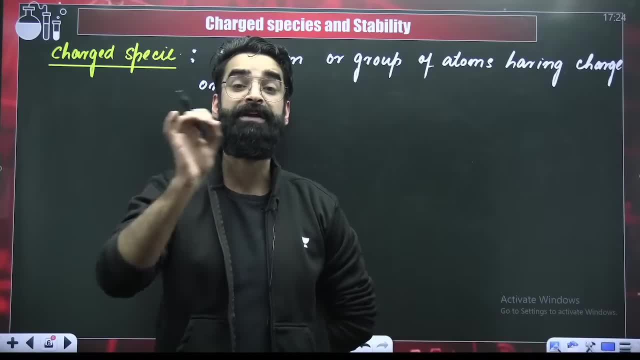 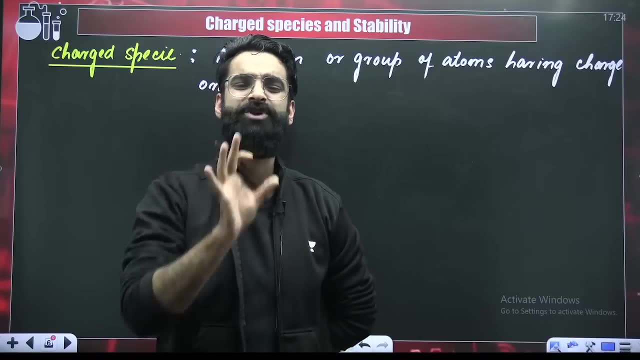 Whenever you see an atom containing any type of charge, be it positive or negative, or whenever you see a group of atoms carrying any sort of charge, be it positive or negative, you'll be calling that as the Charged Spatial Right. So Charged Spatial is nothing. 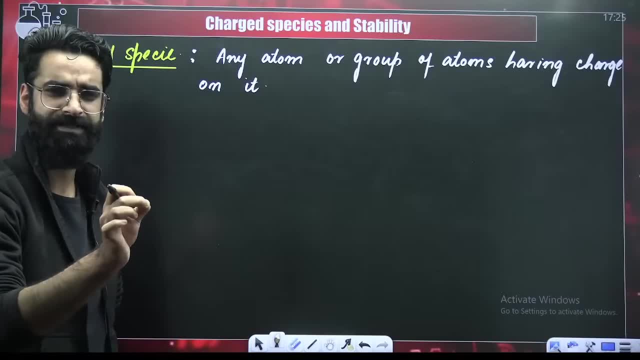 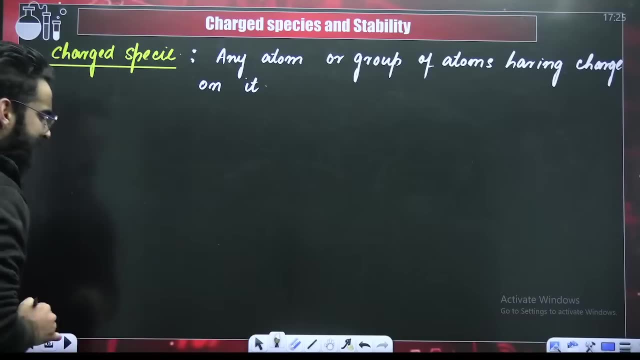 It is the atom or group of atom, atom or group of atoms having any sort of charge on it. It is something which you'll be calling as Charged Spatial. Right Now, my dear students, for the Charged Spatial, for the Charged Spatial. 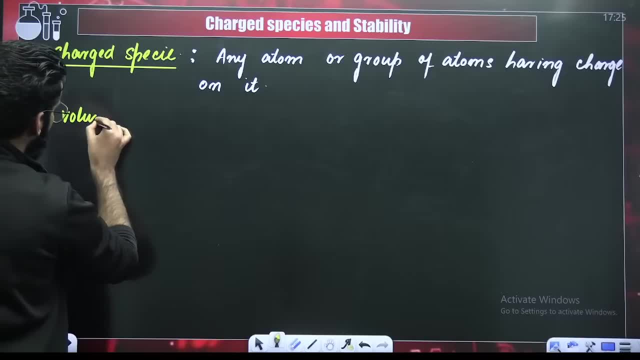 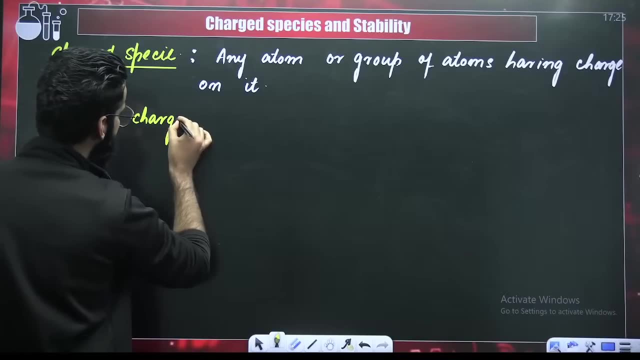 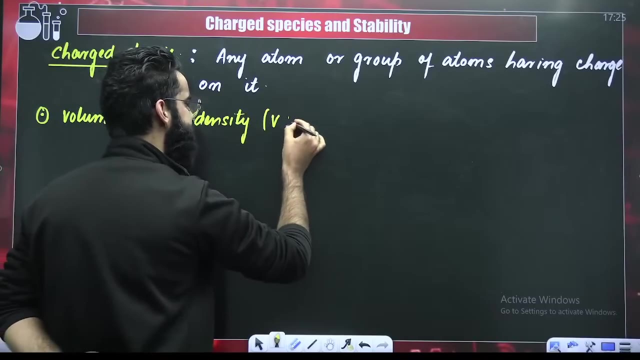 we define a term For the Charged Spatial, we define a term. What is that term? That term is Volume Charge Density. So the term which I'm going to define, Volume Charge Density, VCD. First of all, this particular term. 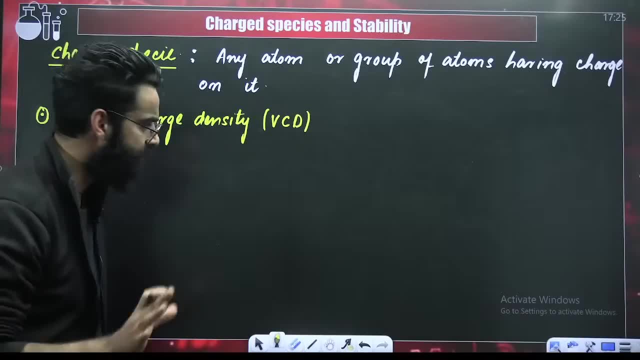 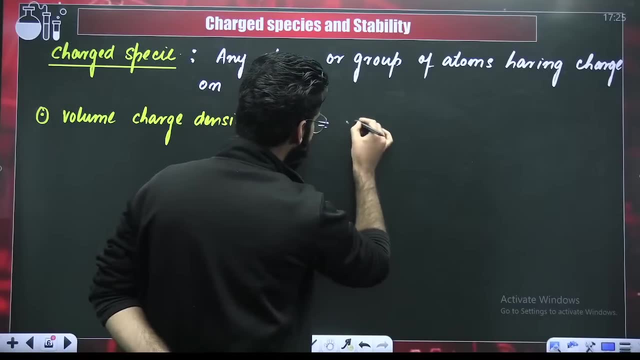 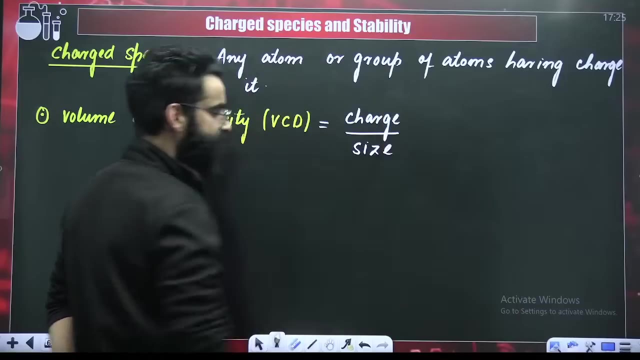 we always define for a Charged Spatial Right. We always define for a Charged Spatial. And how exactly you guys define it: Volume, Charge Density is nothing. It is the ratio of charge present on the Spatial to that of size of the Spatial. 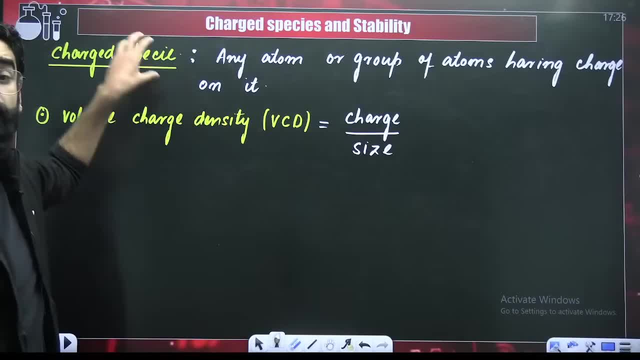 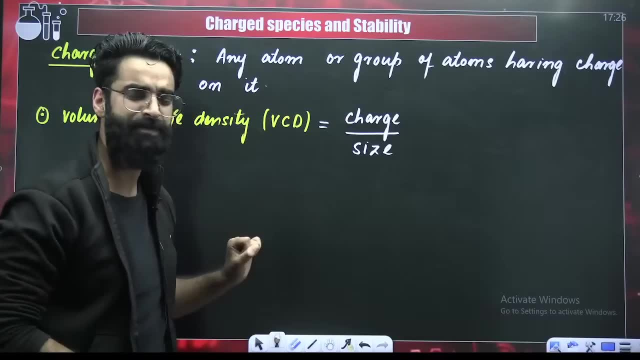 So this particular term, VCD, Volume Charge Density- it is defined only for the Charged Spatial number one And this VCD, it is nothing. It is the ratio of charge present on the Spatial to that of size of the Spatial. 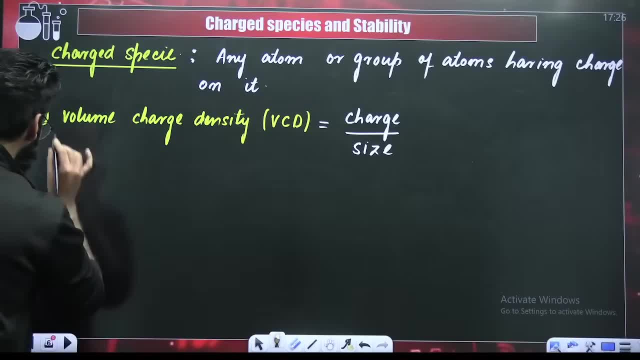 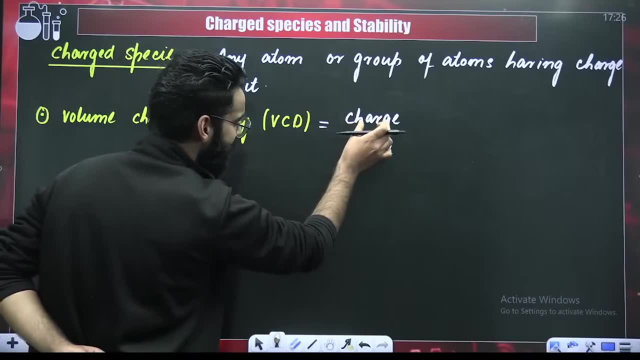 Right people. Now, first of all, try to understand one simple thing, which I'm going to tell you right now: Volume Charge Density. it is directly proportional to charge on Spatial, It is inversely proportional to size of the Spatial. Correct? Now first of all, imagine that. 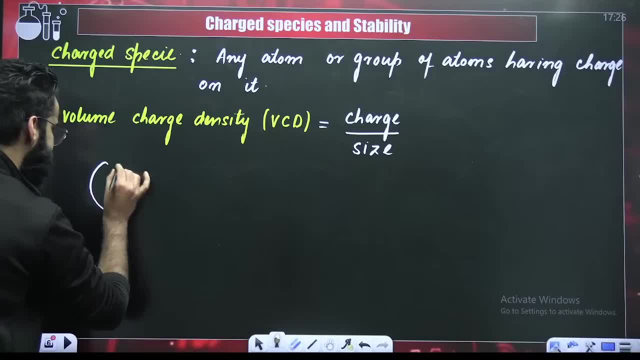 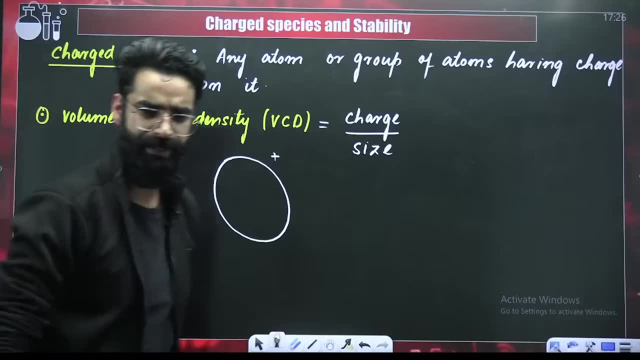 imagine I'm taking two Spatials over here, For example. this is one Spatial carrying positive charge. This is one more Spatial which is bigger in size, containing the same amount of positive charge. So how many Spatials have we taken over here? 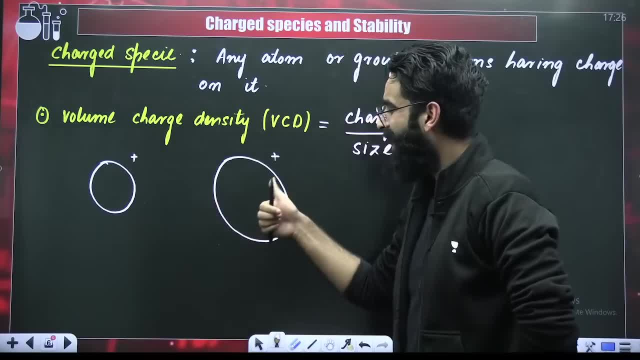 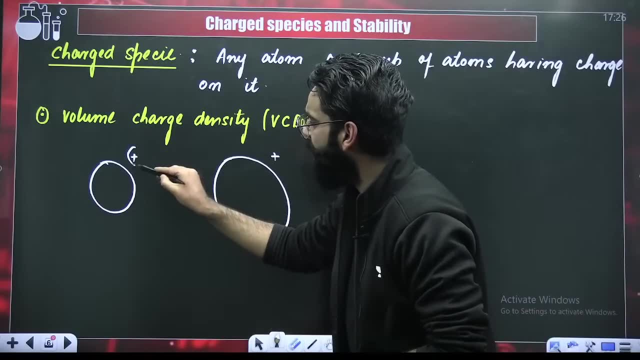 We have taken two Spatials: One Spatial carrying positive, another Spatial carrying equal amount of positive as well. So, first of all, if I'm telling you that the charge present on both the Spatials is same, the magnitude of charge on both the Spatials is same. 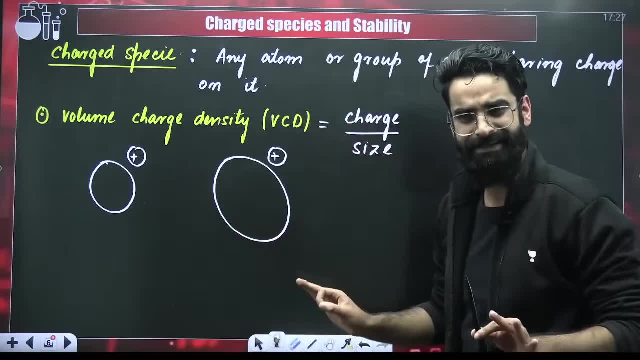 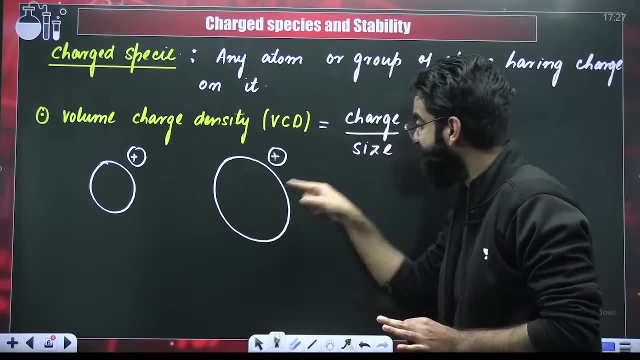 then the difference is like the difference lies in the size. The difference lies in the size This particular Spatial has got more size. if this Spatial has got more size, that means its volume charge density will be less, because VCD is inversely proportional to size. 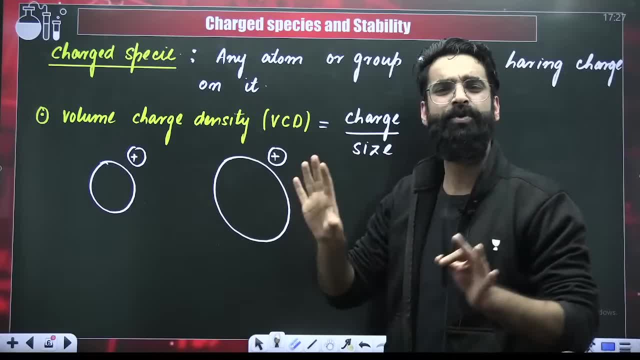 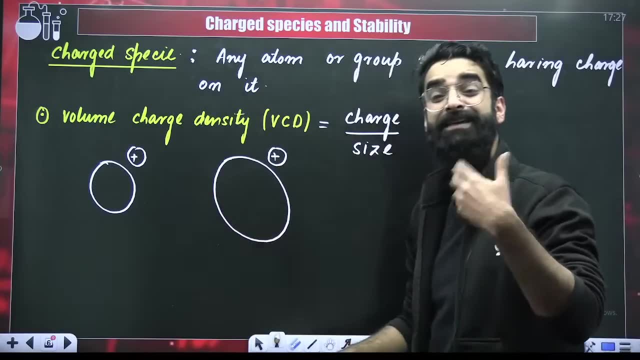 Right. So more the size of the Spatial lesser is going to be the VCD lesser is going to be the volume charge density Right And over here, since these Spatials are carrying the positive charge. so if I ask you, 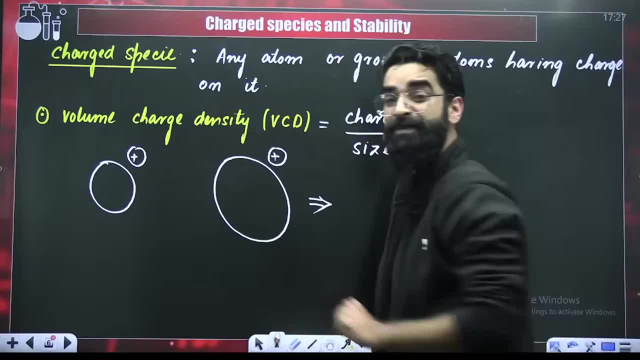 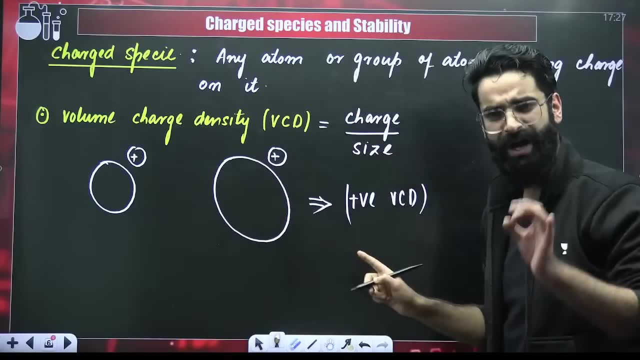 which volume charge density you are defining for these Spatials. you will say it is the positive volume charge density which I'm defining for these two Spatials, Right, So I would say positive volume charge density of this particular Spatial. 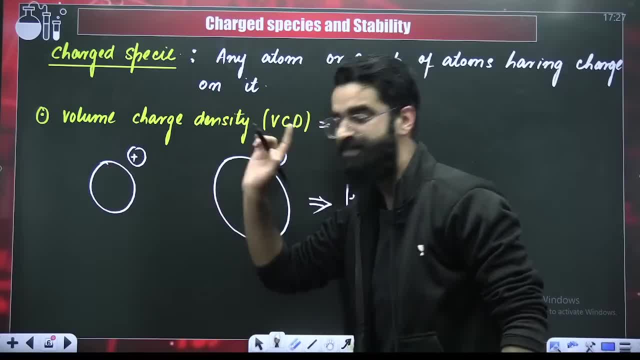 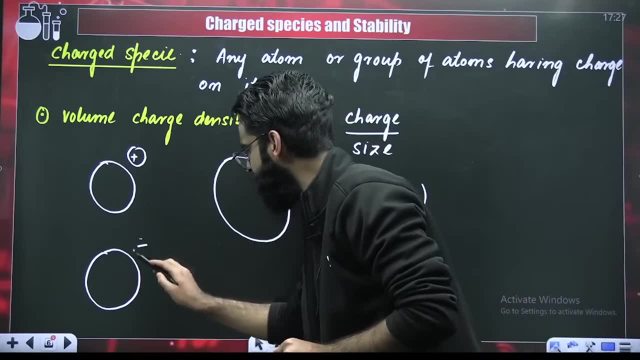 will be less than that of positive volume charge density of this particular Spatial. As simple as that. Similarly, my dear students, let's say: this is one more Spatial which carries the negative charge. Right, I've got one more Spatial which is bigger in size. 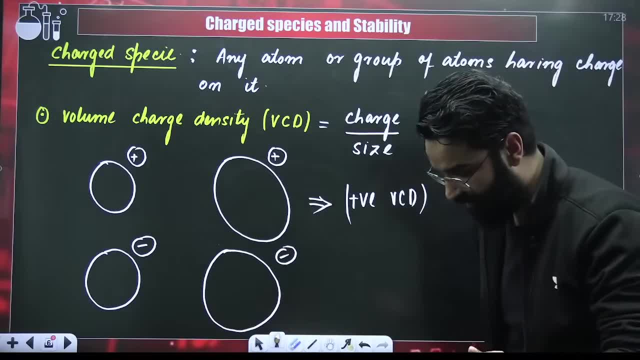 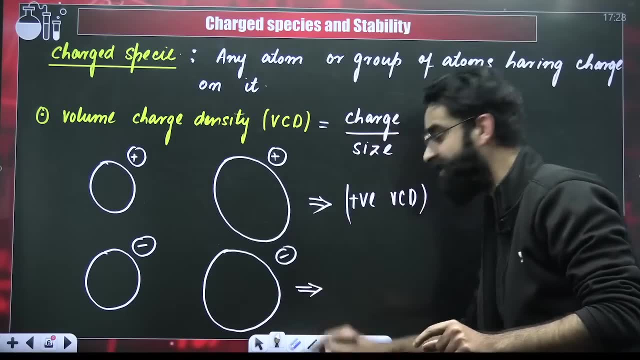 carrying the same amount of negative charge. First of all, if I ask you, if I ask you, if I ask you which volume charge density should I define for these two Spatials, you will exactly say: it is the negative volume charge density. 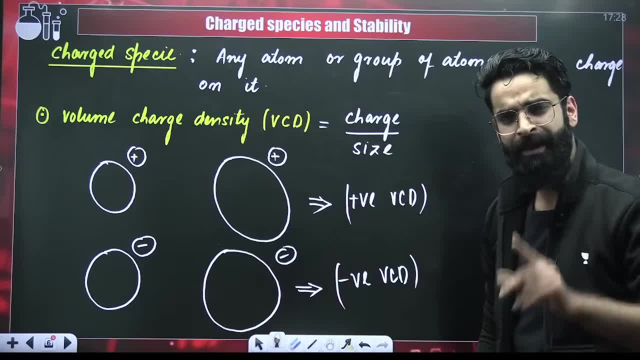 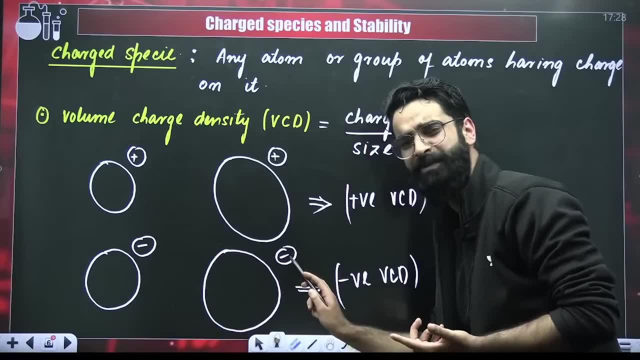 which you are going to define for these two species. As simple as that. Now, my dear students, imagine that the magnitude of charge present here is same as the magnitude of charge present here. Imagine the magnitude of charge on both the species is same. 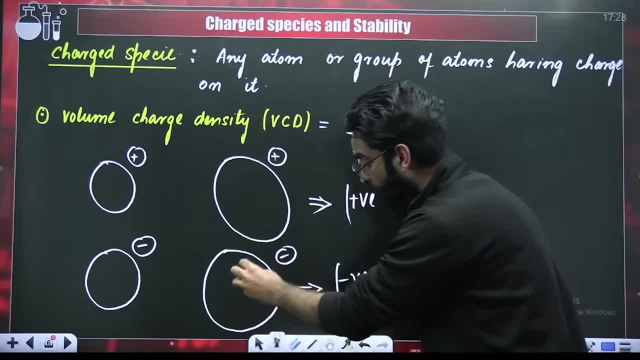 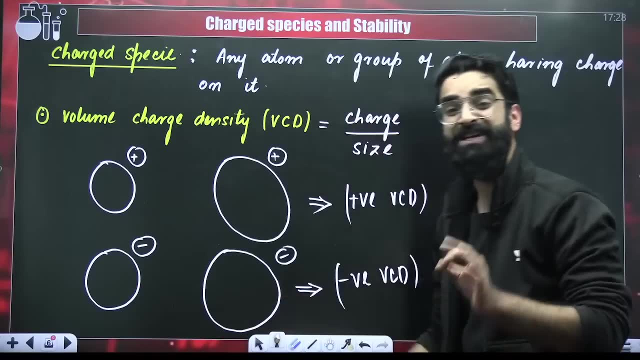 Where is the difference? The difference lies in the size: More the size. more the size, lesser is going to be the volume charge density. So among these two species, which particular species has lesser negative volume charge density? I would say this particular specie. 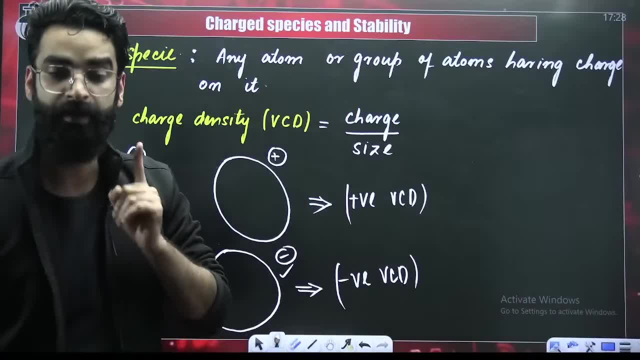 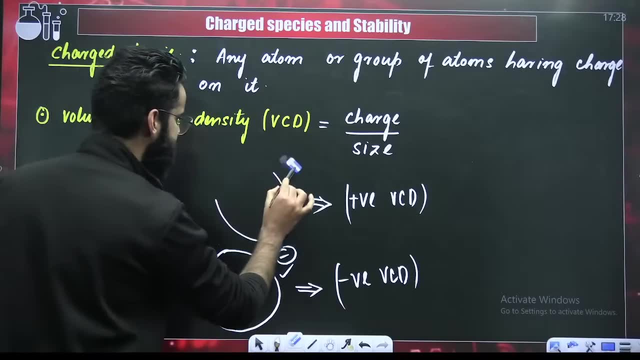 it will be having lesser volume charge density. So point number one. point number one: volume charge density is defined for a charged specie. first of all, For any charged specie, we define the volume charge density, which is the ratio of the charge present on specie. 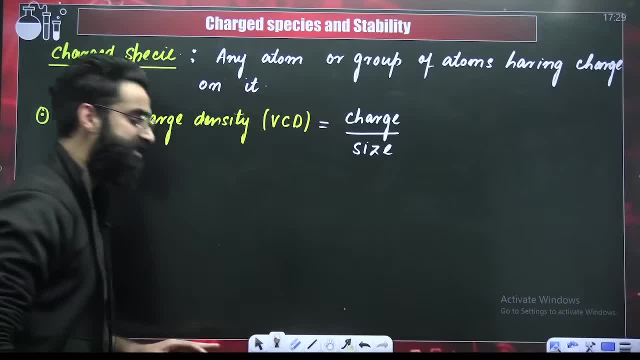 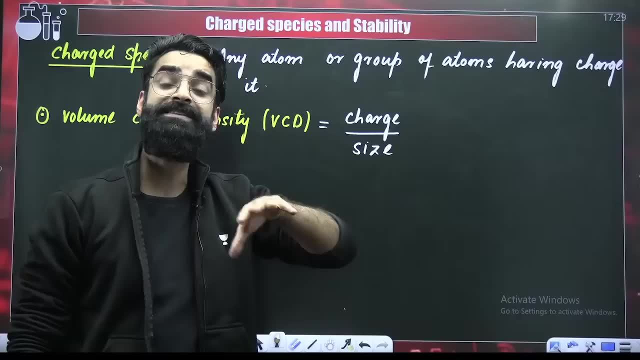 divided by size of the specie. This volume charge density is of how many types? It's of two types: positive volume charge density. negative volume charge density. Positive volume charge density is defined for those species which carry positive charge. Negative volume charge density is defined for those species. 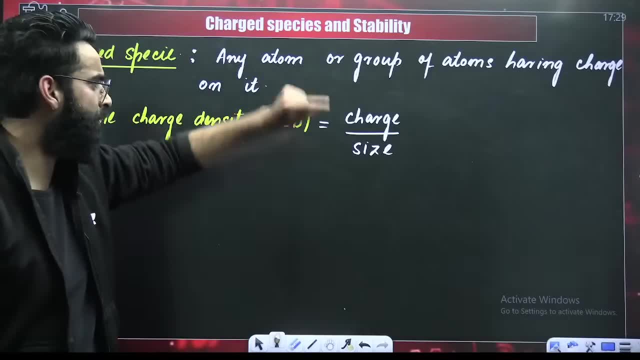 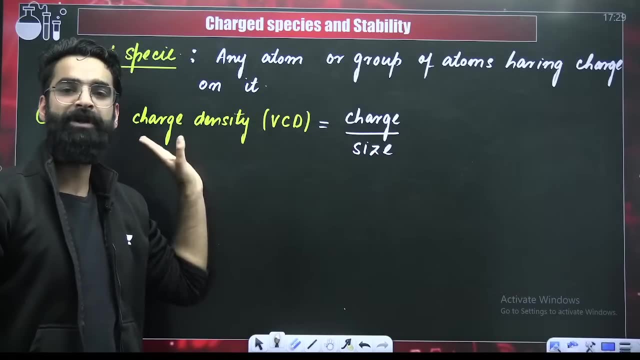 which carry the negative charge Right. And remember, from now onwards, more the charge on the specie, more the volume charge density Right. Lesser the size of the specie, more the volume charge density, be it positive or negative. I hope this is clear to everyone. 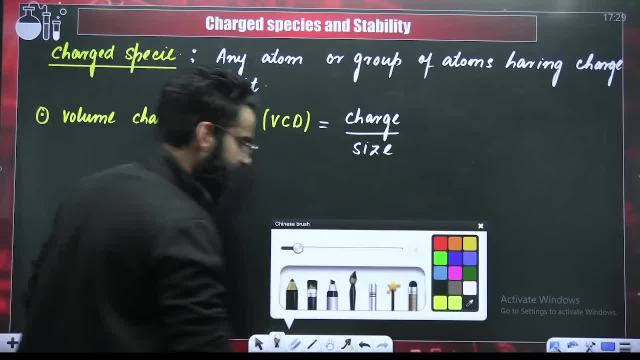 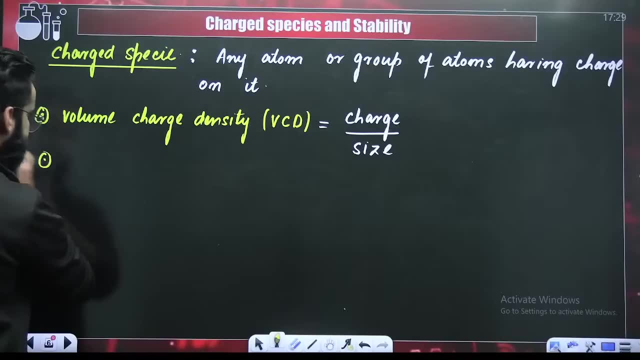 Now, people, why am I giving you this term, this volume charge density? Because, because, because this volume charge density is related to stability. This volume charge density, it is related to stability. Let me tell you, please, and please, take a note of every single thing. 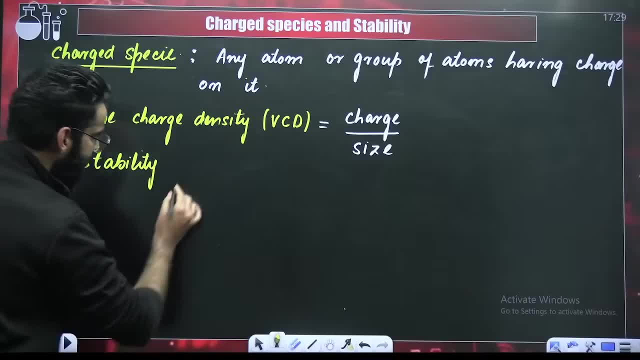 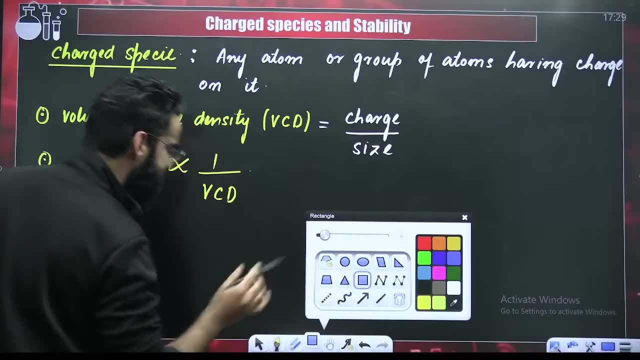 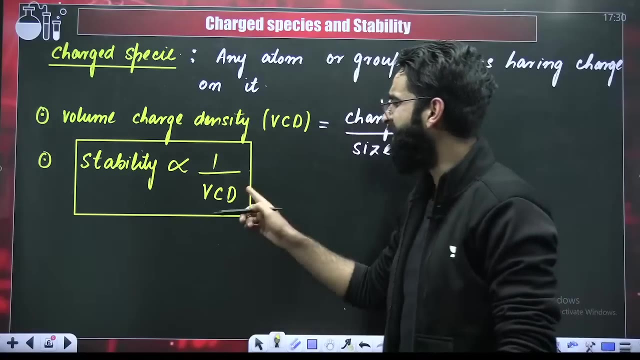 Let me tell you stability. stability is inversely proportional to volume charge density. Stability is inversely proportional to volume charge density. What is meant by this particular point? How can we get different types of questions from this particular point? That is something which you will get to know in some time. 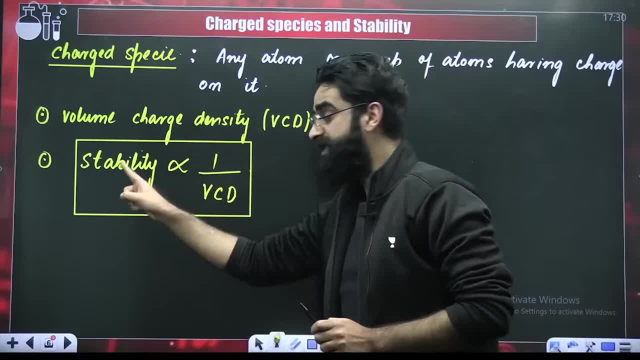 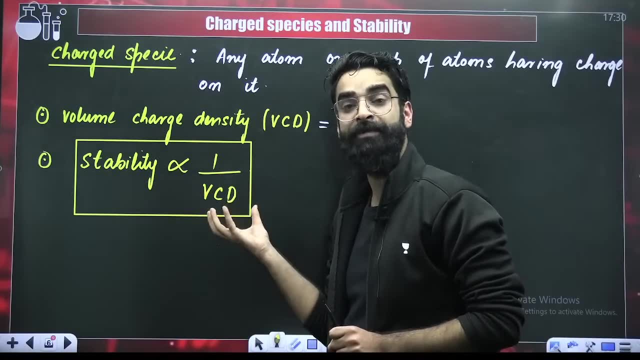 First of all, remember it directly: from now onwards, Stability of the charged specie is inversely proportional to VCD. More the VCD, more the volume charge density lesser is going to be the stability Lesser the volume charge density more is going to be the. 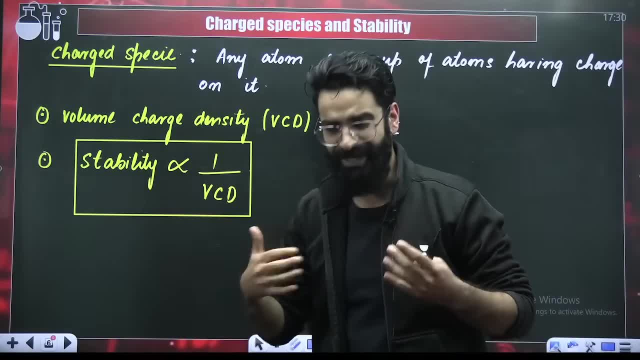 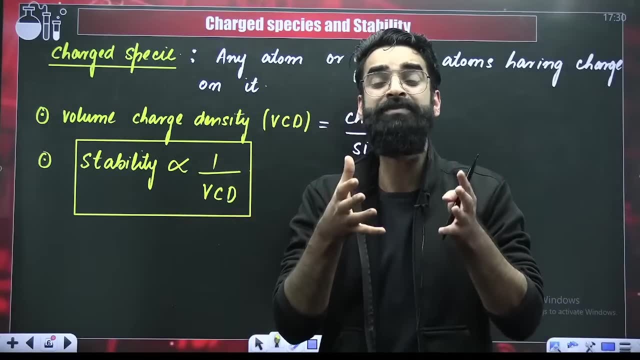 more is going to be the stability Right. Perfect, Basically. what is the logic for it? Why they are inversely related, My dear students, it's pretty much simple: If charge density, if volume charge density on the specie is more, 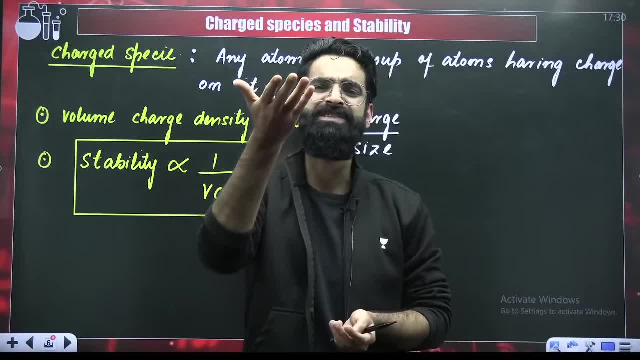 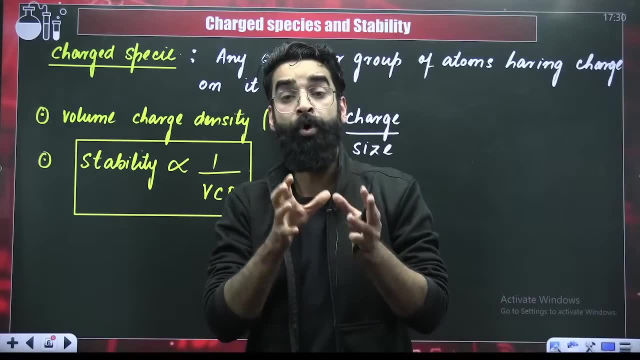 that means its potential energy is more, And if potential energy is more, stability automatically will be less. Right, As simple as that. More positive, more, more volume charge density means more potential energy, and more potential energy means less stability. That's it. 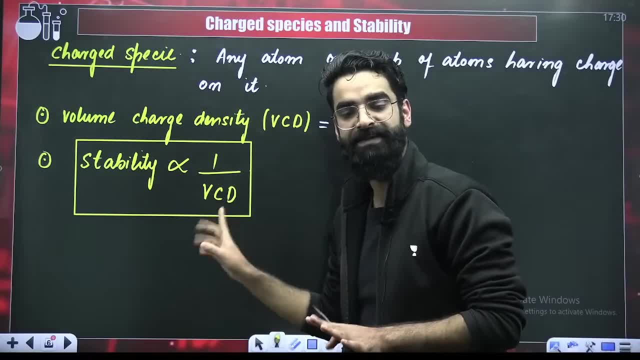 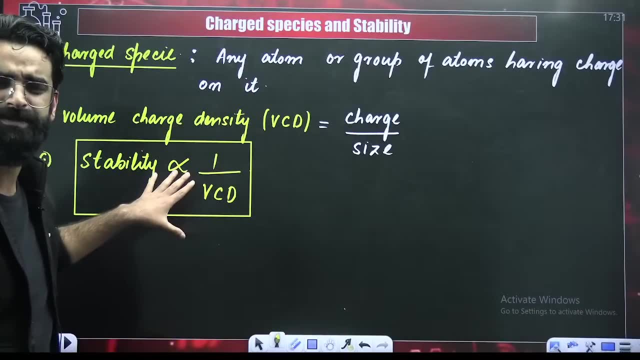 So just remember this particular statement: from now onwards, Stability is inversely proportional to volume charge density. Now, where do I utilize these terms? Where do I utilize these terms? Before utilizing these terms, before showing you the application of these terms over here? 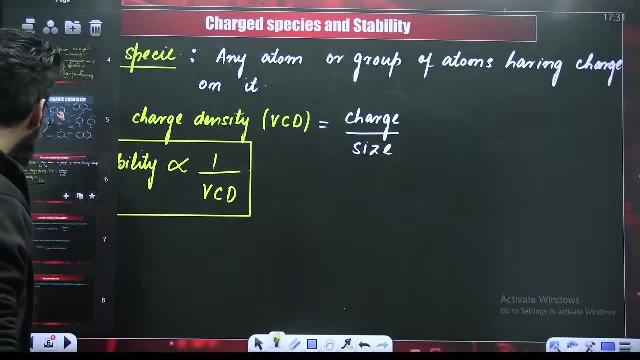 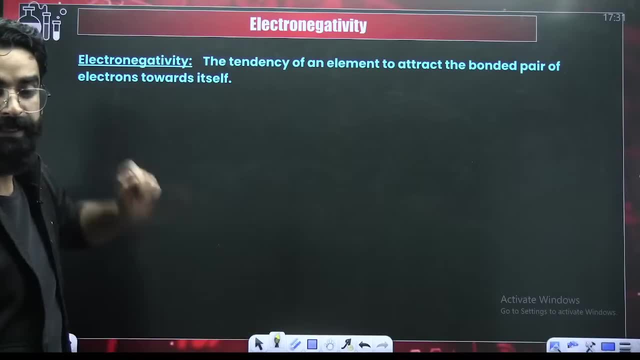 there are few more things which you need to know. first of all, Right, And what are those things? Have a look. I believe every one of you would have come across the term electronegativity. Right, I believe every one of you would have come across the term electronegativity. 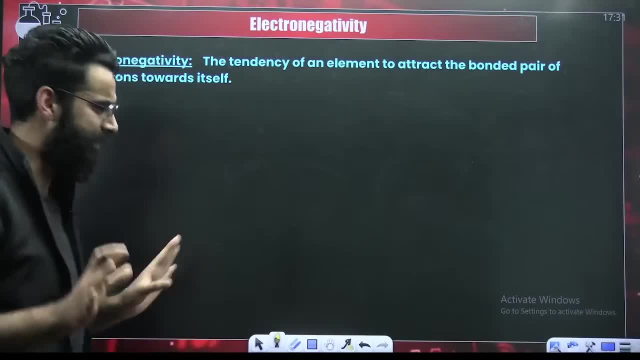 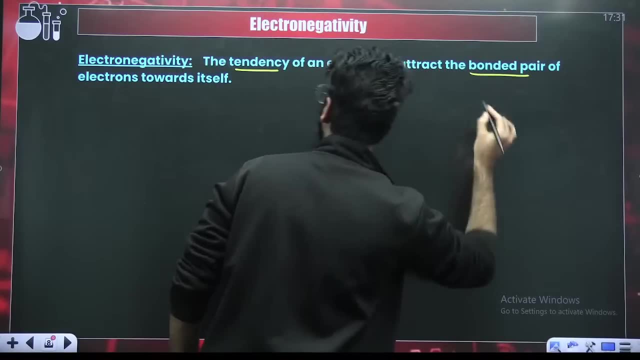 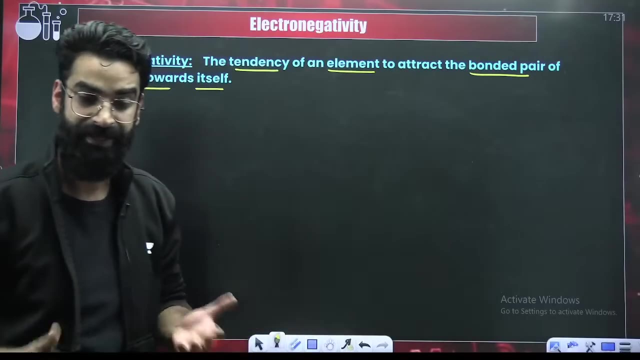 How do you exactly define the term electronegativity? My dear students, look at the definition: The tendency of an element. the tendency of an element to attract the bonded pair of electron towards itself. The tendency of an element to attract the bonded pair of electron towards itself. 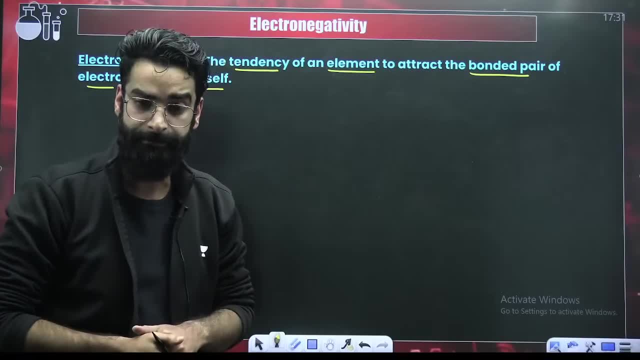 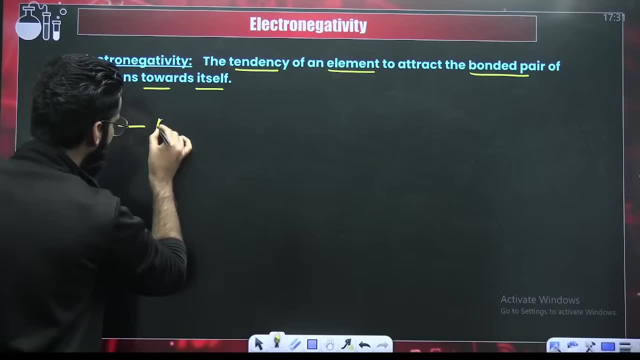 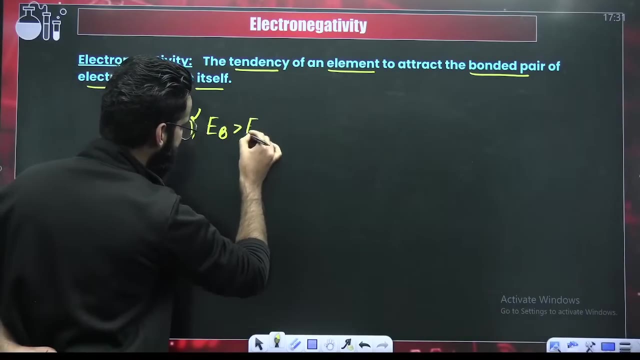 That defines what. That defines: electronegativity of an element, For example. for example- my dear students, have a look. Let's say, let's say there is a covalent bond between A and B. Perfect, I'm assuming that the electronegativity of B is greater than that of electronegativity of A. 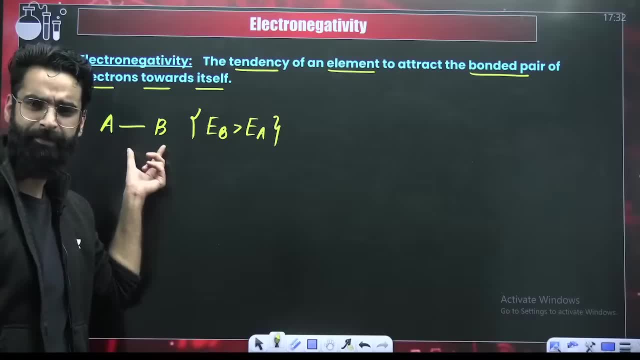 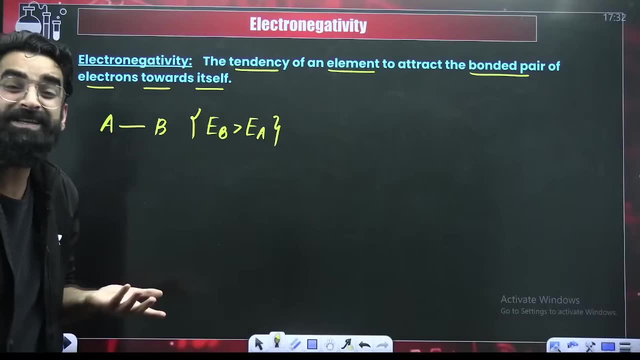 This is something which I'm assuming. Let's say, there is a covalent bond between A and B, And I'm assuming electronegativity of B is more than that of A. Now, what does this term mean? What does it mean that electronegativity of B is more? 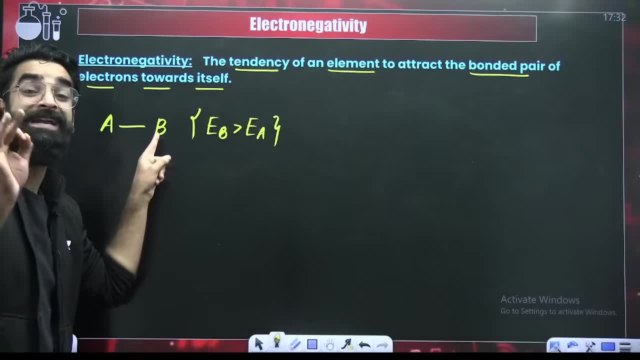 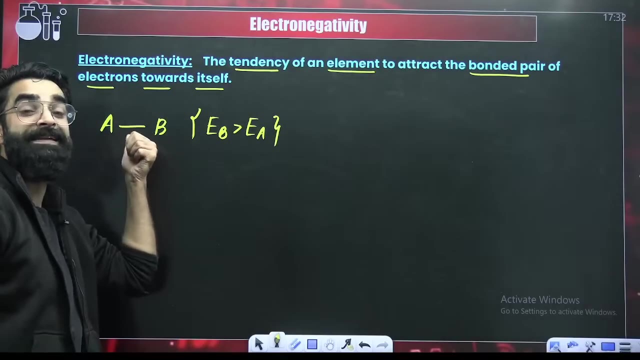 It simply tells you that B has got more tendency. B has got more tendency to attract this bonded pair of electron towards itself. Right Now you tell me if B has got more tendency to attract the bonded pair towards itself, will the electron density towards B increase or decrease? 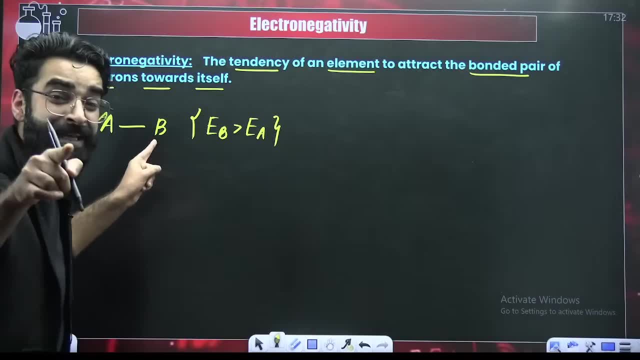 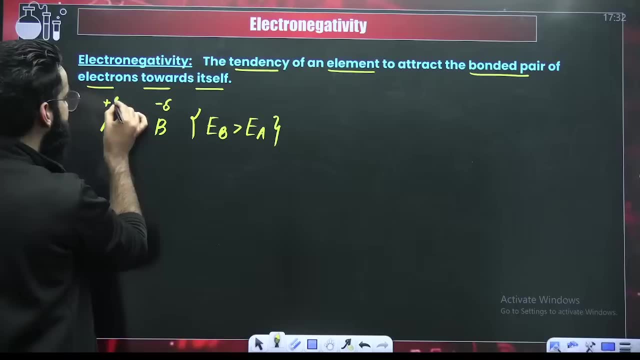 Electron density towards B will increase, And that increase in the electron density towards B is represented by delta negative. And here you'll be writing: delta positive. as simple as that, Right. As simple as that. Perfect, My dear students. one more thing. 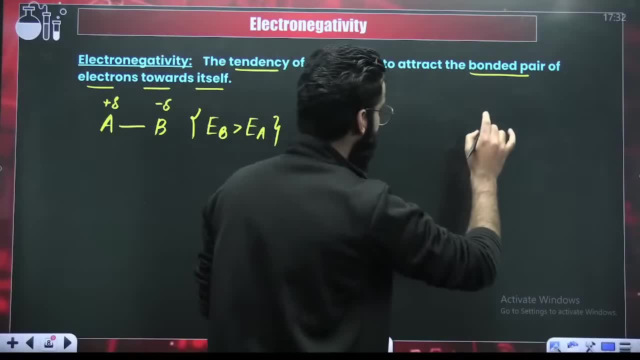 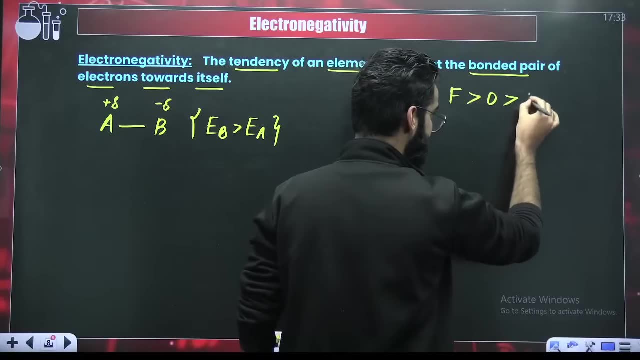 Just tell me one thing. Just tell me one thing: In your periodic table, which element is considered to be maximum electronegative? It is fluorine, Remember this, Followed by oxygen, Followed by nitrogen. I believe all of you would be knowing this particular thing. 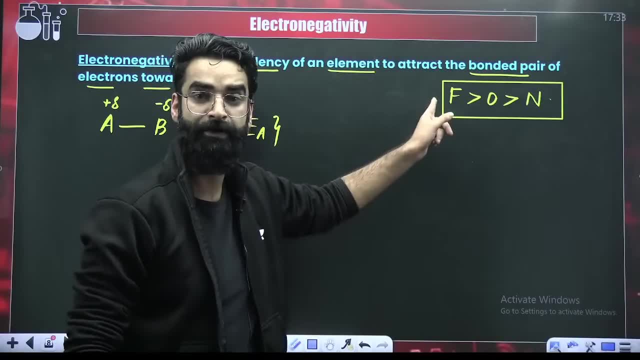 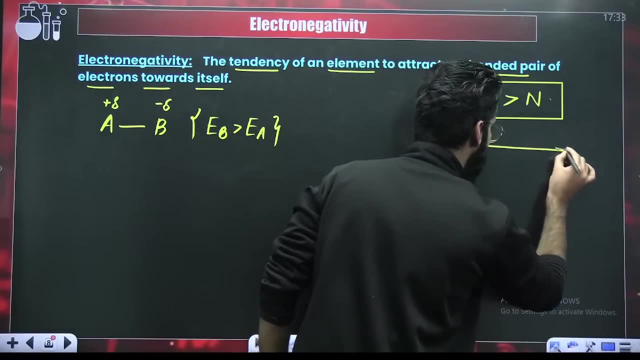 Right In your periodic table, fluorine is the most electronegative element, followed by oxygen, followed by nitrogen. Point number one, Point number two In your periodic table, if you move from left to right, if you move from left to right, 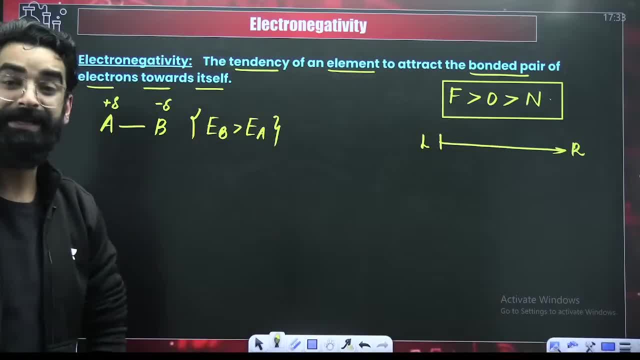 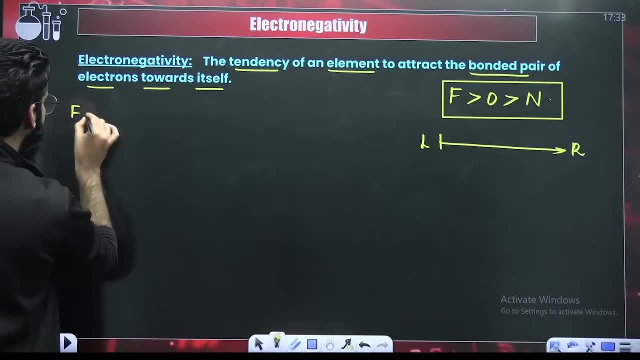 left to right. what happens to electronegativity generally? If you ask me, I'll tell you one simple thing. I'll tell you: electronegativity, electronegativity, electronegativity, it's inversely proportional to size. 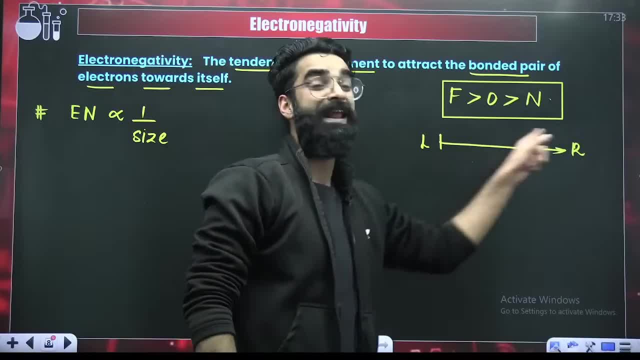 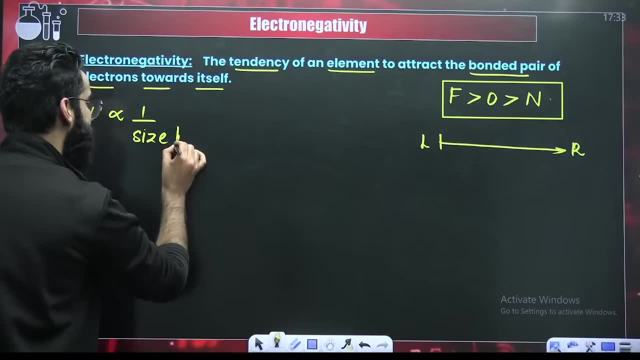 Electronegativity. it's inversely proportional to size. Now, as you move from left to right, as you move from left to right, generally size decreases, Generally size decreases. If size decreases, that means electronegativity will automatically increase. 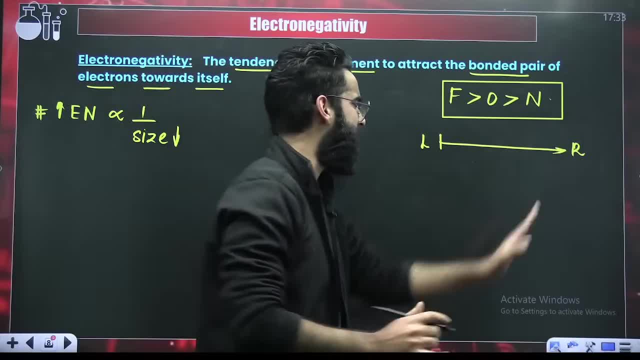 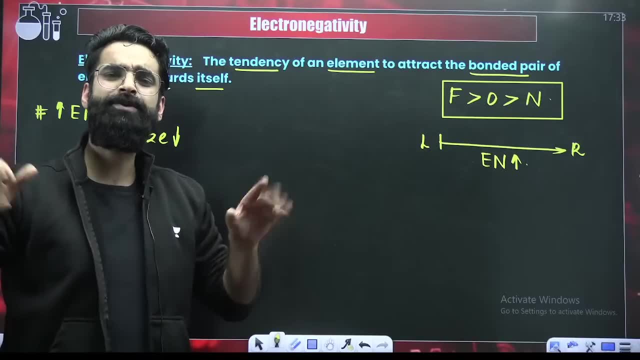 So remember one simple thing: from now onwards, When you move from left to right, electronegativity it increases. It increases generally, Right. Similarly, my dear students, you tell me, you tell me when you move from top to the bottom, 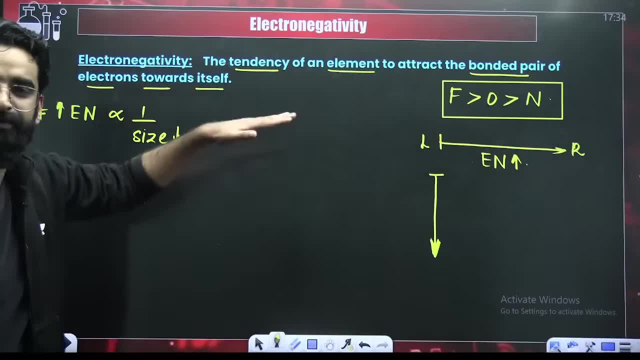 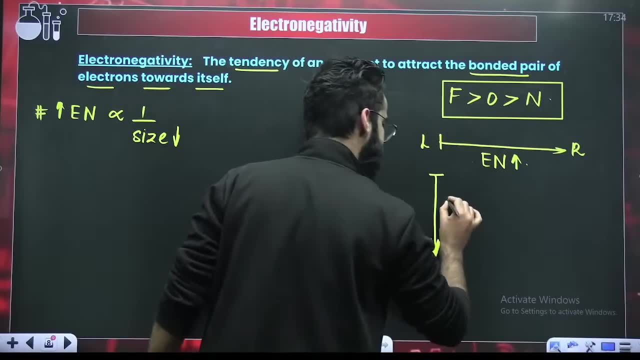 when you move from top to the bottom in the periodic table, when you move from top to the bottom in the periodic table, what happens to size? Size increases generally. If size increases. if size increases, electronegativity decreases. Electronegativity decreases. 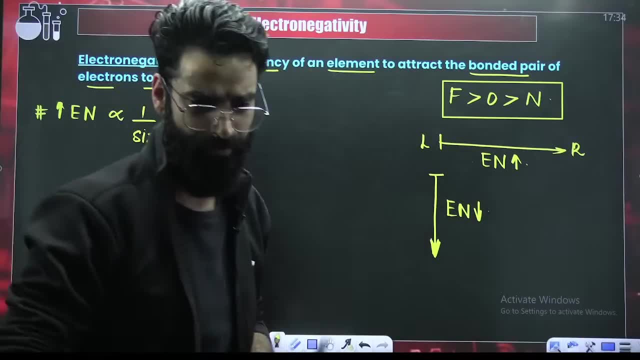 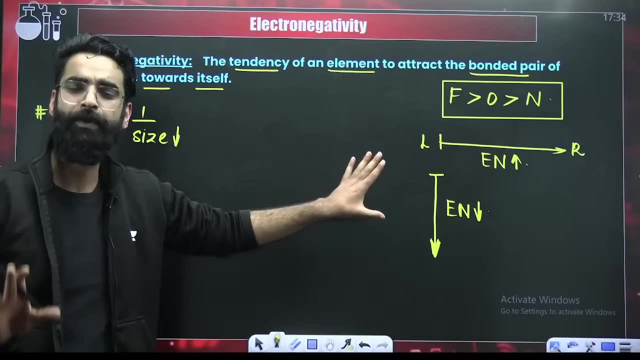 Perfect. This is one simple thing which I want all of you to remember from now on: Right, Right, people, Perfect. One basic thing which I told you, Which I would want all of you to remember from now onwards: Right And my dear students, 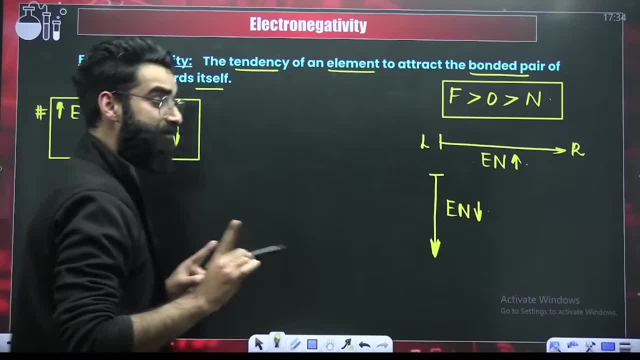 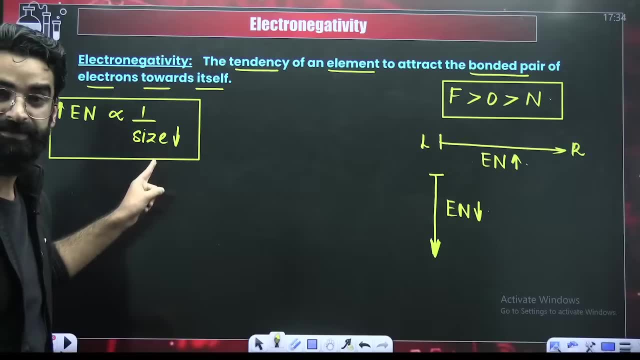 remember this particular statement as well. Electronegativity: it's inversely proportional to size, Because I'll be using this particular statement many a times. I'll be using this particular statement many a times. Now, people, there are few more things which we can conclude from the term electronegativity. 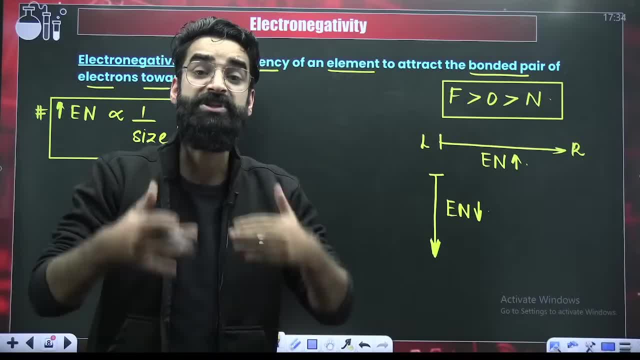 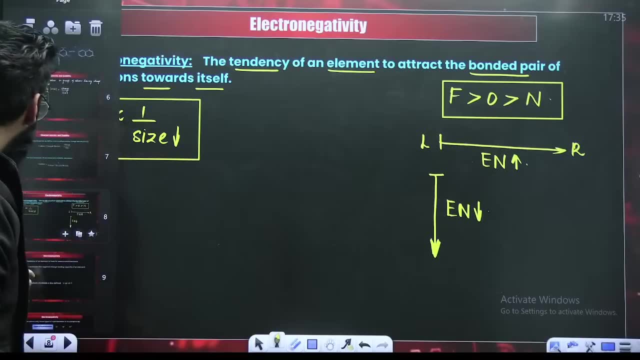 There is, there is a lot of other information which we can conclude from the term electronegativity. And what is that information? Try to understand. Try to understand What kind of other information you get from the term electronegativity. 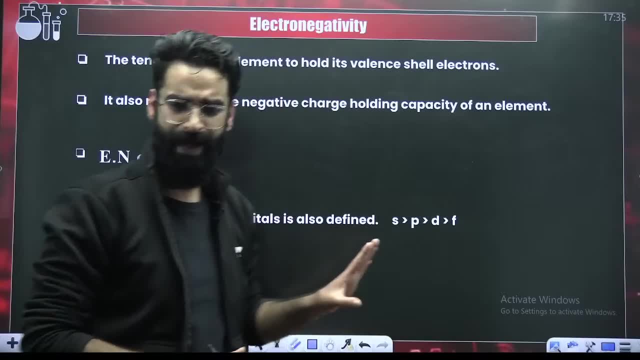 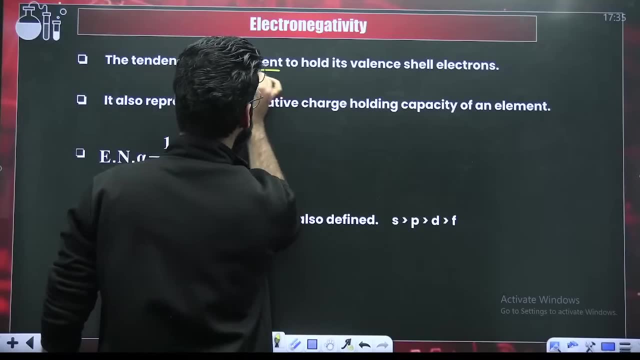 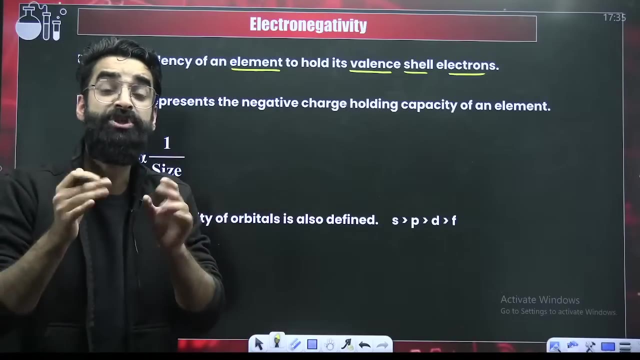 I've mentioned over here few points. I've mentioned over here few points. Just remember them from now onwards. The tendency of an element: The tendency of an element to hold its valence. electrons- Electronegativity gives you the idea about the tendency of an element. 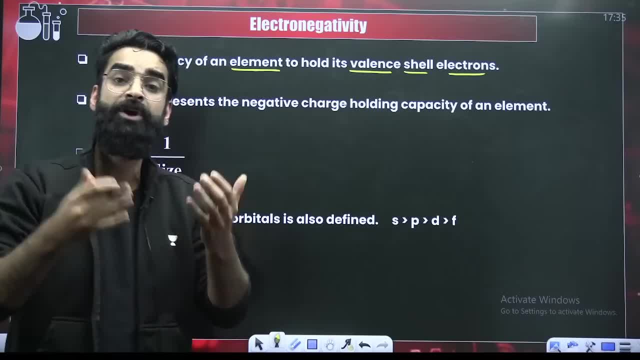 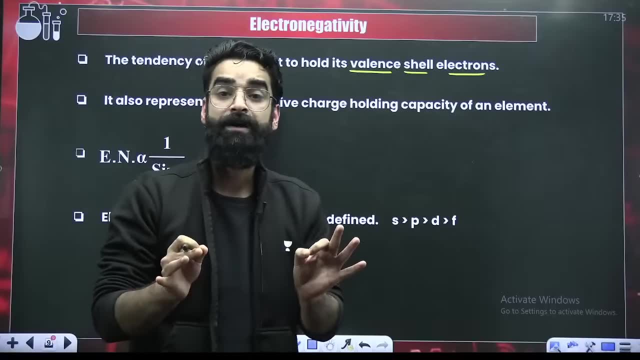 Electronegativity gives you the idea about the tendency of an element. Electronegativity gives you the idea about the tendency of an element To hold its valence electrons. to hold its valence electrons, My dear students, that element, that element which is more electronegative in nature, 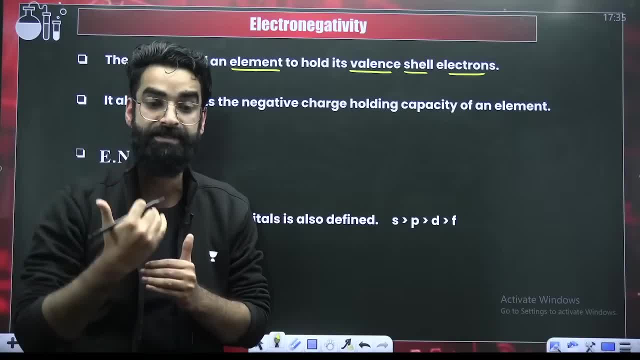 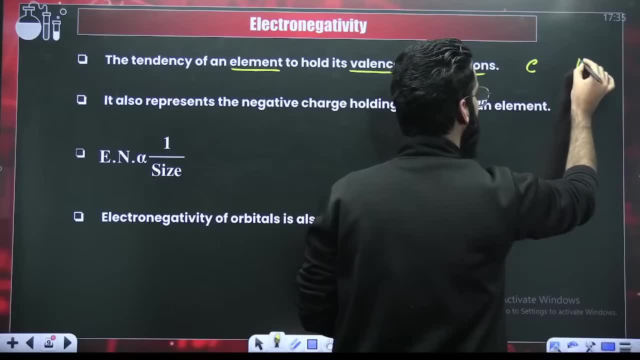 that will be having more tendency to hold its valence electrons. That will be having more tendency to hold its valence electrons. For example, let's say I've got carbon and fluorine. Let's say I've got carbon and fluorine. Which one is more electronegative. Fluorine is more electronegative. If fluorine is more electronegative, that means fluorine will be having more tendency to hold its valence electrons. To hold its valence electrons. 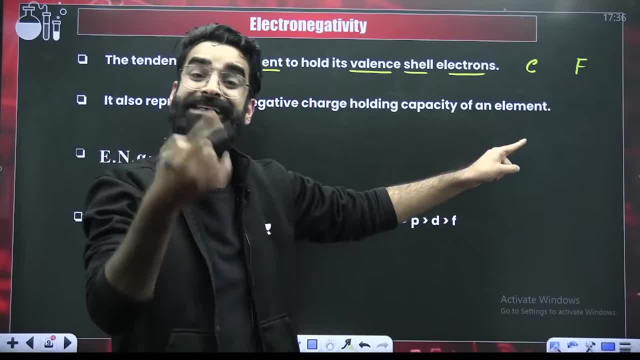 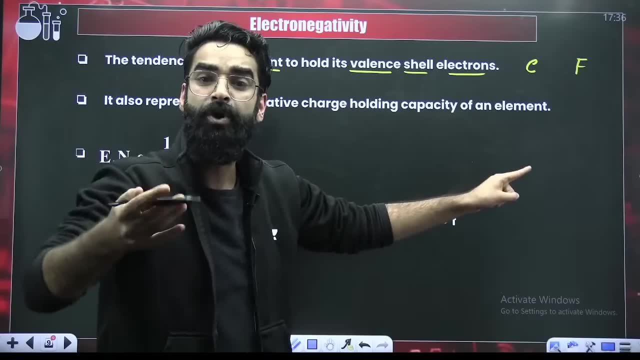 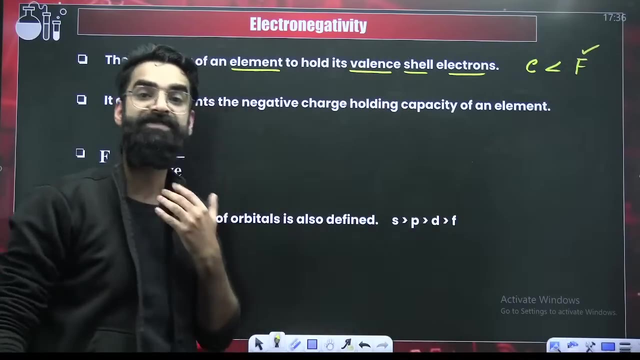 So electronegativity gives you the idea about the tendency of an element to hold its valence electrons. More electronegative element can better hold its valence electrons. As simple as that. As simple as that, Right. So fluorine has got more tendency to hold its valence electrons. 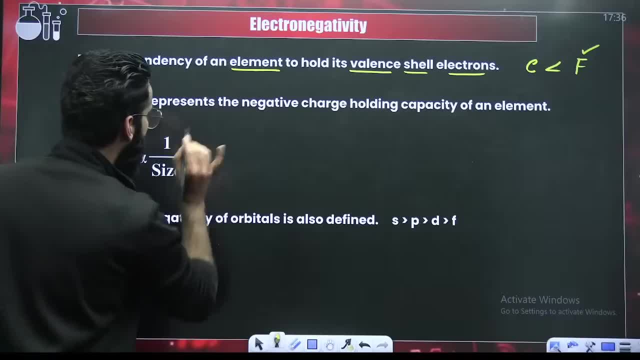 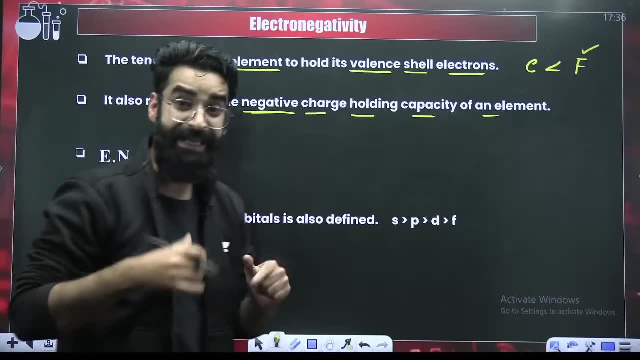 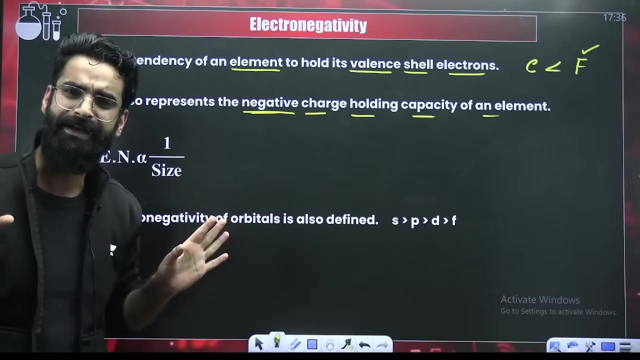 Point number one. Point number two: Electronegativity gives us the idea about the negative charge holding capacity of an element. Electronegativity: it gives the idea about the negative charge holding capacity of an element. What does it mean? It's pretty much simple. 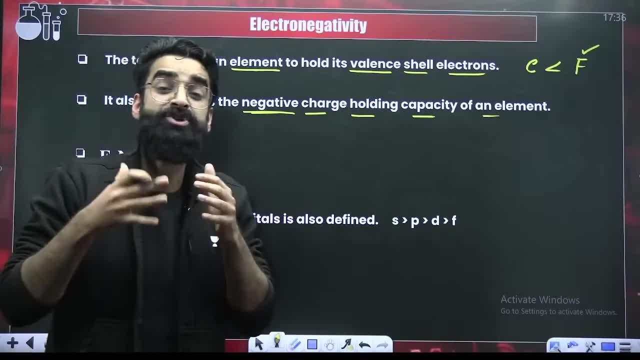 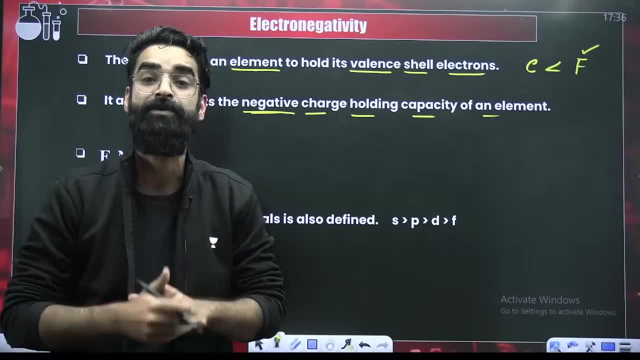 It's pretty much simple: More electronegative element it can sustain, it can hold a negative charge. More electronegative element can sustain negative charge, It can hold a negative charge. For example, Let's say you've got oxygen carrying negative charge. 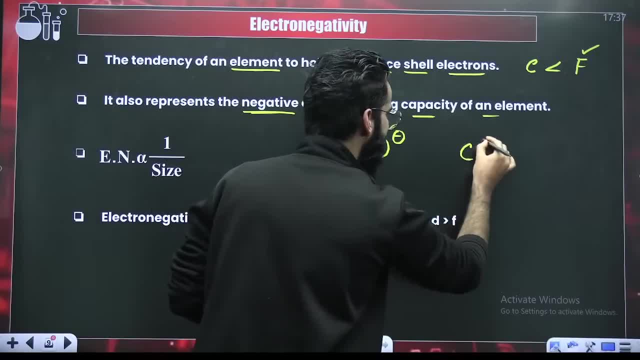 You've got oxygen carrying negative charge. Let's say: you've got carbon carrying negative charge. You've got oxygen carrying negative charge. You've got carbon carrying negative charge. Just tell me one thing in the chats: Which one is more electronegative? 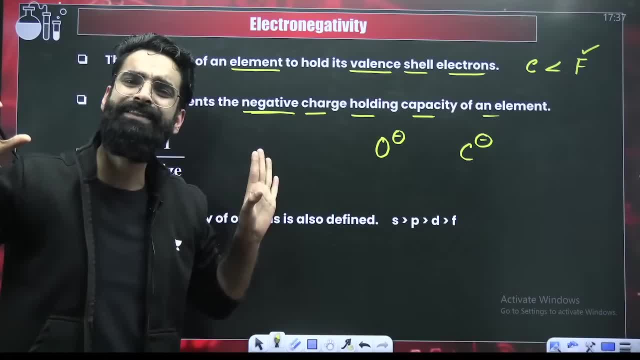 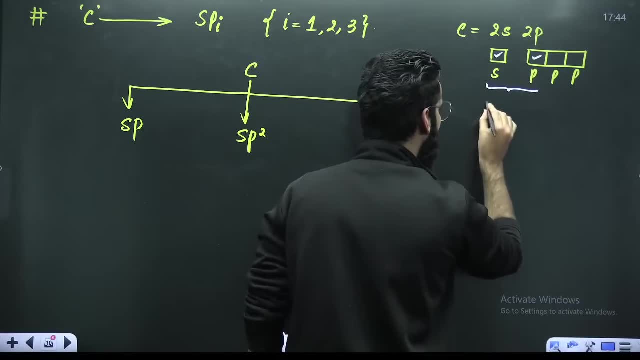 It means that oxygen can hold this negative charge in a better way than that of carbon. It means that oxygen can hold this negative charge in a better way than that of carbon. I'll be getting two hybrid orbitals. number of atomic orbitals intermixing: intermixed is equal to the number. 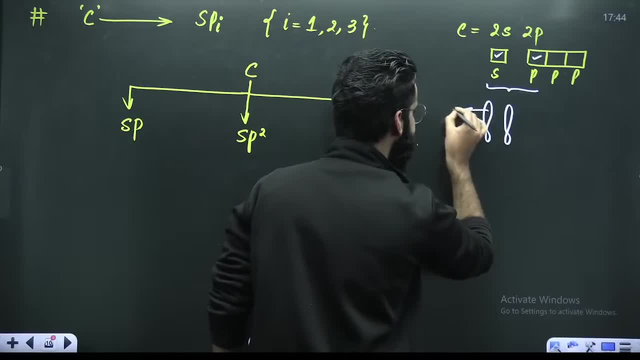 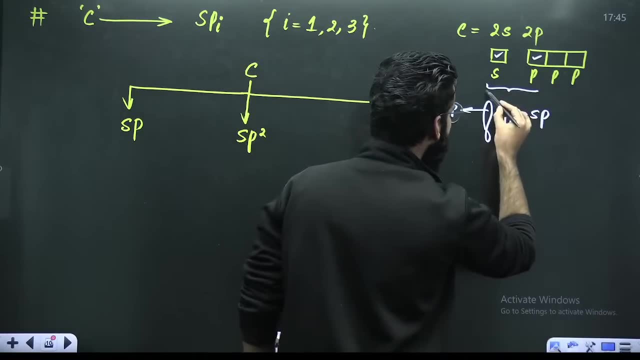 of hybrid orbital form and this particular hybrid orbital I'll be calling as SP hybrid orbital, this particular hybrid orbital I'll be calling as SP hybrid orbital. Similarly, imagine that let's say this S and 2P, this S and these 2P orbitals have participated in the intermixing. 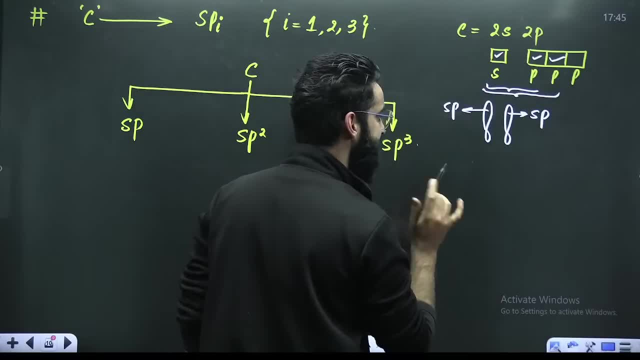 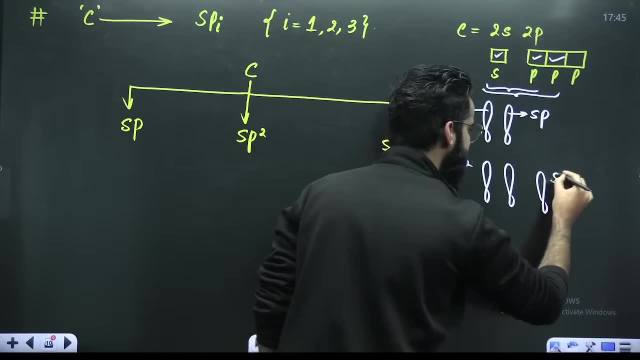 so three atomic orbitals. if participating in the intermixing it will lead to the formation of three hybrid orbitals like this right, and each hybrid orbital you'll be calling as SP2 hybrid orbital right. Similarly, if all these four atomic orbitals will participate, 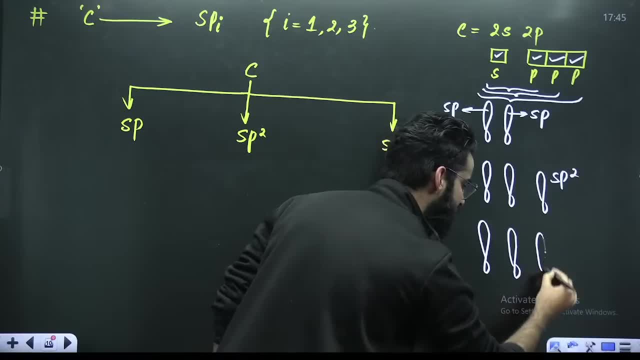 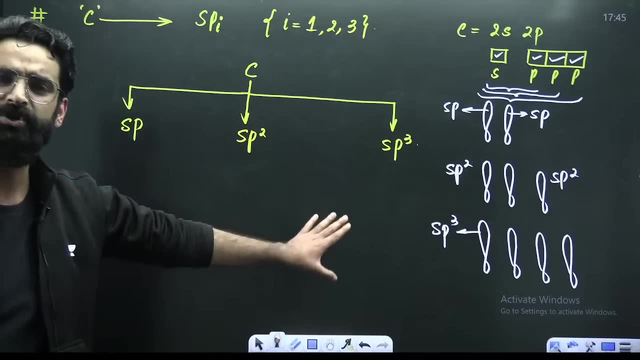 in the intermixing, it leads to the formation of four hybrid orbitals, and I'll be calling each hybrid orbital here as SP3 hybrid orbital, something which you all must be knowing. So carbon shows how many types of hybridization: SP, SP2 or SP3- perfect. Now, people, one thing, One thing in case of SP hybridization. in case of SP hybridization, how many hybrid orbitals do we get? we get two hybrid orbitals. This is your first hybrid orbital and similarly, my dear students, I can say: this is your second hybrid orbital- perfect. 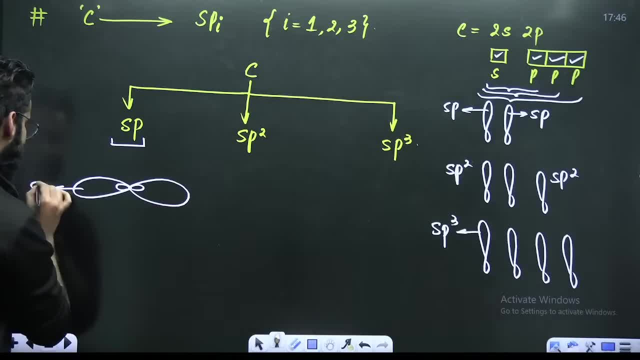 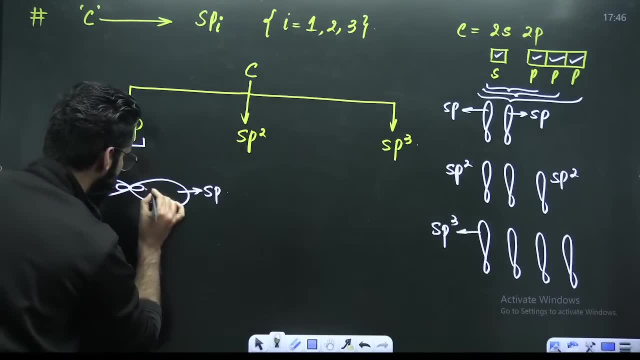 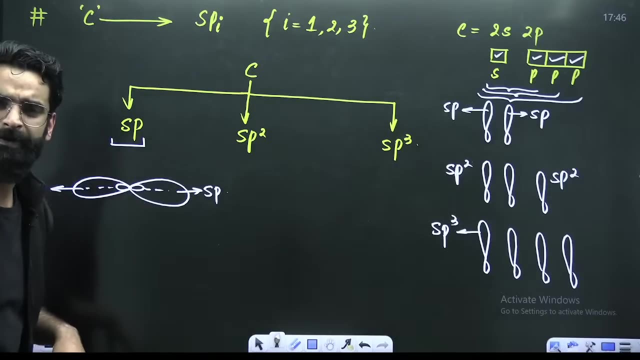 These are your two SP hybrid orbitals. This is SP. even this is SP hybrid orbital. perfect, Okay, if I ask you these hybrid orbitals, if you remember they are, they are placed in such a way That there should be minimum repulsions between them, right? 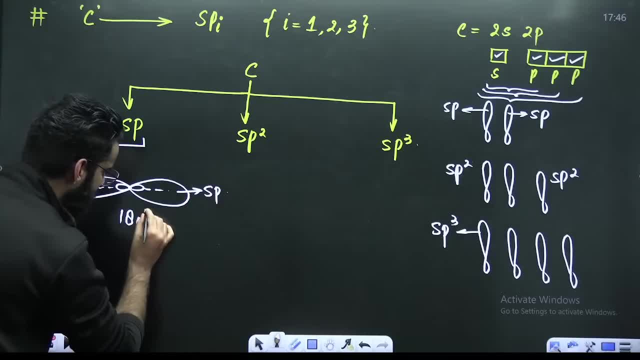 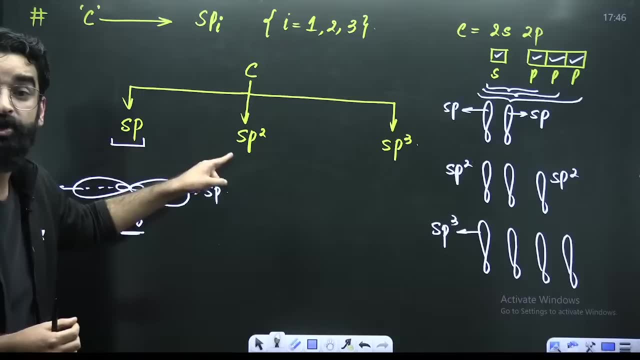 So that means they are placed at an angle of what right? here They are placed at an angle of 180 degree. perfect. SP2- SP2 hybridization. How many hybrid orbitals do we get here? We get three hybrid orbitals. This is your first hybrid orbital. 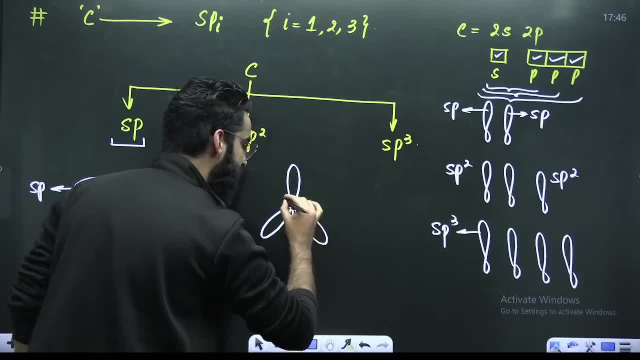 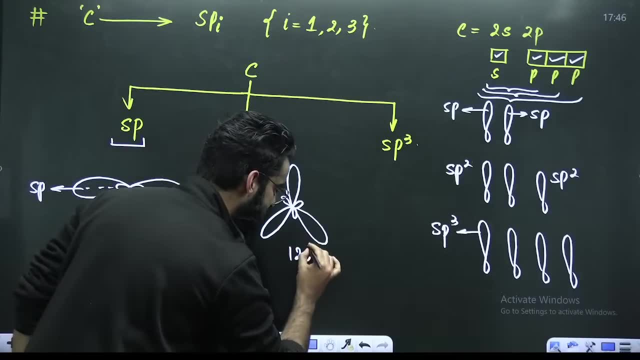 This is your second hybrid orbital right. This is your third hybrid orbital, and they are placed in such a way that there are minimum repulsions between them. So at what angle they'll be? they'll be placed at an angle of 120 degrees. 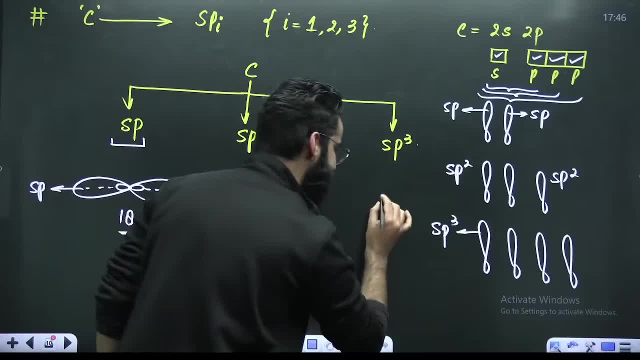 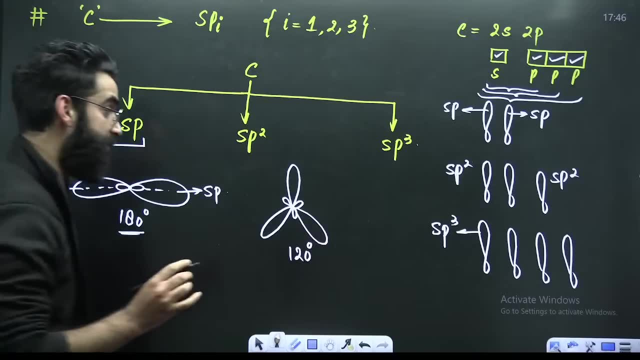 Okay, perfect. Similarly, if I talk about SP3 hybridization, in case of SP3 hybridization, How many hybrid orbitals do we get? We get four hybrid orbitals. We get four hybrid orbitals, and they are placed in such a way that 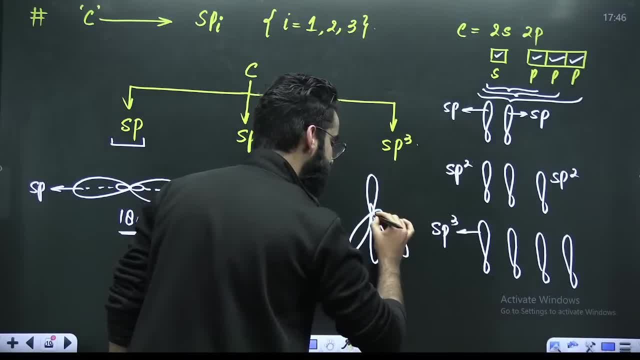 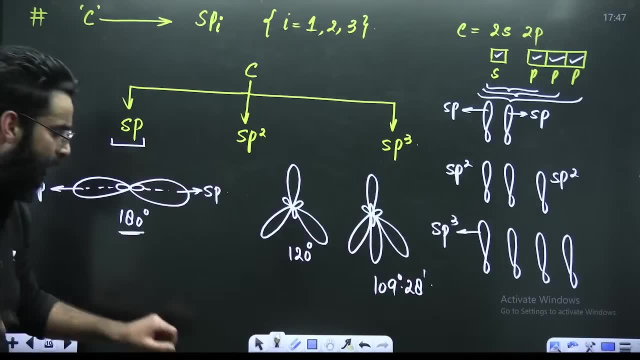 there should be minimum repulsions and maximum stability between them. Perfect. and they are placed at an angle of what? 109 degree, 28 minutes. I believe this is something which you all already know. I believe this is something which you all already know. 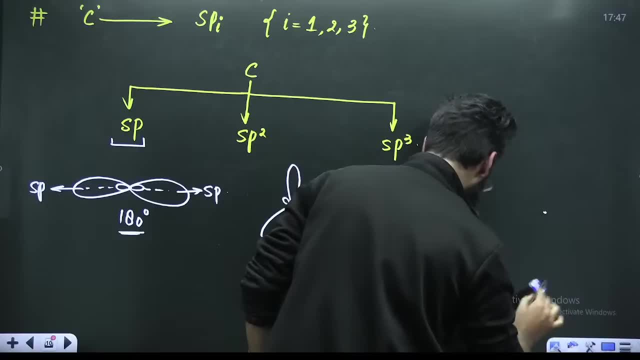 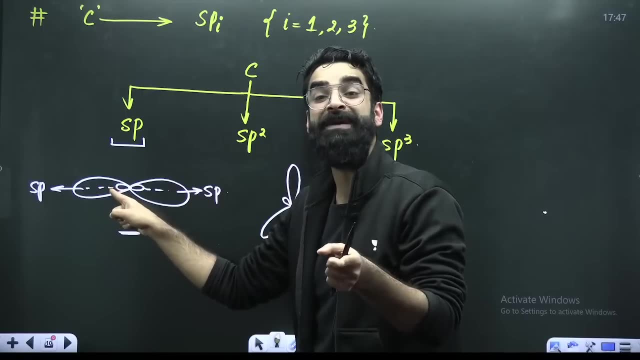 Perfect. If not, then remember it from now onwards. Now is: tell me one thing. Tell me one thing. See, if I ask you how this SP hybrid orbital was made? Basically, when one of the s orbital and one of the p orbital of carbon, when 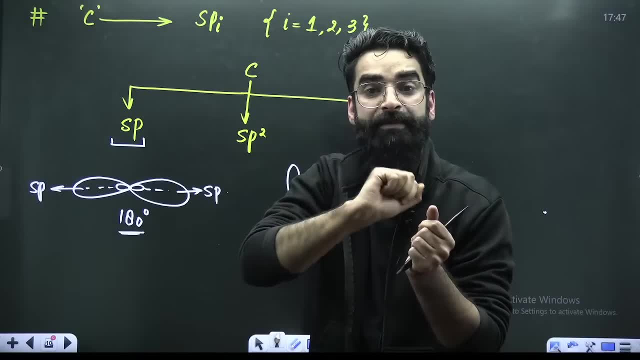 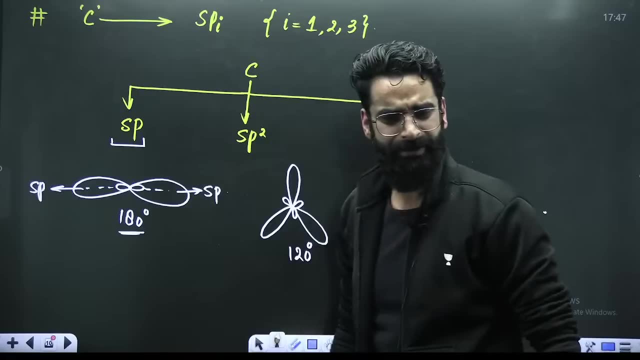 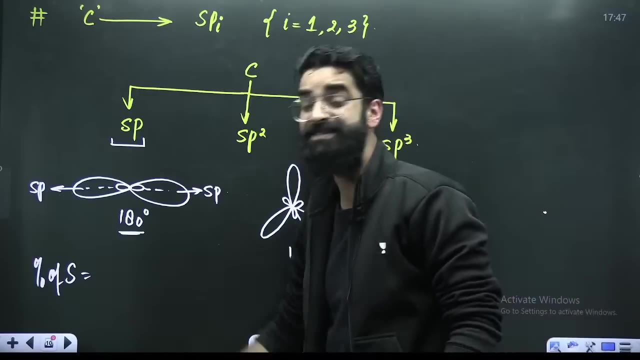 they intermixed, they resulted in the formation of two hybrid orbitals, SP- SP. Can you let me know, will there be any S character present in this hybrid orbital? Absolutely, There will be some S character present in SP hybrid orbital as well. How do you get the percentage of S character in any hybrid orbital? 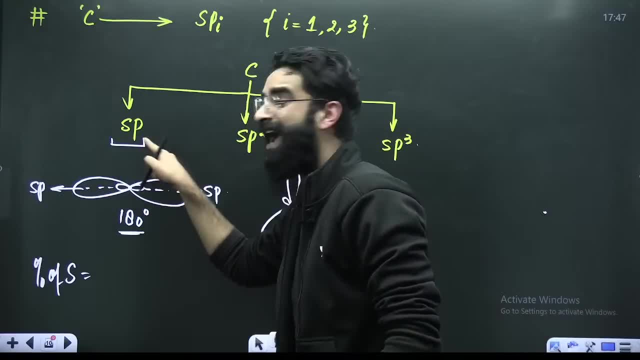 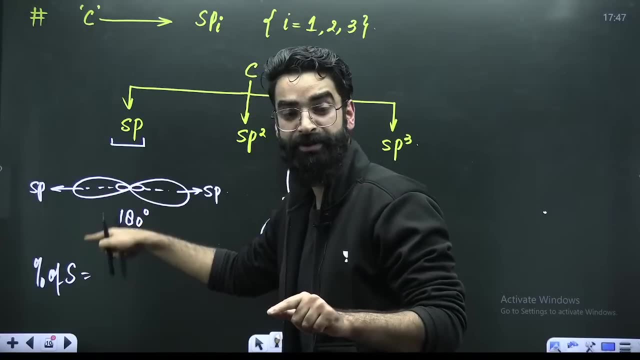 It's pretty much simple. Try to understand in your SP hybrid orbital, in your SP hybrid orbital, which is formed when S and P intermixed, So there is some S character here. in this hybrid orbital There is some P character as well. How do you get the percentage of S character? 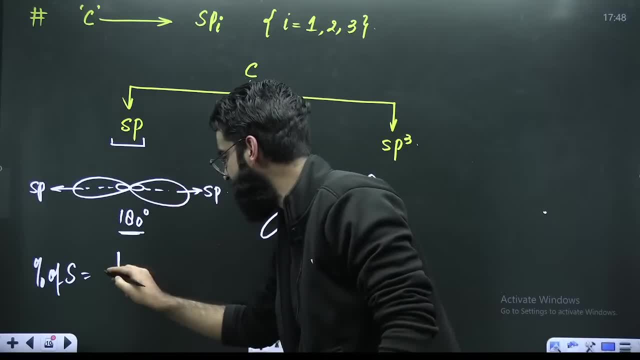 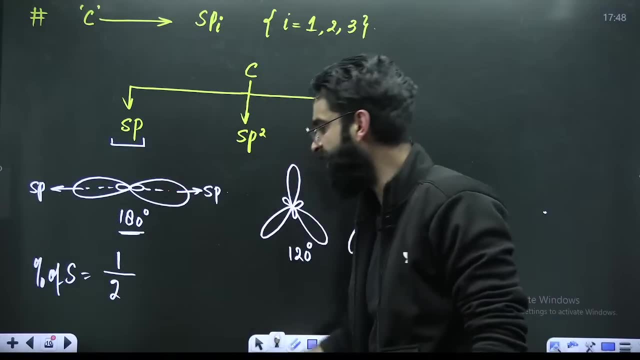 Tell me how many s orbitals participated. one s orbital past participated. divided by how many total orbitals Participated to total orbitals participated in the intermixing, multiply the hundred, the value comes out be 50%. what is meant by this 50%? it means 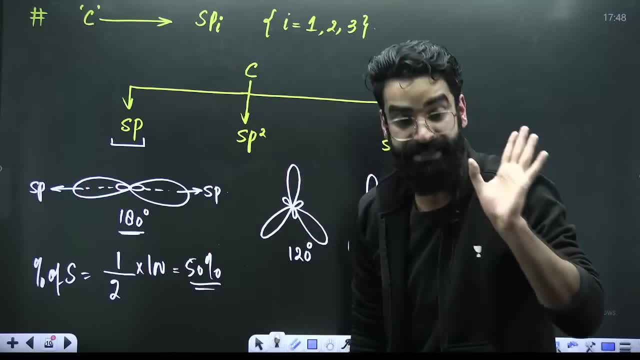 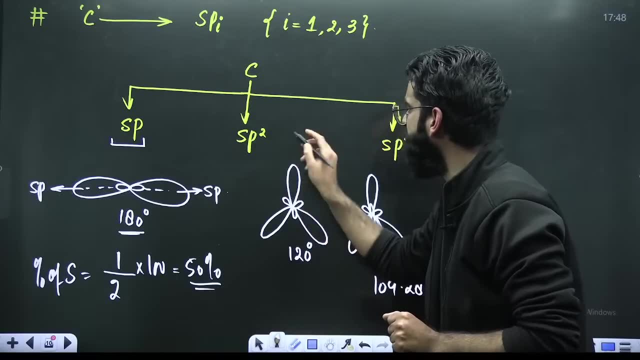 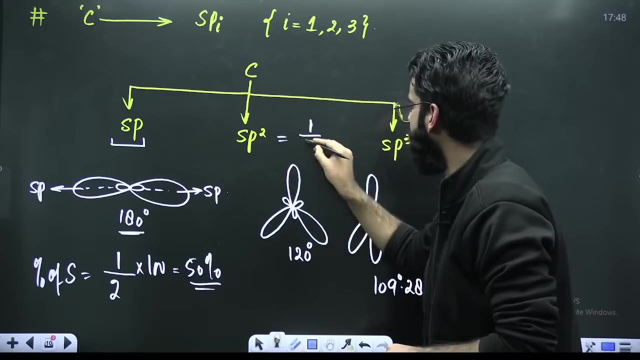 this particular hybrid orbital. It contains 50% of S character. It contains 50% of S character. What about this hybrid orbital? What about this hybrid orbital? If I ask you about the percentage of S character in SP, two hybrid orbital, so one s orbital participated and in total three orbitals participated. 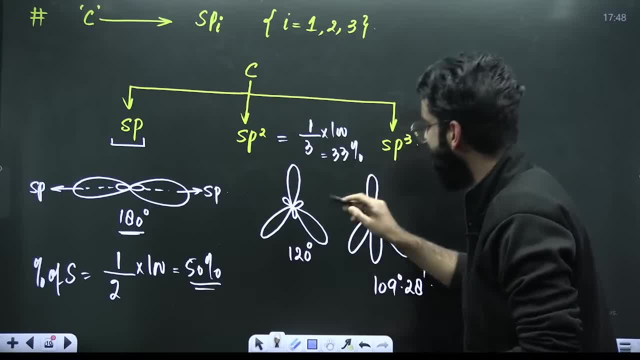 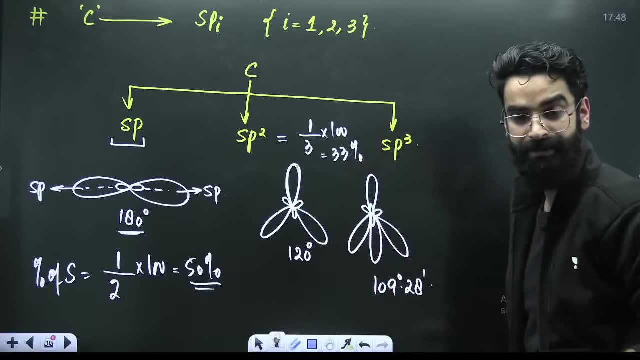 multiplied by hundred, the value comes out 33%. so I would say in this SP two hybrid orbital, in this SP two hybrid orbital, there will be 33 percentage of S character. Similarly, what is going to be the S character here in SP three hybrid? 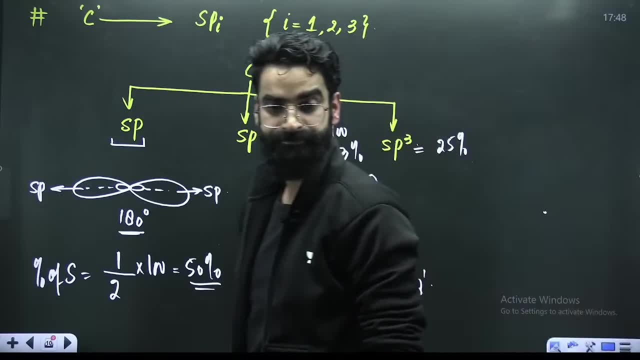 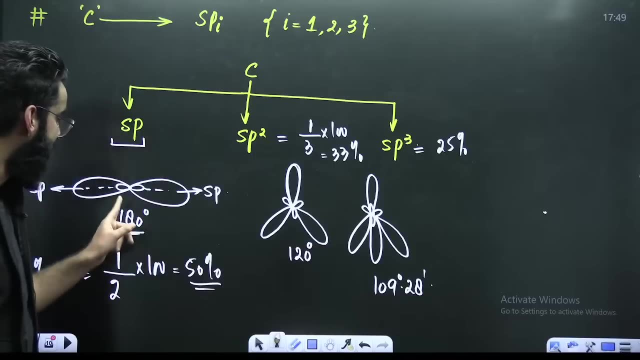 orbital. It's going to be 25%, it's going to be 25%, it's going to be 25%. now, people, you tell me one thing. you tell me one thing: SP, SP two, SP three, SP. bond angle is 180 and it's 120 and it is 109 as you move from left to right. here is: 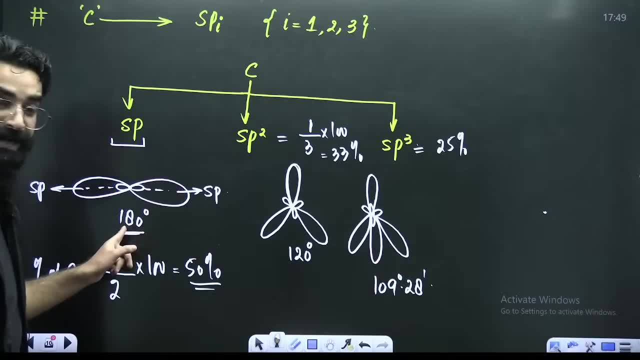 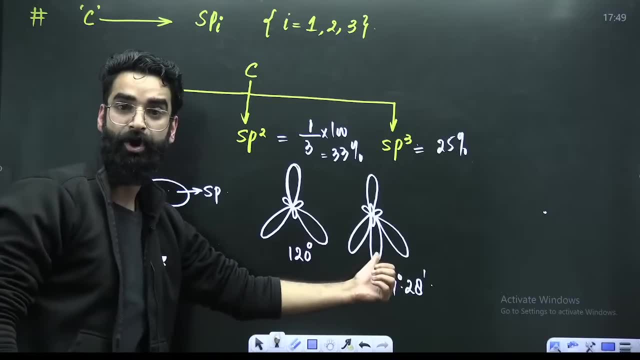 the bond angle decreasing or increasing? 180,, 120,, 109. on moving from left to right, is the bond angle increasing or decreasing? Bond angle is decreasing. On moving from left to right, bond angle is decreasing. Bond angle is decreasing. At the same time, what is happening to the percentage of S character? 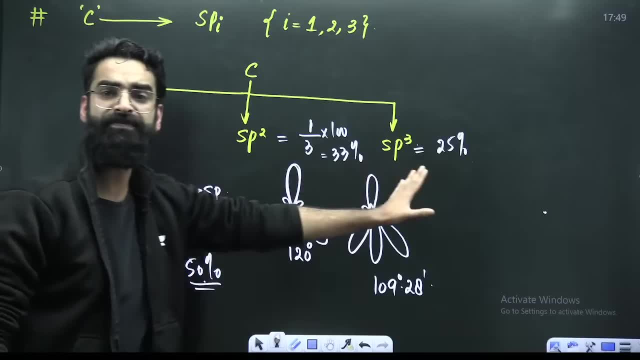 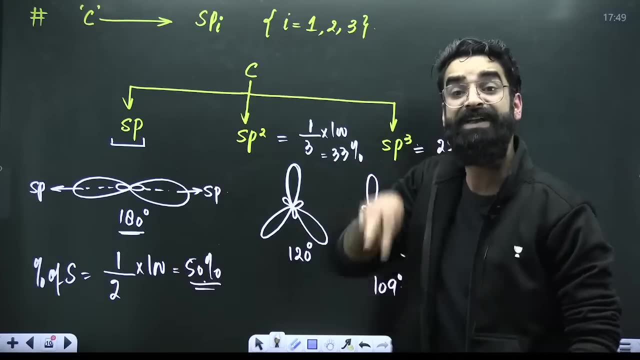 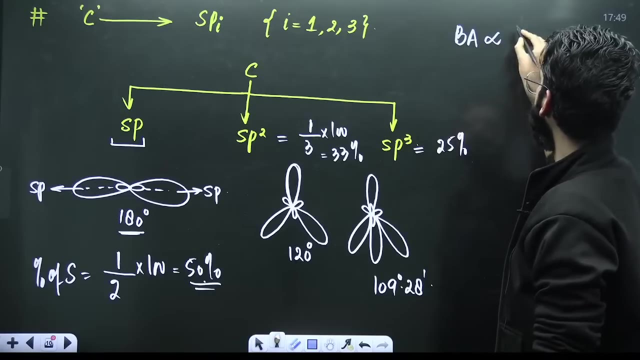 50,, 33,, 25. on moving from left to right, percentage of S character is also decreasing. When you move from left to right, here bond angle is decreasing as well as percentage of S character is decreasing. So can I say this When I say bond angle is directly proportional to percentage of S character? 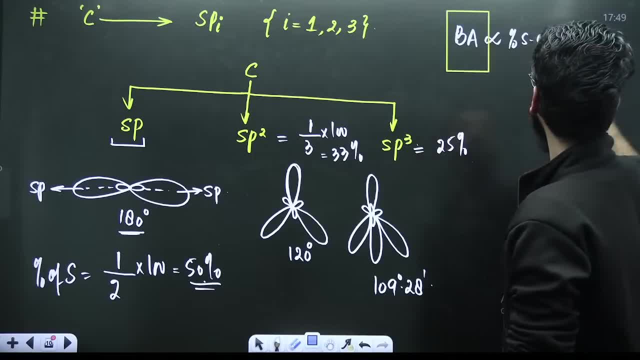 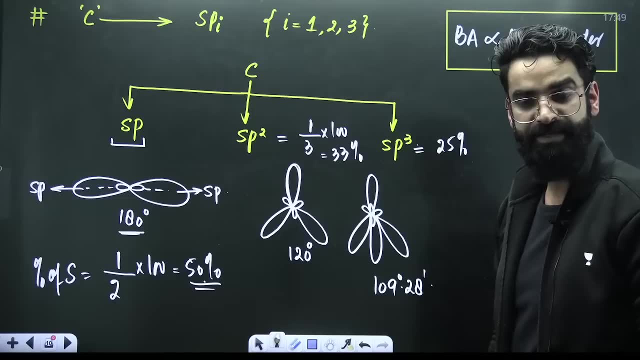 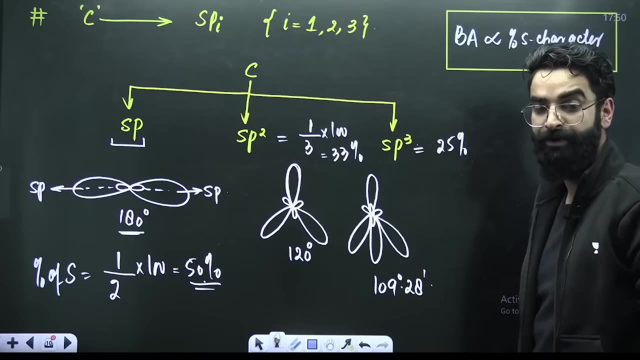 Bond angle is directly proportional to percentage of S character. Right Percentage of S character. Is it clear? Did you get the idea of this particular thing? Did you get the idea of this particular statement? Quickly, let me know in the chats everyone. 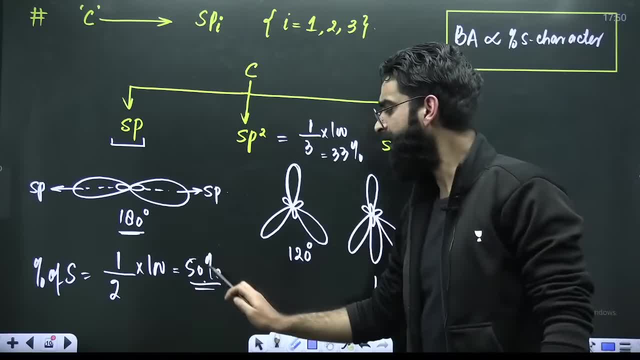 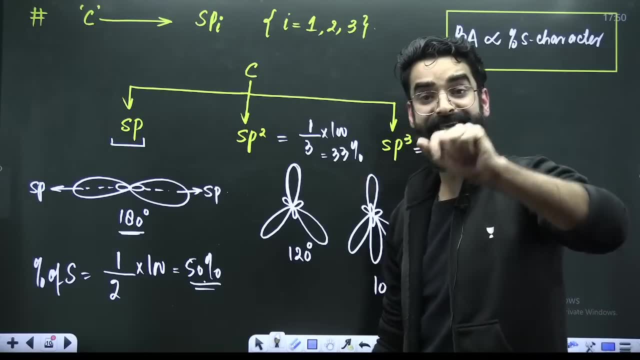 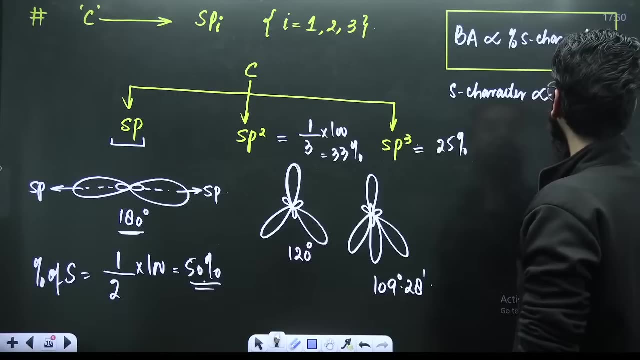 So I would say more the bond angle, more the S character. And, if you remember, S character is related to electronegativity. If you remember, S character is related to electronegativity. S character is related to electronegativity, like this: 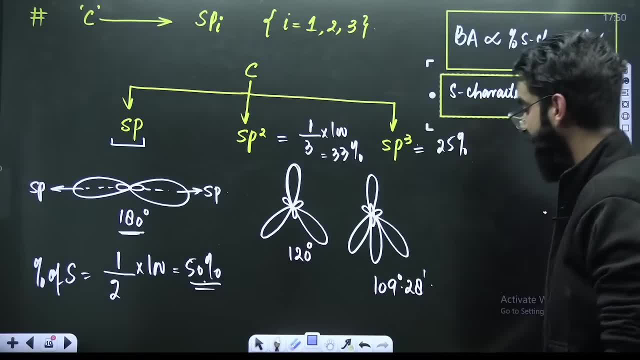 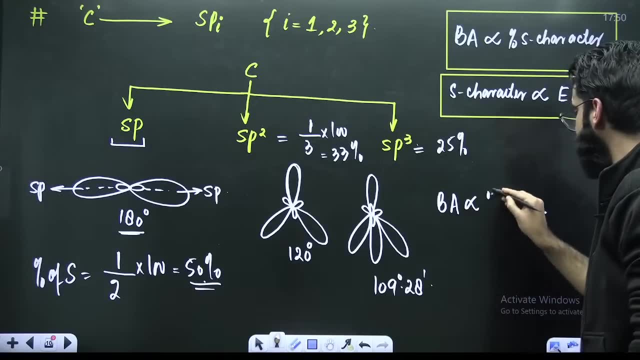 More the S character, more the electronegativity. More the S character, more the electronegativity. So, from this particular slide, what you have to remember, You have to remember something like this: Bond angle Is directly proportional to percentage of S character. 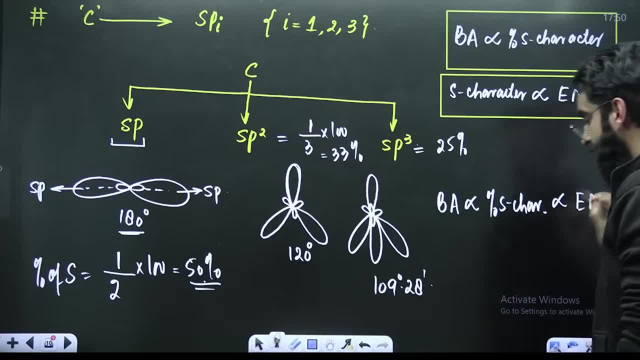 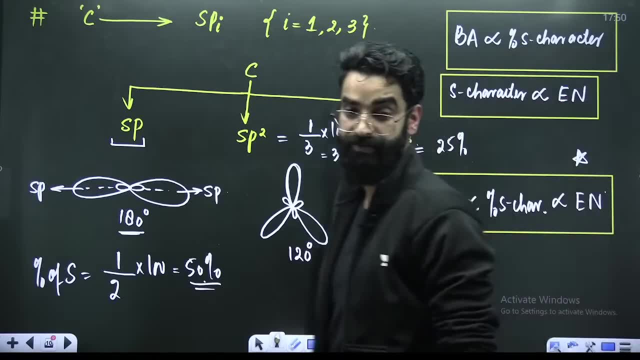 Right Percentage of S character, But is directly proportional to electronegativity Right. So, my dear students, This is the conclusion of the entire thing which I was teaching you till now. I hope this is clear to everyone. I hope this is clear to everyone. 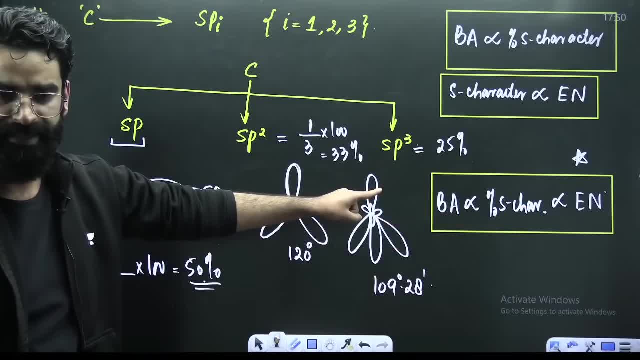 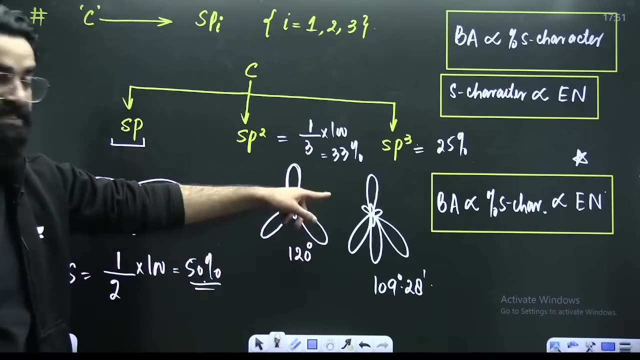 I hope this is clear to everyone. Yes, Quickly, let me know in the chats, with some fire emojis, If you got this particular concept, because this is important, This is important. Quickly, people, Quickly, everyone, Everyone in the chats. This is something which is important. 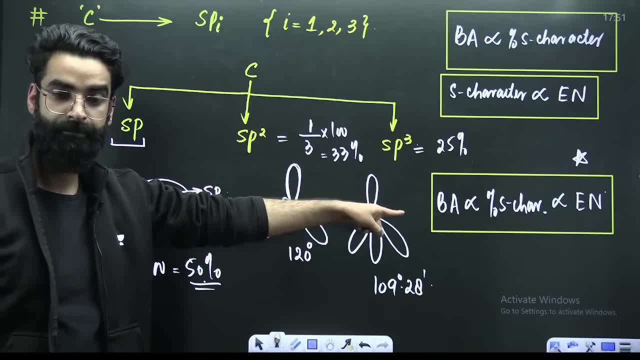 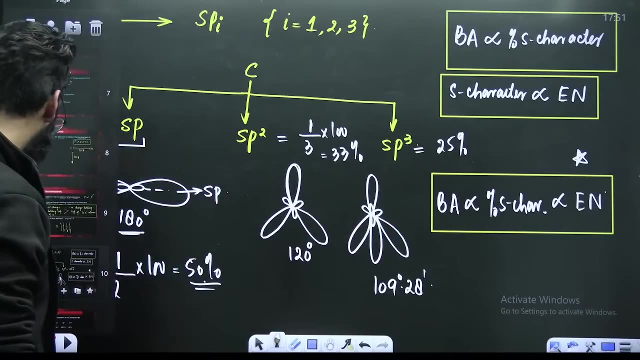 I will be utilizing this concept everywhere. Yeah, In the chats, everyone. I want the chats to go up continuously. Done and dusted, Done and dusted. Perfect guys, If this is done and dusted, If this is done and dusted. 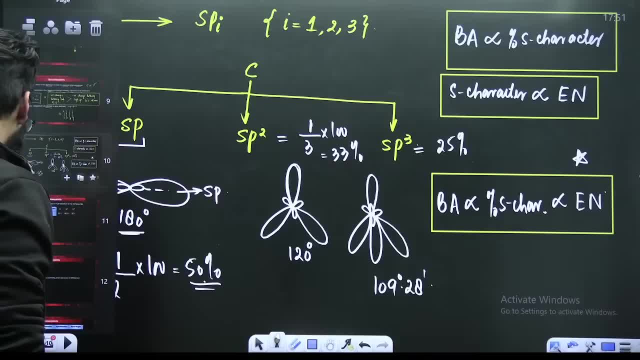 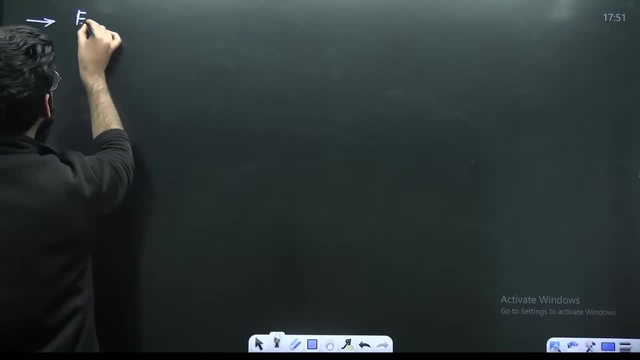 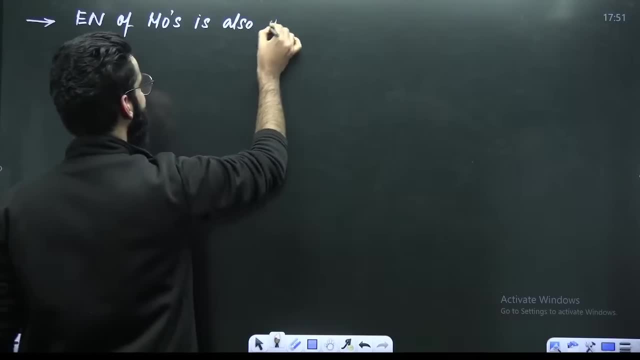 Then, Then. let me tell you one more thing thing. let me tell you one more thing. can i write a simple statement like this? can i say: electronegativity of hybrid orbitals is also defined. you are going to answer this question: electronegativity of hybrid orbitals. 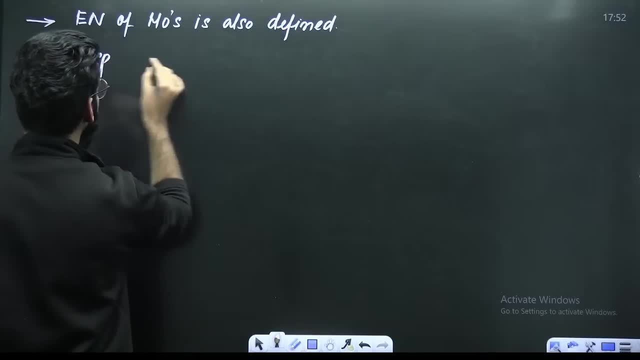 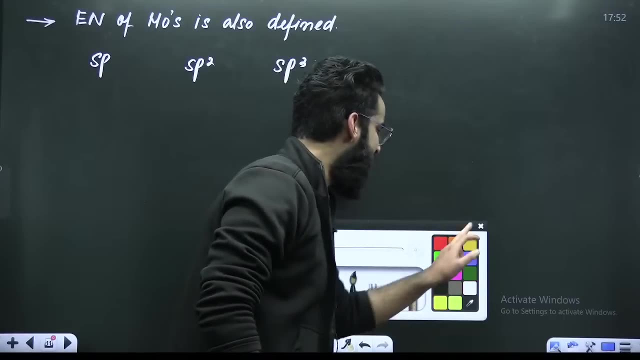 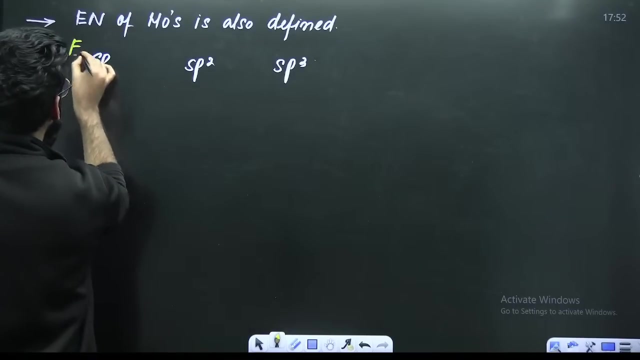 is also defined. if i have sp hybrid orbital, if i have got sp2 hybrid orbital, if i have got sp3 hybrid orbital, can you tell me which hybrid orbital has got more s character? it is, sp s character is directly proportional to electronegativity. so can i say electronegativity of sp hybrid orbital? 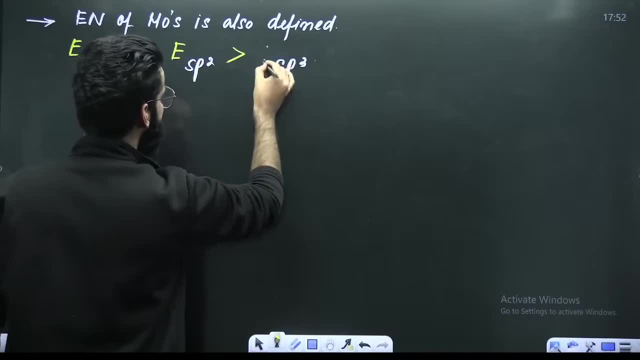 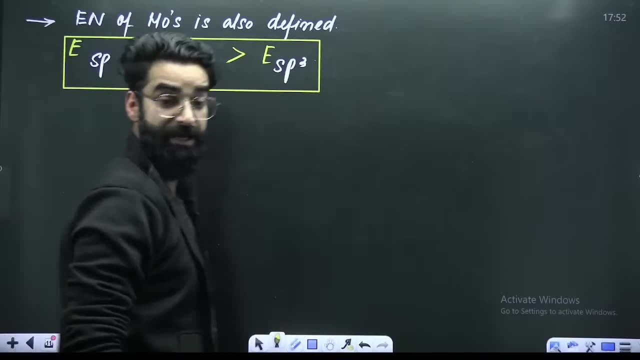 will be greater than that of electronegativity of sp2, which will be greater than that of electronegativity of sp3. so guys do remember this particular statement as well: electronegativity of sp- hybrid orbital- will be more than that of sp2. then that of what? than that of? 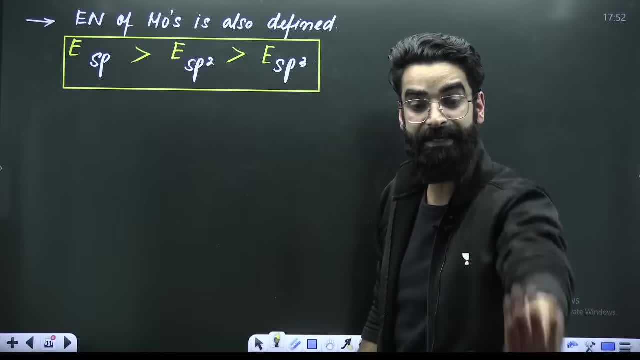 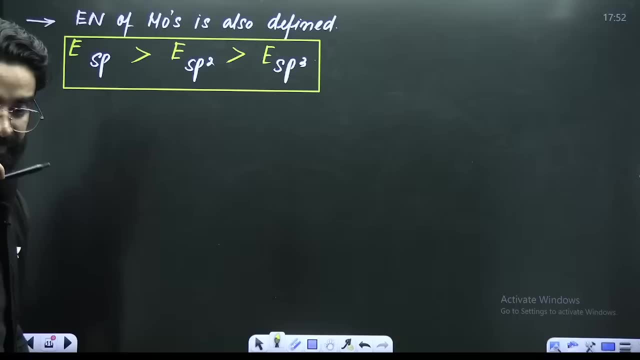 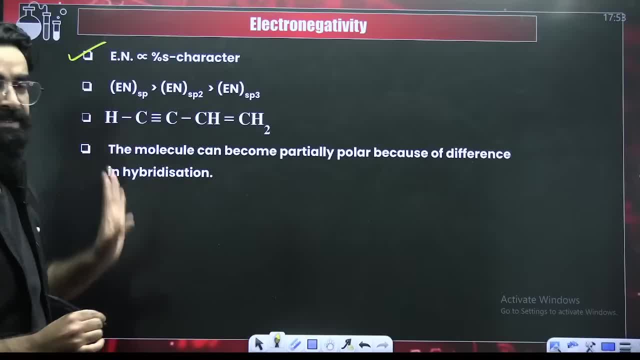 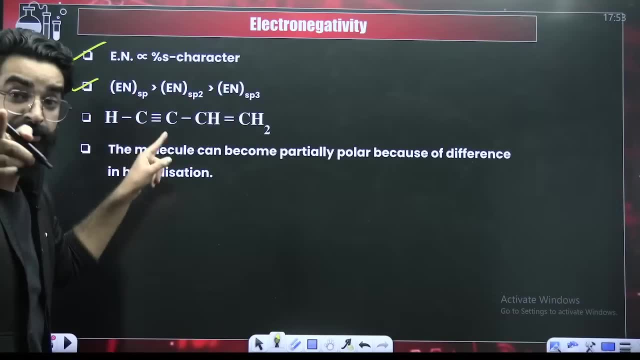 clear to you. number one: electronegativity is directly proportional to percentage of S character. electronegativity of SP- hybrid orbital, is greater than that of SP2, is greater than that of SP3,. you know the logic, you know the reason. point number three, point: 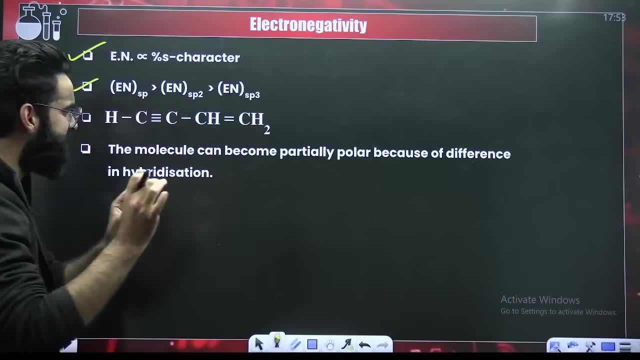 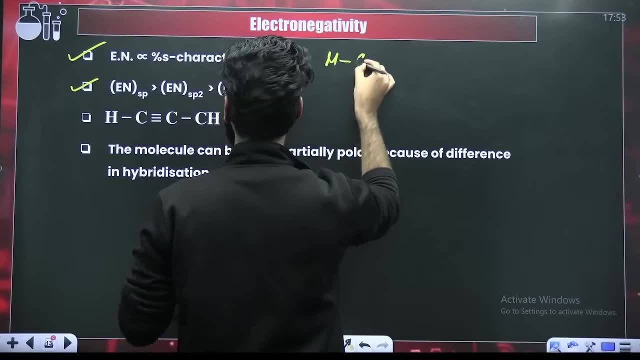 number three. this is just one example which is going to clear you one simple thing, which is going to clear you one simple thing. see, guys, let me make the molecule again like this: this H, this is C, then you have got triple bonded carbon. right? then you have. 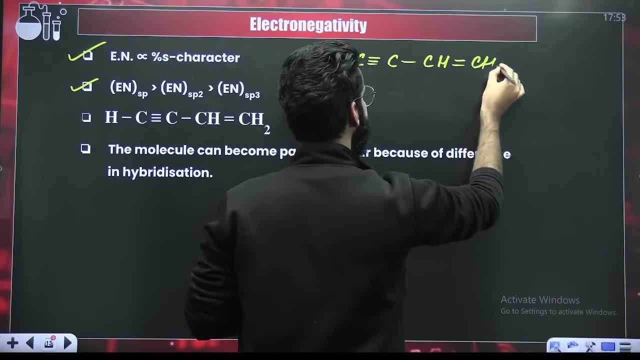 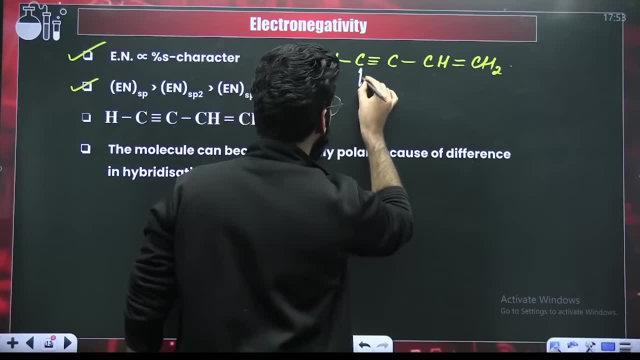 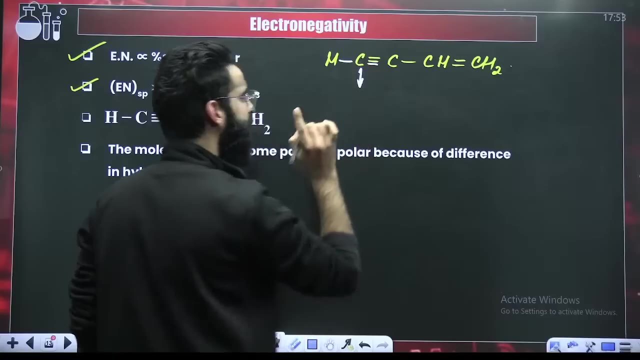 got TH and double bond CH2, double bond CH2, now people tell me just one simple thing: tell me about this particular carbon How many sigma bonds it is forming. how many sigma bonds it is forming? it is forming one and two. it is forming two sigma bonds. it is forming two sigma bonds. it is forming. 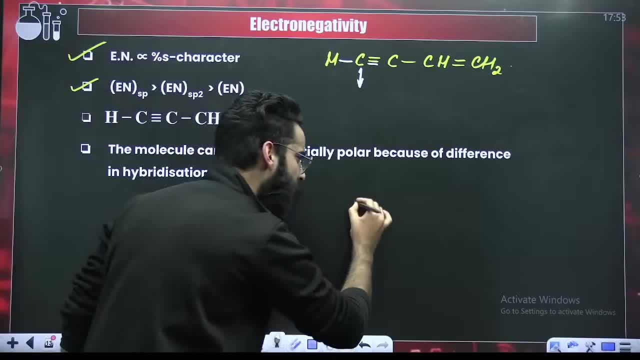 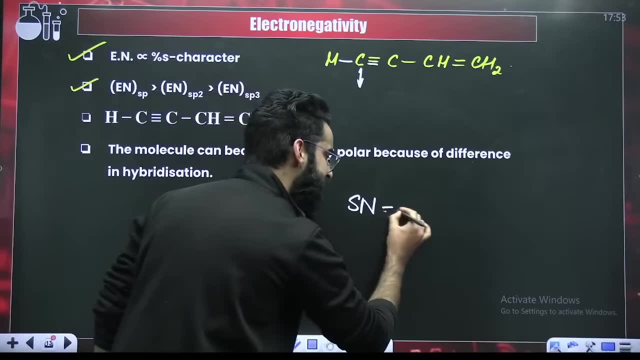 two sigma bonds. try to understand one more thing. I hope you know the term called as steric number. I hope you know the term called as steric number. what is steric number? steric number means sigma plus lone pair. sigma plus lone pair if the steric number comes out. 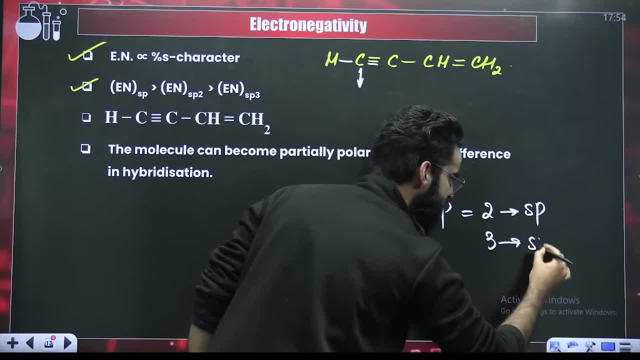 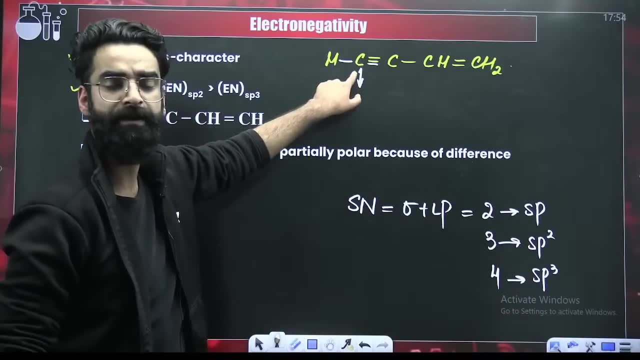 to be two, the hybridization is SP. If it is three, the hybridization is SP2,. if it is four, the hybridization is SP3,. okay, Now, if I talk about this particular carbon, how many valence electrons carbon has? how? 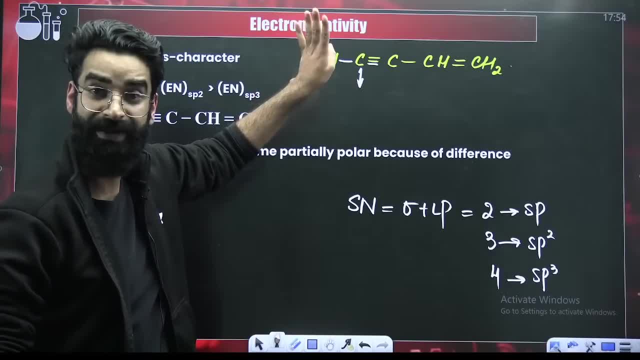 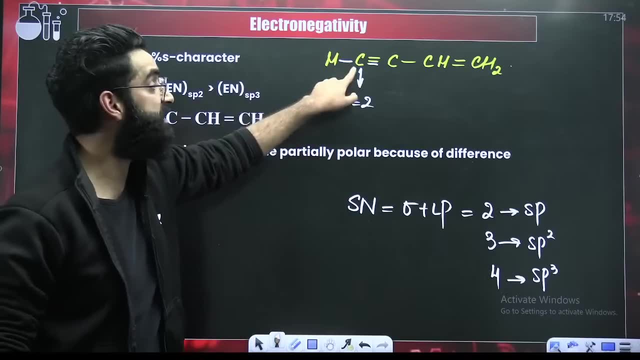 many valence electrons. carbon has four, four valence electrons. how many sigma bonds it is forming. it is forming two sigma bonds. it is forming two sigma bonds. carbon has four valence electrons and how many sigma bonds it is forming. it is forming two sigma. 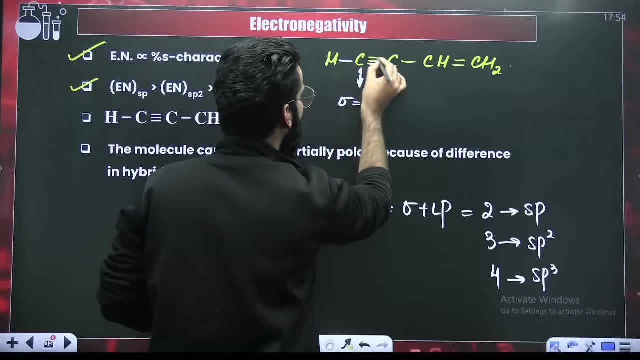 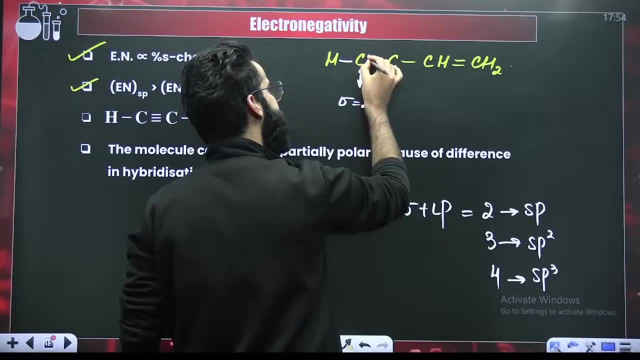 bonds. now tell me how many total bonds this carbon is forming: One, two, three, four. carbon is forming four bonds. right, and in order to form four bonds, can I say, carbon would have utilized all its four valence electrons absolutely. 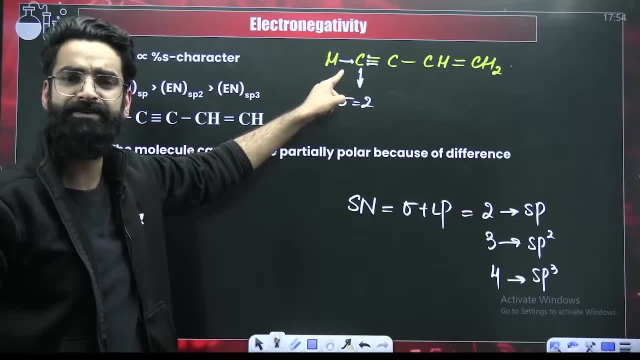 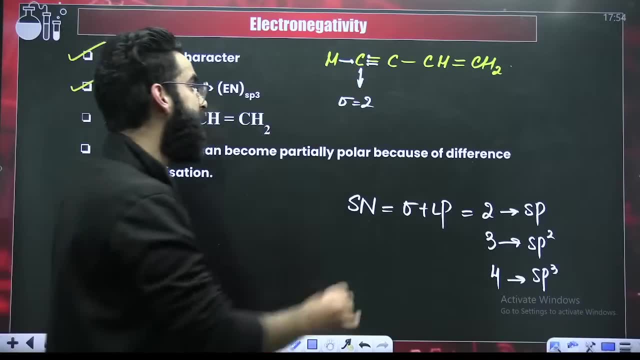 carbon would have utilized all its four electrons or its four valence electrons. carbon had four valence electrons and it has utilized all those four valence electrons for the bonding. so how many lone pairs this carbon will be having? it will be having zero lone pair. 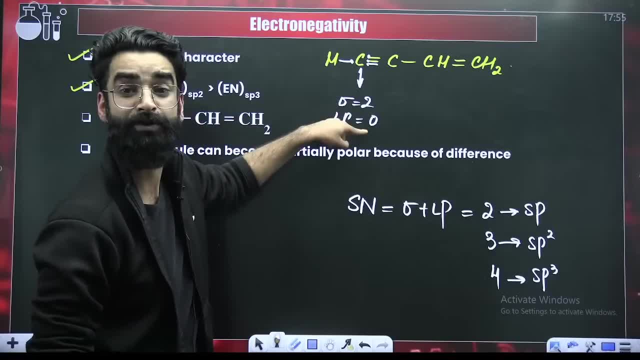 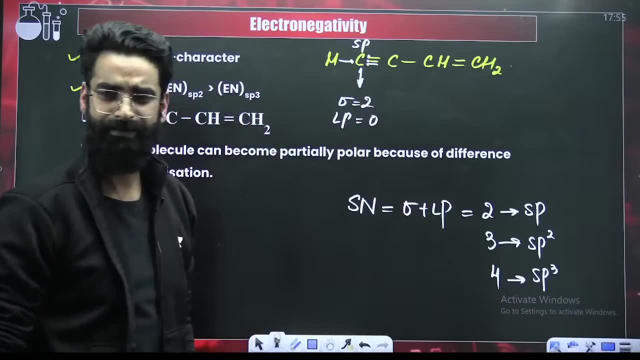 if I ask you steric number of this carbon, sigma plus lone, pair, two plus zero, that is two. If steric number is two, that means hybridization. So this particular carbon has got the SP hybridization head right. yes, right. people in the similar 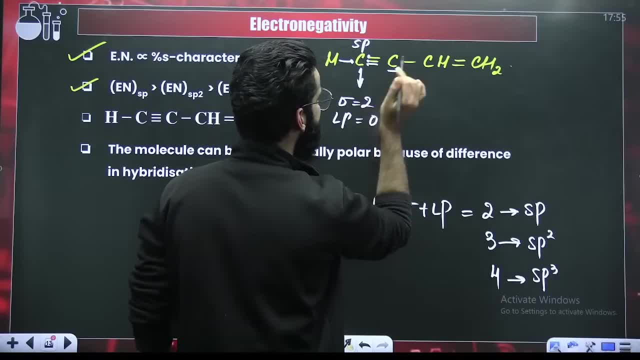 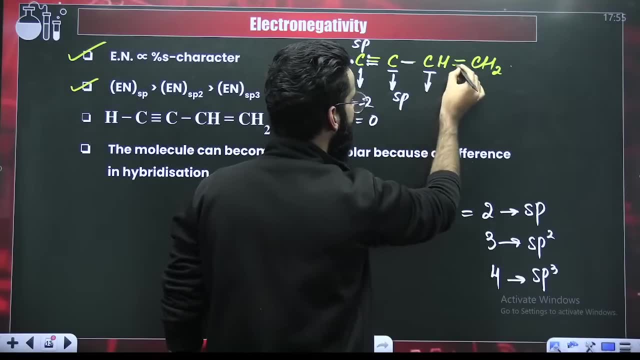 way. look at this particular carbon. look at this particular carbon, how many sigma it is forming, One and two. so again I will say: this carbon is SP hybridized. how many, how many sigma this is forming? one sigma, two sigma and one more with hydrogen right, so three sigma. 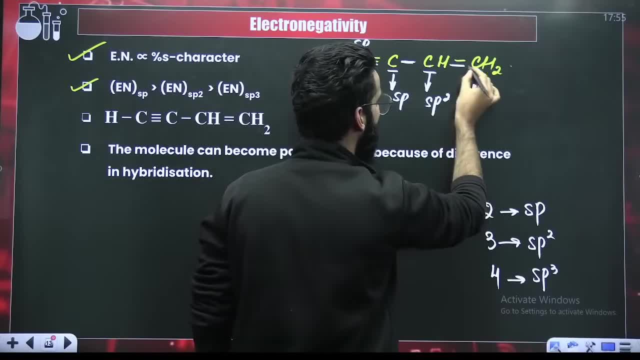 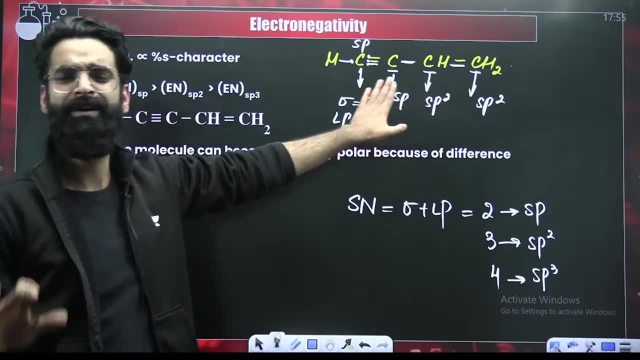 it is forming, so it is SP2, this particular carbon. how many sigma it is forming? one sigma and two with hydrogen, so this again SP2, right, so I believe, from the structure, you can easily let me know, you can easily let me know the hybridization of different. 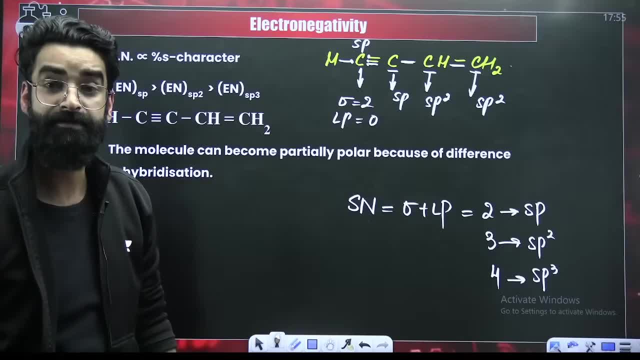 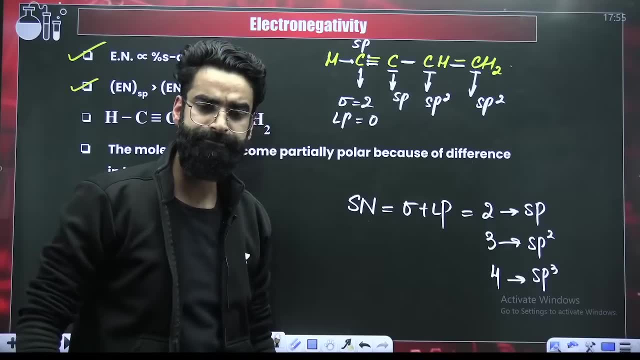 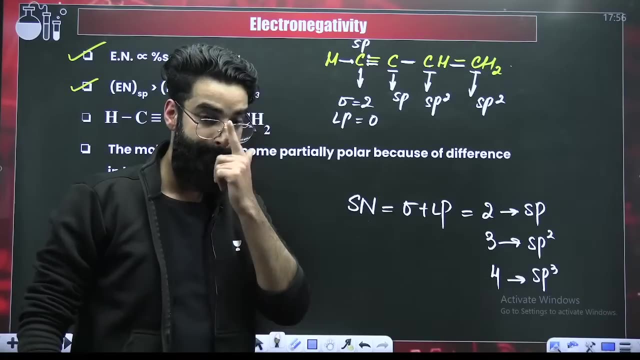 atoms. yes, hybridization of different atoms. I believe this is clear. just tell me one thing. just tell me one thing: do you know how to calculate lone pairs? do you know how to calculate lone pairs? just tell me that. yes or no? yes or no, do you know how to calculate? 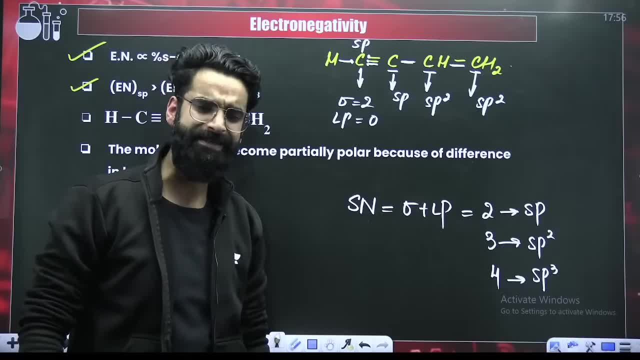 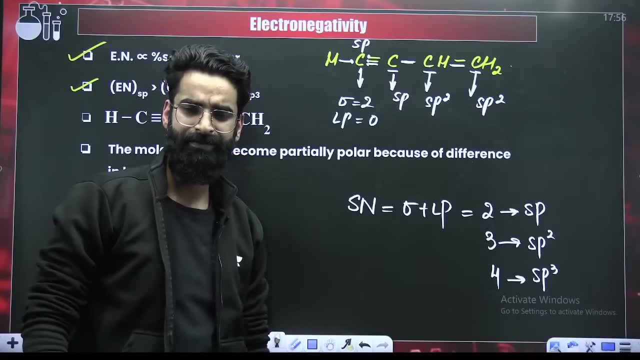 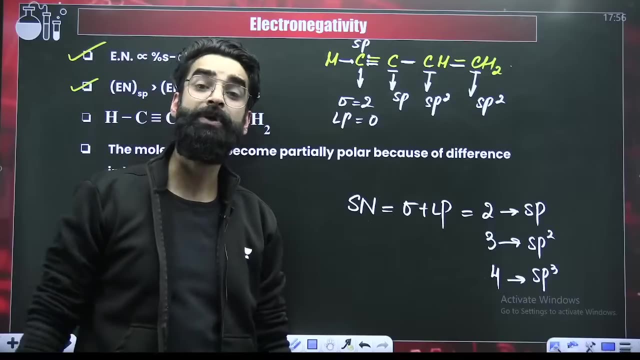 lone pairs Quickly. guys, everyone in the chats, what do you think? yes or no? honestly, there is no need to be shy or something. I am here to teach you everything. that's why I told I will be starting exactly from basics. one example I will take, by means of which you 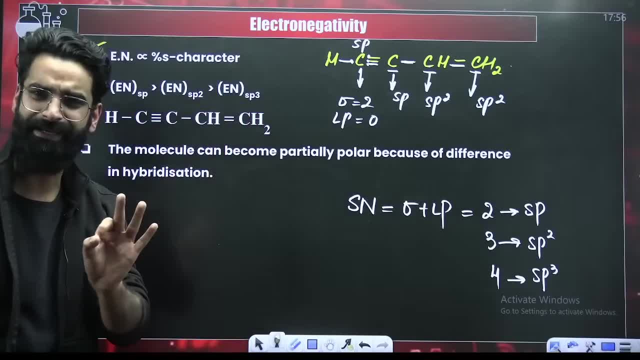 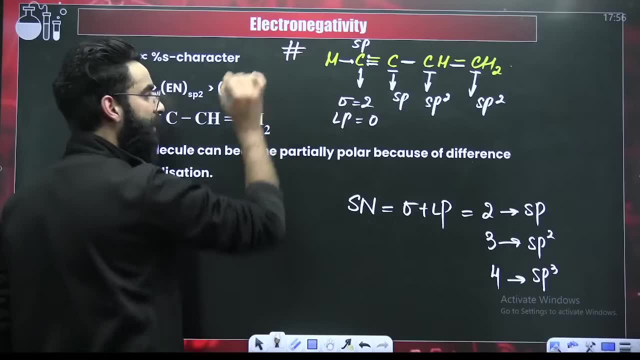 will understand how to calculate the lone pairs. okay, one example I will take. one example I will take. then I will come to this particular case which I have drawn over here. I am keeping this case on halt. one simple example I will take which will make you clear. 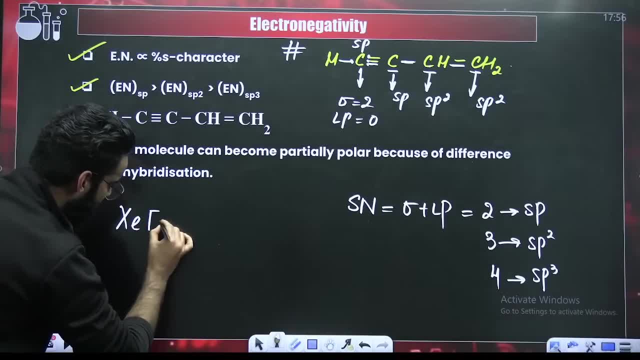 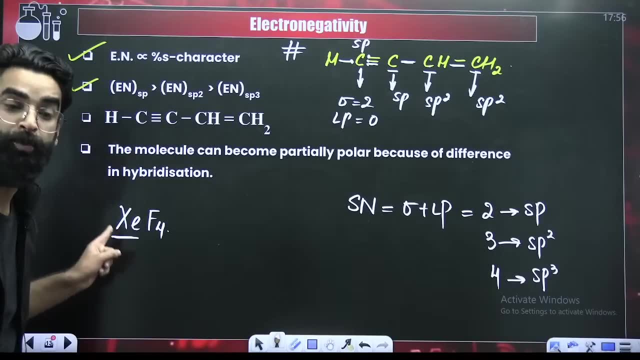 every single thing. see, for example, if you have got the molecule XCF4, if you have got the molecule XCF4, if I particularly talk about xenon, xenon is a noble gas, right? if it is a noble gas right in its outermost shell, how many electrons will be there? 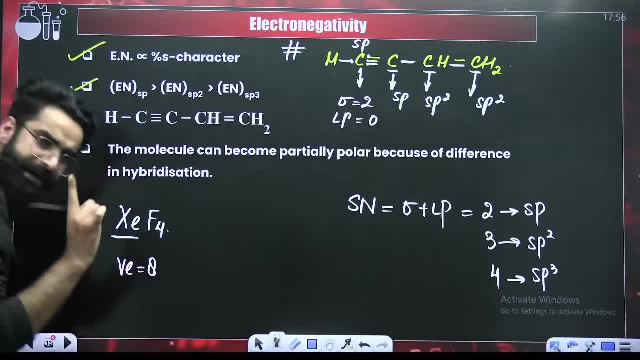 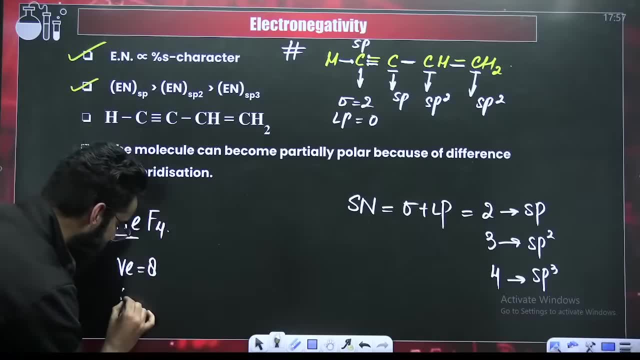 Eight valence electrons. so xenon has got eight valence electrons. okay, tell me how many surrounding atoms it has. it has four surrounding atoms. the number of surrounding atoms is equal to zero. The number of surrounding atoms is equal to the number of sigma bonds. the number of surrounding 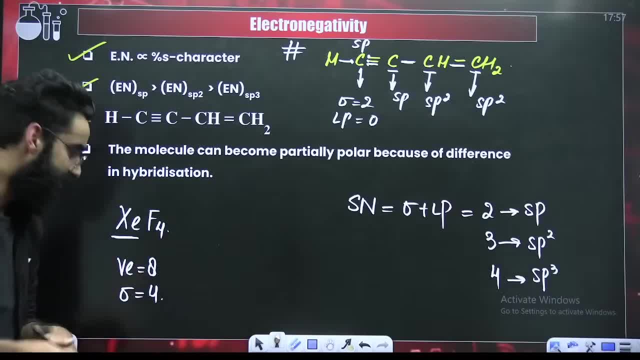 atoms is equal to the number of sigma bonds. now you tell me xenon had eight valence electrons and it is forming how many bonds? four bonds so out of eight valence electrons. can I say xenon has utilized four of its valence electrons to form four bonds out of eight valence electrons. 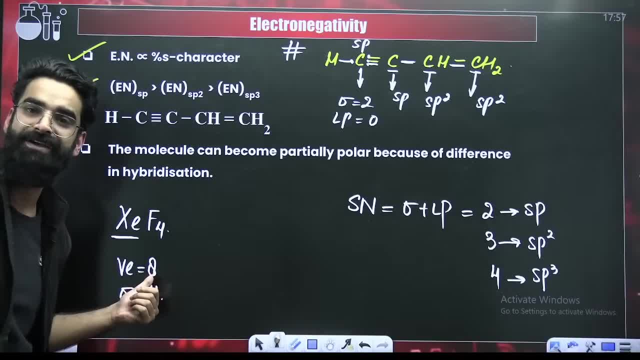 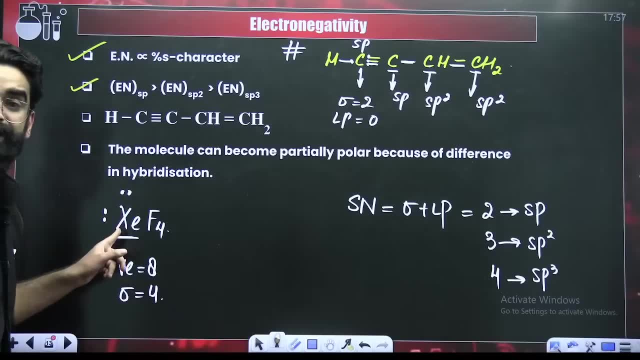 xenon has utilized four of its valence electrons to form four bonds. so how many valence electrons will be still there? There will be four valence electrons left on xenon. There will be four valence electrons left on xenon as such in its outermost shell. so 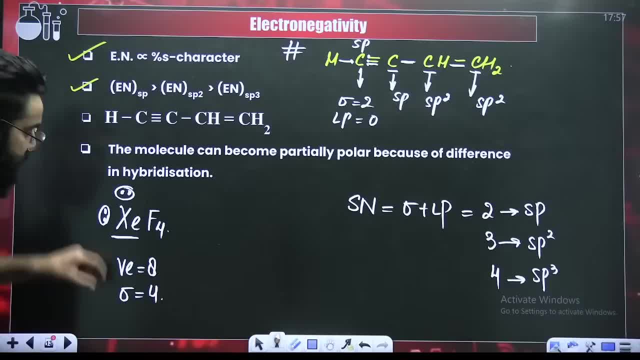 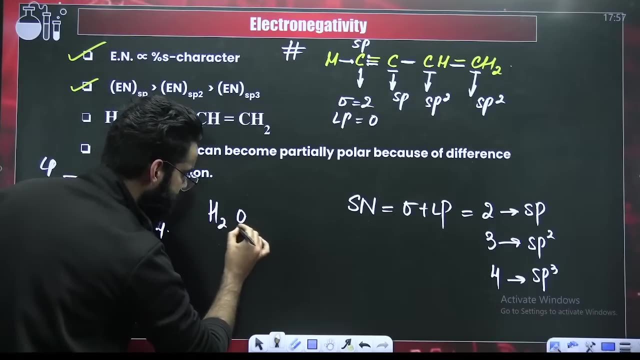 these valence electrons. they have not participated in the bonding and you will be calling these as the lone pairs. so xenon has how many lone pairs? xenon has two lone pairs. four electrons means two lone pairs. simple, right, for example. take the case of water, H2O, take the case. 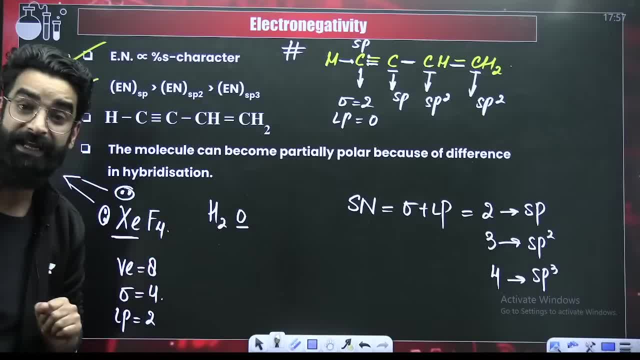 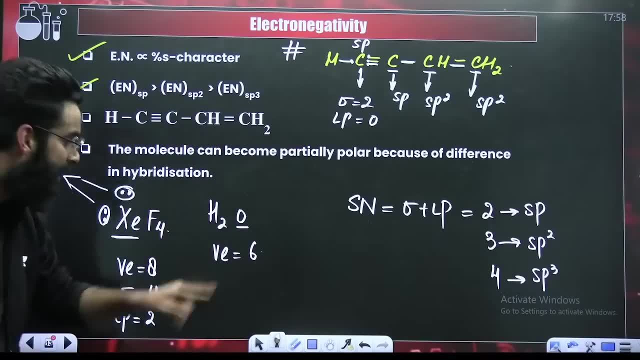 of water. if I talk about oxygen- oxygen it is a group 16 element. how many valence electrons oxygen has. How many valence electrons oxygen has? Six. How many valence electrons oxygen has Six? There are six valence electrons with oxygen. 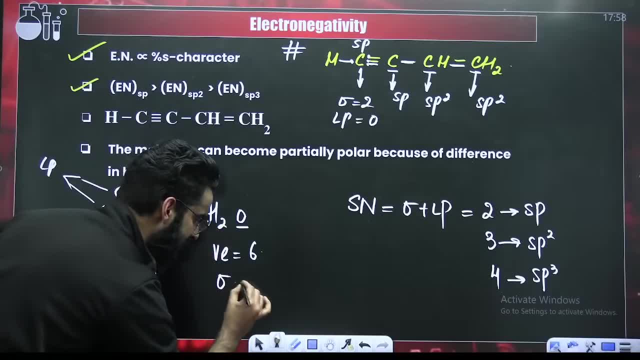 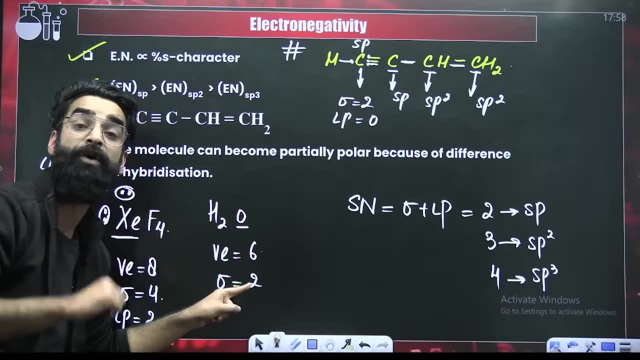 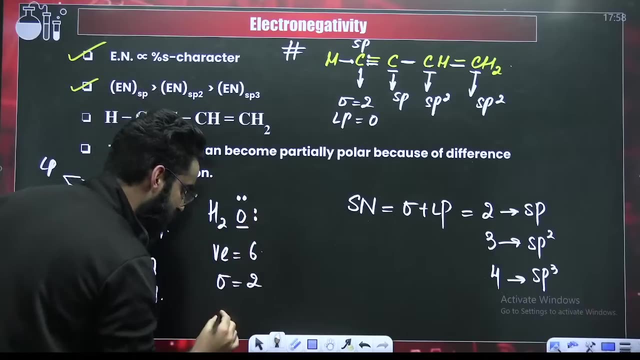 How many surrounding atoms? are there Two surrounding atoms? The number of surrounding atoms is equal to the number of sigma bonds. right? so out of six valence electrons, it has used two valence electrons to form two sigma bonds. so how many electrons will be left on oxygen as such? I will say four. four electrons means how? 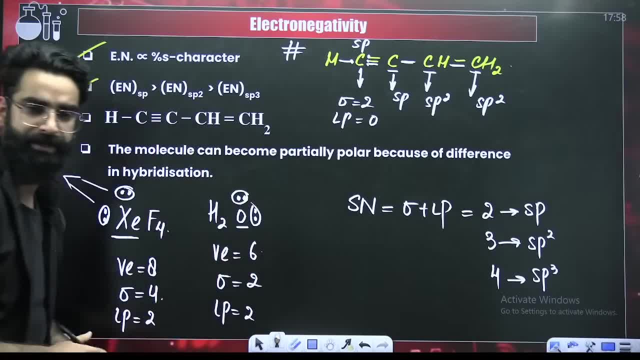 many lone pairs. I will say two lone pairs. this is one lone pair, this is one more lone pair. correct, simple and basic. simple and basic. For example, you have got NH4 positive, you have got H2O positive. 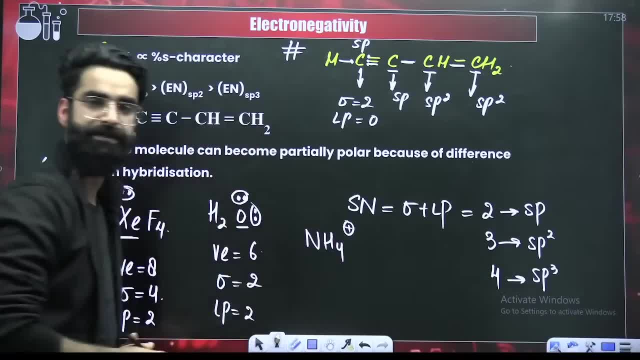 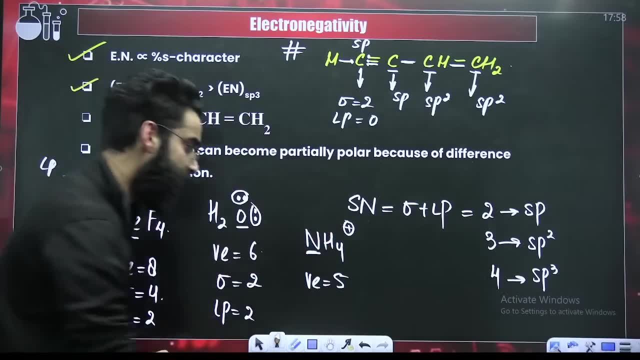 You have got NH4 positive. this is the last example which I am showing here. NH4 positive. Look at this nitrogen. how many valence electrons it has five. but there is a positive charge If there is a positive subtract, this positive, so the value comes out to be four. 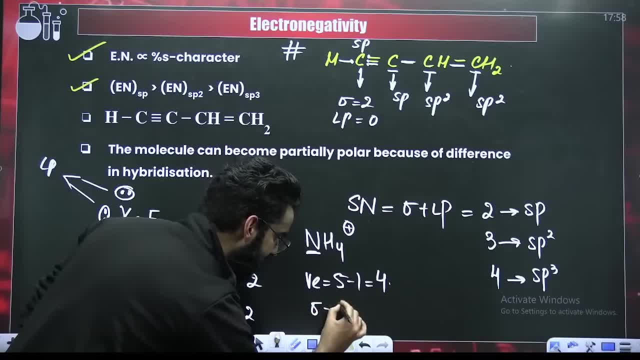 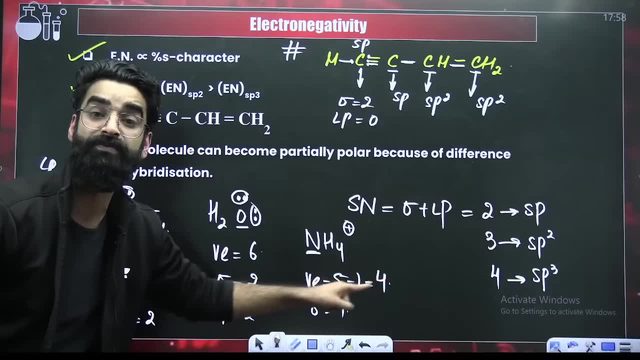 How many surrounding atoms are there? Four surrounding atoms. the number of surrounding atoms is equal to the number of sigma. It had four valence electrons and it has used all these four valence electrons to form four bonds. so how many lone pairs will be there? 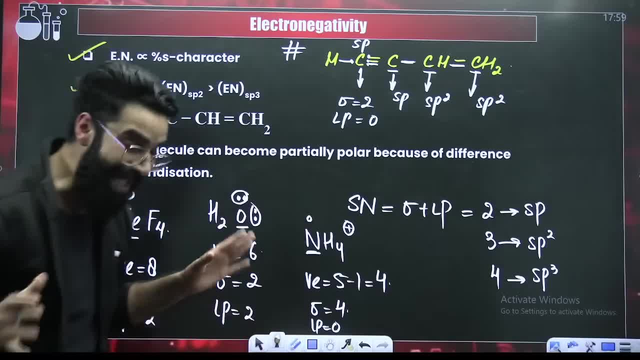 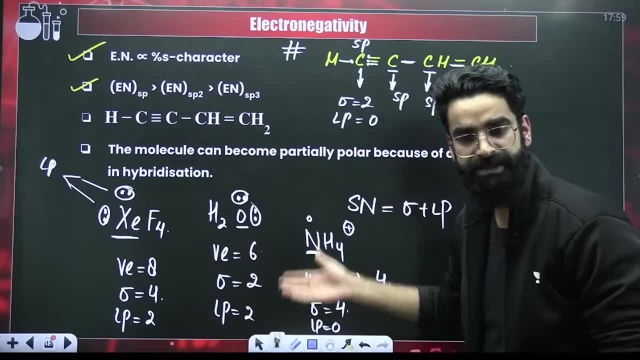 No, There is no nitrogen. perfect, I believe. if you got to know how to calculate sigma, how to calculate lone pairs, you can calculate the steric number, which is sigma plus lone pair, sigma plus lone pair, sigma plus lone pair. and once you get the steric number you can easily talk about the hybridization. 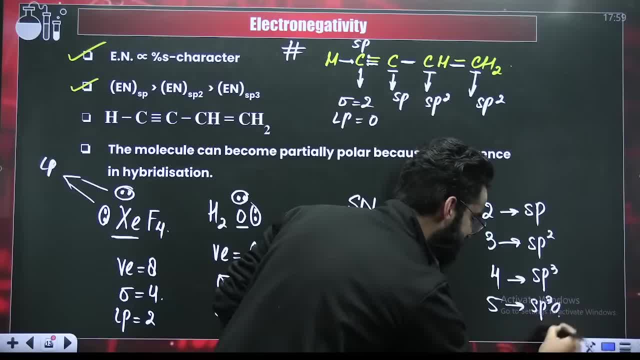 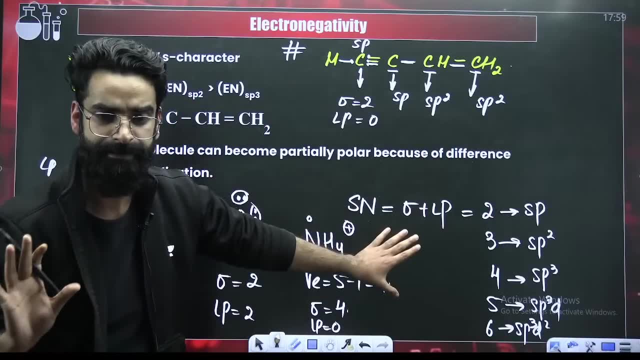 If the steric number is five, hybridization is sp3d. if the steric number is six, hybridization is sp3d2, right and so on. perfect. I believe this basic thing is clear right Now. people try to understand. 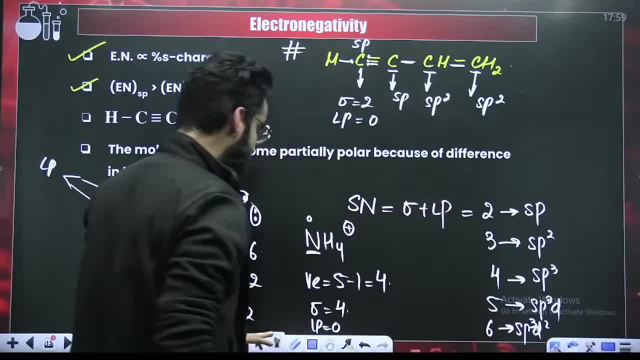 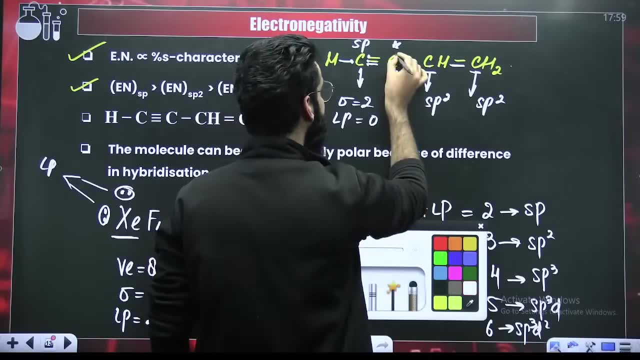 Try to understand one thing. I gave you one particular molecule over here. If you look at this particular carbon, it is sp hybridized. This particular carbon is sp2 hybridized. Let me just show you these two carbon atoms which I am going to take into consideration. 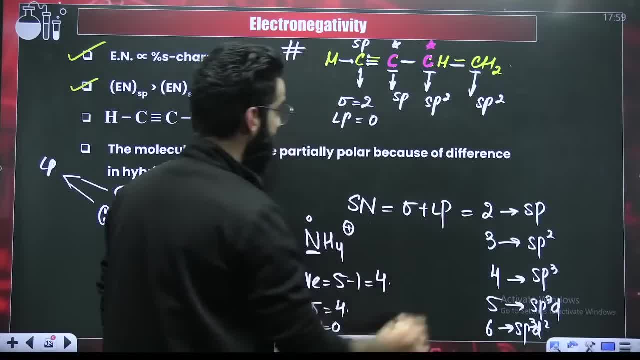 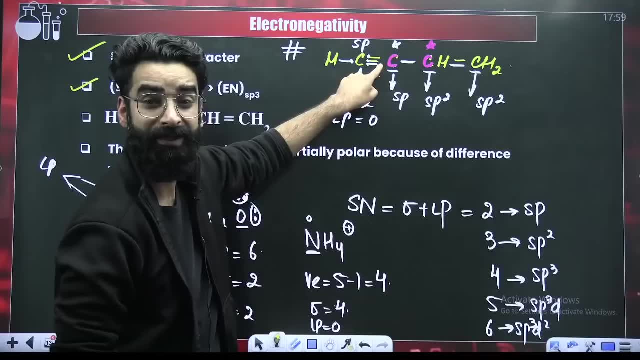 These are the two carbon atoms which I have taken into consideration. One is sp, one is sp2.. If this is sp hybridized, can I say, its s character will be more. If its s character is more, that means its electronegativity will be more. 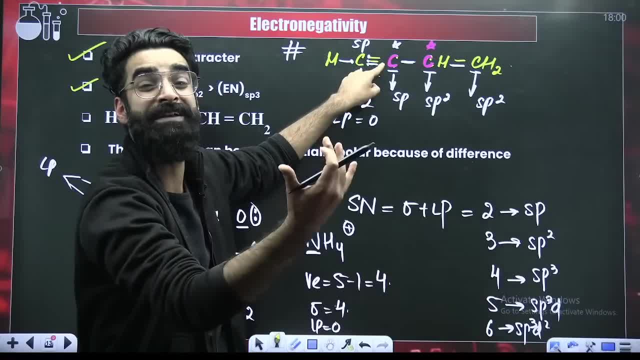 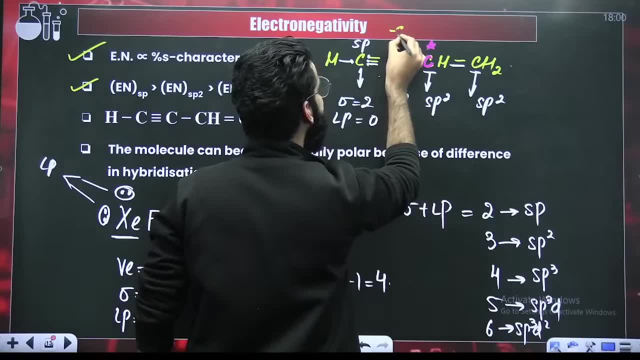 If its electronegativity is more, then its sp2 will be more. If its sp2 is more, then its sp2 will be more. That means it has got more tendency to attract the bonded pair towards itself. So this particular bonded pair will be attracted towards this carbon, due to which it gets delta. 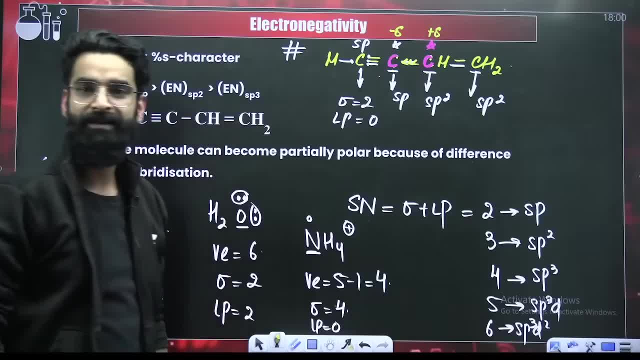 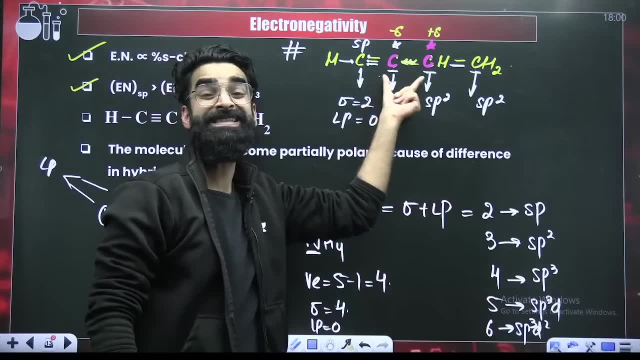 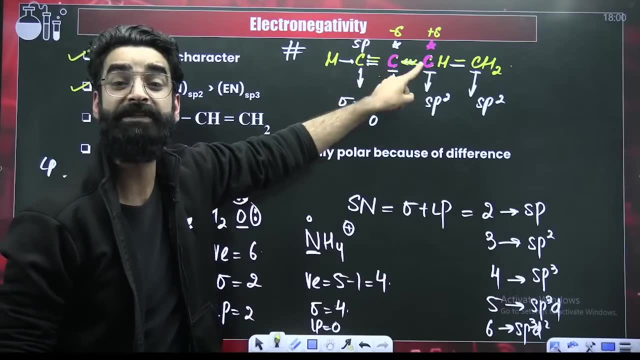 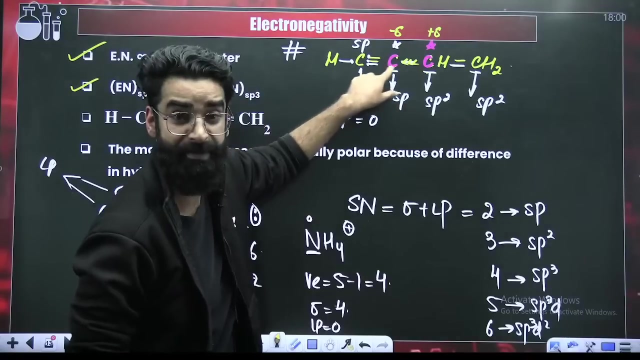 negative and this particular carbon gets delta positive. Right, Right people. So what happened? Due to the difference in hybridization, due to the difference in the hybridization, can you say, a partial polar character got developed here. Right, Can I say? due to the difference in hybridization, a polar character got generated over here. 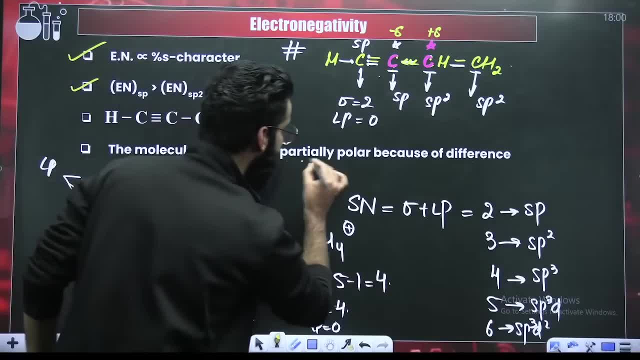 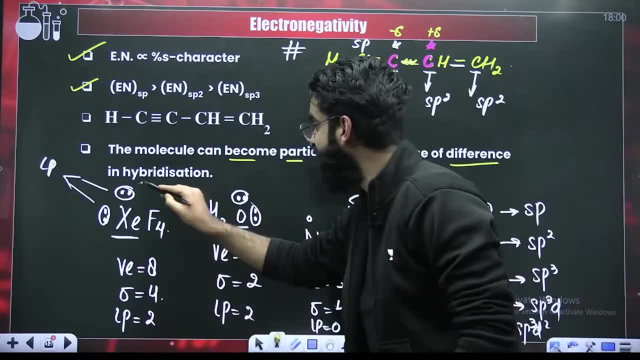 That is the point which I have mentioned over here: The molecule can become partially polar. The molecule can become partially polar Because of what? Because of the difference in the hybridization. Is this statement clear? Is this statement clear? Is this statement clear? 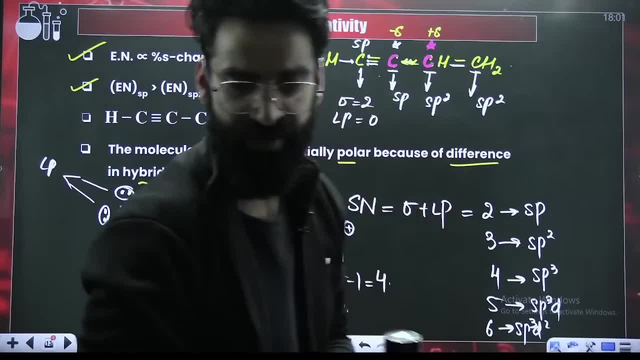 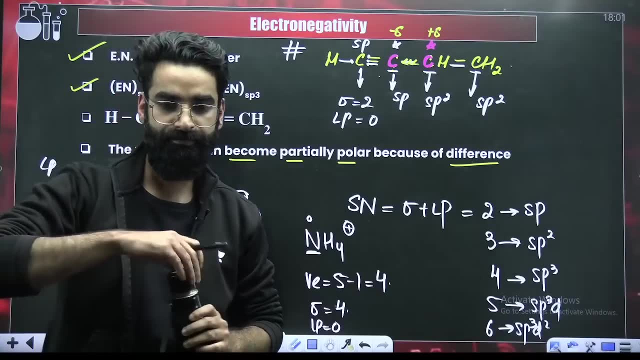 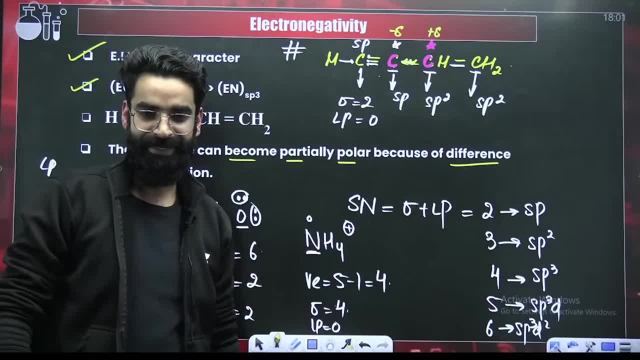 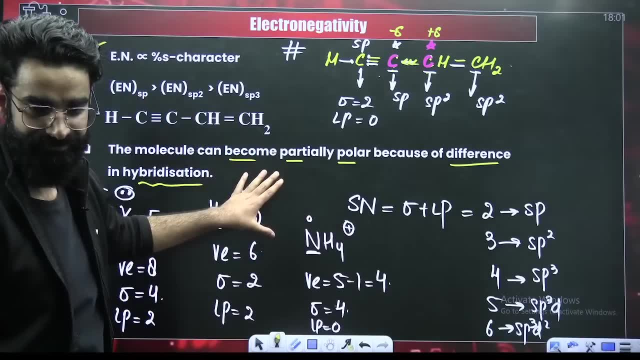 I am happy with the work which I do. Yeah, That is the reason why you guys are here. Quickly, people, Is it clear? I think this particular slide will be absolutely clear to you. Electro-negativity is directly proportional to S-character. 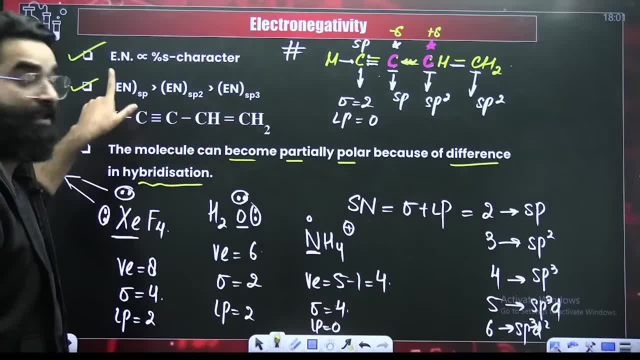 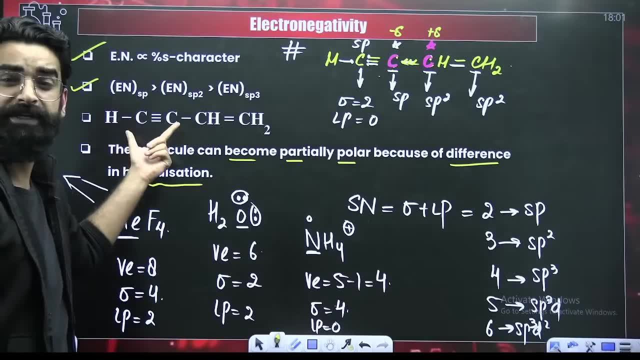 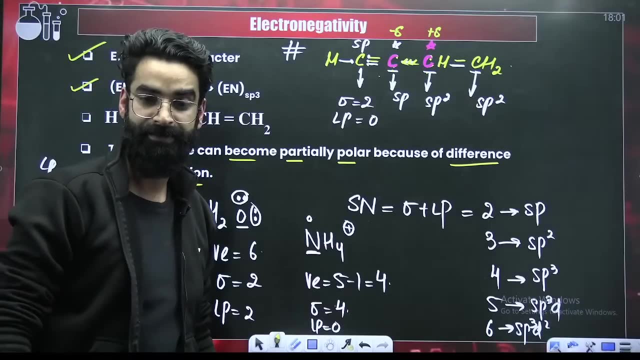 S-character is directly proportional to bond angle. Remember that S-P hybrid orbital, Its electro-negativity is more than that of S-P2.. Than that of S-P3.. One more point, Number three. Due to the difference in hybridization, a partial polar character gets developed in 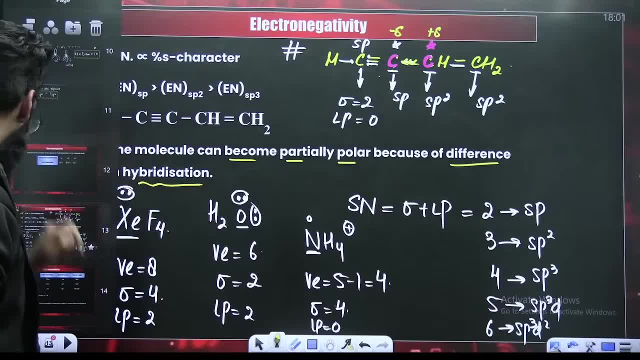 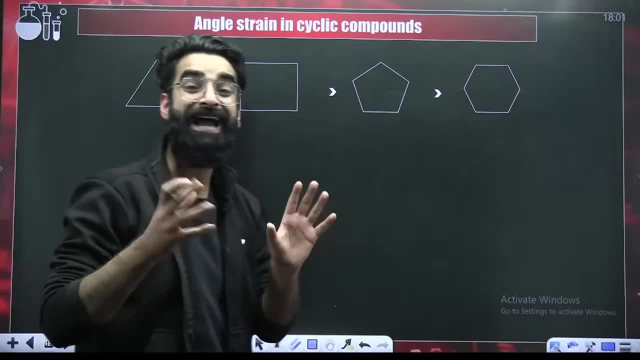 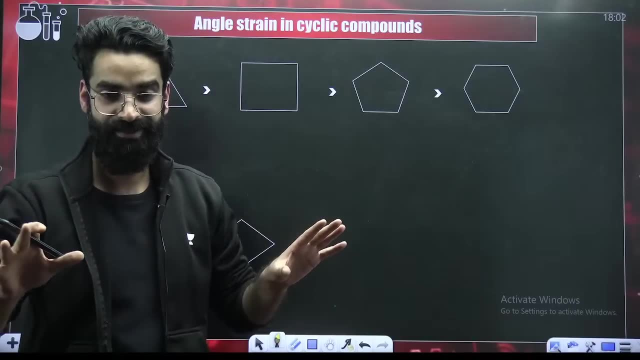 a molecule. Now, guys, Now comes one more important thing. Now comes one more important thing. Have you heard about something called as Angle strain? These are some points, guys, are some points which we are frequently going to use. these are some points which. 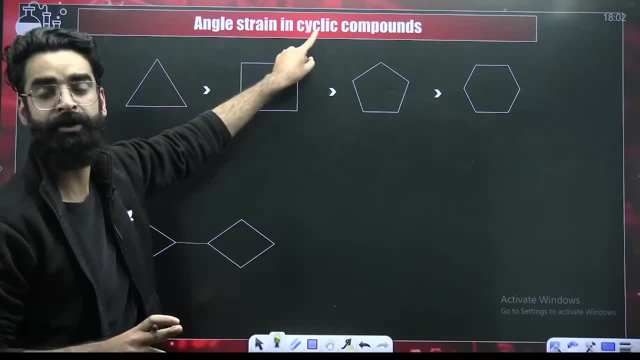 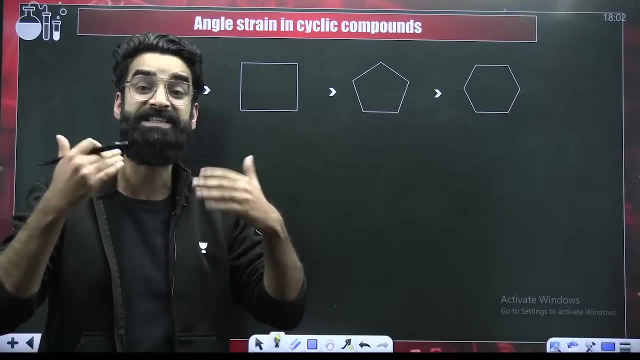 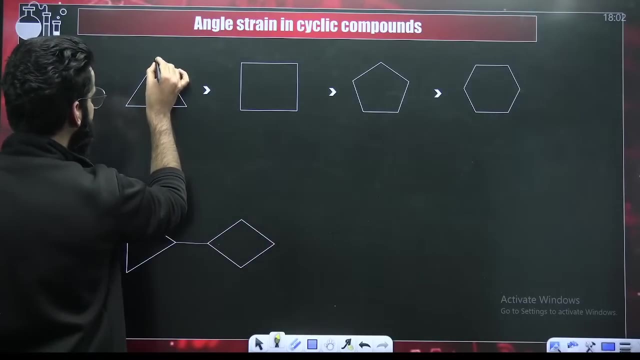 we are frequently going to use. try to understand. there's a term which I mentioned over here: angle strain, angle strain in cyclic compounds, angle strain in cyclic compounds. what is meant by it and why do I need it? try to understand if you look at this particular carbon, if you look at this particular carbon, right. 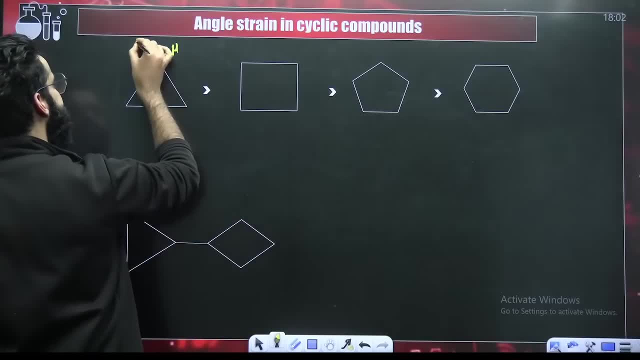 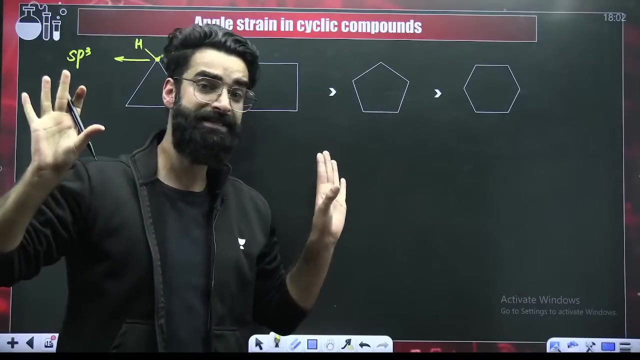 there'll be some two hydrogens which will be associated with it. perfect, right. carbon has to form four bonds: one, two, three, four, perfect. if I ask you what is the hybridization of this carbon, you'll directly say it's sp3, hybridized four Sigma bonds. four Sigma bonds in no lone pair. that means steric number four, sp3. 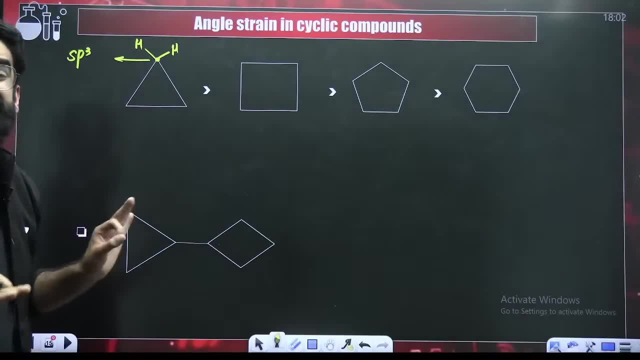 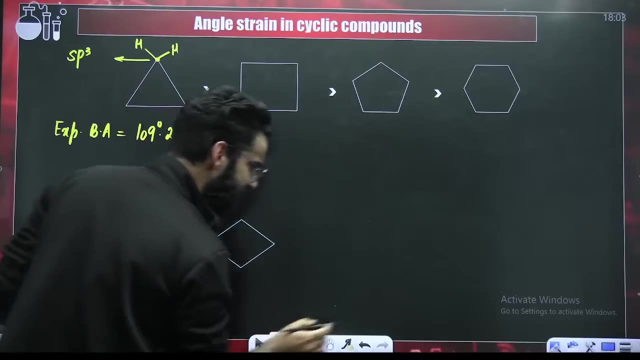 this sp3 hybridized, if this carbon is sp3 hybridized. so what is the expected bond angle here? what is the expected bond angle here? expected bond angle is 909 degree. 20 minutes is expected bond angle. but, my dear students, if I ask you, if I ask you, look at the angle between these two. 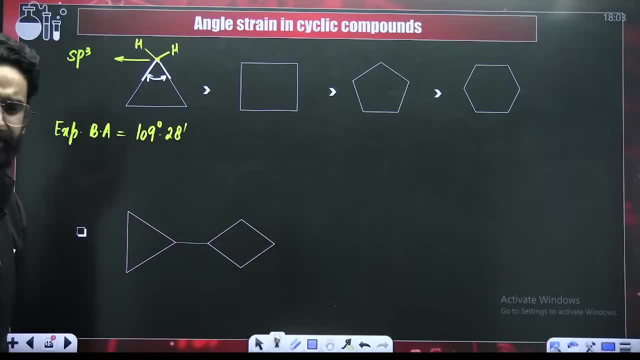 bonds. is it? is it exactly hundred 928? you'll say no, it is just 60 into just 16. if I talk about the actual warning, if I talk about the actual warning, actual warning angle: here is 60, actual warning will: here is 60. look at, 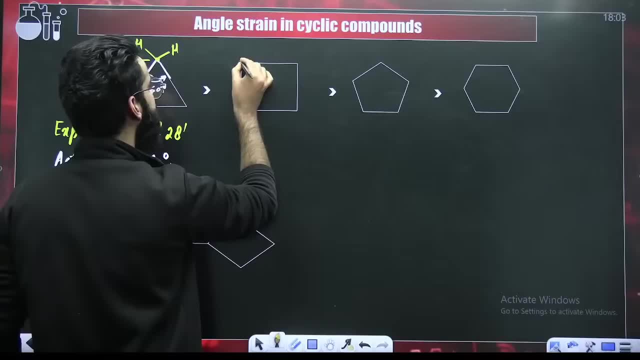 this particular molecule. look at the other molecule. look at this particular particular carbon It's forming. These are two hydrogens associated with it. Now, what about its hybridization? It's again sp3.. Perfect. What is the expected bond angle? Expected bond angle. 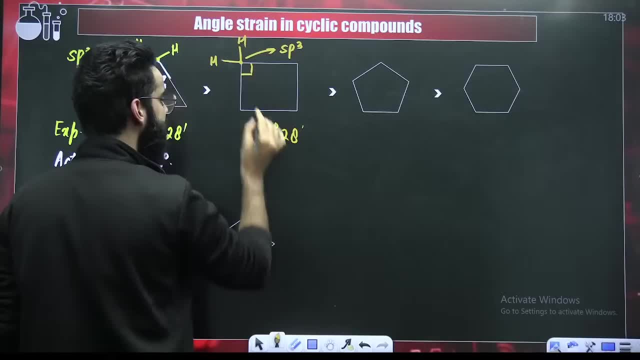 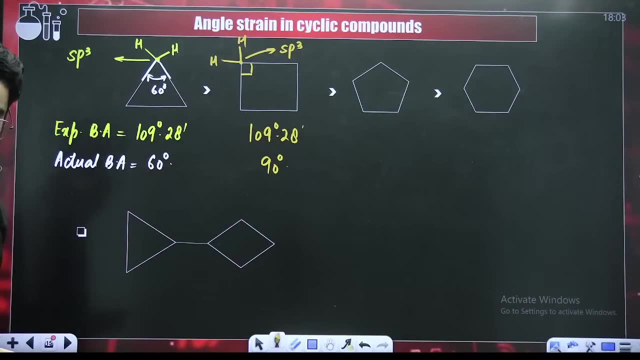 is 109 degree 28.. But what is the expected bond angle here? Expected bond, sorry. what is the actual bond angle here? Actual bond angle is 90.. Actual bond angle is 90, right, Actual bond angle is 90.. Now, my dear students, try to understand one simple thing and remember it from now on. 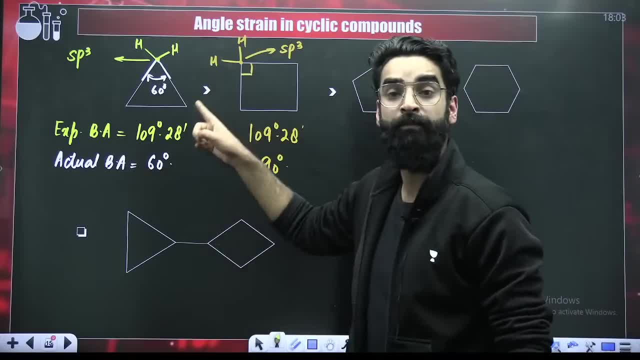 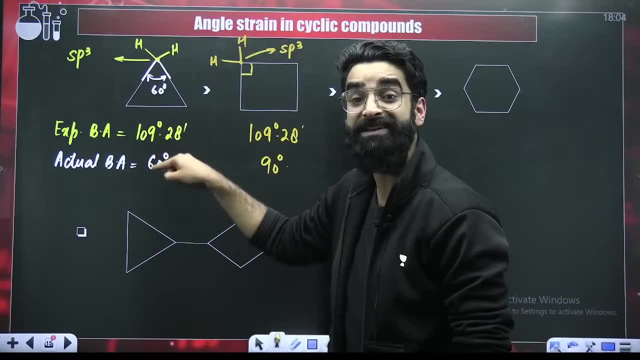 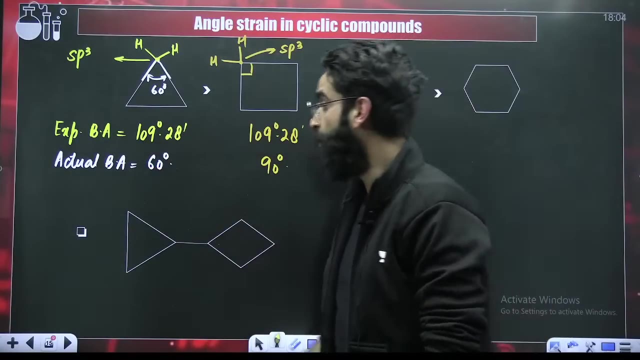 Remember it from now onwards: Whenever in a molecule the actual bond angle is not equal to the expected bond angle, Whenever in a molecule the actual bond angle is not equal to the expected bond angle, We say that molecule is under angular strain. We say that molecule is under angular. 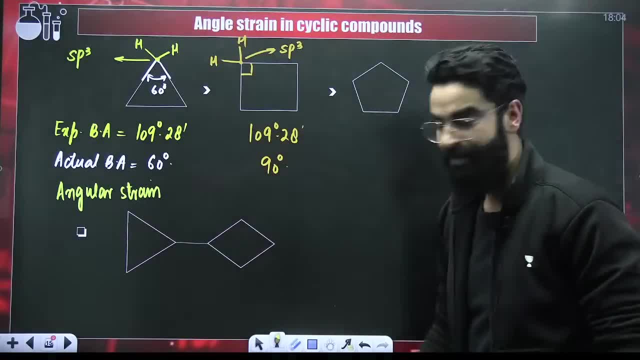 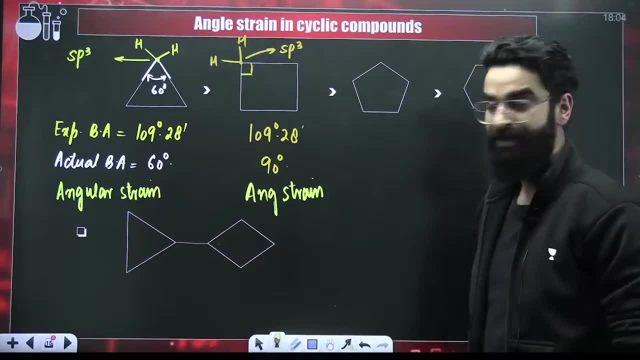 strain. So this particular molecule is under strain. Can I say: even this particular molecule is under strain. Absolutely, this particular molecule is under strain as well. This particular molecule will be also under strain, This particular molecule will be also under strain. So can I say all these? 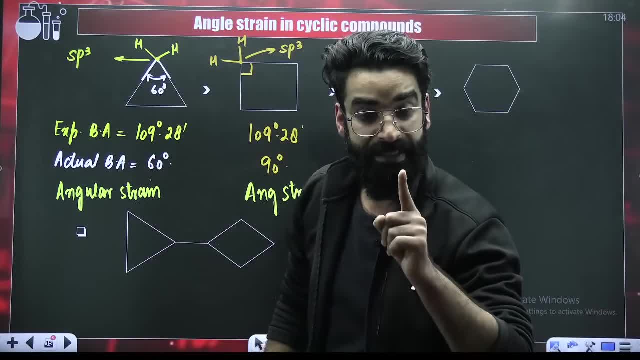 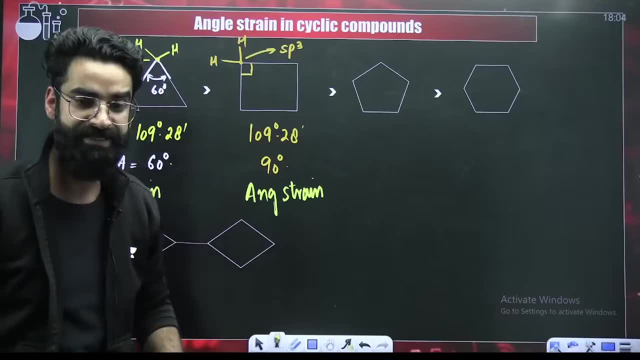 molecules here. they are under strain, Absolutely they are under strain. Now, what is the consequence of this strain? What is the consequence of this strain? Try to understand What is the consequence of this strain. What will happen due to this strain? That is important. Have a look, I'm going. 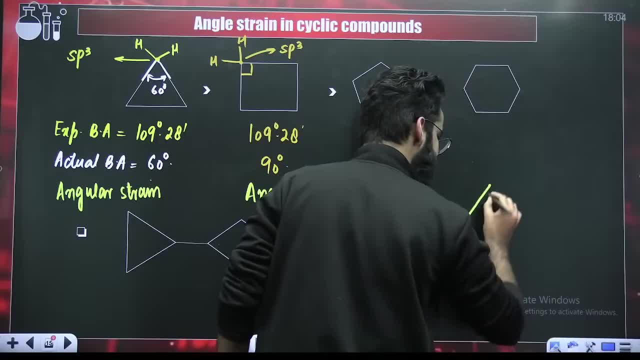 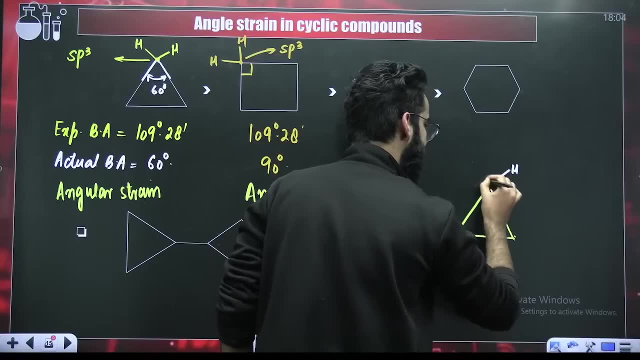 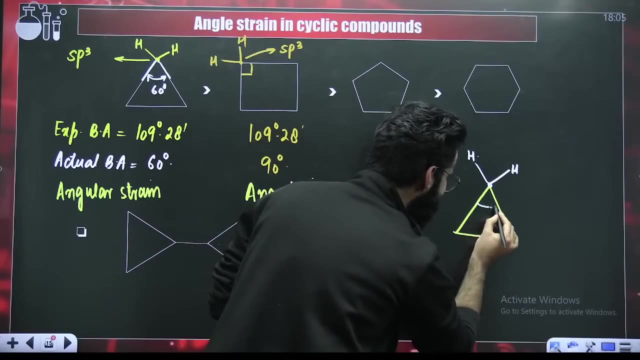 to make the first molecule over here. Now I'm going to make the first molecule over here, again Perfect. This is your molecule, which I took in the beginning, Right, And these are the two hydrogen atoms. These are the two hydrogen atoms. Now, my dear students, if I ask you, this angle should be how much? 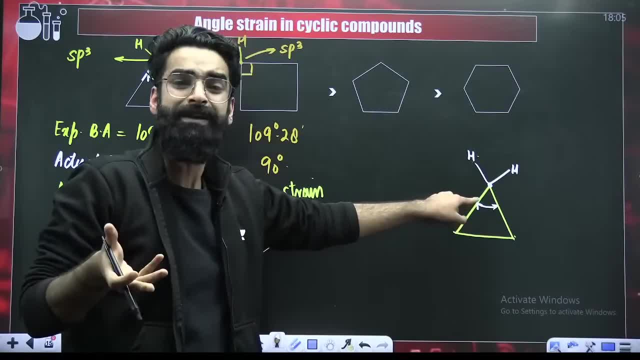 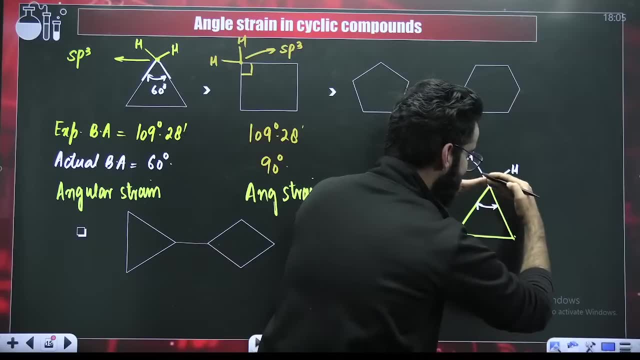 I'm using the term should be: This angle should have been 109.. This angle should have been 109.. So this particular angle, it should have been 109.. It should have been 109. But how much it is? it is less than that. If this angle has decreased, what about the outer angle? Can I say outer? 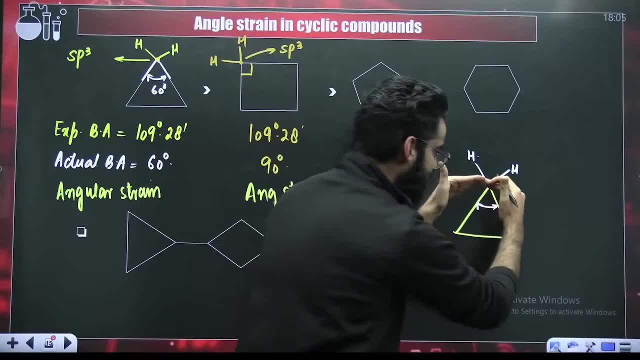 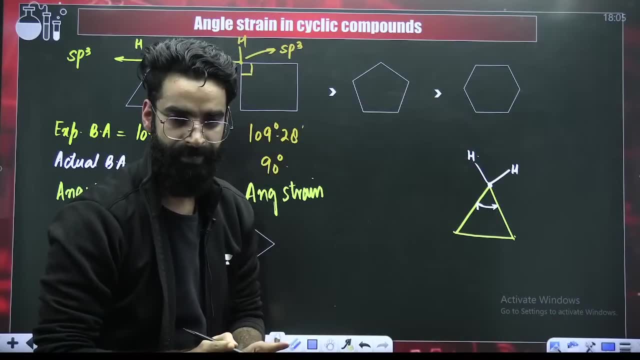 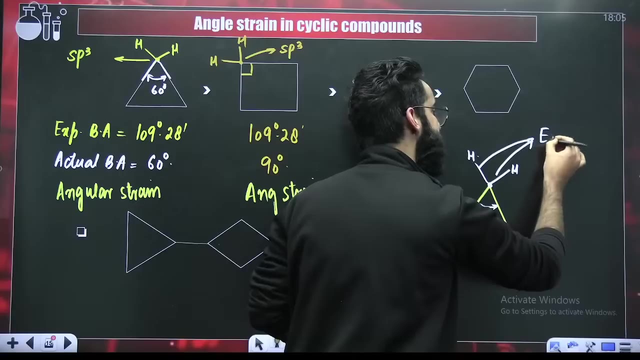 angle would have increased This angle. it should have been 109, but it's 60. So this angle has decreased. So outer angle would have increased. Yes, So if outer angle has increased before that, let me tell you these bonds over here these are called as exocyclic. 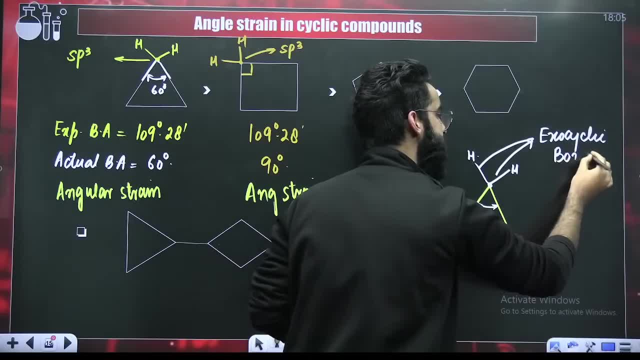 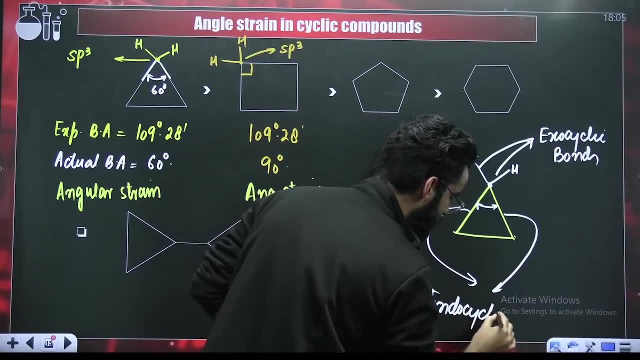 bonds, These are called as exocyclic bonds. And these particular bonds, these particular bonds, these are called as endocyclic bonds. These are called as endocyclic bonds. Now you tell me this particular bond angle should have been 109, but it's 60,, it's less than. 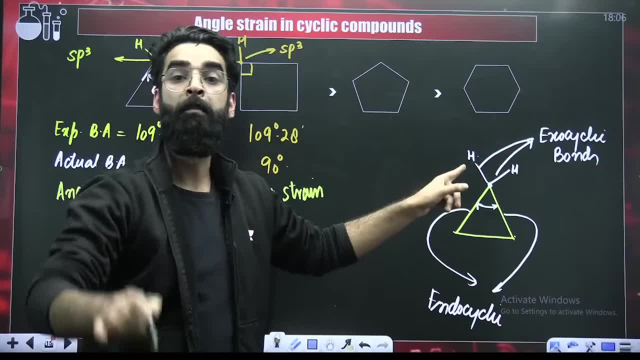 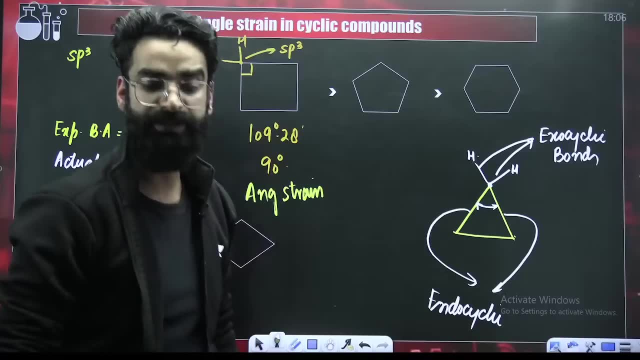 that That means the outer bond angle would have increased, And more the bond angle, more the electronegativity, More the bond angle, more the electronegativity right, More the bond angle, more the electronegativity. 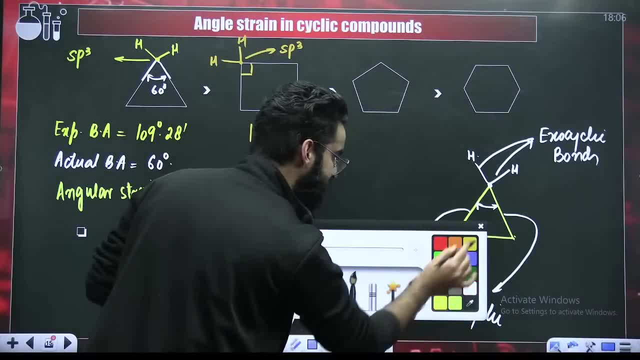 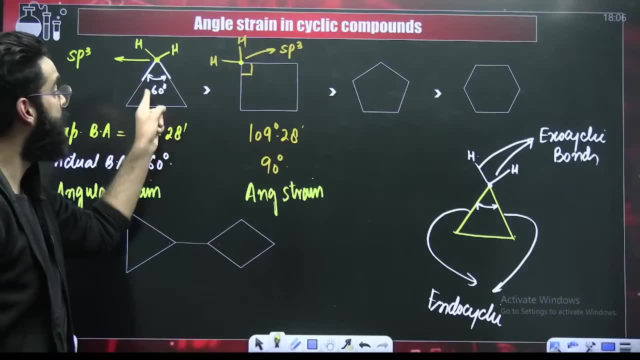 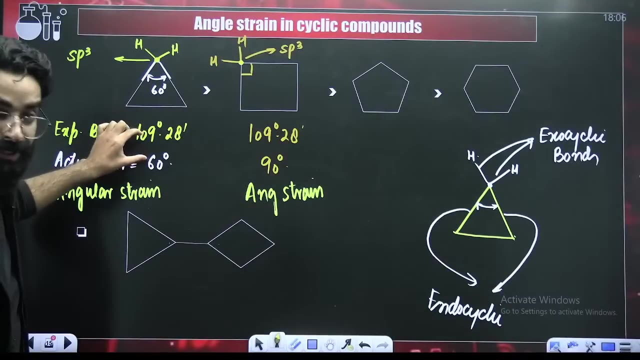 So my idea, students: just compare one thing. just compare one thing. Tell me about this particular carbon and this particular carbon. Tell me, tell me which particular molecule among these two is under more strain. Here the difference is more, Here the difference is comparatively. 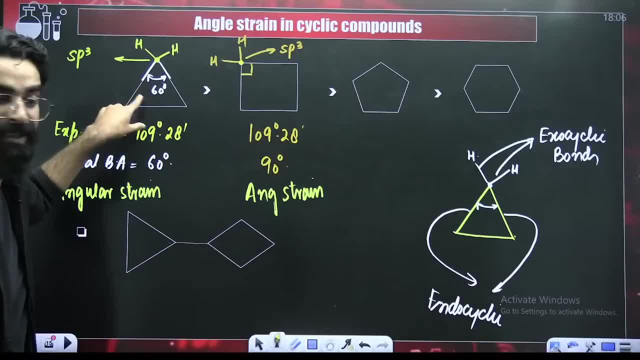 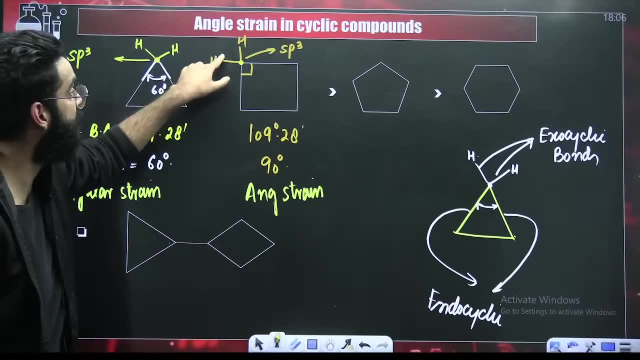 less, So this molecule is under more strain. If this is under more strain, so can I say, this particular bond angle here will be more as compared to this particular bond angle. Bond angle is directly proportional to electronegativity. So if I ask you, what about the electronegativity? 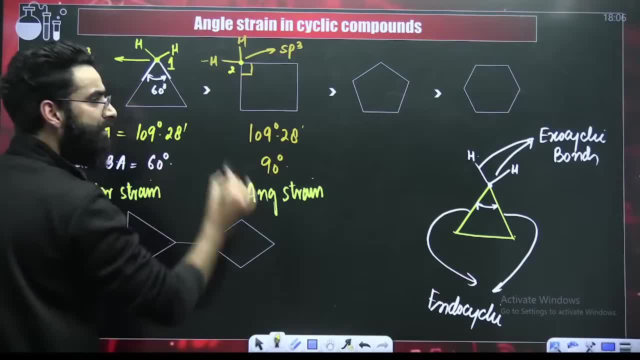 of this particular carbon, 1 and 2?? Can you tell me which carbon will be more electronegative among these two? Is it going to be 1 or 2?? Which carbon, 1 or 2, which one will be more? 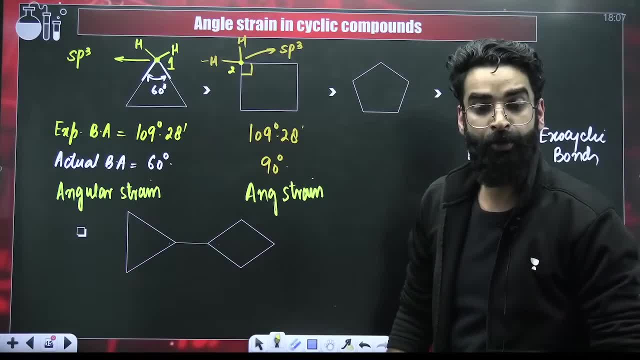 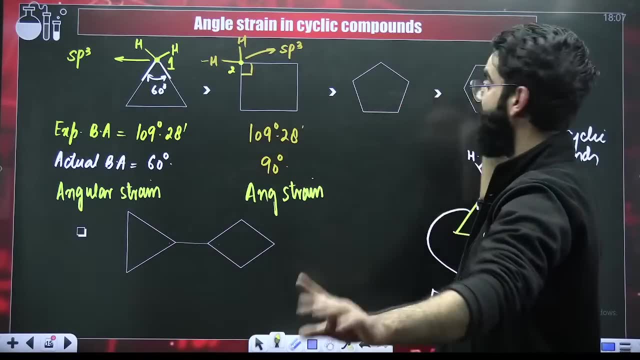 electronegative. You tell me that only. Which carbon will be more electronegative? Quickly in the charts: Absolutely, this carbon will be more electronegative than this, than this, than this. Is it clear? So, in short, what is the conclusion here? What is the conclusion here? Conclusion is: 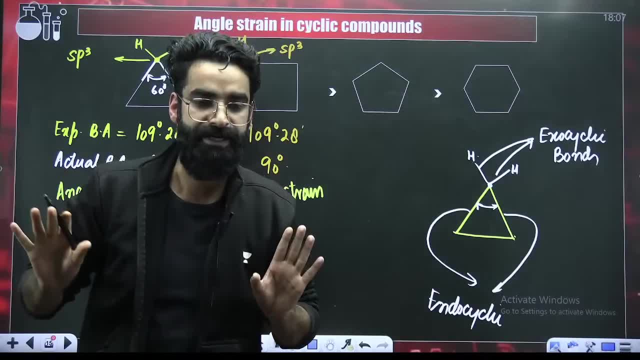 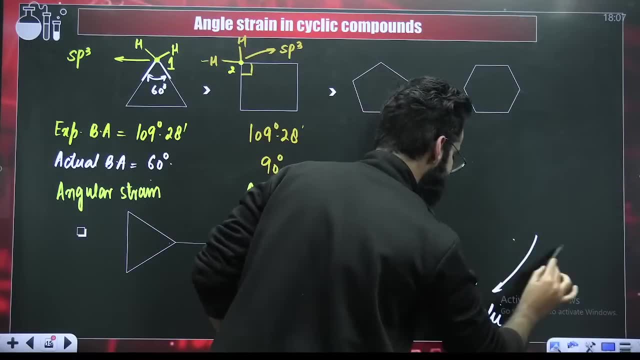 very much simple: More the angle strain, more the electronegativity. More the angle strain, more the electronegativity. I believe this particular statement is clear: More the angle strain, more the electronegativity. So I can, I can write a simple statement. Do you remember? 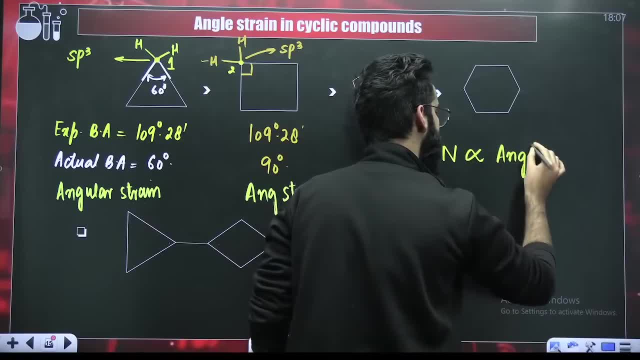 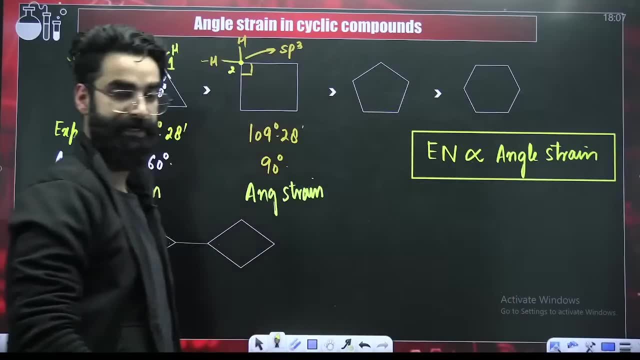 this Electronegativity is directly proportional to what It is directly proportional to angle strain. More the angle strain, more is going to be the electronegativity. I believe you know that completely. I believe this particular point is also clear to you. Yes, right people. 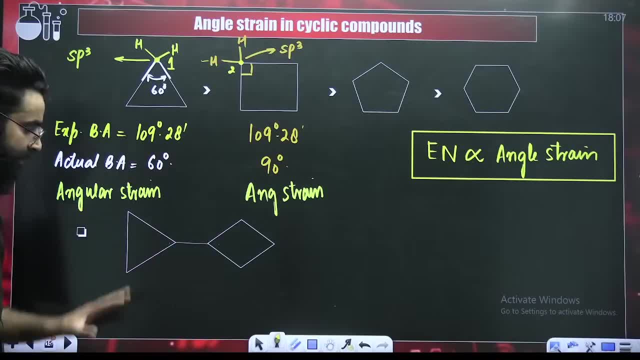 Is it clear? Okay, if it is clear, if it is clear, Over here, I have taken two rings. This is a three membered ring, this is a four membered ring and I have joined them. I have joined them. Right, my dear students, if you look at this particular carbon which I'm calling as carbon, 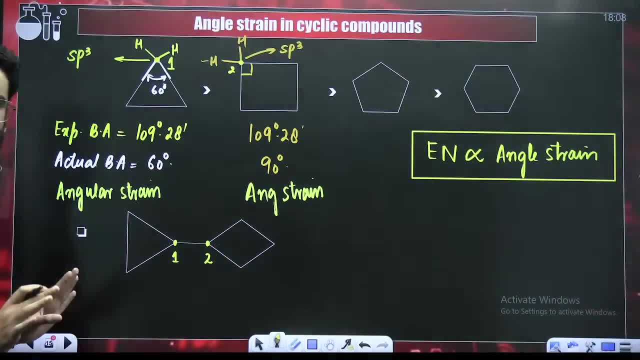 1, for example. I'm calling this carbon as carbon 2, for example. okay, Now, among these two rings, can you let me know which ring is correct? Our answer can be: which Cross雨 under more strain? three-membered ring: it is under more strain than that of four-membered. 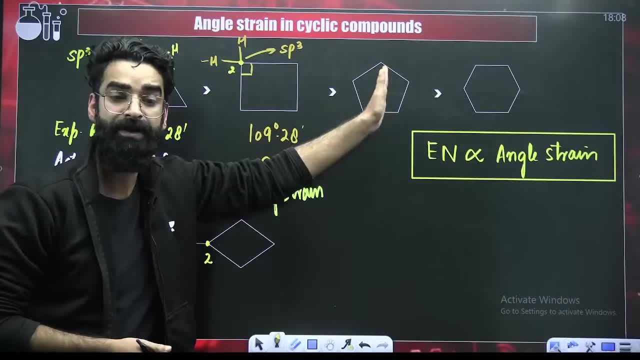 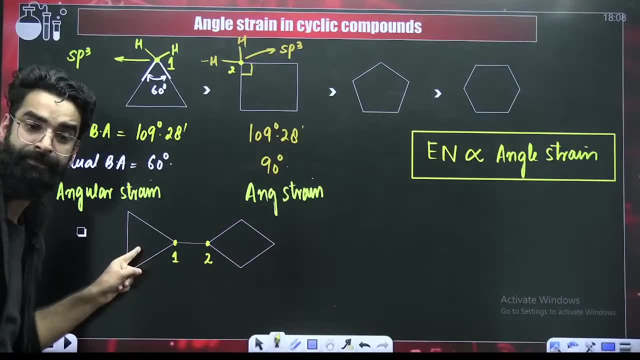 ring, Four-membered ring is under more strain than that of five-membered, than that of six-membered. So can I say, can I say this particular ring is under more angular strain. If this ring is under more angular strain, more the strain, more the electronegativity, So can I say electronegativity. 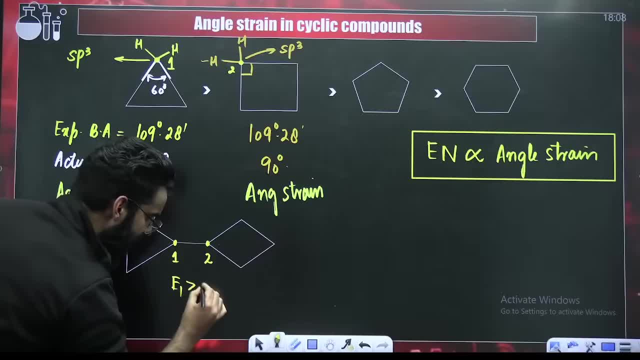 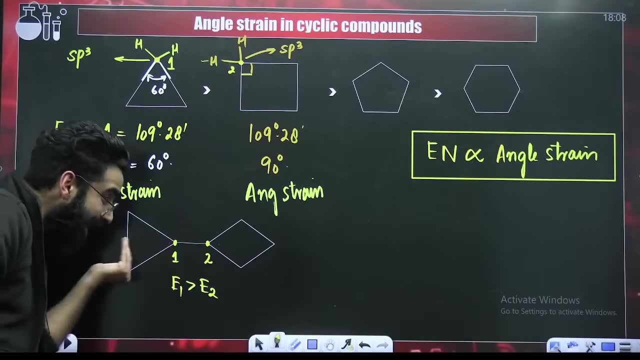 of this particular carbon. electronegativity of this particular carbon will be more than that of this. Okay, If electronegativity of this carbon is more so, it has got more tendency to attract the bonded pair towards itself. So I'll say, if it has got more tendency to attract the bonded, 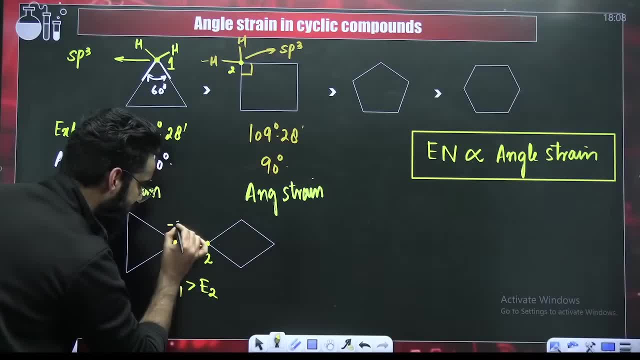 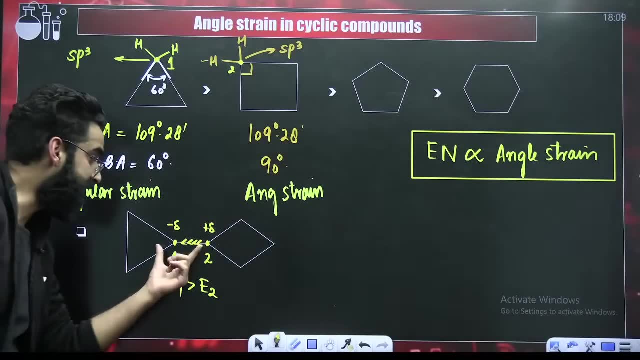 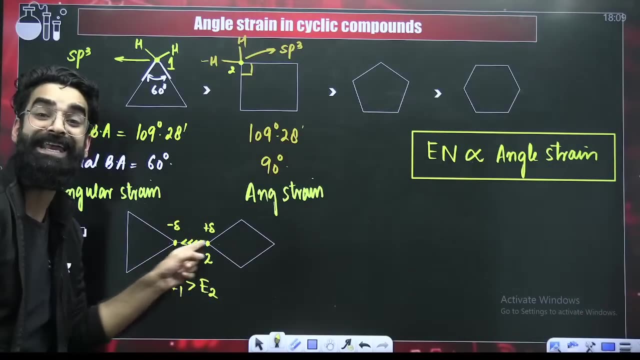 pair towards itself. that is the reason why this carbon will get delta negative. this carbon will get delta positive. Agreed, Now tell me one thing, Can I say: due to the difference in the angular strains, due to the difference in the angular strains, again, partial polar character got. 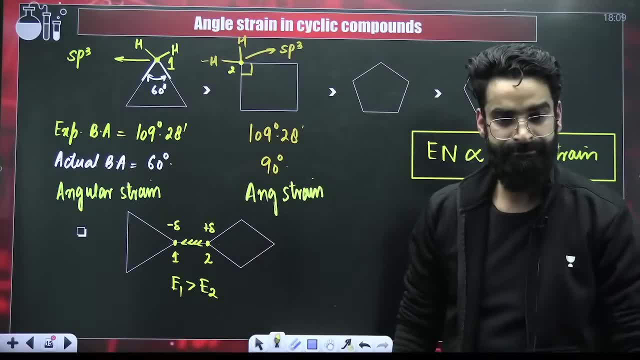 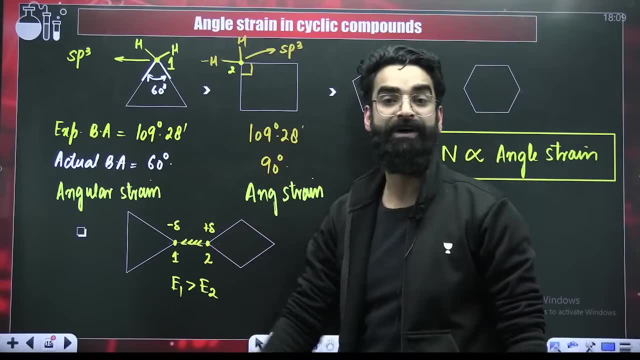 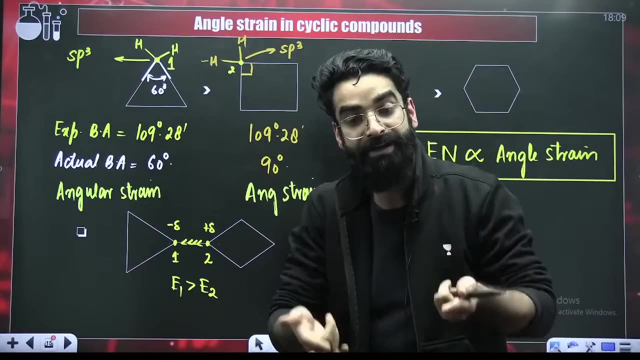 developed in the molecule. Yes, Can I say due to the difference in the angular strains. again I would say partial polar character got developed in this molecule. So do remember one thing: due to the difference in the angular strains, partial polar character can get developed in the molecule. 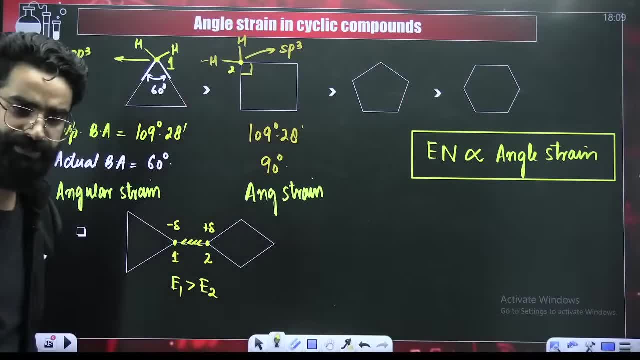 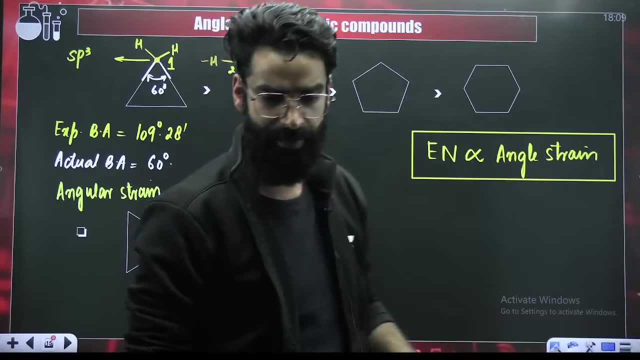 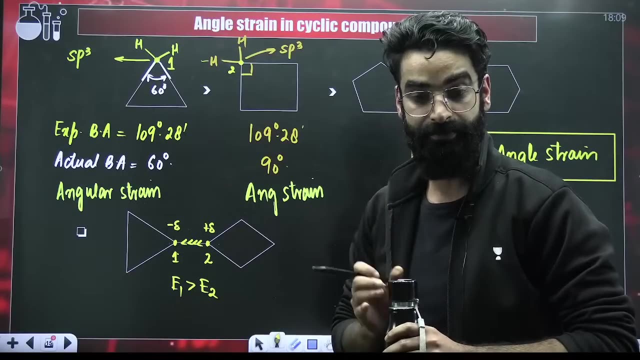 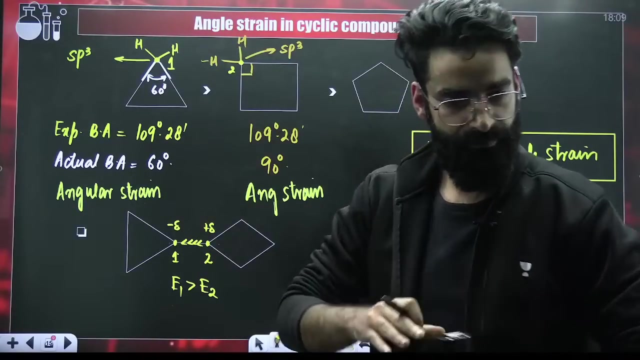 Yes or no in the chats? everyone Yes or no in the chats? everyone Yes or no in the chats? everyone Quickly. Yes or no. everyone in the chats quickly. Everyone in the chats. Guys, this is complete basics which I'm teaching you And you have to remember each and every point. Agreed, Perfect. 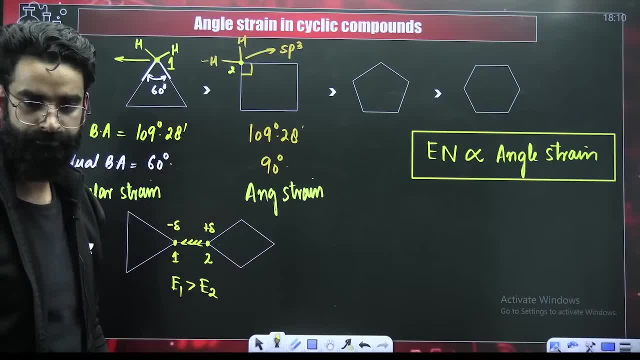 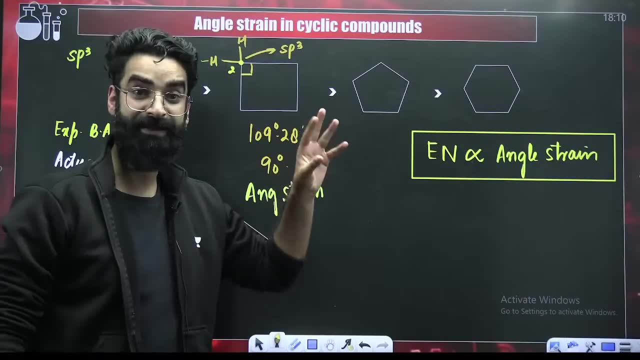 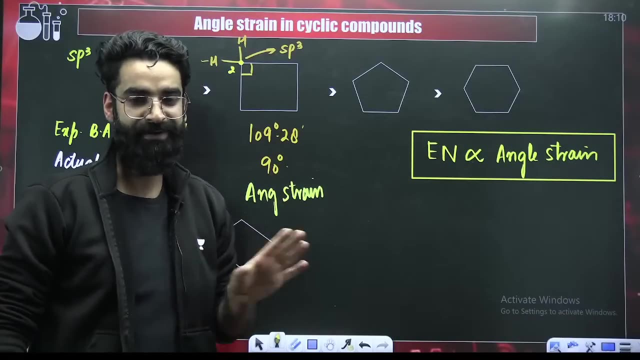 Wonderful, Wonderful guys. Now your screen will be blinking a bit because electricity is over, So maybe we might have to shift to dark mode soon, And I hope every one of you is fine with that. Yeah, we might have to shift to the dark mode soon. 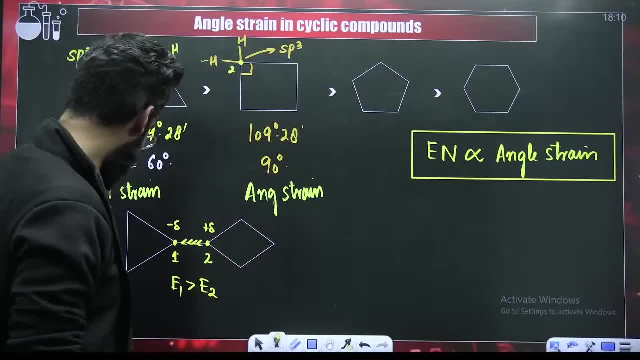 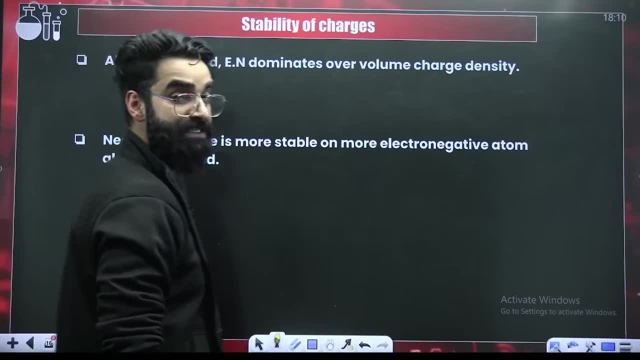 And the people who who watch my sessions regularly, they will know exactly what is dark mode. Alright. so, people, the things, the basics which I was teaching you, tell me where do we use this basics? Where do we use this basics? 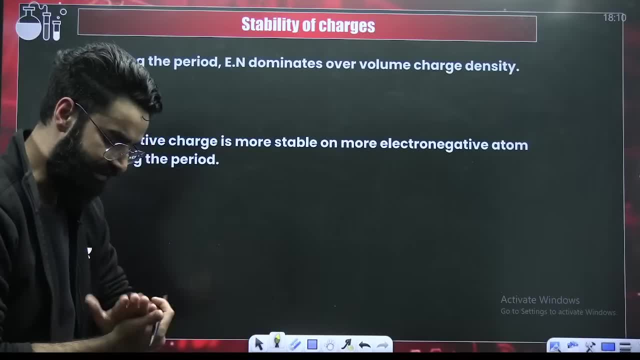 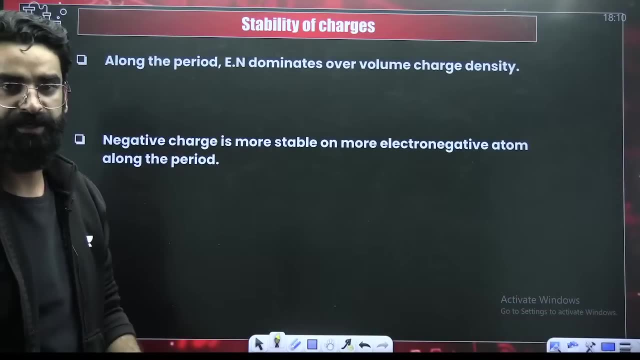 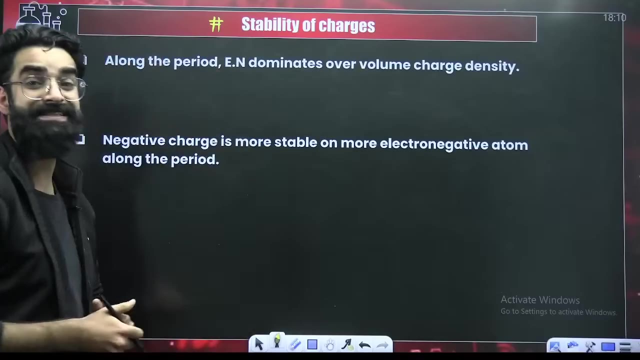 Where do we use this basics? Before utilizing all these concepts in the questions, there is one more thing which I would want to share with you, My dear students. there is a term called as stability of the charges. There is a term called as stability of the charge, For example. let's 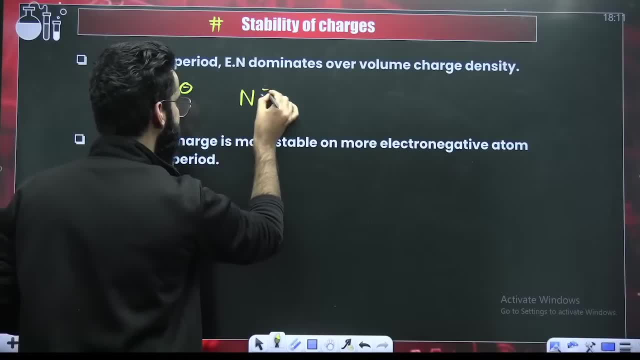 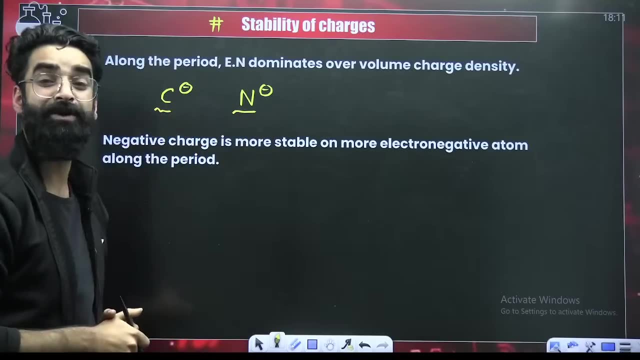 say, we have got the carbon carrying negative charge, we have got nitrogen carrying negative charge, Carbon carrying negative, nitrogen carrying negative. Tell me one thing: whether these elements, whether they belong to same period or same group, what do you think? Carbon? 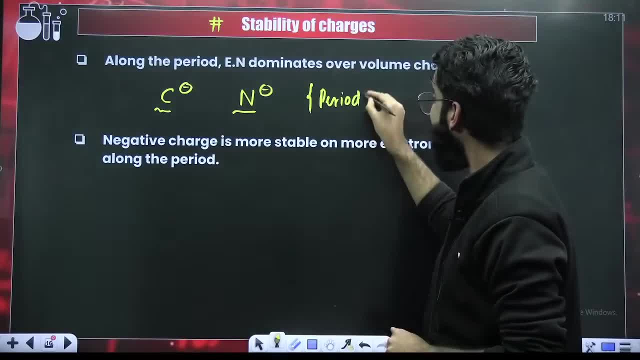 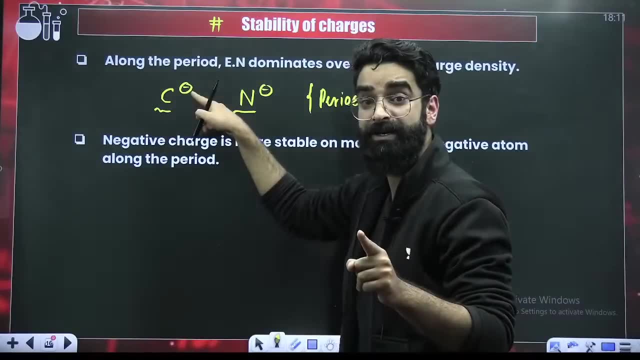 nitrogen. they belong to same period. they belong to same period, My dear students, whenever you have to compare, whenever you have to compare the stability of the charges, whenever you have to compare steeply of the charges on the elements that belong to same period. 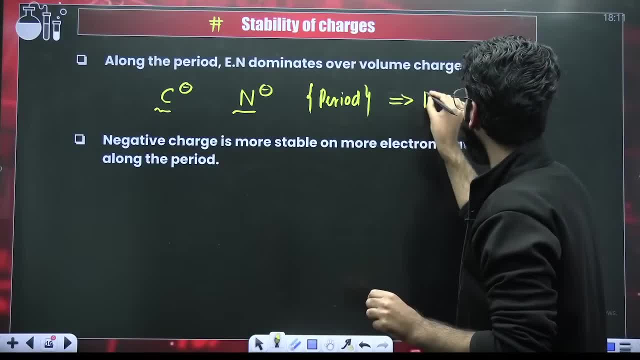 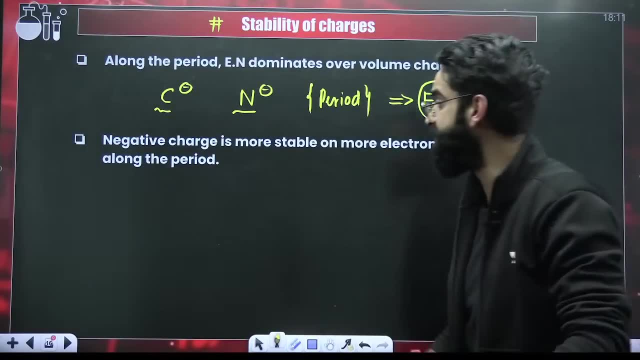 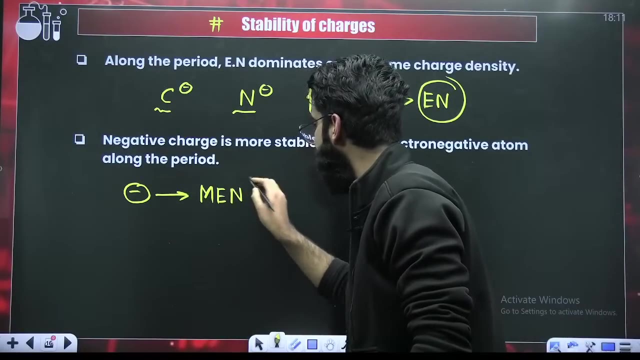 you will be giving your answer as per electron negativity. You will be giving your answer as per electron negativity, electronegativity And, as per electronegativity is concerned, negative charge is more stable on more electronegative element. Negative charge is more stable on more electronegative element. 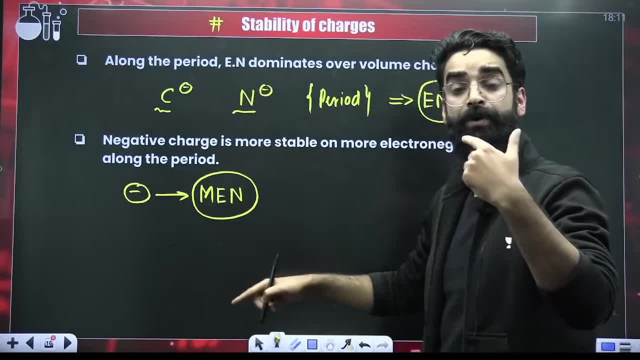 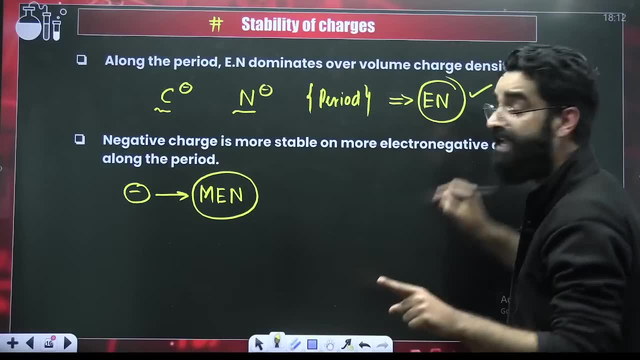 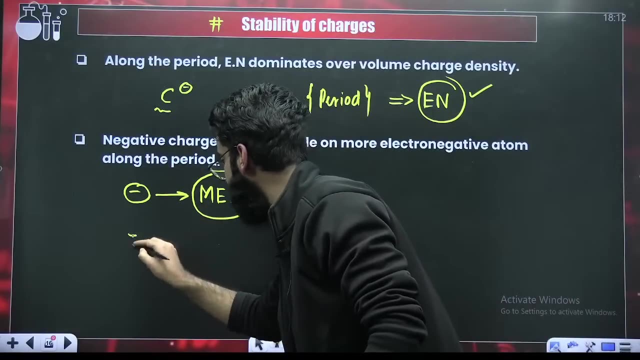 Right, Whenever you have to, whenever you have to compare the stability of the charges on the elements which belong to same period. at that time electronegativity plays a role. Negative charge is more stable on more electronegative element. Similarly, opposite of this opposite. 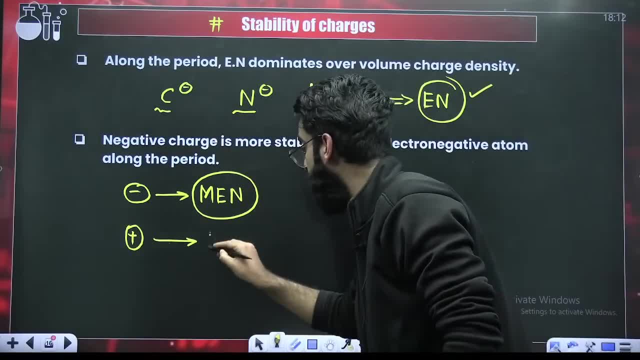 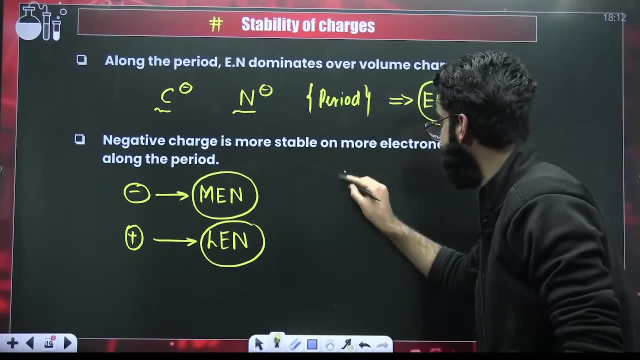 of this, positive charge will be more stable on positive charge will be more stable on less electronegative element. less electronegative element, less electronegative element. Now look at the case, for example, carbon carrying negative nitrogen carrying negative oxygen. 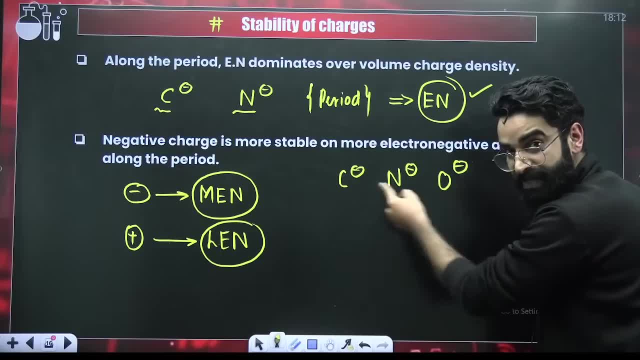 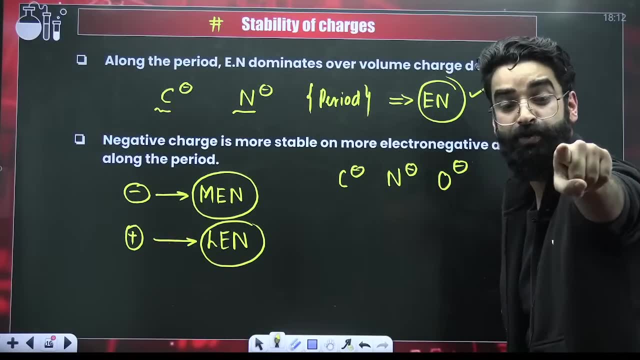 carrying negative These elements. they belong to same period. They belong to same period. And whenever you have to compare the stability of the charges on the elements which belong to same period, which concept- Electronegative Electronegativity And negative charge- is more stable on more electronegative Right, Which one? 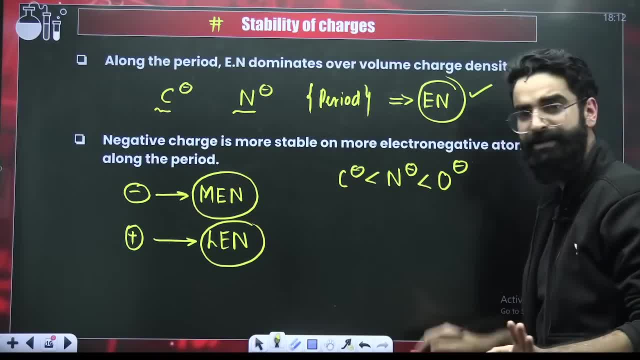 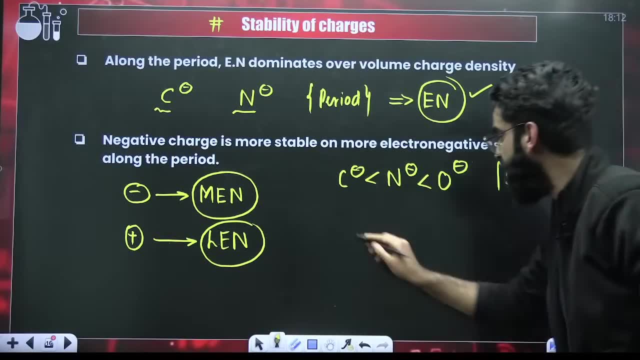 is more electronegative Oxygen, So negative charge will be maximum stable here, followed by this, followed by this, Correct, This is the stability order of the negative charges. This is the stability order of the negative charges. For example, you have got carbon carrying positive. 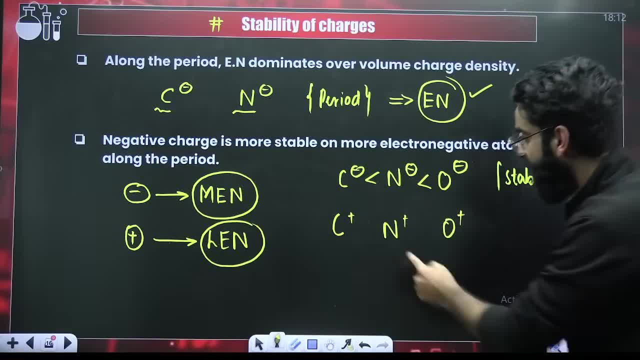 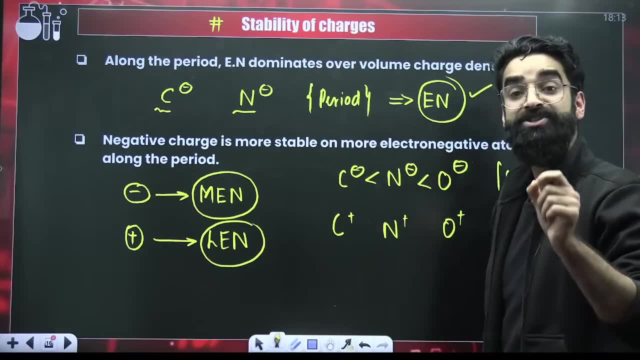 nitrogen carrying positive oxygen carrying positive. Again, have a look These elements. they belong to same period. In the period we prioritize electronegativity And you know positive charge is more stable On less electronegative element. Positive charge is more stable on less electronegative. So which one is? 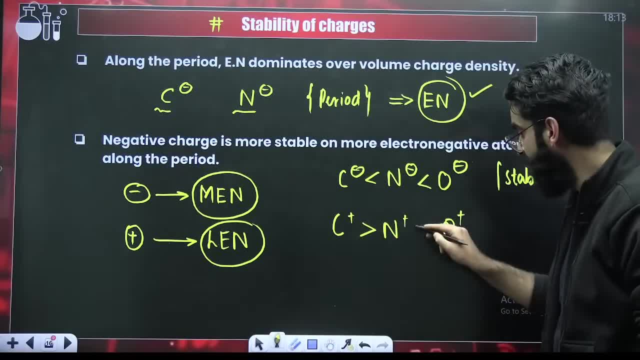 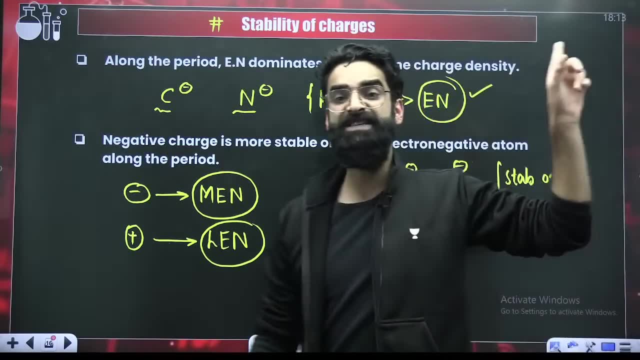 less electronegative among these Carbon, So positive charge will be more stable here. followed by this. followed by this: This is the stability order. This is the stability order, Right? Let me know if this particular slide is clear. Let me know if this particular slide is clear. Whenever. 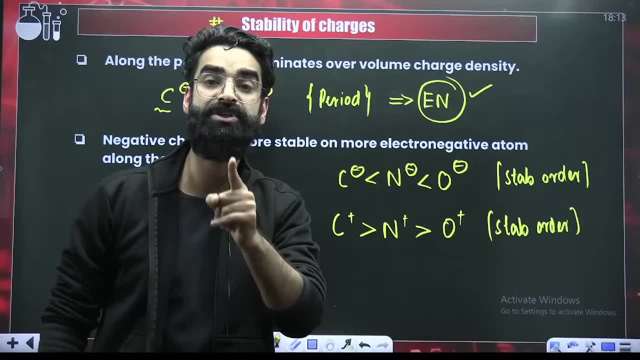 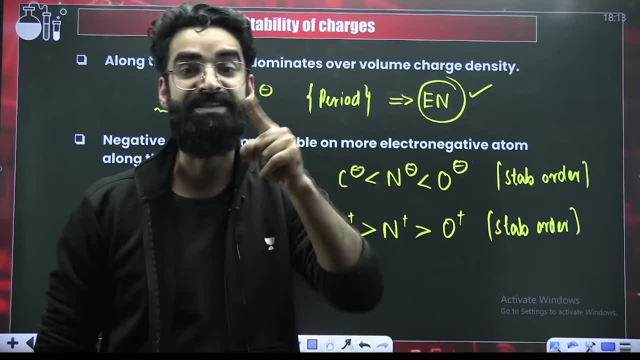 you have to compare the stability of the charges on the elements which belong to same period. you will be talking in terms of electronegativity. Negative charge is more stable on more electronegative. Positive charge is more stable on less electronegative. 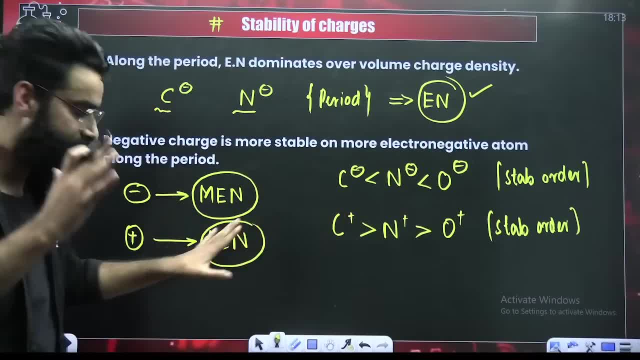 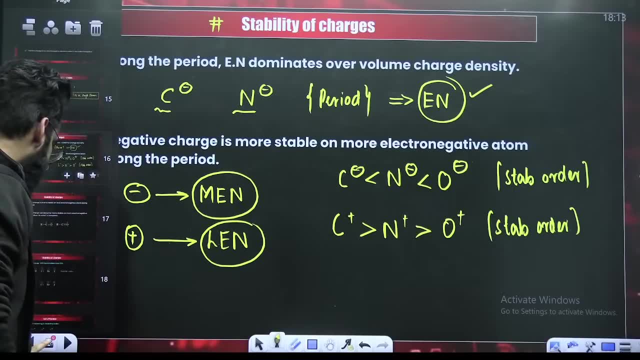 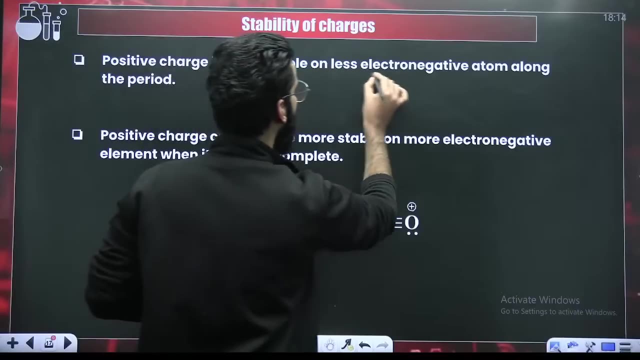 As simple as that, As simple as that, Clear Point number one, Point number one, Point number one. My dear students, since I told you, since I told you positive charge is more stable on less electronegative, Since I told you positive charge is more stable on less electronegative, On less. 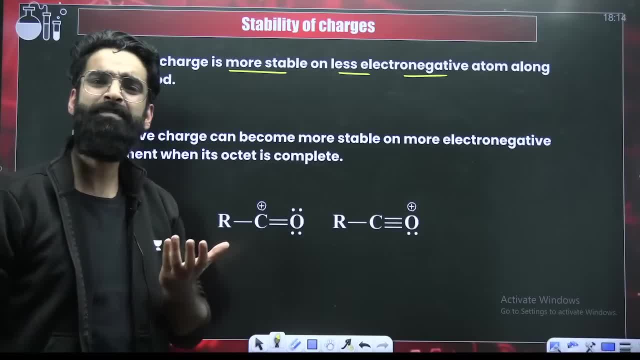 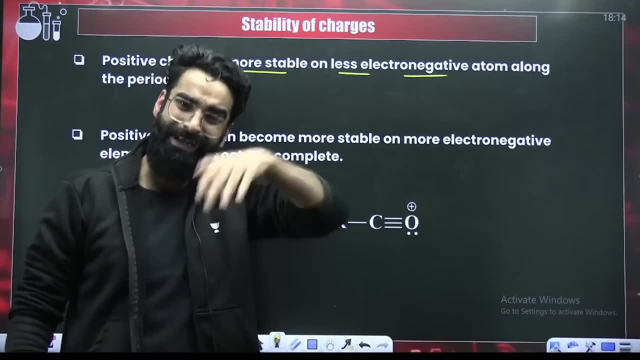 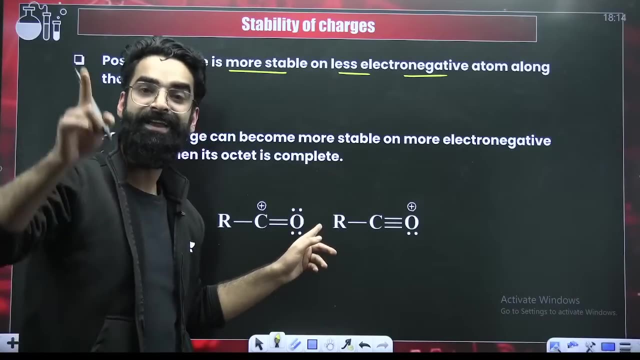 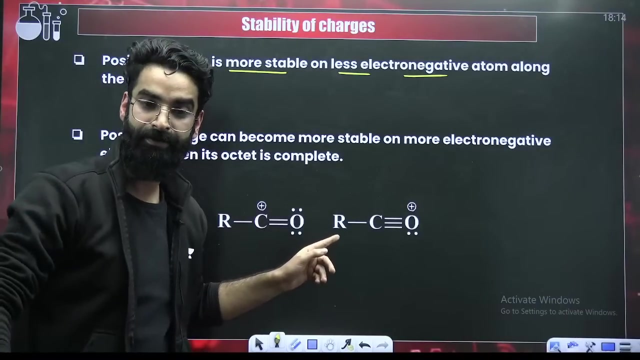 electronegative. Now the question is: can positive charge be more stable on less electronegative anytime? Can positive charge be more stable on less electronegative anytime? See, I think I'm telling you the reverse way, Since we know positive charge is more stable on less electronegative. Now the point is: can positive charge become more stable on more electronegative? 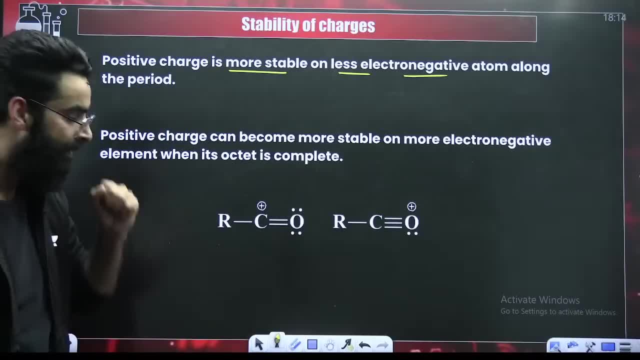 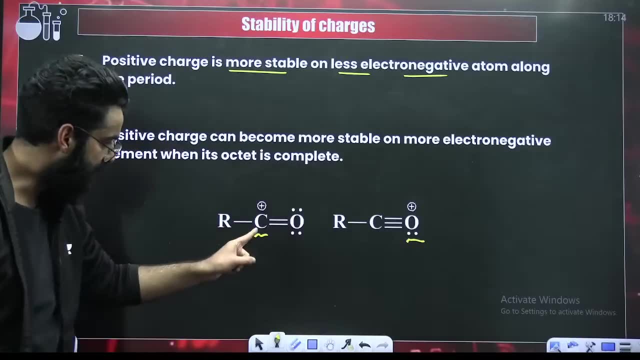 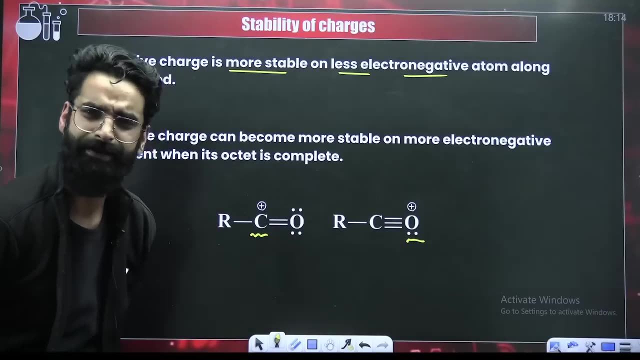 Is there any case like that as well? Yes, Yes, My dear students, try to understand. This is the carbon carrying positive, This is the oxygen carrying positive Carbon carrying positive Oxygen carrying positive Carbon and oxygen. do they belong to same period or same group? They belong to same period, right? 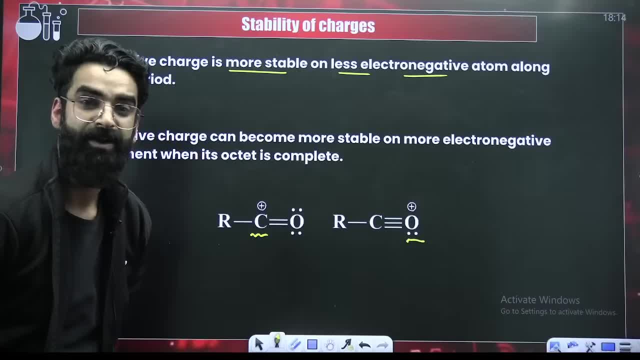 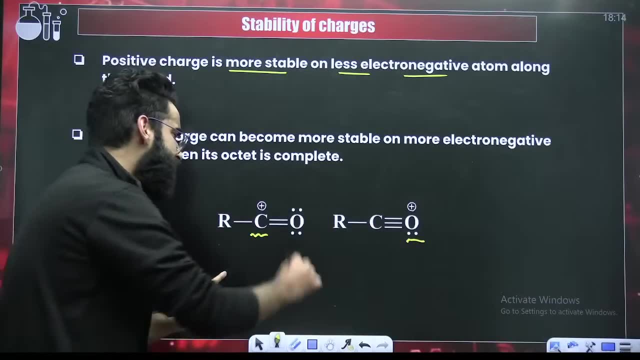 And in the period we'll look after electronegativity. We know normally positive charge is more stable on less electronegative. So where should be the positive charge more stable? Positive charge should be more stable on carbon, because that is, carbon is less electronegative than oxygen. but here the 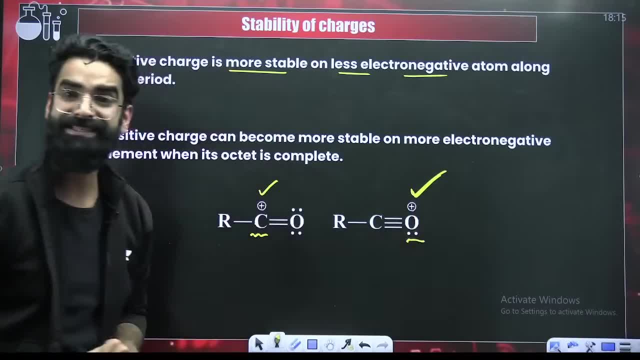 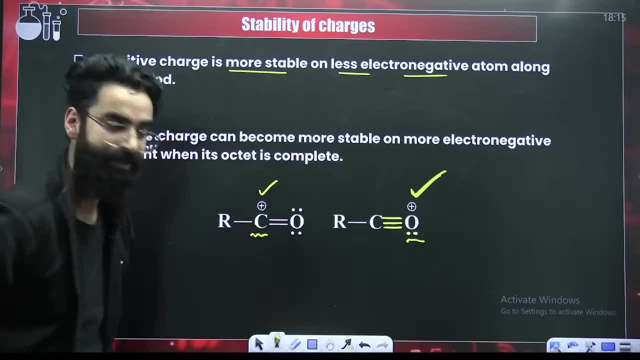 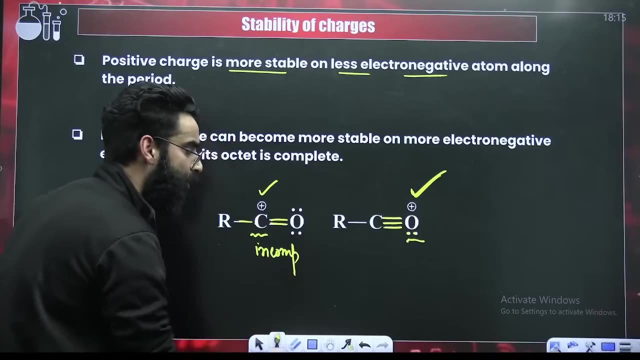 case is reverse: positive charge is more stable than oxygen here. why is that? because look at the octet of oxygen: 2, 4, 6 and 8. the octet is complete. look at the octet of carbon: 2, 4, 6. this is incomplete octet. this is incomplete octet. here you have. 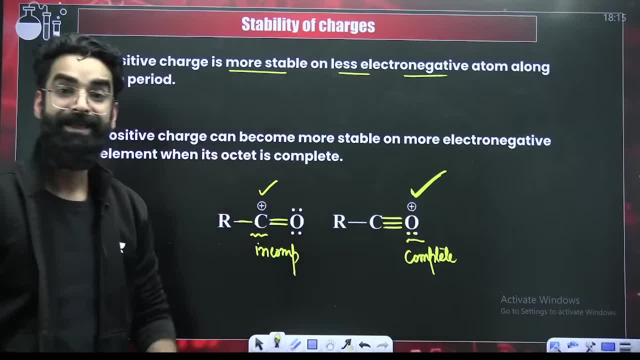 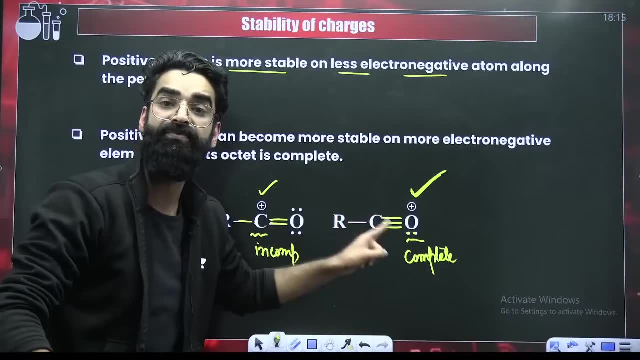 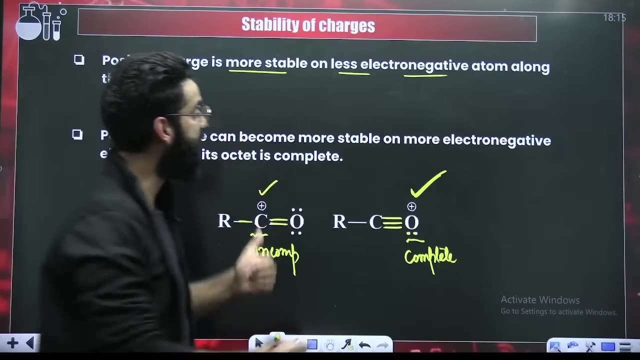 got complete octet. here you have got complete octet. let me tell you: positive charge can become more stable on more electronegative as well if the octet is complete. if the octet is complete- that is the statement which I have written over here- positive charge can become more stable. 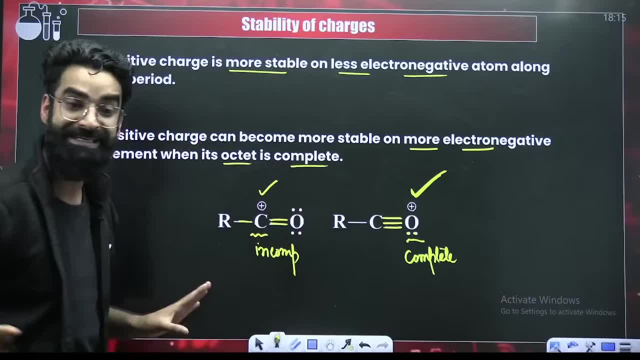 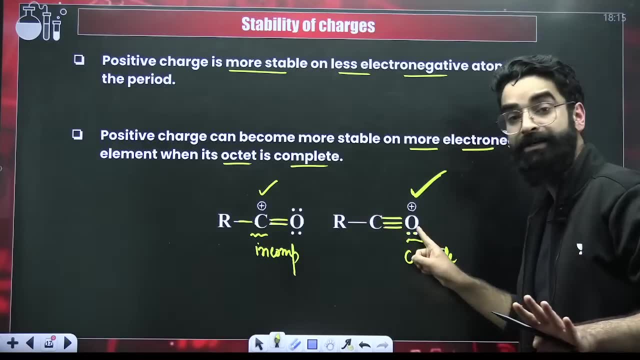 on more electronegative element when it's octet is complete. is this point clear? is this point clear normally? what is the trend? carbon oxygen- they belong to same period, same period. electronegativity plays a role. positive charge is in normally more stable come We might watch a movie. 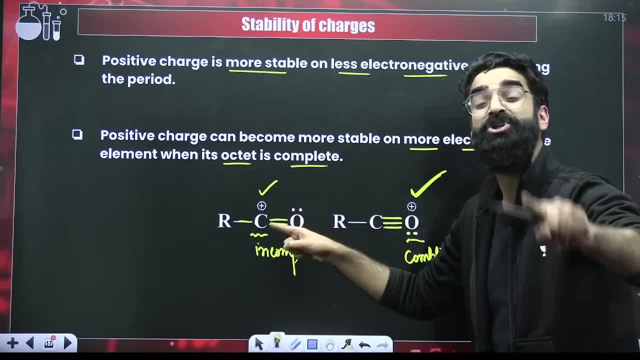 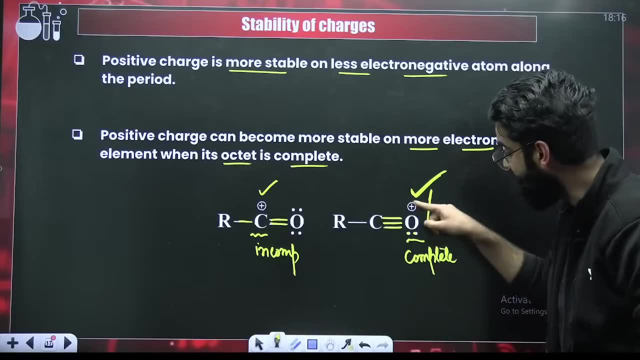 on less electronegative. so this positive charge on carbon should be more stable. but here oxygen carrying positive is more stable. positive and oxygen is more stable. why is that? because here the octet is complete, here the octet is incomplete. so do remember, positive charge can become more. 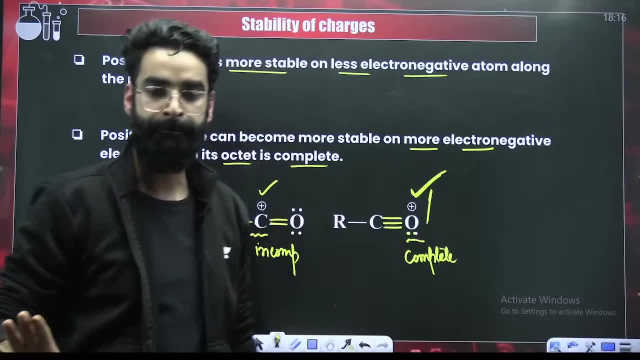 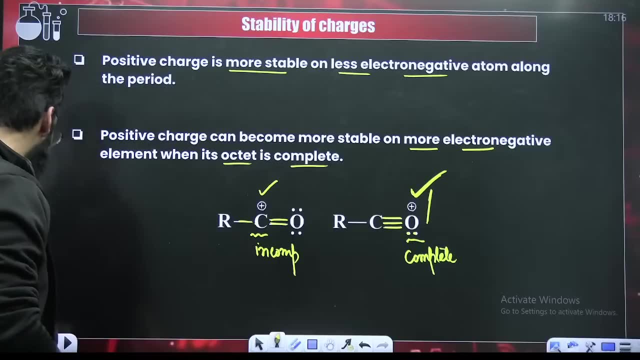 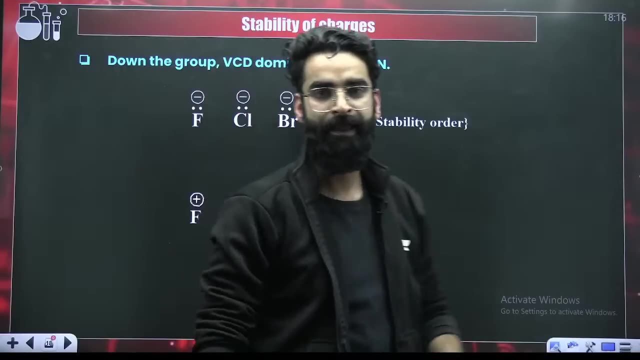 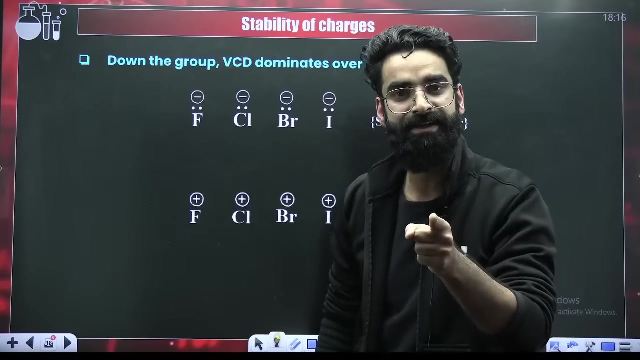 stable on more electronegative element if the octet is getting complete, yes or no in the charts. everyone, everyone, everyone, quickly in the charts. my dear students, remember these points, remember these points, remember these points. now comes one more point. now comes one more point. whenever, whenever you have to compare the stability of the charges on the elements, 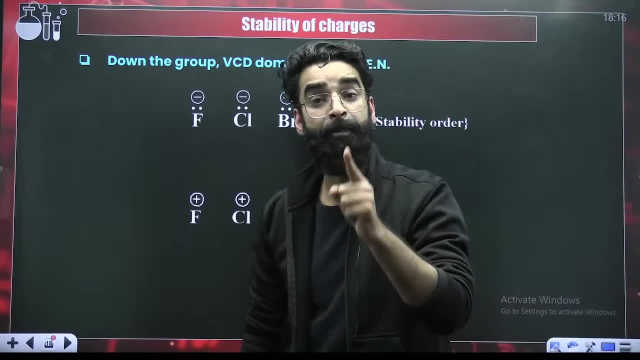 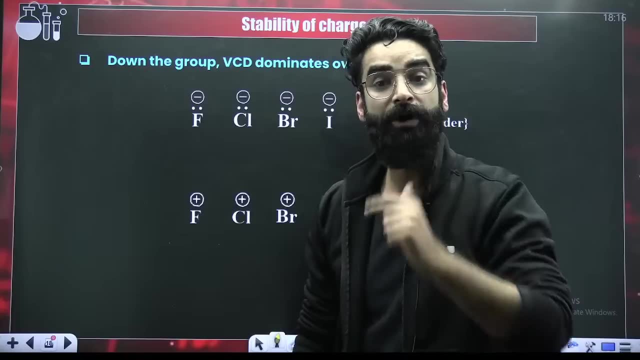 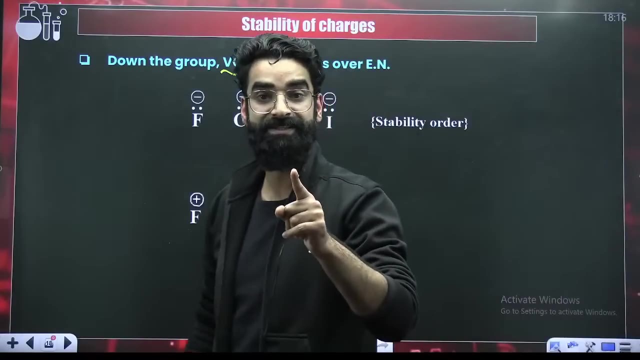 which belong to same group. whenever you need to compare the stability of the charges on the elements which belong to same group, at that point of time you are not going to consider electron negativity. you are going to prioritize volume charge density. you are going to prioritize volume charge density along the period. always talk. 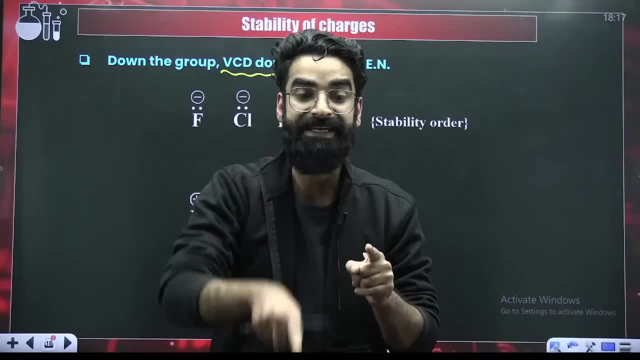 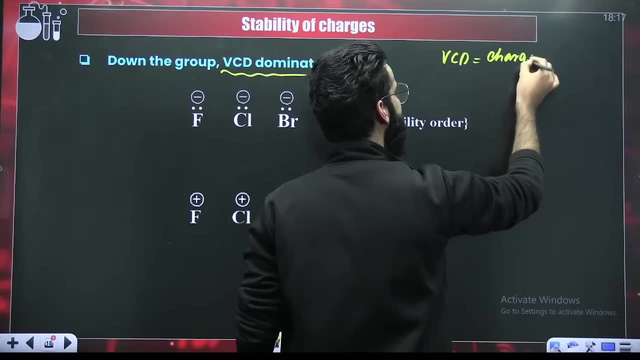 in terms of electro negativity group, talk in terms of vcd. talk in terms of vcd- and i hope you know your volume, charge density is equal to charge present on the specie divided by size of the specie and you must be knowing already- you have discussed stability- is inversely proportional. 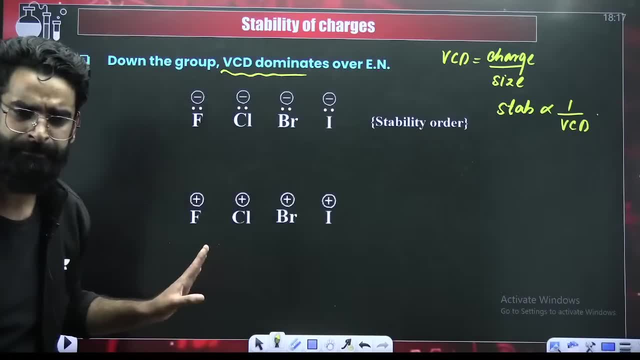 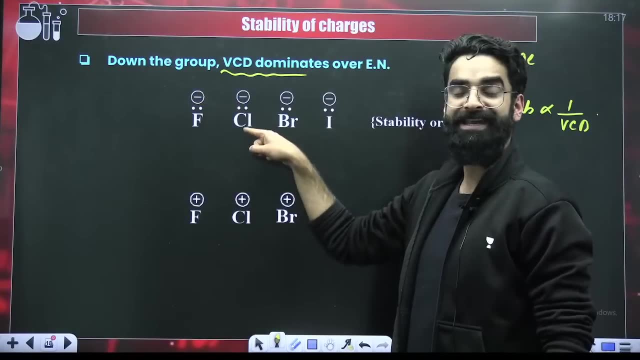 to volume charge density. right, these are the two things which you have to remove, nothing else. now we will try to understand. try to understand. try to understand. chlorine carrying negative, chlorine carrying negative, bromine caring negative, iodine carrying negative: do these elements, do they belong to same period or same group? you tell me the answer. 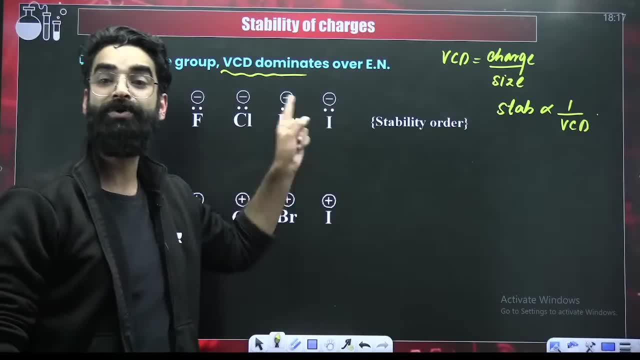 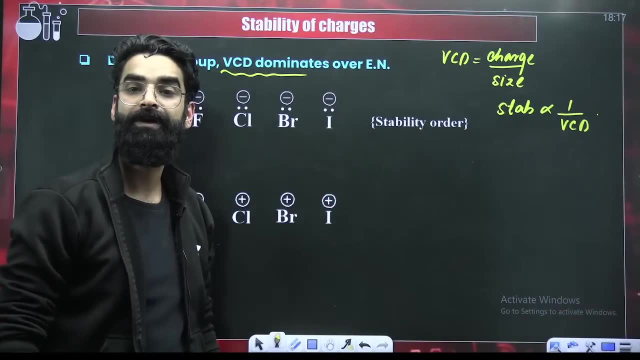 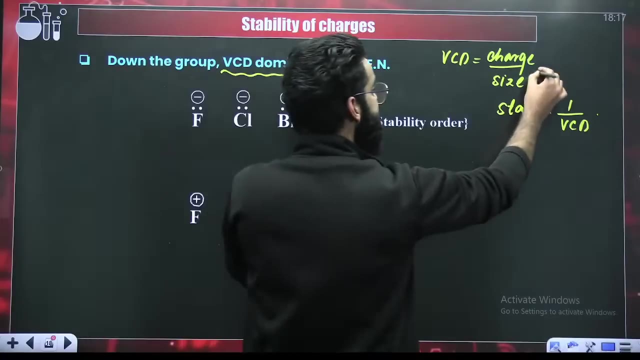 do they belong to same period or same group? these elements belong to same group and in the group vcd plays a role. in the group, vcd plays the role. the charge on every specie is same, but the size is different. this particular specie has got more size. more size means less vcd. 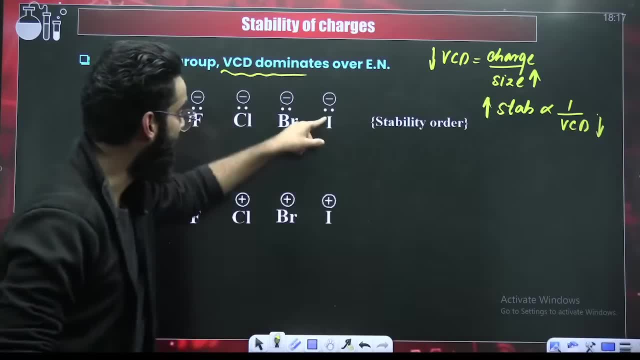 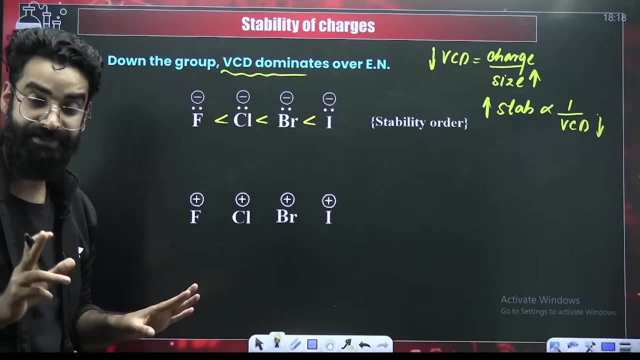 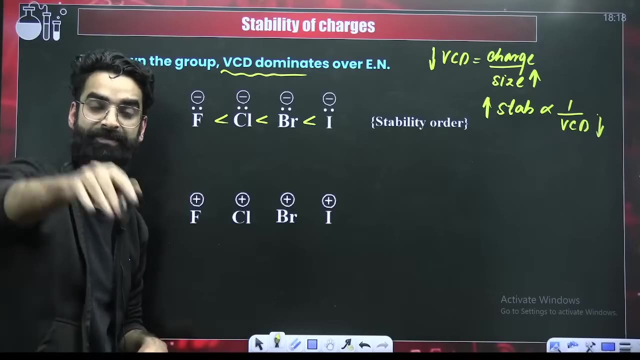 Less volume charge density means more stability. now Tell me, where is the negative charge more stable? I would say this is the stability order of negative charge. Yes, I Hope you are getting this. I hope you are getting this again: Chlorine carrying positive. chlorine carrying positive. bromine carrying positive. iodine carrying positive. now you have to answer me. 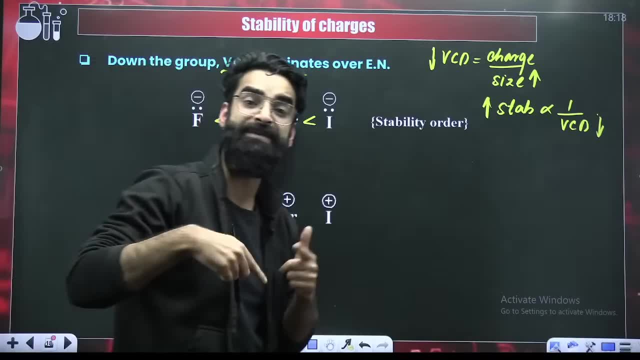 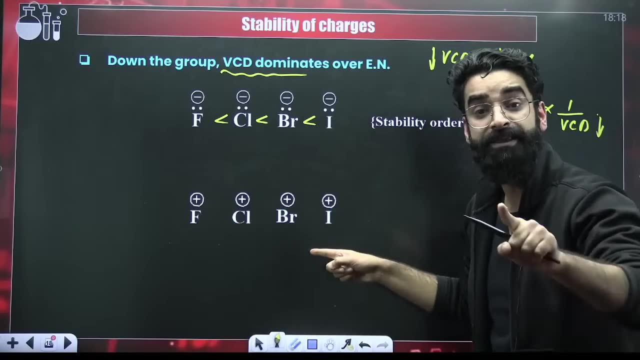 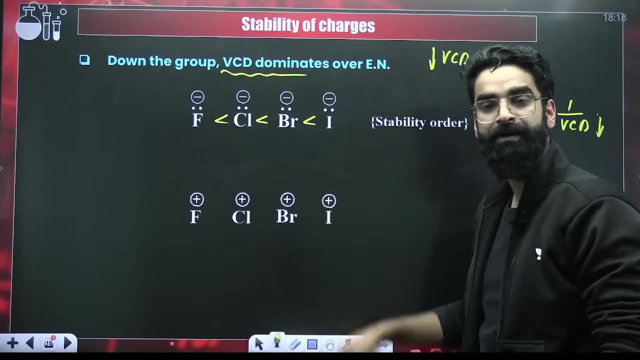 You have to answer me whether these elements, whether they belong to same period or same group. Whether these elements belong to same period or same group. They belong to same group. in the group VCD plays the role. Volume charge density plays the role. now you tell me: the charge everywhere is same. the charge everywhere is same. 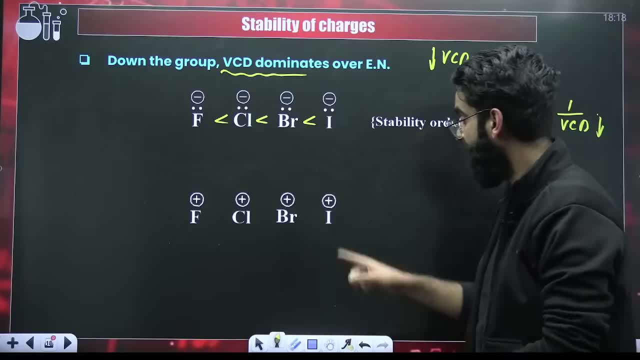 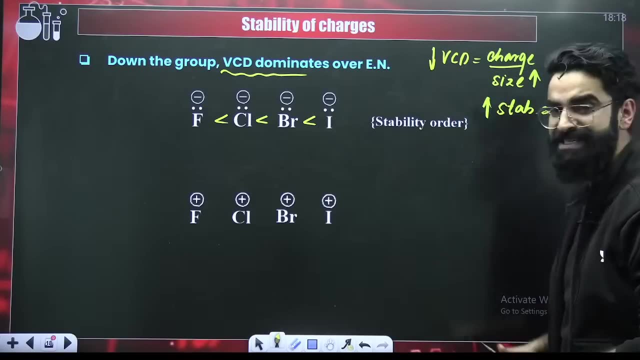 But? but the difference lies in size. Iodine, it has got more size, more size, Less volume charge density: less the volume charge density, more the stability. So where is the positive charge more stable? This is going to be the stability order. say yes or no in the charts if it is clear. 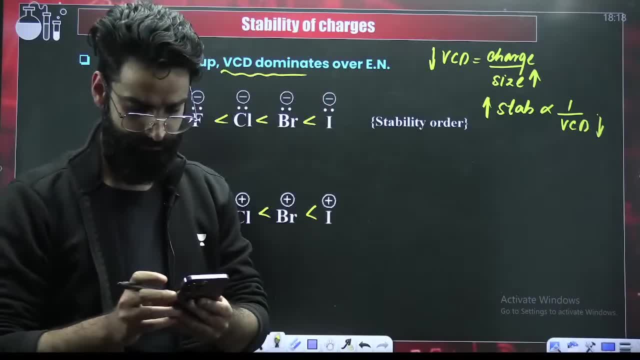 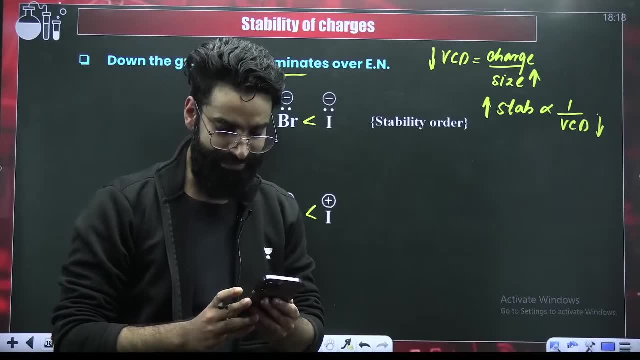 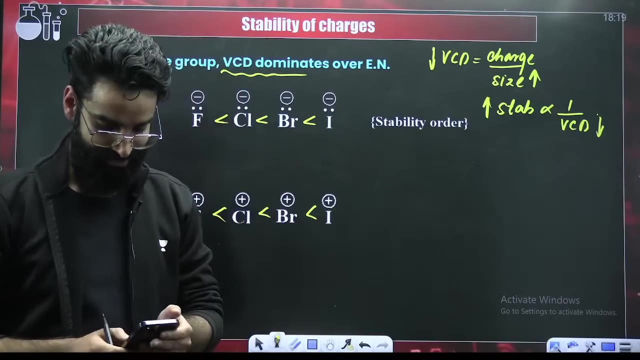 Say yes or no in the charts, But it's clear: everyone Wiggly people, everyone in the charts guys, I want the Josh to be high all the time. It's a big marathon. It is a big marathon, Okay. so you have to keep me motivating as well with your charts. 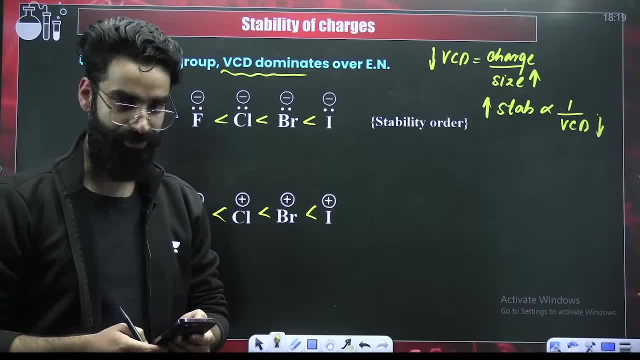 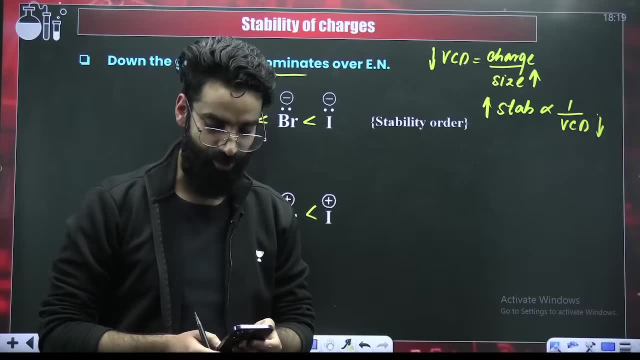 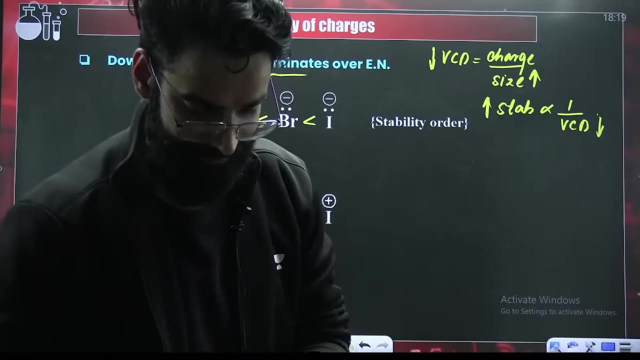 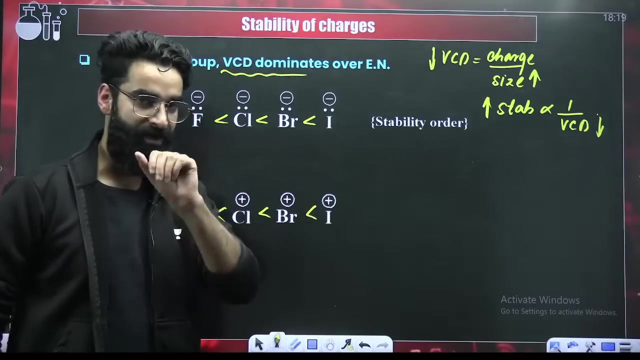 I want the charts to run continuously and I can see not everyone has liked the session yet to do like the session right now. Right now means right now, Or else you are over, you're gone. Yeah, Everyone, people, everyone, Everyone in the charts. yeah, Perfect. what are the concepts we have discussed till now? 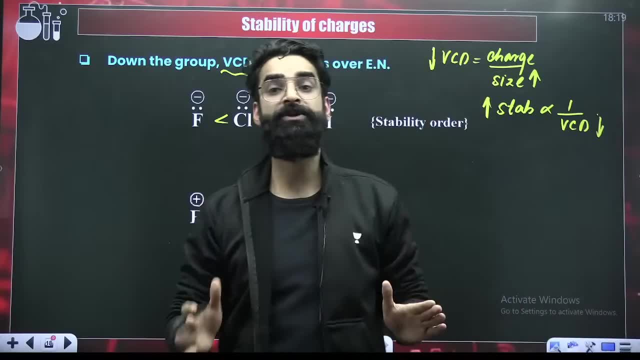 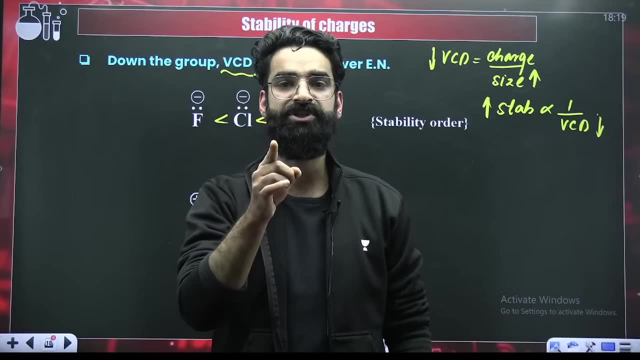 I'm going to utilize all the concepts now in the questions, But before showing you the questions, just a quick revision of everything. just a quick revision on everything. Whenever we need to compare the stability of the charges on the elements Which belong to same period, we have to talk in terms of electronegativity. 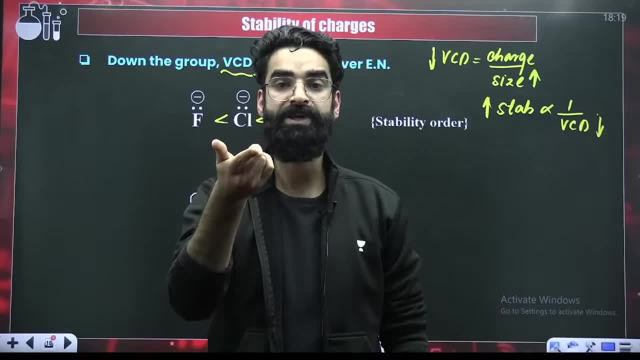 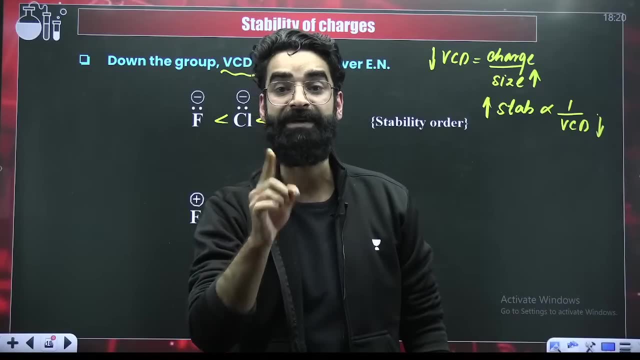 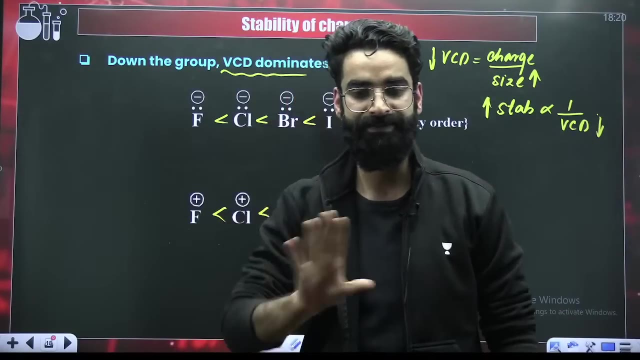 negative charge is more stable on more electronegative. positive charge is more stable on less electronegative. number one, number two: Whenever we need to compare the stability of the charges on the elements which belong to same group, volume charge density plays a role. Volume charge density plays the role. Stability is university proportional to VCD. That's all. that's all. now people try to solve the questions. 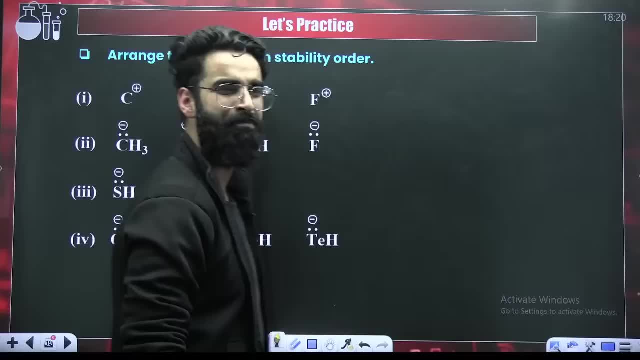 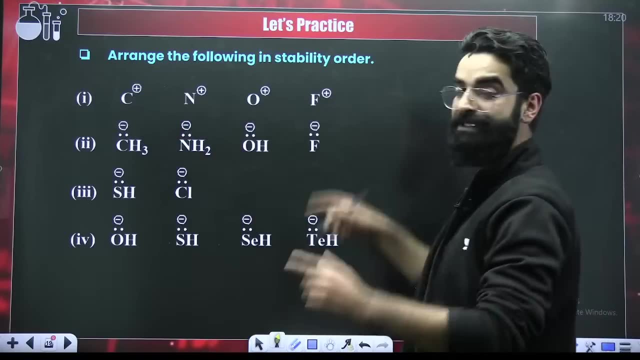 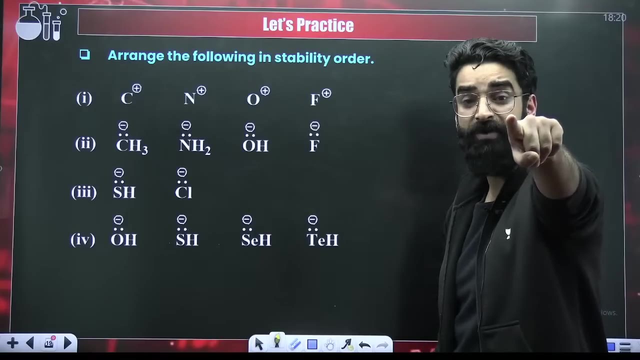 Which I'm giving you Almost almost. I have got more than 500 questions today, Almost almost more than 500 questions today. All right, arrange the following in the stability order: Can you let me know Where is the positive charge maximum stable? I would want to see your answers first. I would want to see your answers first. 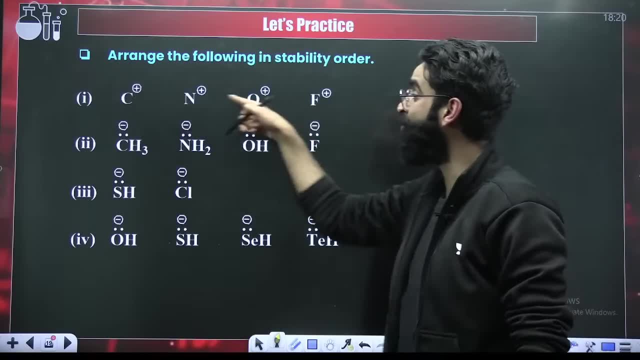 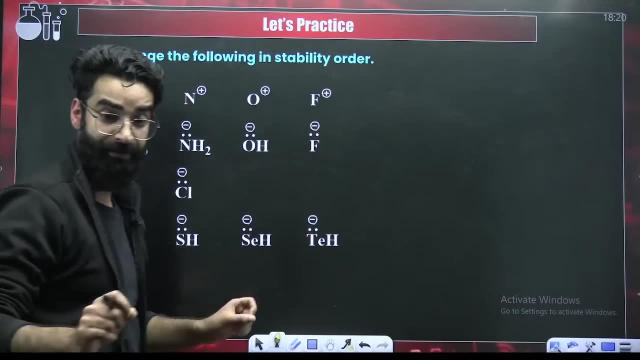 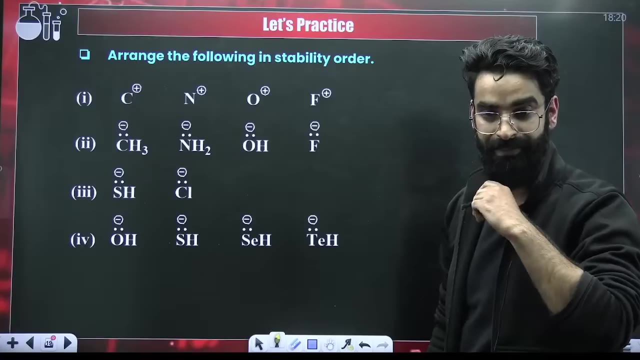 I would want to see your answers first. Where is the positive charge more stable among all these four or five species? Quickly, everyone, quickly. You should be in a position to answer this question. You should be in a position to answer this question. You should be in a position to answer this question. everyone. everyone means everyone. 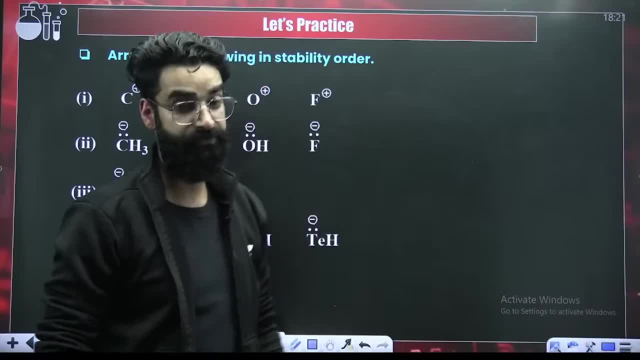 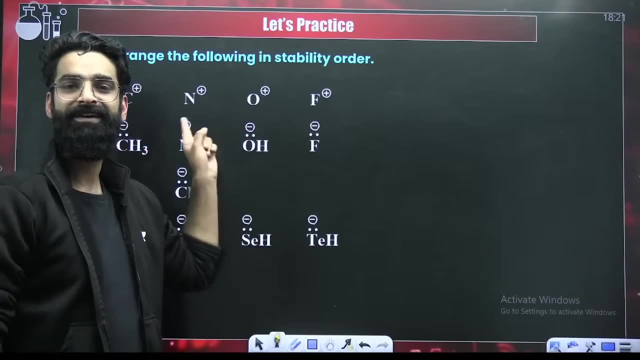 Are you sure? Are you sure? What kind of logic did you use here? See guys, carbon positive, nitrogen positive, oxygen positive, chlorine positive. These elements belong to same period. in the period Electronegativity plays a role, right, positive charge is more stable on less electronegative. 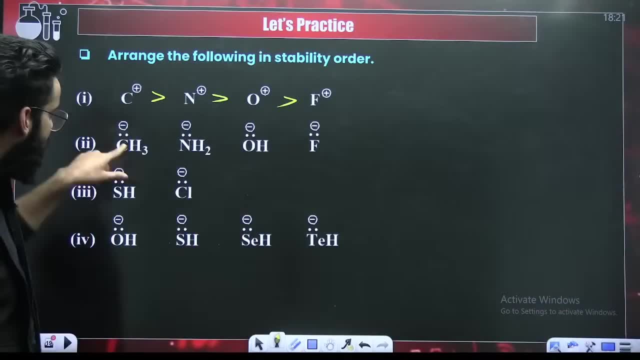 Oxid charge is more stable on less electronegative. Look at the second question: Carbon carrying negative Nitrogen, negative Oxygen, negative Fluorine, negative Carbon, nitrogen oxygen, fluorine. Again, they belong to same period. 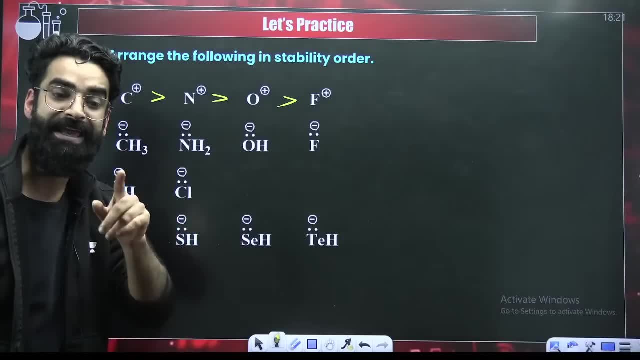 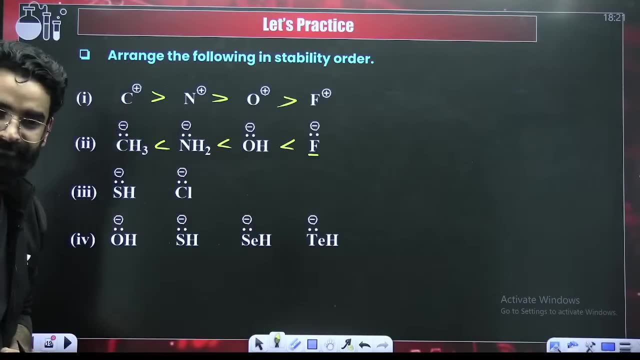 Electronegativity plays a role. Electronegativity plays a role. Negative charge is more stable on more electronegative. Negative charge is more stable on more electronegative. So this is the stability order: Sulfur carrying negative. 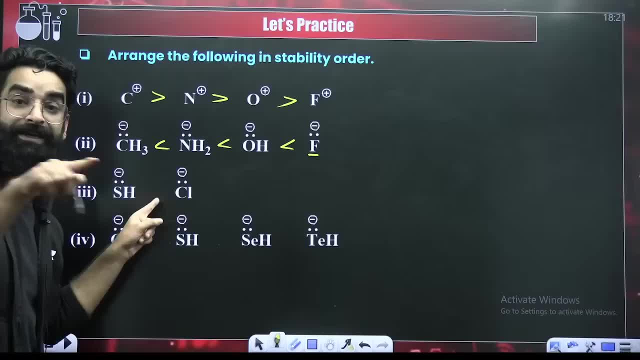 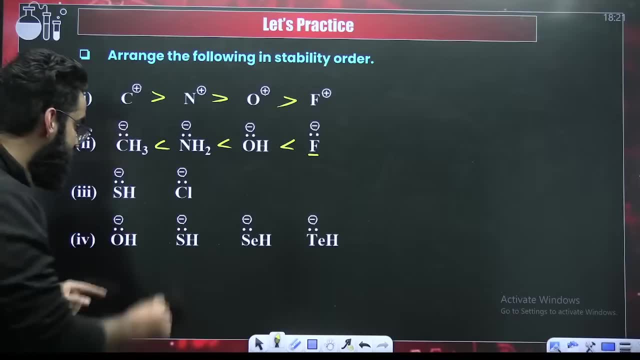 Chlorine carrying negative. Where is the negative charge more stable? Sulfur and chlorine? Same period Electronegativity. Electronegativity plays a role. Negative charge is more stable on more electronegative. So which one is more electronegative among these? 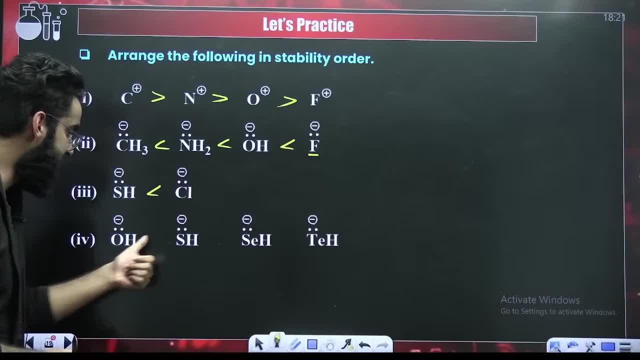 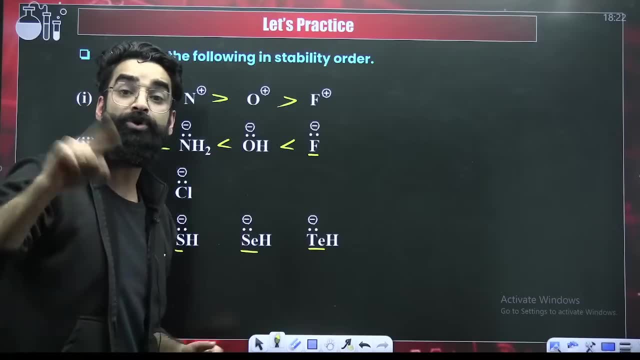 Chlorine. So negative charge is more stable here. Oxygen negative: This is oxygen, This is sulfur, This is SE, This is TE. They belong to same group. They belong to same group. We have to consider VCD here. 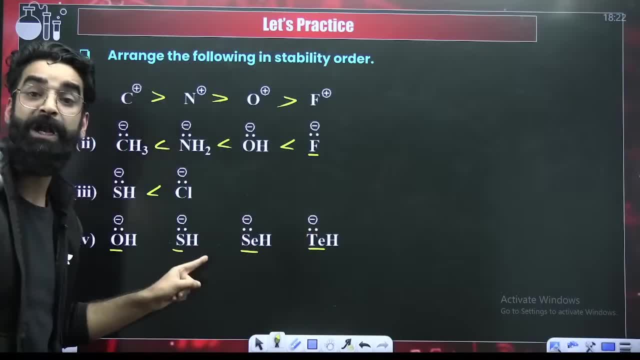 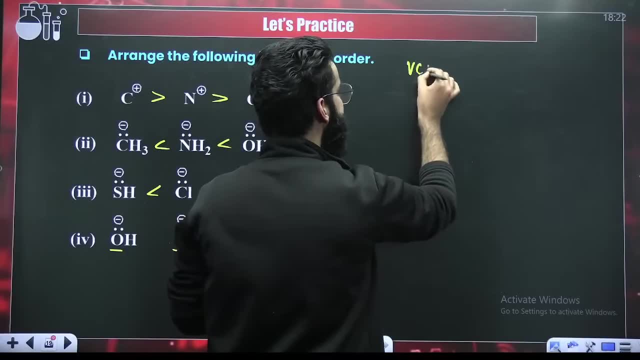 We have to consider VCD here. Now, charge everywhere is same. Look at the size Down. the group size increases. Size is maximum here. Size is maximum here, And you know VCD: It is inversely proportional to size. 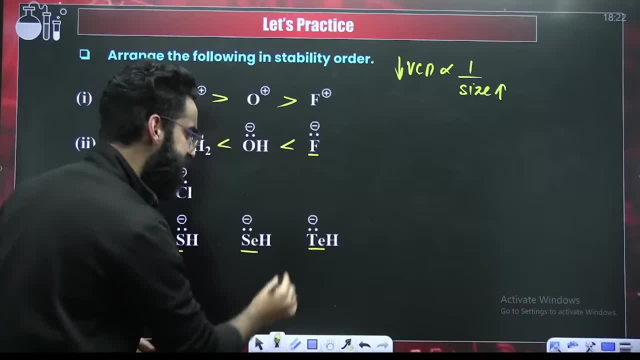 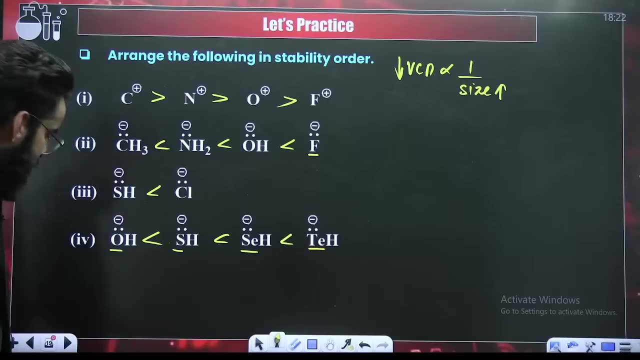 It is inversely proportional to size: More the size less the VCD: Less the VCD: more the stability. This is the order of stability of these negative charges. Yes, Perfectly done. Perfectly done, Perfectly done. 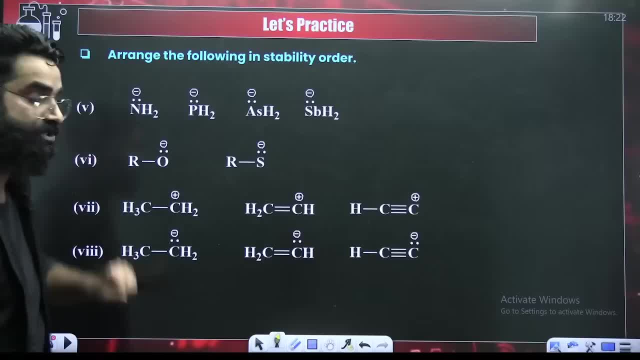 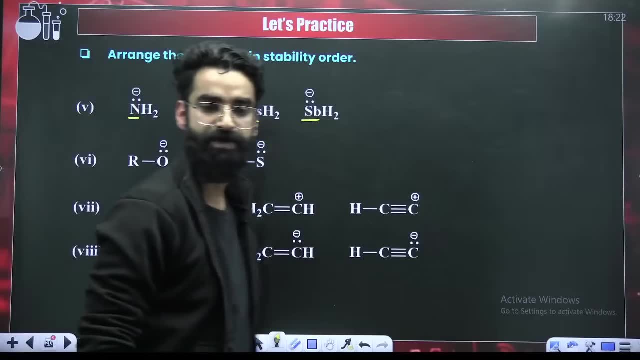 Yes or no? Look at the more questions. More questions on your screen. Have a look. Nitrogen carrying negative, Phosphorus negative. Arsenic negative, Antimony negative. Do these elements belong to same period or same group? Everyone. 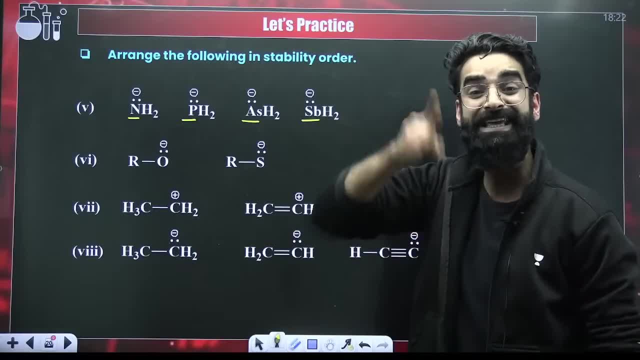 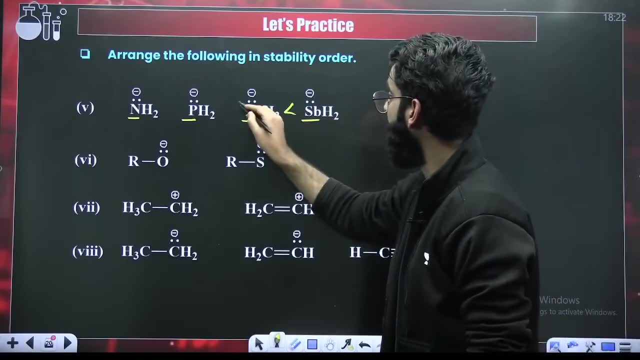 Same period or same group. They belong to same group. VCD plays a role. More the size, less the VCD. Lesser the VCD. more the stability Right. This is the stability order of the negative charges, Right? Tell me here. 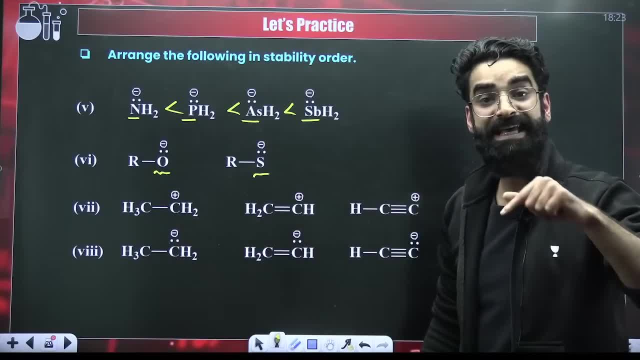 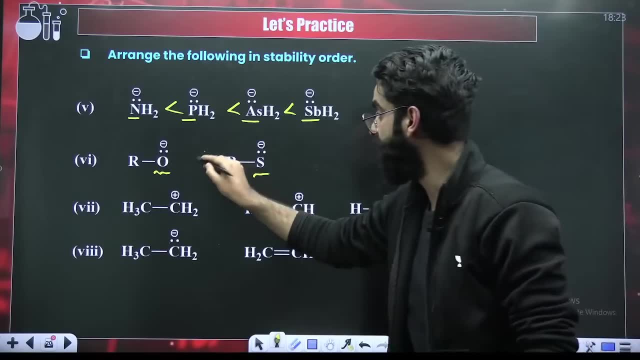 Oxygen carrying negative Sulfur carrying negative Oxygen: sulfur- Oxygen sulfur. Same group, Same group VCD. More size, less VCD, more stability. Is this, Is this the order? Quickly, Let me know here. 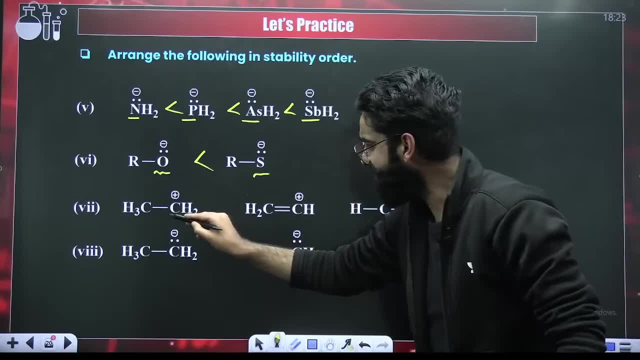 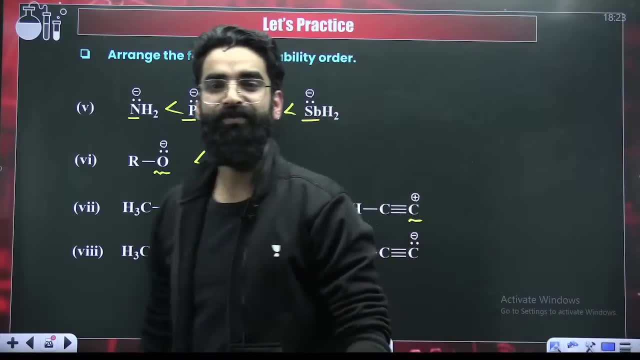 Let me know here. If you look properly, this is single bonded carb. This is double bonded carb. This is triple bonded carb. Where is the S character more? Where is the S character more: Single bonded, double bonded or triple bonded? 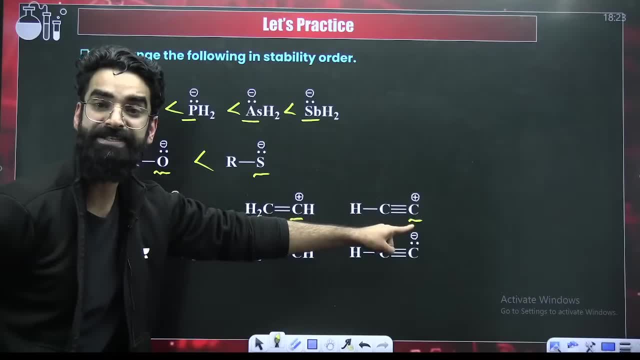 Where is S character more Here? the S character is more. So I would say electronegativity of this one is more Right. But we know positive charge is more stable or less electronegative Right, We know positive charge is more stable or less electronegative. 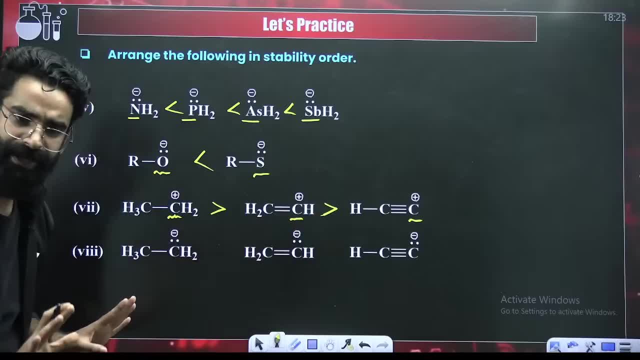 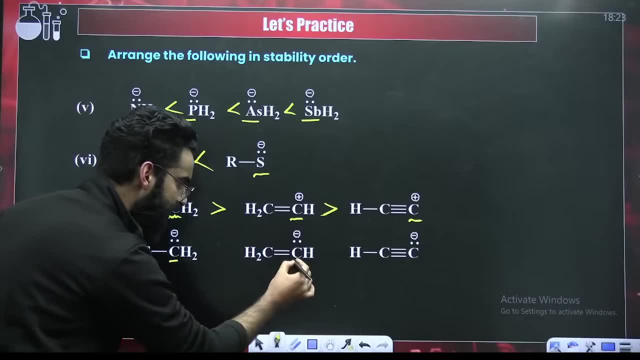 This one is less electronegative. So this is the stability order. Done, Simple trick to remember, That's it. Okay, Look at the next one: Carbon carrying negative. double bonded carbon carrying negative. triple bonded carbon carrying negative. 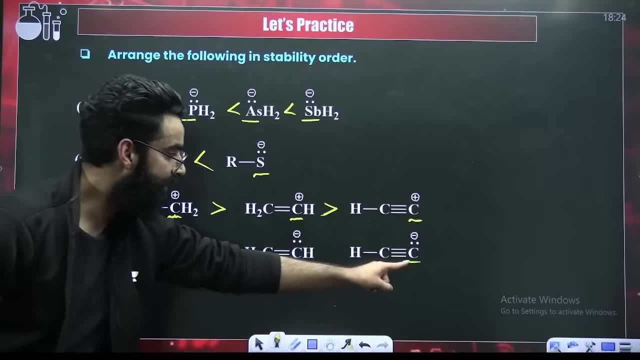 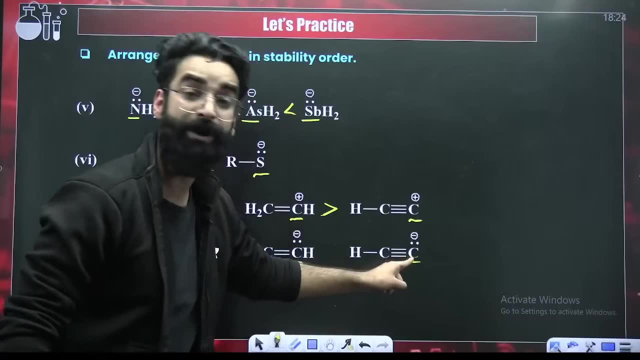 Where is the S character more? Where is the S character more? S character is more here. Right S character is more here, S-P hybridized. If S character is more here, that means it's electronegativity is more. 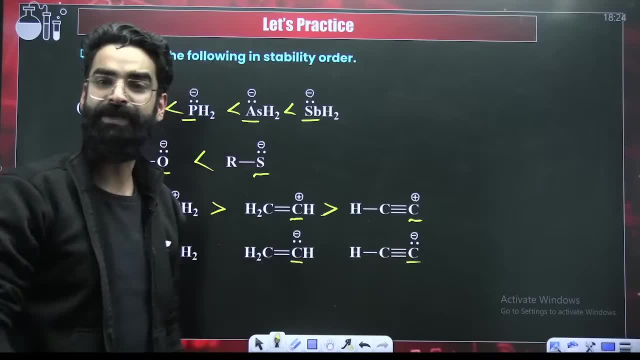 And you know, Nagiru charge is more stable on more electronegative. Nagiru charge is more stable on more electronegative. So is this going to be the stability order? Absolutely, this is going to be the stability order. 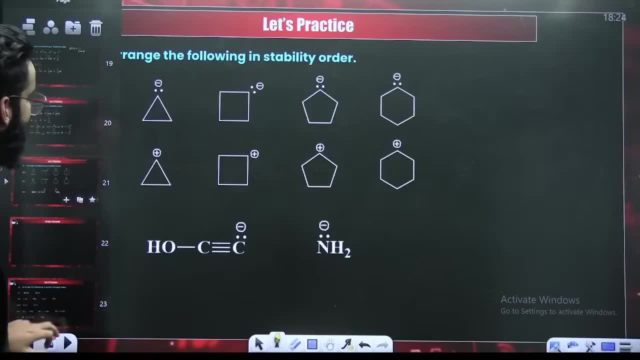 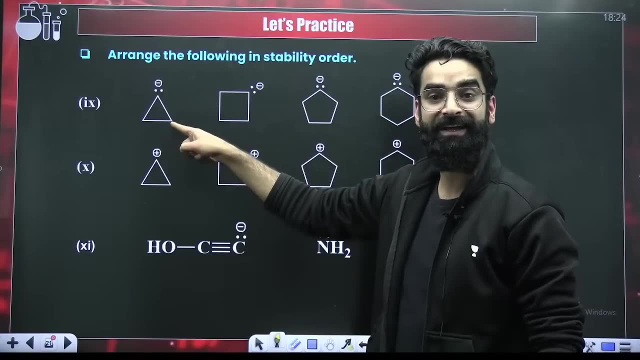 Absolutely. this is going to be the stability order. These questions tell me their answers. Tell me their answers, people. Nagiru charge on 3-membered ring. Nagiru charge on 4-membered ring. 5-membered, 6-membered. 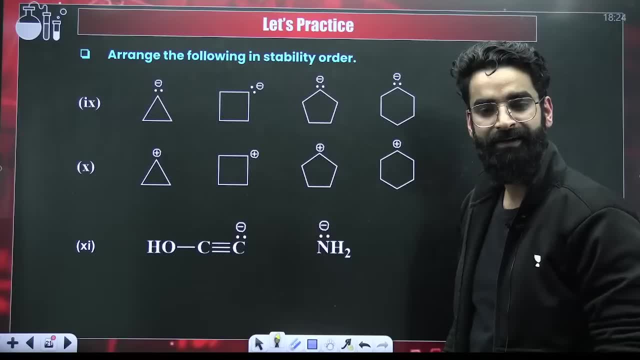 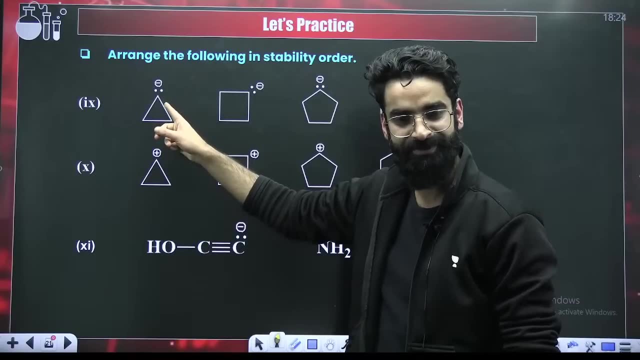 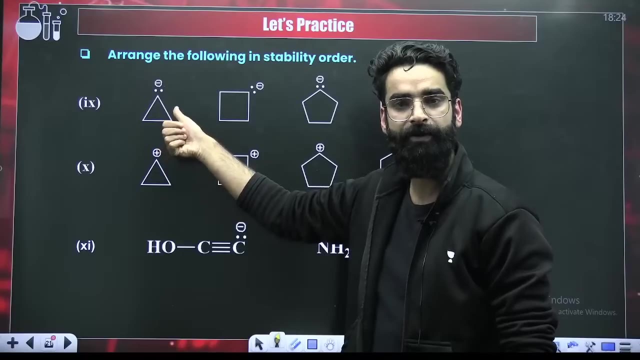 Which one has got maximum angle strain. Which one has got maximum angle strain? Sir, you look like Kashmiri. Yes, I am from Kashmir, from Srinagar. Tell me, Have a look people here, Have a look here. 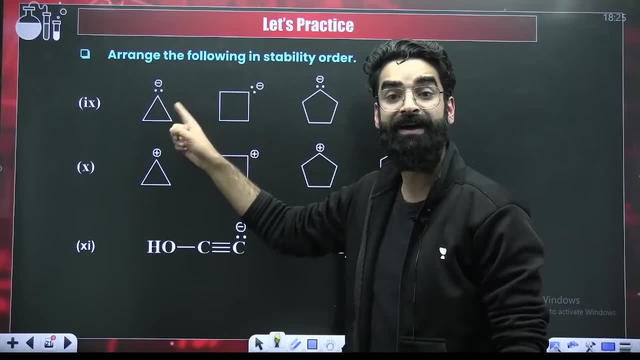 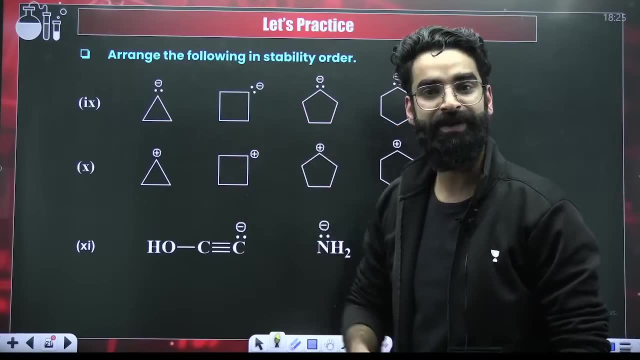 Which one is under maximum angle strain. I will say: first one is under maximum angle strain, First one is under maximum angle strain Right: More the angle strain, more the electronegativity, So electronegativity of this carbon. 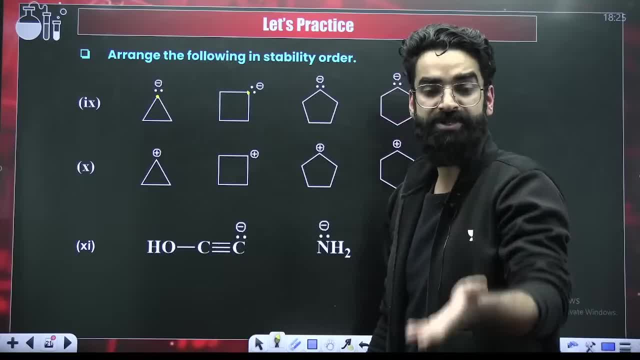 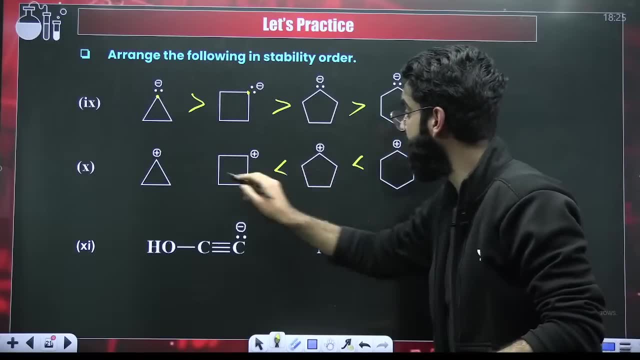 will be more than that of this Right And Nagiru charge is more stable on more electronegativity. This is the stability order. Positive charge is more stable on less electronegativity. This is the stability order. Now tell me this particular scenario. 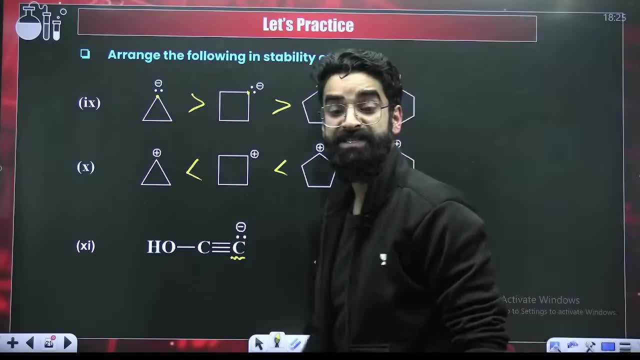 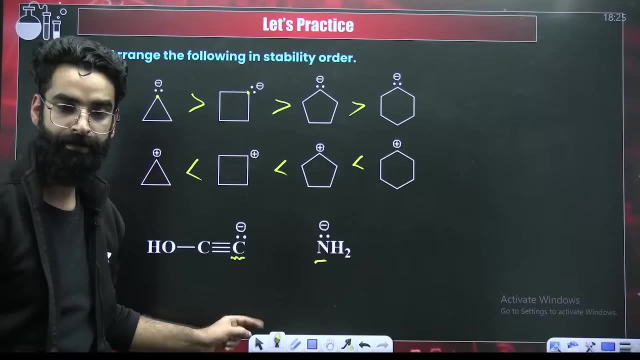 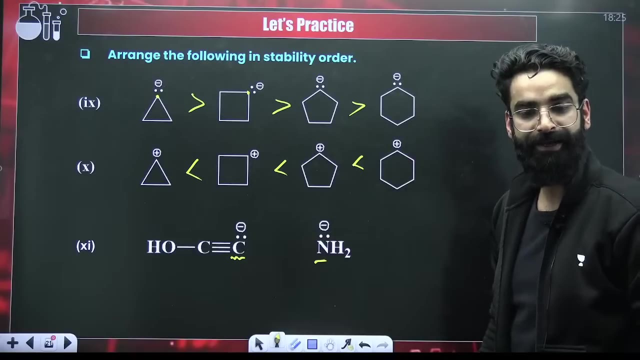 Carbon carrying negative and nitrogen carrying negative. Where is the Nagiru charge more stable? You need to answer this. You need to answer this everyone. You need to answer this. You need to answer this people quickly. Where is the Nagiru charge more stable, on carbon or nitrogen? 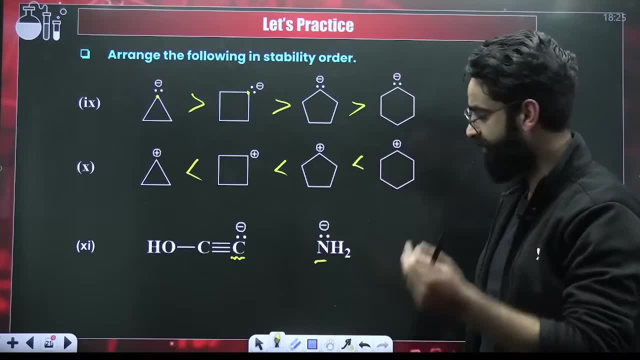 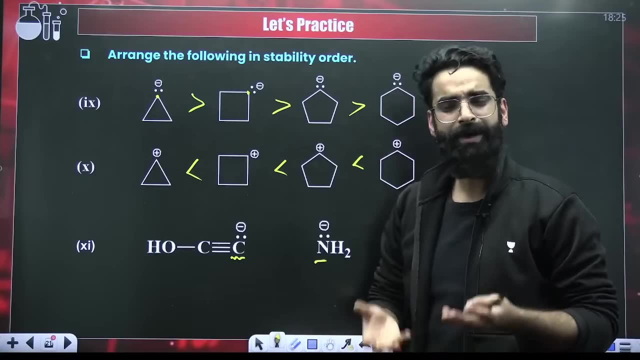 So normally, what should you think? Normally you will think like this: Carbon and nitrogen, they belong to same period, In the period electronegativity dominates Right, And you know, Nagiru charge is more stable on more electronegative. 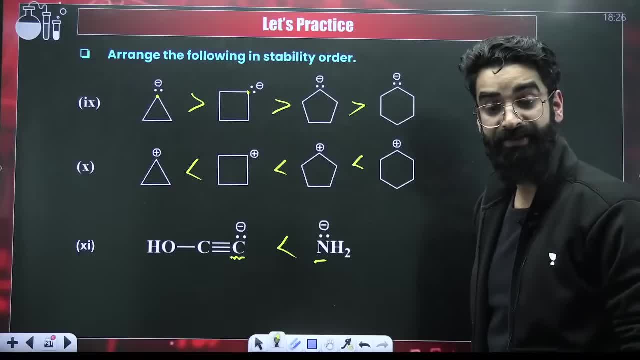 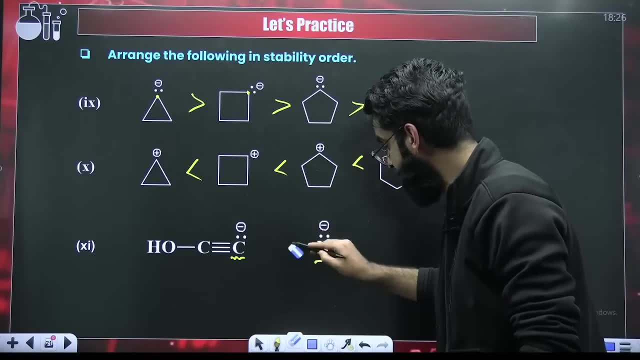 So this has to be the stability order, But if I ask you, is this the actual stability order? This is not the actual stability order. This is not the actual stability order. Remember this, Remember this, people, Remember this. This is a special case. 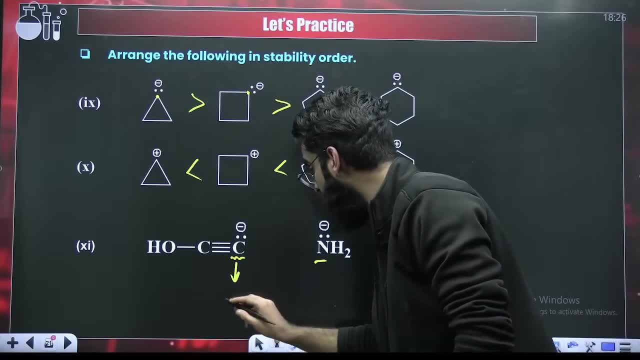 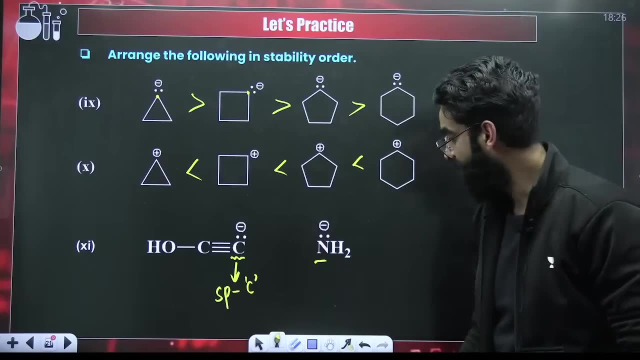 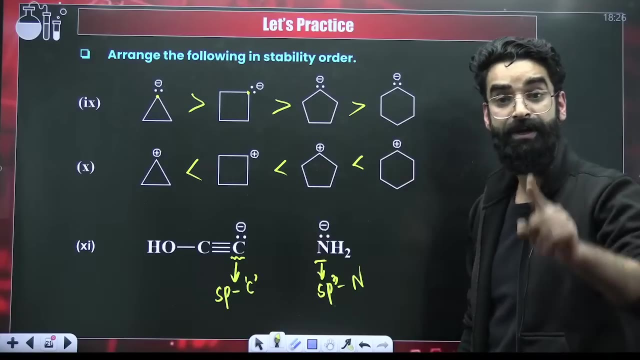 This is a special case. Here you have got sp-hybridize carbon. The carbon which you have here is sp-hybridized Nitrogen. It is sp3-hybridized nitrogen. It is sp3-hybridized nitrogen. 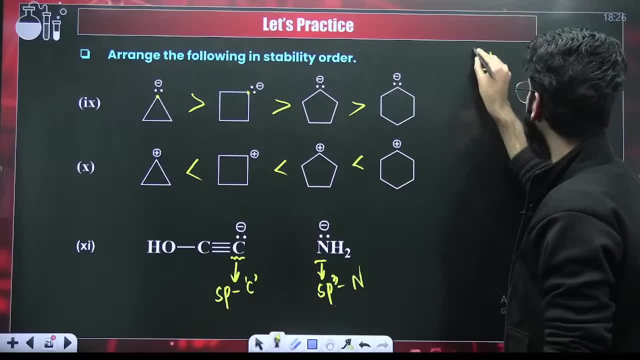 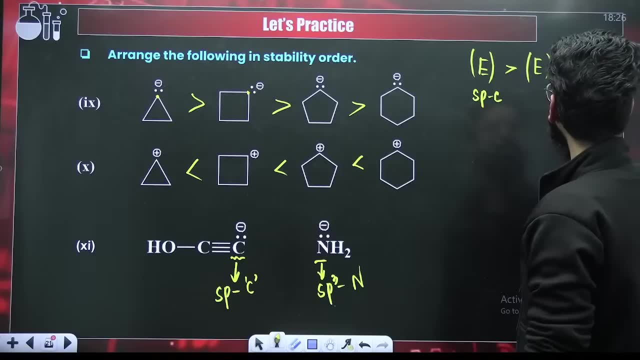 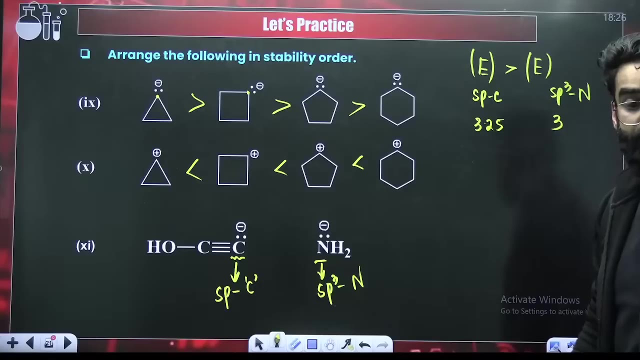 Do remember: electronegativity of sp-hybridized carbon is more than that of electronegativity of sp3-hybridized nitrogen. If you want to remember the values, the value here is 3.25, here the value is 3.. Electronegativity values. I am giving right. 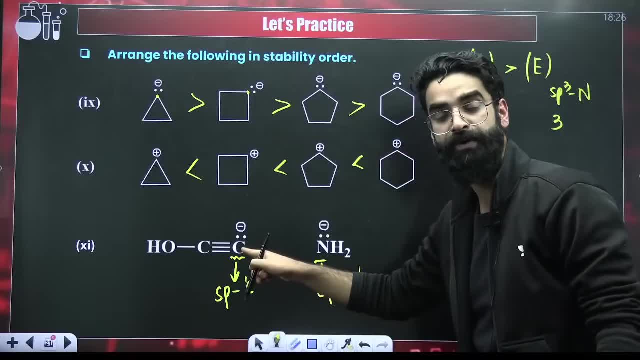 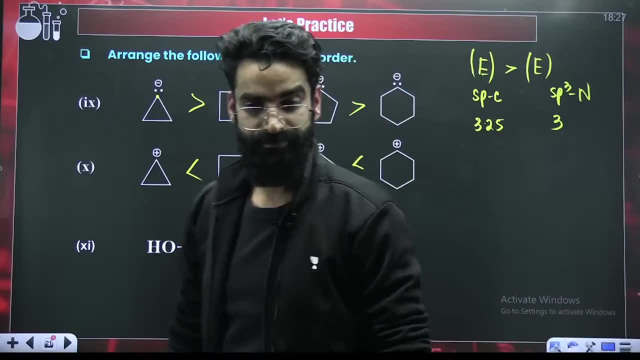 Now which one is more electronegative? I would say this particular species is more electronegative. If it is more electronegative, then it is evident: negative charge is more stable and more electronegative. So this is the order. This is the order. So this was the first type of question which 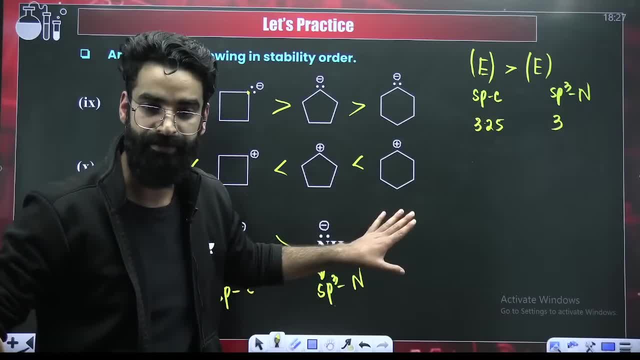 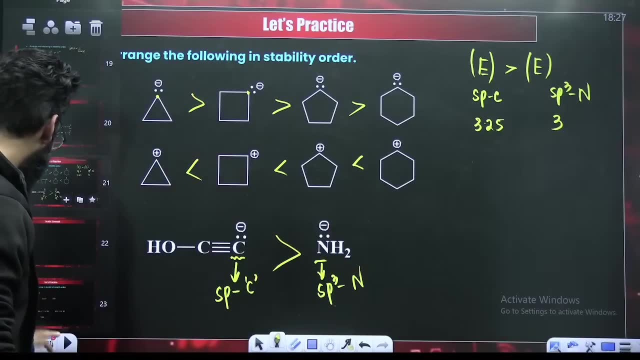 we did here, Arrange the charges on the basis of their stability. right, Right people. Let me know that in the chats with the fire symbol, If every single thing is clear, then I will show you one more type of question Which we can do from the same concept which I taught. 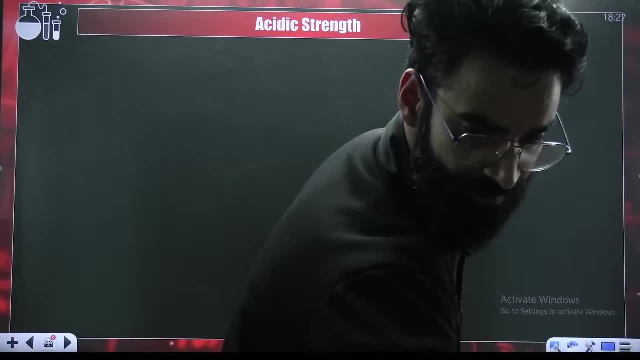 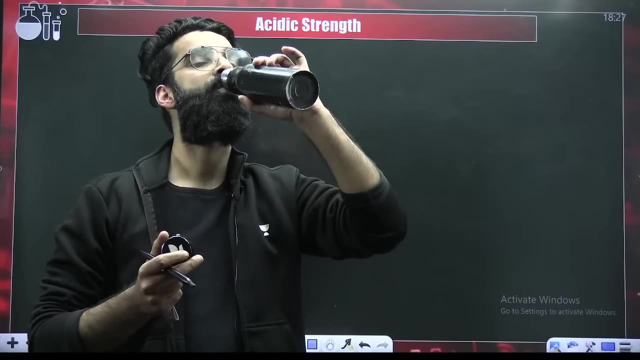 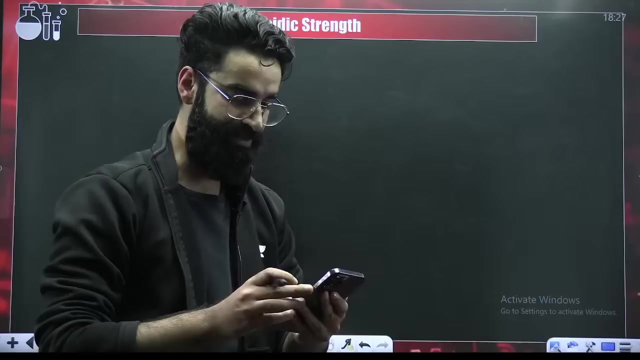 you Tell me, first of all in the chats With the fire emojis, guys, I don't want the chats to be slow at all. I don't want the chats to be slow at all. I don't want the chats to be slow at all people. 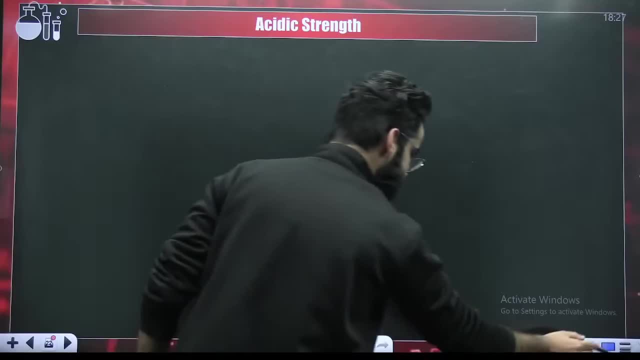 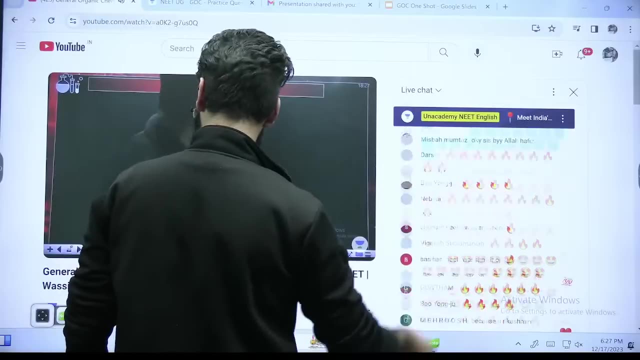 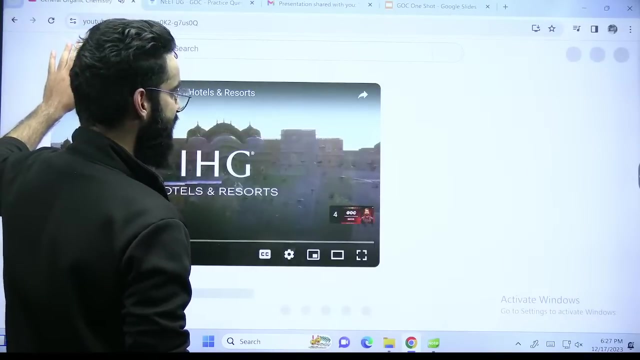 No value offers No performance. offers the chats to be slow at all. let me first of all see how many people are watching us and what is happening in the chats, because i'm unable to see your chats from there. is it live? i think i need to refresh it once. okay, this is the refresh screen, but i am unable to see. 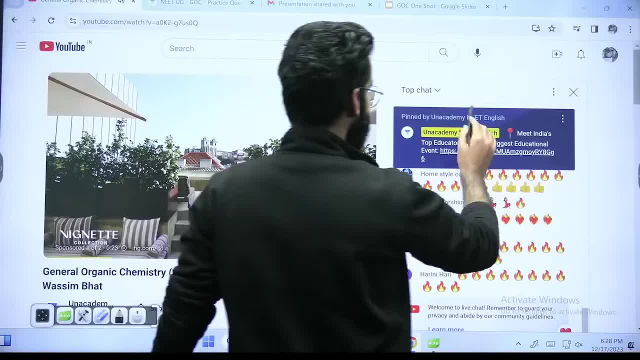 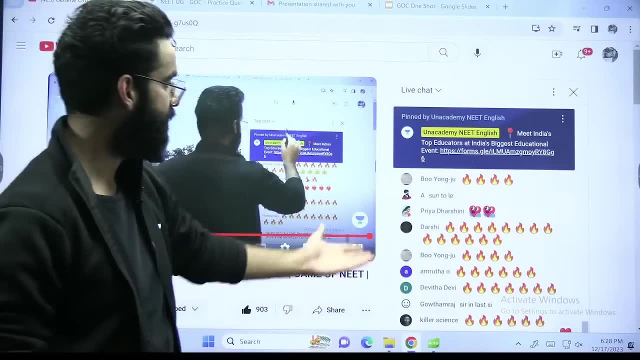 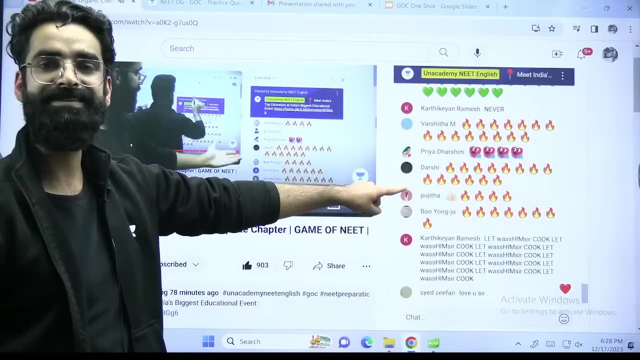 the chats again. wow, nice, good. okay, where are your live chats? here are your live chats, guys, i want the chats to run fast. what is this? what is happening? they are stagnant. right, the chats are stagnant if every single thing is clear till here. i want the chats to light up with the fire. 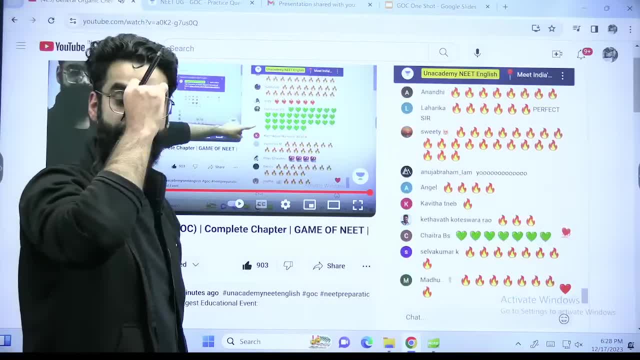 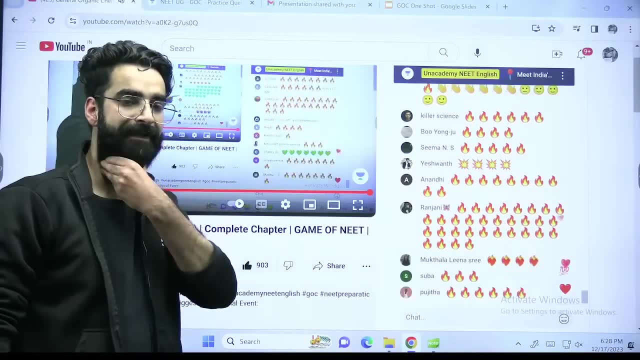 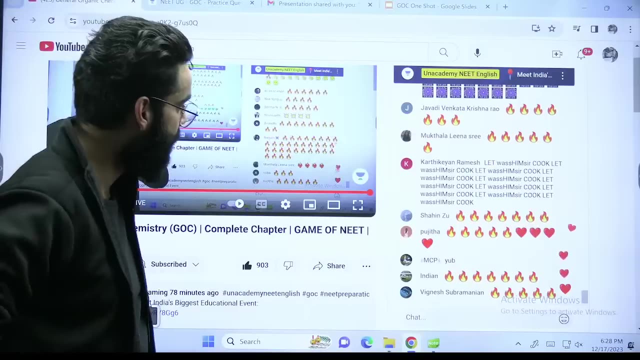 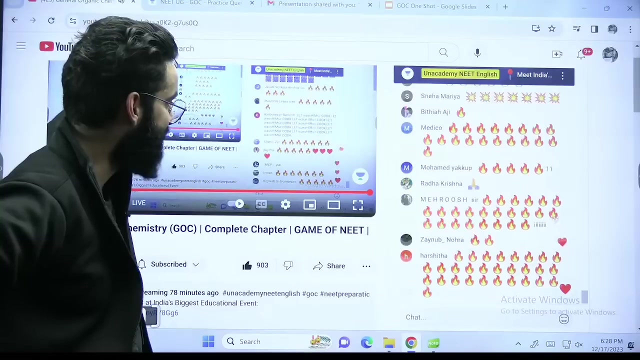 fire emoji, everyone, if every single thing is little- and i believe i've taught an entire death guys. yes, all clear, all clear. so we have got zee fun, we have got akshmi, we have got a lot of people. well, i am unable to see. now we have got suja, we have got killer science. killer science is a very old student. 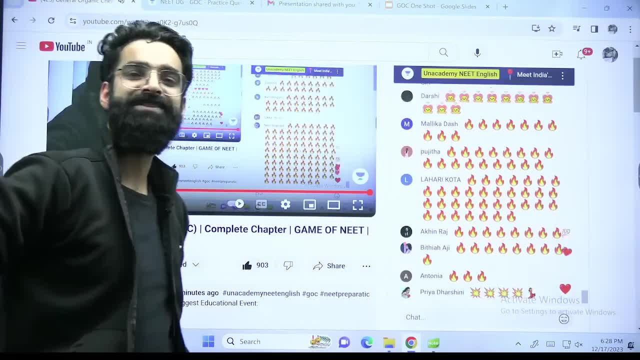 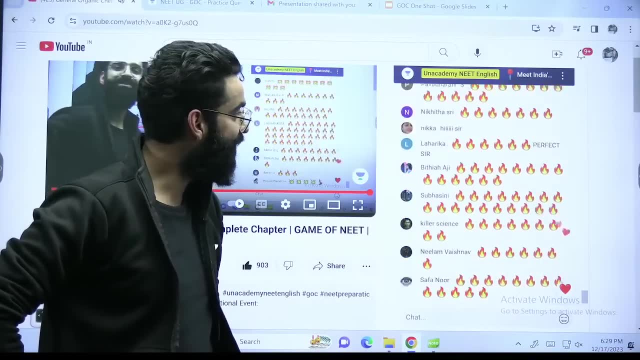 by the way, since we- it's been almost seven months we have started this channel and i have seen this killer signs guy from day one itself on this channel. wonderful, good. oh, we have got yawar manzoor sir as well in the chats. right, we have got yawar manzoor sir as well. 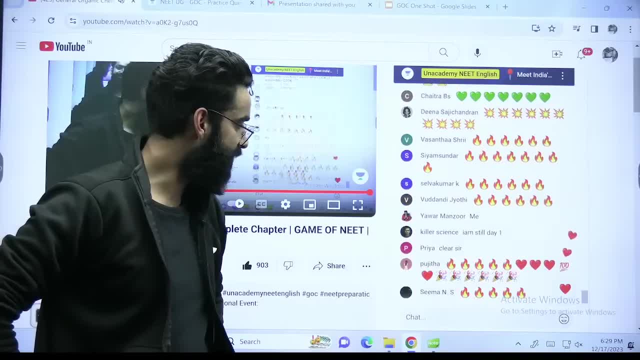 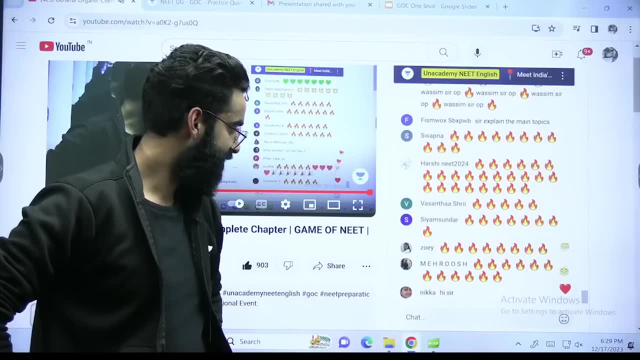 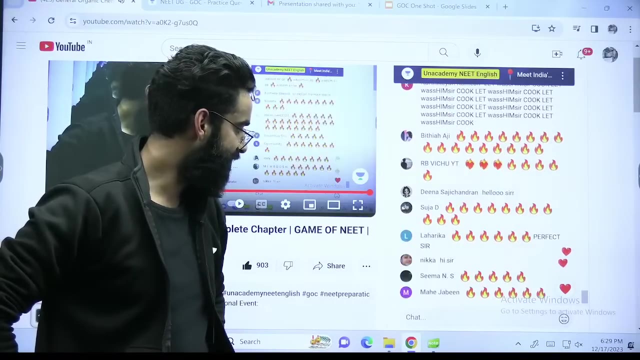 in the chats as well. Wonderful, We have got Selva Kumar as well. Selva is also an old student. Laharika is an old student. Nice, nice, nice, Good, good, good, Good. We have got Nikki, We have got Namrata, We have got Priya. All are regular students here. Good, 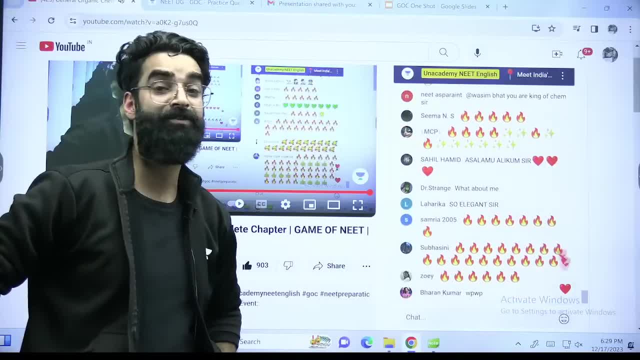 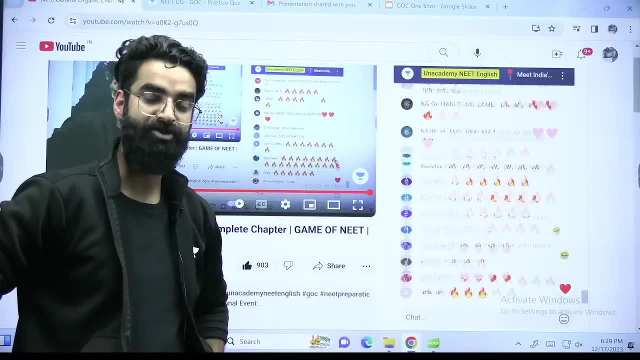 job, guys. I want you to be regular till the end. By the way, tomorrow we have got one more amazing session, guys, in the evening at 7.. I will be revealing one more important, one more amazing surprise with you Tomorrow at 7pm on this particular channel itself. 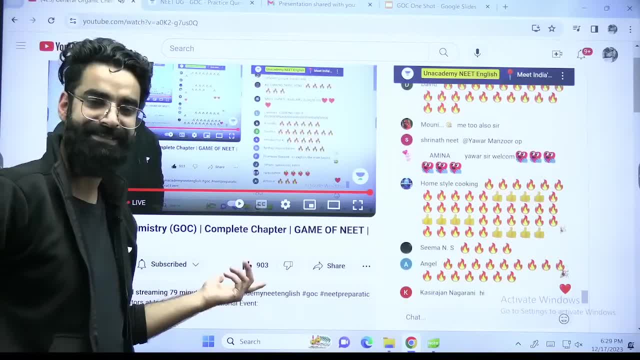 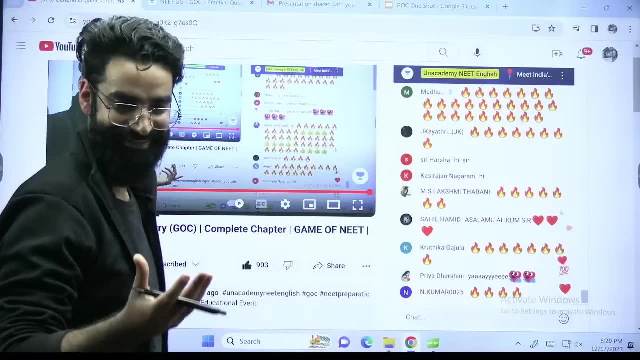 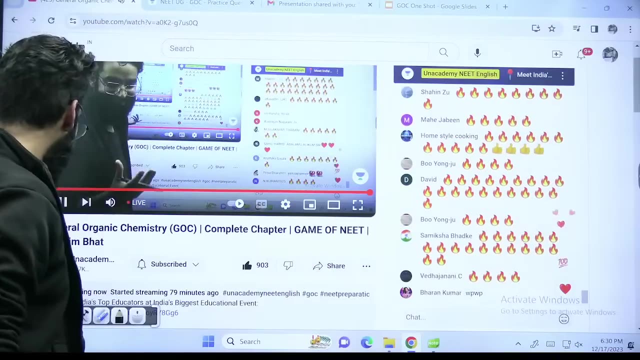 And I can see the likes are pretty much less. Why is it? Don't I deserve a single like from you, Right? Don't I deserve a single like, guys? Okay, so should we move on? So first step of the question is done and dusted, Let's move on now. Let's move on now. 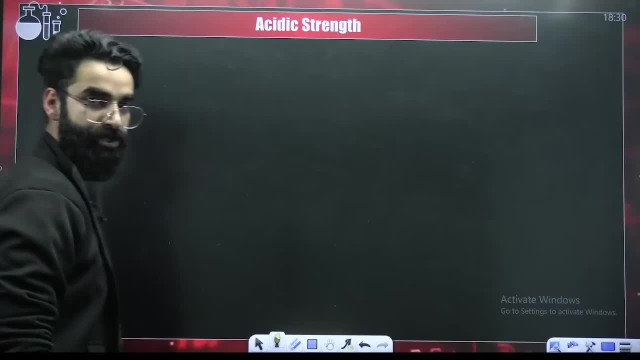 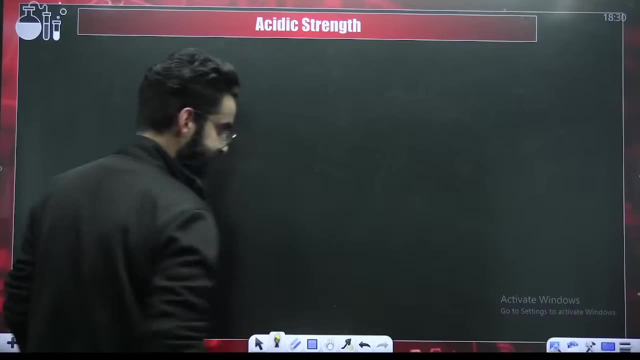 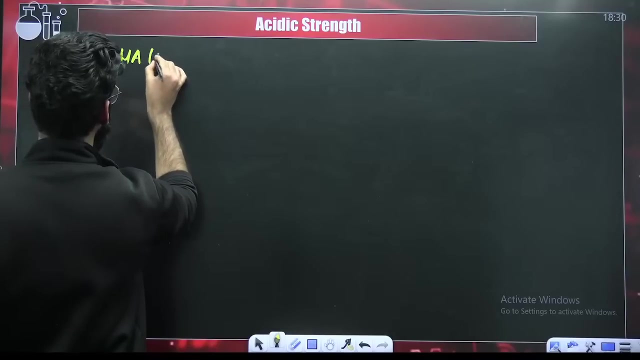 One more type of question: Acidic strength. Acidic strength- Try to understand what exactly I am going to say, My dear students. for example, I am going to take an acid over here. This is acid H-A-A-C-O-S. It is an acid. It is an acid, right, I will introduce the acid. 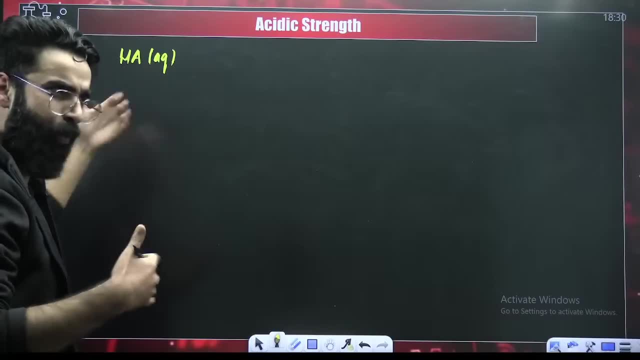 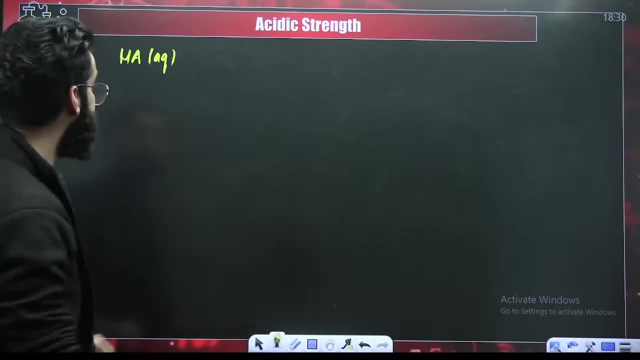 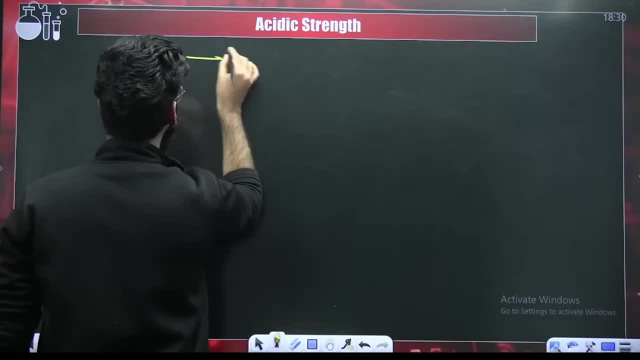 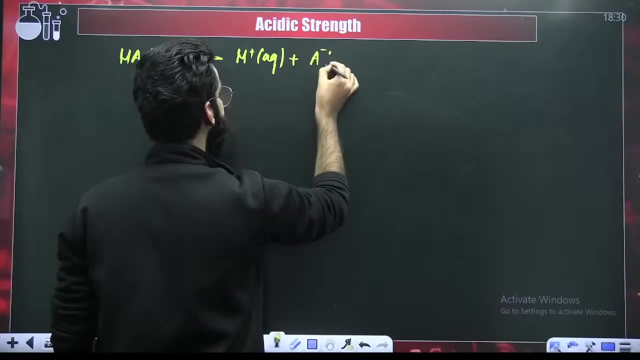 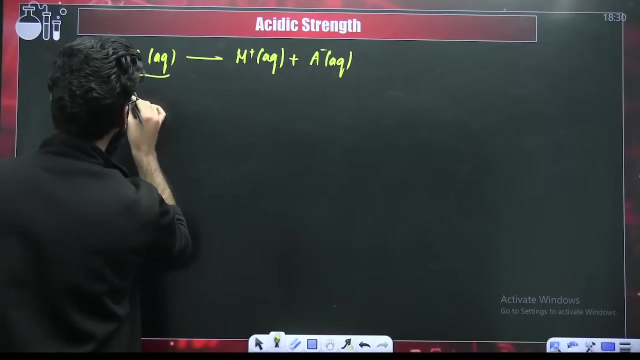 introduce this acid in water, it is going to donate what It is going to donate: H-positive. After donating H-positive, it is going to get converted into A-negative. After donating H-positive, it is going to get converted into A-negative. This is something which you were. 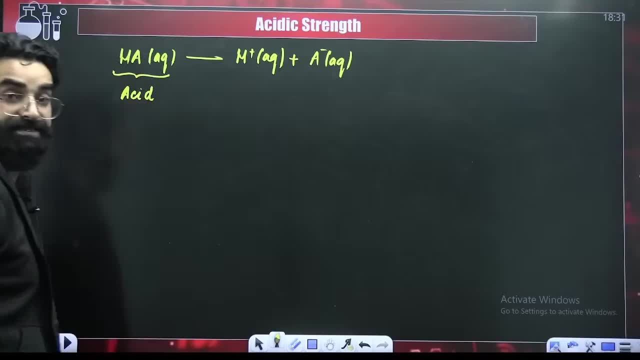 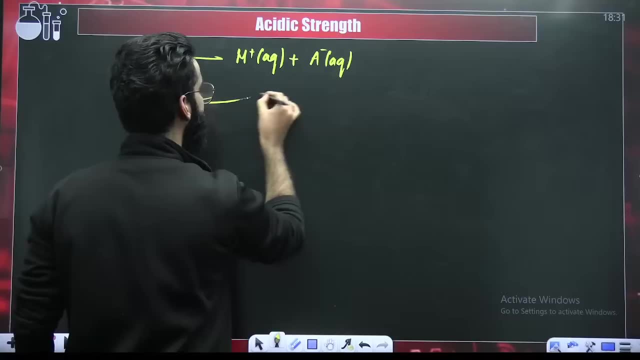 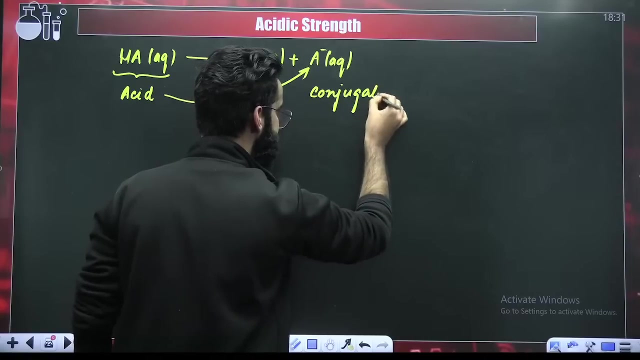 calling as acid. This is something which you were calling as acid And after the liberation of H-positive, after the liberation of H-positive, this acid, it got converted into A-negative right. This A-negative here I will be calling as the conjugate base. This is the conjugate base. 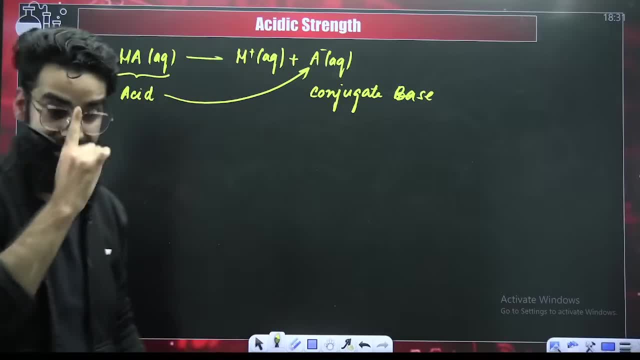 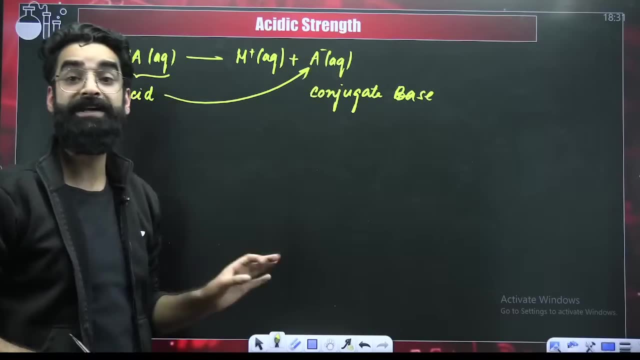 of the acid which I have taken over here. Right, This is acid Acid. after donating H-positive, it is getting converted into A-negative. This A-negative I will be calling as conjugate base here. This is something which I will be calling as conjugate base here. This is: 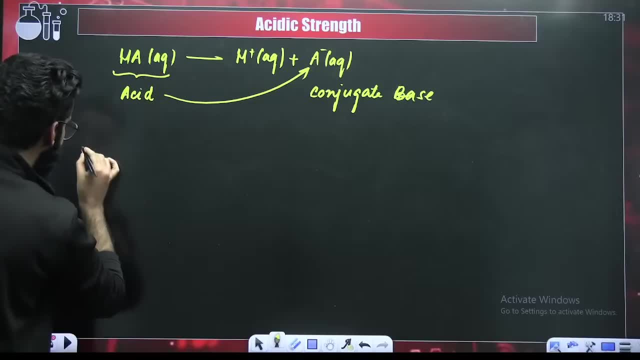 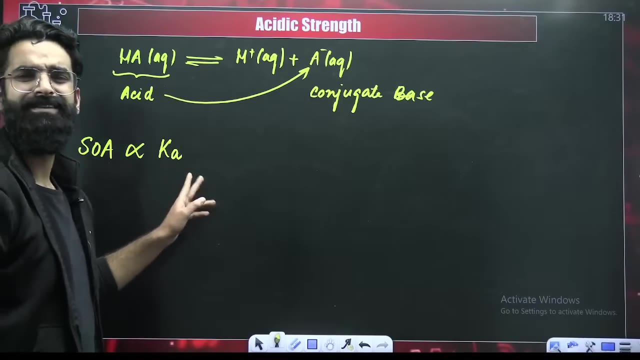 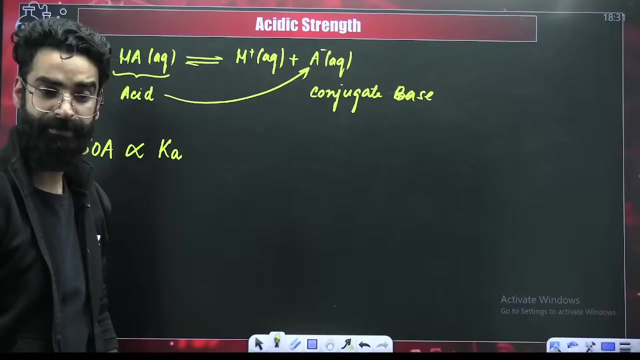 Solomon C Law Currently present. this A-negative is claiming abundance but it negates as군 to develop at all visiting assets from the relative plane of host. Now do remember, do remember. strength of the acid, Strength of the acid, Strength of the acid, people Strength of the acid. No front is directly proportional. 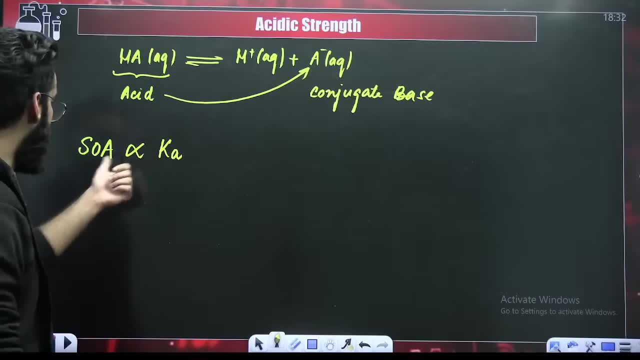 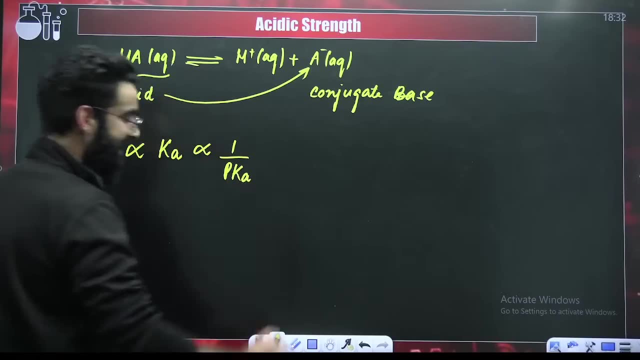 to Ka value. do remember- I believe that you would have studied Ka somewhere, The eigenvection directly, proportion to Ka, which is inversely proportional to P of Ka, which is inversely proportional to P of K. So, basically, there will be a set of questions which will be asked on. 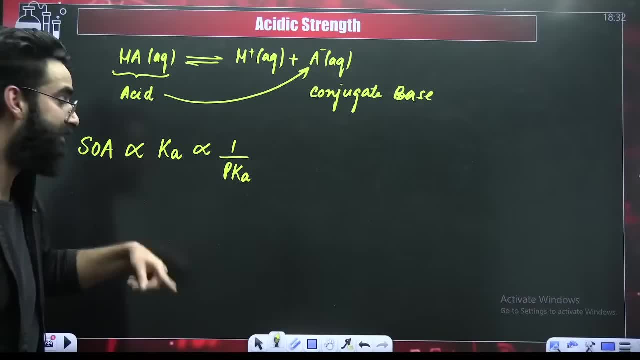 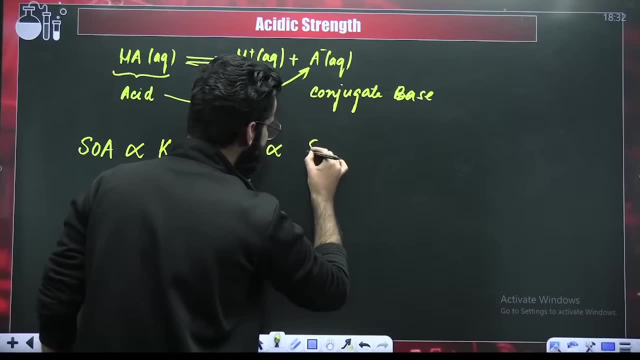 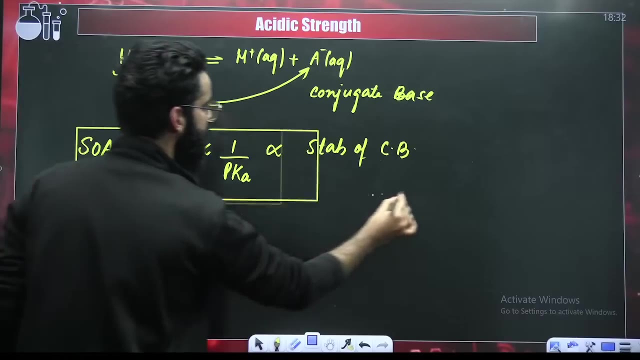 strength of acid. There'll be a set of questions which will be asked on Ka. There'll be a set of questions which will be asked on Pk. Now, do remember: strength of acid is directly proportional to the stability of the conjugate base. This is the only statement which I would want you guys. 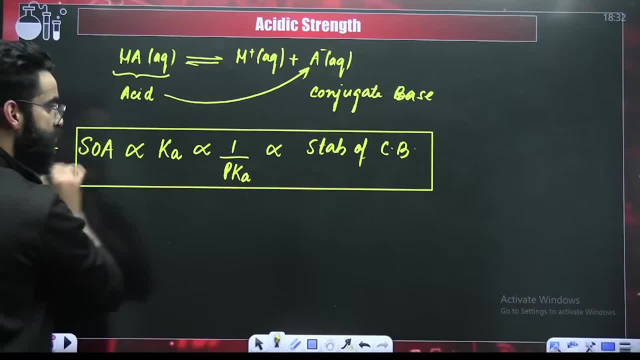 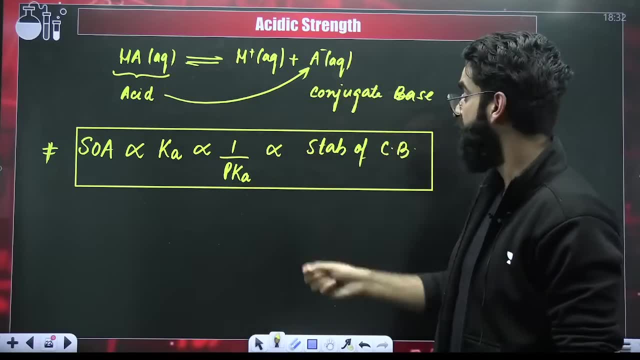 to remember here. strength of the acid. it is directly proportional to the stability of the conjugate base. strength of this acid is directly proportional to the stability of its conjugate base. more stable the conjugate base, stronger the acid, more its ka value, less its pka value. 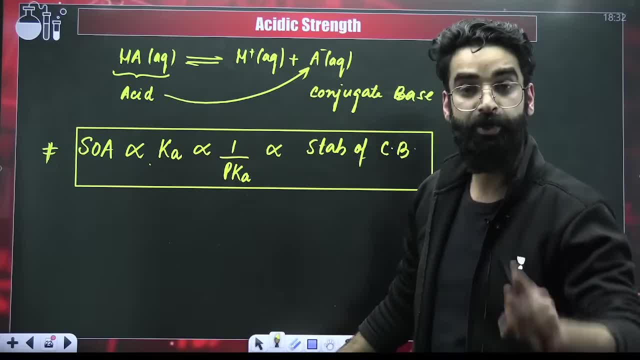 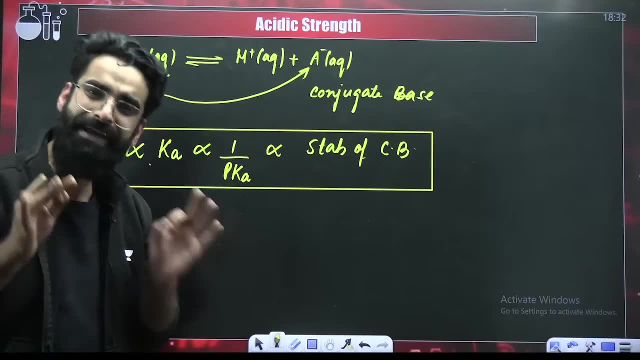 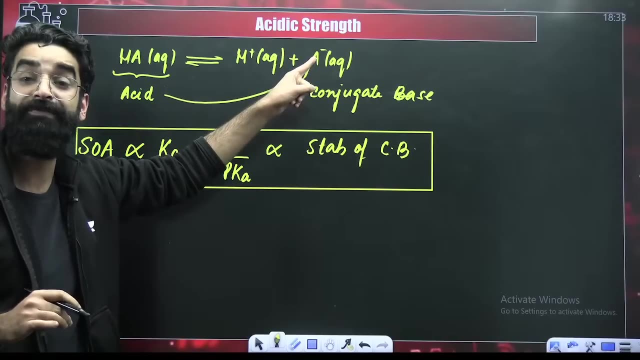 simple as that, right, don't remember this. strength of acid is directly proportional to stability of conjugate base. now i'm going to do many equations on this particular one statement. strength of the acid is directly proportional to stability of its conjugate base. right, just remember it and have a look see how i'll be dealing with equations. 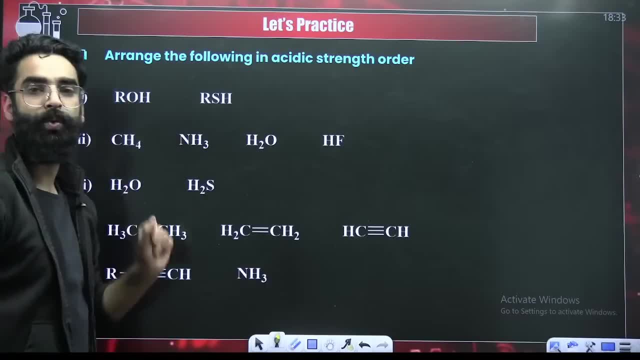 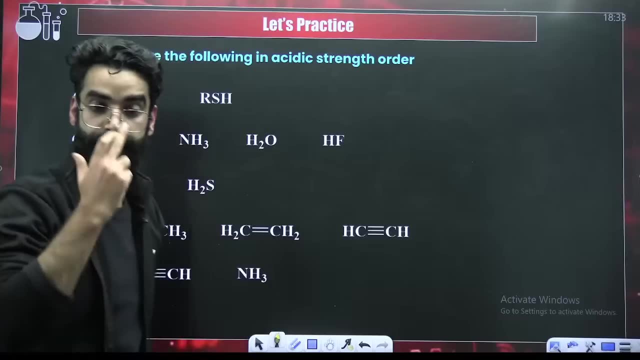 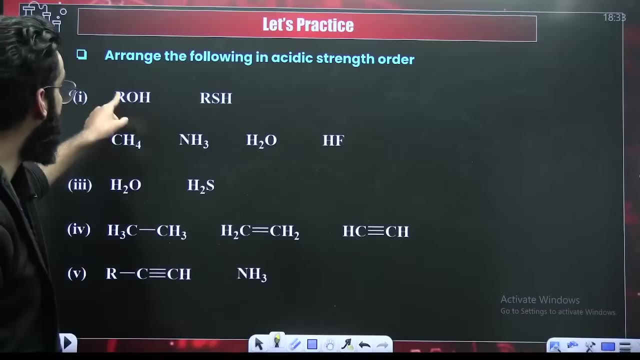 my dear students, among these two, you have to identify which acid is stronger, roh or sh. which one is stronger among the two, which one is stronger among the two, the concept which i gave you. right now you're going to utilize that concept itself: roh or sh which? 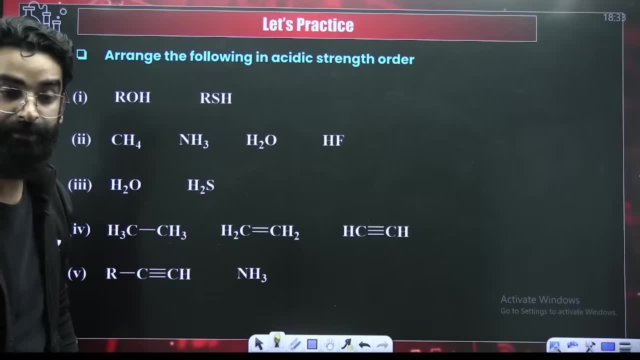 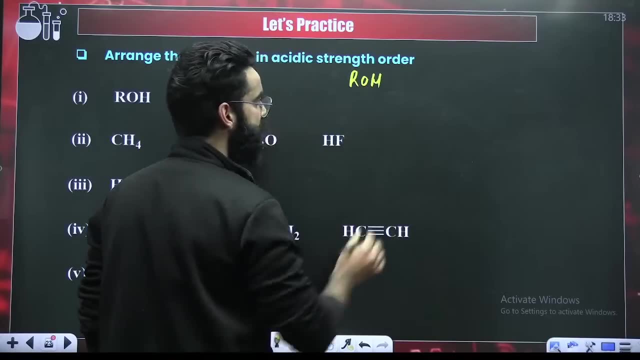 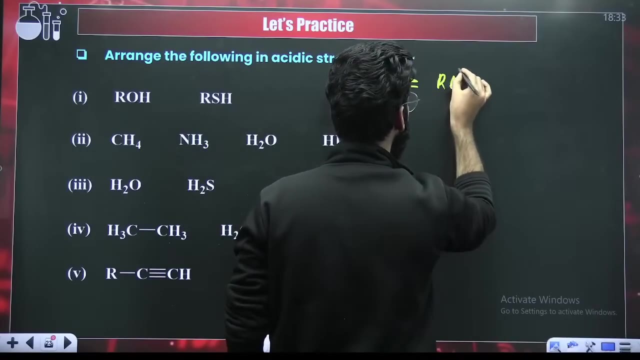 one is more acidic? which one is more acidic? how exactly you're going to do it? try to understand, first of all, if i talk about roh. if i talk about roh, my dear students, after, after the liberation of h positive, after the liberation of h positive, the conjugate base which we get over here, that is: 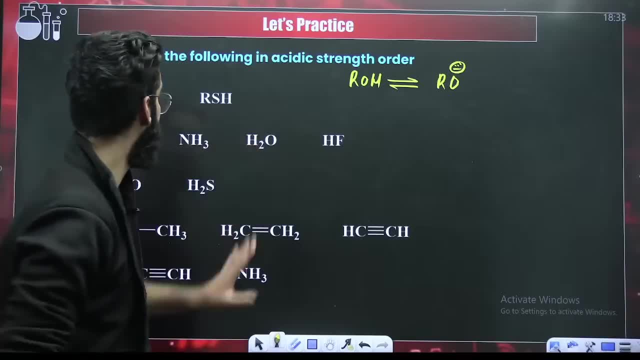 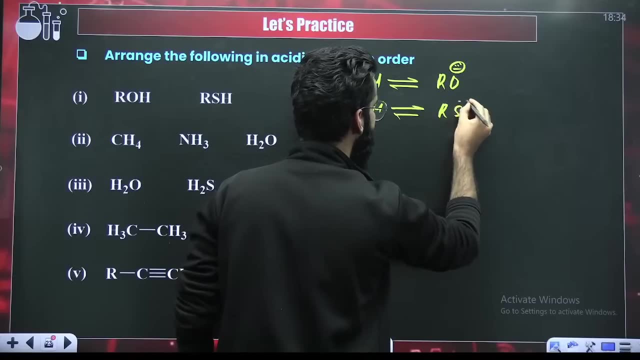 ro negative. ro negative is the conjugate base of this acid. similarly, we have got rsh after the liberation of h positive. after the liberation of h positive it gets converted into rs negative. so i made their conjugate bases. i made their conjugate bases. now look at the stability of 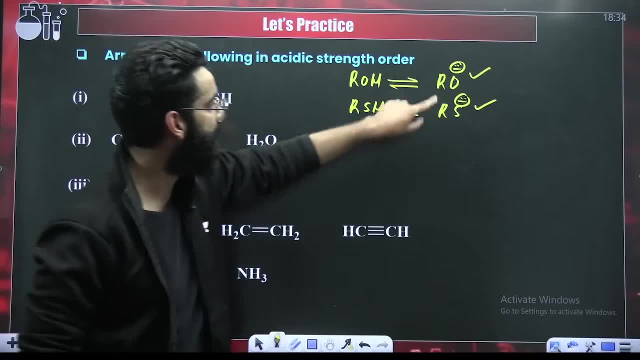 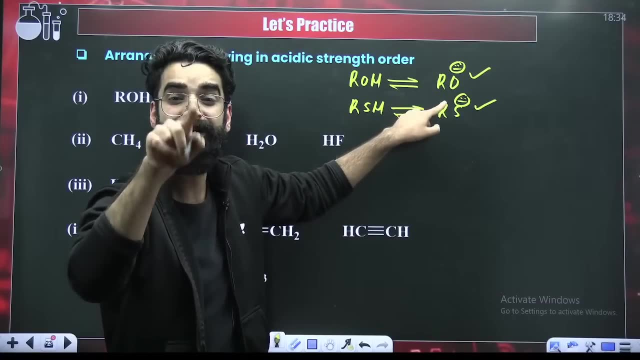 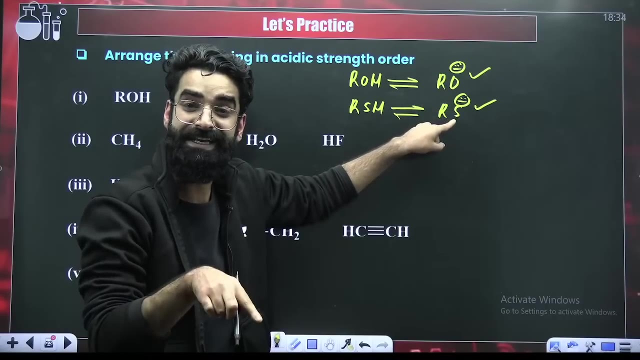 these conjugate bases. look at the stability of these conjugate bases. tell me, oxygen carrying negative sulfur, carrying negative oxygen carrying negative sulfur, carrying negative oxygen and sulfur- same group. vcd plays a role. vcd plays a role. more the more the size. less the vcd, more the stability. 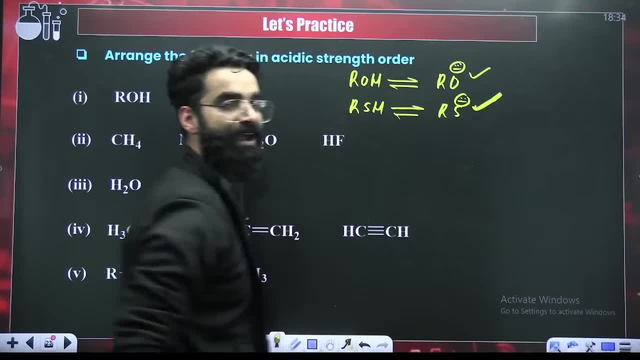 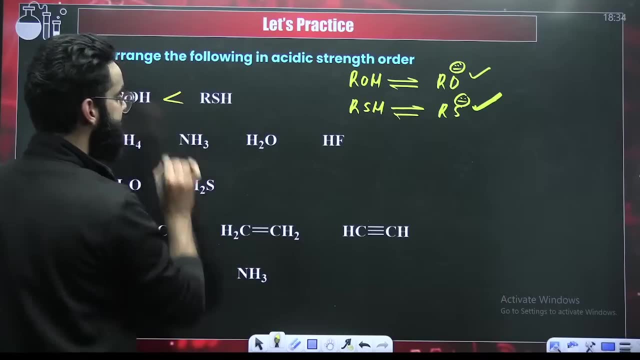 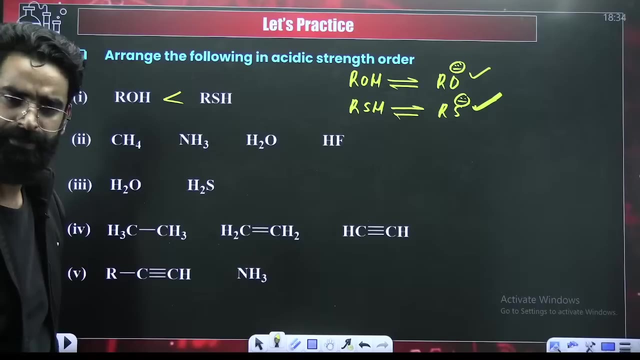 so this conjugate base is more stable and that acid which gives more stable conjugate base, strength of that acid will be more right. so which acid is stronger? rsh is stronger than roh. simple, yes, simple. the kind of concepts which i gave you. i'm utilizing those concepts, only i'm not. 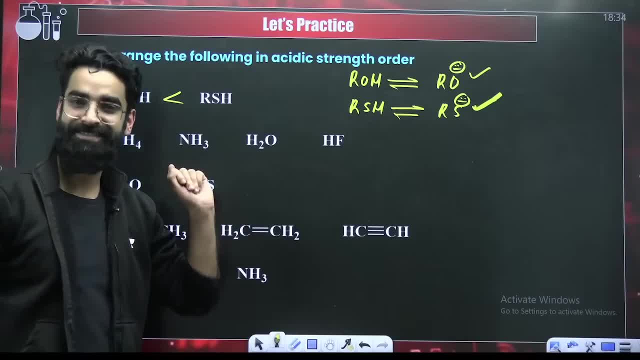 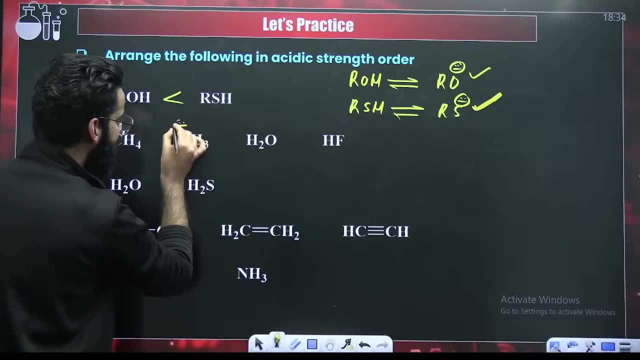 something new. look here: make their conjugate bases. make their conjugate bases first of all. take h positive out from here, you'll get- you'll be getting- a negative one. carbon: take h positive out from here, you'll be getting negative. on nitrogen, take h positive out from here. 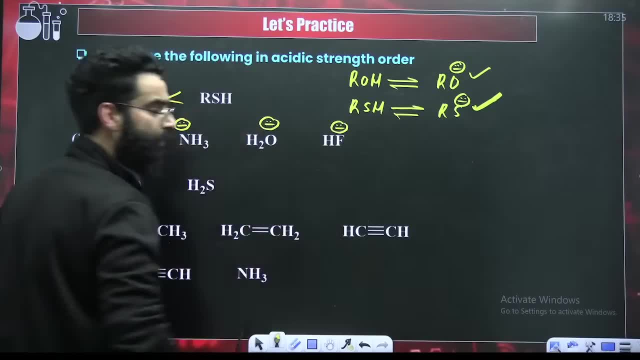 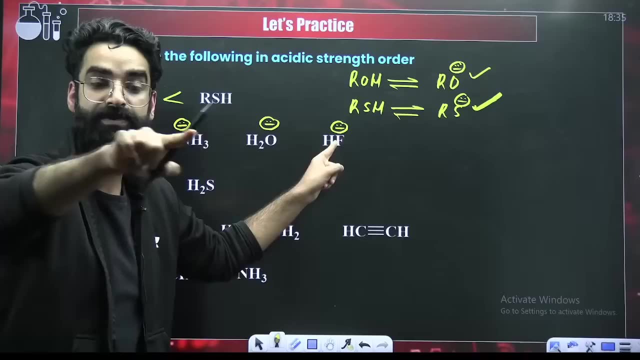 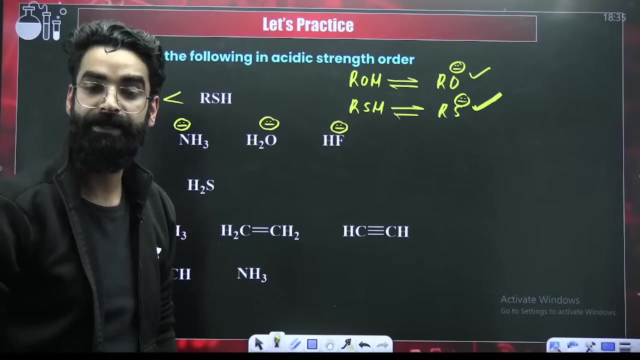 you'll be getting negative oxygen. take h positive out from here. negative on fluorine, negative on fluorine. now you tell me carbon with negative nitrogen, negative oxygen, negative, fluorine negative. all these elements they belong to same period. in the period we talk. in terms of electronegativity, negative charge is more stable. on more electronegative, negative charge is more. 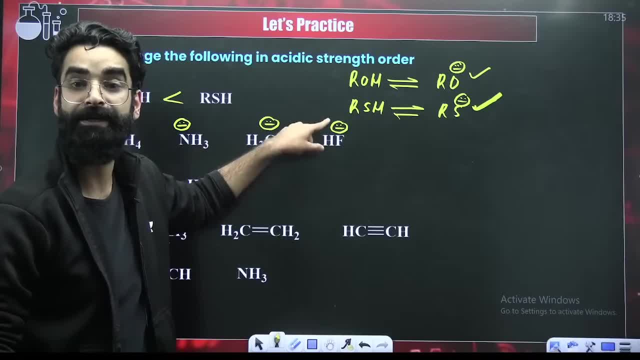 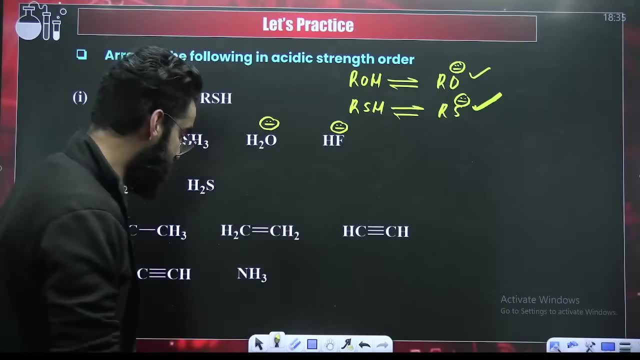 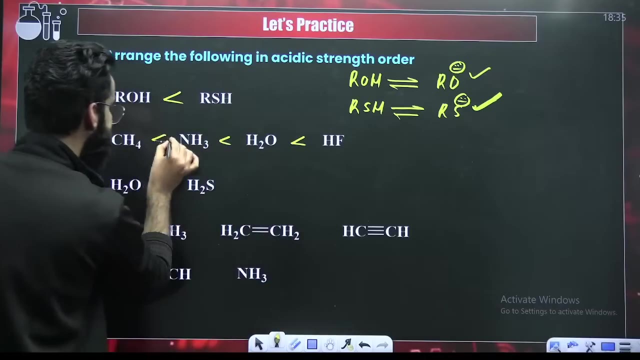 stable on more electronegative, so negative charge will be more stable on fluorine. so the conjugate base which you get from hf, that is more stable if the conjugate base is more stable. if the conjugate base is more stable, i would say the acidic strength of these acids will follow the same order. 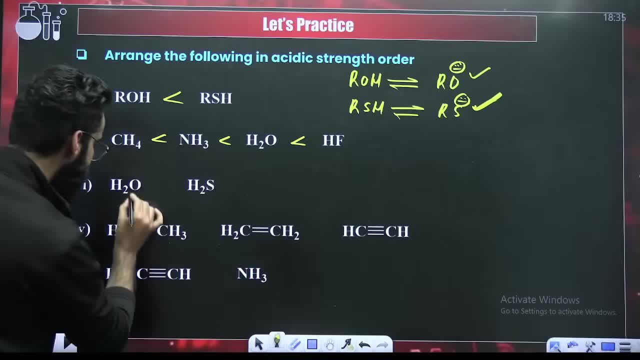 done and dusted absolutely h2o, h2s. take h positive out, there'll be a negative charge on oxygen. take h positive out, negative charge on sulfur right if? on taking h positive out, negative charge on oxygen. on taking h positive out, negative charge on sulfur. 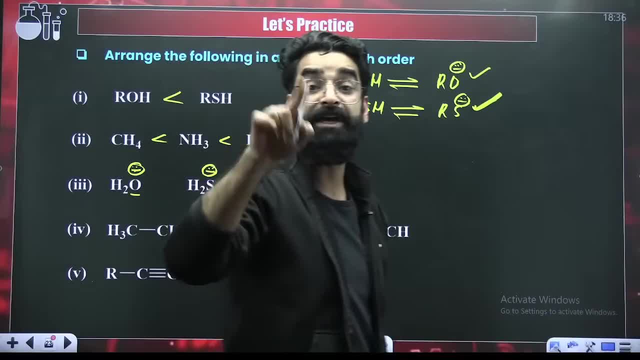 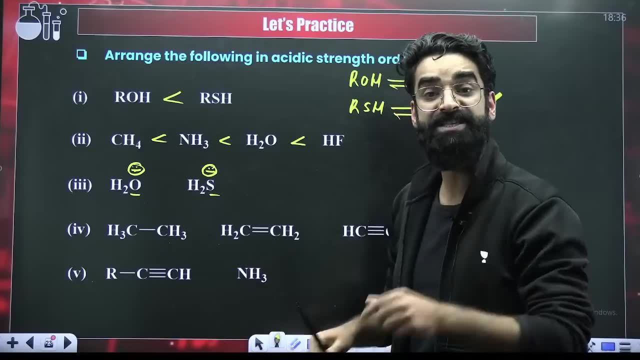 Now look at oxygen and sulfur. Oxygen, sulfur, same group In the group VCD, More the size, more the size, less VCD, more stability. So the conjugate base which I get from H2S that is more stable. 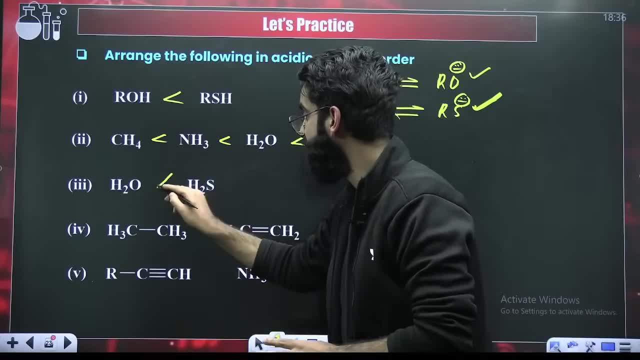 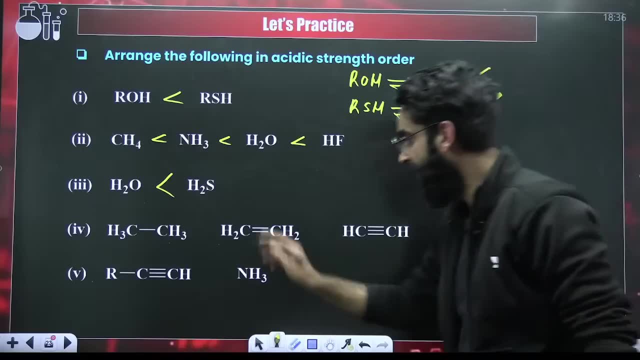 If that is more stable. if that is more stable, that means this has to be the strength of these acids. Right Done, Look at the next one. Look at the next one. Say: take H-positive out from air. carbon will carry negative 2.. 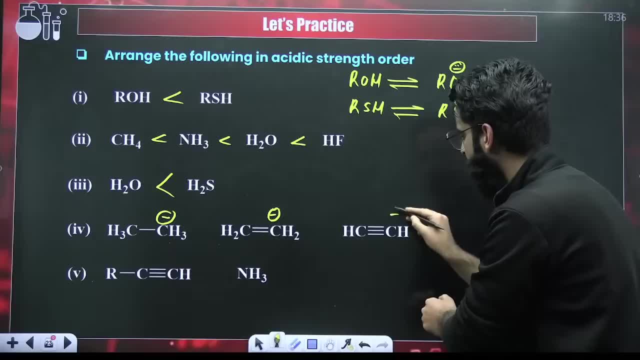 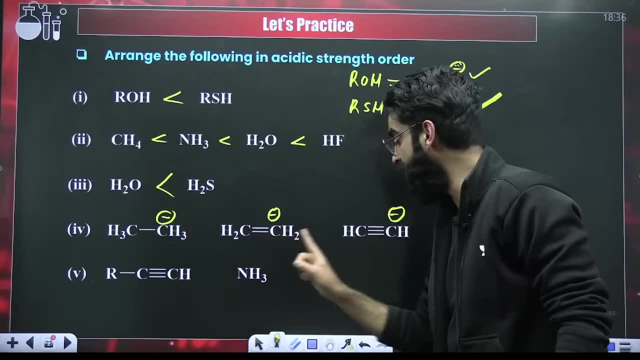 Take H-positive out from air, This carbon will carry negative. Take H-positive out from air, This carbon will carry negative. So you have made the conjugate bases. Now see Single bonded carbon, double bonded carbon, triple bonded carbon. 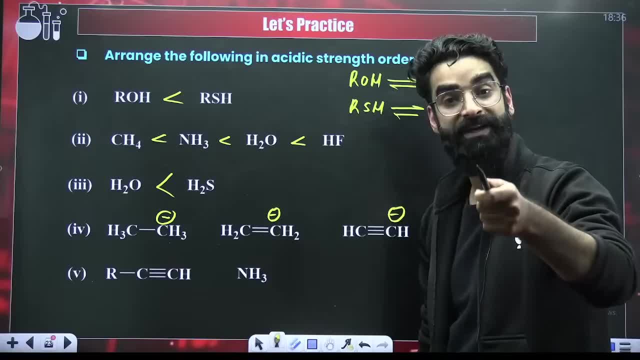 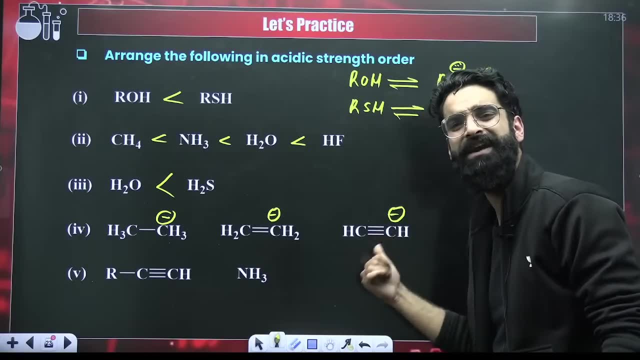 Triple bonded carbon has got more S-character. More S-character means more electronegativity And you know Nagiru charge is more stable on more electronegative. So the conjugate base which you generate from air, that is maximum stable. 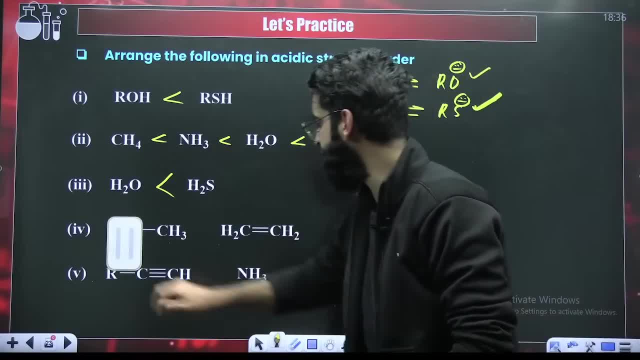 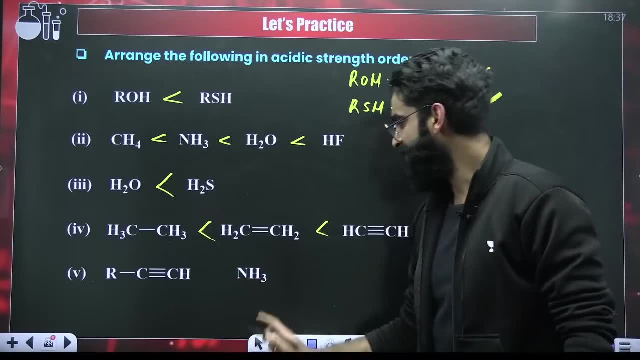 And more stable the conjugate base, better is the acid, More is the strength of the acid. So this is the Acidic strength Order. Yes, Okay, Tell me about this one. Tell me about this one quickly. This is H here. 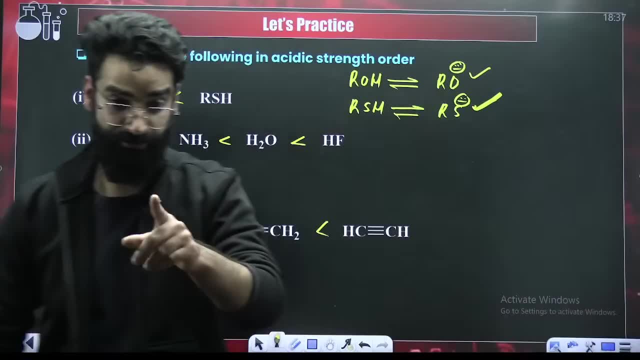 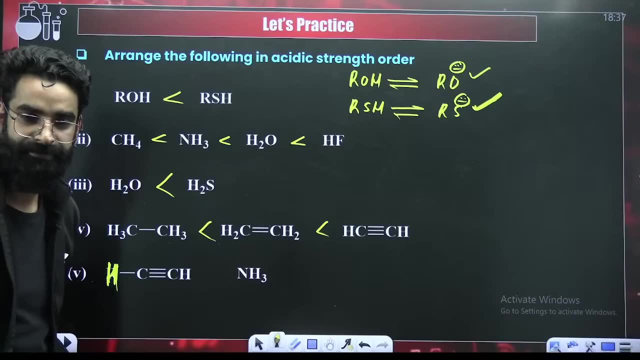 Tell me about this one. Among these two, which one is more acidic? You have to tell me the answer. Among these two, which one is more acidic? You have to tell me the answer. Dr Strange, you need to watch this session from the beginning. 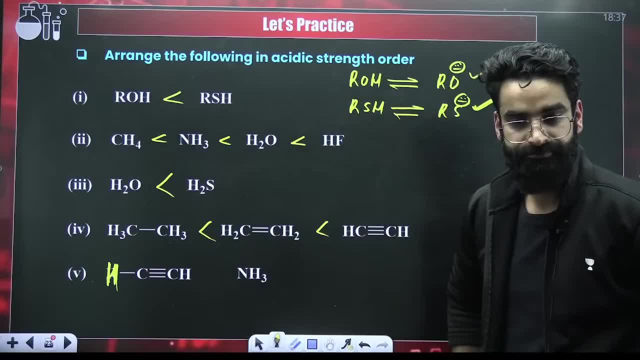 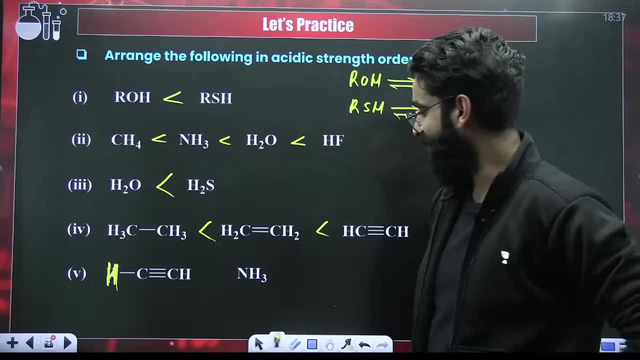 Then you will get to know what is S-character. Which one is more acidic, Guys? this concept also, I have given you This concept also. I have given you This concept I have given you too. Which one is more acidic? You have to answer me this. 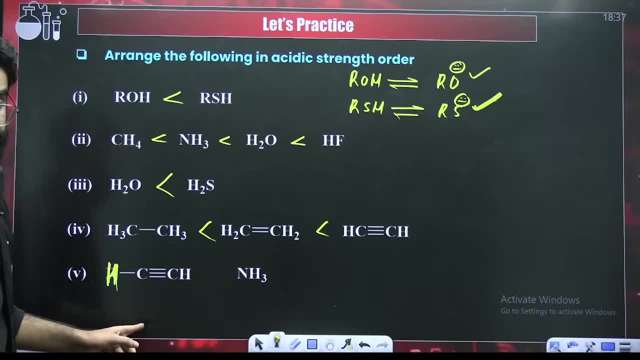 And the answer has to be correct. It has to be appropriate. If you give the wrong answer here, it will be a heartbreak for me. It is actually going to be a heartbreak for me if you give the wrong answer here. I can see majority has given the correct answer. 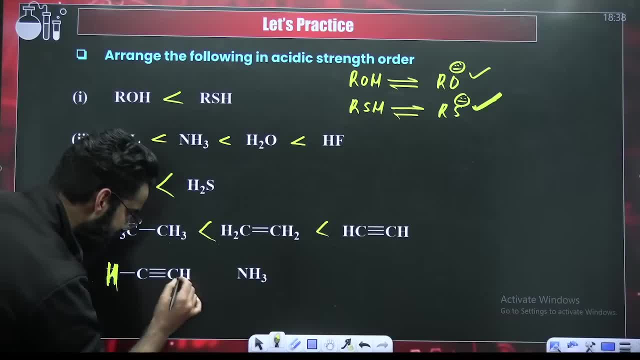 Wonderful, Good job, Hey guys. what you will be doing: Make their conjugate bases. Take H-positive out from here. You will be getting something like this: H-C triple bond, Carbon carrying negative. Take H-positive out from here. 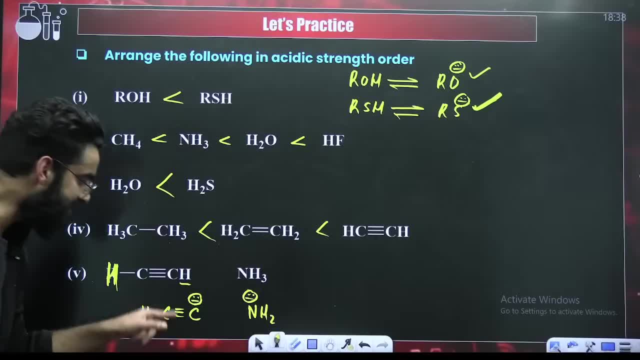 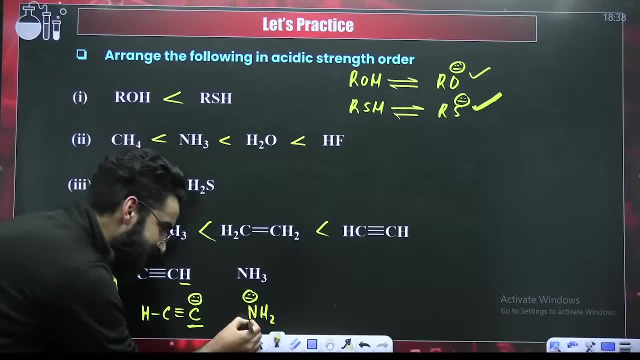 It is going to be NH2 carrying negative Right Now. these are the conjugate bases. These are the conjugate bases. Look at their stability. This is SP hybridized carbon. This is SP3 hybridized nitrogen. Electronegativity of SP hybridized carbon is more. 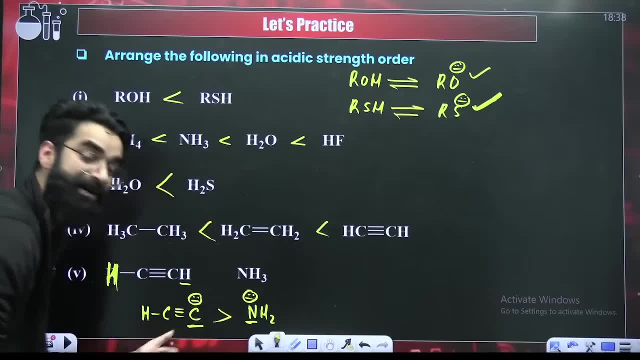 And you know negative charge is more Sib on more Electronegative. So this is the stability order of these conjugate bases. And whatever is the stability order of the conjugate bases, same is the order of their acidic strengths. 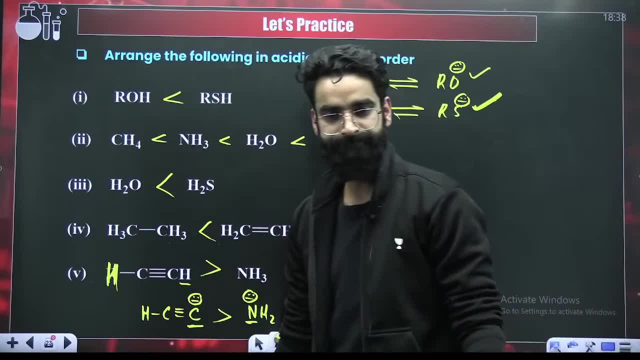 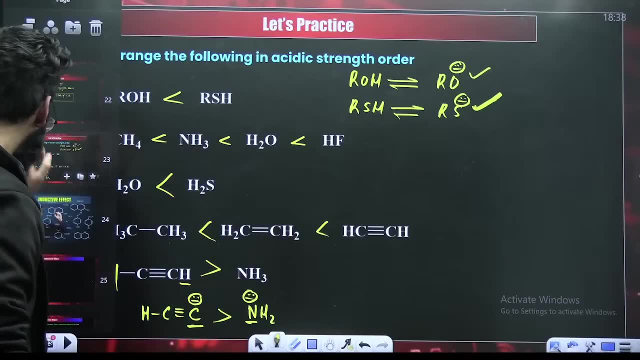 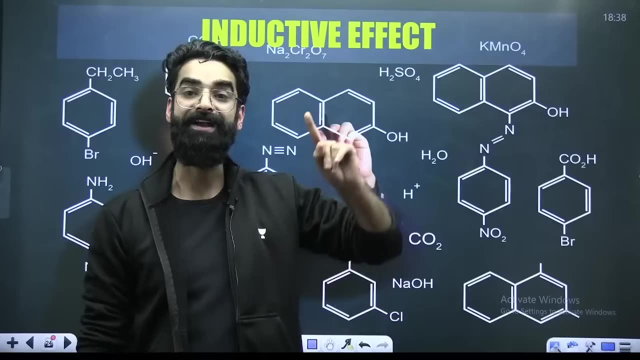 Done and dusted Right. Yes, Is it clear. I believe every single thing. Whatever I have taught you till now is clear. So the basics which was required to learn the general organic chemistry, that is clear. And by learning the basics you could solve two types of questions. 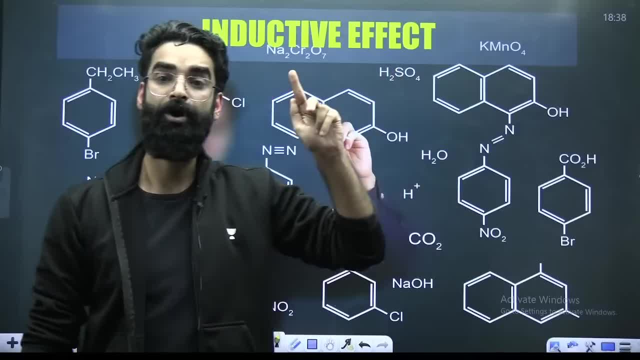 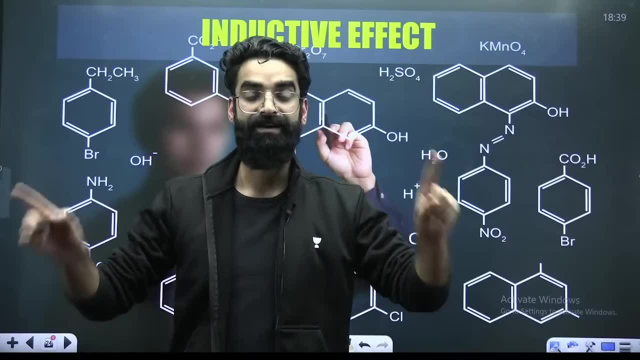 By learning the basics you could solve two types of questions. First question, on the basis of First question, was stability of charges on different species. Second question was the acidic strength. Remember acidic strength is directly proportional to stability of conjugate base. 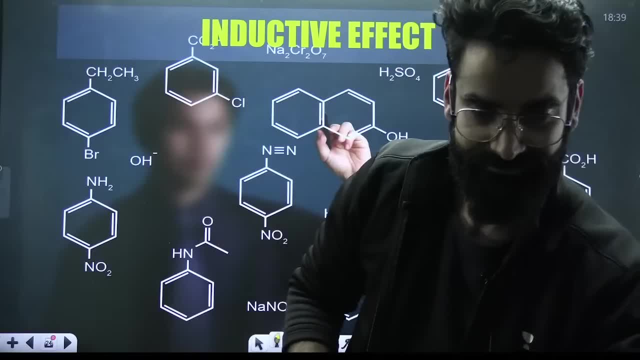 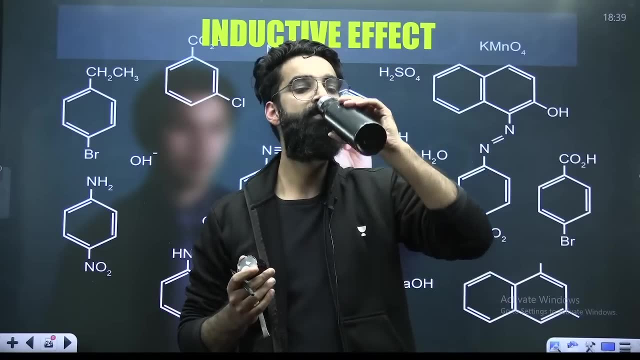 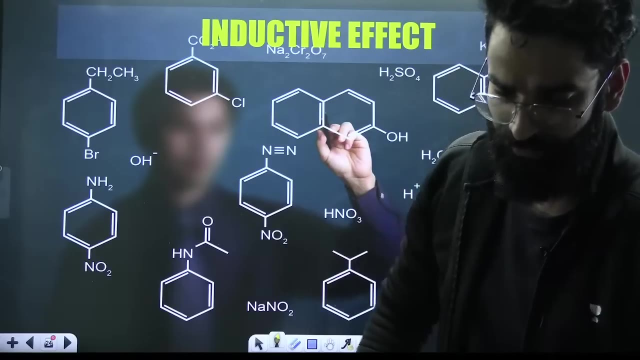 Nothing else you have to remember. That's it. Is it clear? Are you ready for the inductive effect now? Are you ready for the inductive effect? Are you ready for the inductive effect? I want the chats to move fast. 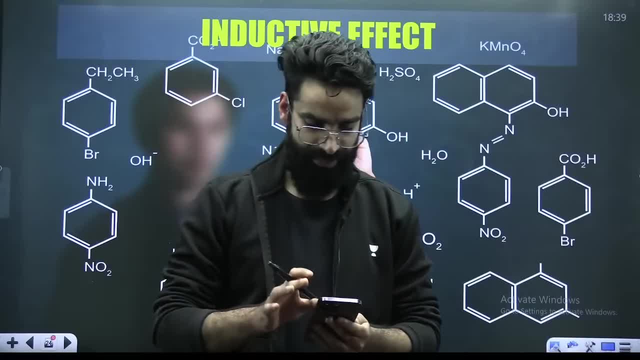 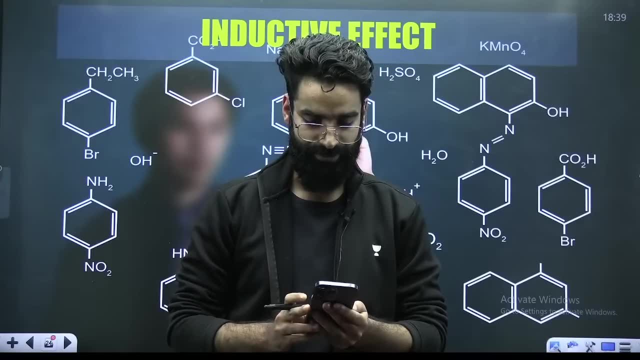 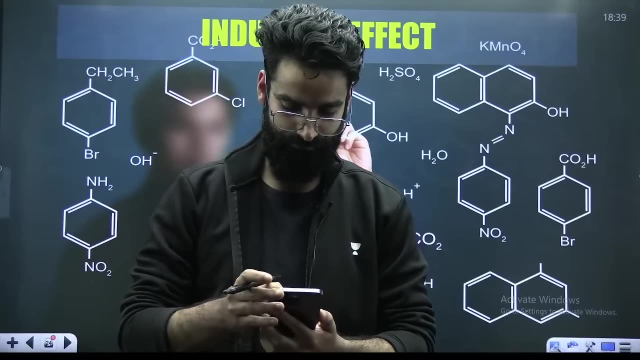 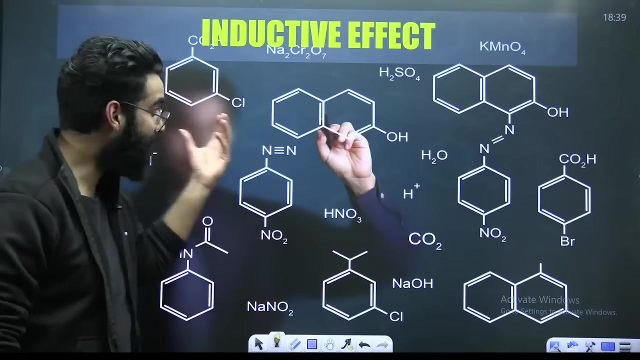 They are pretty slow. I want the chats to run fast. They should run, They should not walk, They should run, They should run, They should run. Yes, Basic strength questions will be given too, But wait for it. We have to do certain concepts first. 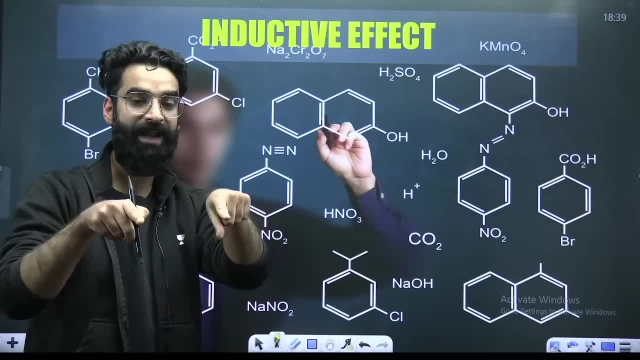 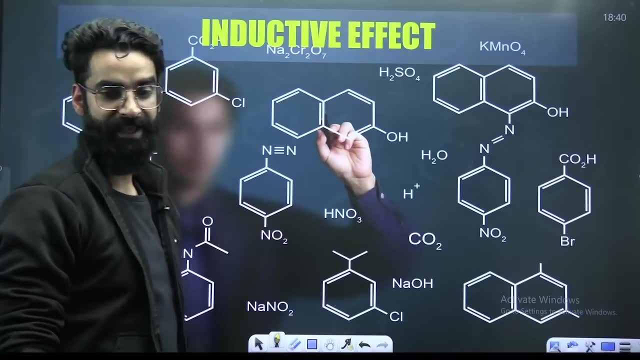 But wait for it. We have to do certain concepts first And the ones again who have not liked the session yet like the session right now. I want the likes to be more than 1k quickly. I can see not everyone has done that. 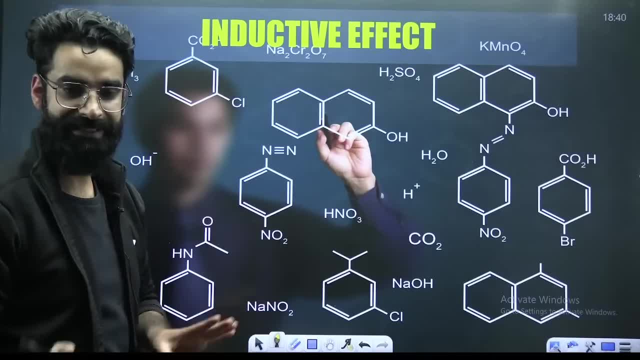 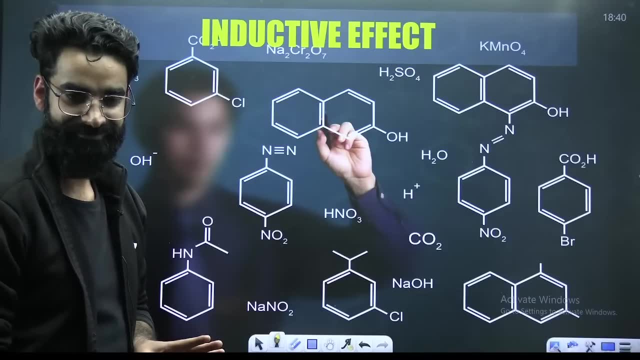 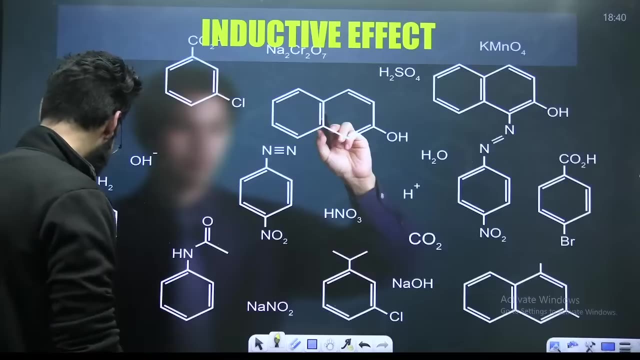 Guys, it does not. I mean you need not to pay for the likes, it's free. Yeah, It is free, But when you enter into your medical college, then I'll make you pay. okay, Just remember that When you enter into your medical college, I'll make you pay. 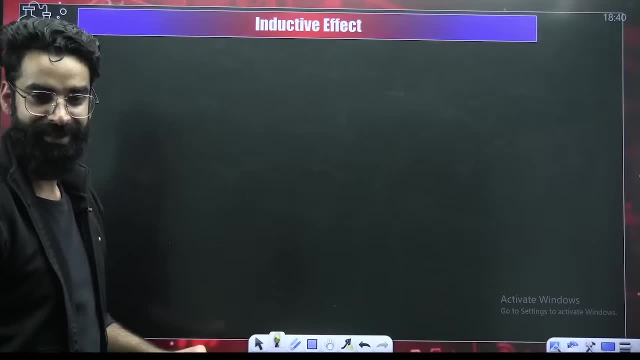 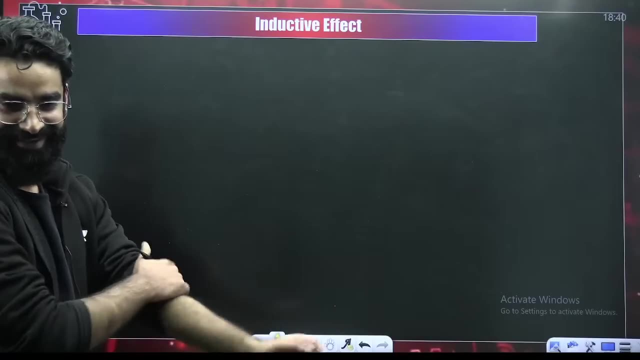 For whatever I've done on YouTube, whatever the team has done on YouTube. Yeah, And I believe at that time you should And you will, And I'll make sure you do. Okay, Perfect. So, guys, let's move on to something called as inductive effect. 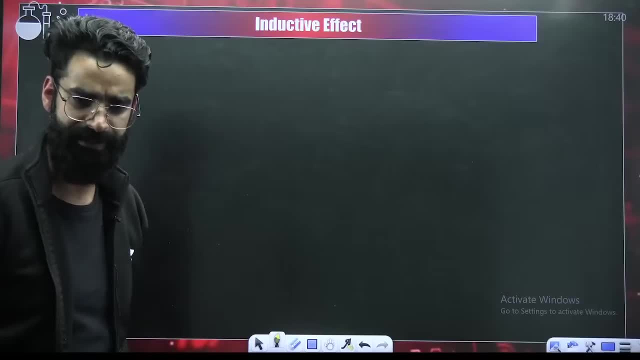 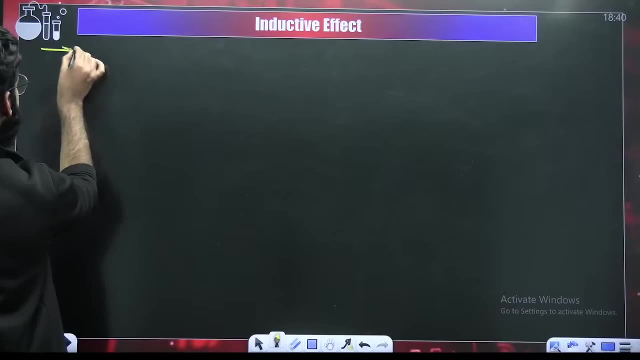 This is again one important concept and simple at the same time. Simple at the same time. Have a look: How do you exactly define the inductive effect? I guess, students, I'll be writing. I'll be writing a simple statement over here. 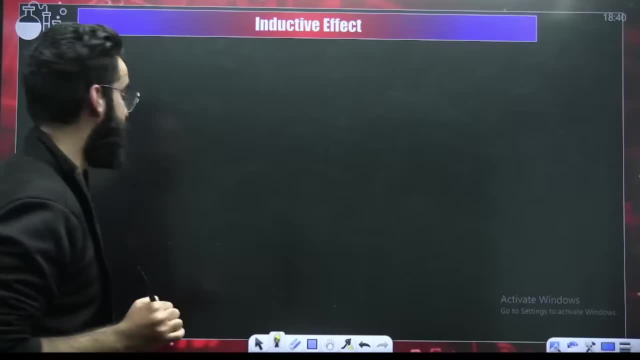 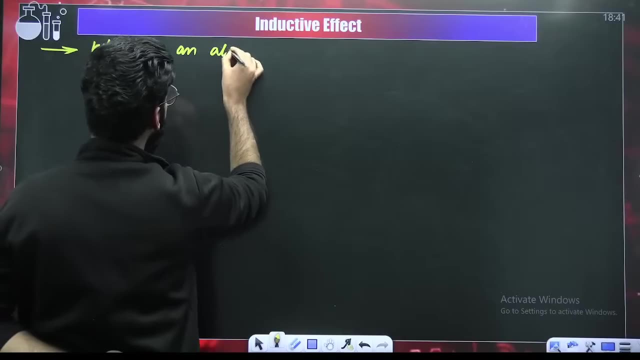 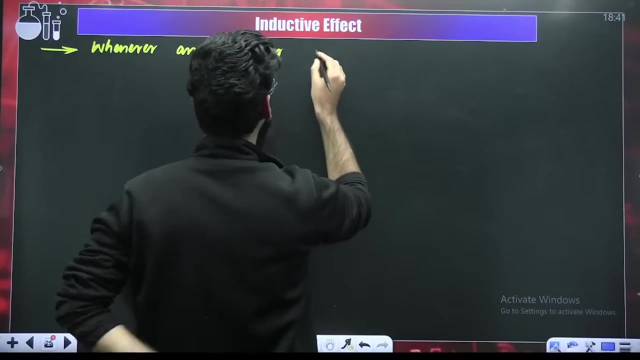 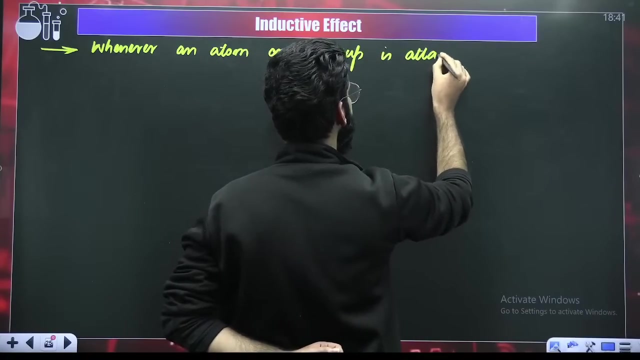 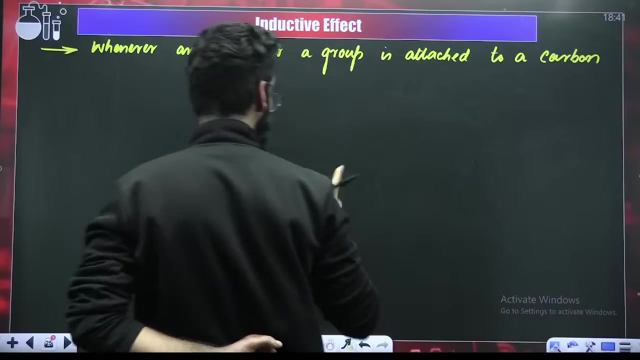 Then I'll make you understand what that statement exactly is all about. Inductive effect: Whenever, Whenever an atom, or Whenever an atom, or Whenever an atom or a group, A group is attached, Is attached to a carbon chain. Whenever an atom or a group is attached to a carbon chain. 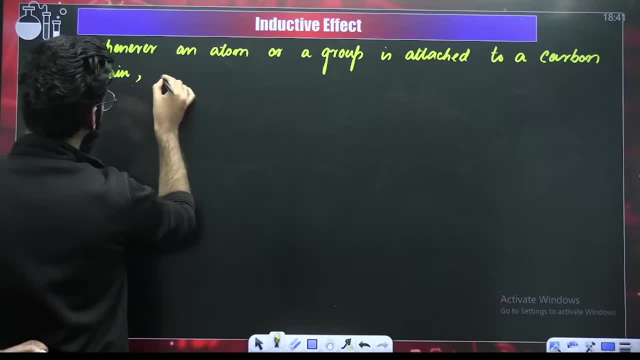 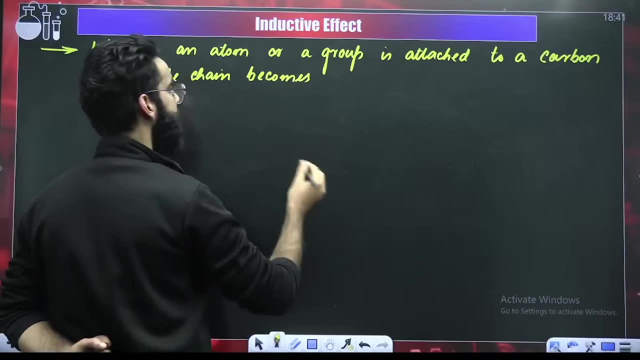 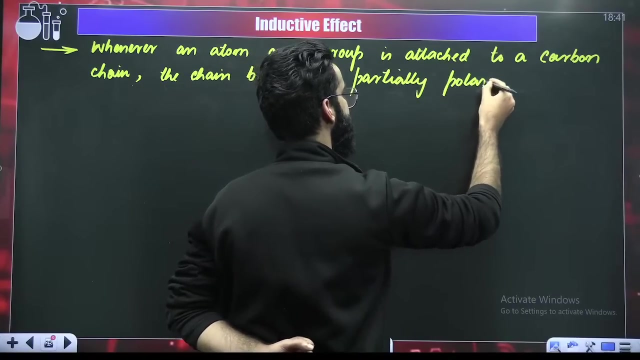 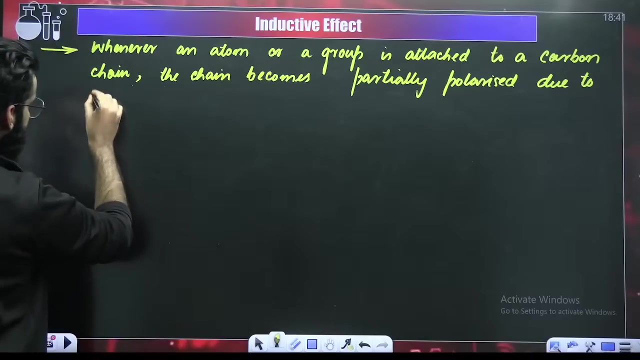 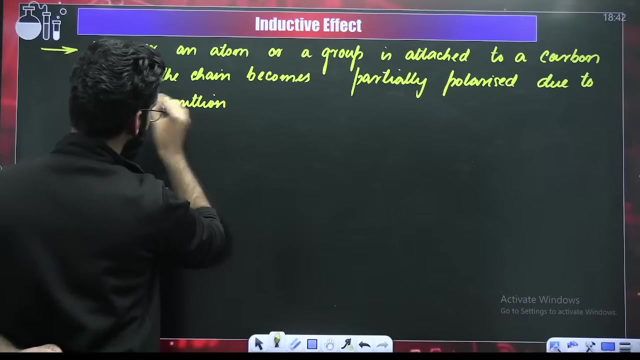 Is attached to a carbon chain, The chain becomes partially polarized. The chain becomes partially polarized Due to the transmission of sigma electrons, due to due to the transmission. due to the transmission of sigma electrons, or let me write, due to the transmission of sigma. 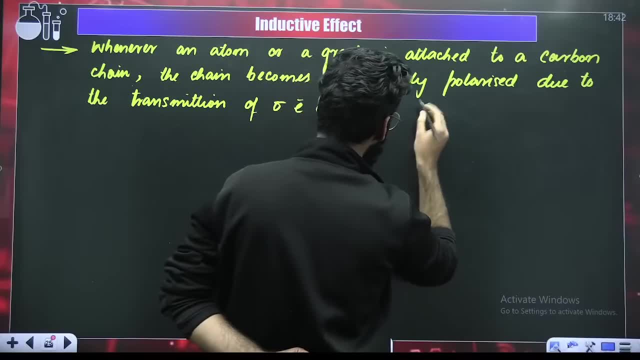 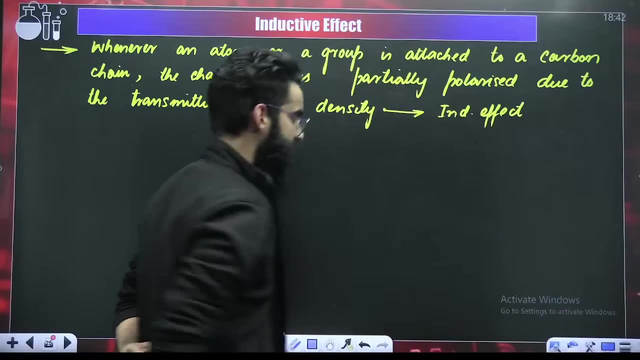 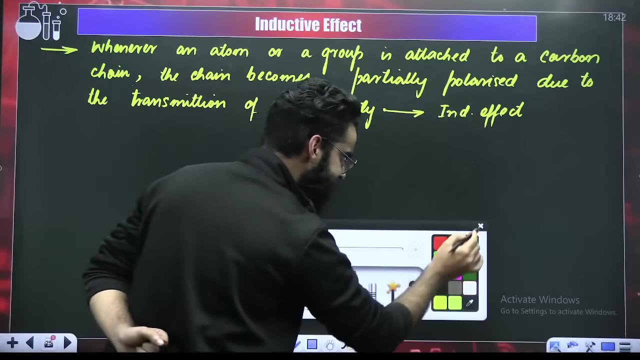 electron density. this effect is something which we call as inductive effect. this effect is something which you call as inductive. now, what does it mean? how can we understand this? how can we understand this? how about people? for example, i'm taking a carbon chain over here. let's assume you have got. 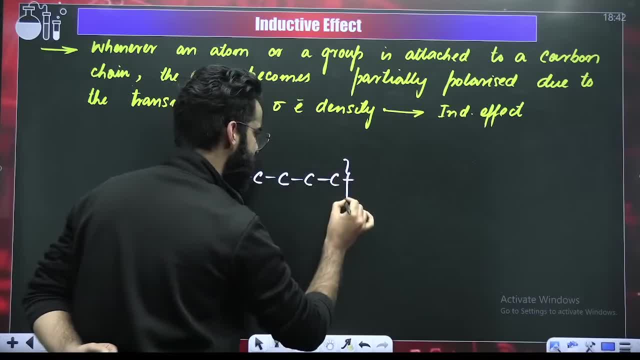 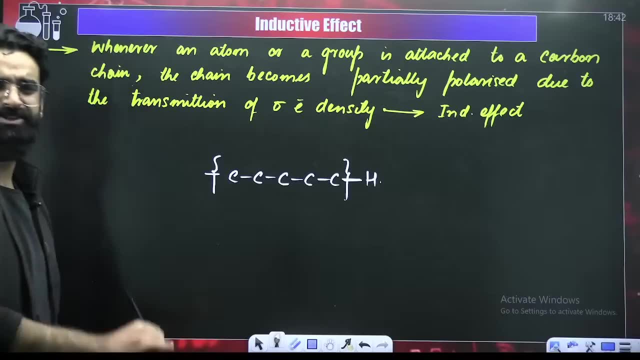 this particular carbon chain? right, this is the carbon chain which we have. okay, this is the carbon chain which we have. and this particular carbon, imagine it is attached with hydrogen. imagine it's attached with hydrogen. right, my dear students, in this particular chain, can i say there are only 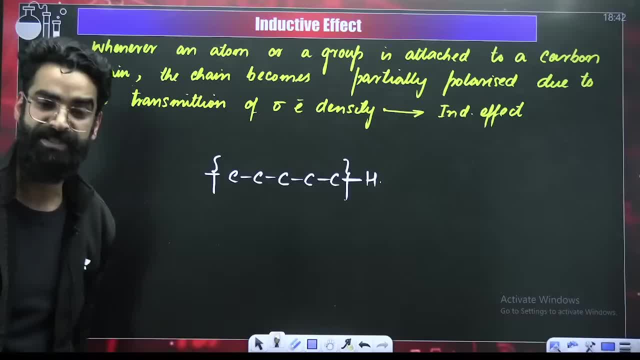 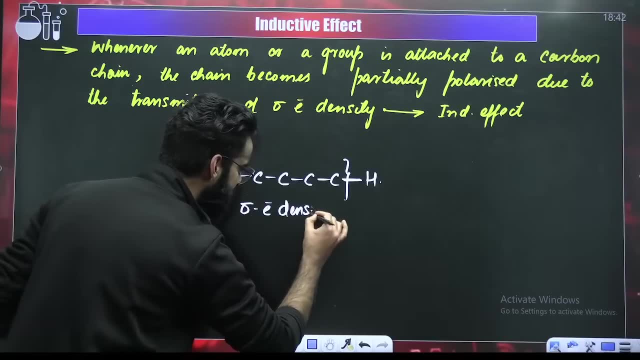 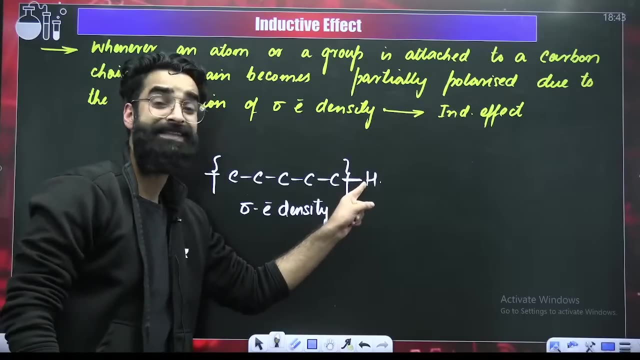 sigma bonds present. yes, in this chain there are only sigma bonds present, right? so can i say, in this chain there is only sigma electron density? absolutely, in this chain, right now, there is only sigma electron density. now, what exactly i'll be doing? i'll be replacing this hydrogen. i'm going. 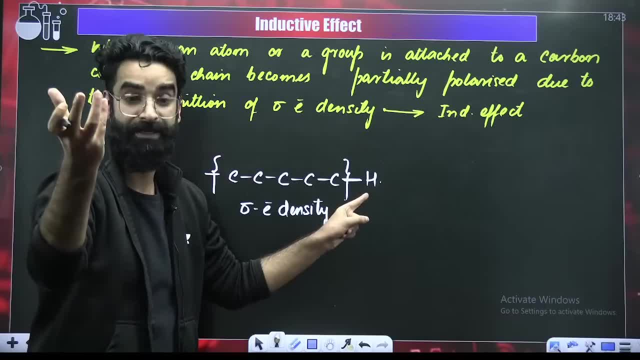 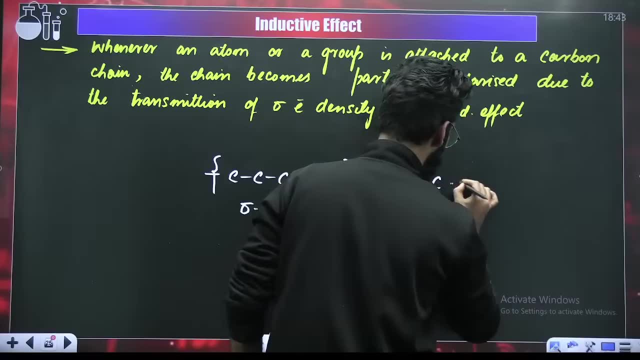 to replace this hydrogen by an atom or a group of atoms. i'm replacing, i'm going to replace this hydrogen by an atom or group of atoms. for example, these were one, two, three, four, five. these were five carbon atoms in the chain: one, two, three, this is four and this was five. right now i'm 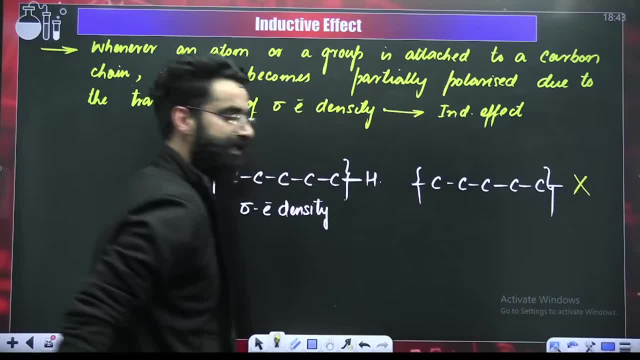 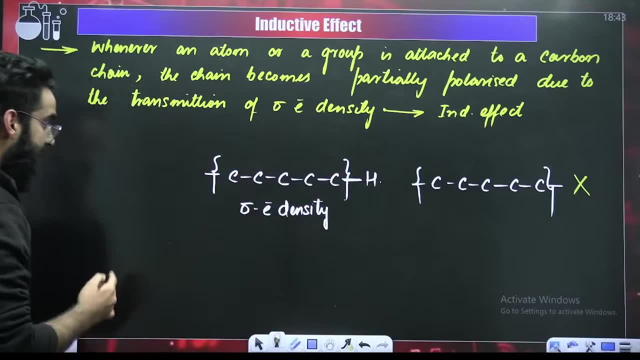 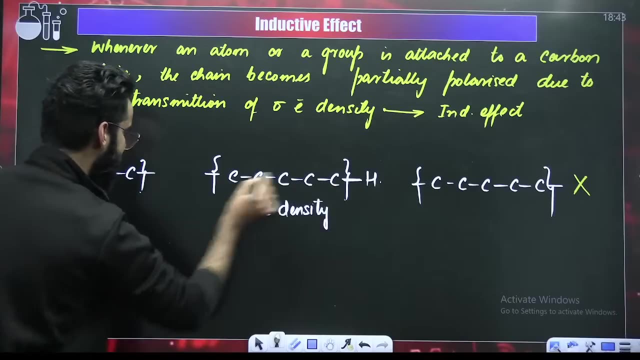 by an atom X, by an atom X, right by an atom X. and similarly, my dear students, similarly, I'm again going to replace this hydrogen by an atom Y. so these are your one, two, three, four, five, five carbon atoms. this was your carbon chain. now, instead of hydrogen, here I'm attaching what? yeah, I'm attaching an atom or group. 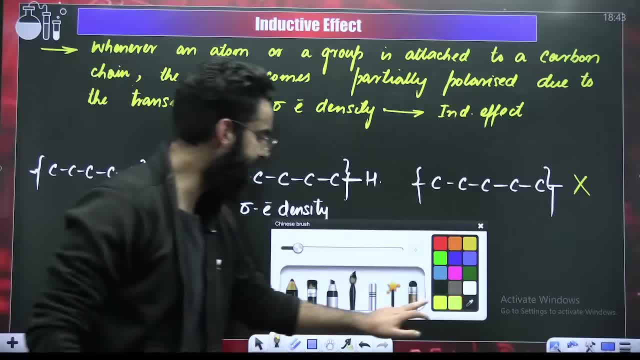 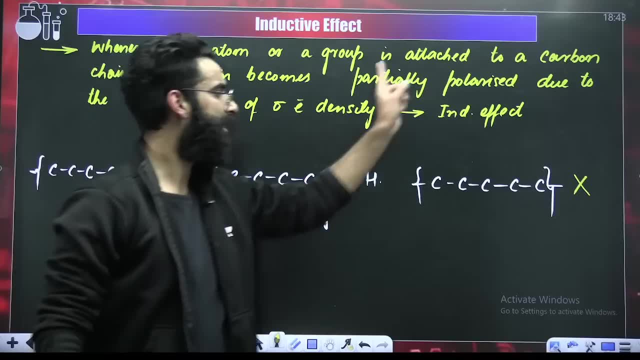 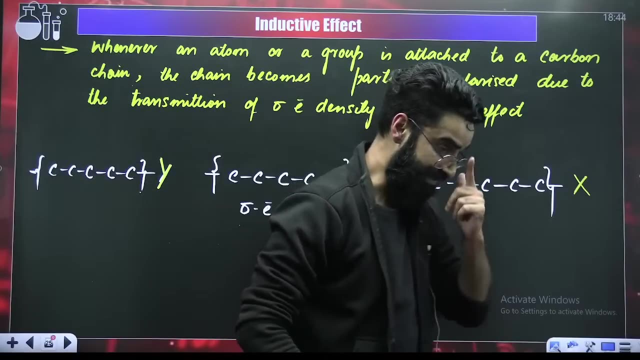 Y, an atom or group Y. so what I exactly did? I took a carbon chain which includes only the sigma electron density. now, instead of hydrogen, I placed X and here I placed Y. my dear students, let's look at this particular scenario. first of all, I'm assuming, I'm assuming over here, I'm assuming, I'm assuming electron. 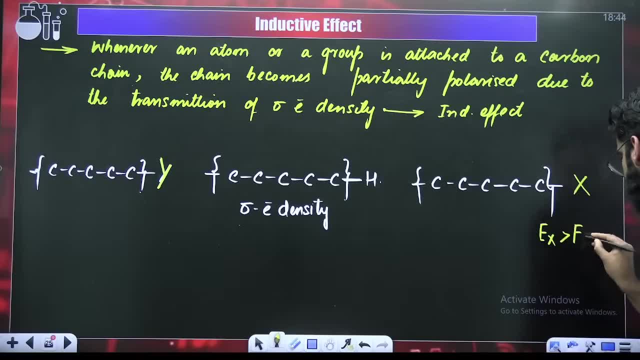 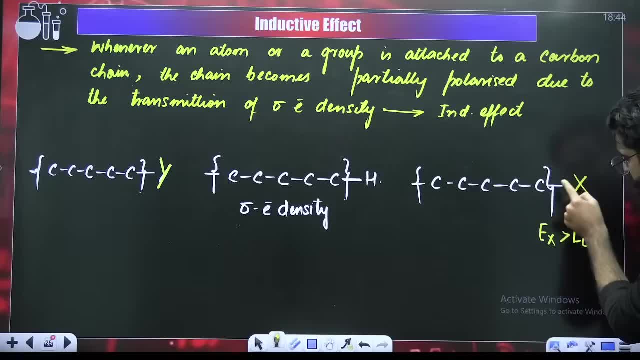 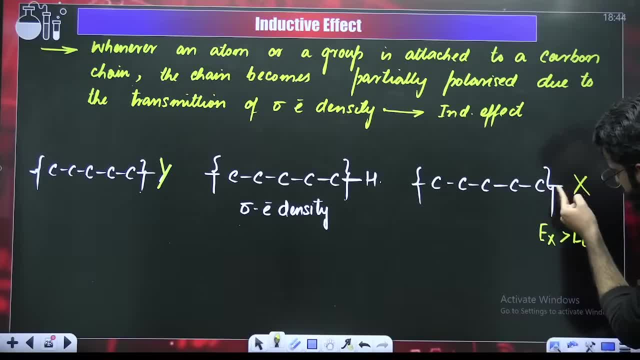 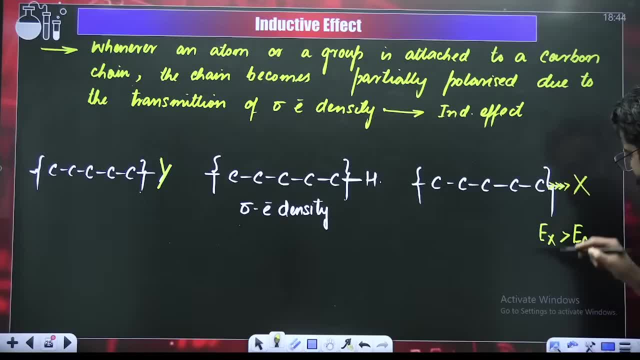 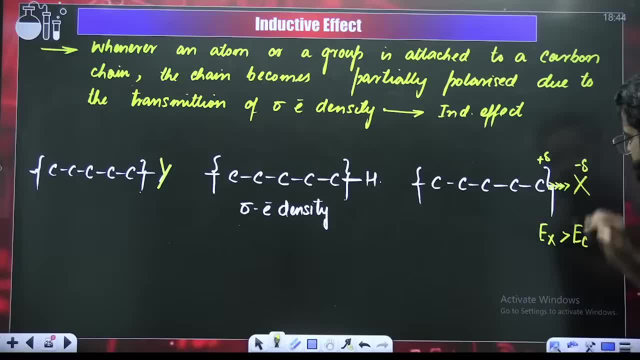 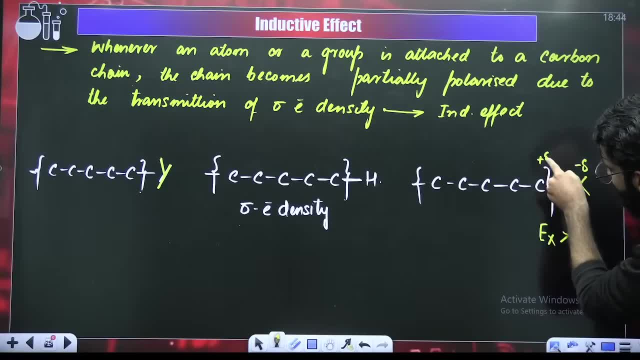 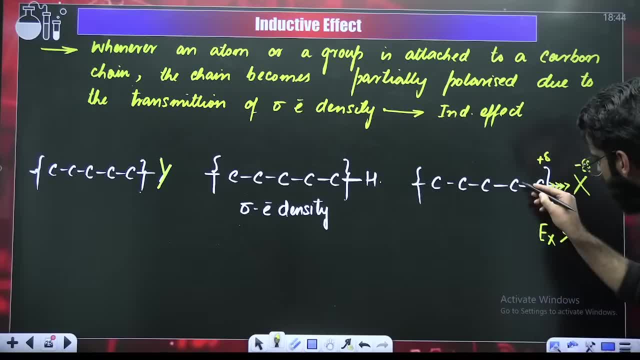 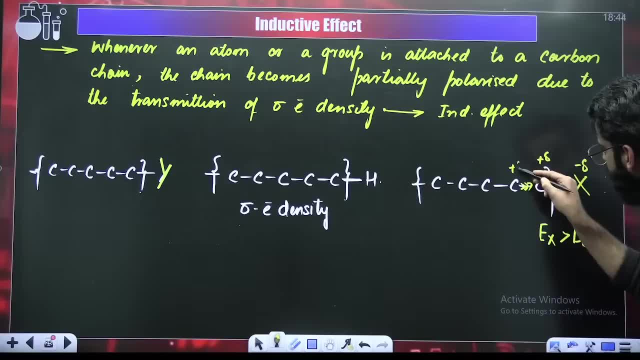 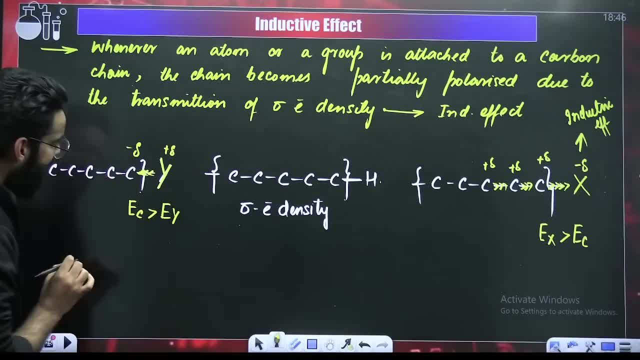 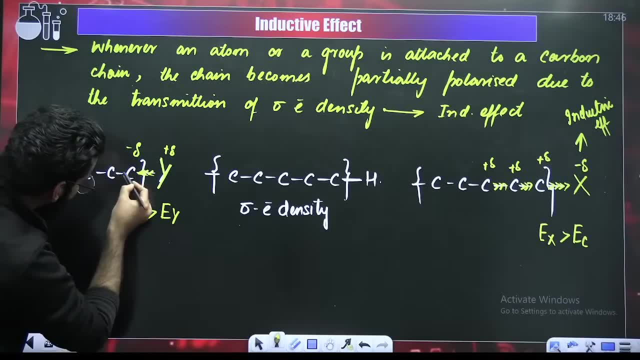 this carbon gets delta negative and this Y gets delta positive. right Now, my dear students, this carbon carrying delta negative, this delta negative, can I say it's going to ripple this electron pair. If it ripples the electron pair, if it ripples the electron pair, I'll say this: 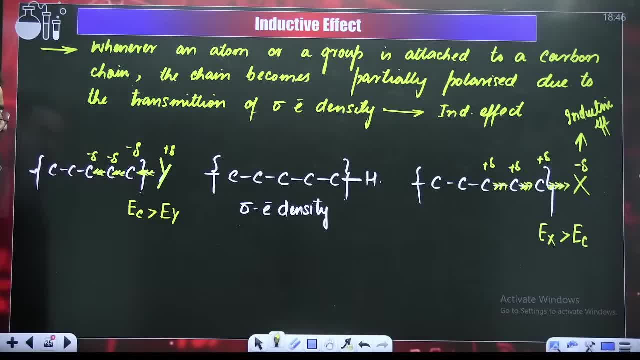 carbon will get delta negative. Now, similarly, due to repulsion, this carbon will get delta negative. So what happened over here? What happened over here? When you introduced an atom or a group, the chain got partially polarized due to the transmission of sigma electrons. 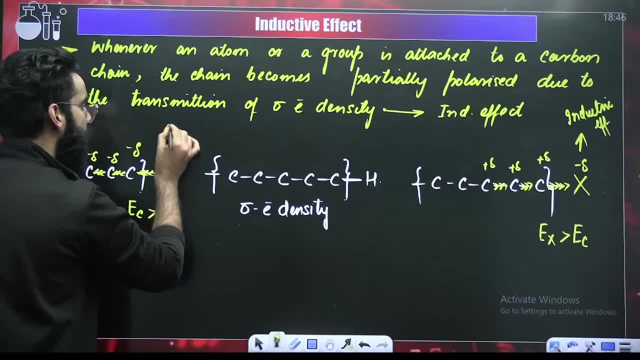 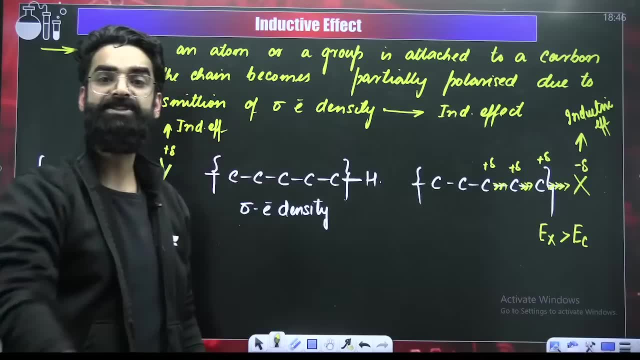 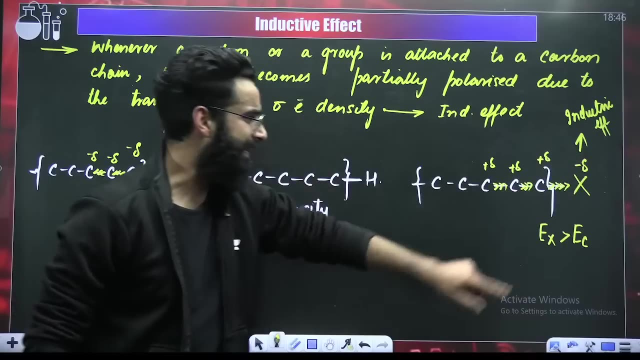 So again, I would say, this Y over here is showing which type of effect. It is showing inductive effect. It is showing inductive effect. Now, my dear students, try to understand one very simple thing, One very simple thing: Tell me, what do you see exactly? Is this X, is this X increasing? 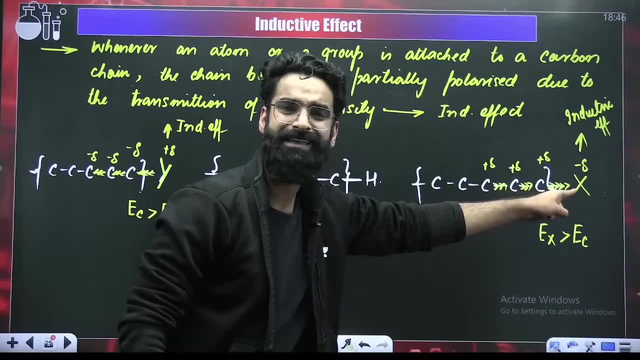 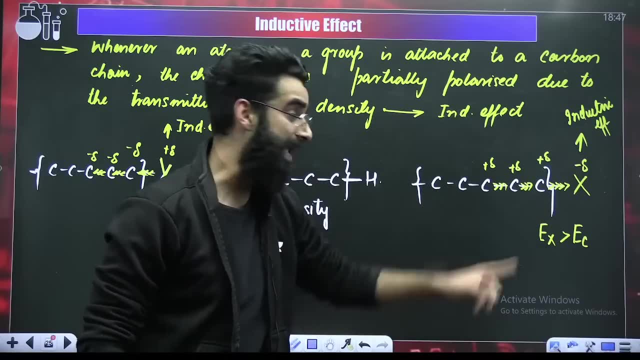 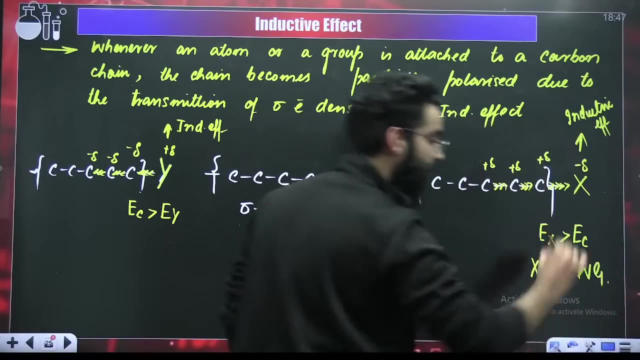 the electron density in the chain or decreasing. This X is pulling the sigma electrons towards itself. So this X, it is decreasing the sigma electron density. So can I call this X as electron donating or electron withdrawing? Here I'll be calling it as electron withdrawing group. This X will be called as electron withdrawing group Here. 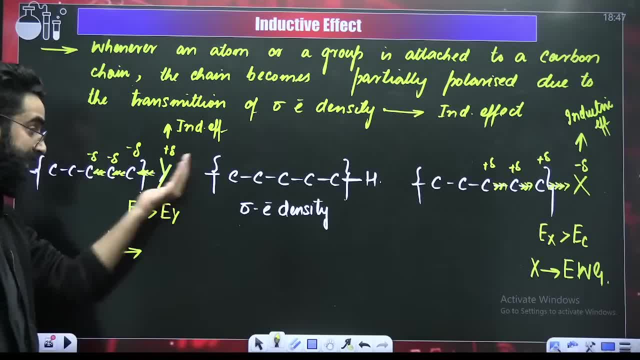 this Y, this Y. should I be calling this as electron donating or electron withdrawing? This Y is donating, right, It's donating. It is pushing sigma electron density in the chain right. So I would call it as electron donating group. My dear students, that particular group. 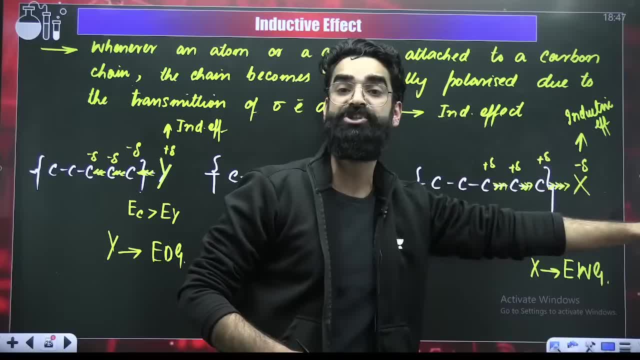 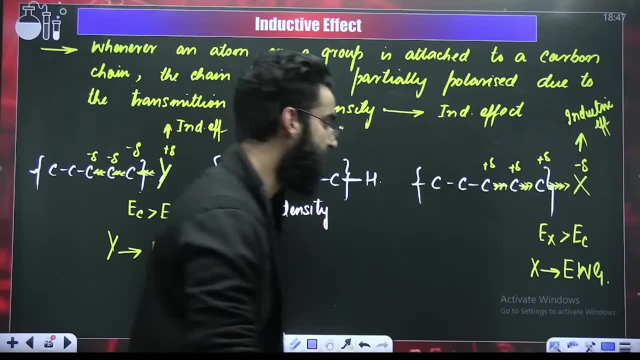 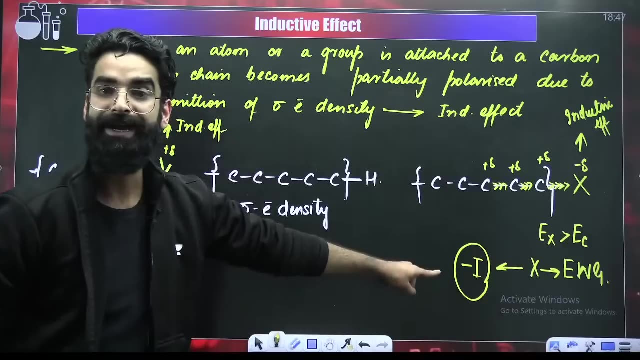 that particular group which withdraws sigma electron density from the chain, that particular group which decreases the sigma electron density in the chain. we say that group shows minus I effect. So I would say the group or atom X which I've attached over here, it is showing. 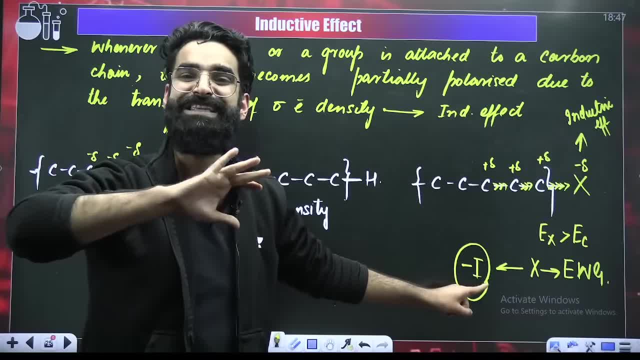 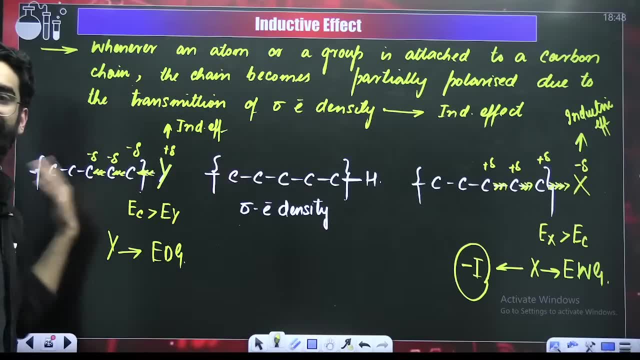 minus inductive effect. From now onwards, remember: minus means withdrawing, plus means donating, Minus means withdrawing, plus means donating. right Over here, this electron donating, I would say this particular group is going to show plus. I So do remember this particular. 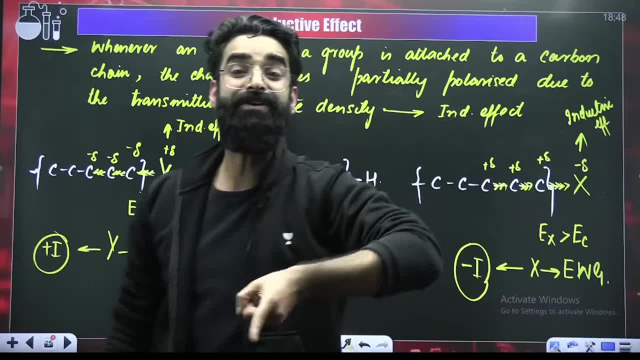 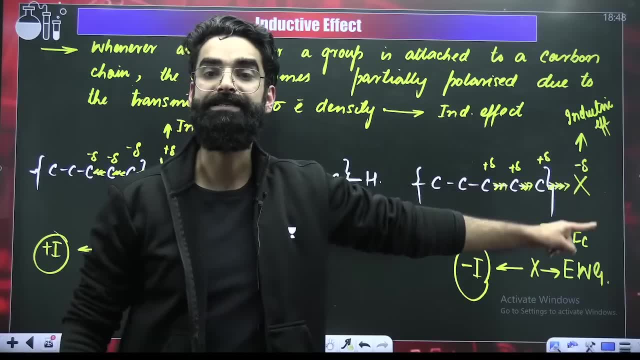 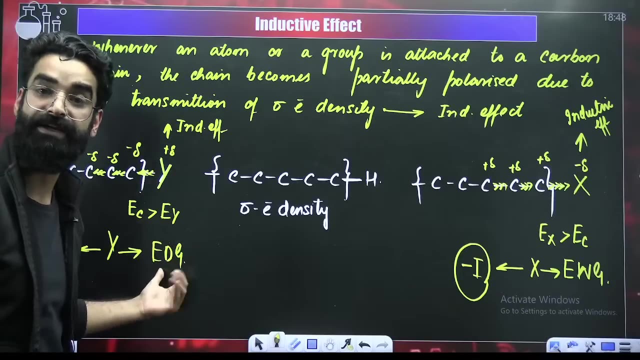 statement as well That atom or group which decreases the sigma electron density in the chain due to the transmission of sigma electrons, that group is electron withdrawing. and we say that group shows minus I effect. And here I would say the group is shown plus I effect, It's electron. 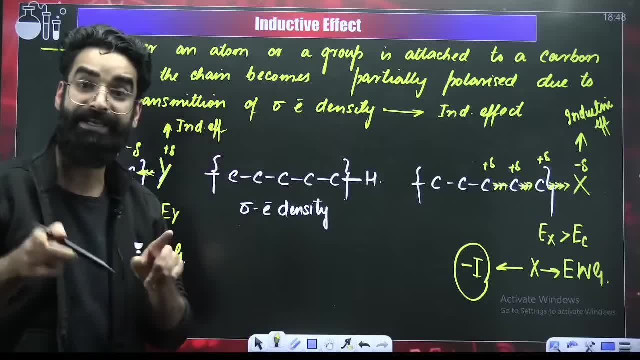 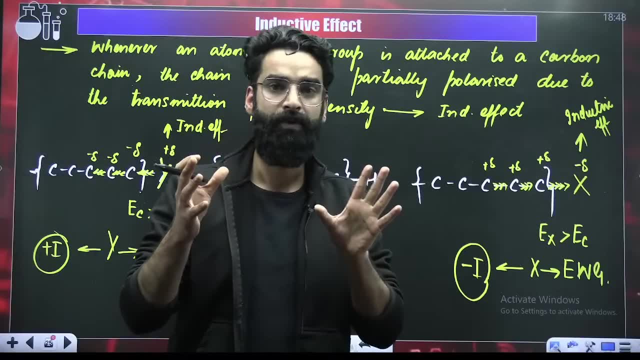 donating. Donating is plus, withdrawing is minus. Donating is plus, withdrawing is minus. That's all. Is this clear? I hope you got the idea of what this inductive effect is all about. And, my dear students, this inductive effect, it is a weak effect. 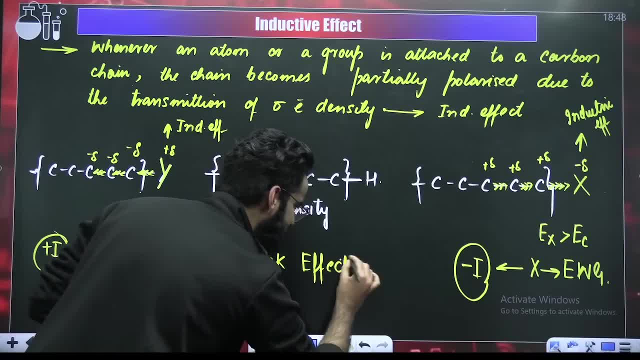 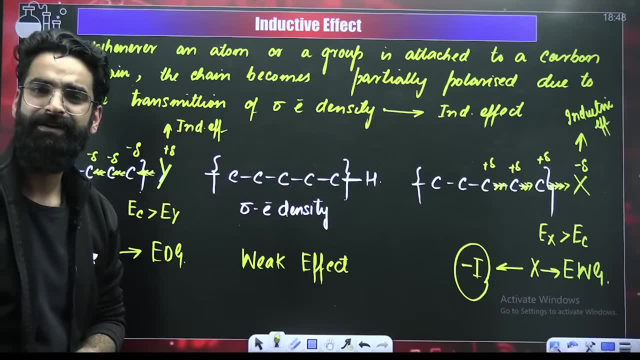 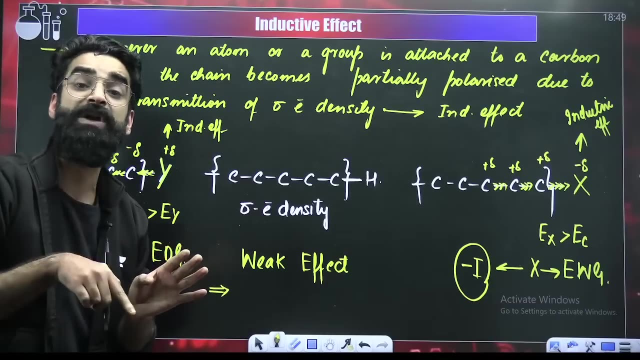 It is a weak effect. What is meant by this particular term? it's a weak effect. What is meant by this particular term? it is a weak effect. My dear students, let me tell you. let me tell you: we do not consider the inductive effect after three. 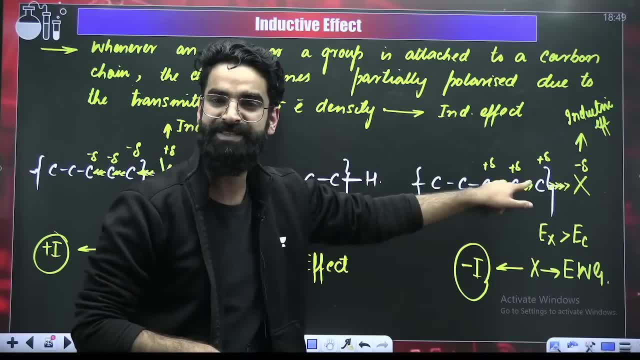 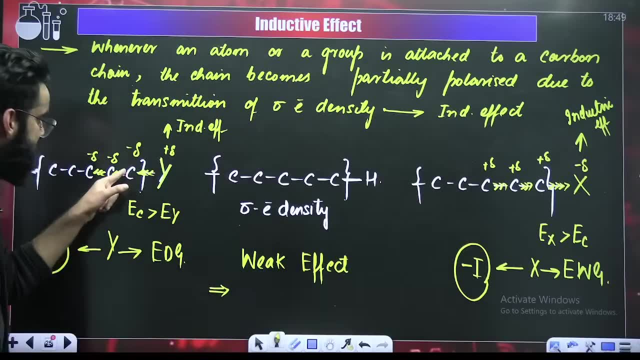 carbon atoms. But I will explain the context. I do explain the context. So, first of all, the case is that here, when the indicted outcome after the negative, the positive bullishpodium changes From the negative bullish pi to positive bullish pi, take any undesirable 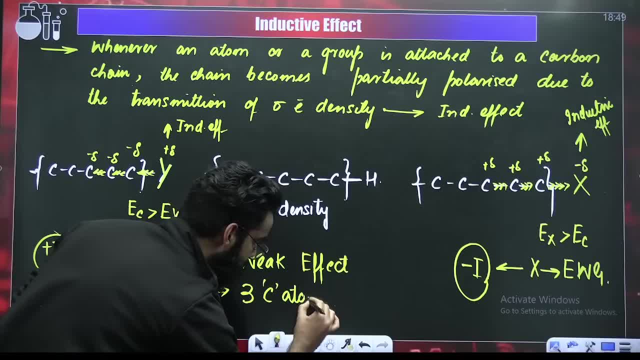 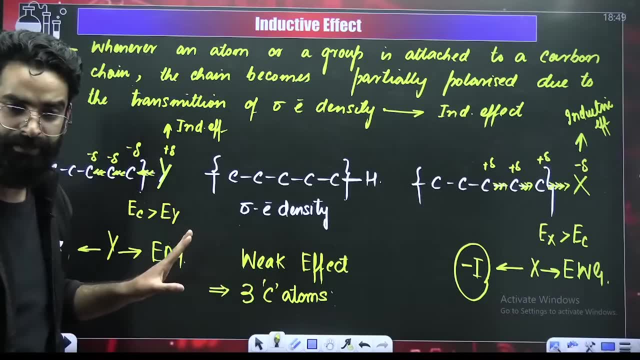 executives, any direct executives, which are really the amino acids calling when, again, by index of the index is negative square. So index of the index is negative square. Then again, afterK plus one, you are told negative with positive, because you are Parker and what I. have shown was positive, plus positive. After that I did not show any Pikachu- This carbon. I showed negative- this carbon. I showed negative This open. I showed any charge. After that I did not shown any charge. So indicator effect: we are only going to take up to three carbon atoms. The charges due to the 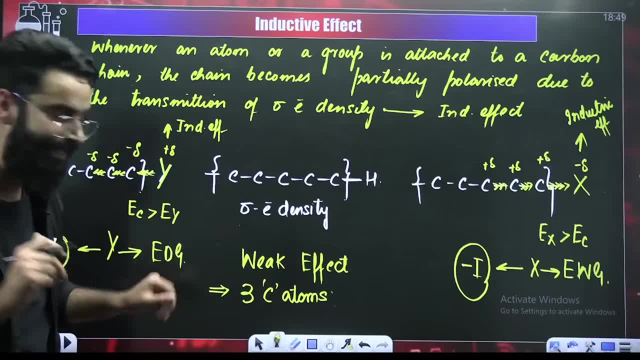 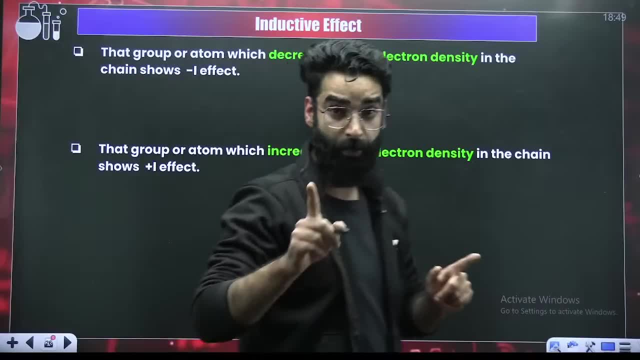 vanishes, After that inductive effect vanishes. I believe this is clear. Okay, I believe this is clear. These two statements I already told you. Look at these statements and understand whether these are clear to you or not. That atom or group which decreases the sigma electron. 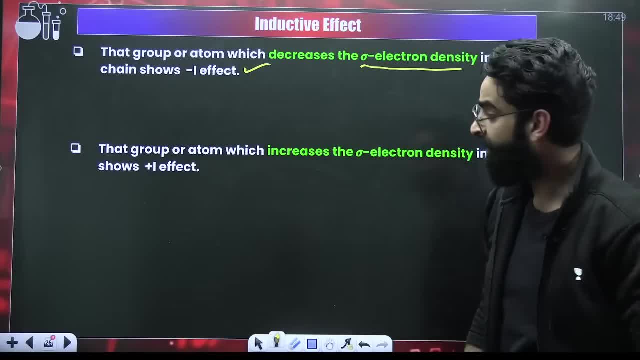 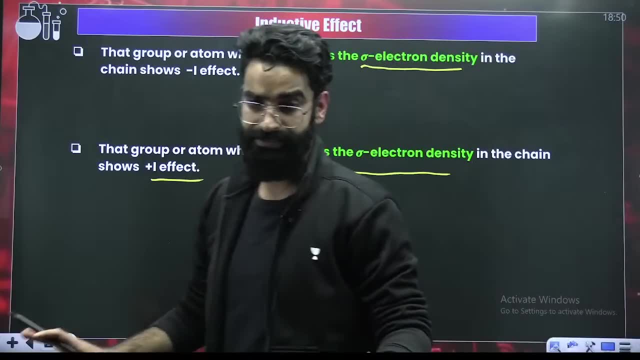 density in the chain. we say that group shows minus, I effect That group or atom which increases the sigma electron density in the chain. we say that atom or group shows plus, I effect Right. This is understood now. This is understood now. This is understood now. Now, my dear students, 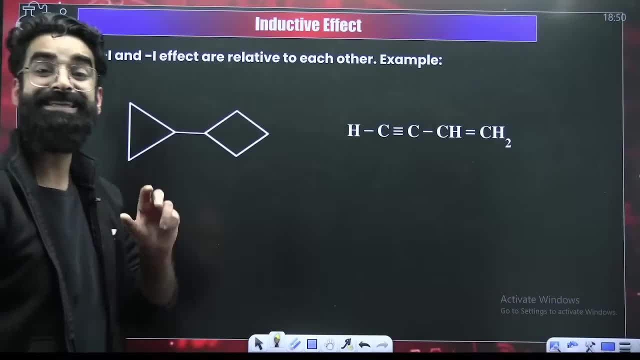 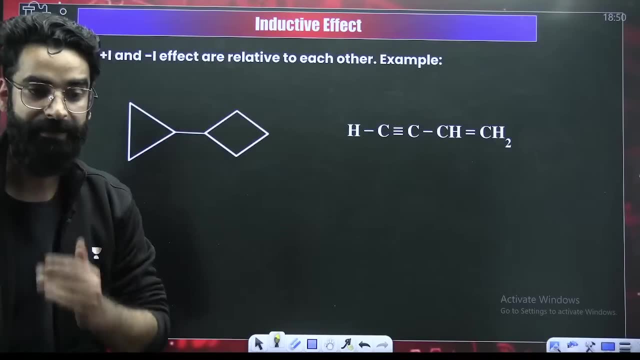 there is one more term: Plus I and minus I. we say they are relative to each other. We say they are relative to each other. What does that mean? What does that mean? We say they are relative to each other. Try to understand one thing. Look at this particular molecule. 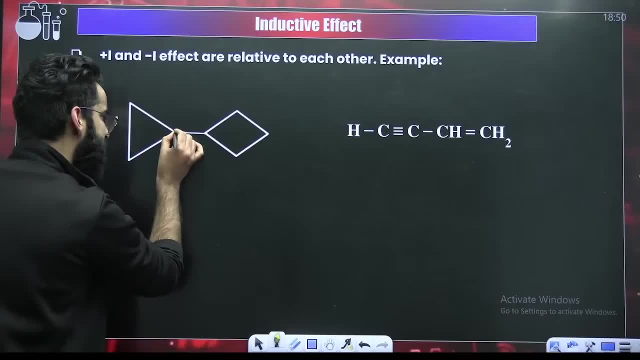 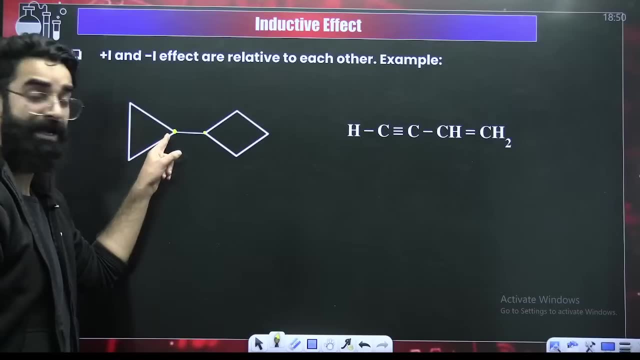 Here you have got 3 membered ring, Here you have got 4 membered ring. I would say this particular carbon is more electronegative. This particular carbon is comparatively less electronegative. We know due to angle strings This is more electronegative, So it will attract. 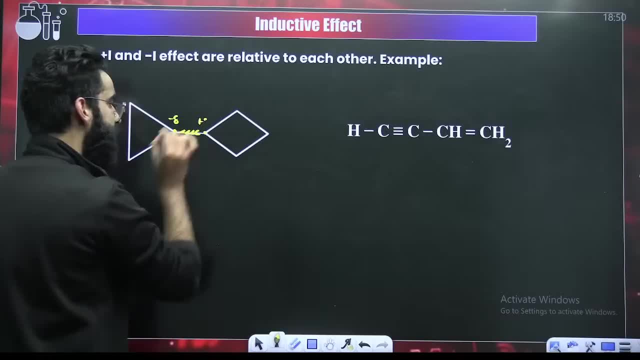 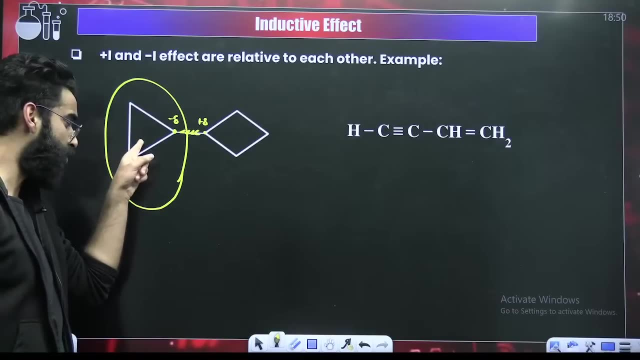 this bonded pair towards itself, due to which it gets delta negative. This gets delta positive. If you particularly look at this particular group, If you particularly look at this group, What do you think Is this group? is this group pulling the electron density pulling? 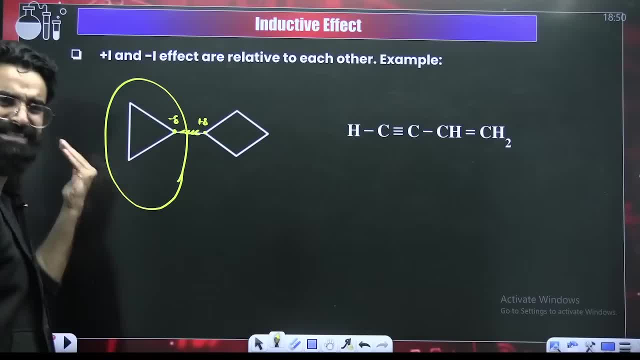 the sigma electron density towards itself. I would say, yes, This group is pulling the sigma electron density towards itself. And that group which pulls the sigma electron density towards itself, we say That group shows minus. i effect. Now people look at this particular group, Look at this. 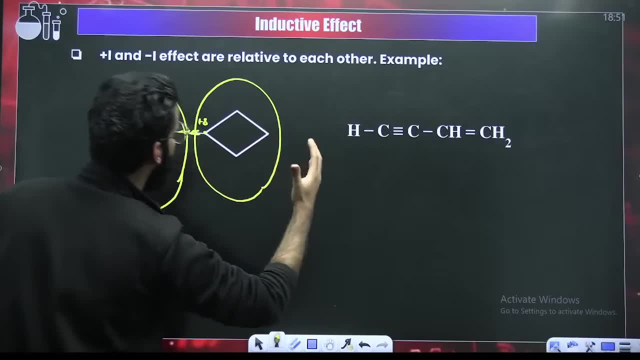 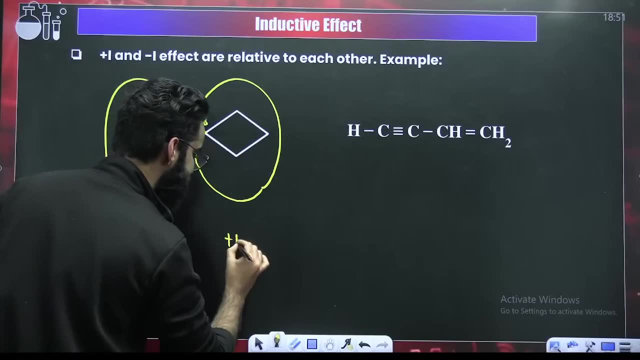 particular group. Is this group pulling the sigma electron density or pushing? It? is pushing the sigma electron density towards the other one Right? So I will say this particular group is showing plus i. So basically this: plus i and minus i, they are relative to each. 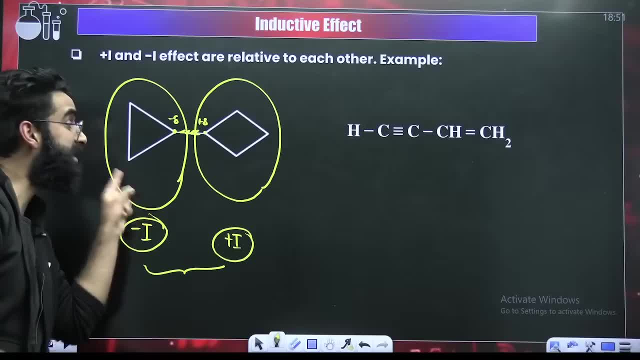 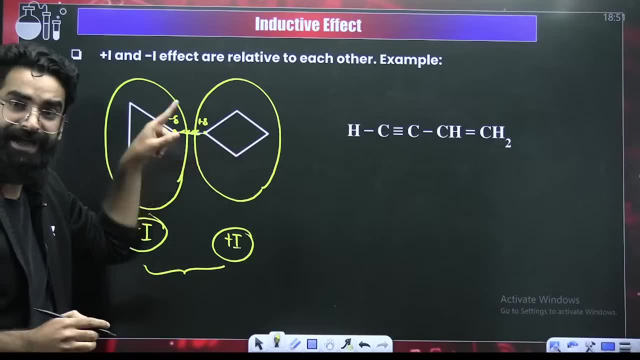 other. I would say: this group is showing minus i with respect to this one And this is showing plus i with respect to this one. Right, This group is showing minus i with respect to this And this is showing plus i with respect to this. So, plus i and minus i, they are going. 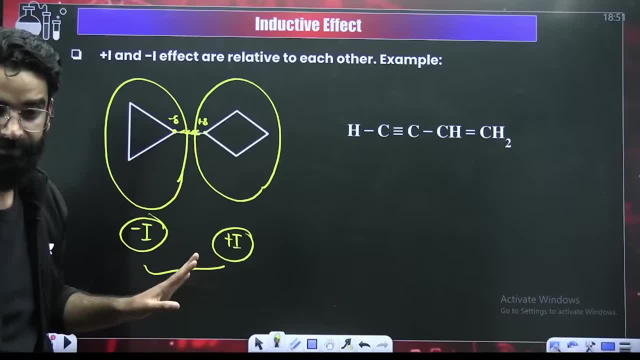 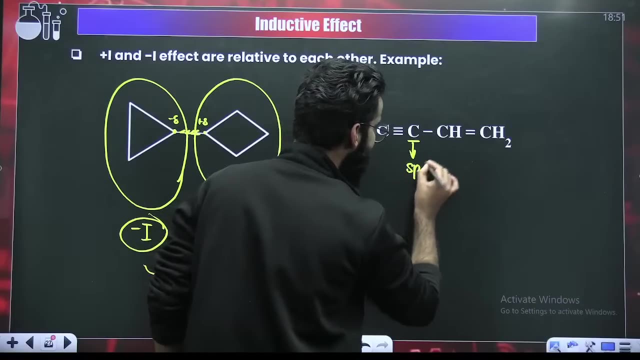 to be relative to each other. They are relative terms. They are relative terms. One is withdrawing with respect to another, Another is donating with respect to another. Yeah, Similarly, look at this particular case. Here the carbon is sp hybridized. Here the carbon is sp2 hybridized. 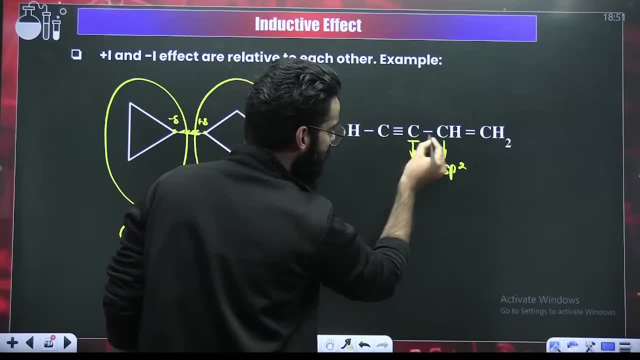 Perfect. So this carbon will be more electronegative. If it is more electronegative, it will attract the sigma electron density towards itself. Now, this carbon is more electronegative it itself. it will attract the bonded pair towards itself, due to which it gets delta negative. 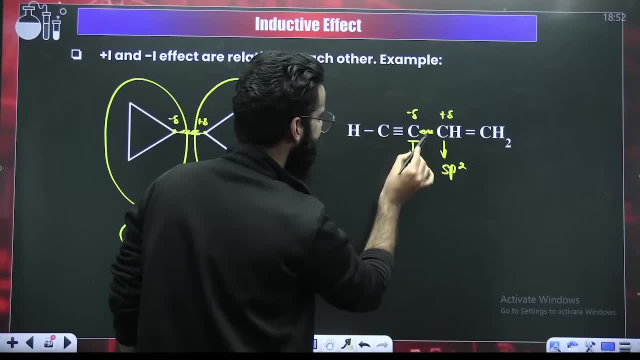 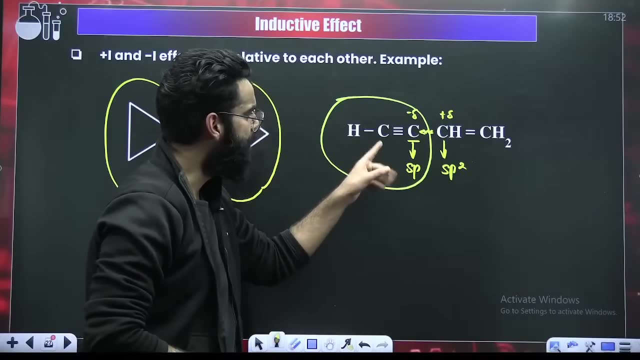 this gets delta positive. Now people just try to understand one simple thing: Look at this particular group, Look at this particular group. This particular group is it pushing the electron density or pulling the electron density? It is pulling the electron density. 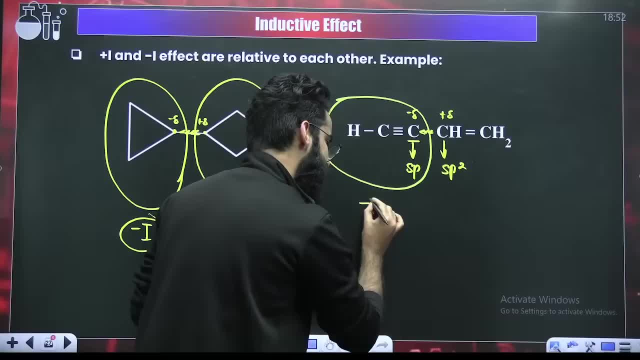 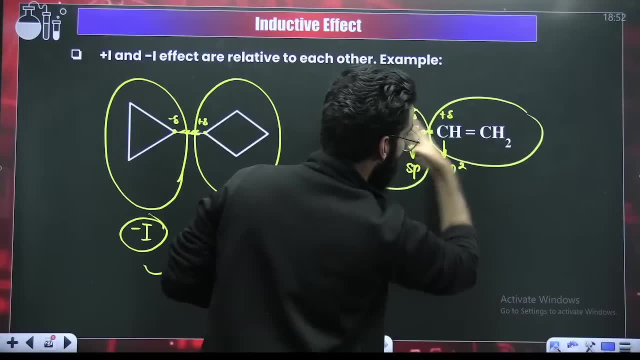 If it is pulling the electron density, that means it is going to show minus sign. This particular group, is it pulling the electron density or pushing the electron density? It is pushing the electron density, So this group is showing plus sign. This group is showing 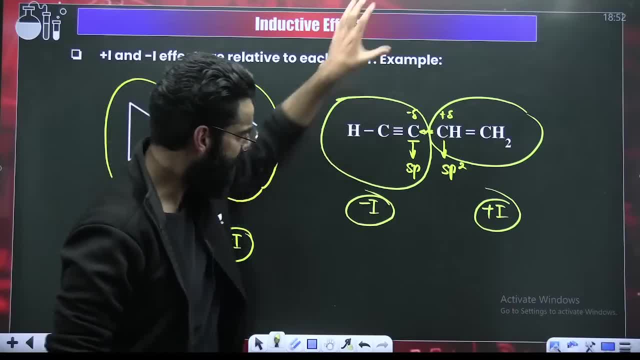 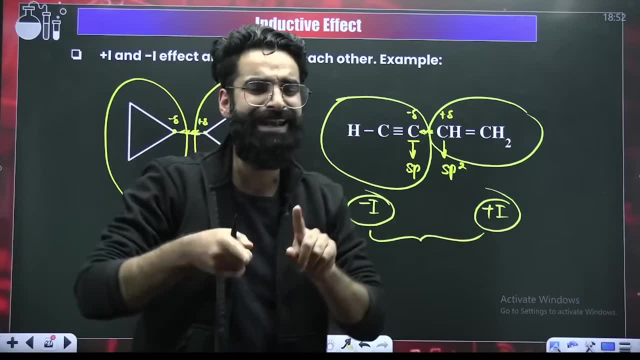 plus sign. I will say: this particular group is showing minus sign with respect to this one and this shows plus sign with respect to this one. So again, I can categorically say this: plus sign and minus sign, they are relative terms. They are relative terms. They. 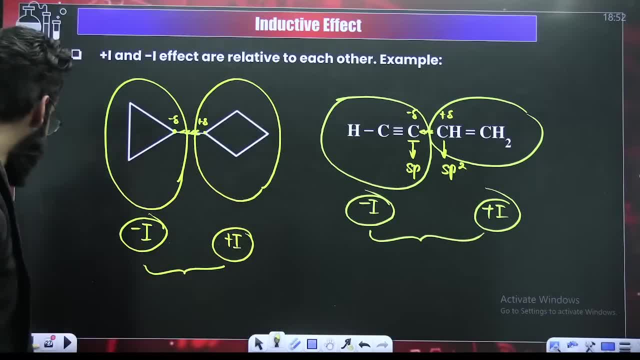 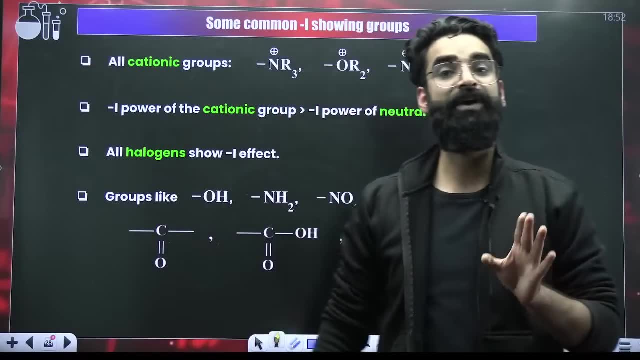 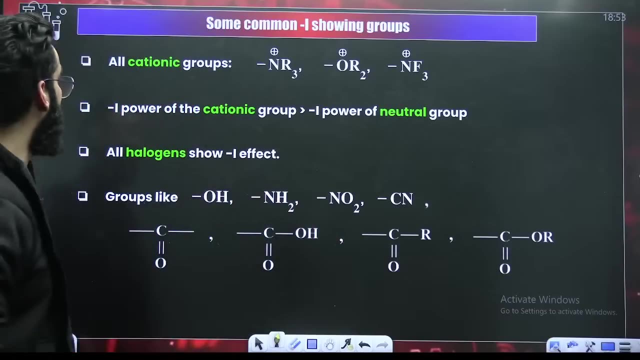 are relative to each other. I believe this particular statement is also clear to you. Now, guys, in order to do the questions on inductive effect, we have to remember certain things. In order to do the questions, we have to remember certain things. Point number 1. All the cationic. 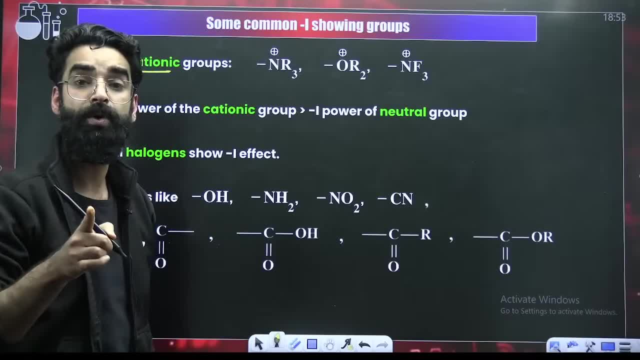 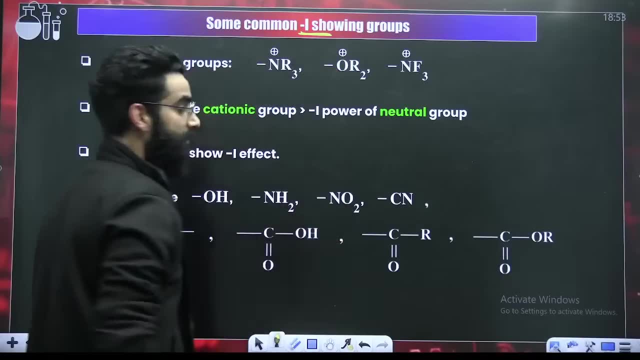 groups. all the cationic groups. they show minus sign effect. All the cationic groups. they show minus sign effect Right. All the cationic groups. Cationic groups means group carrying positive, group carrying positive. group carrying positive: Any group which carries. 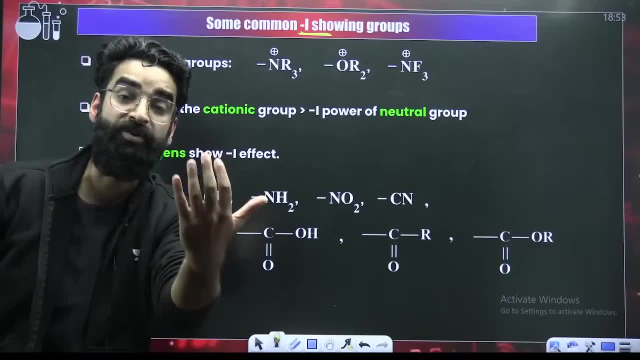 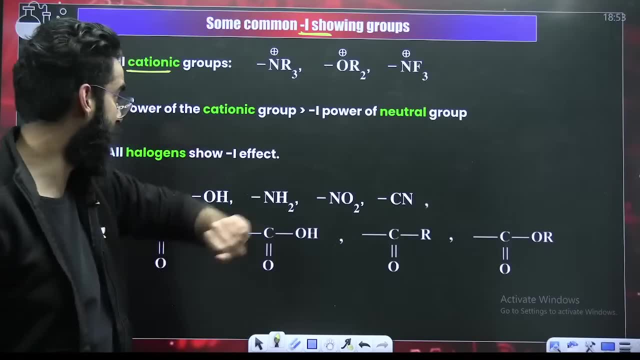 the positive charge. remember it is always going to show minus sign. It is going to withdraw the sigma electron density. It is going to be electron withdrawing. It is going to be electron withdrawing, Point number 1.. Point number 1. All the cationic groups. they 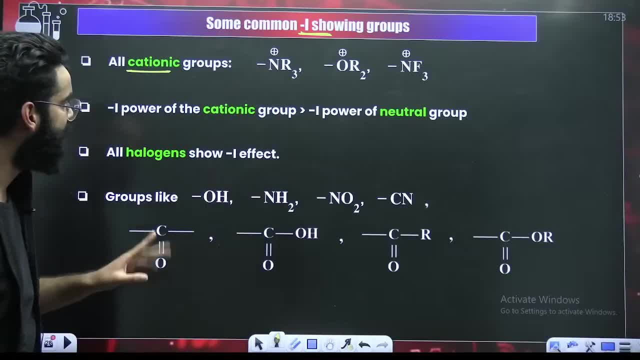 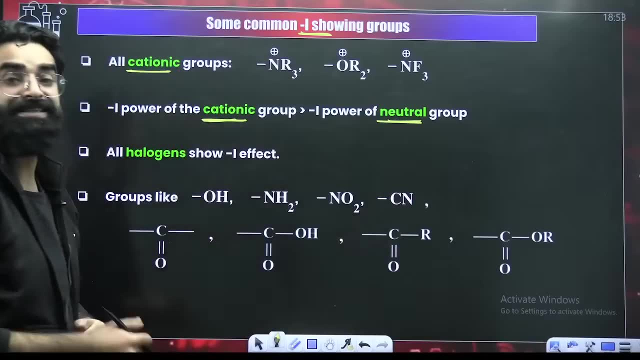 show minus sign effect. They are withdrawing in nature: Right Minus i power of cationic group: minus i power of cationic group will be always greater than that of minus i power of neutral group: Minus i power of cationic group will be always greater than that of. 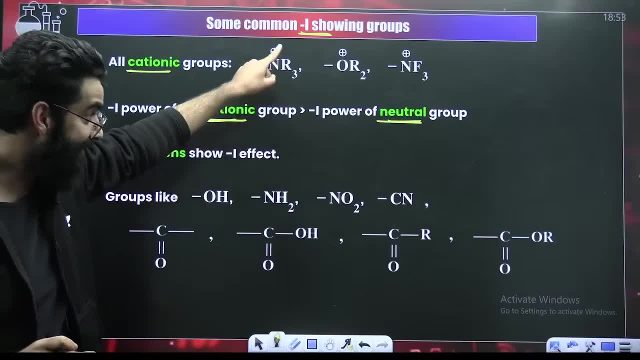 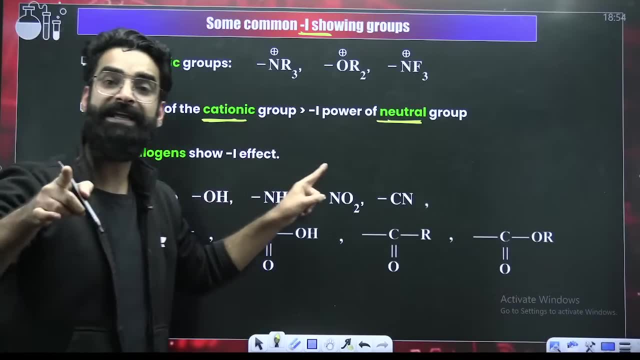 minus i power of neutral. One more thing, Guys: I will have to use all these things in the questions. That's why I keep on telling you all the time to remember all these things, All the cationic groups, they show: minus i power, Minus i power of cationic group will. 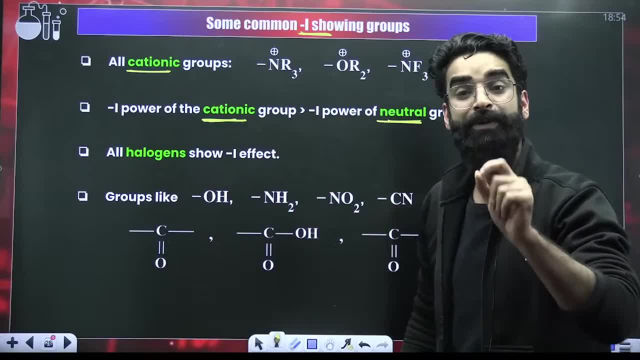 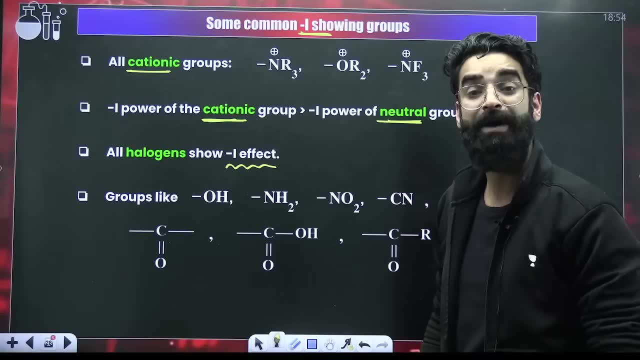 be greater than that of minus i power of neutral group. All your halogens- chlorine, chlorine, bromine, iodine, all your halogens. they show they are withdrawing in nature. They show minus effect, minus i effect. All your halogens. they are withdrawing in nature. They are electron. 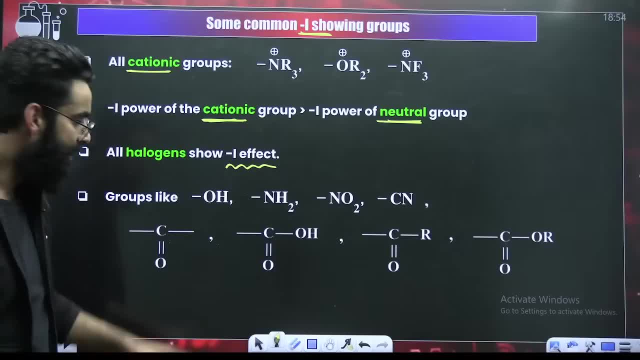 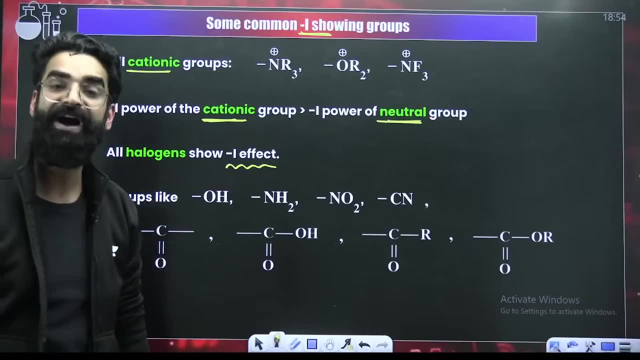 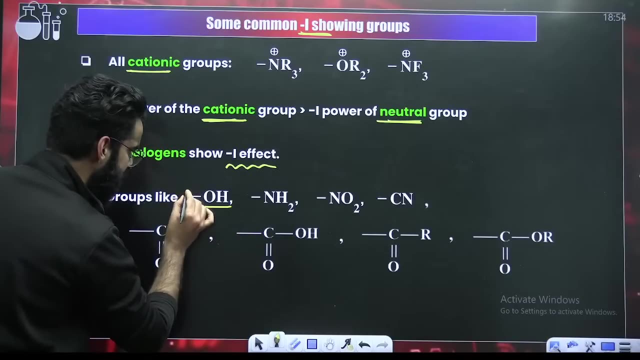 withdrawing in nature. They show minus i, effect Right Groups like OH, NH2, NO2, CN, they are also minus i. They also show minus i. Now the point is why? Now the point is why, Understand, My dear students, if this OH, if this OH is attached to a carbon chain, 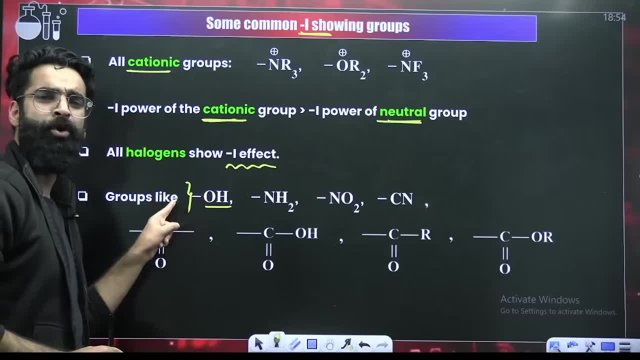 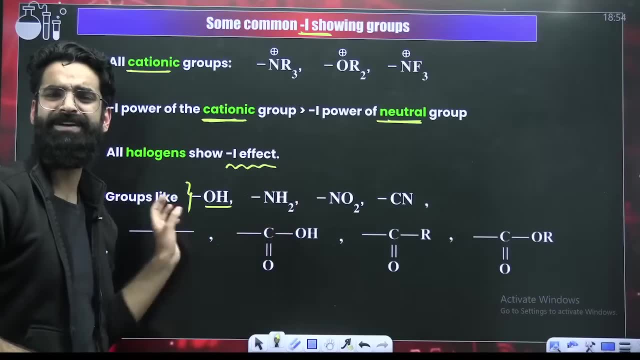 if this OH is attached to a carbon chain, oxygen is more electronegative than carbon, So it will attract the bonded pair towards itself. Right, It's behaving like electron withdrawing. If it is electron withdrawing, it will attract the bonded pair towards itself. 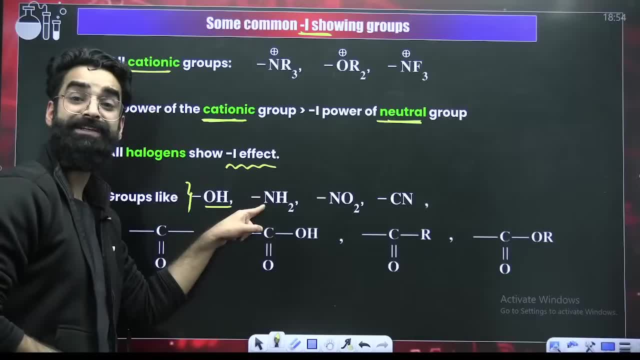 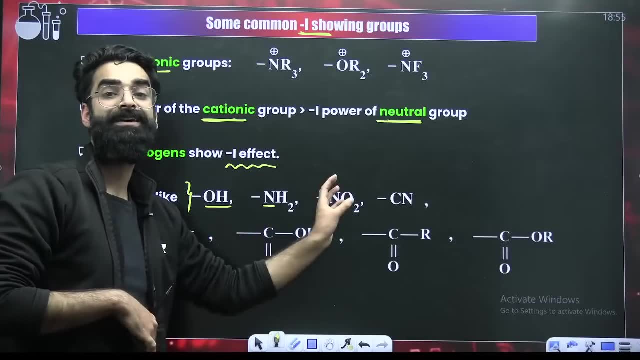 So minus i Right. Look at this one. If this nitrogen is attached to the carbon chain, look at the first atom, nitrogen. If this is attached to the carbon chain, nitrogen is more electronegative than carbon. It will attract the sigma electron density towards. 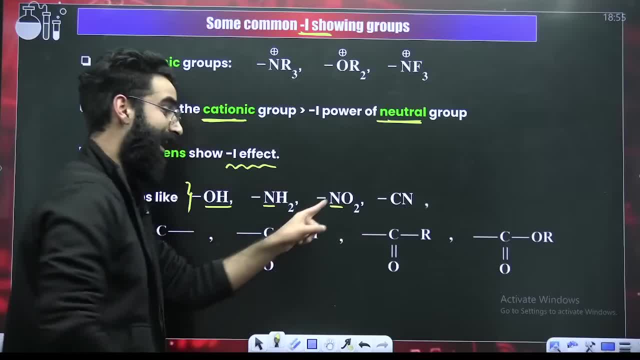 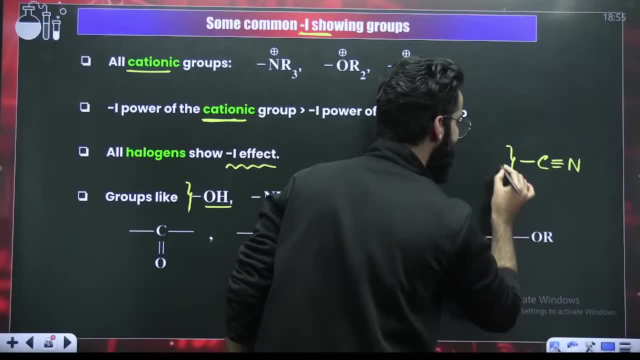 itself. Right Again, minus i, Nitrogen. attach this with carbon chain. Again, minus i. This is CN. This is C triple bond N. Attach this with carbon chain. Attach this with carbon chain. What you'll observe? What you'll observe? Look at the hybridization of this particular. 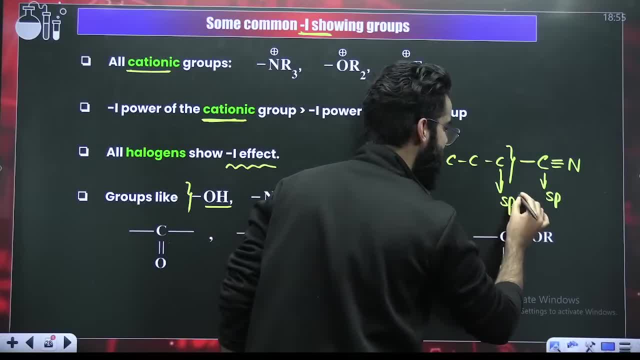 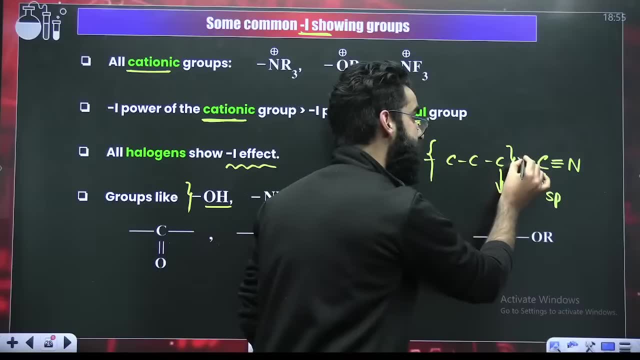 carbon, It's sp. Look at the hybridization of this particular carbon: It's sp3.. Right, This one is more electronegative. If this one is more electronegative, it will attract the sigma electrons towards itself, Right Attracting. So it is behaving like electron withdrawing group. So this is 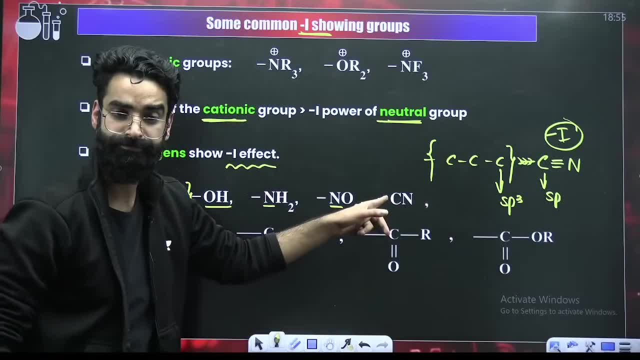 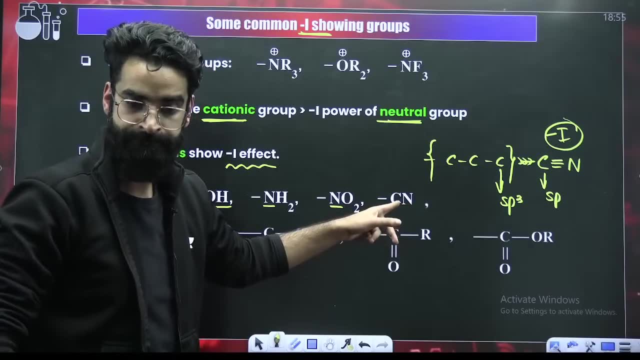 going to show what This is going to show: minus i. So CN also shows minus i. I'm showing you exactly, I'm showing you exactly how to identify whether the group is showing plus i or minus i. Right, I'm exactly identifying how to. I'm exactly identifying how to. I'm. 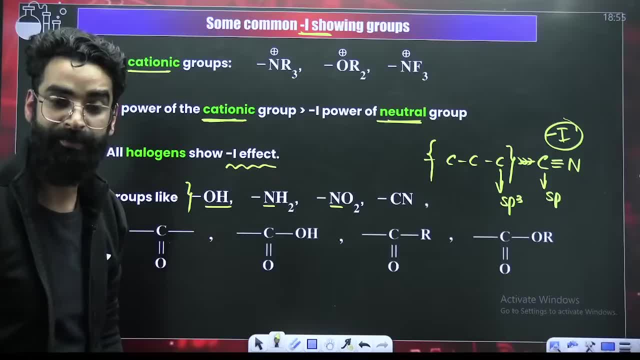 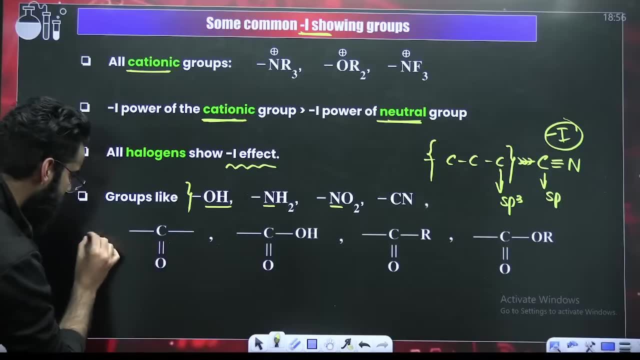 exactly showing you how to identify whether the group is showing plus i or minus i. People try to look at this particular case. This is C, double bond, O. Imagine this particular group is attached with a carbon chain. Imagine this particular group is attached with a carbon. 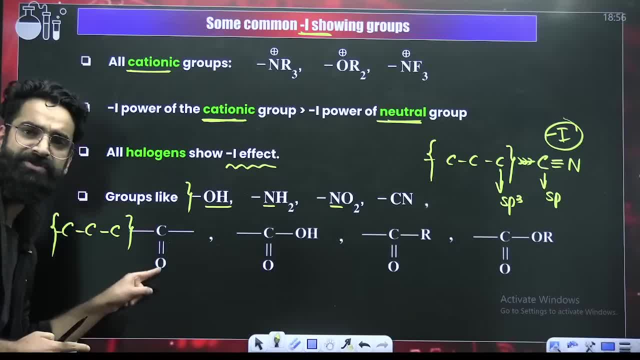 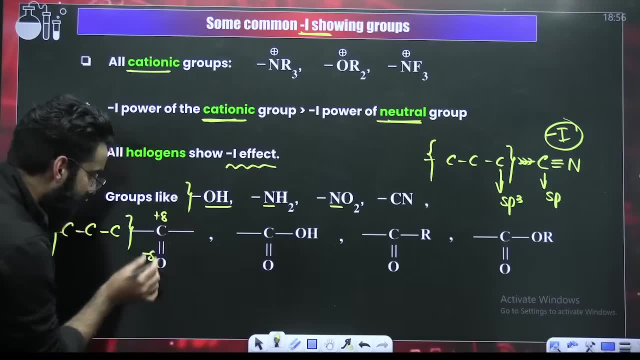 chain What you will observe: Carbon, oxygen, Which one is more electronegative? Oxygen If oxygen is more electronegative. so this will carry delta negative, This will carry delta positive. Now, this delta positive on carbon will attract these sigma electrons. 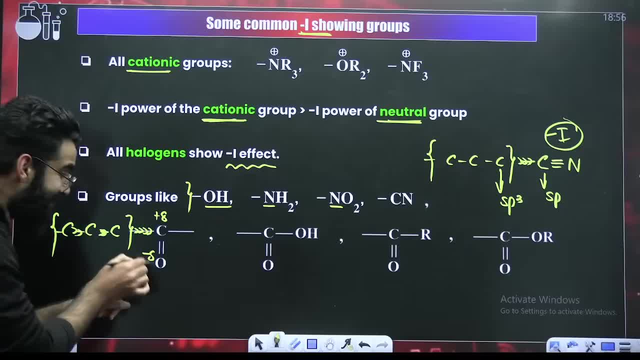 towards itself, Right, Perfect. So is this group behaving like electron withdrawing or electron donating? This is electron withdrawing, So I'll say it will directly show minus. i Right, It will directly show minus. i Look at this particular case. This will also show minus i, because this is. 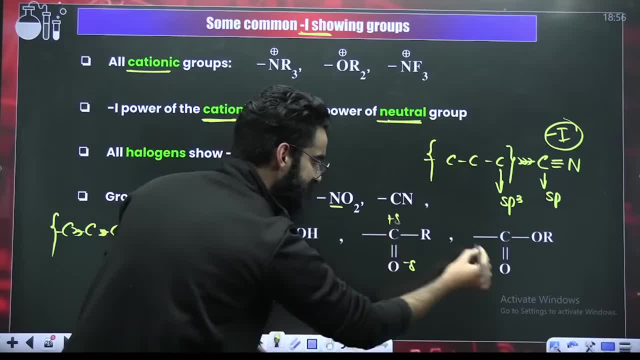 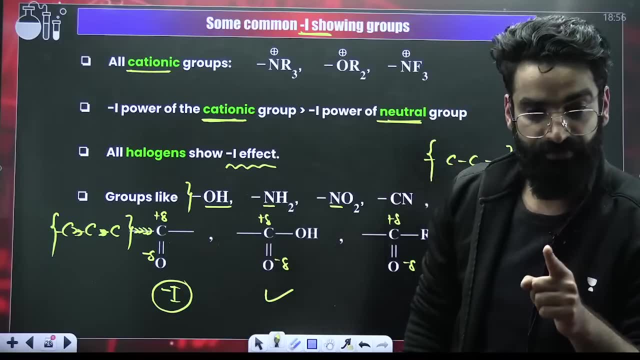 minus delta. This is plus delta. This is minus delta. This is plus delta. This is minus delta, This is plus delta. So all these groups, whatever are mentioned on the screen, they are going to show minus. i effect. They are going to show minus, i effect. All these things are. 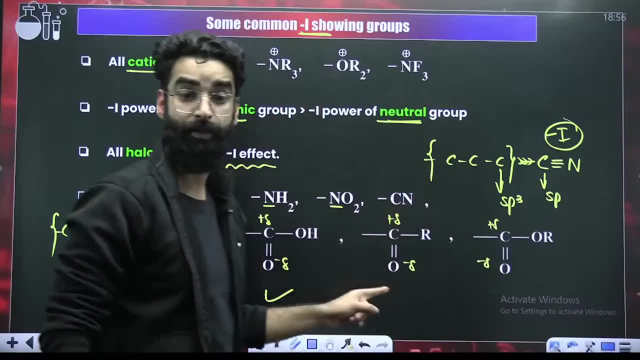 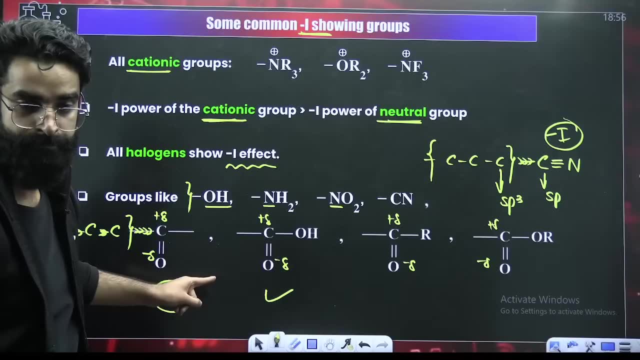 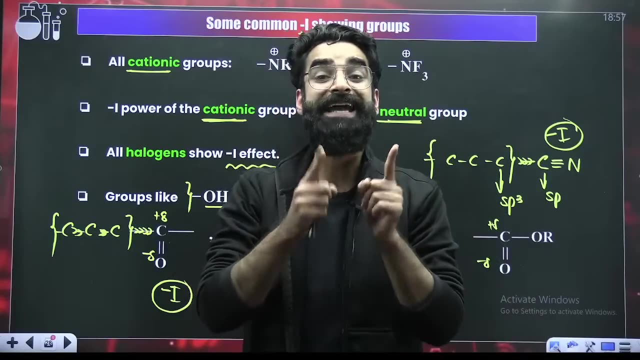 clear. Say yes or no once in the chats. I will have to utilize all these things in equations. people, I will have to utilize all these concepts in equations. Everyone, Quickly, Quickly, everyone. So from this particular slide, what we have to remember: Minus all the cationic groups they show, minus i, They 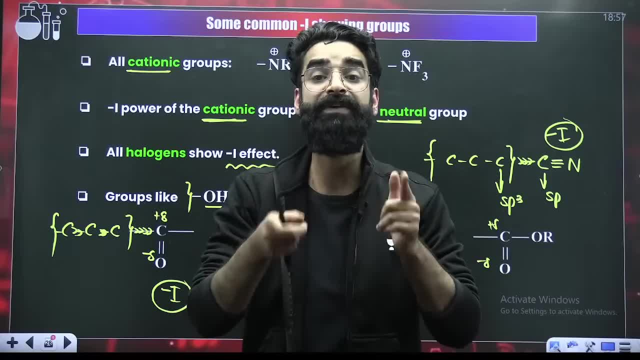 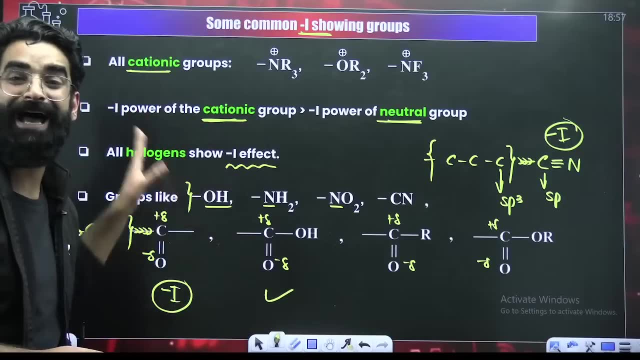 show minus i. They are withdrawing Right. Minus i power of cationic group will be greater than minus i power of neutral group. Second thing And third thing: all these halogens, all the halogens, they are electron withdrawing. 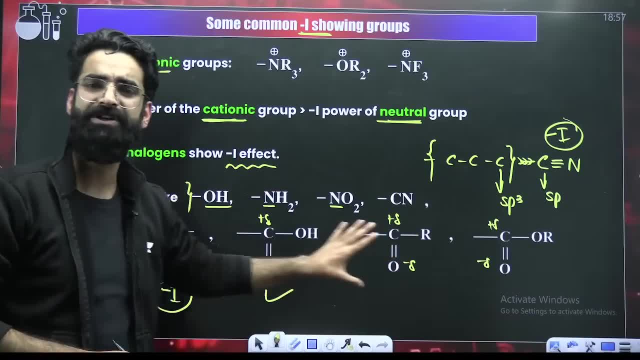 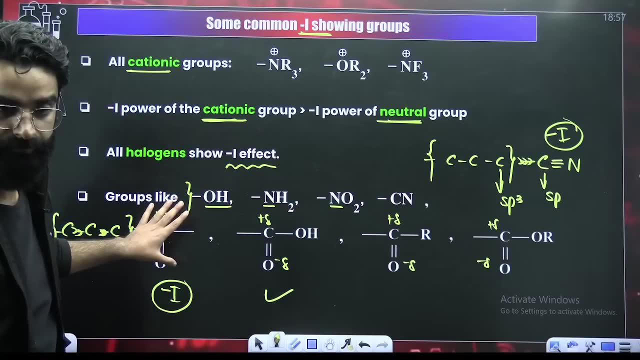 They show minus I And all these groups, all these groups, whatever are mentioned on the screen, they show minus I. Right When attached to the carbon chain. Yes, Perfect people. I believe this is clear Now. similarly, similarly, similarly. 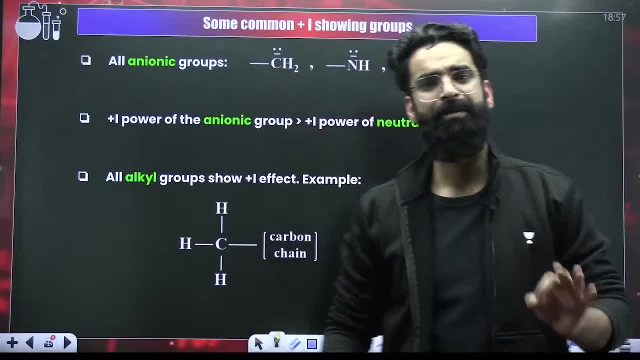 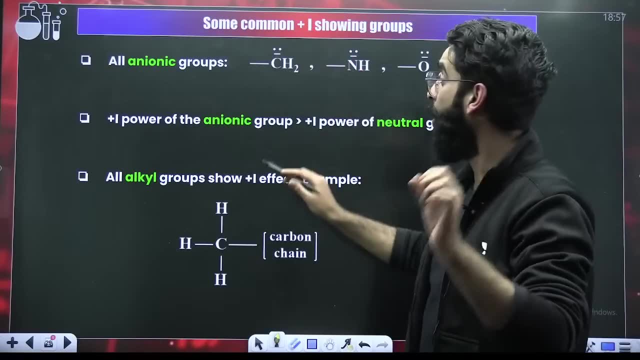 what are plus I showing groups? What are plus I showing groups, My dear students, just opposite of what I told you, Just opposite of what I told you. Plus I means electron donating, Plus I means electron donating All the NID groups. 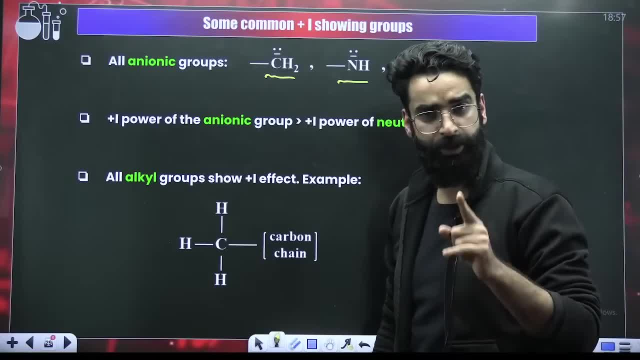 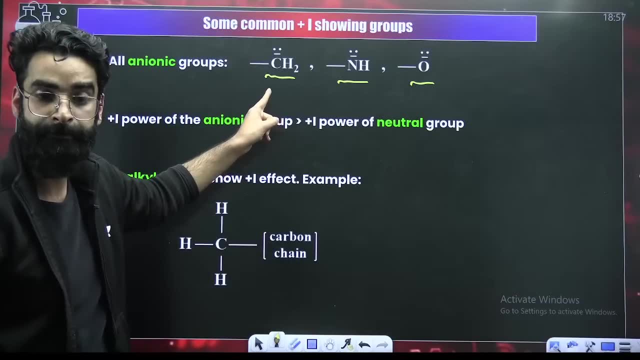 all those groups which carry the negative charge, All those groups which carry the negative charge, All the NID groups. they are electron donating. They show plus I. They show plus I. They show plus I Number one, Number two Plus I power. 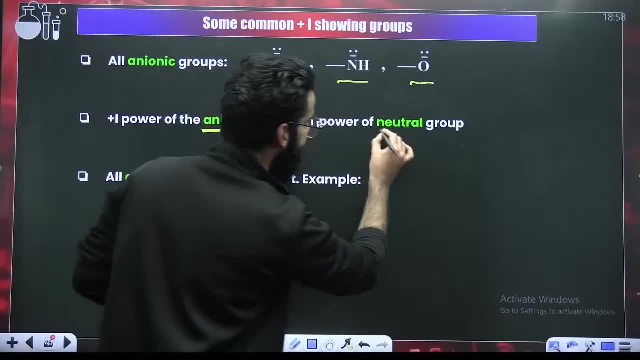 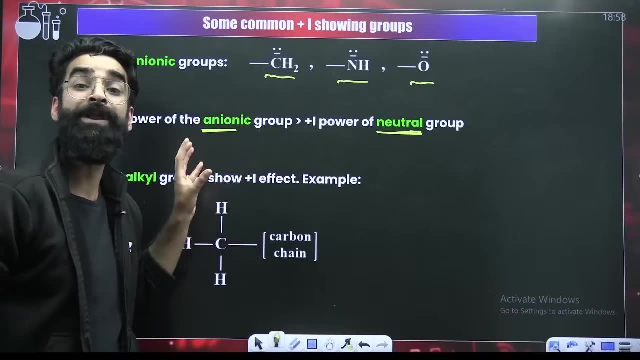 plus I power of NID groups, plus I power of NID groups will be greater than that of plus I power of neutral groups. So NID groups, they are more electron donating than that of your neutral groups. Then all your alkyl. 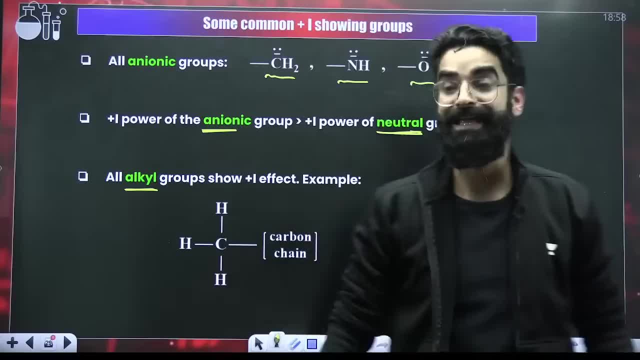 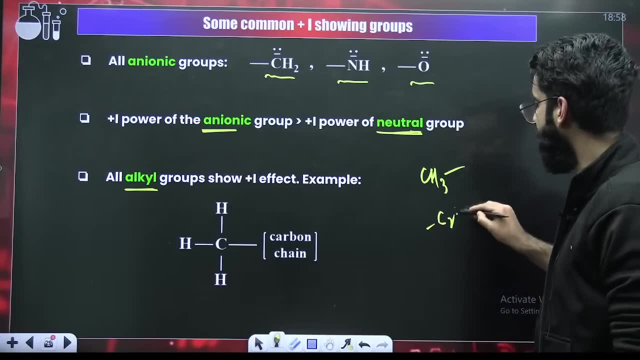 all your alkyl groups. alkyl alkyl group. alkyl group ch3.. Right, This is methyl. This is methyl Right- T2H5.. This is ethyl. Perfect, All your alkyl groups. alkyl groups. 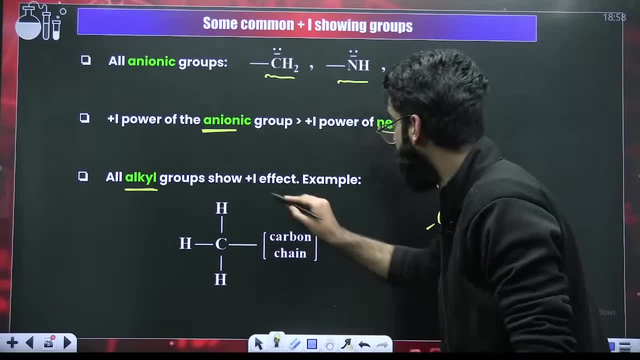 they always show plus I. That means they are electron donating or withdrawing. They are electron donating. Why they are electron donating? Have a look on this one as well. Imagine this is ch3.. What to imagine? This is ch3, right. 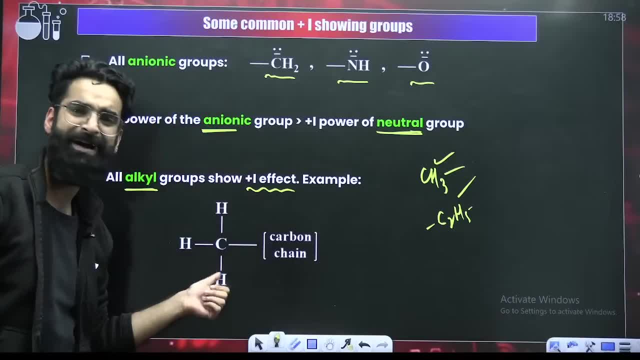 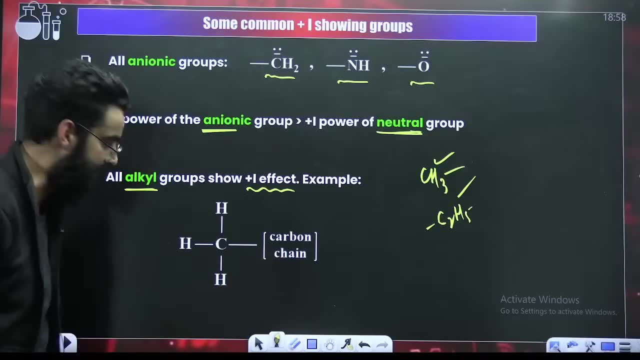 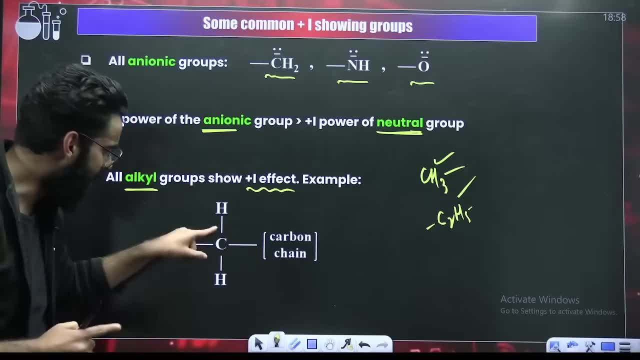 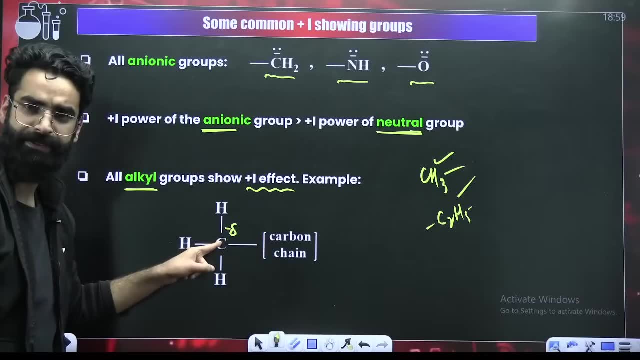 Now, among carbon and hydrogen, which one is more electronegative? You tell me, Among carbon and hydrogen, carbon is more electronegative. So this carbon will be definitely getting delta negative Right, Because carbon is more electronegative. 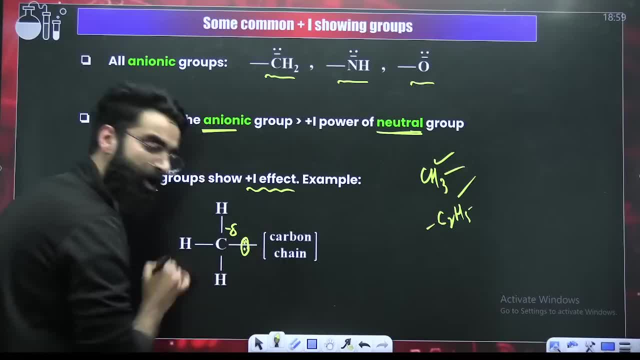 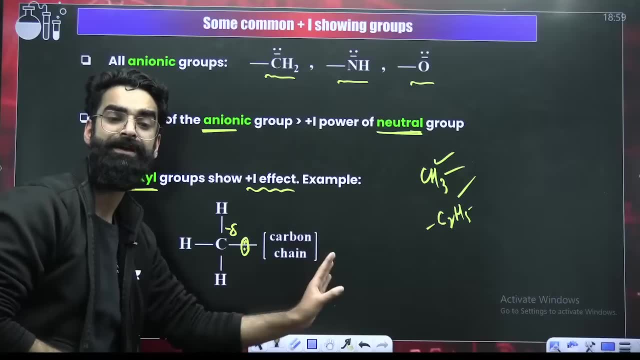 If carbon gets delta negative, there is a bond pair here. There will be repulsions. There will be repulsions. This negative charge will repel this bond pair and will push the sigma electron density in the chain. If it is pushing the sigma electron density in the chain, 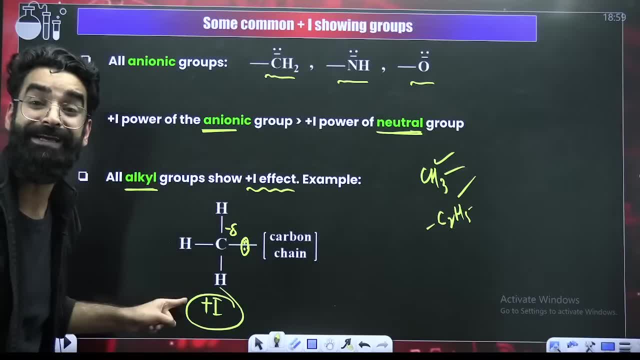 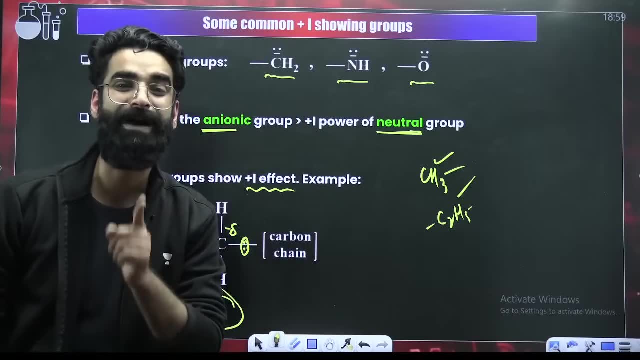 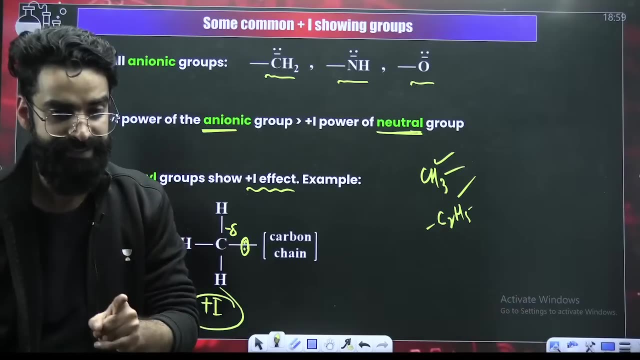 I'll say this particular group, is it donating or withdrawing? this is donating and you're donating. here are called as plus i all your alkyl groups, be it methyl, ethyl, propyl butyl, whatever i'll right, they're always going to be donating, right, as per plus i. yes, let me know in the chats quickly. let me know in the. 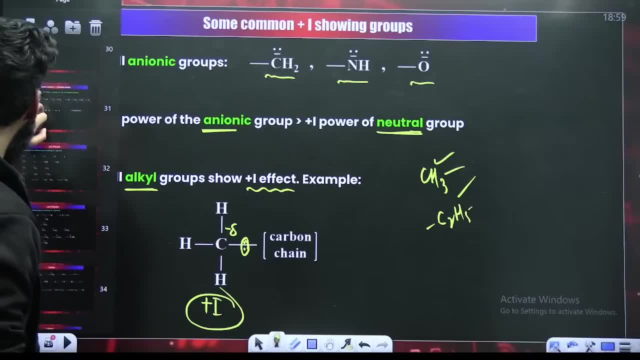 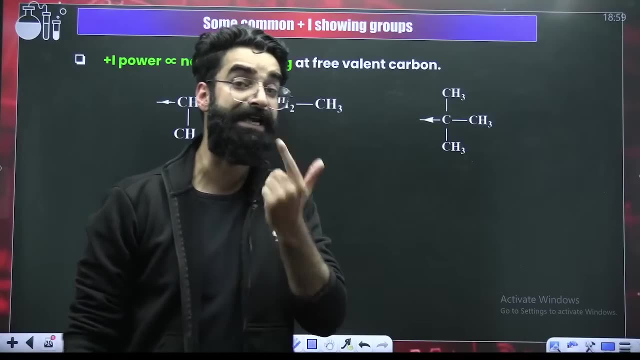 chats quickly. people, let me know in the chats quickly everyone. everyone means everyone, everyone means everyone quickly. i'll tell you one more important statement. there are two, three, few things which i need to tell you about inductive effect. then we'll see its application, we'll see. 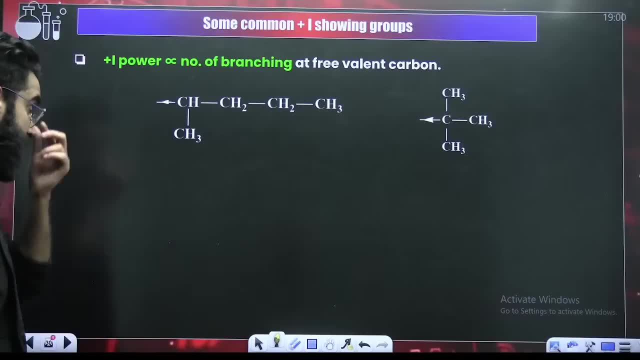 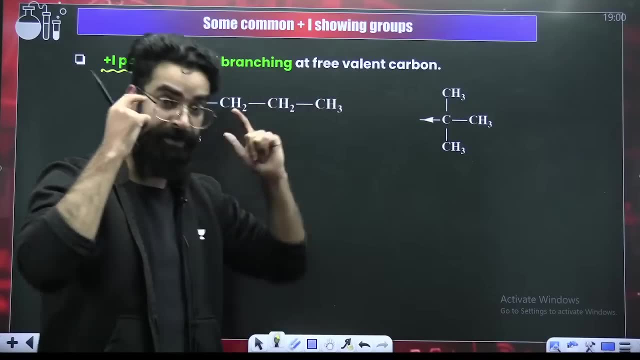 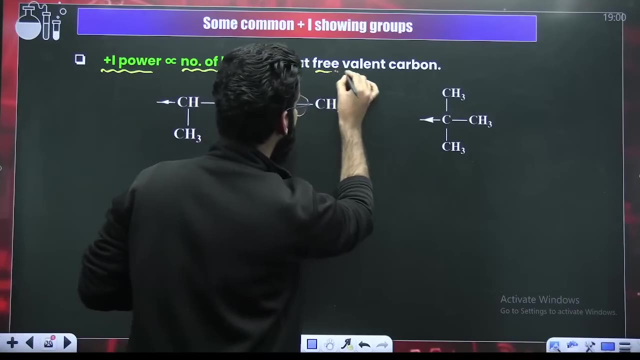 the types of questions which are asked. my dear students. one more important thing: plus i. whenever you hear the term plus plus means electron donating, and right now i'm talking about plus i power, plus i power. it is directly proportional to number of branching at the free valent card. 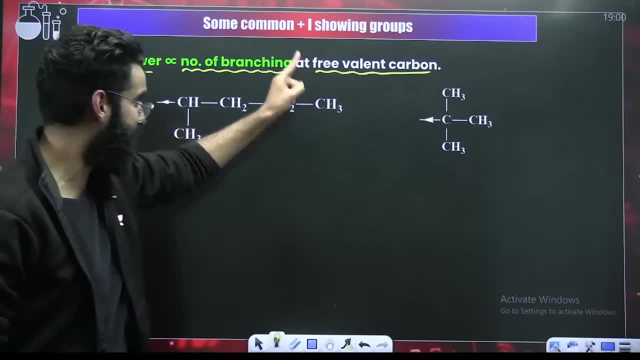 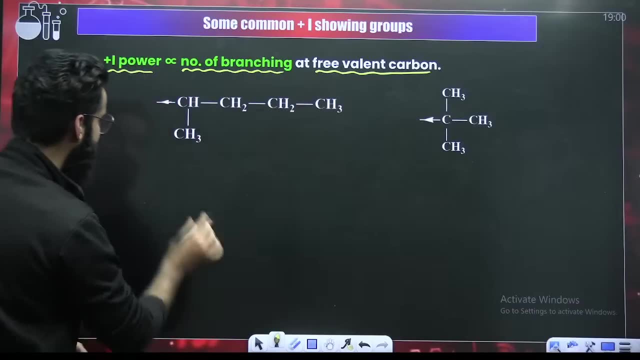 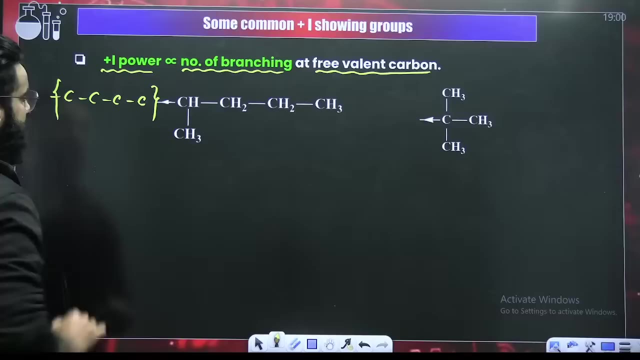 plus i power. it is directly proportional to number of branching at free valent carbon. what does it mean? imagine this is a group. imagine this is a group. imagine you are attaching this group with a carbon chain. imagine you're attaching this group with a carbon chain. this is a carbon chain with. 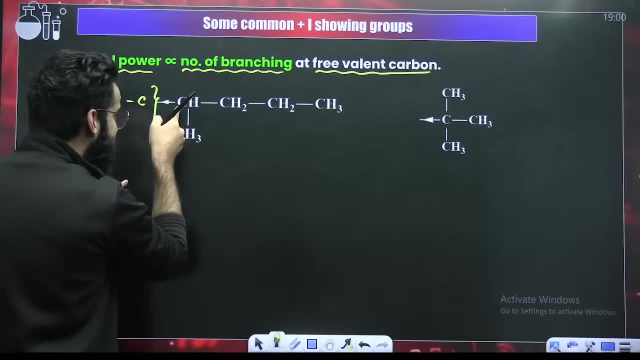 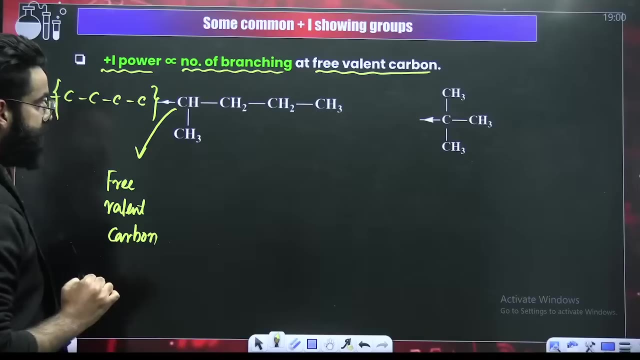 which you attach the group, that carbon of the group, that carbon of the group which is directly attached with the chain. you'll be calling that as free valent carbon. this is your free valent carbon. this is your free valent carbon as per this particular statement. 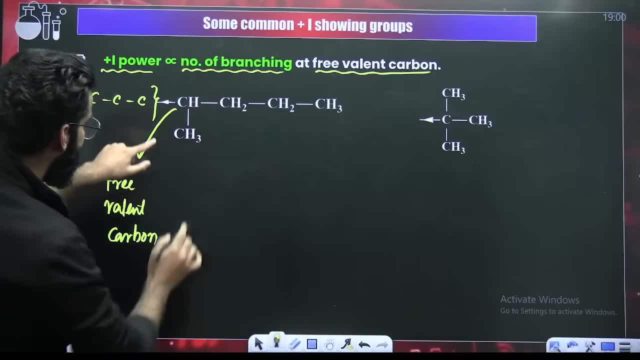 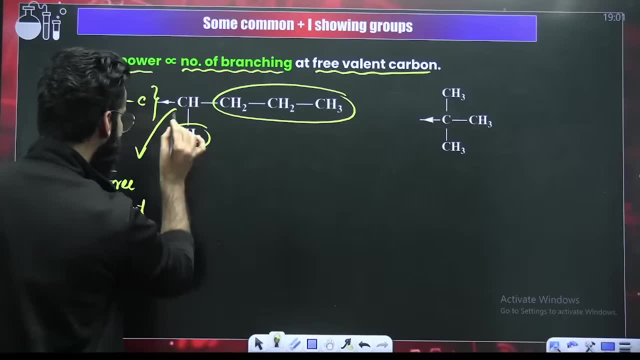 plus i power is directly proportional number of branches. if i ask you how many branches this free valent carbon has, this is one of the branch which it has, this one more branch. so this free valent carbon, it has got two branches here. it has got two branches here right. look at the other case. 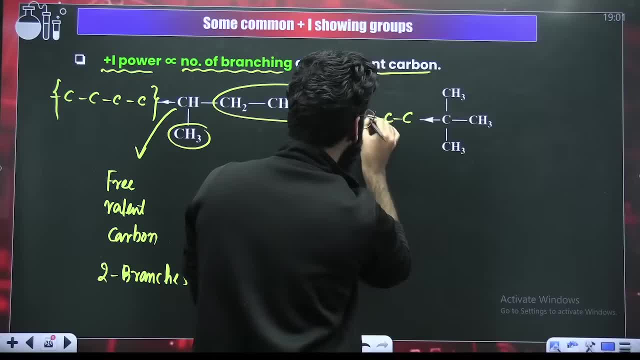 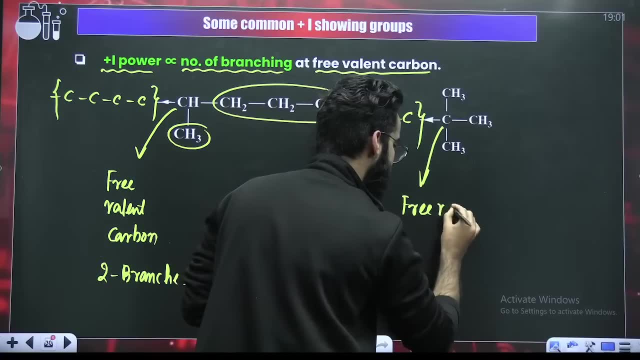 if this is the group and you're attaching this with a carbon chain, you're attaching this with a carbon chain. this carbon is directly attached with a carbon chain. so this is your free valent car, this is your free violent carbon. and one, two and three. there are three branches which. 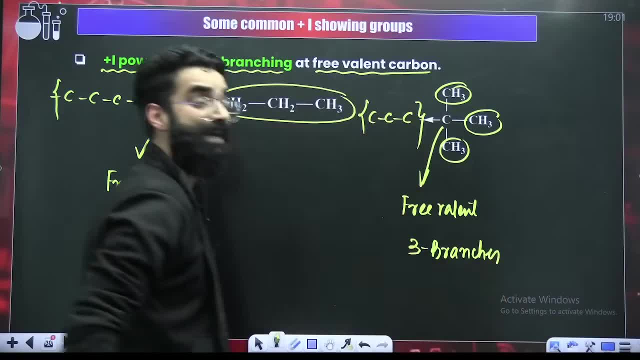 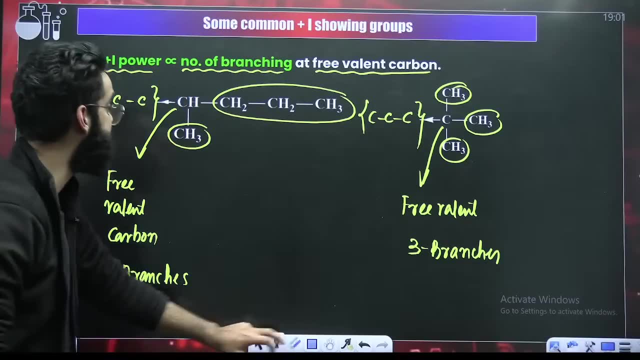 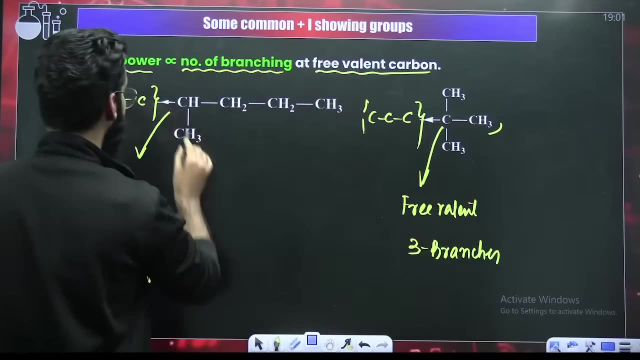 are associated with the free valent carbon. do remember one thing: more branches means more plus. more branches means more of a sign. more branches means more of a sign. now you tell me. you tell me one simple thing. you tell me one simple thing if i talk about this particular 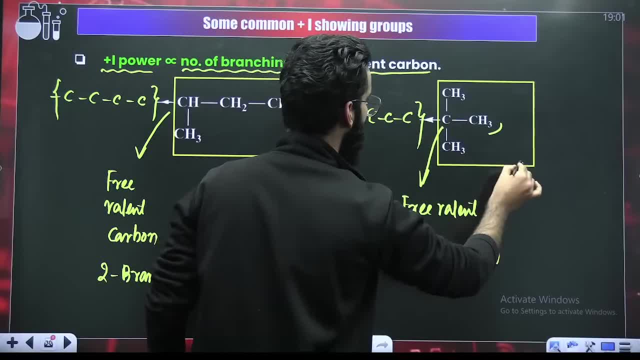 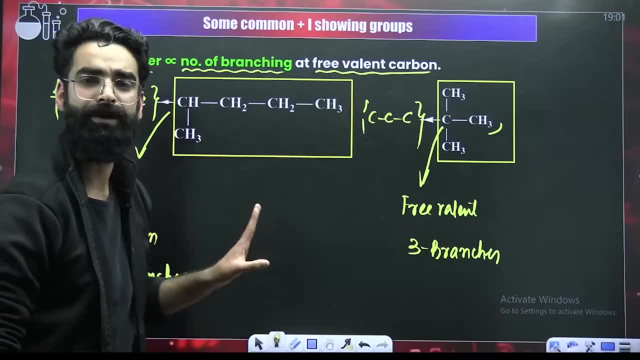 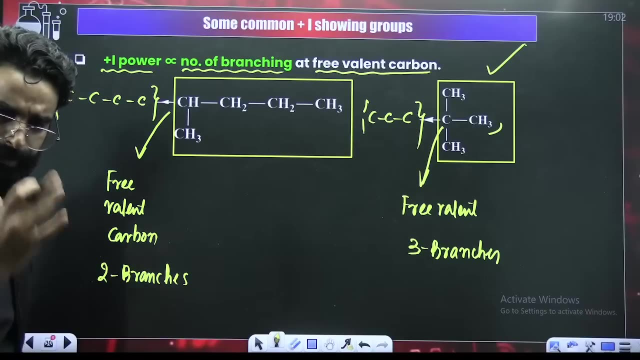 group. this is group one and this is group two. which group is maximum branched at the free valent carbon? the second one, right, so it's plus. i power be more. so this group will have more plus i power. as simple as that. because branching is more. yes, simple, simple, now, now. now, if the branching 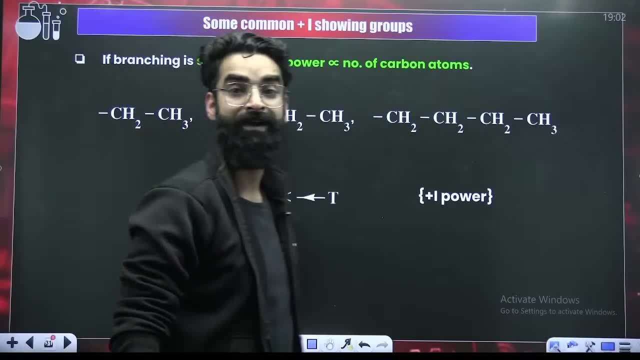 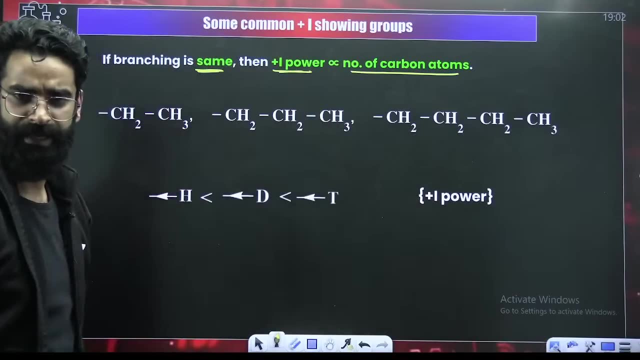 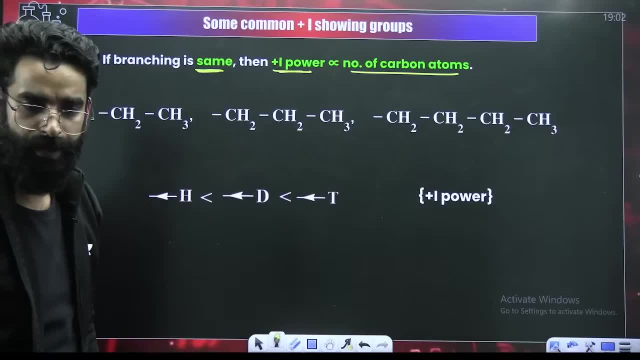 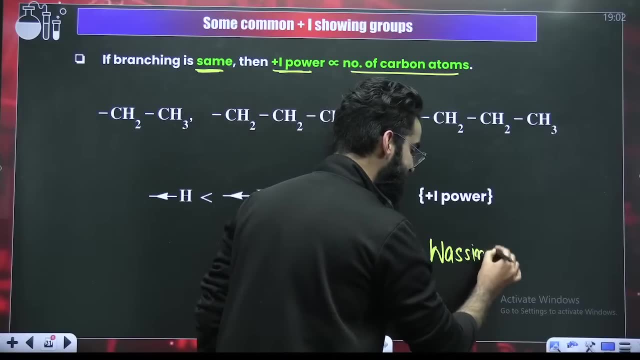 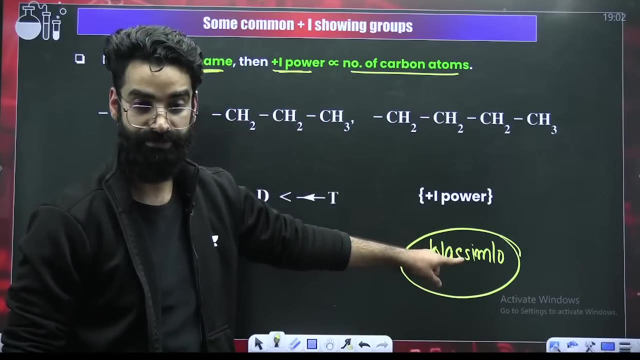 uh, invite code for tomorrow's 11 am extra problem session. this is, guys. it might ask you: the code was seen, one zero. is the code was seen? one zero is the code for tomorrow's or tomorrow's 11 am extra problem session of goc? okay, perfect, all right. 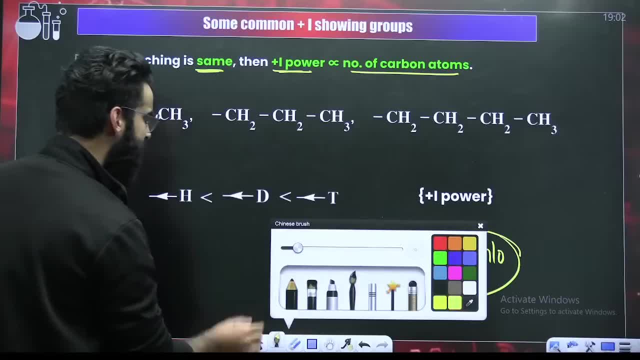 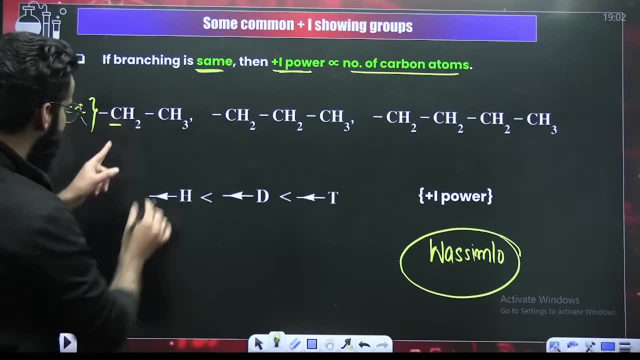 look at this particular thing, guys. what? what i was talking about. if the branching is same, for example, this is the group which is attached to the carbon chain. this is the carbon chain. for example, this is the free valent carbon. if this is a free valent carbon, how many branches? just one branch. 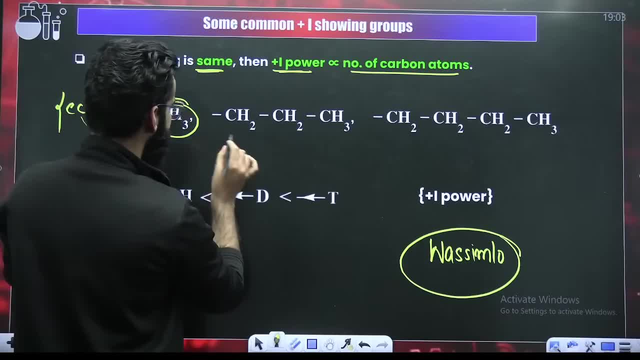 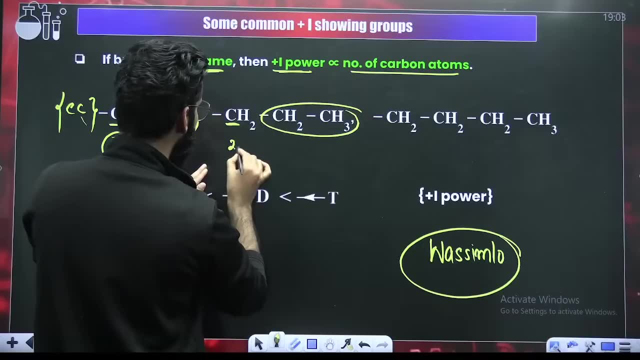 it has, right, one branch it has. similarly, if this is the group, if it is attached with a carbon chain, this is a free valent carbon. here it's a free valent carbon. how many branch it has. it has two branches, right, this is the free valent carbon. here it also has got one branch only. why am i? 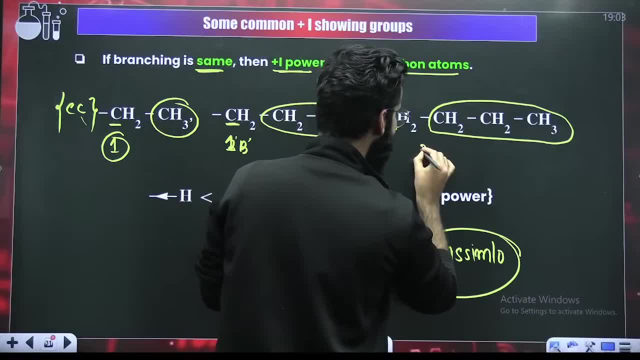 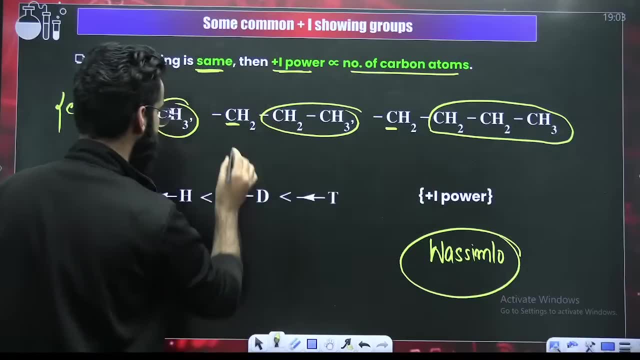 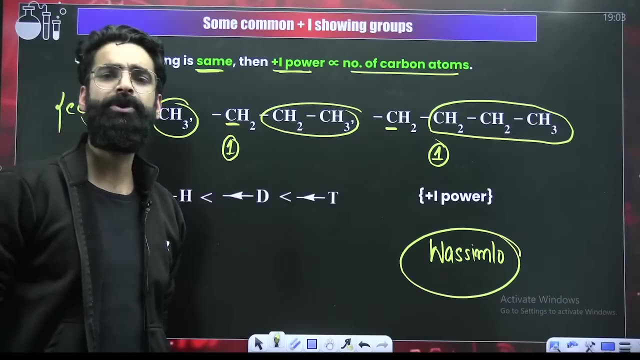 writing two branch. it has one branch, right, this particular carbon, how many branch it has, it also has one branch, perfect. so, whatever free valent carbons we had, in these three cases, all the free valent carbons are having one one branch, perfect, one, one branch. now, if the branching is same, how? 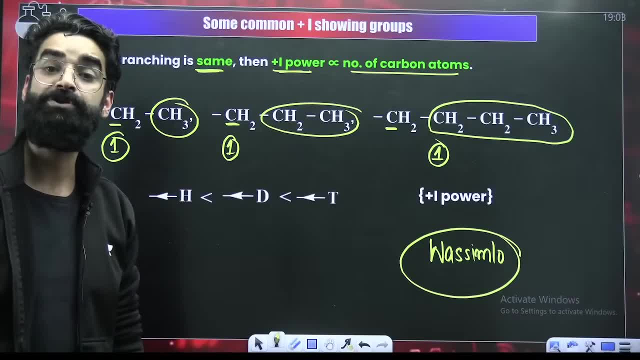 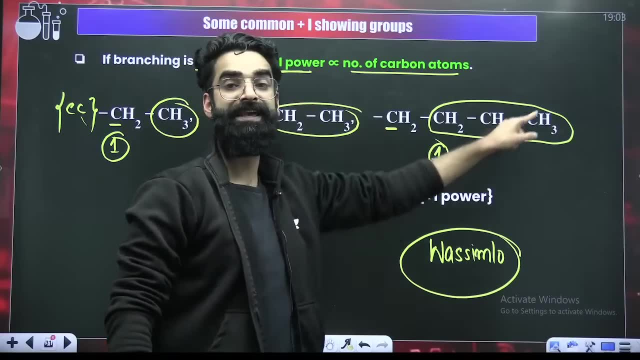 do you relate? plus i power, plus i power is directly proportional number of carbon atoms. tell me in which branch carbon atom is more. carbon atoms are more here, so this particular group will be showing more plus i. this will be showing more plus i by this particular one, followed by this particular one. so do remember if the branching is different. 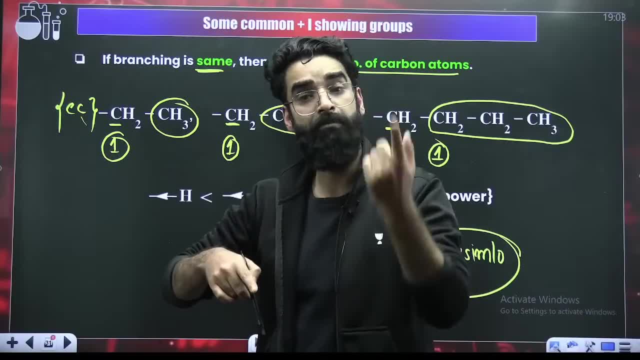 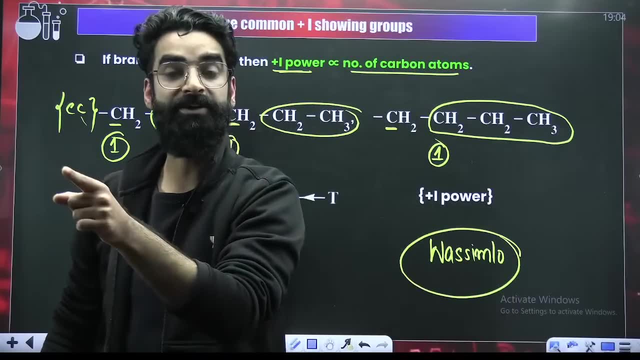 more the branches, more, more the branches at free valent carbon, more the plus i. if the branching is same, then then what do you have to do? then you have to look at the number of carbon atoms in the branch. more carbon atoms in the branch means more plus i. i believe this is clear. 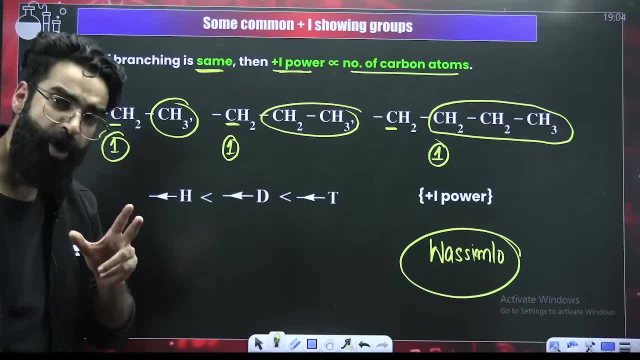 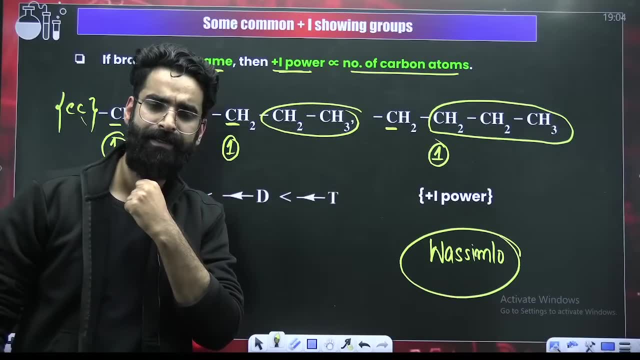 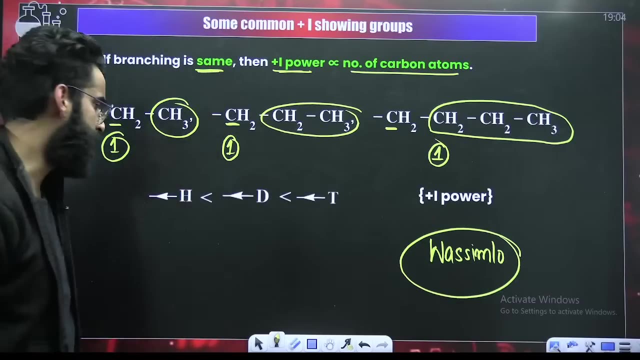 yeah, perfect. similarly, if you talk about hydrogen, do you know how many isotopes of hydrogen do we have, how many isotopes hydrogen has? you should know it. how many isotopes hydrogen has, quickly three: protean deuterium tritium. protean deuterium tritium. 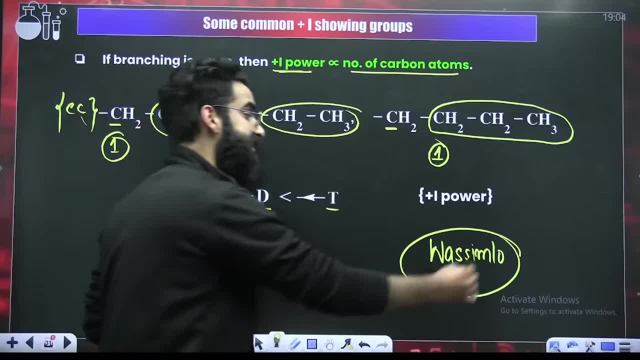 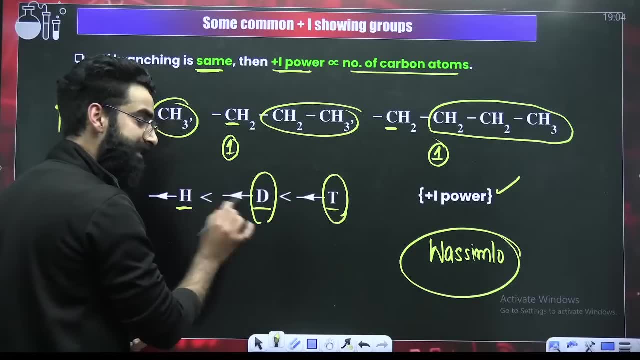 and all these isotopes of hydrogen. they show plus i power. we see, they show plus i power, and do remember: plus i power of tritium is maximum, then that of deuterium, then that of hydrogen is maximum, then that of what? then there are protean. on this particular thing, again, there will be few questions. 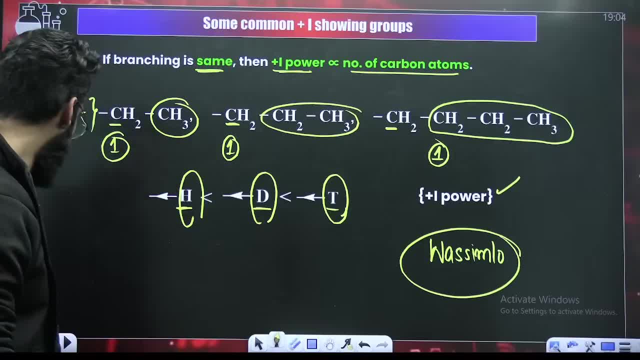 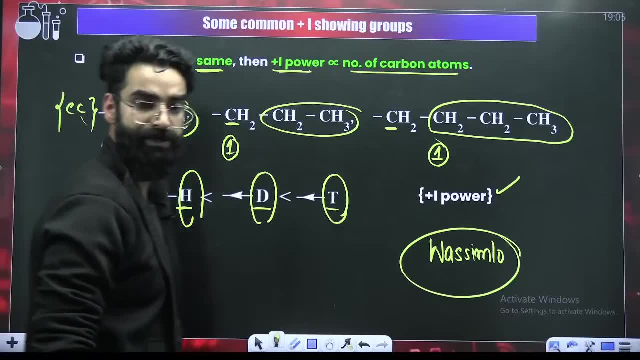 that should be asked. perfect. are you ready to solve the questions now? are you ready to solve the questions, people? are you ready to solve the questions? are you ready to solve the questions? are you ready to solve the questions? you can only solve the questions if you remember all. 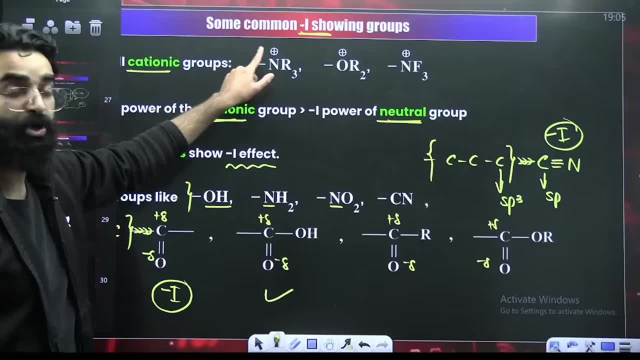 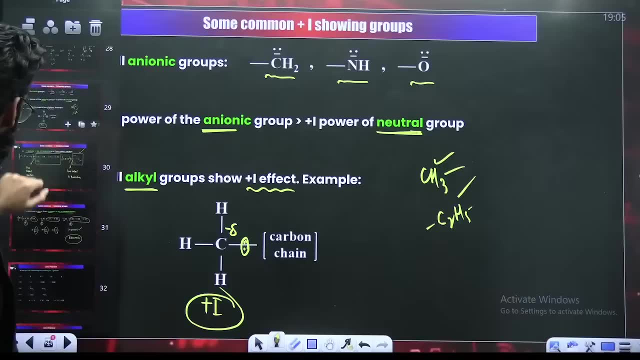 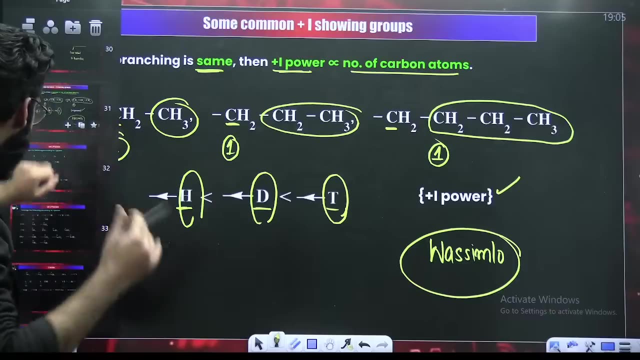 these things- this was the first thing which you have to remember- some common minus- i showing groups. remember these particular points: common plus- i showing groups, right. similarly, branching right, how it affects, how it affects a particular set of questions i'm going to give you you have to answer. you have to answer a particular set of question. there is a lot. 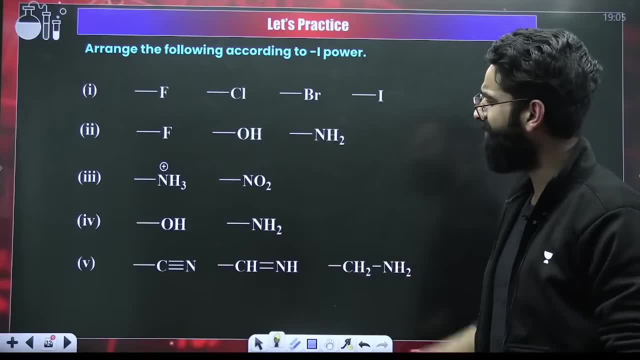 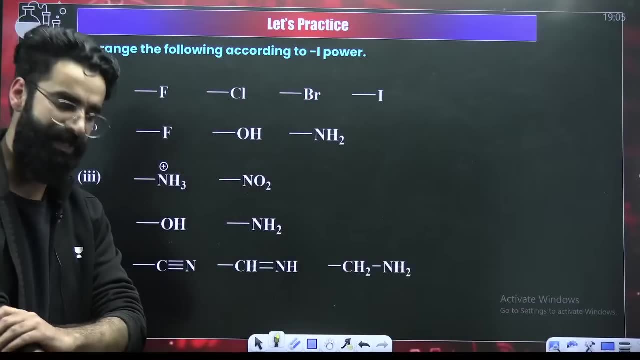 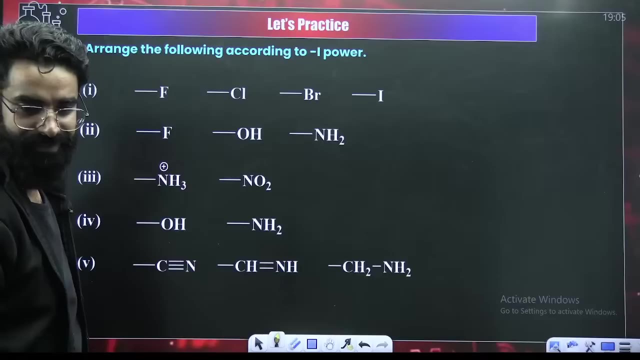 of application. as per this inductive effect right a particular application, arrange the following according to their minus i power. arrange the following according to their minus i power you tell me. arrange the following as per their mindset power: quickly, quickly guys. chlorine, chlorine, bromine, iodine, which one will be having more mindset? 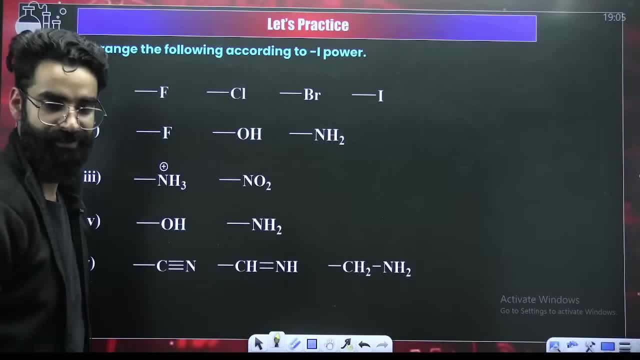 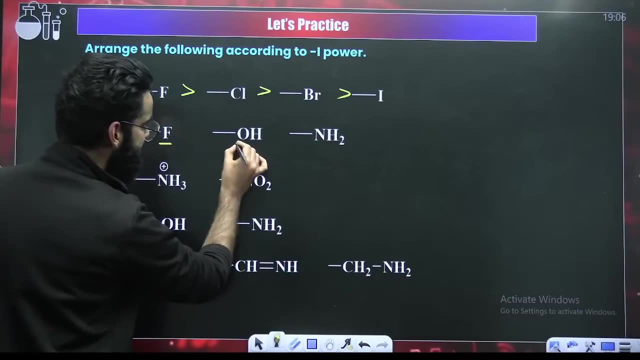 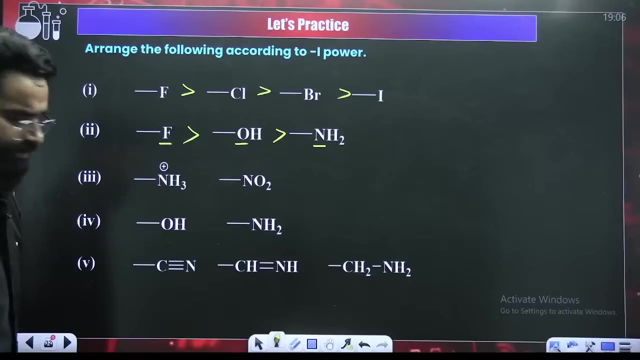 which one will be having more mindset. you know it, chlorine is more withdrawing than chlorine, then bromine, then iodine. right, chlorine attached with carbon chain, oxygen attached with chain, nitrogen attached with chain. which one is more withdrawing? this will be more withdrawing, simple. this is a cationic group, this is a neutral group. all the cations. 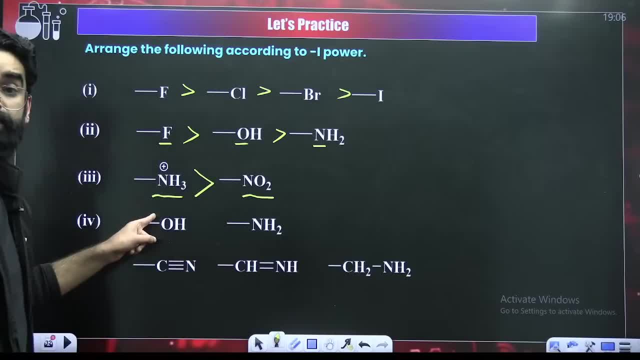 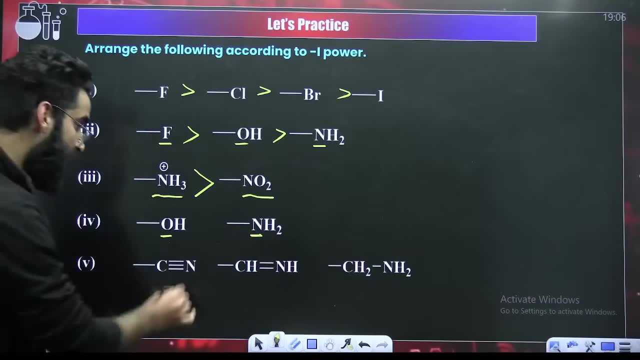 tiny groups. they have got more plus sign, sorry, more minus sign. so this more withdrawing, this more withdrawing. look at the next one: oxygen attached with the chain, nitrogen attached with the chain oxygen is more withdrawing. more minus sign, more minus sign. right, more minus sign. this is your sp. hybridized carbon, because it's forming two sigma bonds. this is your sp2, this is your sp3. 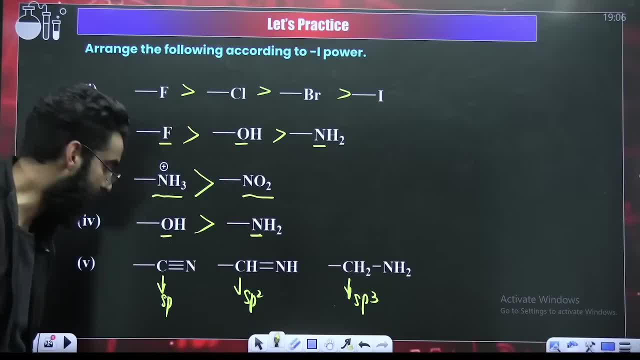 this is your sp3. where is the s character? more s character is more here. electron negativity is more here, so it will be more withdrawing. this will be more withdrawing. this is how you arrange these groups on the base of their minus i power. simple, simple. this is how you are going to arrange. 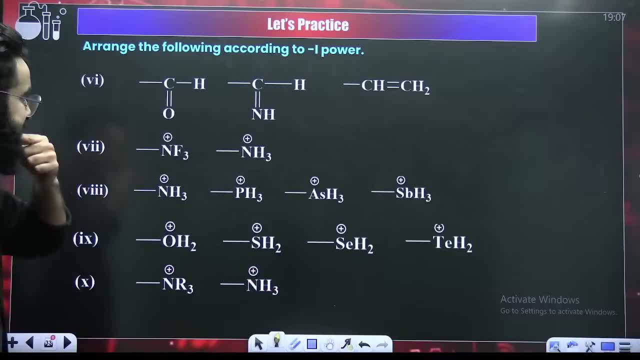 them on the base of their minus. i power now, tell me about these. tell me about these: among these three, one, two or three, which one will show more minus? i power all the concepts. i gave you all those concepts. only you have to utilize all those concepts. i'll give you a break once inductive effect is completed. inductive effect. 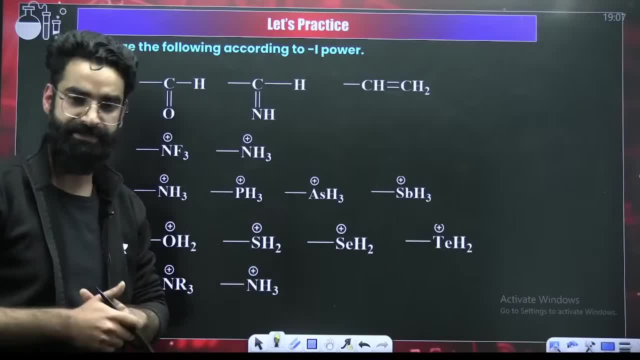 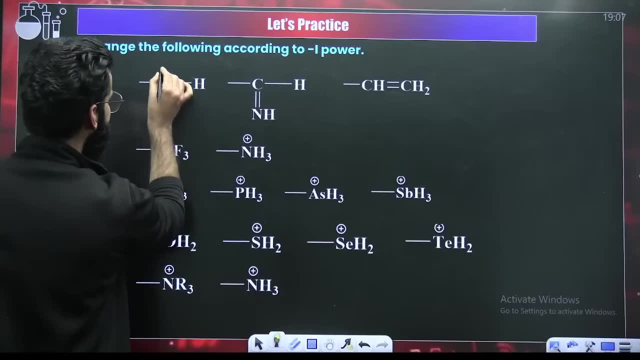 and its application part is completed, then i'll give you a break and after the break we'll start the resonance quickly. it's very evident, guys: if this group is attached with a carbon chain, this group will carry delta positive, because oxygen carries delta negative- electronegativity difference. 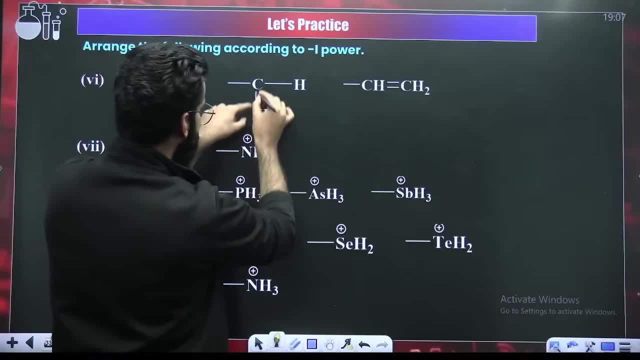 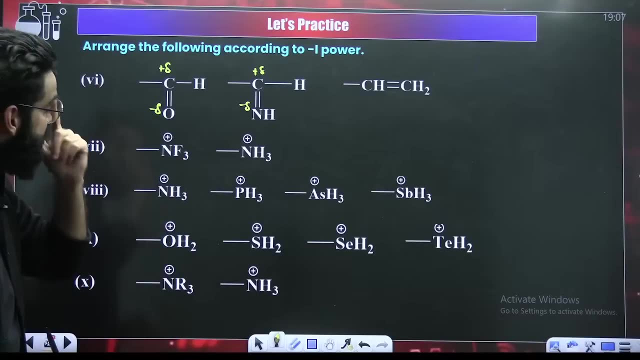 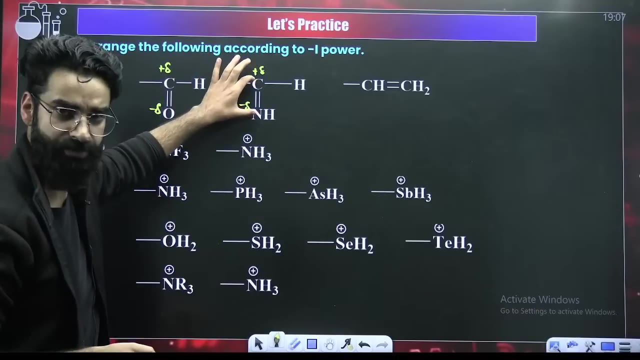 oxygen is more electronegative. so delta negative, delta positive. even this, there is electronegativity difference here. so this delta positive, this delta negative, right, perfect. now you tell me just one thing: carbon-oxygen electro-relativity difference is more than that of carbon nitrogen. if the electro-relativity difference hair is more, that means the magnitude. 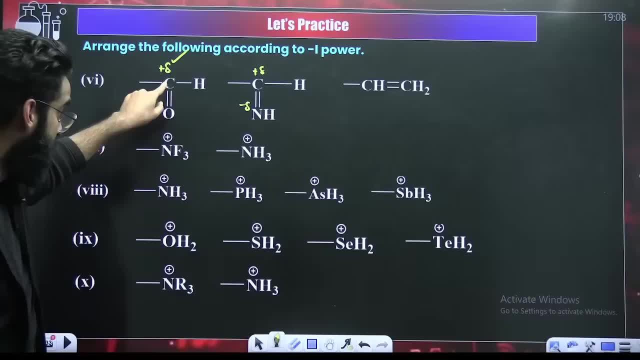 of positive charge here is more, right. so magnet magnitude of positive charge here is more than that of magnitude of possible charge here, right, if the magnitude of positive charge there is more, can i say it will? it will pull sigma electrons more towards itself, right? so what has to be the electron withdrawing nature myself? externality sounds good to me as an 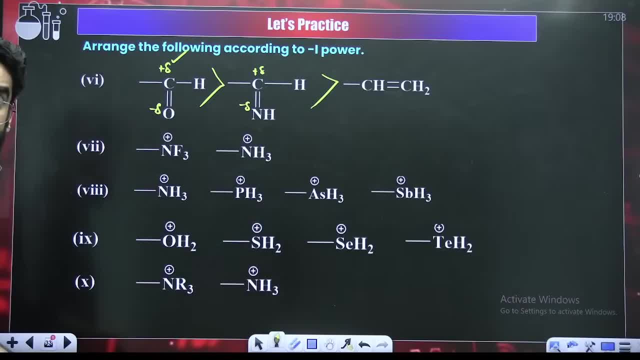 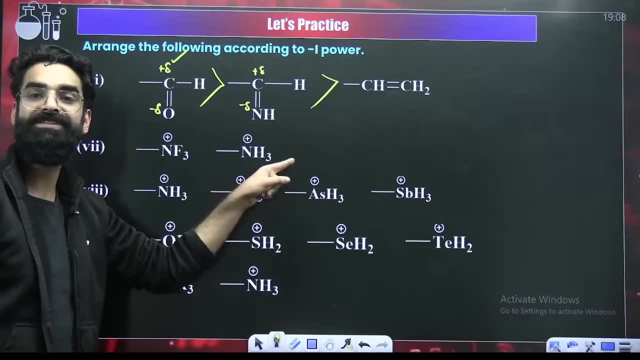 Mind-side power. This is the mind-side power, Simple and basic Right. NF3, NH3.. Both are cationic groups, NF3, NH3.. Here nitrogen is attached with fluorine. Here, nitrogen is attached with what? 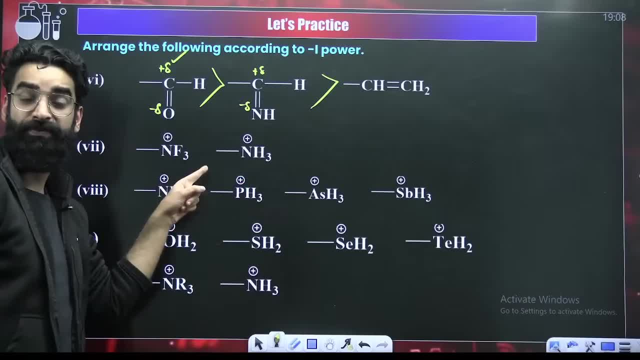 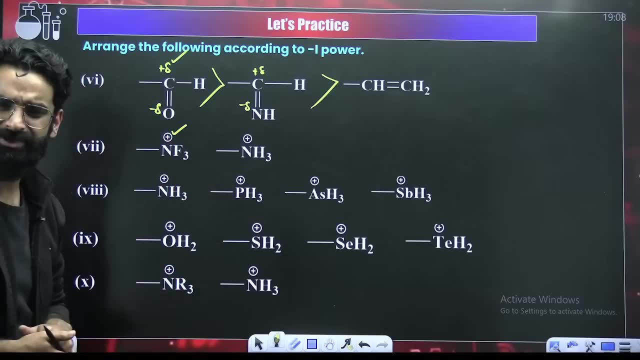 It's attached with hydrogen. Fluorine is more electron. Fluorine is more electron negative than nitrogen, So fluorine will increase the intensity of positive charge on nitrogen. Fluorine will increase the intensity of positive charge on nitrogen, Due to which it becomes more withdrawing. 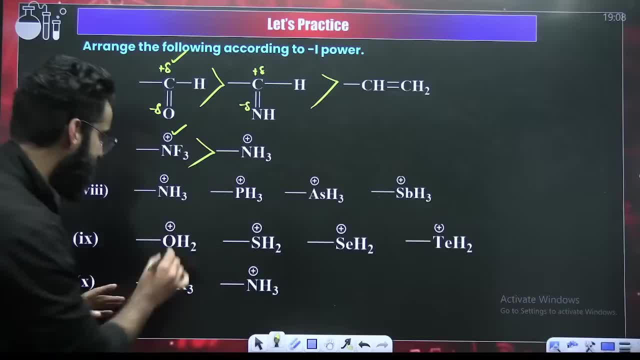 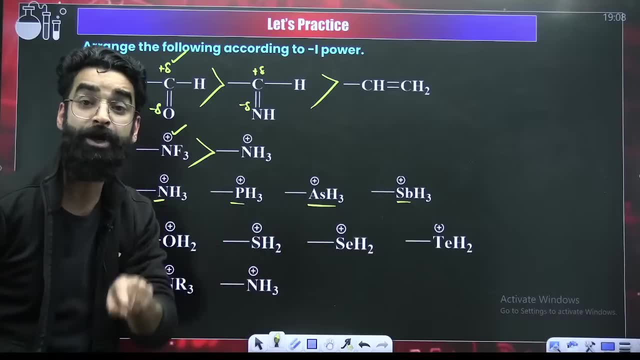 Right, But NH3,, pH3, ASH3.. One simple thing: Nitrogen, phosphorus, arsenic, antimony. Do they belong to same period or same group? They belong to same group. In the group, VCD plays a role. 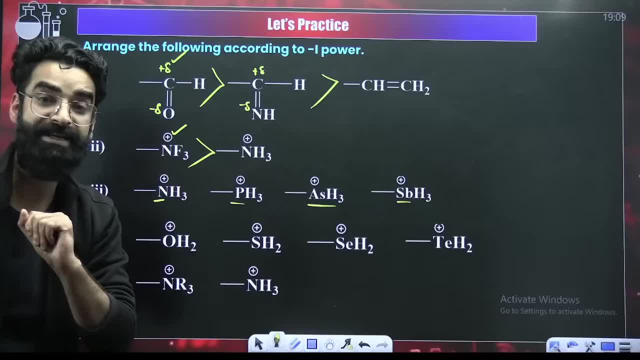 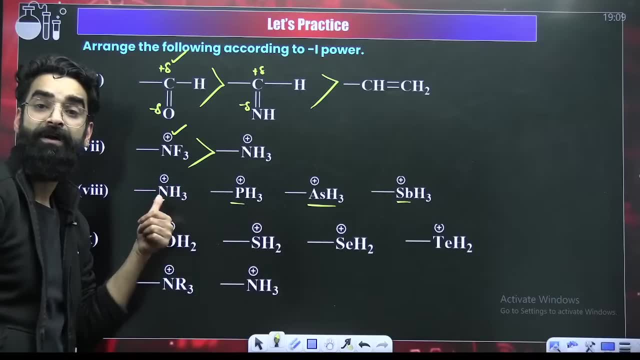 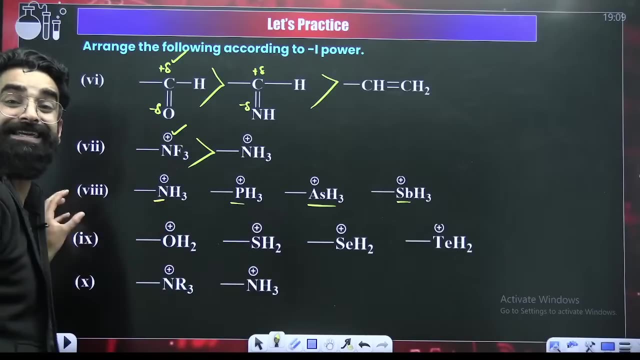 In the group VCD plays a role. Right In the group VCD plays a role. This one has got lesser size. Lesser size means more volume charge density. More volume charge density means more positive volume charge density. If over here you have got more positive volume charge density, 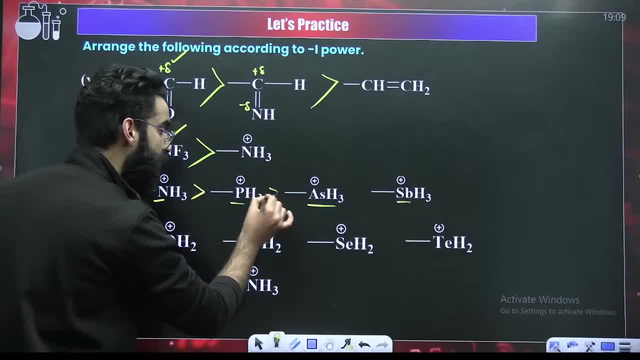 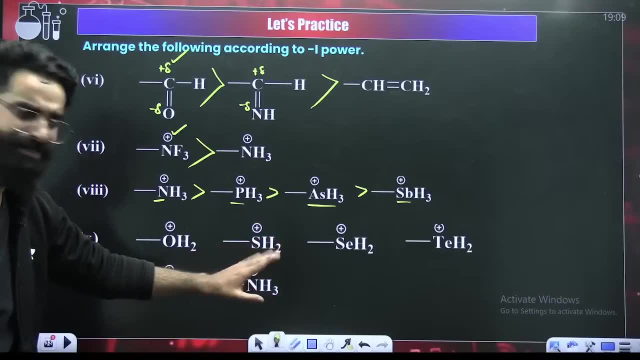 So it's going to move the sigma electrons more towards itself, So it will show more minus. i Simple and basic: OH2 positive, SH2 positive. Same reason. Oxygen carrying positive sulphur SET: Oxygen sulphur SET. 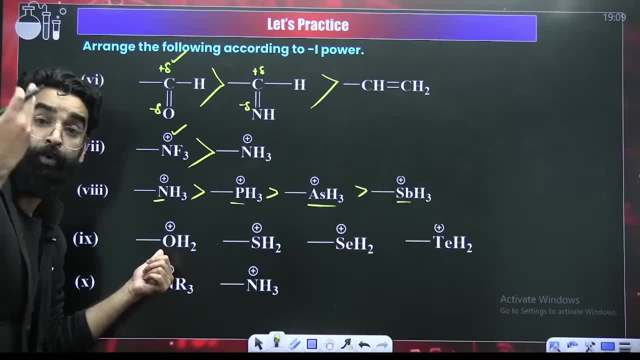 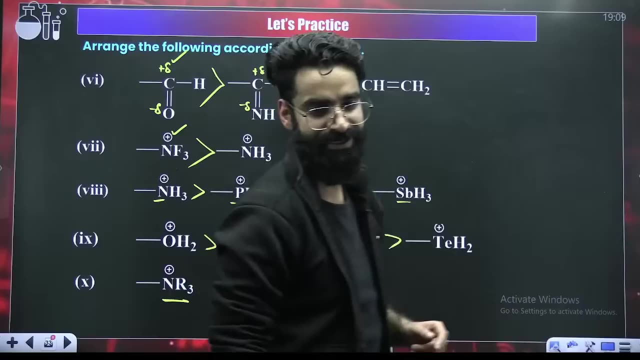 They belong to same group Again: VCD: Lesser size, more positive volume charge density. More positive charge volume density means more withdrawing. So this is more withdrawing, More minus. i. Right Now N are three positive positive, NH3 positive and R3 positive. NH3 positive: Can you let me know in the chats? 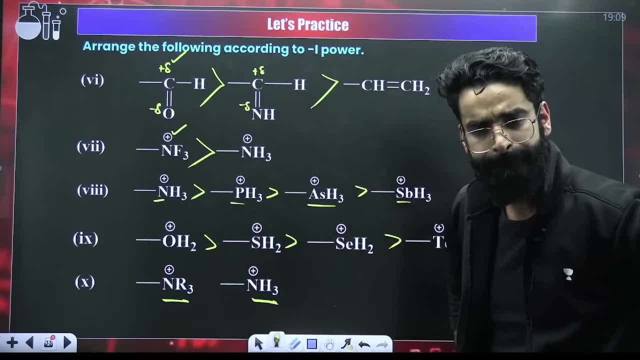 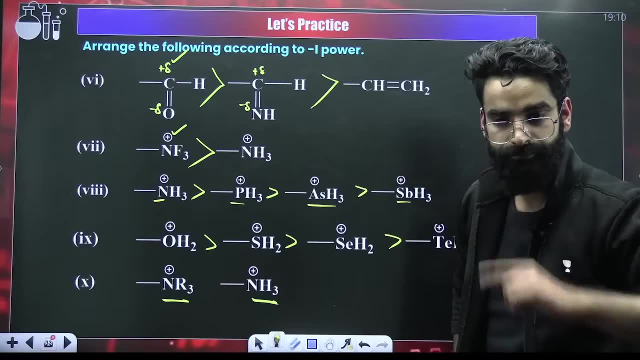 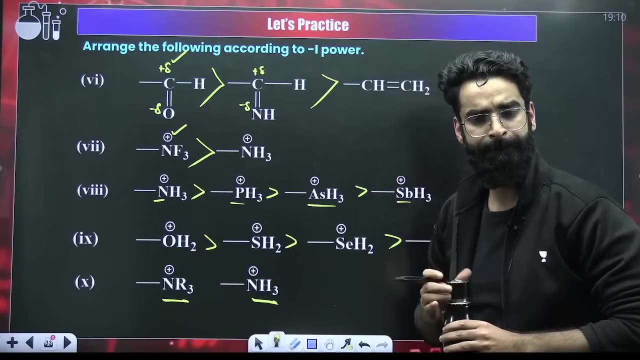 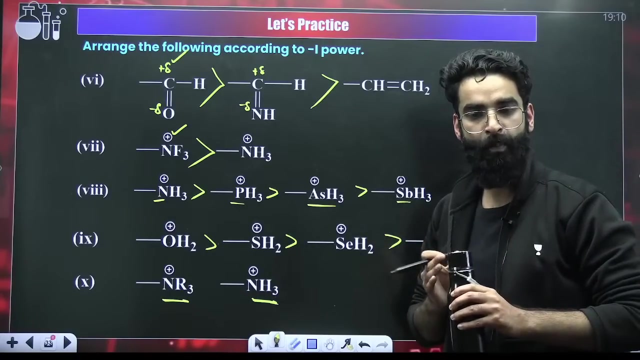 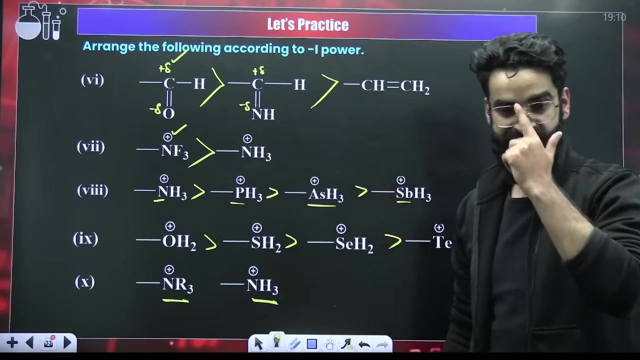 what do you think? Which one will show more minus? I, Quickly. Which one will show more minus? I? I'm asking you- This is the question: I'm asking you Quickly: Which one will show more minus? I Quickly, guys, Everyone quickly. Normally, it seems like this should have more. 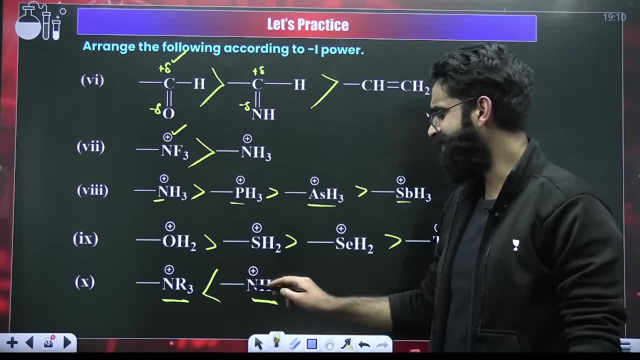 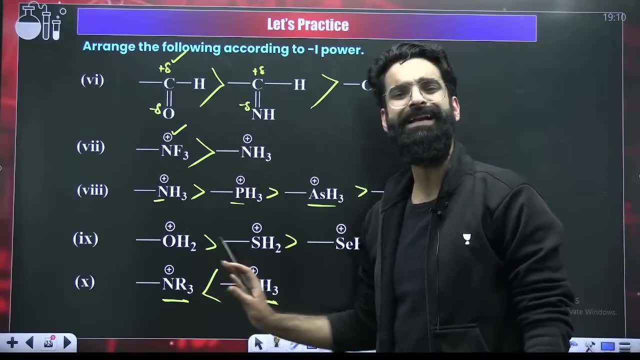 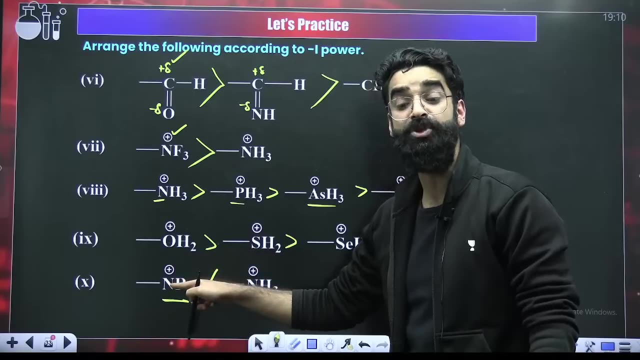 minus I, It seems like, because nitrogen here is attached with hydrogen. Right Here nitrogen is attached with alkyl groups. Alkyl groups are donating, So normally a common man thinks that alkyl groups are donating. Alkyl groups are going to decrease the intensity of positive. 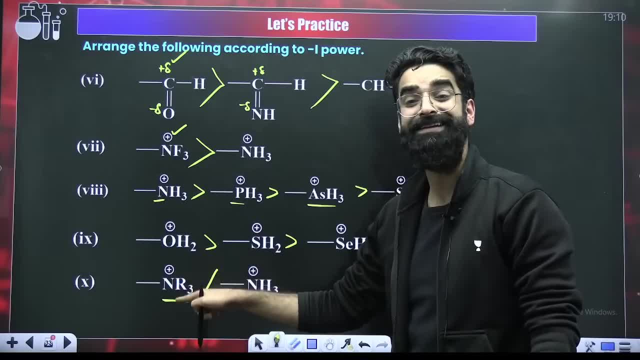 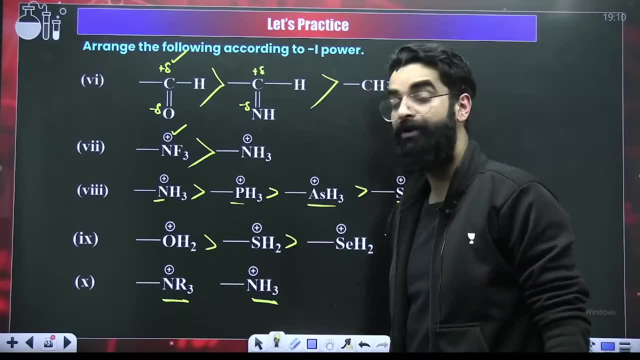 charge. here Alkyl groups are going to decrease the intensity of positive charge here. This has to be more minus. I, Normal people think like that, But we are not going to think like that. We are not going to think like that. See, We have got NH3 positive. This is R. 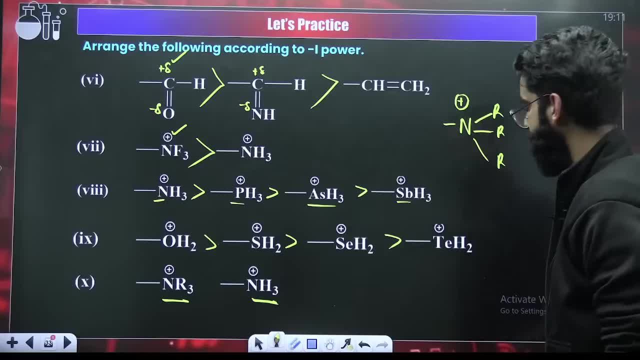 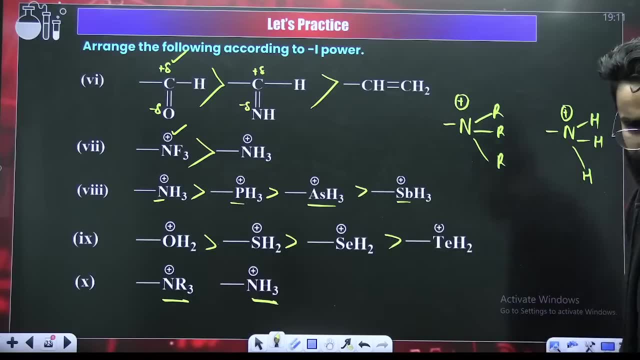 This is R. This is R, Nitrogen carrying positive. This is N. This is Hydrogen. This is Hydrogen. This is one more Hydrogen carrying positive Right, Perfect. Let me first of all tell you, The first one has got more minus. I There. 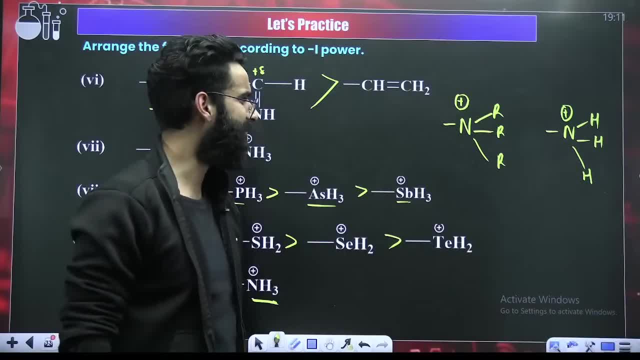 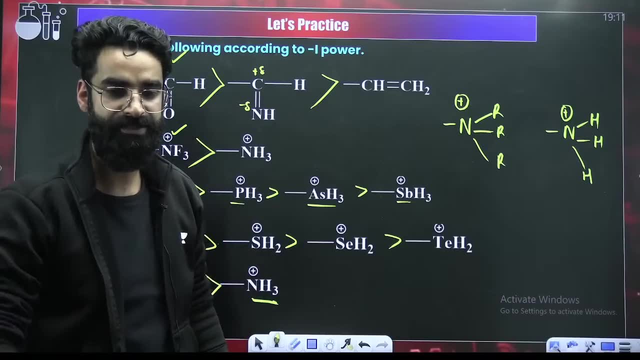 are lot of reasons for it. One reason is solvation, reason Right. Or, in simpler words, just to remember it. Just to remember it, What you should remember, exactly so that you can remember it. Have a look: RRR, Alkyl, Alkyl, Alkyl. Are these bulky groups You can remember it like? 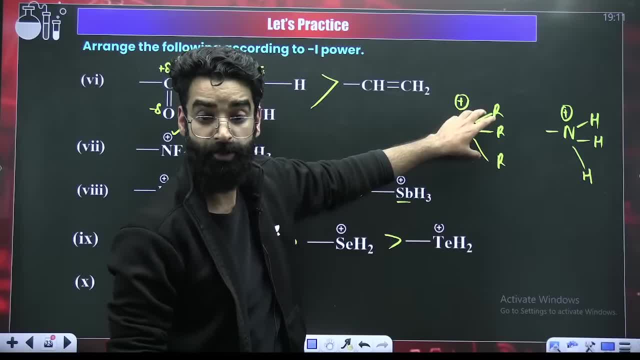 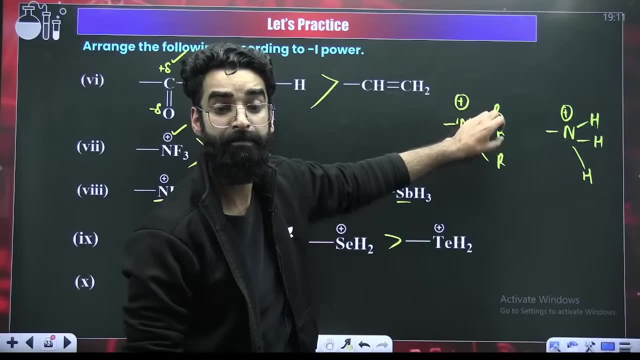 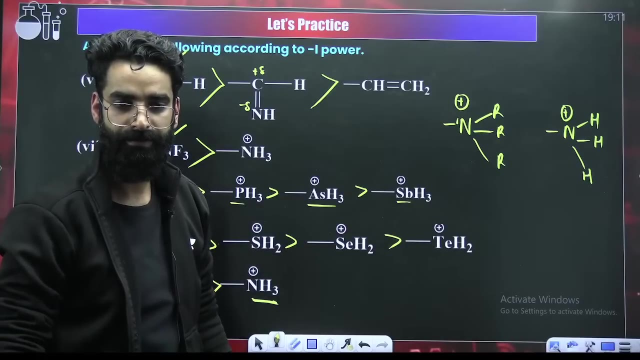 this. Are these bulky groups? These are bulky groups. If they are bulky groups, will there be repulsion? Yes, there will be repulsion. If there is repulsion, bond angle increases or decreases. Bond angle increases. If bond angle increases, electronegativity automatically. Yes, Right. 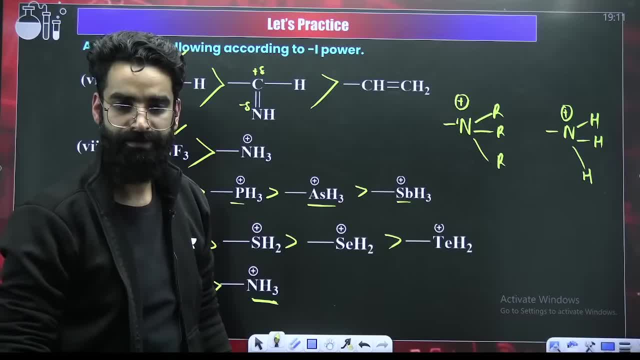 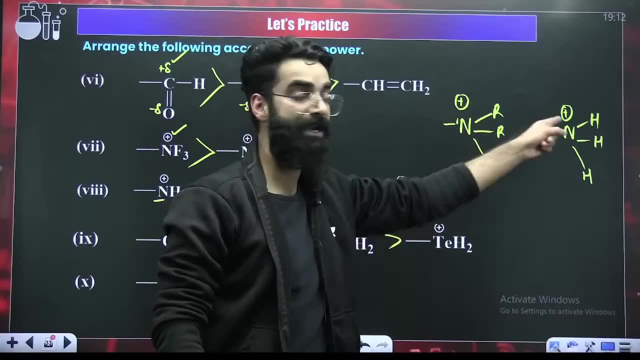 Perfect, Electronegativity automatically increases. So which nitrogen do you see more electronegative here? The first one, Right, This one, You can see this, This one. This is way highereté if first one is more electronegative. 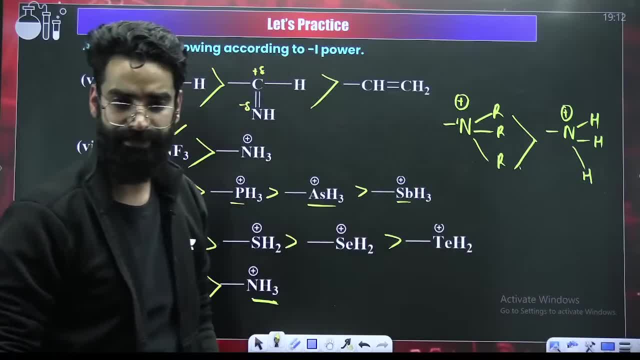 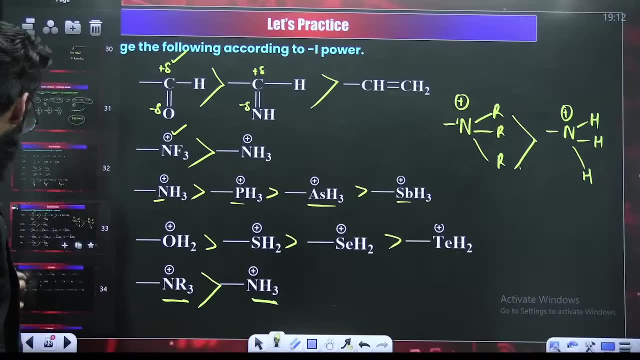 it's going to withdraw more electron density from the carbon chain, So it will show more minus. There is one more logic. that is solvation. I'm not going into the details. Right, I believe this particular statement is clear. I believe these are the questions. 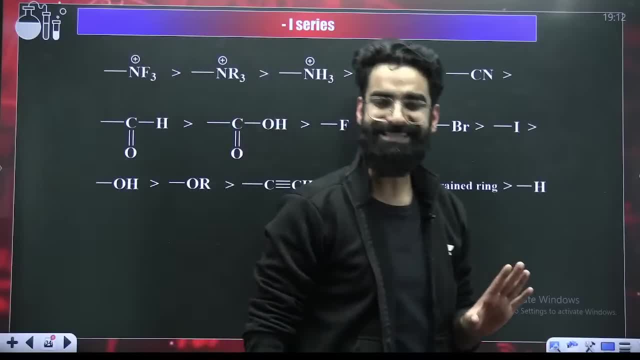 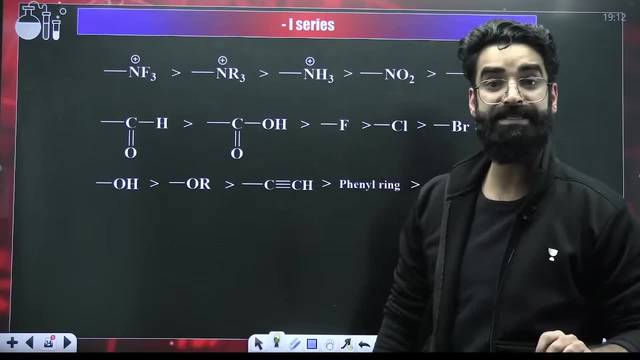 you can easily solve. Now, guys, this is the minus I series, Since I have showed you exactly how to check which one has got more minus I, which one has got more plus I on the basis of all those points. this is the series which you have to remember. 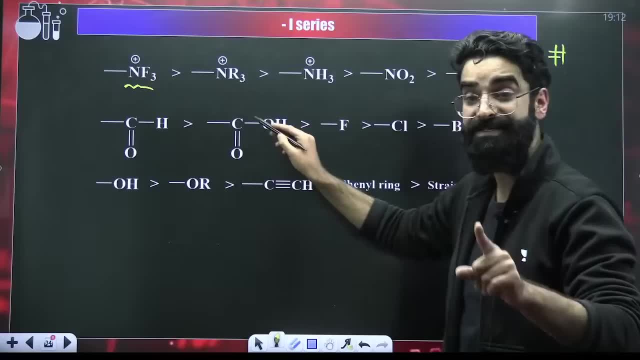 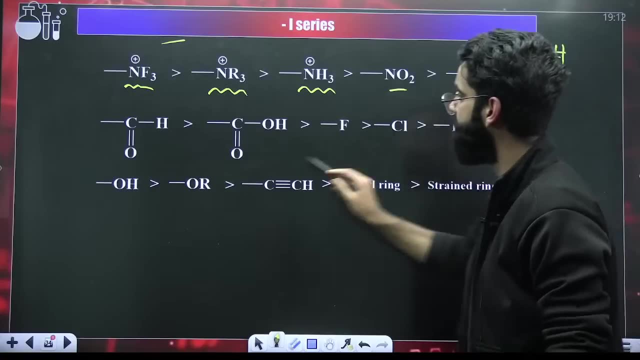 N-3 positive will show maximum minus I power, followed by N-R-3 positive, followed by N-H-3 positive. All these three are cationic groups. Then comes your neutral groups, Then comes these. You have to remember this particular series. 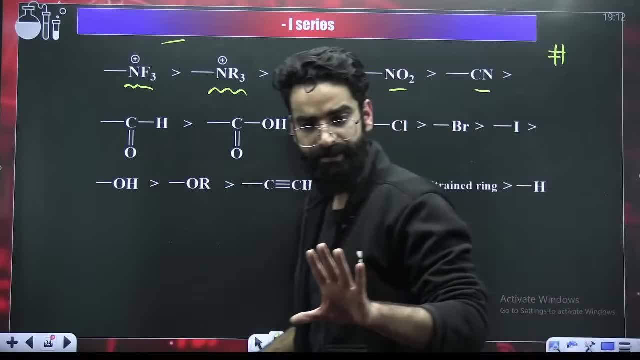 You can create a mnemonic based on your own thing. Yes, Yes, Dhanush, you can watch it Perfect. This is the minus I series. Similarly, there is a plus I series as well. There is a plus I series as well. 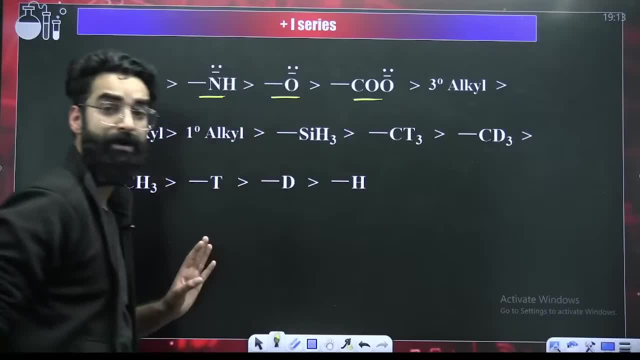 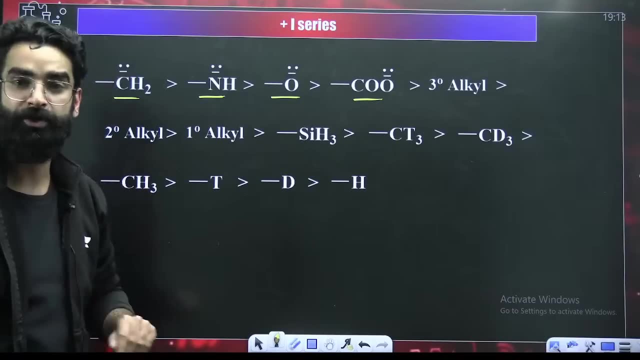 First of all, look at all these. These are anionic groups And you know all the anionic groups they do what. And all the anionic groups they have more plus I power than the neutral groups. So that's why anionic groups are the first. 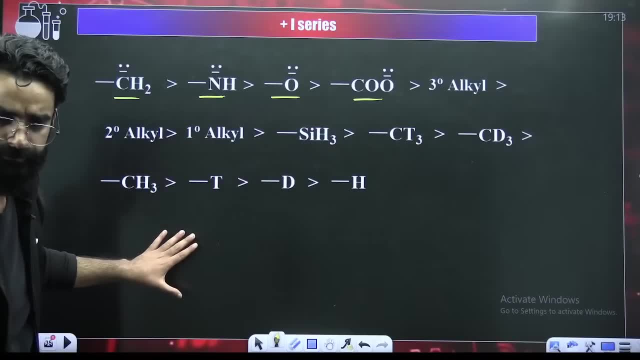 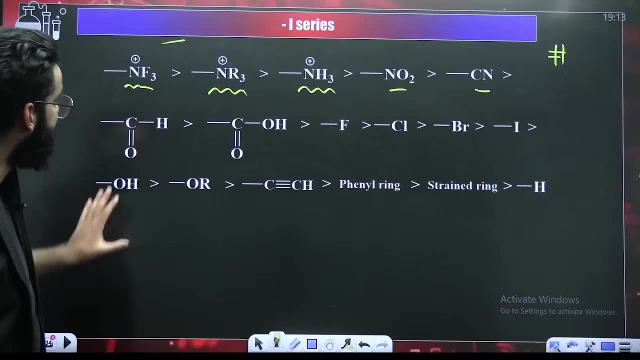 Then comes your neutral and all. You have to remember this particular series as well. You have to remember this particular series as well. One is for minus I series and another series is plus I series. Okay, Plus I series. One thing which I told you already: 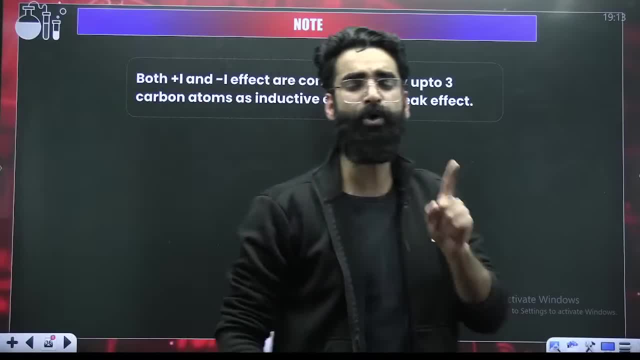 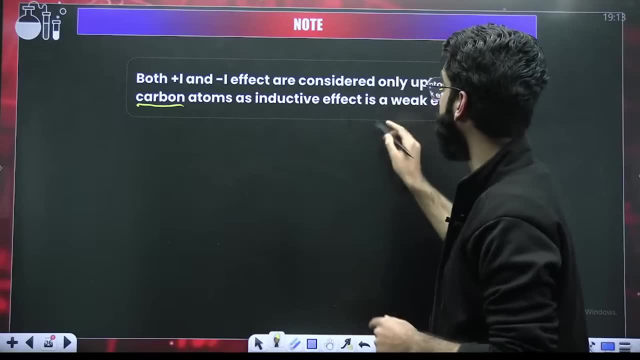 One thing which I told you already. I believe you remember this: Both plus I and minus I are considered only up to three carbon atoms. Both plus I and minus I. they are considered only up to three carbon atoms Because inductive effect it's not a strong effect. 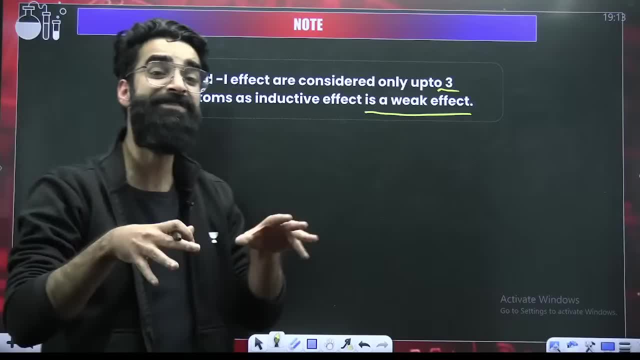 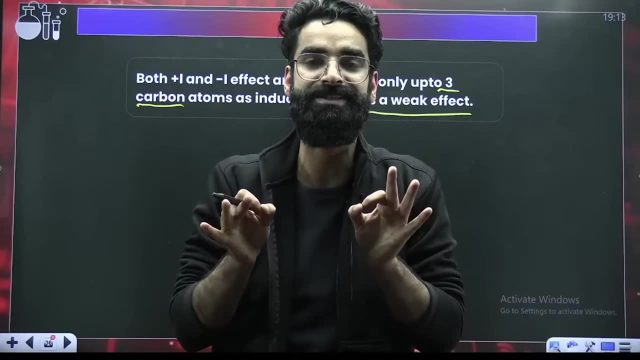 it's a weak effect. Okay, So this was all the theory which was needed in the inductive effect. Now is the time for questions. Now is the time for questions, But before doing the questions, I need to tell you certain things. 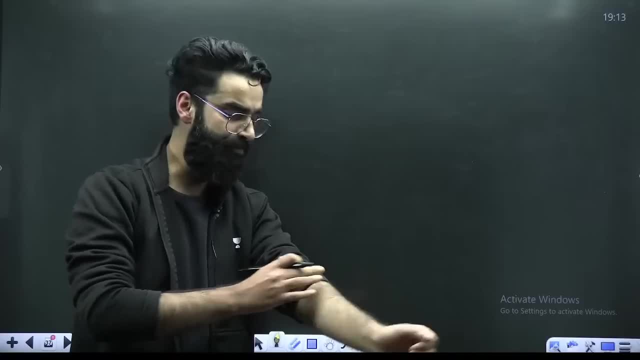 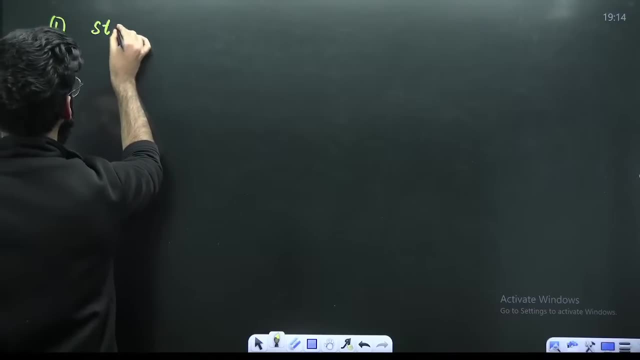 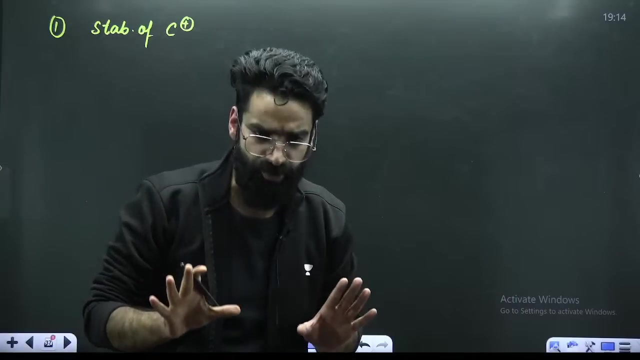 which will help you, which will help you, which will help you in order to solve the equations. My dear students, the first point which I would want you guys to remember, That is stability of carbocations. Stability of carbocations as per inductive effect. As per inductive effect. Remember stability of carbocation. Carbocation is stabilized by electron donating groups. Carbocations are destabilized by electron withdrawing groups. Carbocations are stabilized by electron donating groups. They are destabilized by electron withdrawing groups. That means, in short: 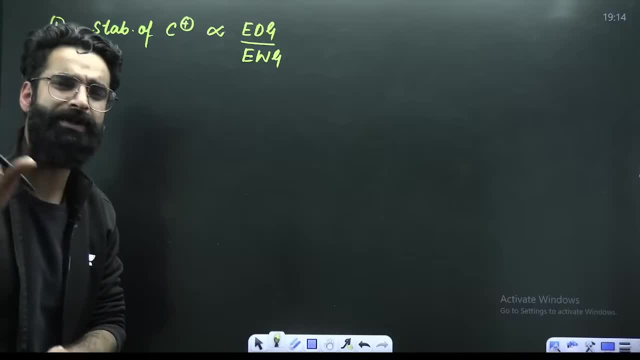 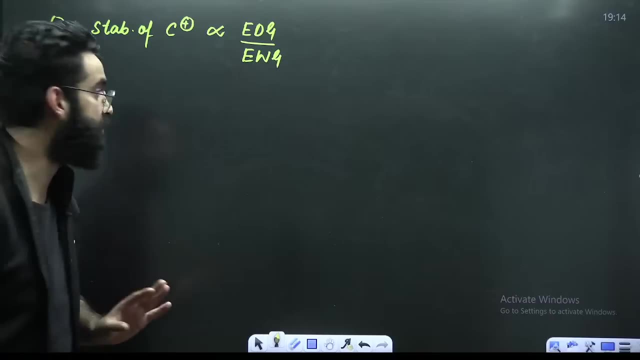 since till now we have studied only inductive effect, so I'm not going to take any other effect into consideration. I'm just going to solve equations as per what. I'm just going to solve, equations as per inductive effect- Electron donating. as per inductive means. 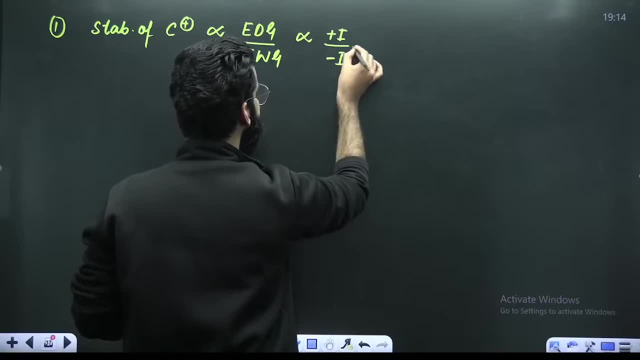 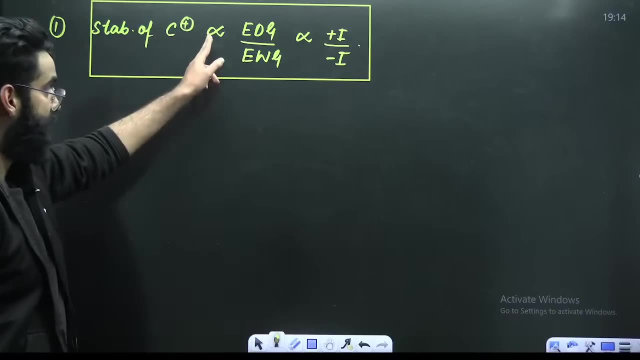 Plus I. Electron withdrawing as per inductive means, Minus I. So the first type of question will be done from this particular equation which I gave you. Stability of carbocation. Right Electron donating group. it stabilizes carbocation. 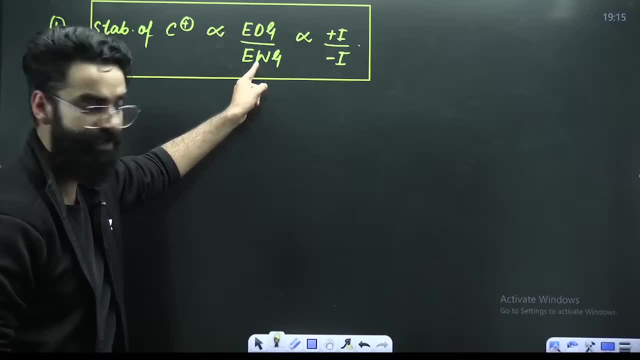 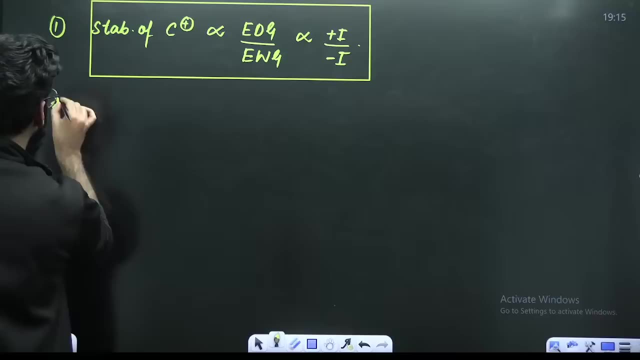 Electron withdrawing group, it destabilizes carbocation. Perfect. So stability of carbocation is directly proportional to plus I and inversely proportional to minus I. Point number one. Point number two: Stability of carbanion. Stability of carbanion. 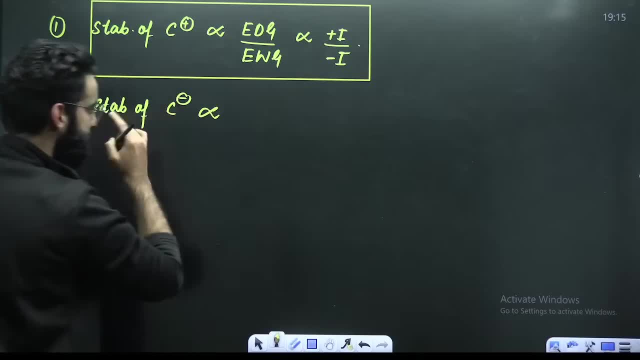 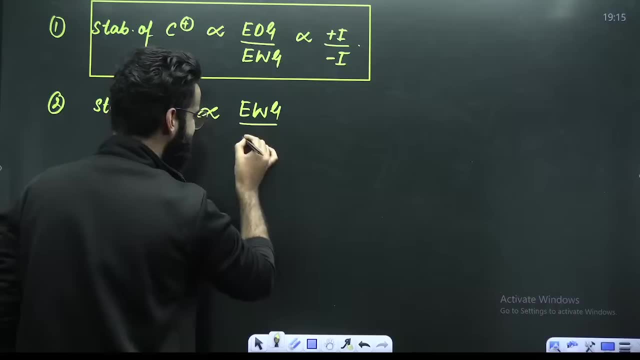 Stability of carbanion. Carbanion is stabilized. Carbanion carbon carrying negative Carbanion is stabilized by electron withdrawing. They are destabilized. They are destabilized by electron donating groups. They are destabilized by electron donating groups. 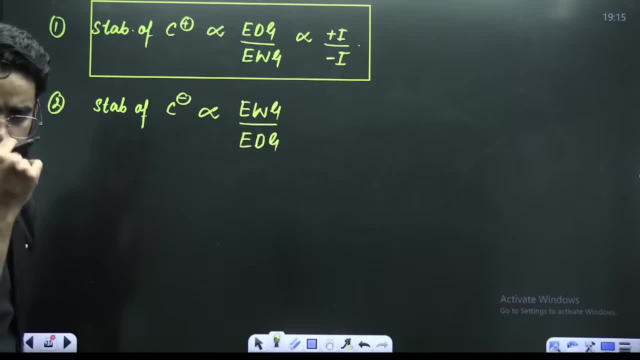 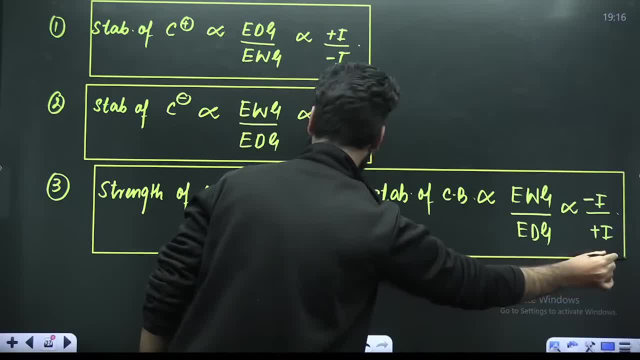 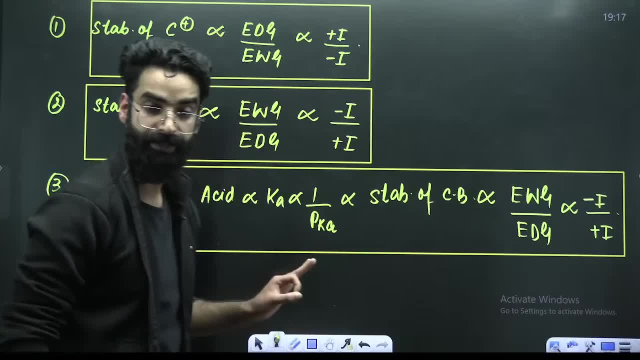 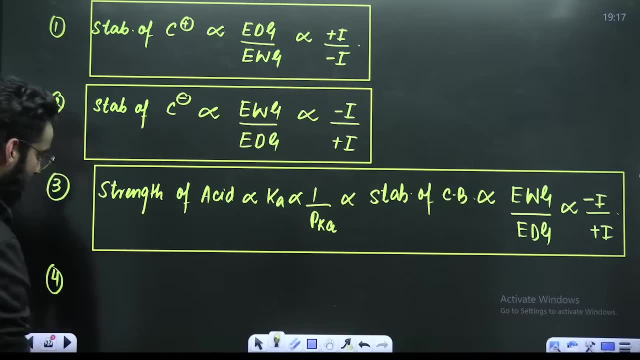 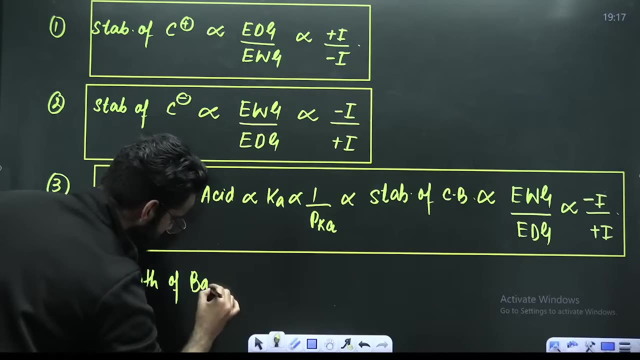 this particular statement. Since I, till now, taught you only inductive effect, we are going to do the questions only based on inductive effect. now, yeah, Now, similarly, the fourth question. the fourth question, that is, strength of a base. strength of a base, strength of a base. 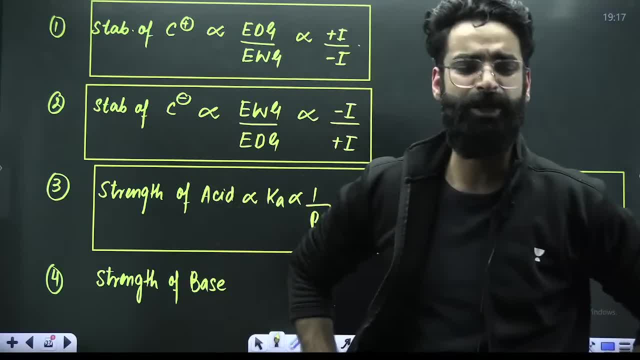 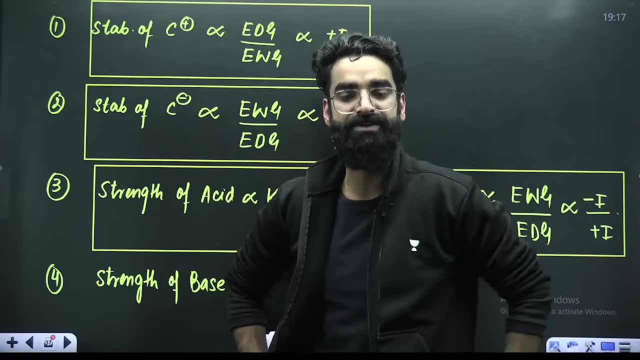 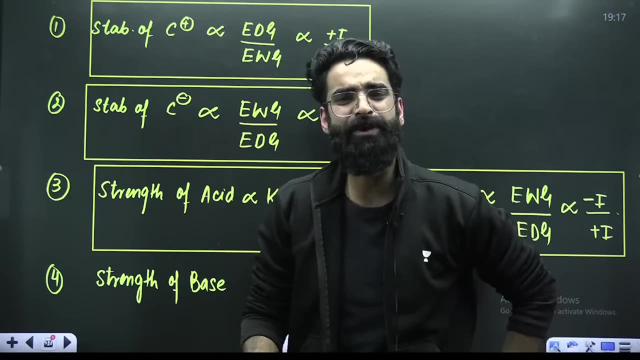 My dear students, if I ask you what a base is as per Lewis concept? as per Lewis concept, how do we define a base? Does the base accept a pair of electron or lose the pair of electron? tell me that. Does a base accept a pair of electron or lose a pair of electron? 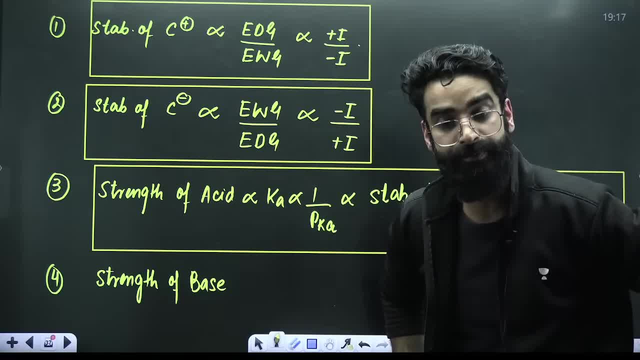 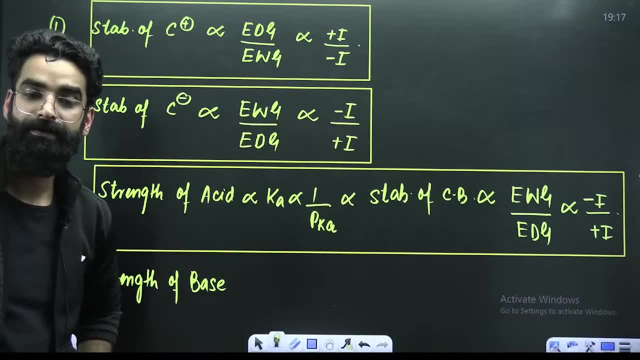 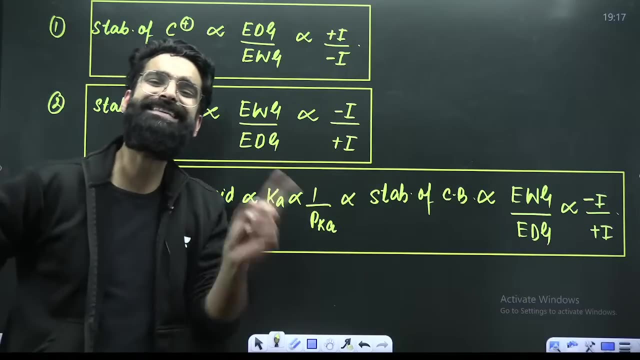 A base loses a pair of electron, donates a pair of electron. a base donates a pair of electron, right, You know that It donates a pair of electron, correct? Does the base accept H positive or donate H positive? tell me that. 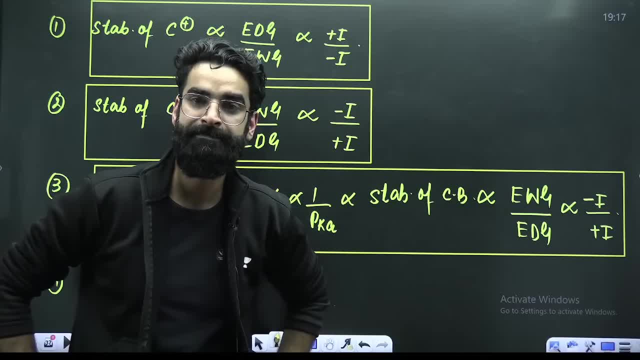 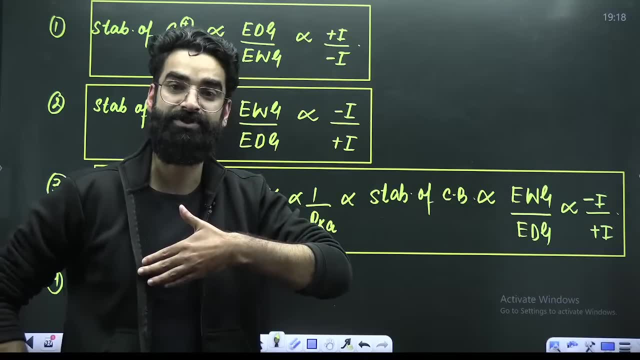 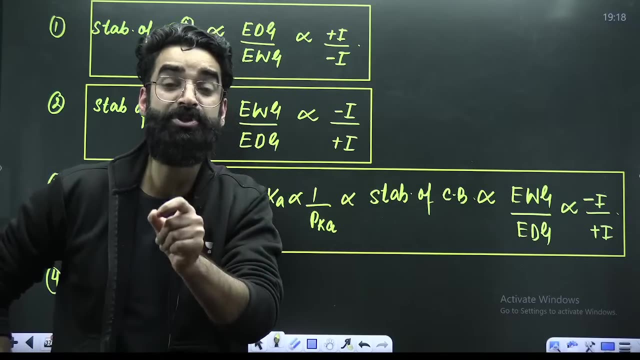 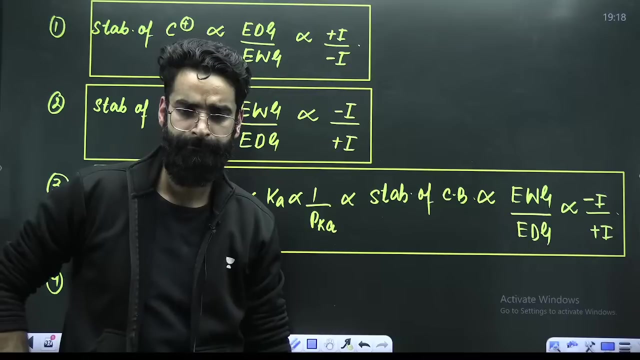 Does a base accept H positive or donate H positive? Does the base accept H positive or donate H positive? It accepts H positive. base accepts H positive. Can I say H positive can attack on the base positive, can easily attack on such a base where the electron density will be more H. 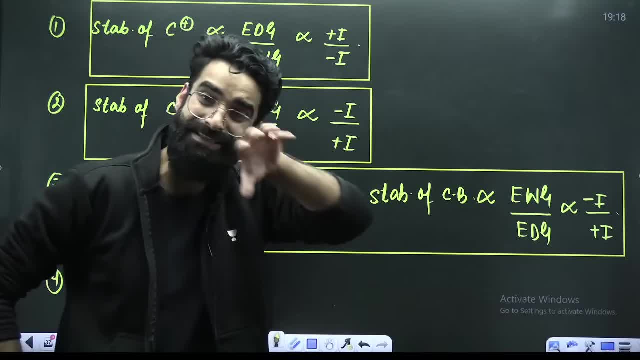 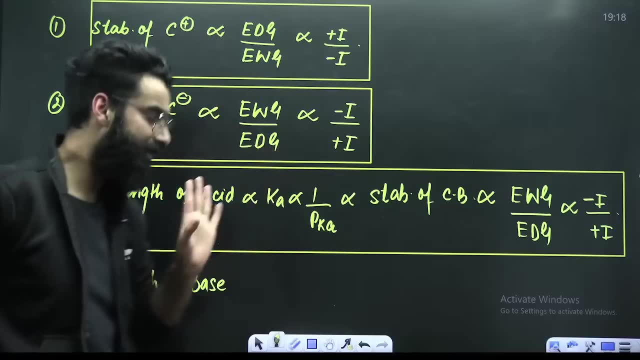 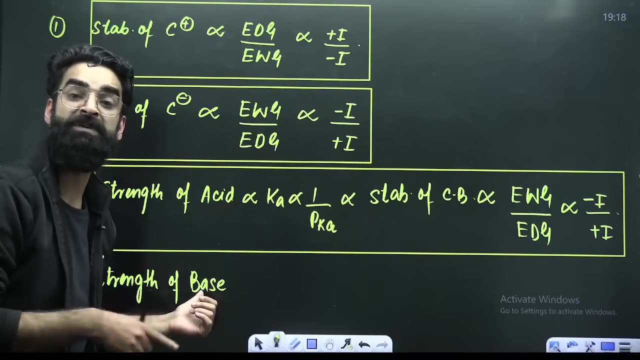 positive will accept will. H positive will attack easily on such a base wherein the electron density at some site will be more Agreed, Right. So tell me, string for base, base: for the H positive to attack easily, electron density has to be more or less, it has to. 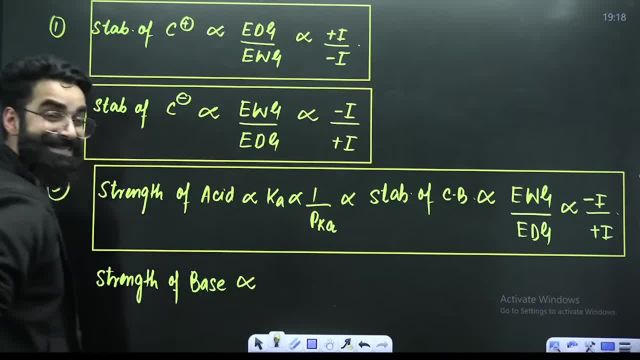 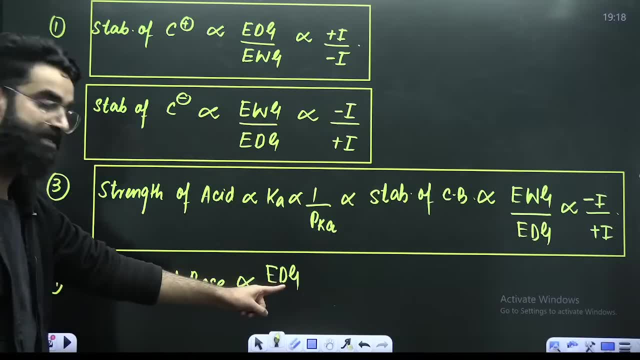 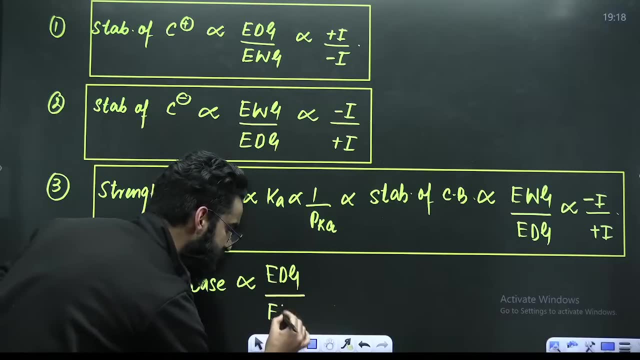 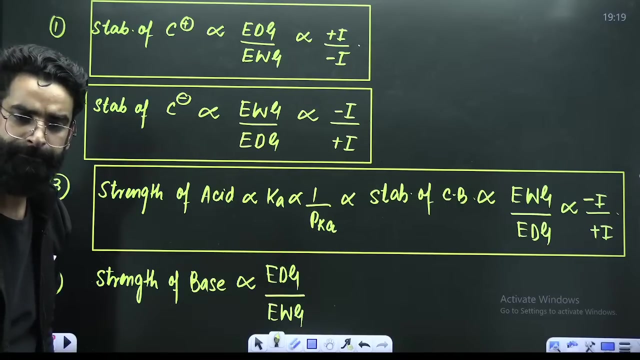 be more, How electron density is going to be more. Can I say electron donating groups? Electron donating groups. electron donating groups if attached to a base will increase the strength of the base, and electron withdrawing groups. electron withdrawing groups if attached with a base are going to decrease the strength of the base Right Now. electron donating. 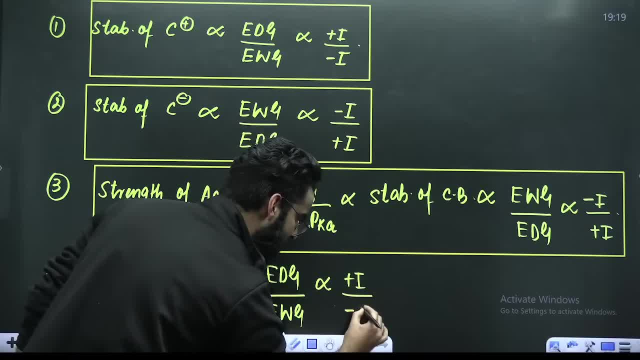 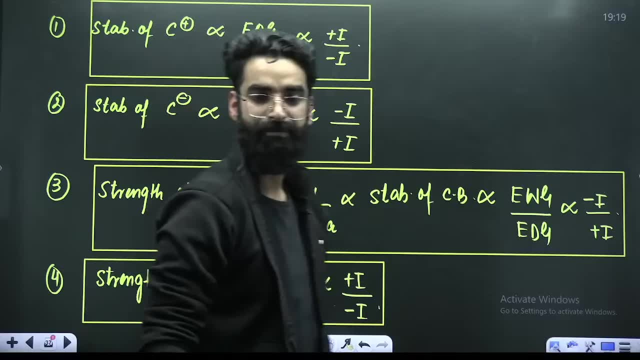 means over here. in terms of inductive effect, It's plus I, electron withdrawing. in terms of inductive effect, it's minus I. So can you solve all these questions? Can you solve all these questions by considering only inductive effect? Till now we have studied only inductive effect. Now anything can be asked from this. 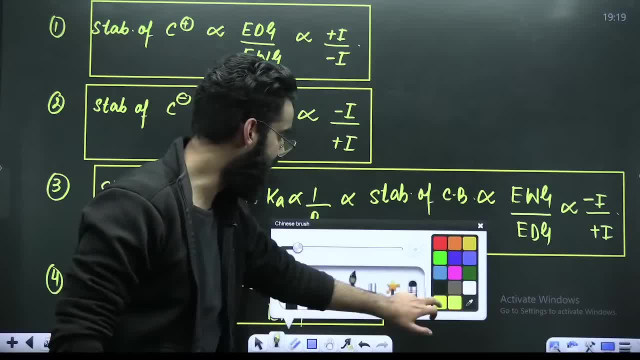 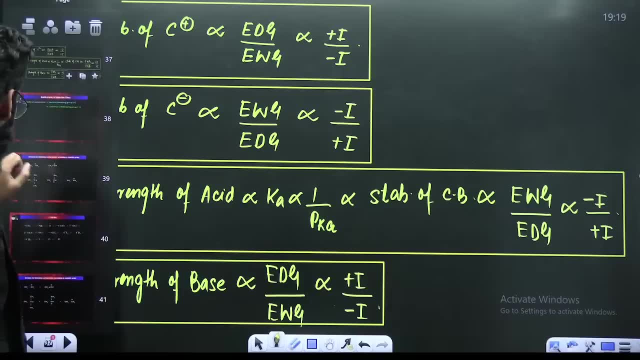 particular slide: Anything. anything means anything. Anything means anything. Now, now, now, let's try to solve certain questions so that it will be absolutely clear to every one of you, Absolutely clear to every one of you. Okay, Just a second people. 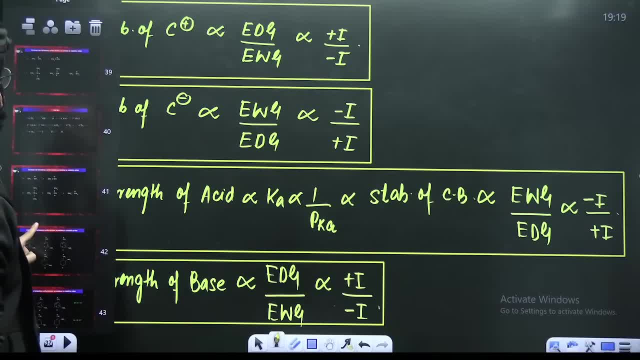 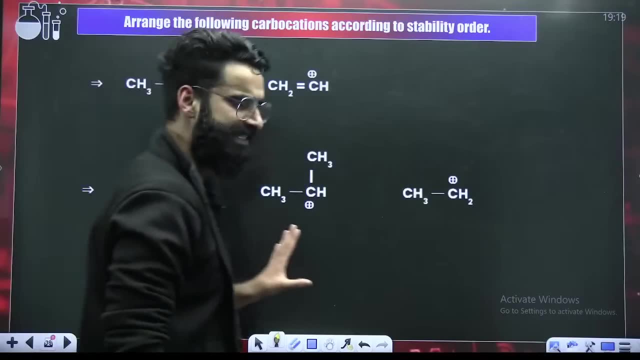 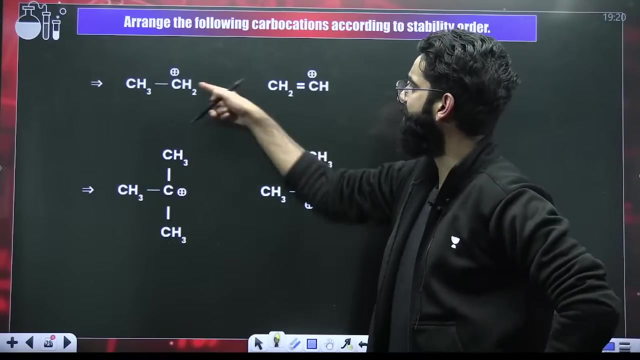 Just a second. Just a second. The first ten basic question You are going to answer me in the chats. Now I want the charts to move fast. Among these two, among these carbocations, which one is more stable? Among these two, which one is more stable? Which one is more stable? 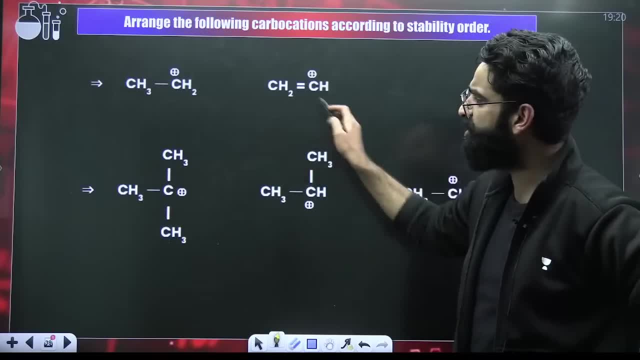 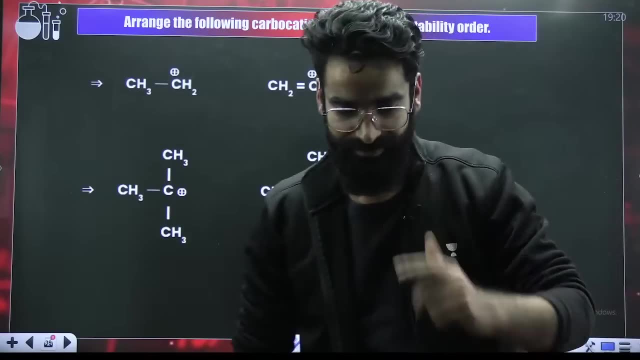 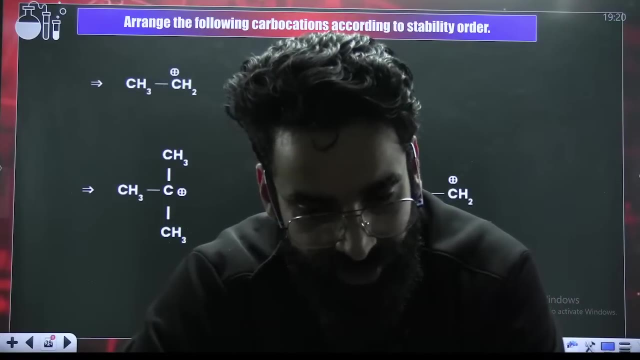 No more stable. What do you suggest? So rehabна table quickly. who is this model, bro? please stop spamming. please stop spamming. let people study. you are writing east or west. alak sir is the best. of course he is the best. we appreciate him right. 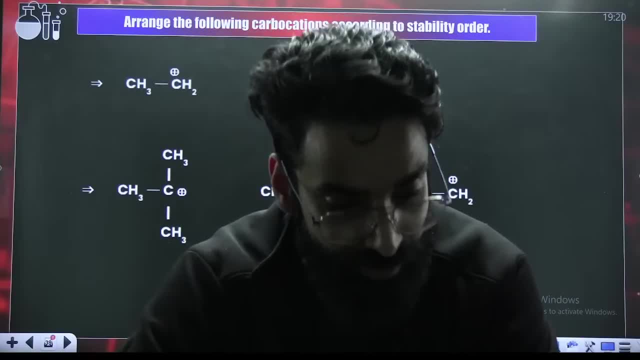 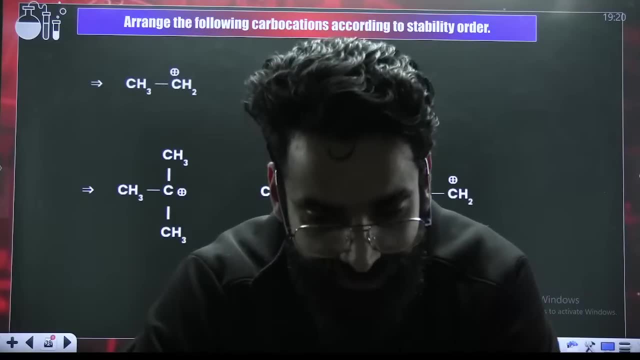 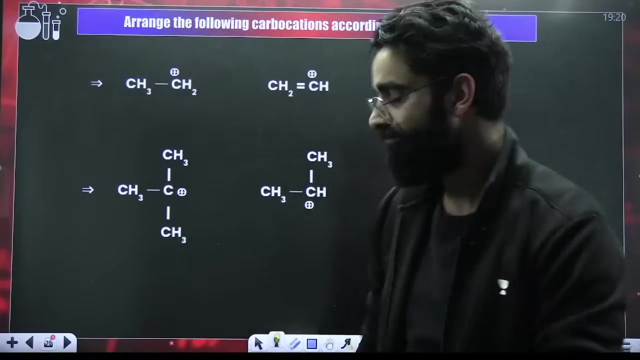 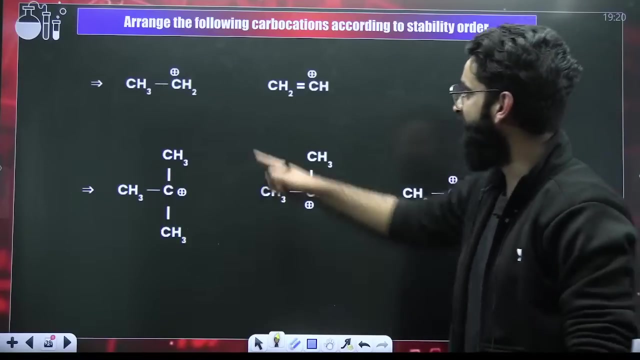 we love him. every teacher in the country loves him because of the contribution which he has made. right, but don't write all these things. let people study right. let people study okay, okay, right. look at this one now. look at this one. tell me, among these two, which is which is more stable? 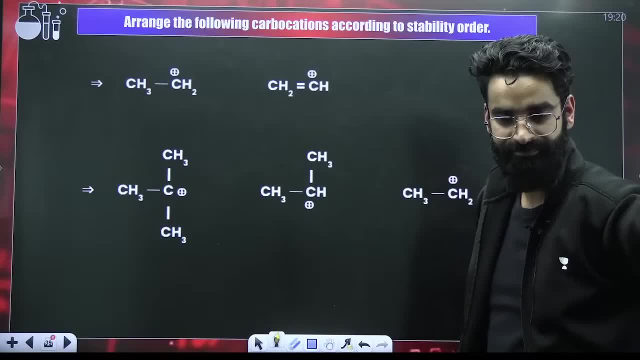 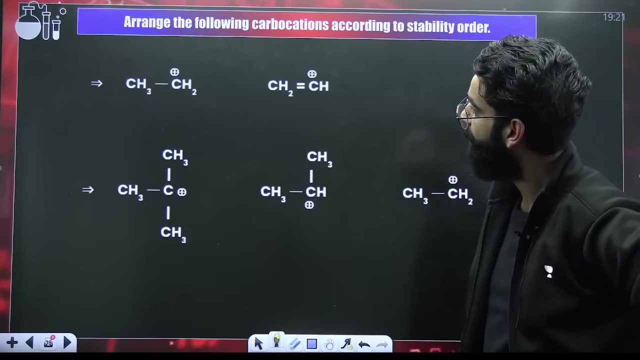 quickly, guys. you are not supposed to take this much of time. you are not supposed to take this much of time. you are not supposed to take this much of time quickly. one or two, one or two, one or two, quickly, asha, wait, wait, wait. i'll do this at the end. i'll do this at the end. 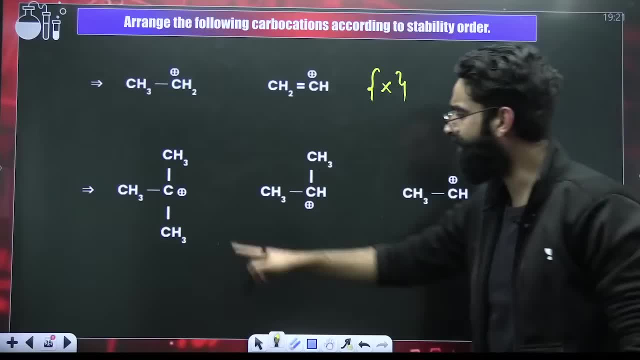 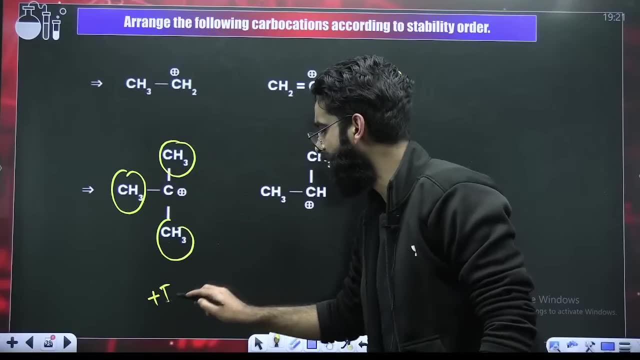 tell me among these three? tell me among these three. carbocation is stabilized by plus side. see, this is plus i showing plus i showing plus i showing. so three plus equation. since i've only taught you inductive effect yet, so i'm going to answer the questions only on the basis of inductive effect. 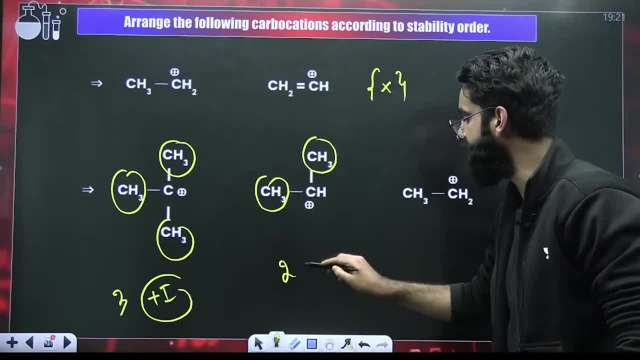 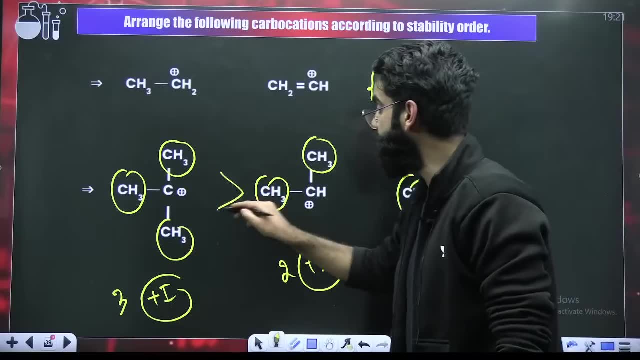 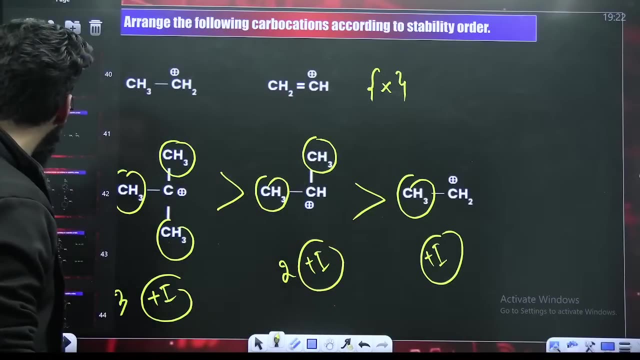 so three plus action groups, how many? two plus actually groups, how many? only one plus i showing group right. so more plus i showing groups, more the stability, one, two, three done. question number one. question number one: Look at this one, Look at this one. All these are carbocations, right? 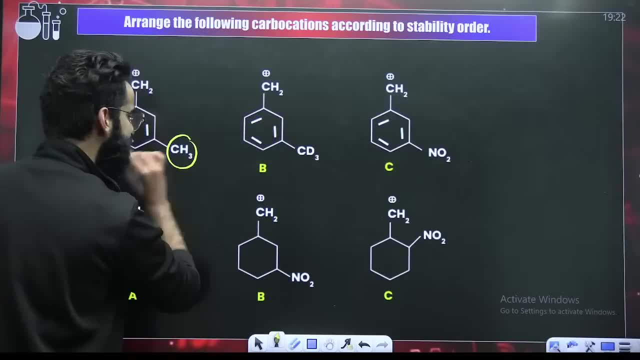 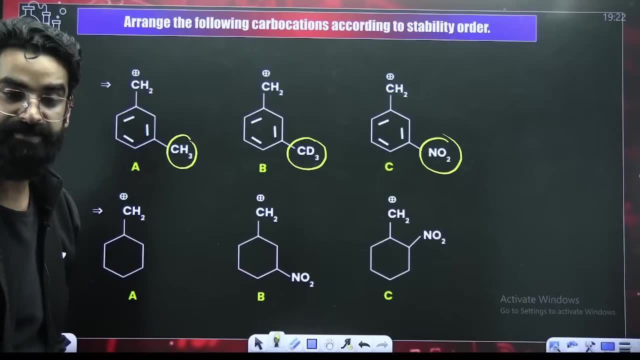 Carbon carrying positive carbon positive, carbon positive. Here you have got CH3 attached, CD3 attached, NO2 attached. Carbocations are stabilized with plus I. Carbocations are stabilized with electron donating groups. Now CH3. CH3 shows plus I, of course, right. 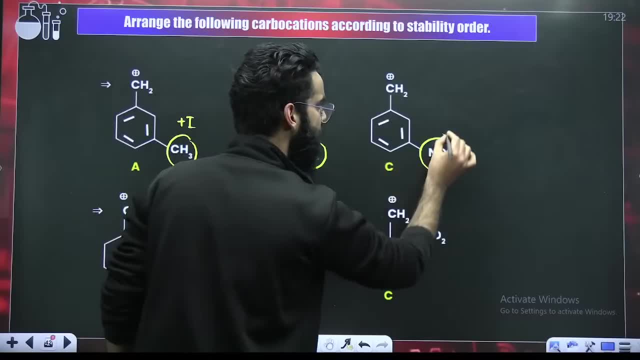 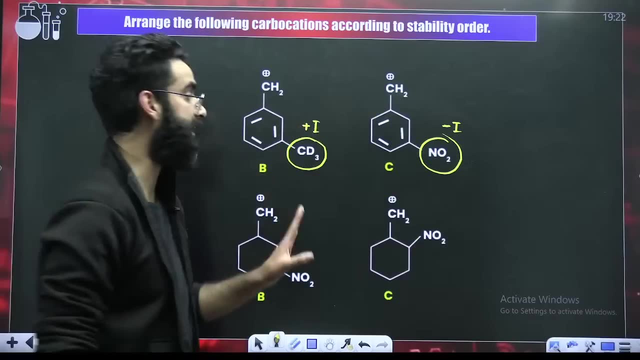 CD3.. It also shows plus I right NO2.. It shows minus I right, So minus I showing group. It destabilizes the carbocation. So stability of the C at the end, right Now among 1 and 2.. 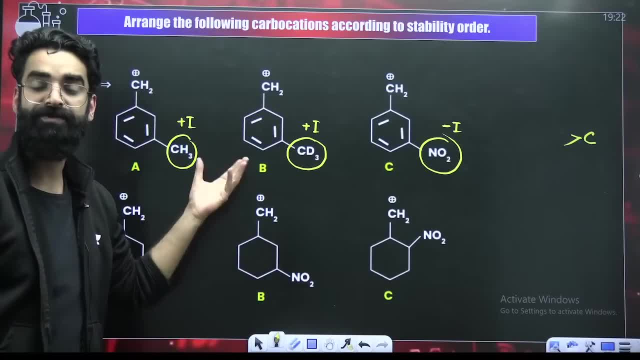 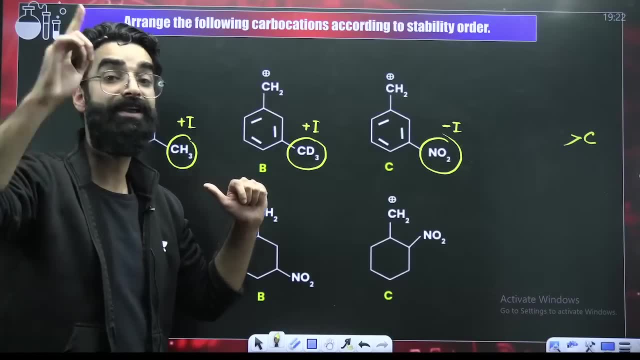 Which one does show more plus I? Which one shows more plus I? Is it CH3 or CD3?? I hope you remember 3TM shows more. If you remember in that part, 3TM more, followed by D, followed by H. 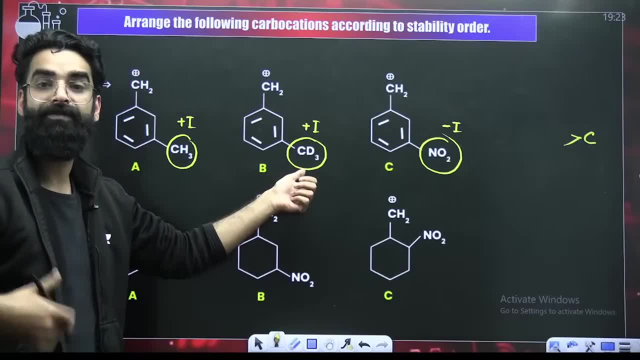 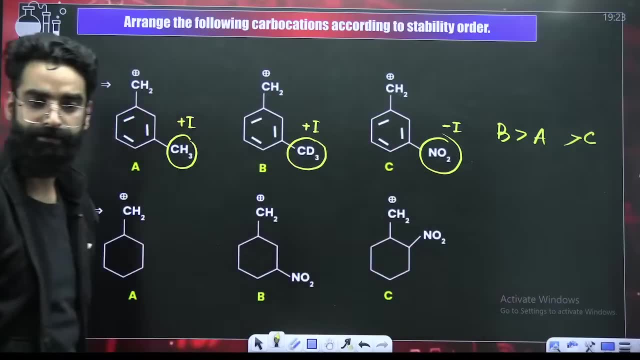 Similarly CD3.. CD3 will show more plus I than that of CH3, right, Right, More plus I means more stability. So BAC is the order Simple. Look at the next one. Look at the next one. 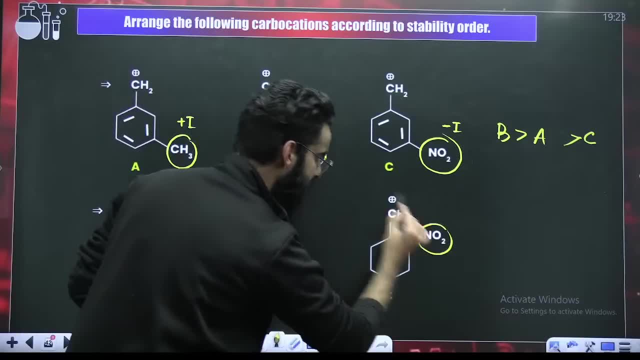 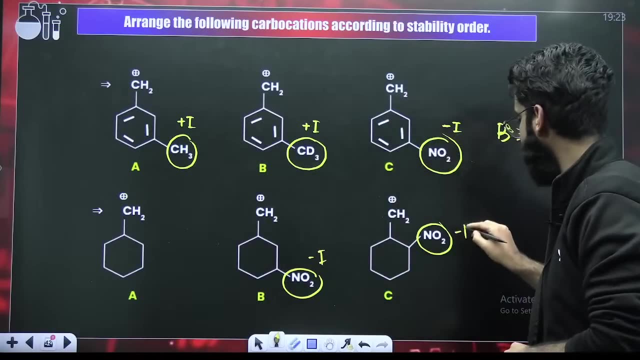 No group. Over here you have got NO2 attached. Over here you have got NO2 attached, NO2.. Is it withdrawing or donating? It's withdrawing right, It's withdrawing. It shows minus I Inductive effect. 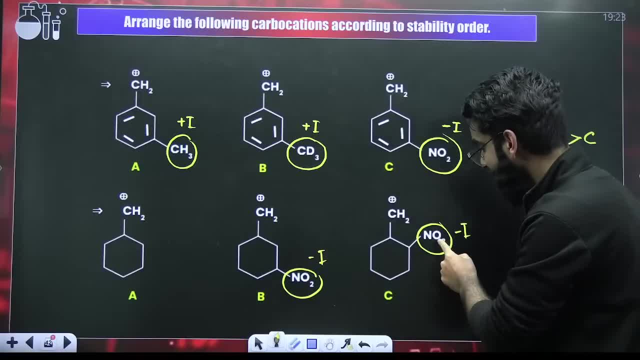 Is it distance dependent? Yes, it's distance dependent. So can I say NO2 will be more withdrawing in the third case, NO2.. NO2 will be more withdrawing in the third case and if in the third case NO2 is more withdrawing, 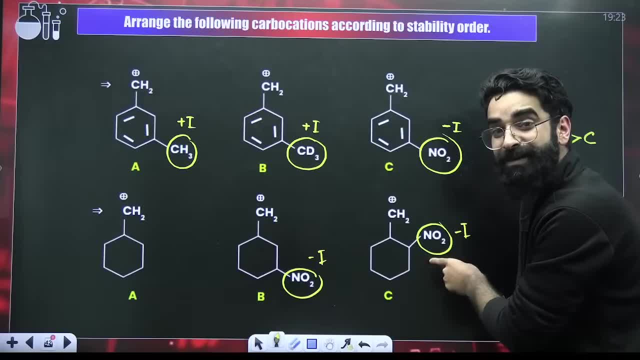 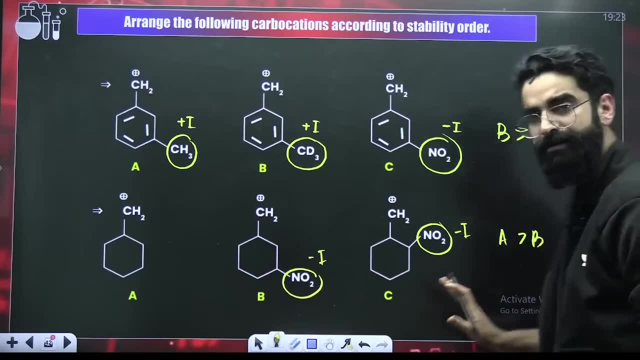 it will destabilize this particular specie to the maximum. So the stability of C is the least right. A will be maximum, followed by B. Simple ABC is the order. ABC is the order. ABC is the order. Nothing to do. 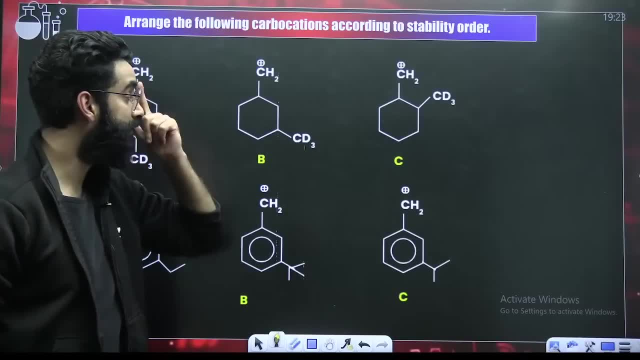 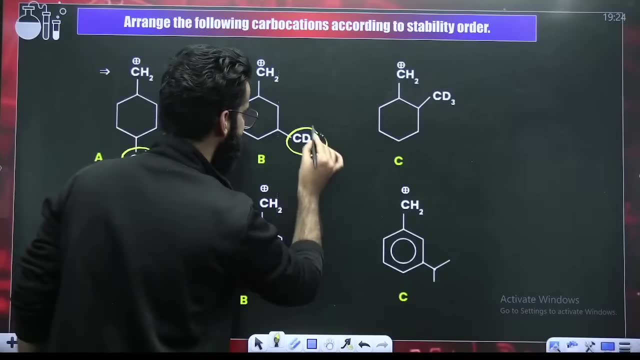 Tell me about the answer of this particular equation: A, B or C. Again, these are carbocatines. Again these are carbocatines, CD3.. Right Electron donating. plus I, CD3.. Plus I, CD3. 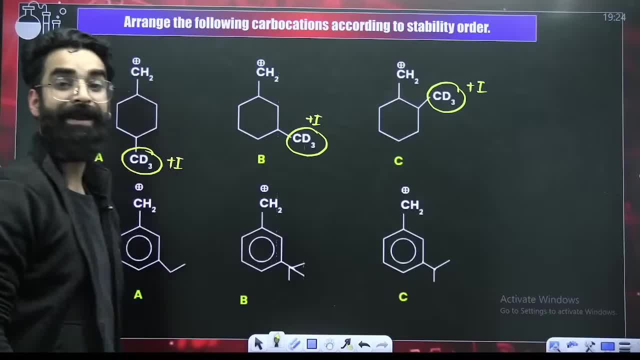 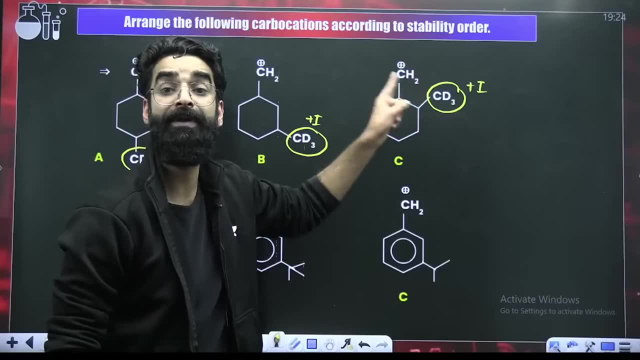 Plus I Right Now. inductive effect is distance dependent. Where is the distance less? Here the distance is less. So more promenading, plus I nature. More promenading, plus I nature, Right. So what has to be the stability order? 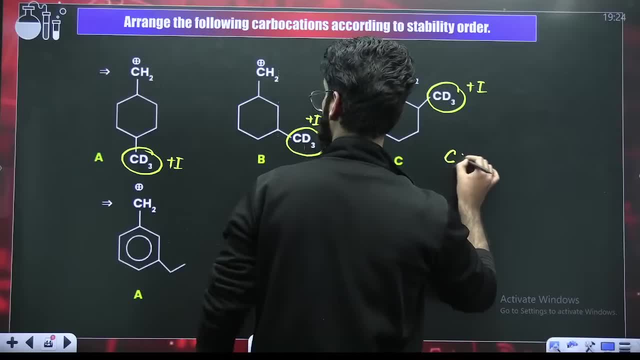 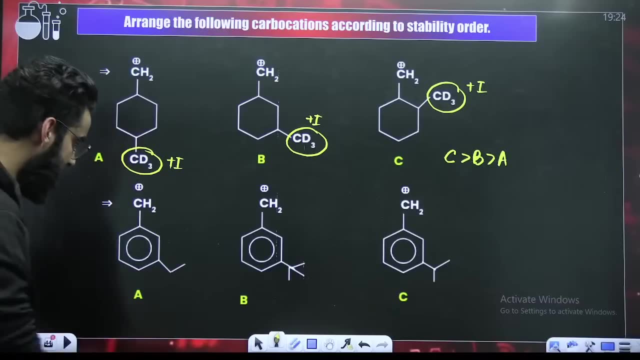 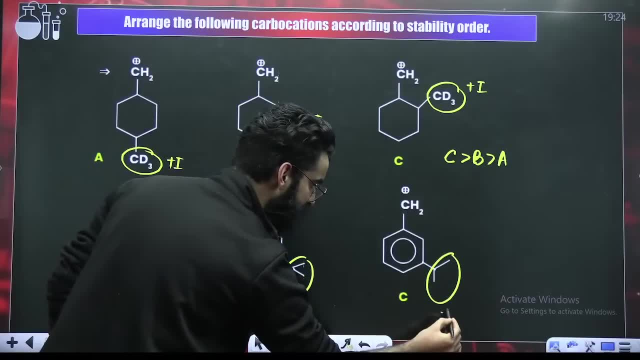 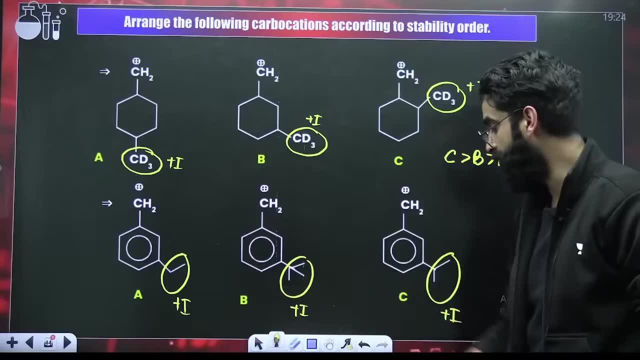 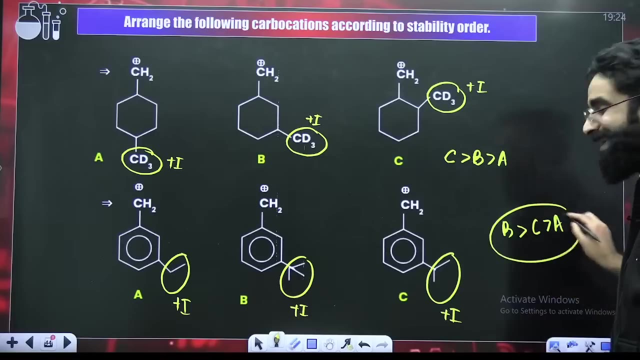 your alkyl group plus i. this again: your alkyl group plus i. right now, which alkyl group shows more plus i? where the branching is more? where is the branching more b, b? so this will be maximum stable carbocation, followed by what, followed by c, followed by a, b, c, a is the order. 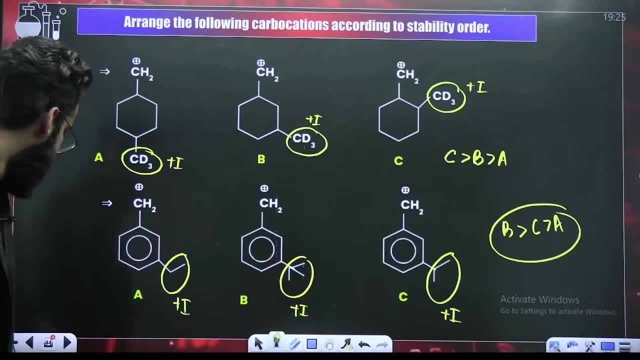 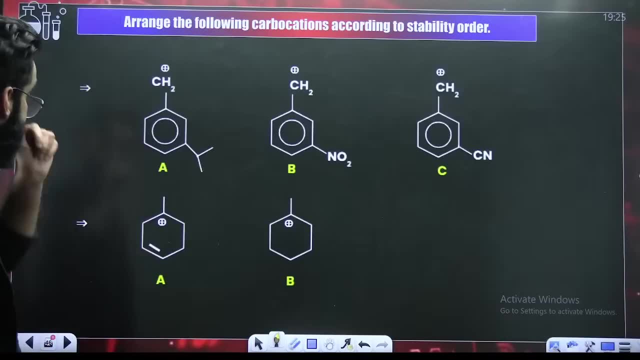 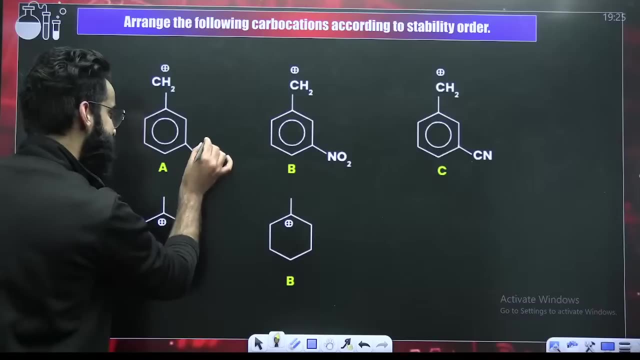 yes, clear guys. the chat should run continuously. the chat should run continuously. you are supposed to answer all the equations, all the equations. look at this one: a, b or c, which one is more stable? all these are carbocations. carbocations are stabilized by plus i. this is alkyl showing. 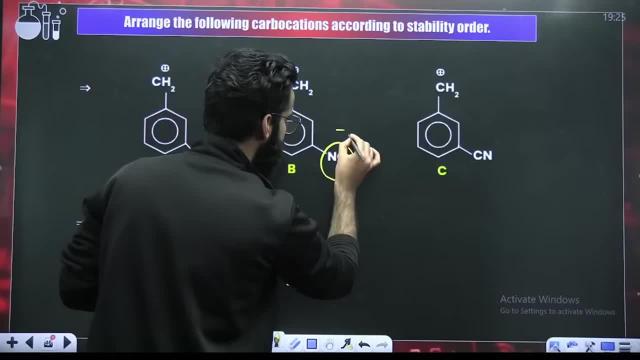 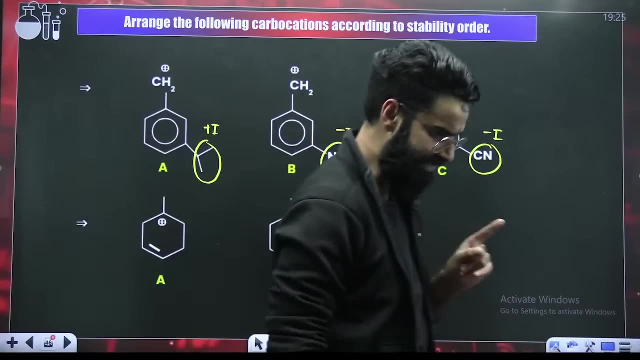 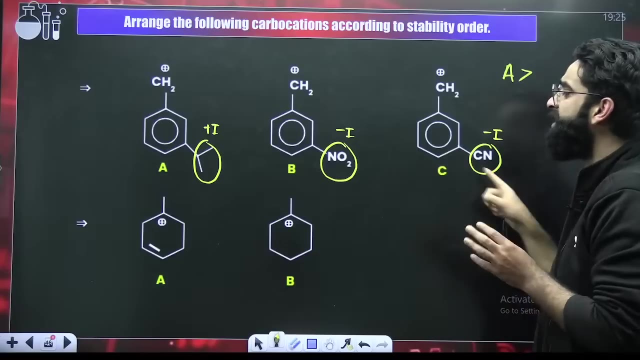 plus i right no2. showing minus i right cn showing minus i plus i groups: they stabilize the carbocation. plus i groups they stabilize the carbocations. so a will be maximum stable. right now, among b and c, which one is less electron withdrawing? cn is comparatively less electron withdrawing than no2, so c will be more stable followed. 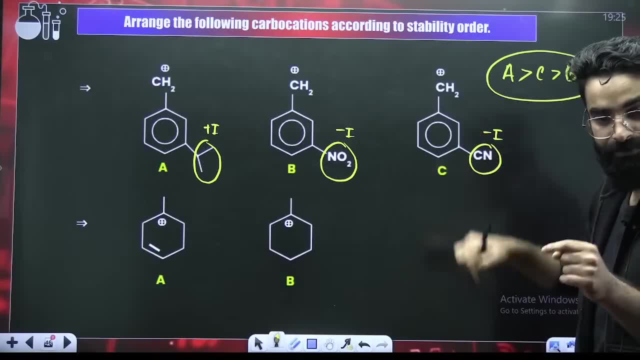 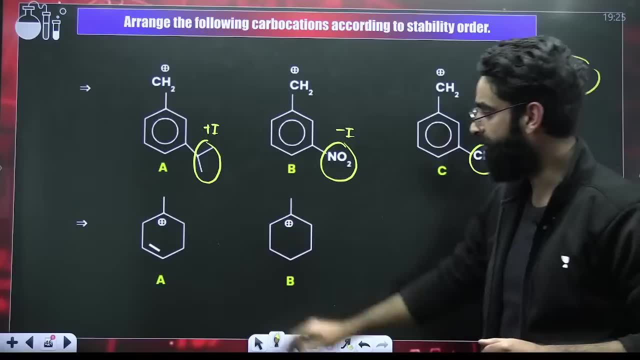 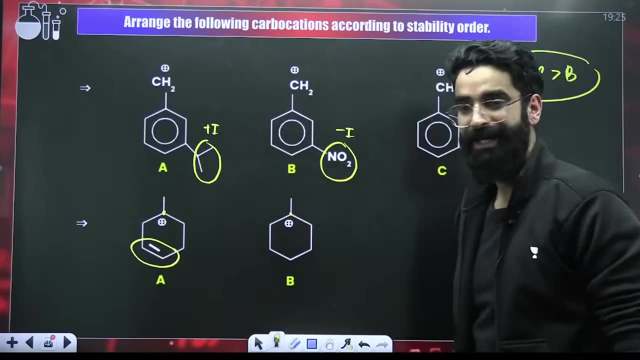 by b. if you remember the series, series, i gave you right. no2 is more shows, more minus i than that of cn. now, look at this one. look at this one: positive charge is here and positive charge is here. right, look at this double bond. this is sp2. sp, this is sp2. 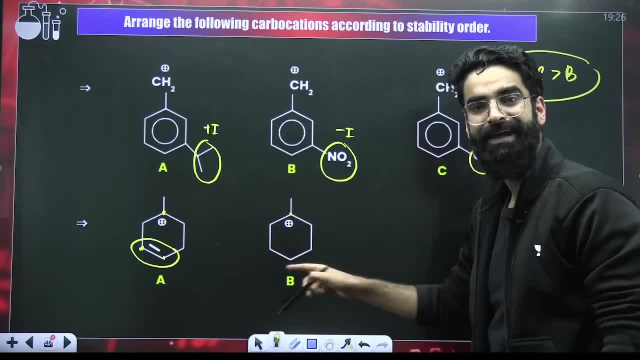 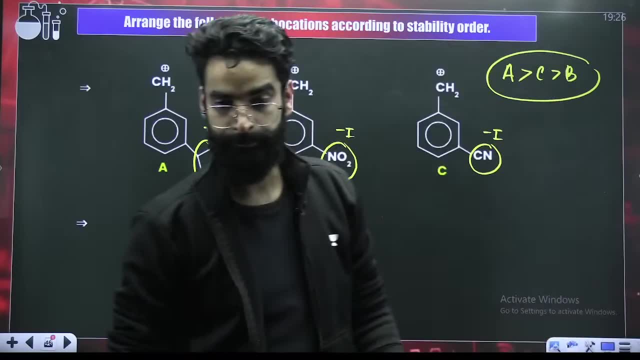 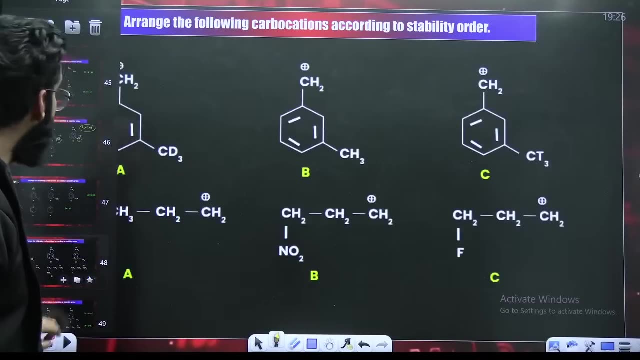 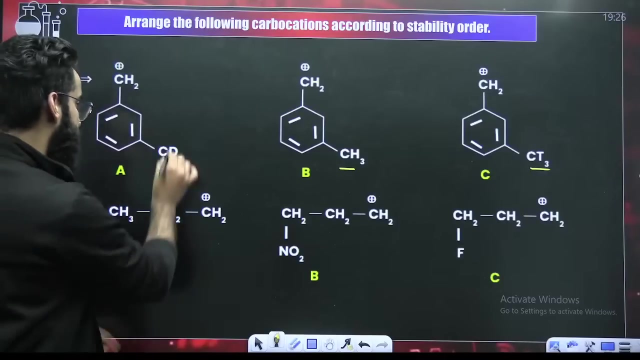 right, this is also sp2, but here all are sp3. sp2 means more withdrawing. withdrawing: they destabilize the carbocation right. so stability of b is more than that of a. yes, right, going ahead, going ahead. look at this one: cd3, ch3, ct3, plus i showing even this is plus i showing even. 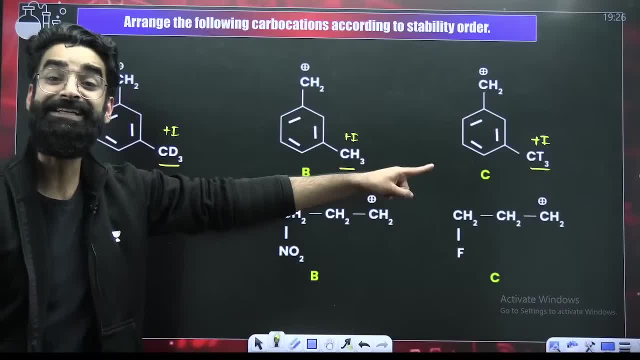 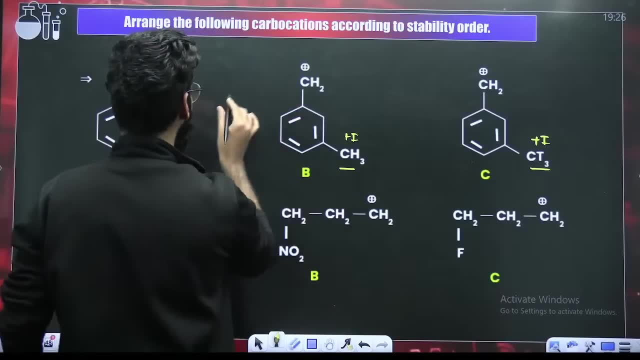 this is plus i showing. now which one is more plus i showing. even this is plus i showing. even this is also plus i showing. even this is plus i showing. even t3 is more plus i showing, then cd3, then ch3 and plus i showing groups. they stabilize the carbocation time, so stability. 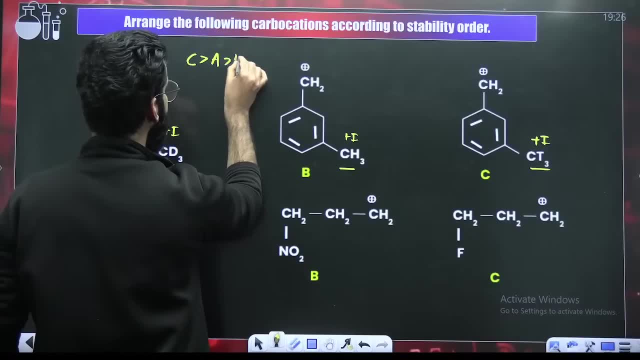 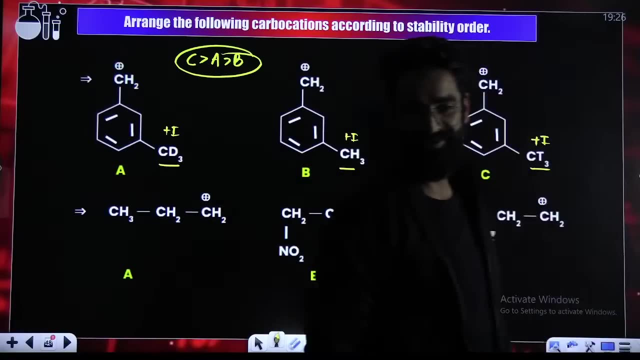 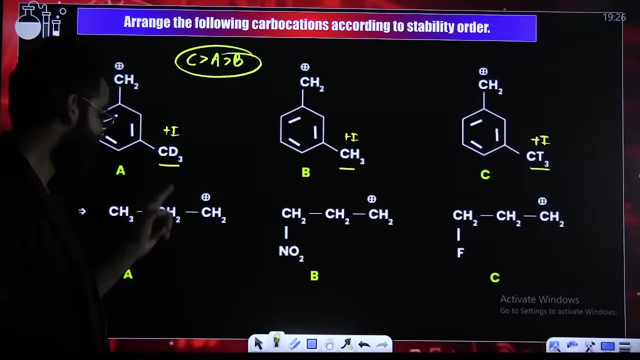 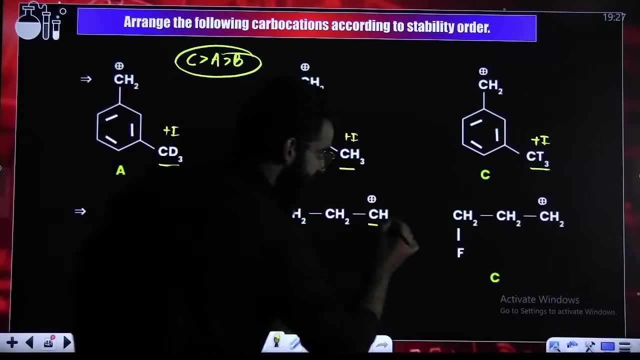 of c will be maximum, followed by what, followed by a, followed by b, is the stability order. oh yes, welcome to the night mode. welcome to the night mode. welcome to the night mode. okay, look at the next one, look at the next one. at the next one: carbon carrying positive. here carbon is carrying positive. carbon carrying. 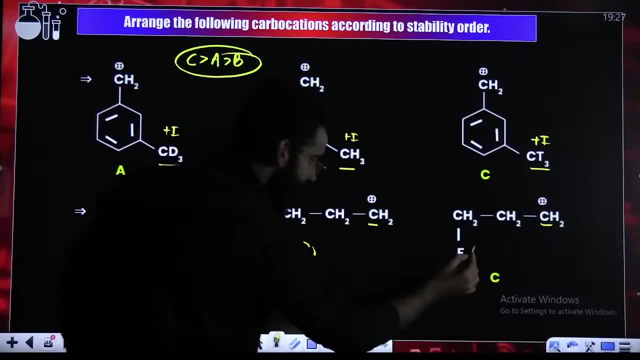 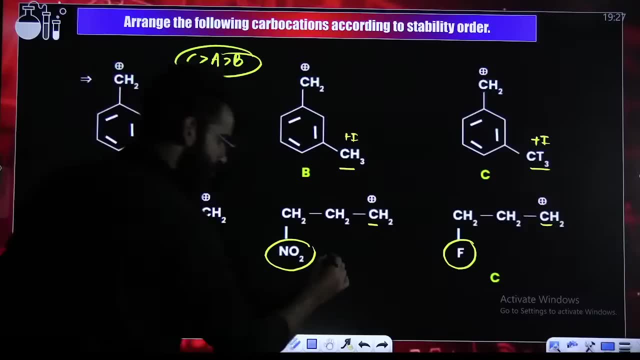 positive right over here. nitro group is attached here. fluorine is attached here. no such group, no withdrawing group is attached as such. right, perfect. so this shows minus i, this shows minus i and minus i groups. they destabilize the carbocation. here you do not have any electron. 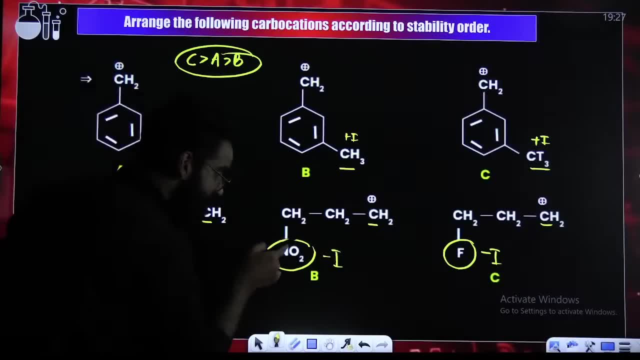 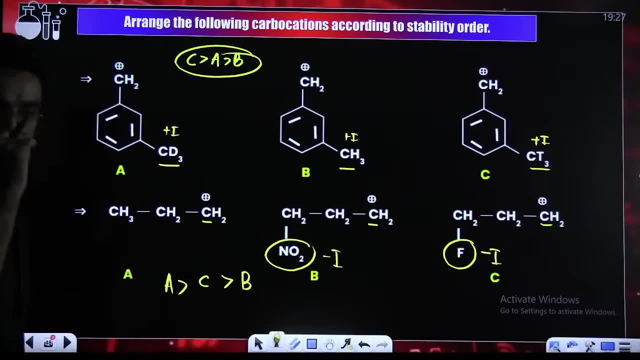 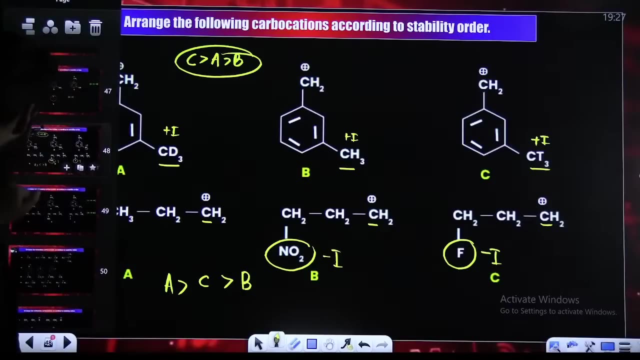 withdrawing group. so stability of a is maximum. now this is more withdrawing. if this is more withdrawing it will destabilize the carbocation into the maximum. so b at the end here is going to be c. so acb is order. acb is order. yes, acb is the order. look at the next one. look at the next. 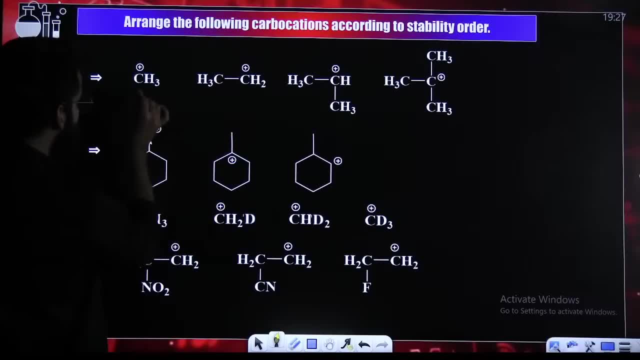 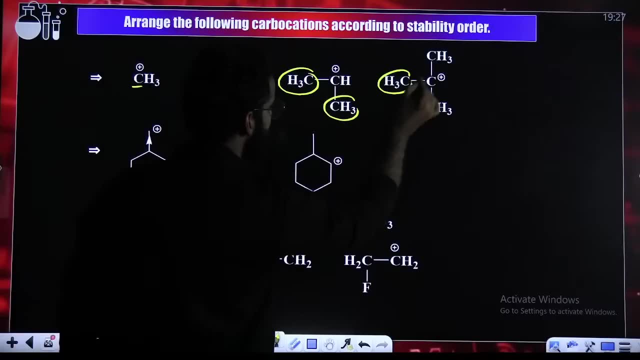 one. look at the next one. i think this is the question which we already solved: p carrying positive here. positive also: one plus i showing group here over here. two plus i showing groups here. you have got three plus i showing groups, right. so stability order will be like this: 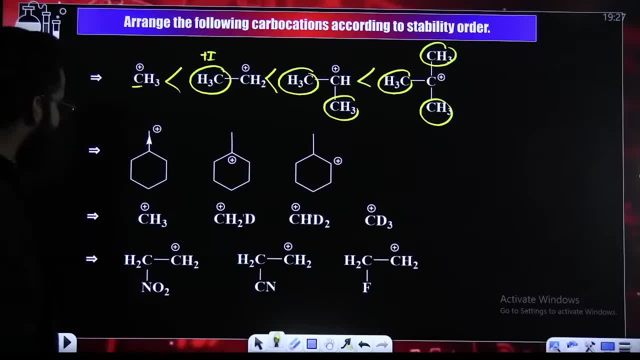 because, plus i showing groups, they stay destabilize the carbocation right now, since, since i did not teach you hyper conjugation or anything yet, i am solving the equation directly on the base of inductive effect. now this particular carbon, carrying positive, it's getting electrons from one side, this particular 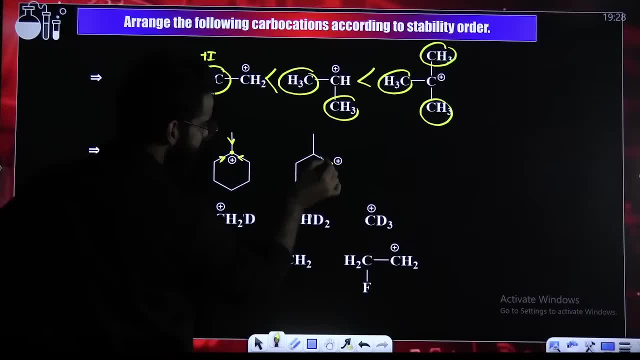 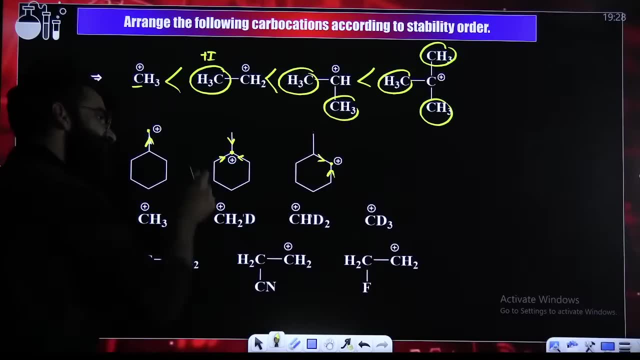 carbon carrying positive. it's getting electrons from three side. this particular, it's getting electrons from two sides. right, perfect, right. so where will be the positive charge compensated, the maximum positive charges compensated, the maximum here, right. if the positive charge intensity is decreased, here the maximum, the maximum decrease in the intensity of positive charges here, right, so it. 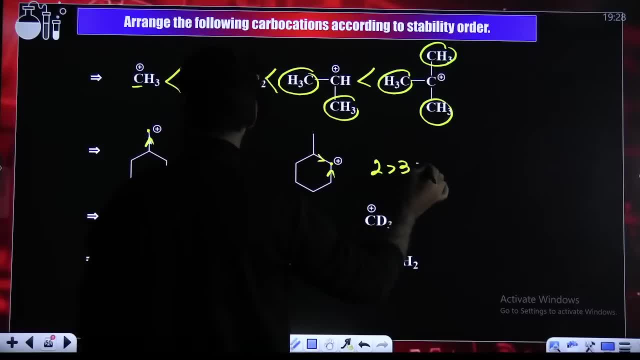 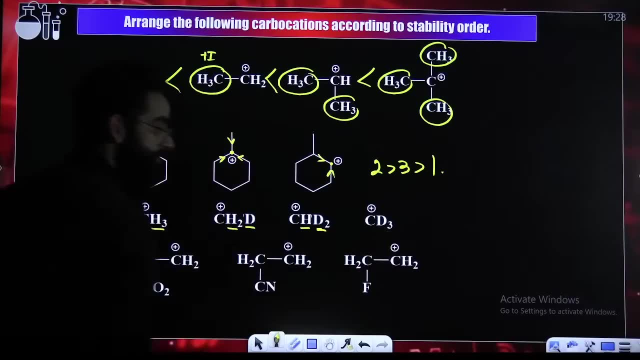 will be more stable. so two will be more stable than that of three and at the end it's going to be one. now, ch3, ch2d, deuterium, chd2, cd3, positive right, more the d's, more the d's more is the. 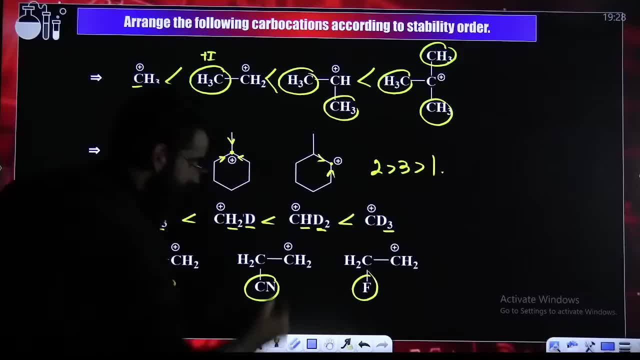 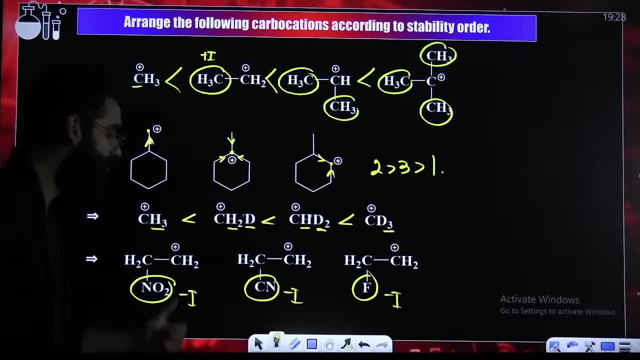 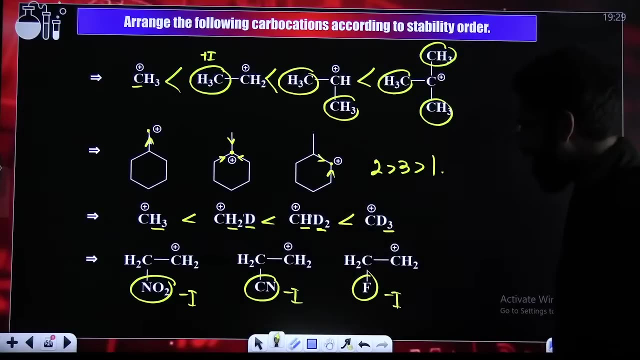 stability right. nitro, cnf, nitro, cnf, all are all are electron withdrawing. so minus i, minus i, minus i. the one which shows a lesser minus among the three, the one which shows lesser minus i among the three, which one shows lesser minus i. so third shows lesser minus i, so its stability will be more. 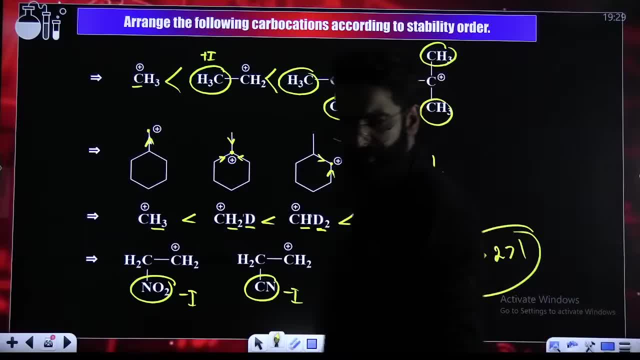 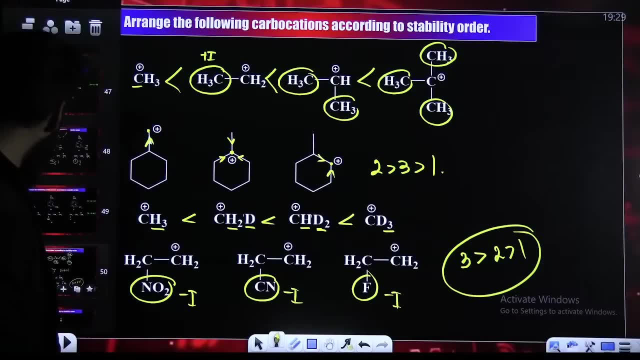 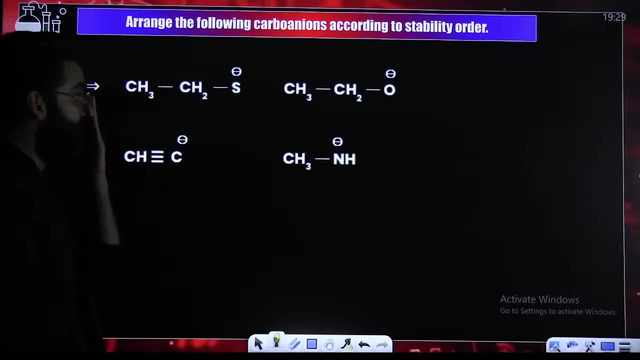 followed by two, followed by one. right perfect, i believe you are. you are able to solve these questions easily now. now, now, one more, one more. among these two species, which one is more stable? can you let me know, among these two species, which one is more stable? carefully look: sulfur, carrying negative oxygen, carrying negative rest, everything. 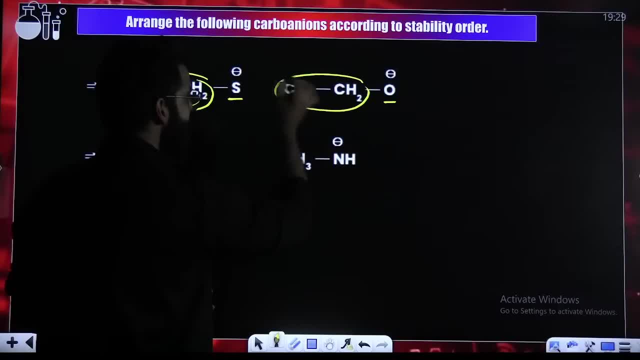 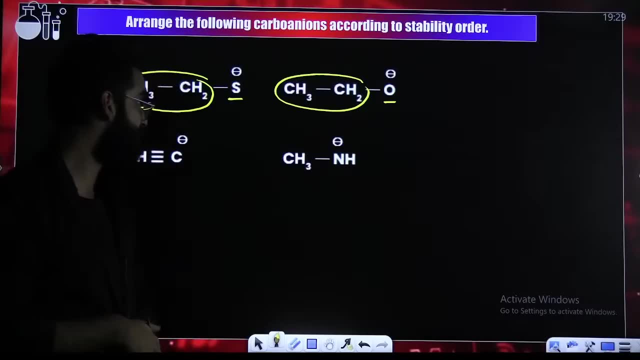 is same. this part is same. even this part is same. sulfur carrying negative, oxygen carrying negative. you tell me the answer: sulfur and oxygen, they belong to same group. same group means vcd volume charge density: right volume charge density. sulfur more size. you tell me the answer: sulfur and oxygen, they belong to same group. same group means vcd volume. 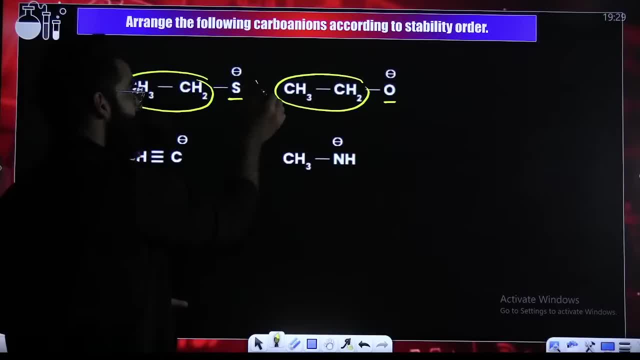 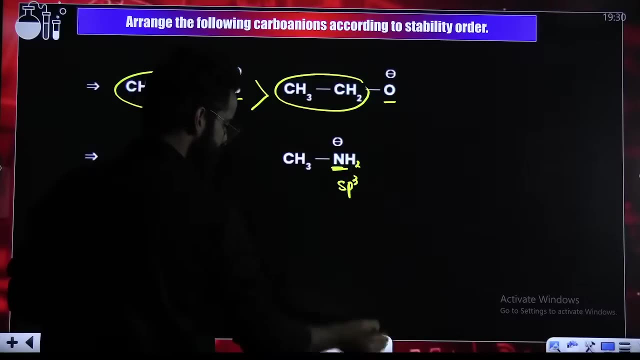 less vcd. less vcd means more stability, so this is the stability order, right? perfect, this question, we've already solved. this is your sp hybridized carbon carrying negative. this is your. this is your sp3 hybridized nitrogen. right, this is your sp3 hybridized nitrogen. perfect, now you tell me which. 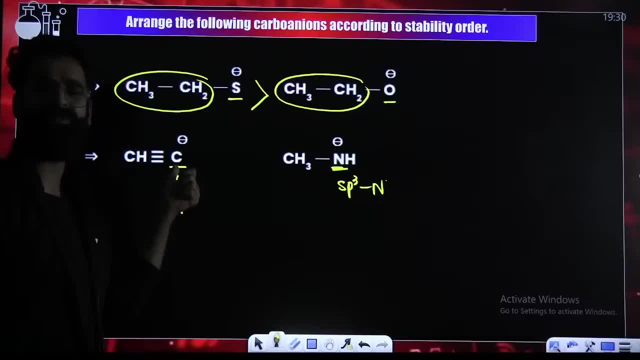 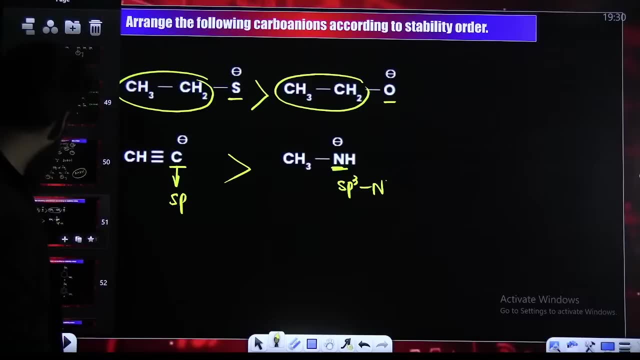 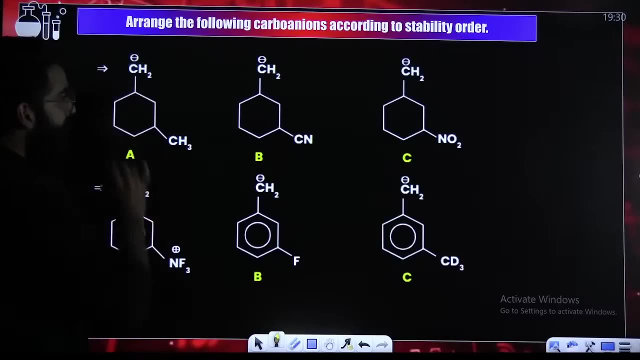 one is more electronegative? which one is more electronegative? sp. hybridized carbon is more electronegative. negative charge on an electronegative element is considered to be stable. so this is the stability order. done, perfect, perfect. tell me the order of these questions. i think yeah, okay, now these are not. 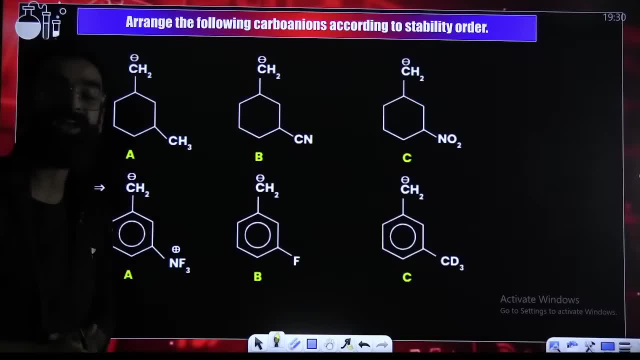 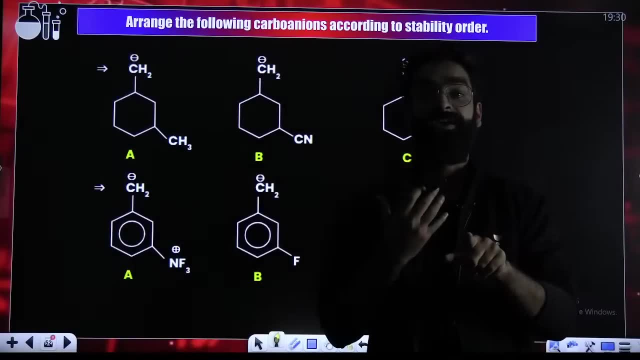 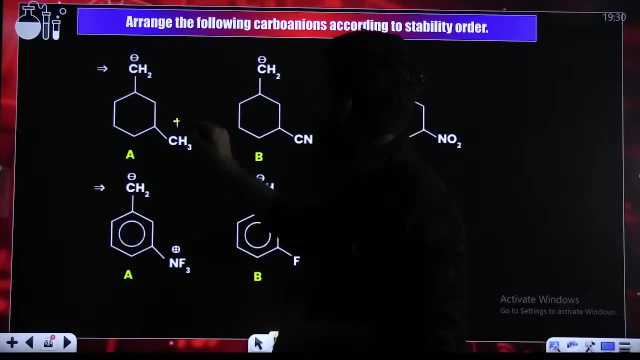 your carbocatines. these are not your carbocatine, these are your carbanians. carbon carrying negative carbon carrying negative carbon carrying negative carbanians are stabilized by electron withdrawing minus isoing carbanians are stabilized by minus isoing groups. yeah, now th3 it's plus i cn, minus i. 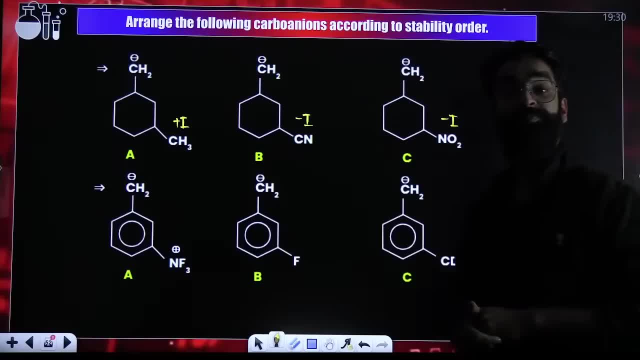 and o2, minus i, minus i showing groups. they stabilize the carbanian. now which one shows more? minus i nitro. nitro shows more mindset. so c, then b, then a. this is the order, right, guys? keep on telling me the answers in the chats. i'm looking at your chats. look at the next one. 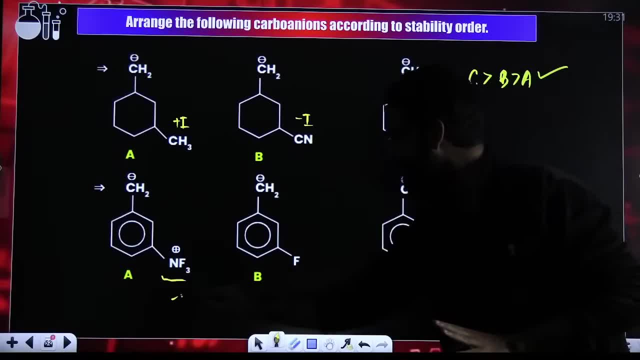 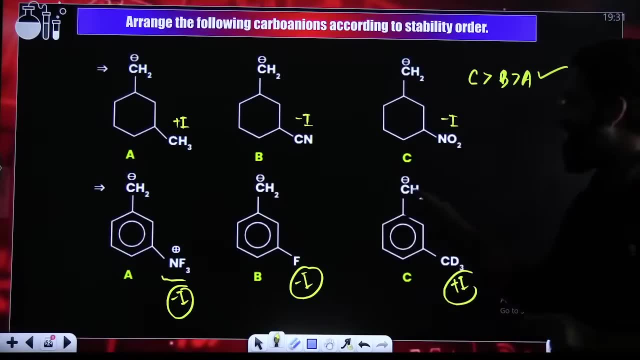 look at the next one. all these are carbines. this shows minus i. right, even this fluorine shows minus i. perfect. pd3, it shows plus i. and since these are carbanians, carbanians are stabilized by electron withdrawing. so there is electron withdrawing, this electron withdrawing. now, which one is more? 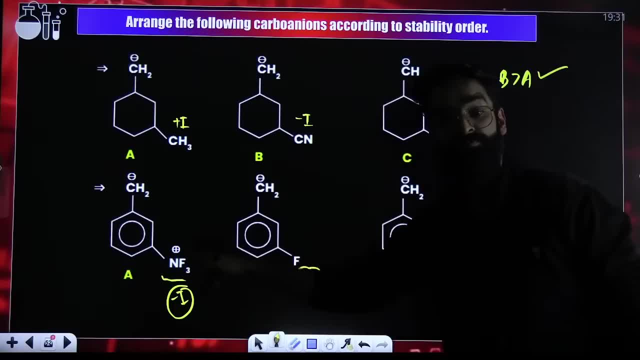 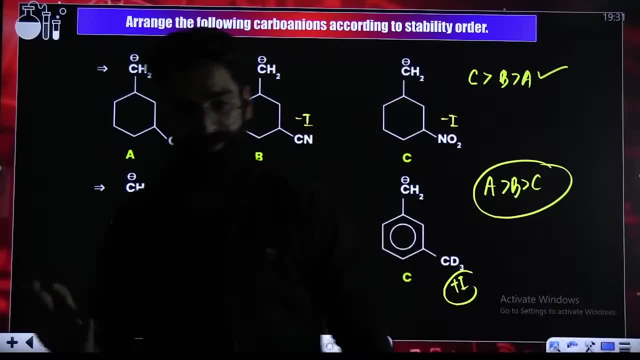 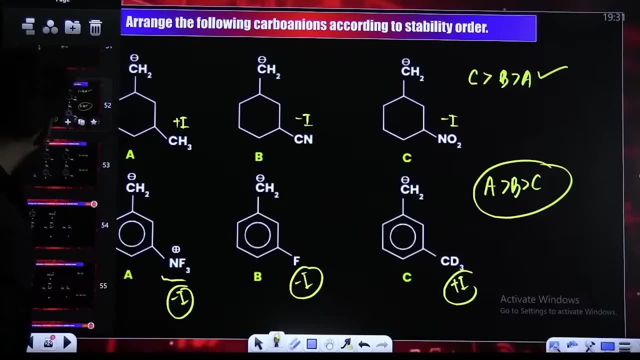 electron withdrawing and f3 positive is more electron withdrawing. it shows more minus, i right. so a is more stable, followed by b, followed by c. right, done and dusted. done and dusted. now look at the other cases. look at the other cases. just a second, just a second people, just a. 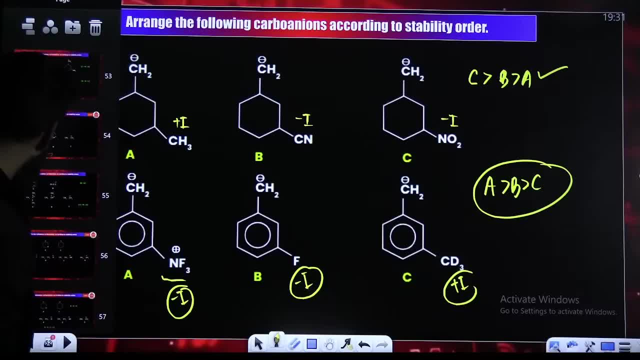 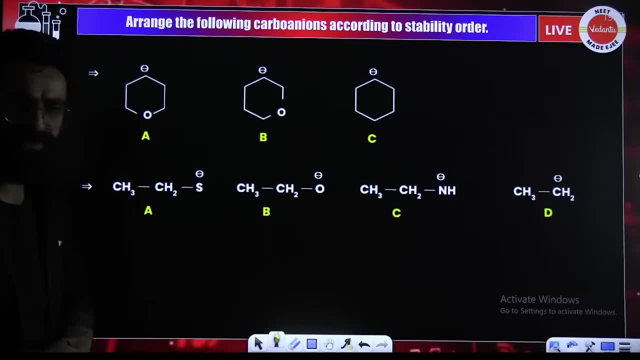 second, just give me a second. okay, look at this particular case. Again, these are Karbanians, Karban carrying negative, negative, negative. Tell me, where is the stability maximum? Where the stability is maximum? I need the answer. I need the answer. 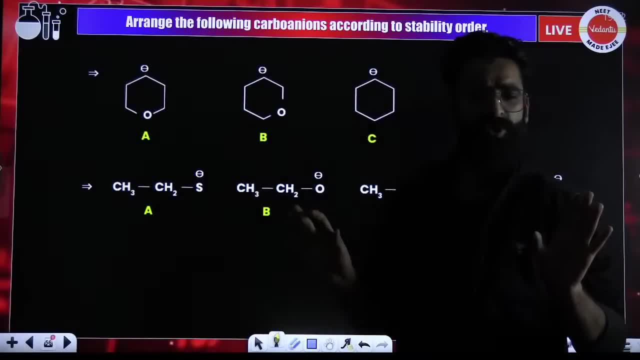 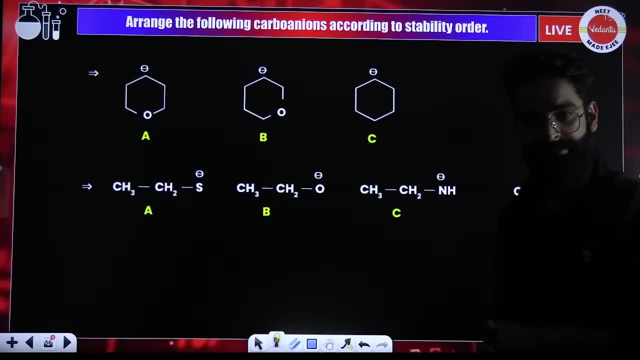 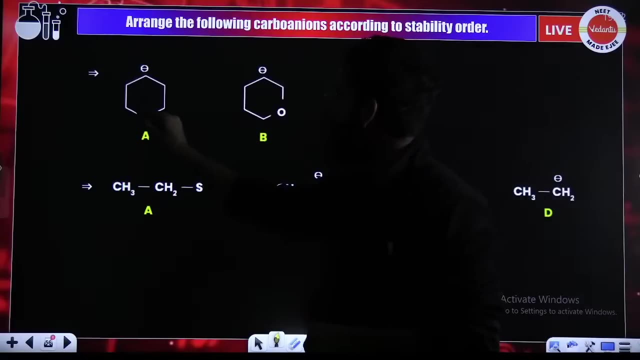 Where is the stability maximum? Whatever concepts I gave you, use those concepts, only nothing else. I'm going to give you the break after this inductive effect is done. Quickly, quickly. What do you think? See, this is oxygen. 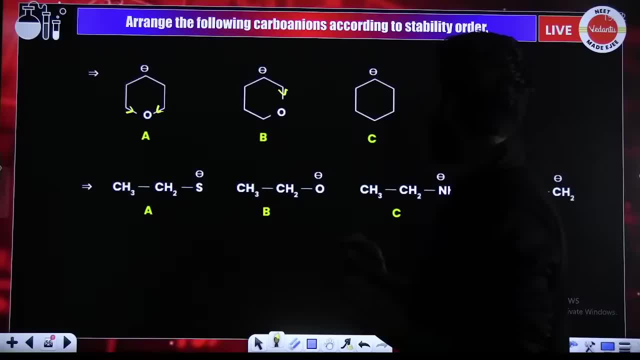 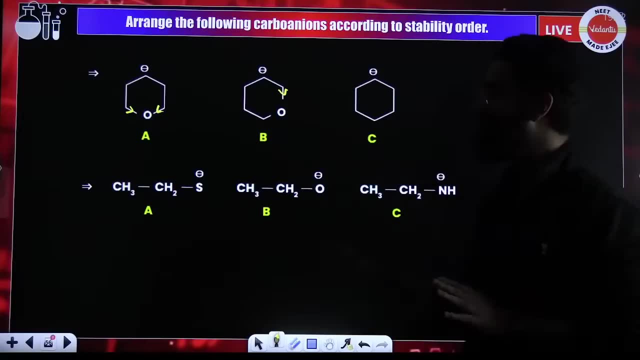 There will be withdrawing electrons. Here the oxygen is comparatively close. Here there is no oxygen. Wherever oxygen is close, wherever withdrawing group is close, there only Karbanian stability is maximum. So B will be maximum stable, followed by A, followed by C. 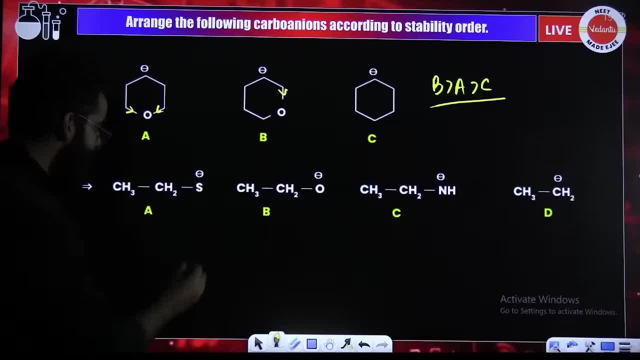 This question I believe you should easily be able to solve. Sulphur carrying negative oxygen carrying negative Sulphur, carrying negative oxygen carrying negative Sulphur and oxygen- they belong to same group. BCD plays a role. This has got less VCD. 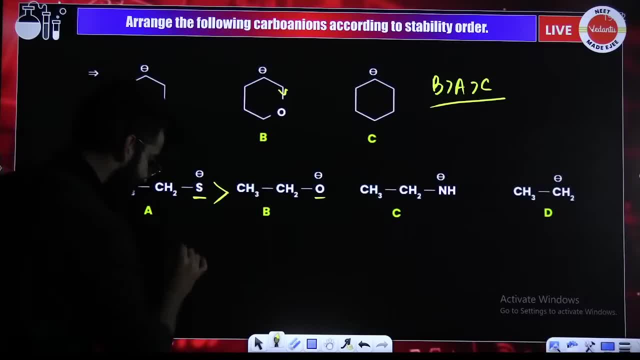 Less VCD means more stability, So negative charge is more stable in this. So A is more stable than B. A is more stable than B. Now compare B and C. Compare B and C. A is more stable than B. Compare B and C now. 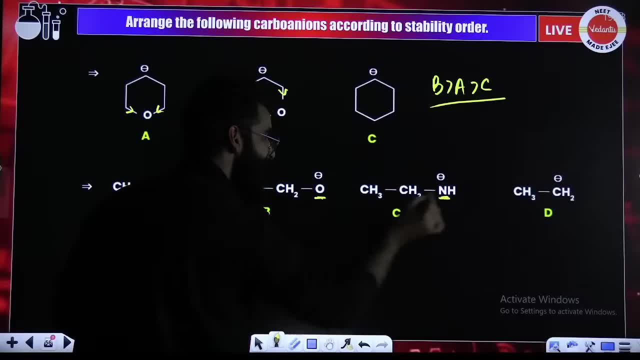 Oxygen, carrying negative nitrogen, carrying negative Oxygen and nitrogen. they belong to same period. In same period, electronegativity plays a role. Negative charge is more stable on more electronegative. Negative charge is more stable on more electronegative because oxygen is more electronegative. So B is more stable than C. B is more stable than C, So order has to be: A: B is more stable than C. B is more stable than C, So order has to be A: B is more stable than C, B is more. 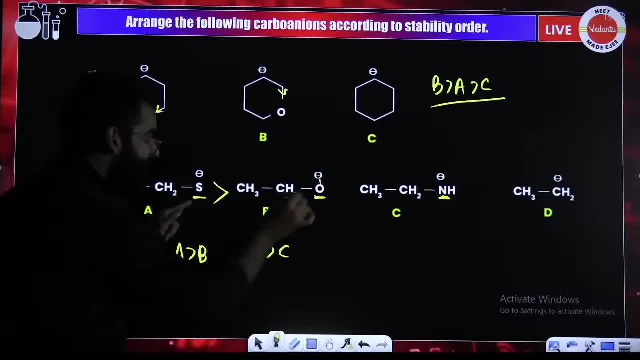 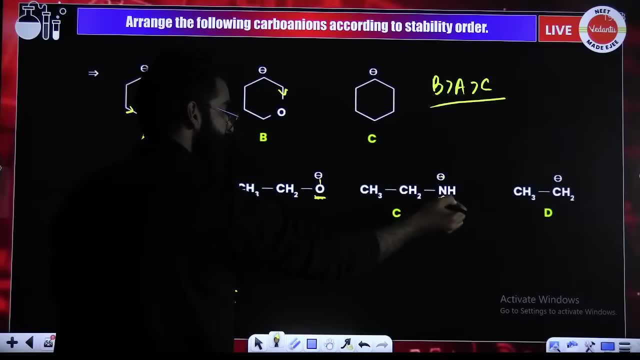 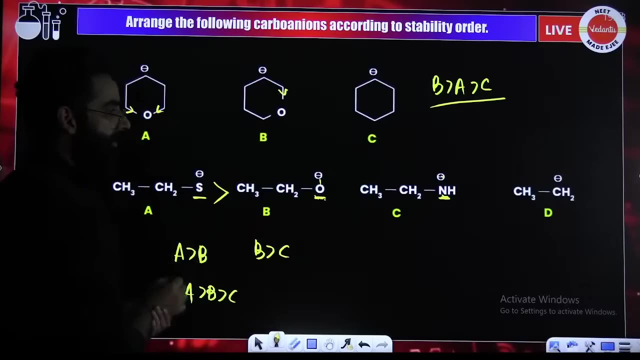 stable than C. When you compared these two, you took VCD into consideration. When you compared these two, you took electronegativity into consideration. Since they belong to same period. electronegativity plays a role. Negative charge is more stable on more electronegative. 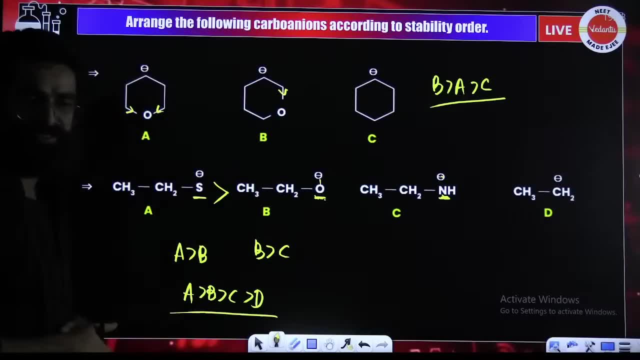 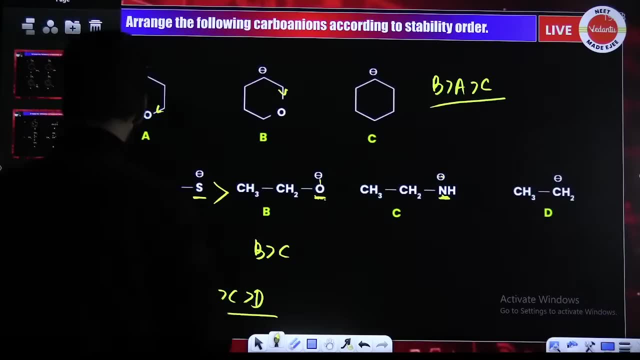 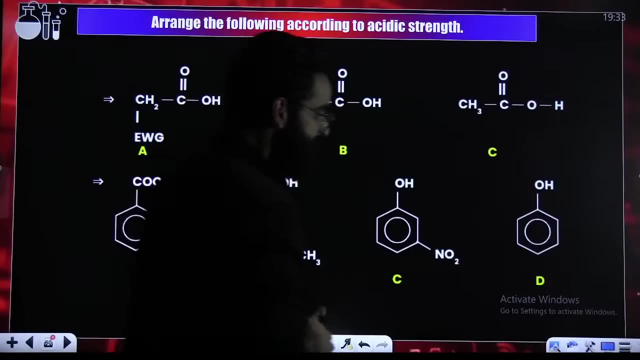 And at the end it will be carbon carrying negative. So this has to be the order: ABCD. Right, guys. ABCD has to be the order Perfect. Now, guys, Look at this particular question. What do you think? What do you think? 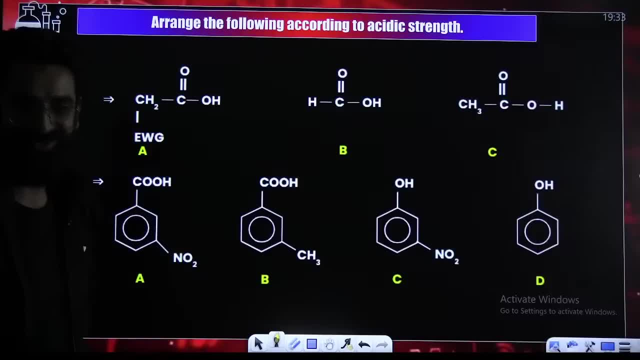 Quickly, Okay, Okay, Okay, Okay, Sorry, Sorry, Sorry, Sorry, Quickly. What is the answer of this question? What is the answer of this question? That was my previous organization, by the way. I used to work. 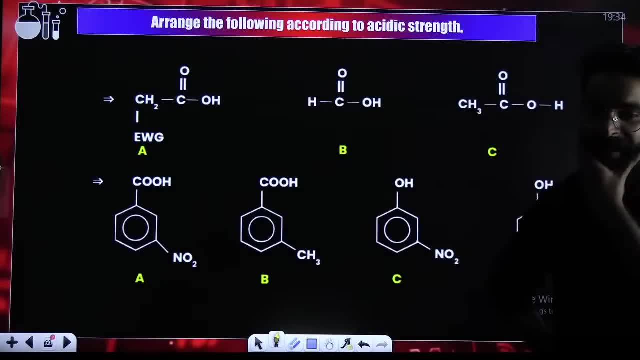 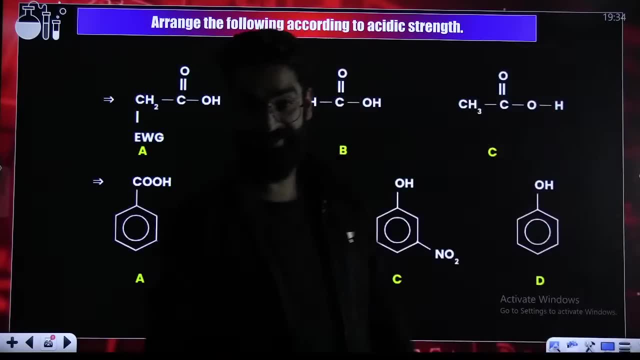 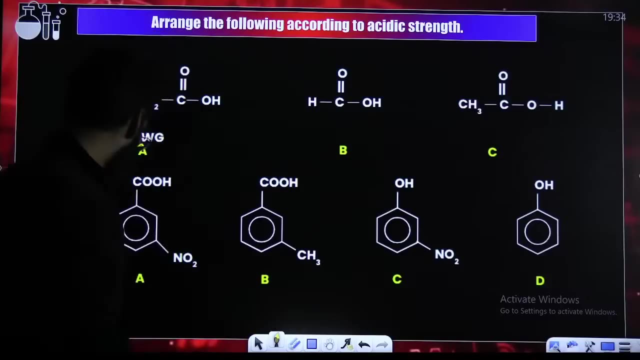 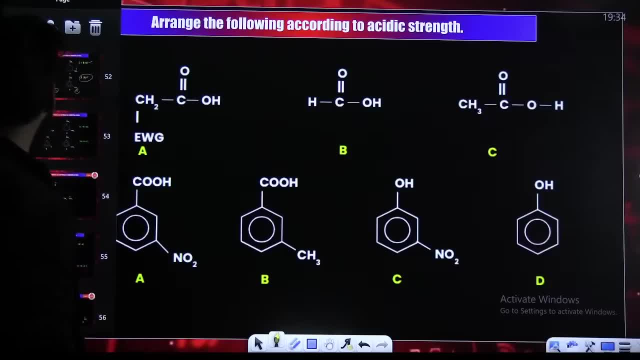 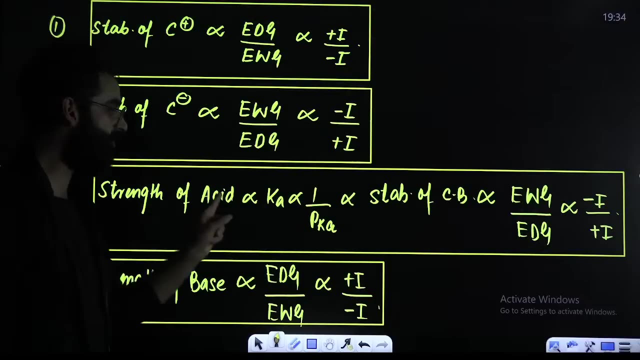 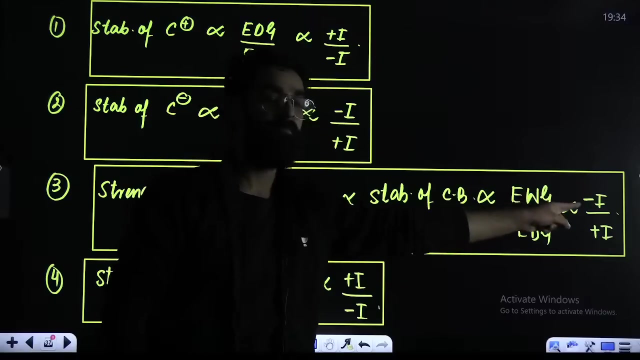 I hope you remember that table which I gave you. I said strength. I hope you remember the table which I gave you: Acidic strength. Acidic strength- Strength of acid- is directly proportional to stability of conjugate base, And conjugate base is stabilized by minus I. So, in short, I would say: minus I groups, they increase the strength of acid. Minus I groups: they increase the strength of the acid Right. Plus I groups: they decrease the strength of the acid. Now, Now you are going to give me the answer. 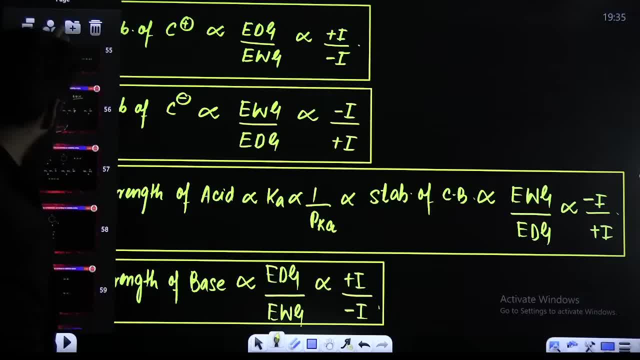 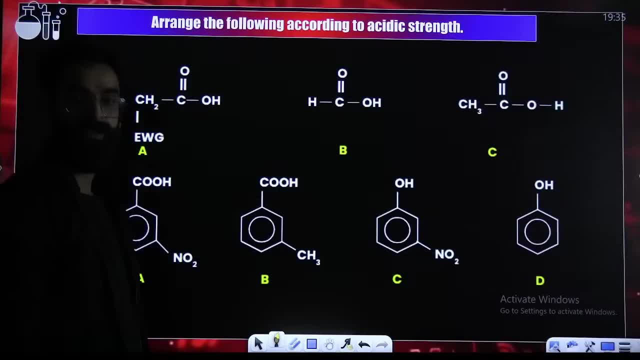 Since you know it already, you are going to give me the answer now. Quickly, guys, Just a second. It was slide number 60.. I believe this is slide number 60.. Yes, Okay. So first of all, identify the site from where hydrogen is going to donate. 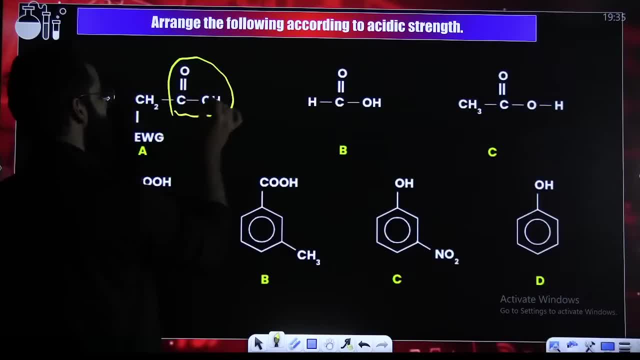 Hydrogen is going to go away as H+. This is the site from where hydrogen is going to leave as H+. This is the site from where hydrogen is going to leave as H+. This is the site from where hydrogen is going to leave as H+. 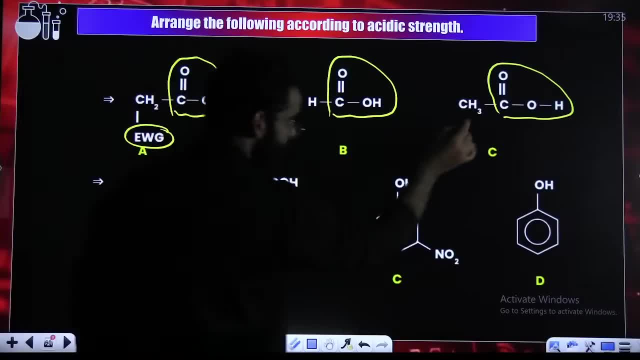 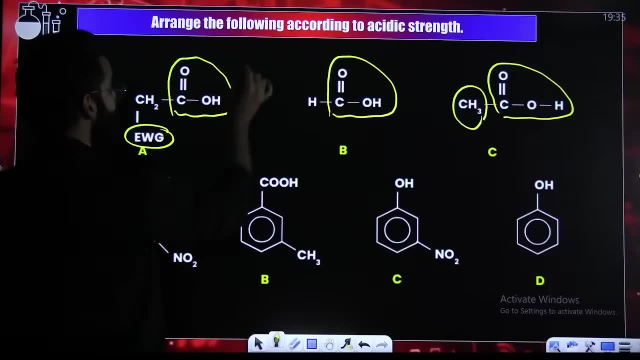 Here you have got electron withdrawing, Right Here You have got electron donating, Electron donating, Electron withdrawing groups. They increase the strength of the acid. So I would say A strength will be maximum, Followed by B, Followed by C. 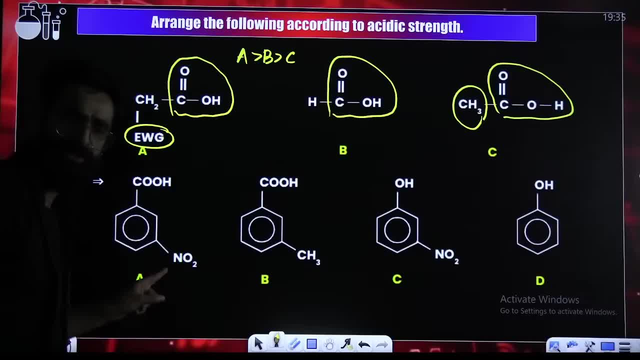 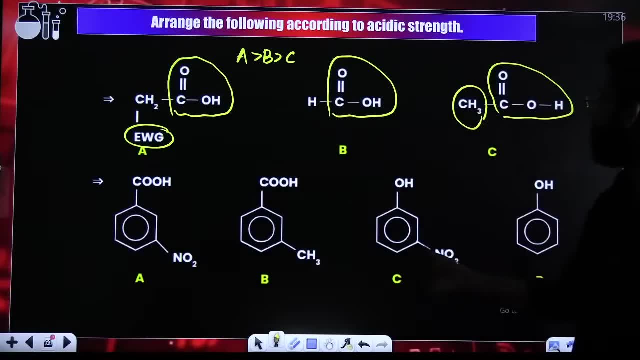 Right Now. Majority of the students will do a mistake, I believe, here in this question. Tell me Which one is more acidic. I think a lot of students will do a mistake here. Quickly, Which one is more acidic here? 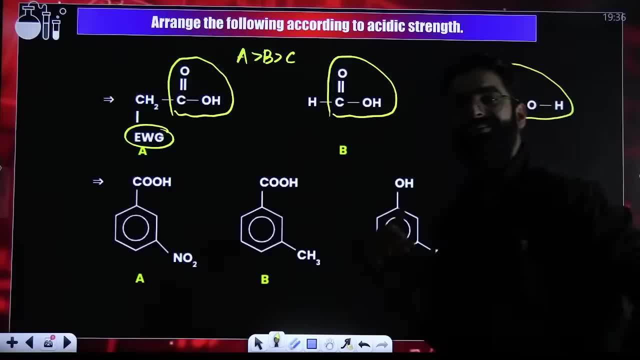 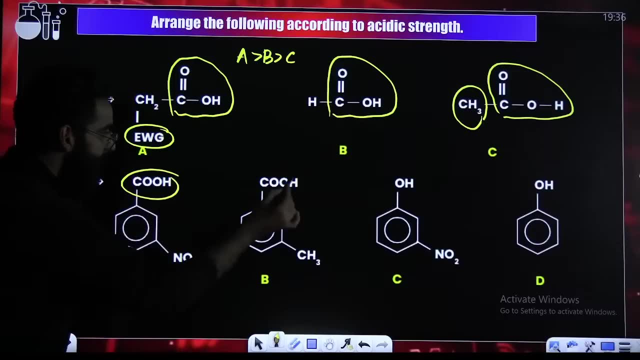 Guys, after looking at this question, Do not straight away: C plus I minus I plus M minus. I Do not do that. Do not do that Why? Because this is carbo-oxalic acid. This is carbo-oxalic acid. 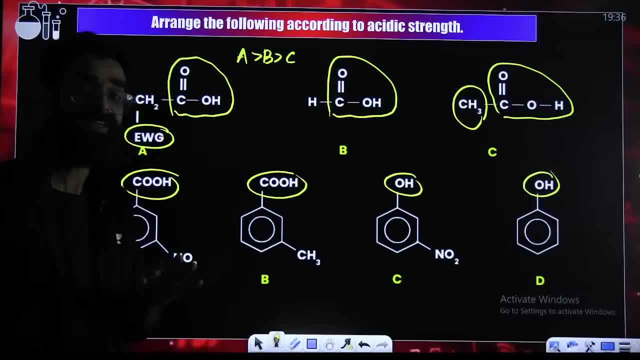 This is phenol. This is phenol And generally you know it. Carbo-oxalic acids are stronger acids than phenols. Carbo-oxalic acids are stronger acids than phenols, So definitely A and B is going to be more acidic than C and D. 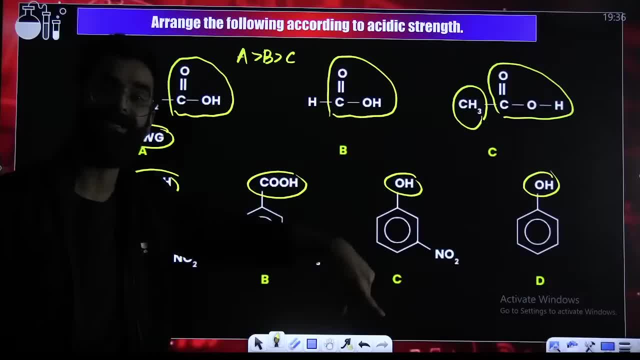 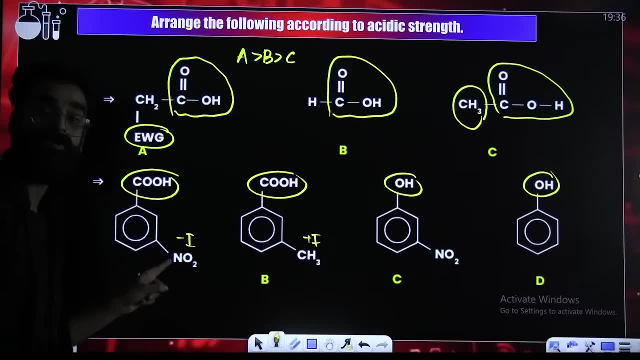 Okay, Okay, A and B is going to be more acidic than C and D. Now, among A and B, Among A and B. This is minus I showing. This is plus I showing. Withdrawing Electron withdrawing group. It increases the strength of acid. 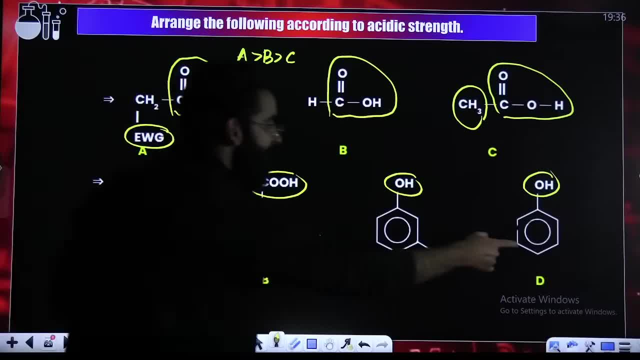 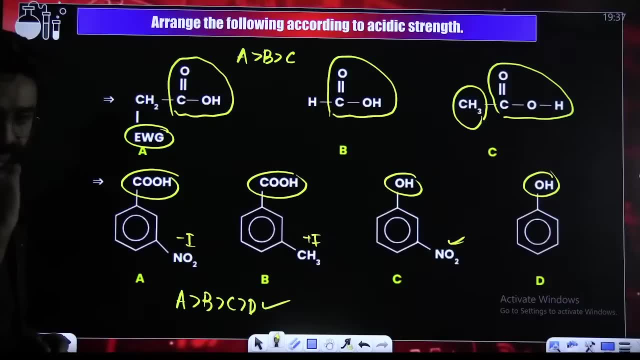 Right, So A will be maximum acidic, Followed by B, Now among C and D. This is withdrawing. There is no withdrawing group, So I will say C, Then D. I believe this particular question is done Again, Right. 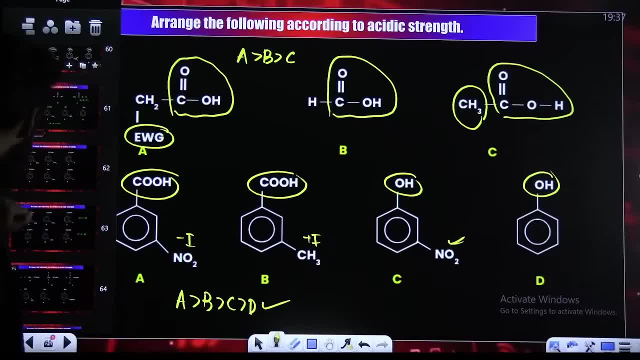 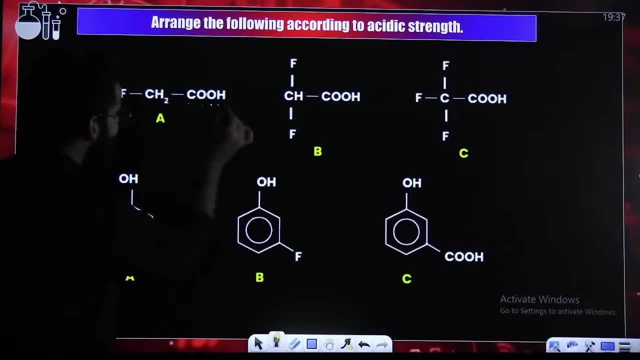 Agreed, Right guys. Okay, What about this one? What about this one? First of all, look at the site from where hydrogen is going to go away as H positive. I identified the site Right Over here. One fluorine. 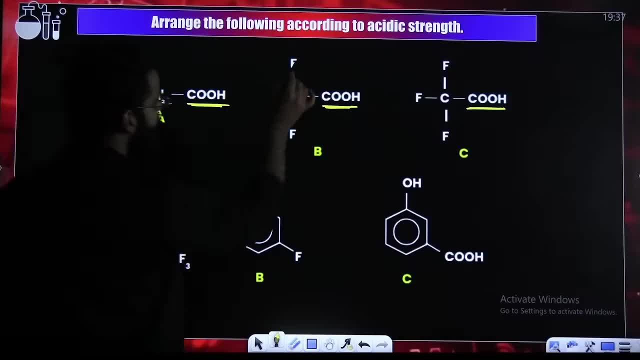 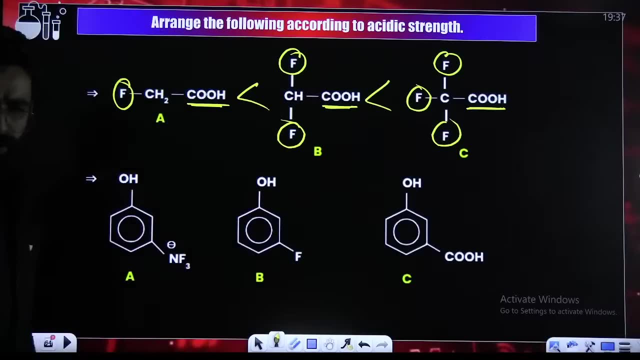 Two withdrawing, Three withdrawing: More the withdrawing groups, More the acidic strength, More the withdrawing groups, More the acidic strength. Done and dusted. Look at the next one. This is NF3 positive. Okay, Okay. First of all, 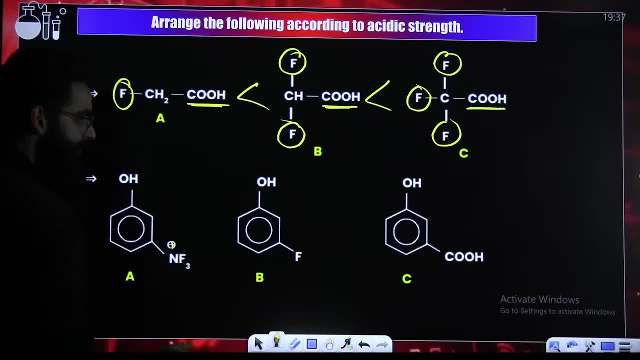 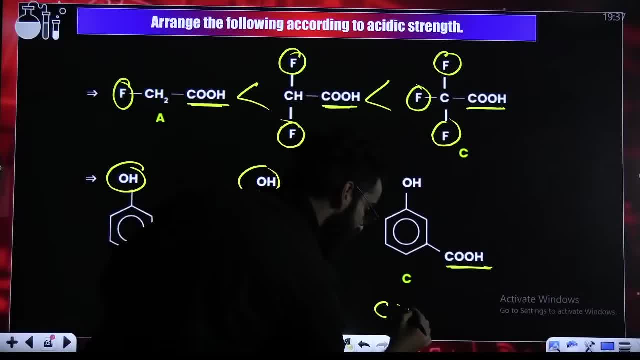 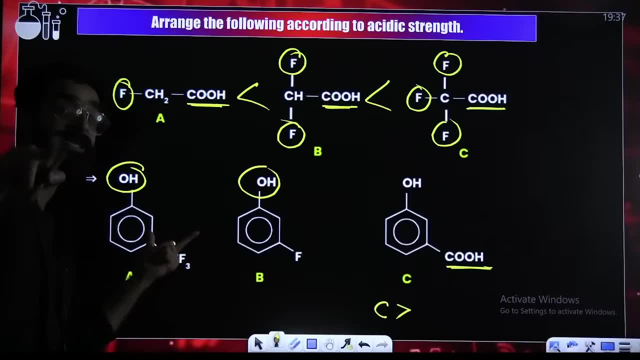 Carbo-oxalic acid. Carbo-oxalic acids are stronger acids than they are phenols, So C will be maxima-acidic. Now, among A and B, Strength of acid is directly proportional to minus, I Right, Minus I. 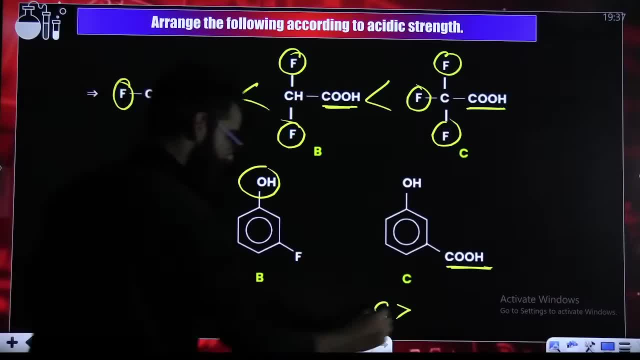 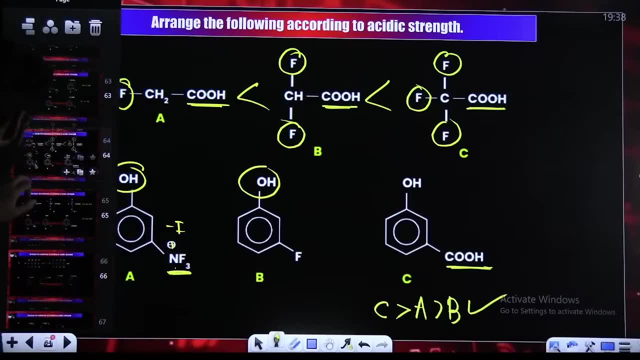 This shows more minus. I. This is more withdrawing. This is more withdrawing. So, after C, I will prioritize A, Then I will prioritize B. Right, I believe this is also clear. I believe this is also clear. Okay, Okay. 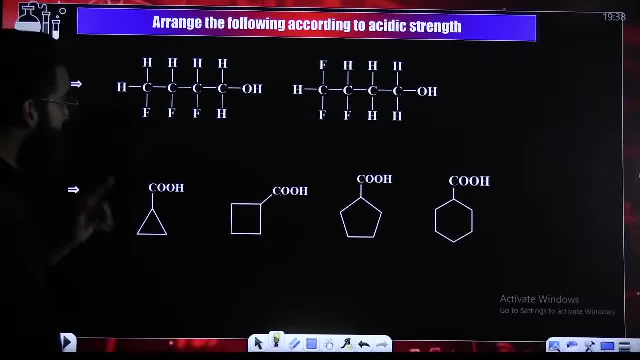 What about this particular equation? or two, one or two, three. from here, hydrogen is going to go away as h positive. from here, hydrogen is going to go away as h positive. perfect now, one, two at carbon number two, there is withdrawing. one, two, three at carbon number three, there is withdrawing. so where will the fluorine show? 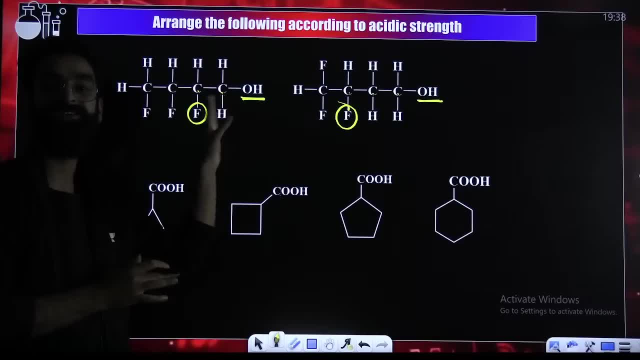 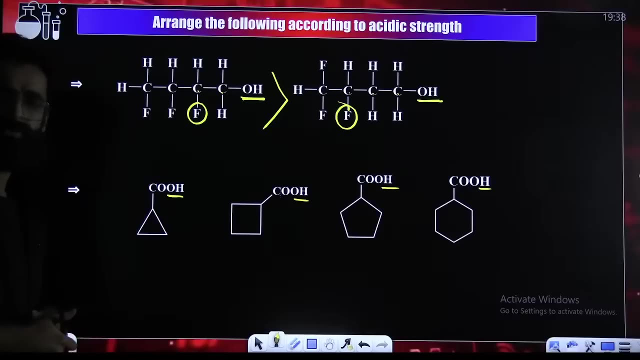 more prominent minus sign: where the distance is less, where the distance is less. so, in the first case, more withdrawing. more withdrawing means more acidic strength. right, okay, now. now, first of all, this is the site from where hydrogen is going to go away as h positive. perfect now, you know. strength of acid is directly proportional to stability of conjugated base. 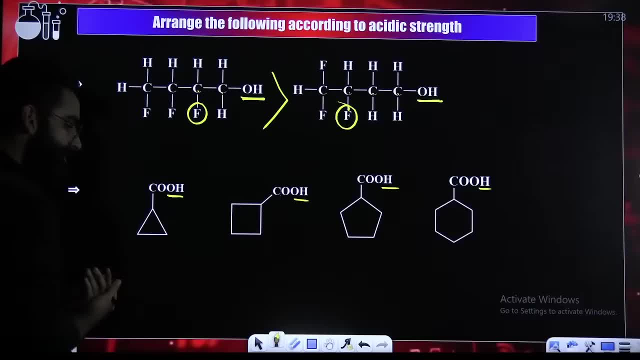 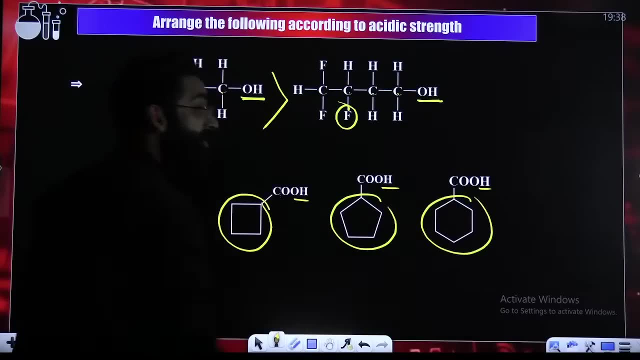 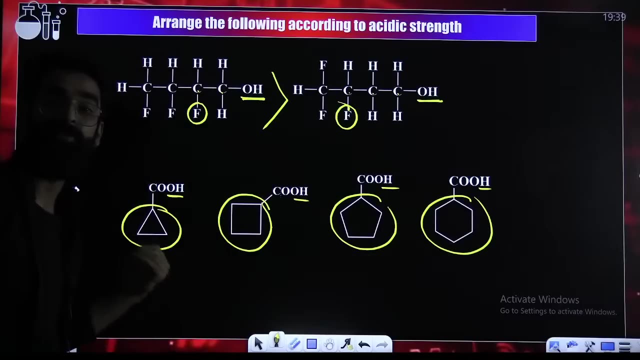 perfect stability of conjugated base, right or directly. tell me one thing: which, which ring over here, will be more withdrawing: angle strain concept, angle strain- three membered, four membered, five membered, six membered, three membered ring: more angle strain, more electronegativity, more withdrawing, more withdrawing. if it is more withdrawing, that 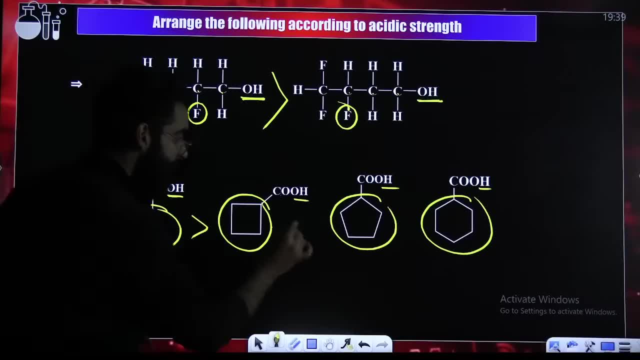 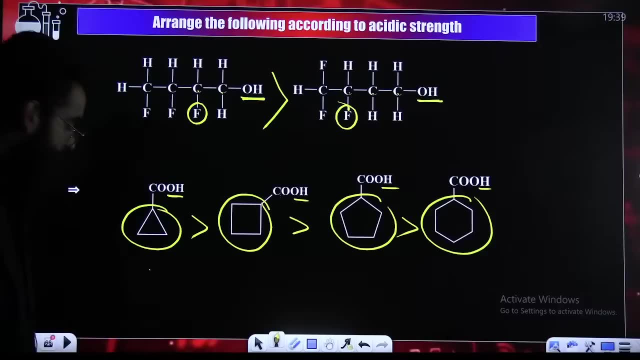 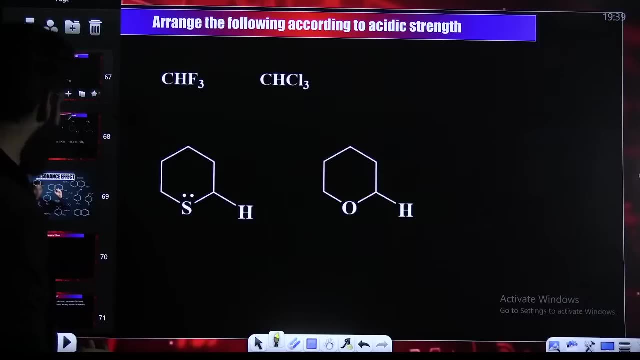 means it will stabilize the conjugate base, the maximum right. so this is the stability order of the conjugate base, as well as the stability, as well as the order of the strength of the acids. right, okay, here you might do a mistake. here you might do a mistake. you might do a mistake. 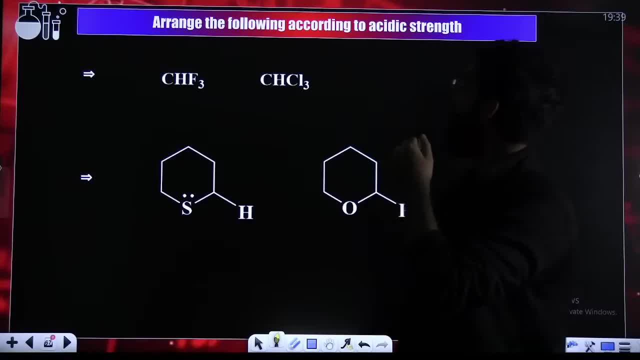 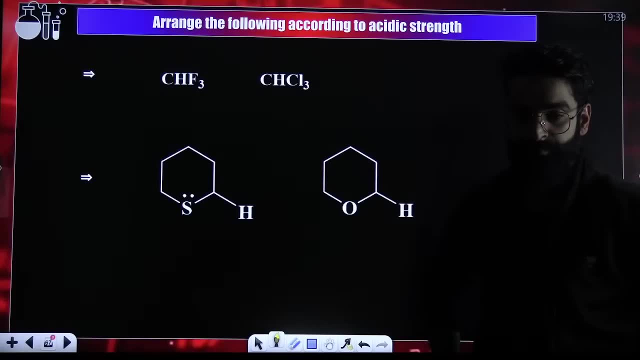 right. so it's best to just leave a indefinable condition. one more: are you certain you are you sure you are sure? yeah, really pretty happy with yours. i am sure bit of panic, but you non tank fo you, im sure, in stone, Shanwen, hold on, hold up, hold on이�intérieur of thatanda, Jerry, and the link you mike being deleted. we'll take a couple second. that apply such when iranian lies on your trip in Bangalore, india, in India, on which one is more acidic. tell me that in one and two, which one is more acidic in one and two, which one is more acidic. tell me that in one and two, which one is more acidic among one and two, which one is more acidic? quick, do we know that among one and two particulars, which one is more acidic? quickly? 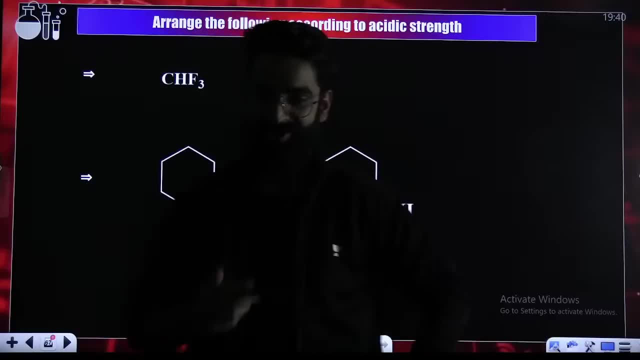 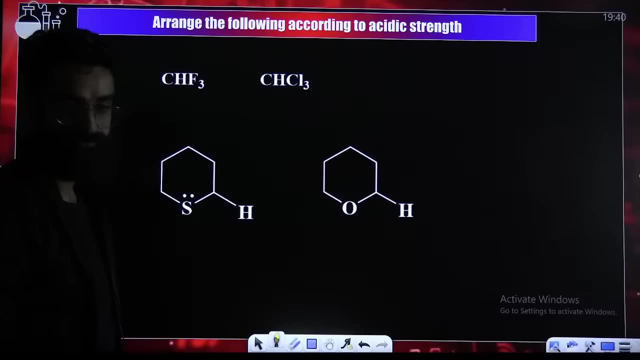 Are you sure? Are you sure Among 1 and 2, which one is more acidic? Have a look, guys. First of all, make their conjugate basis. Take hydrogen out as H+, this will be CF3-2.. Take hydrogen out as H+, this will be CCL3-2. 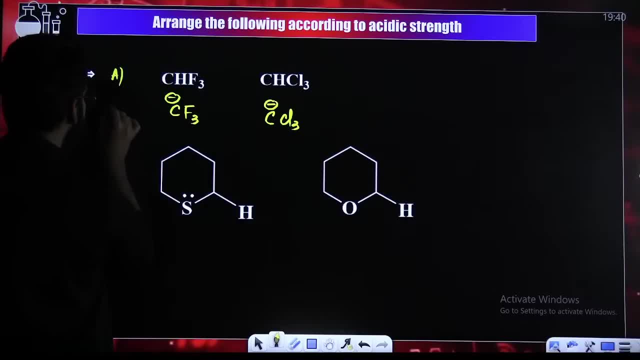 These are the conjugate basis. See, these are your acids and these are their conjugate basis. Now check the stability of these conjugate basis. Check the stability of these conjugate basis. Have a look, guys. Try to understand Carbon carrying negative carbon carrying negative right. 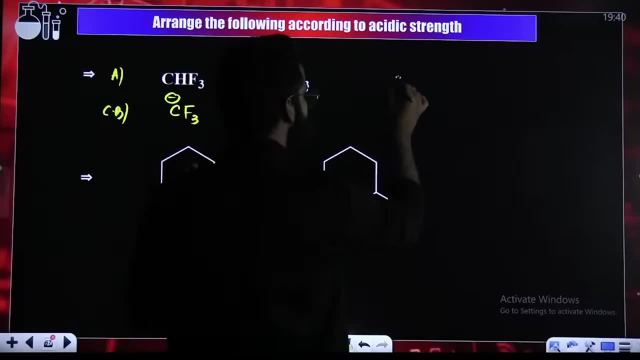 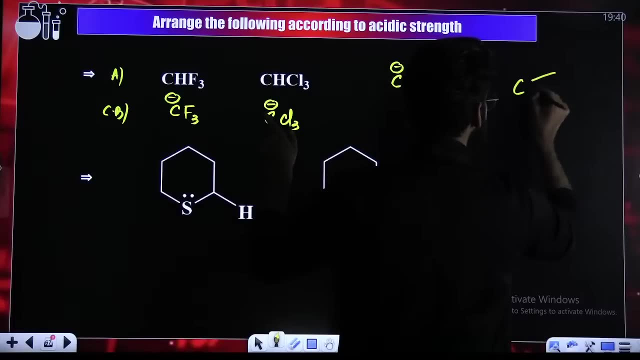 But this particular carbon is attached to 3 fluorine atoms. right, This is carbon and you have got 3 fluorine atoms. Perfect. Look at this particular carbon. It is attached to 3 chlorine atoms, 3 chlorine atoms. These are the. 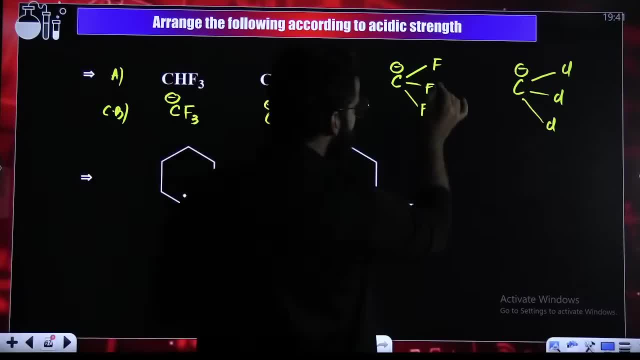 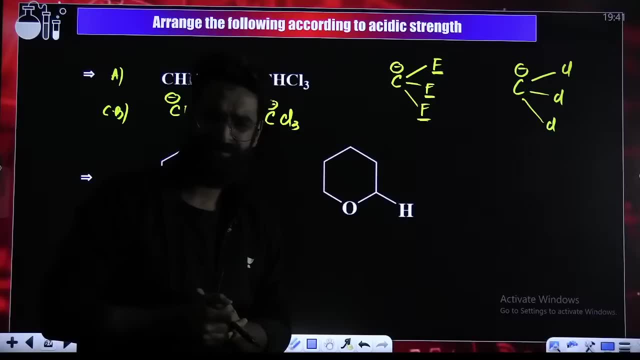 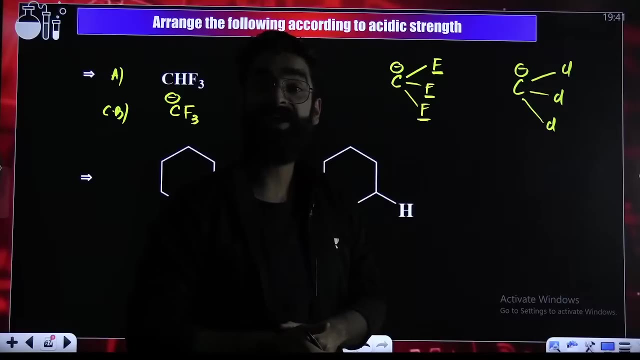 These are the conjugate basis, basically, which we have. Now. tell me one thing: In the fluorine, do you have any vacant orbitals? In fluorine, are there any vacant orbitals? No right, In chlorine, if you remember chlorine. in chlorine there are vacant d-orbitals. 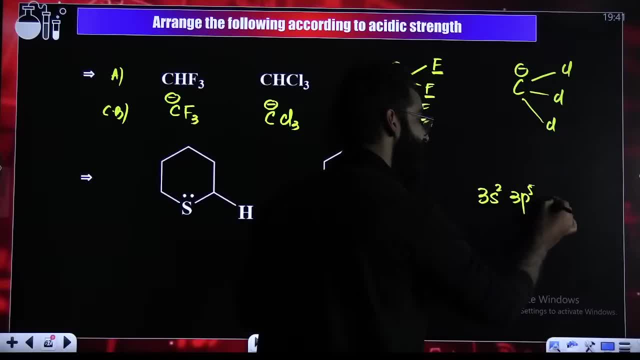 Chlorine configuration is 3s2, 3p5.. But there is 3d as well, 3d0, there are vacant d-orbitals. So if there are vacant d-orbitals in chlorine, can I say: 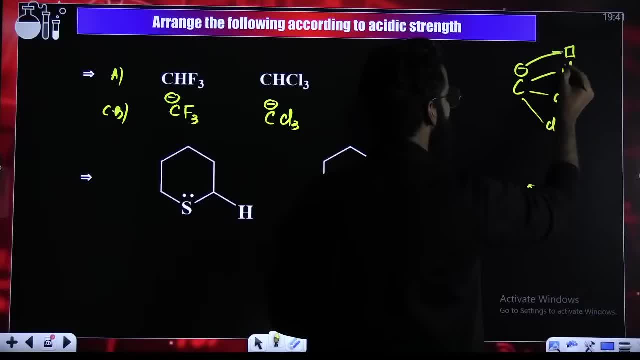 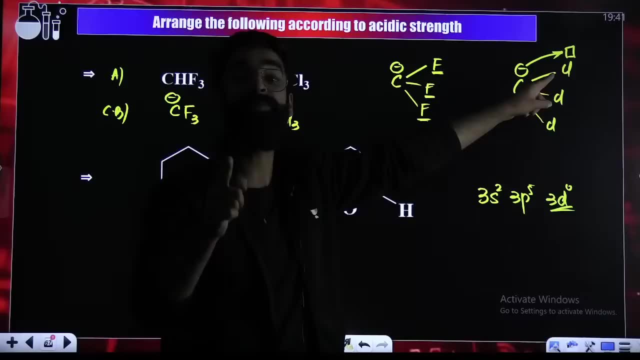 if there is a vacant d-orbital in the chlorine, can I say it can show the backbonding. It can show the backbonding If it shows backbonding. backbonding stabilizes the carbanion, But I would say backbonding it stabilizes your conjugate base. 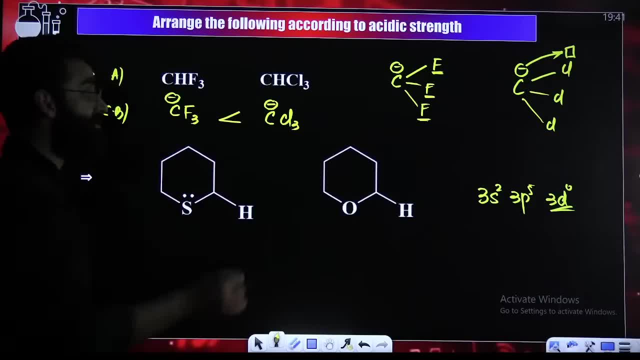 So which conjugate base is more stable? This conjugate base is more stable. More stable the conjugate base, stronger the acid. More conjugate, more stable the conjugate base, stronger the acid. Look at the next one. Take hydrogen out as H positive. 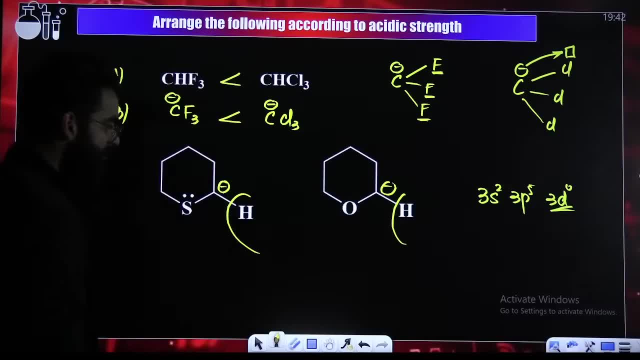 Negative charge. Hydrogen out as H positive negative charge. Right Perfect, Now. this is sulfur. Sulfur outermost configuration 3s2, 3p4.. And there is 3d as well, containing 0.. 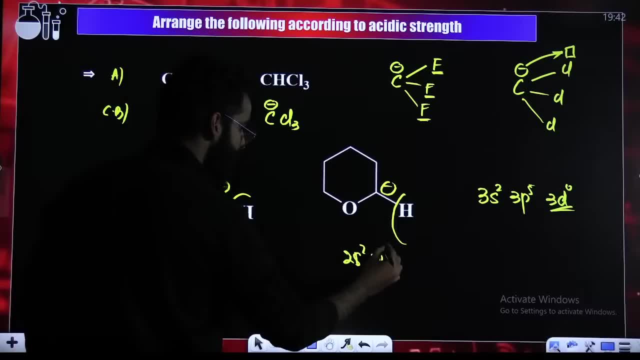 Oxygen oxygen is simple: 2s2, 2p4.. Right, There is no d, there is no vacant orbital. Here you have got vacant orbital. If there is vacant orbital, there is a chance of backbonding. 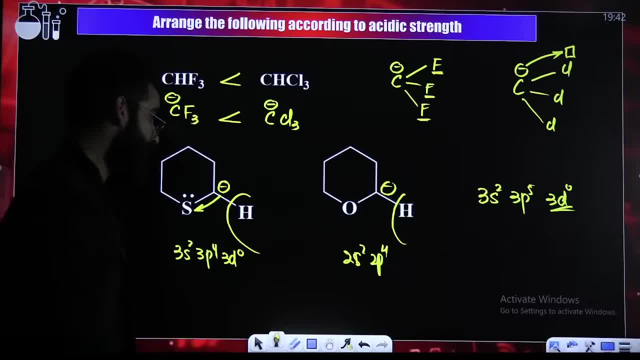 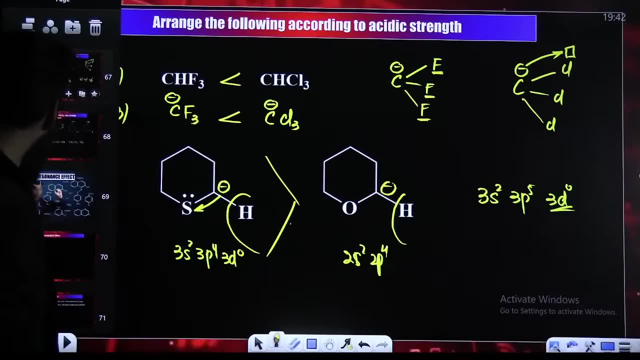 And backbonding stabilizes the conjugate base. So wherever the conjugate base is more stable, that acid is going to be stronger. I believe this is clear to everyone. Yes, So with this, your inductive effect is clear. Now is the time for resonance, guys. 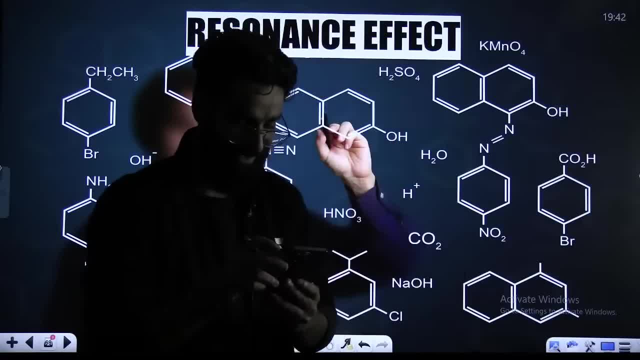 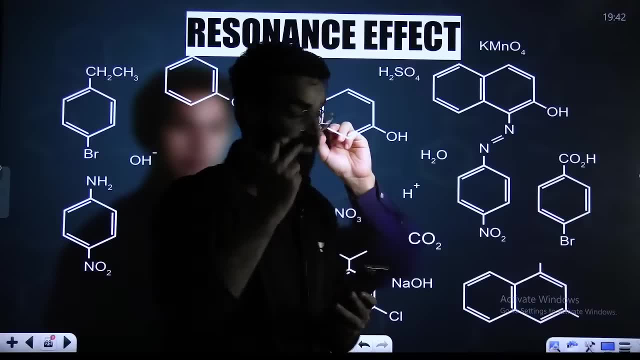 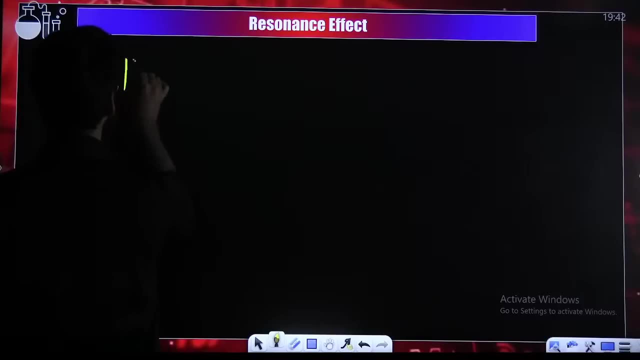 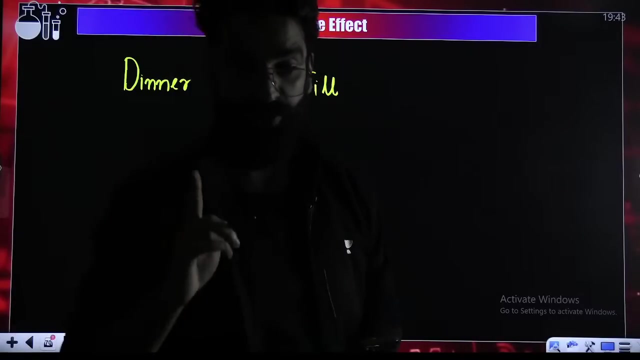 So do you want a break? Do you want a dinner break right now? Yes, Do you want a dinner break right now? Then we'll start the resonance. Yes, but guys, come back. Are you going to come back? Let me first of all see what you are saying. 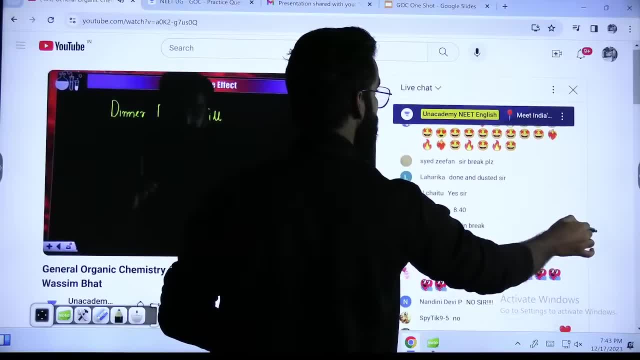 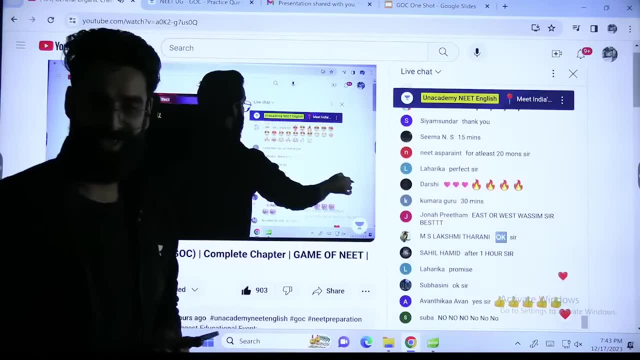 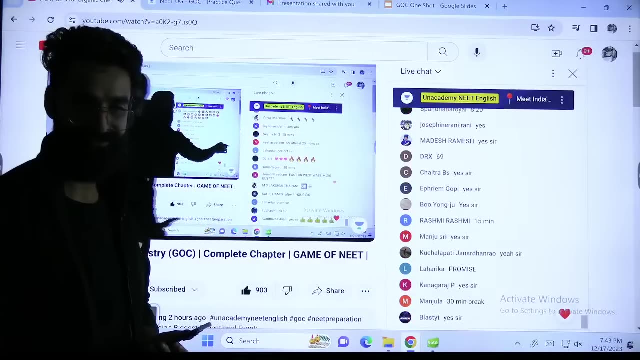 Let me open your chats once. Are you planning to come back? Tell me that. If you are not planning, then I'll end the session. It's okay. Are you planning to come back? I need that promise from you. Okay, tell me one more thing. 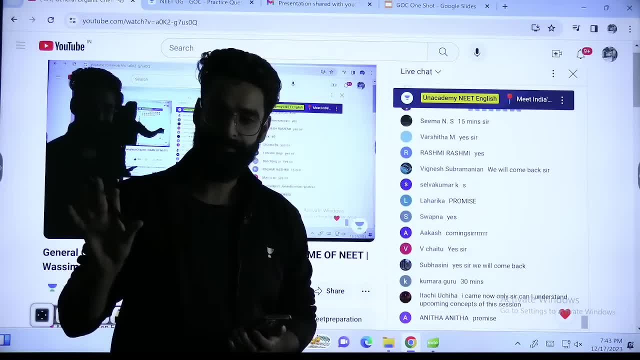 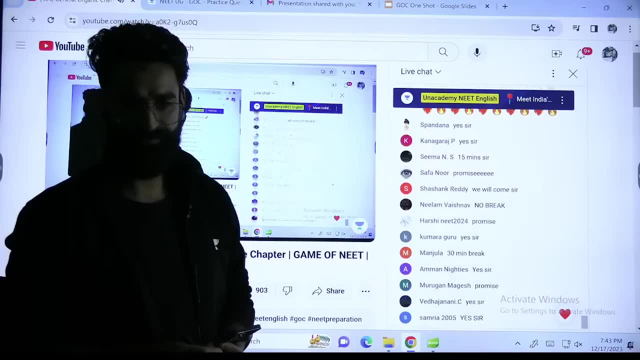 Whatever I've taught you till now, is every single thing clear? Honestly, Can you do the questions based on the concepts which I gave you till now? Honestly, you are going to let me know. Honestly, you guys are going to let me know? 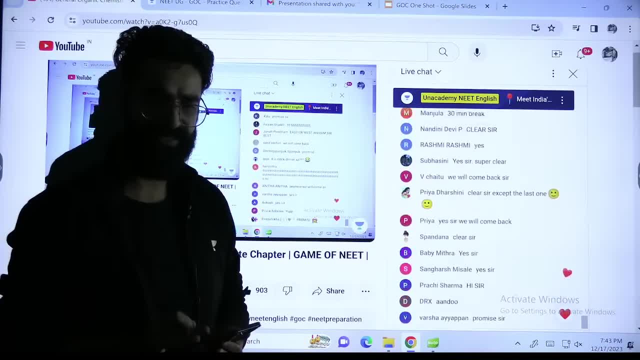 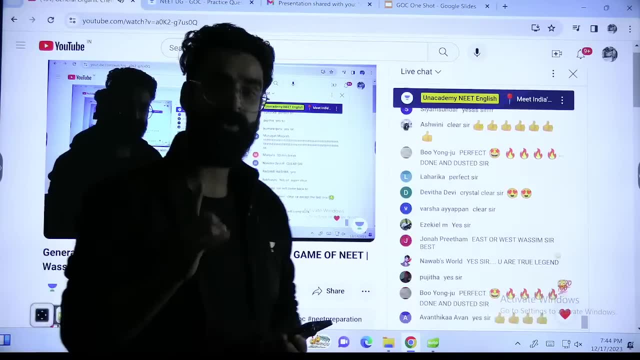 I want everyone to let me know quickly Whatever I've taught you till now. is every single thing clear? Yes, I would want every one of you to join back again on time, Right? So what time will be meeting? It's 745 right now. 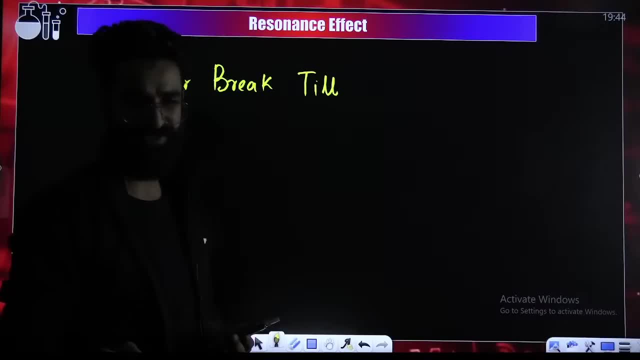 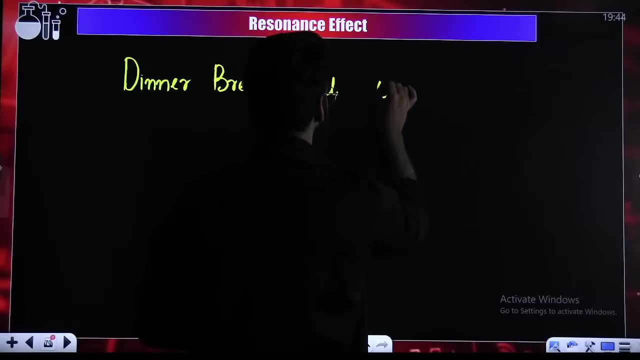 745 right now. So maximum it will take you 30 to 40 minutes for dinner, right Even I'll have dinner So. so we'll be back at 8.. 825 will be back, Okay, So session resumes at 825.. 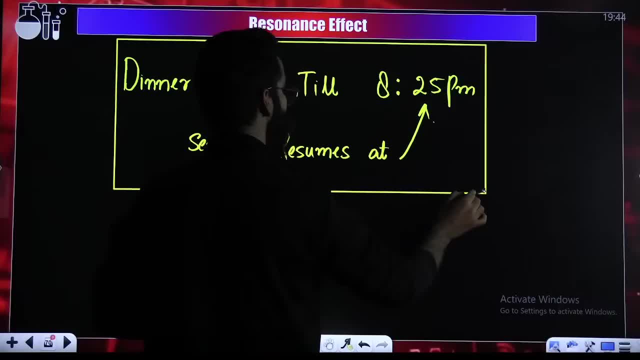 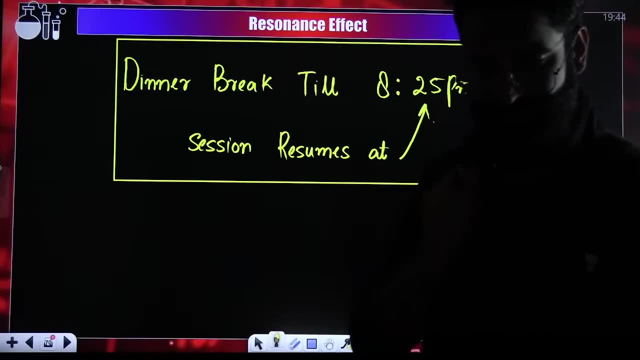 Perfect, Have dinner. come back, because it's a long marathon going to happen. Okay, It's a long marathon. You have to be with me till the end. Okay, Right, But be back on time, guys, Be back on time. 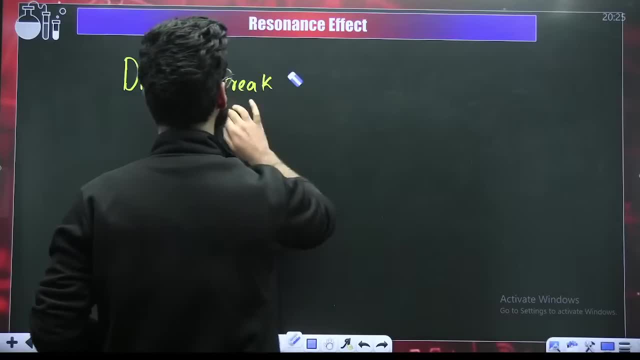 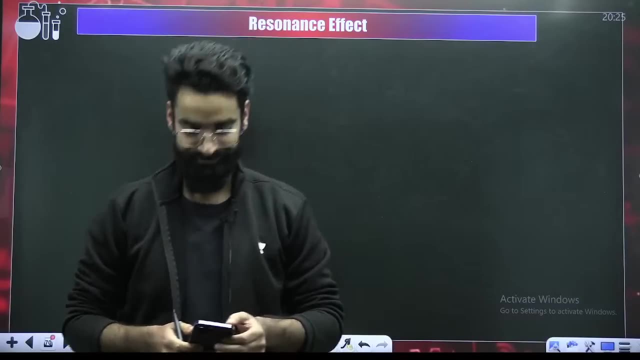 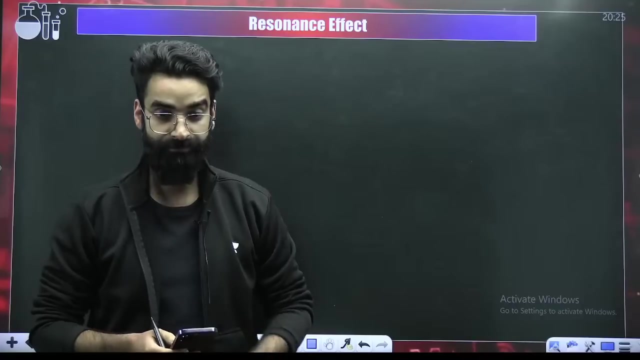 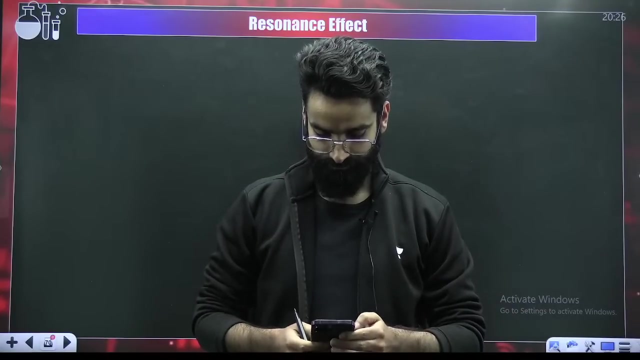 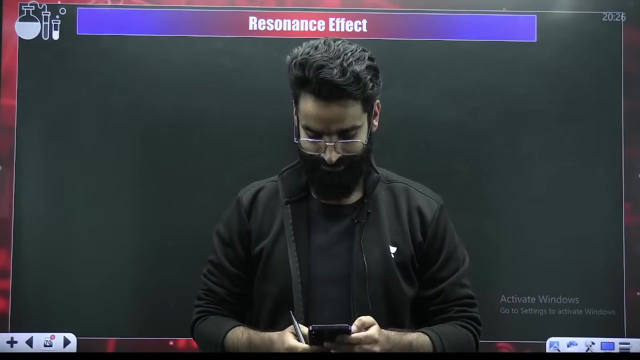 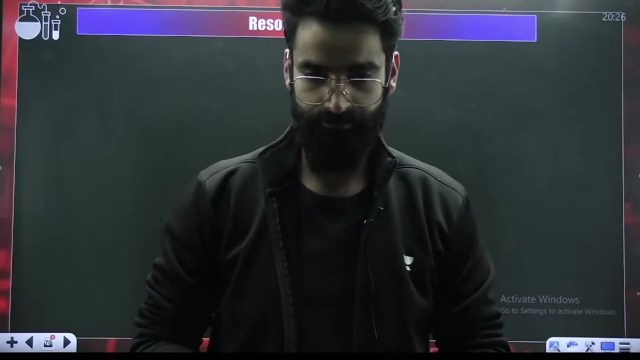 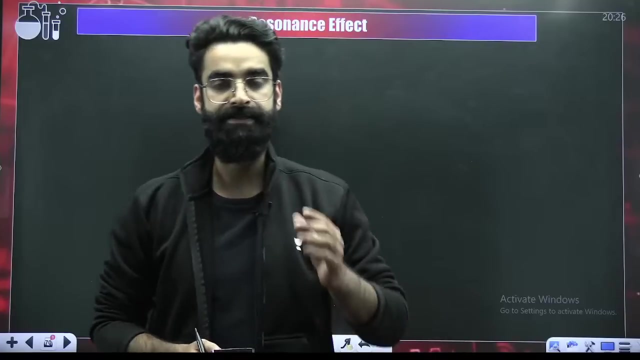 Let me know quickly in the chats: Yes, yes, I'm done, I'm done, I'm done, guys, I'm done. What about you? Are you all done? People are still having Guys tell me one thing: like: whatever concepts we discussed till now, is every single thing clear. 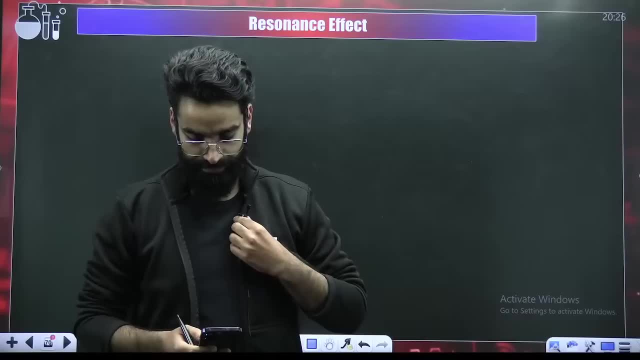 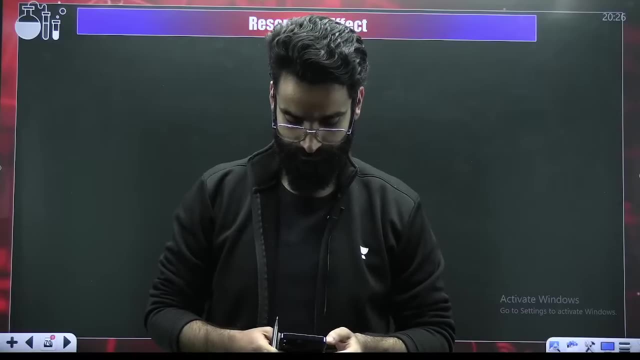 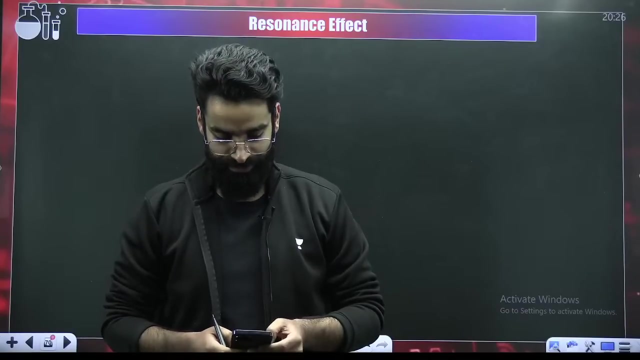 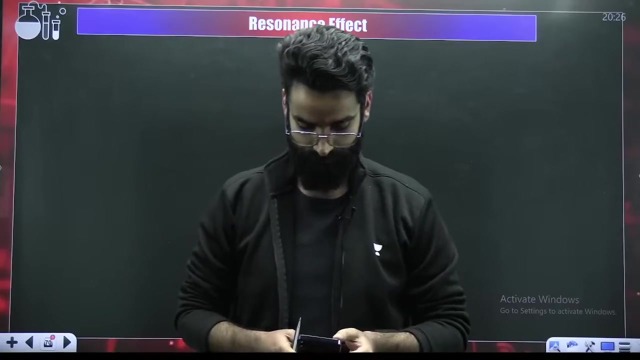 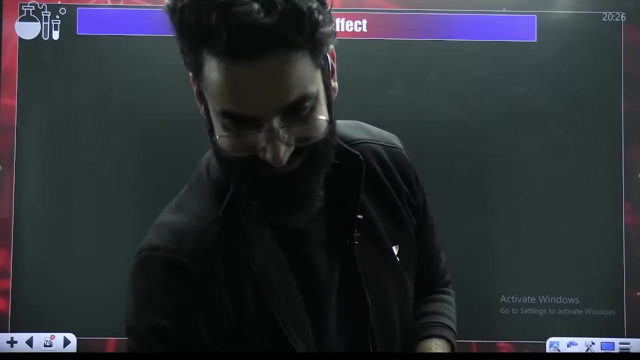 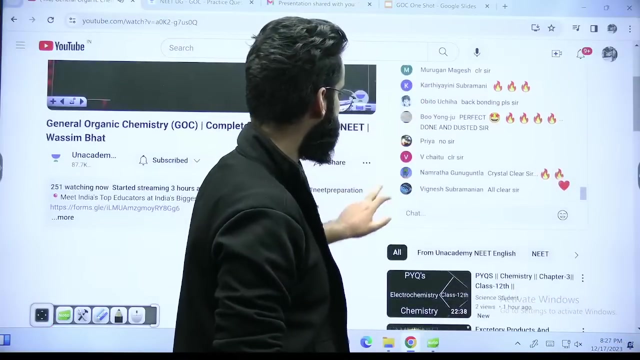 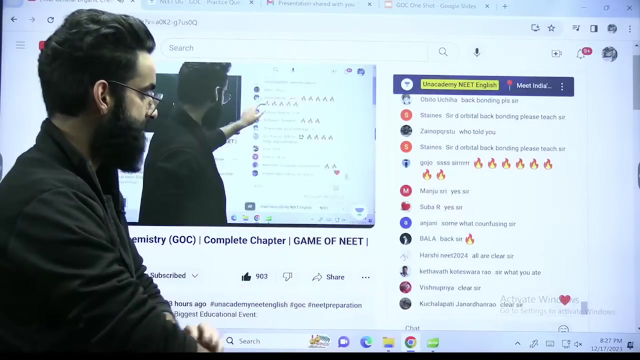 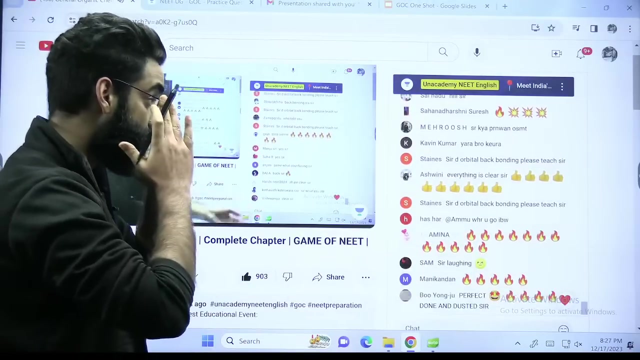 Let me know in the chats quickly: Yes, Sushant, Yes, yes, Quickly in the chats – whatever we discussed till now is every single thing clear. So let me know quickly, guys, all the things are clear till now, All right. 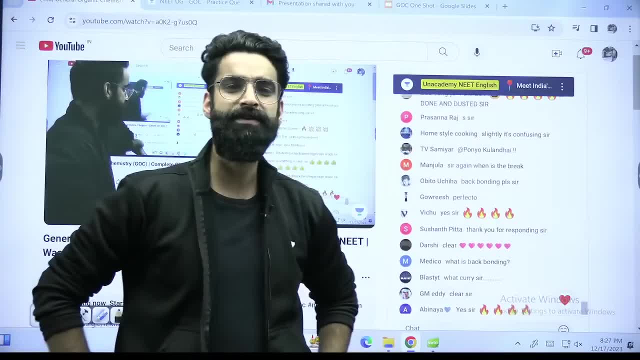 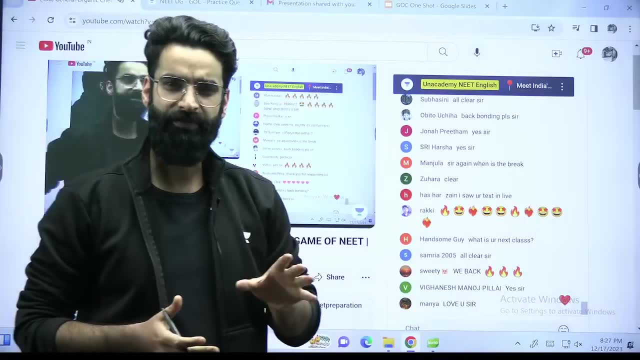 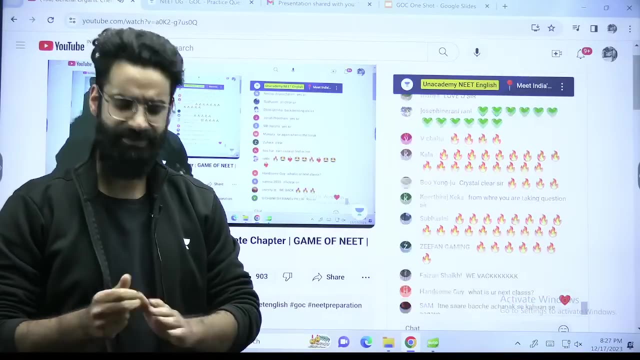 All right. So the last topic which we discussed- what was that? That was Indictive Effect and its applications. right, We saw different types of questions based on Indictive Effect, in which you were supposed to talk about the stability of carbocation, stability of carbanion acetic strength, right. 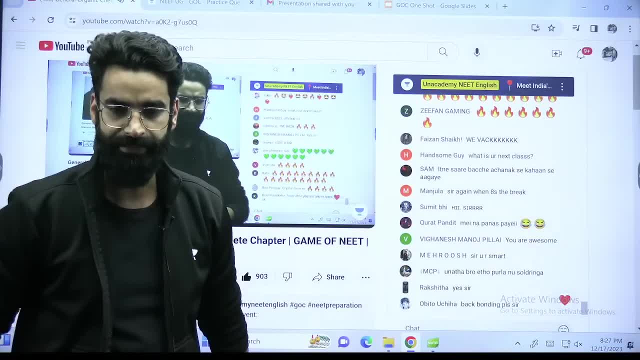 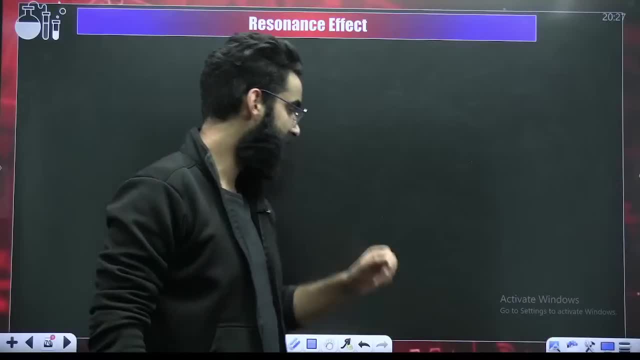 Strength of acids, strength of bases, all those things were discussed in detail. So now, my dear students, we are going to move into one more important topic of this particular chapter. You can call it as the most crucial part of the chapter. 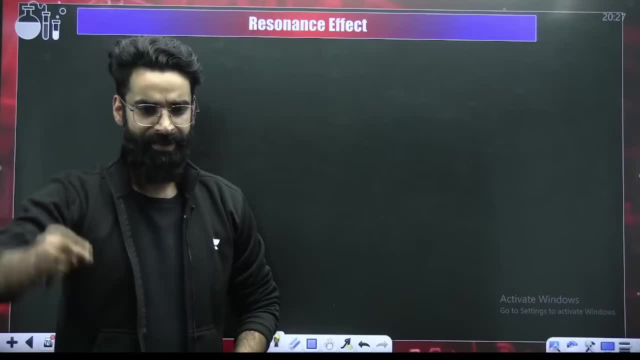 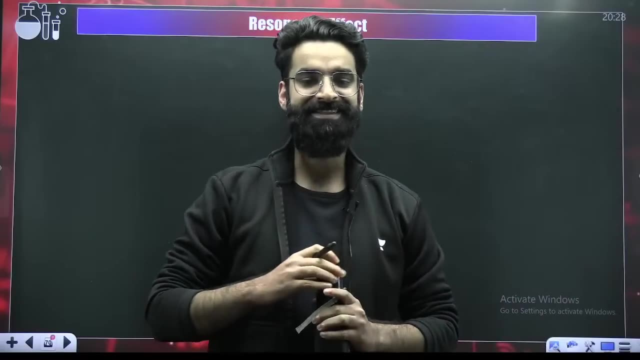 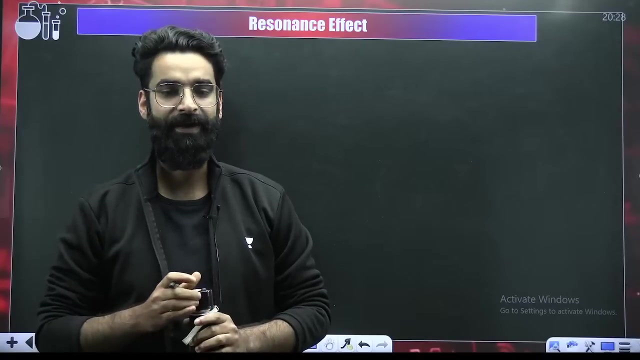 And that is going to be Resonance. Just let me know once in the chats how many of you have studied Resonance before Someone is asking, Sir, when is the break? again Will complete Resonance, its applications and lot of things related to Resonance, right? 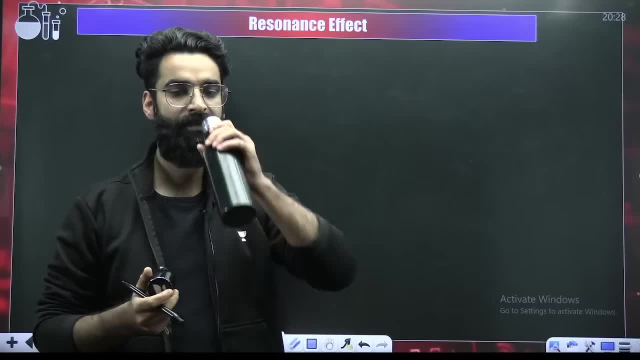 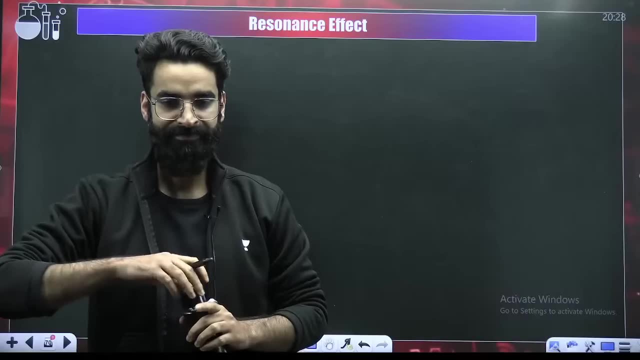 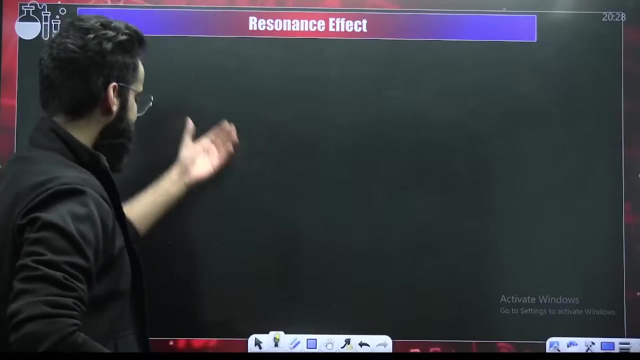 And after two, two and a half hours, I will give you one more break for 15 minutes. Okay So, let's get started. Okay So, let's move on. then Let's have a look on what Resonance exactly is all about. 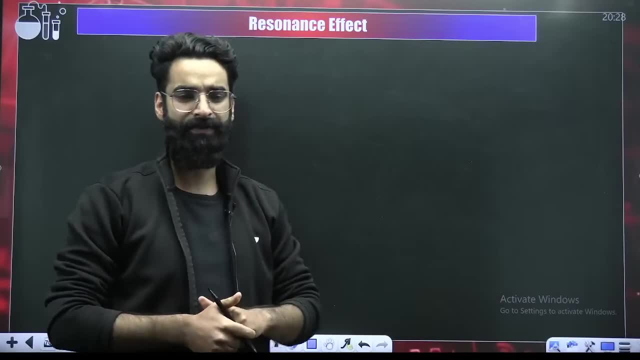 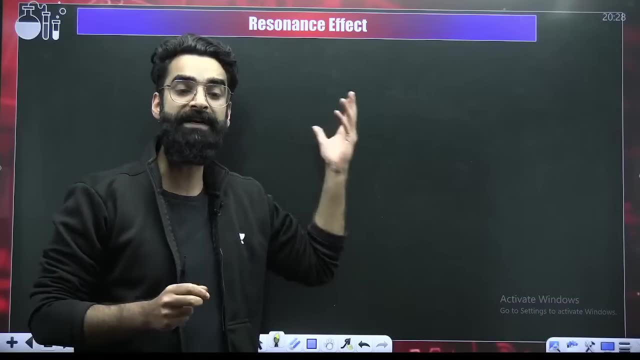 My dear students, before letting you know the exact meaning of Resonance, we should know first of all which kind of molecules do exhibit this property. Which of the molecules can show Resonance, Which of the molecules can not show Resonance? 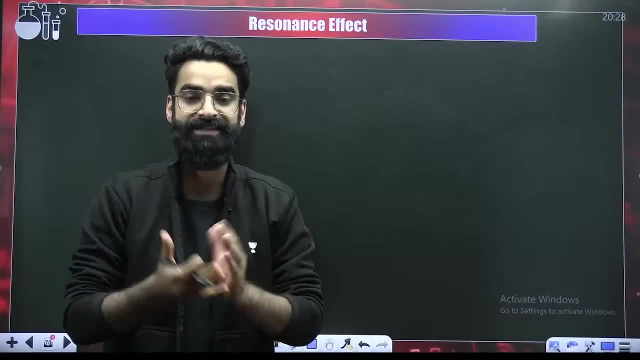 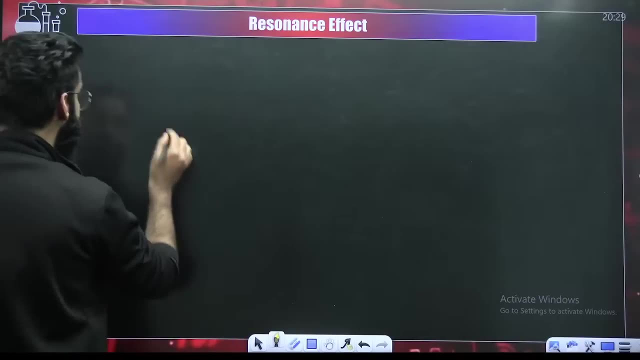 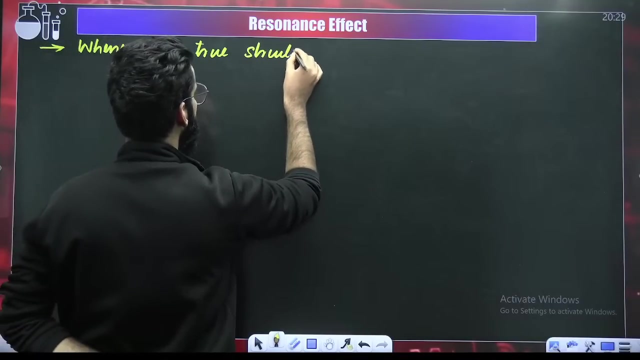 And after that I will let you know what this Resonance exactly is. My dear students, I am going to write one simple statement over here. try to understand. The statement is like this: Whenever a true structure, Whenever a true structure of a molecule cannot be shown, 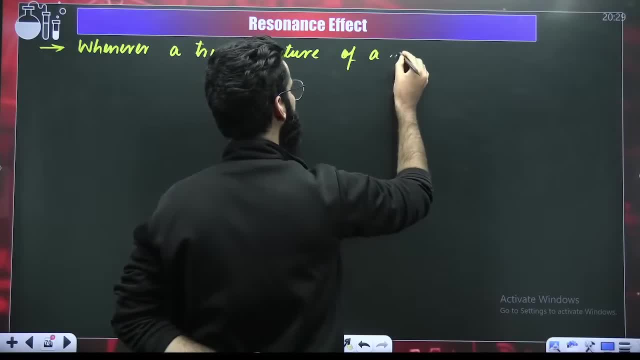 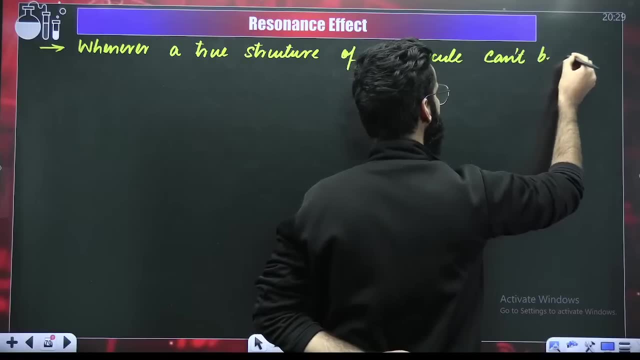 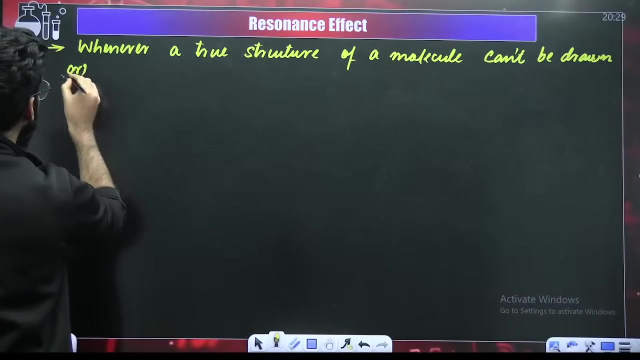 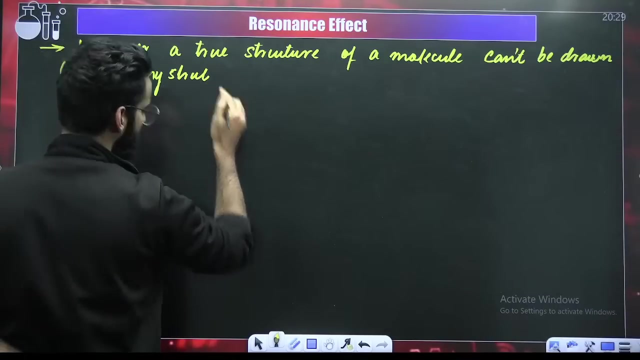 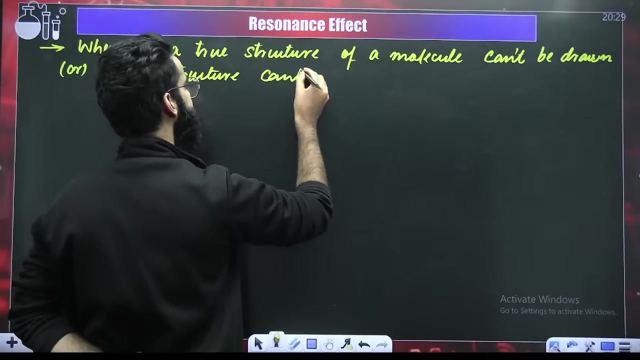 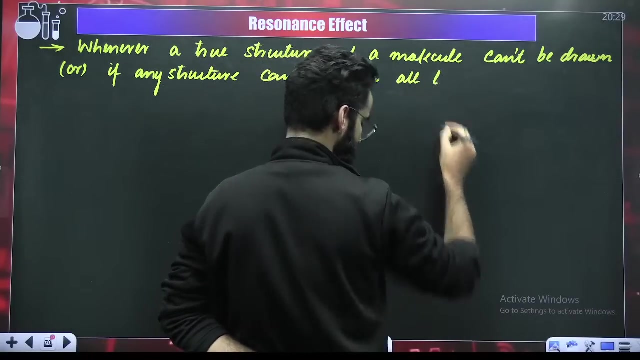 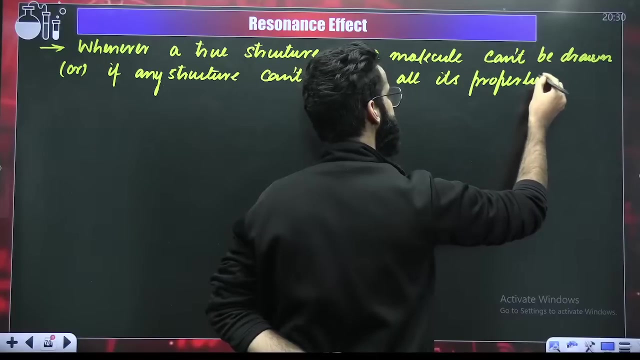 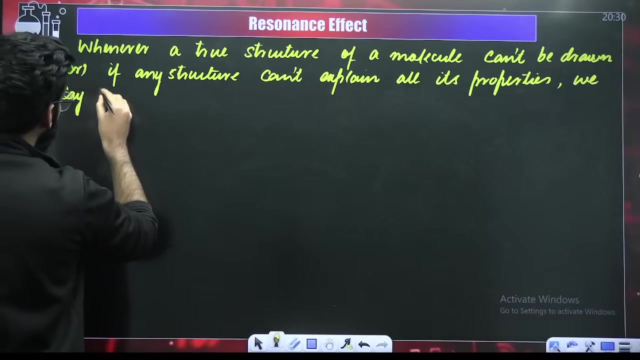 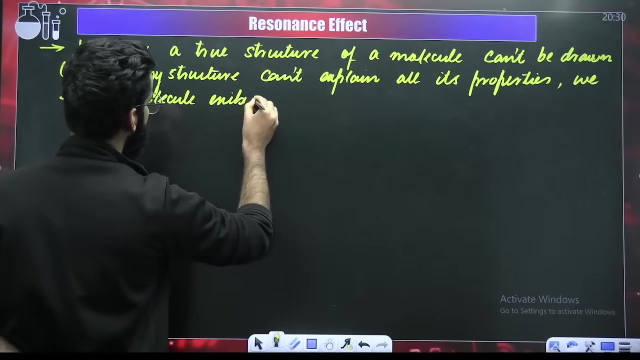 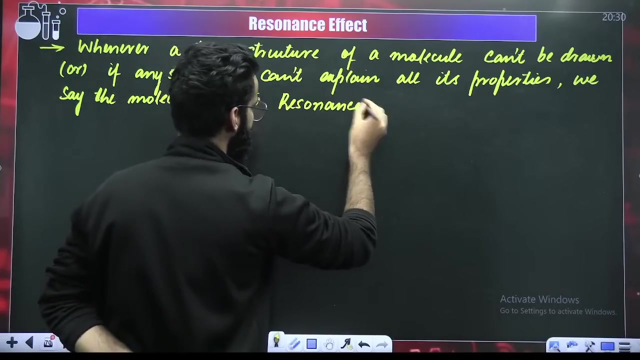 Okay, So whenever, Whenever A molecule cannot be drawn, whenever true structure of a molecule cannot be drawn, or if any structure cannot be drawn cannot explain all its properties, all its properties. but we say, we say the molecule exhibits resonance, We say a molecule exhibits resonance. 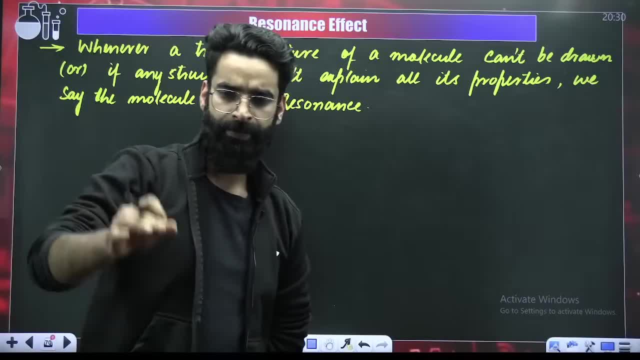 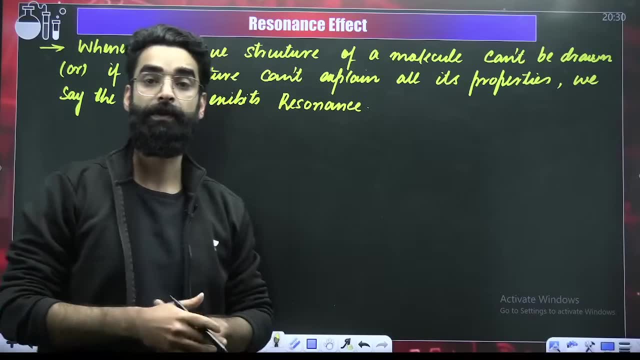 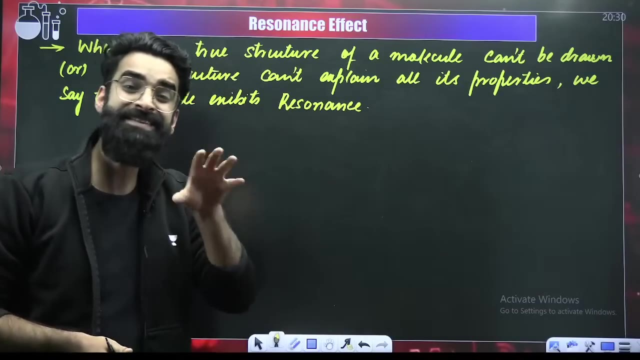 This is one very, very, very important point, My dear students. whenever you will be unable to draw true structure of the molecule, whenever you will be unable to draw the actual structure of the molecule, or if any structure of the molecule will not be able to explain all its properties, 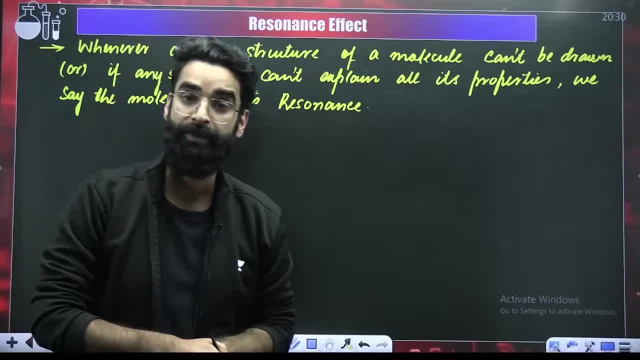 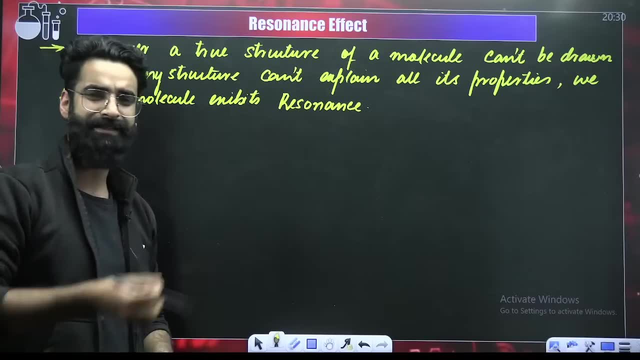 If any structure of the molecule will not be able to explain all its properties at that point of time, we say that the molecule exhibits resonance. Now, what is meant by it? Let's try to understand this a bit more in detail. Try to understand, guys. 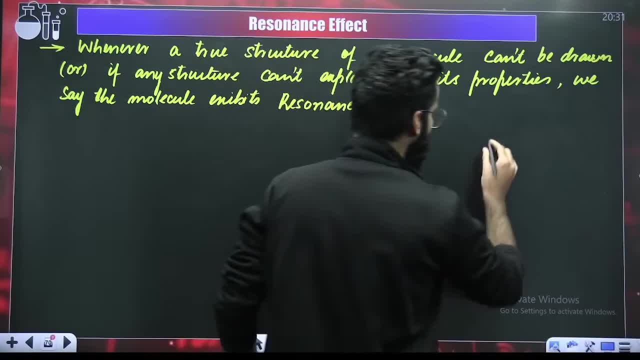 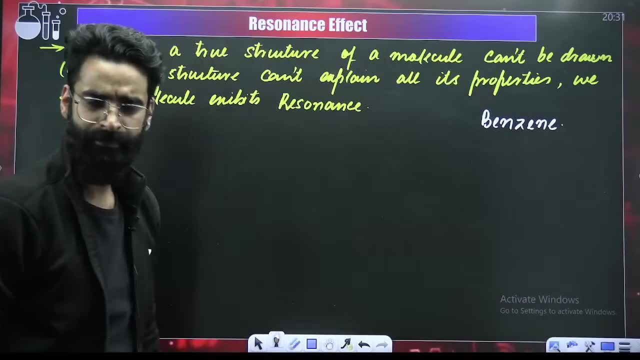 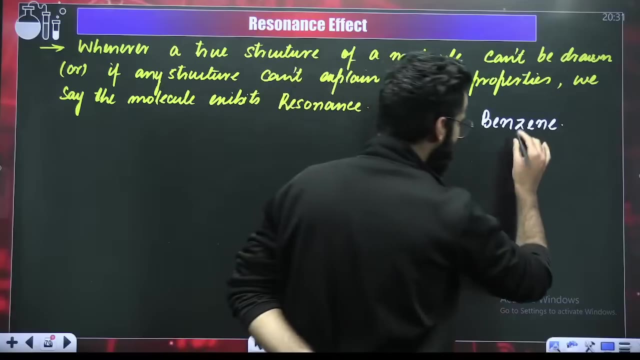 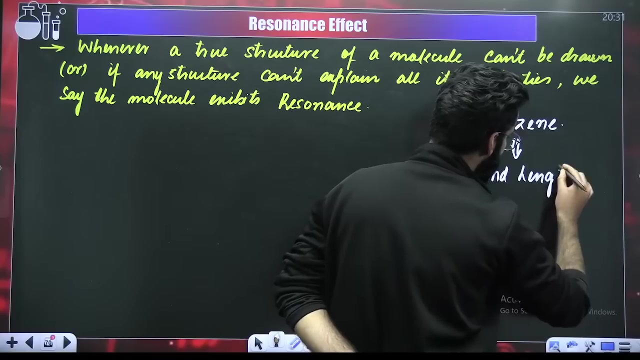 First of all, I'm sure every one of you would have come across the term benzene, right, Benzene. every one of you would be knowing. Now, my dear students, experimentally it has been observed. Experimentally It has been observed that in benzene all the bond lengths are equal. 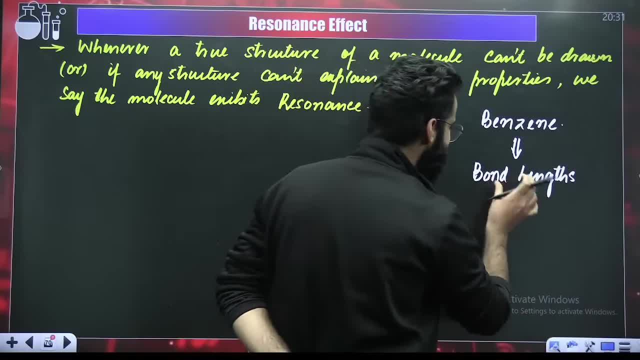 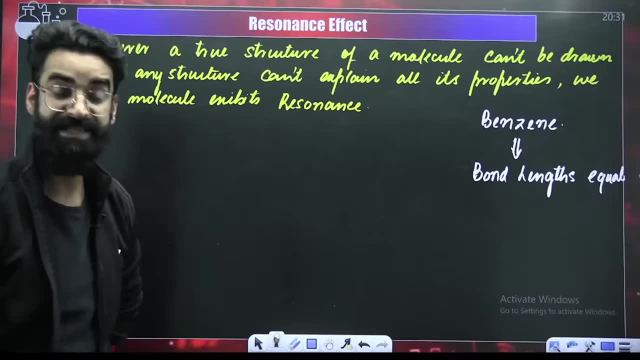 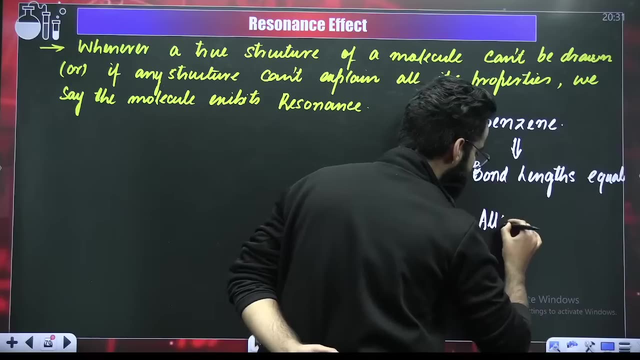 Experimentally it has been observed, in case of benzene, all the CC bond lengths are equal. All the carbon, carbon bond lengths are equal. This has been observed experimentally, Point number one. And at the same time it has been observed that benzene, it does not behave like a normal. 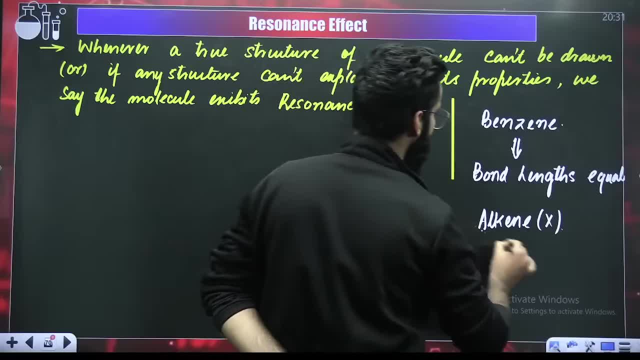 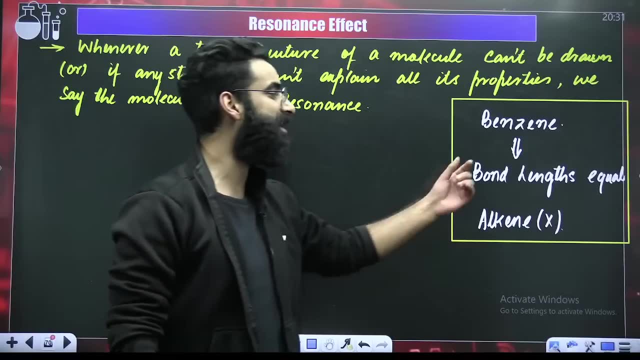 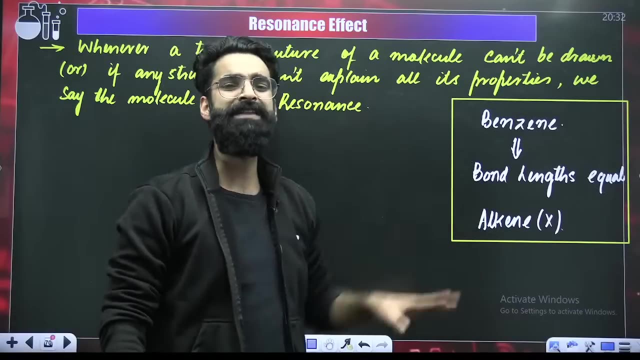 alkene. It has been observed that I mean it has been checked, my dear students- that in case of benzene, all the carbon, carbon bond lengths are equal. Experimentally it has been observed. And apart from that, it has been observed that in case of benzene, I mean benzene does. 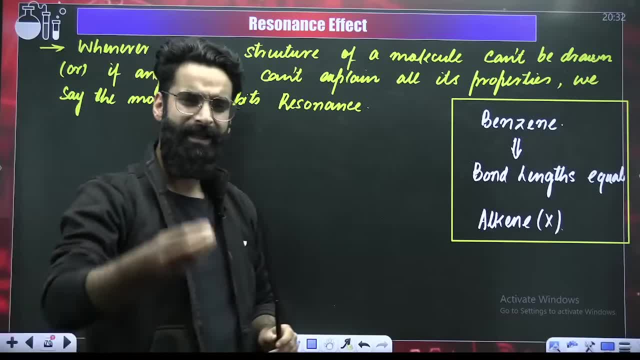 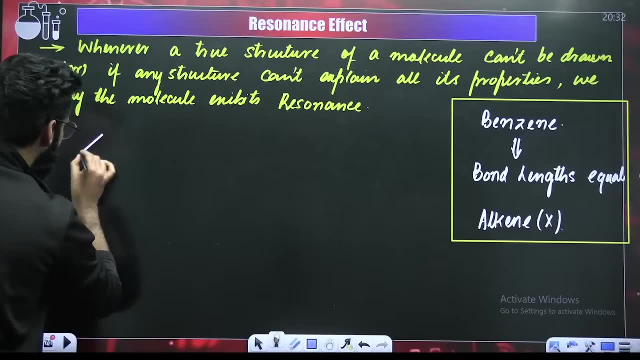 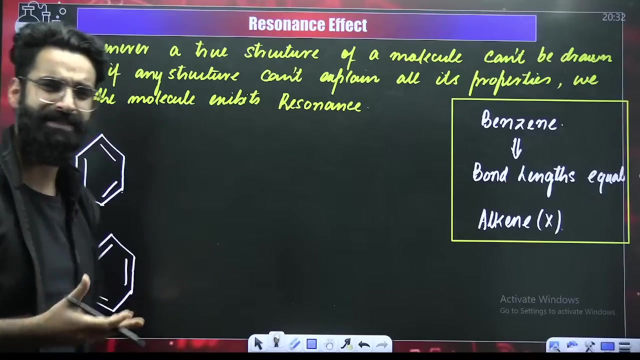 not behave like a normal alkene, correct? If I ask you, guys, what is the structure of benzene? some of you will come up with this particular structure. Some of you will come up with this particular structure. If I ask you what is the structure of benzene, some of you will say that is the structure. 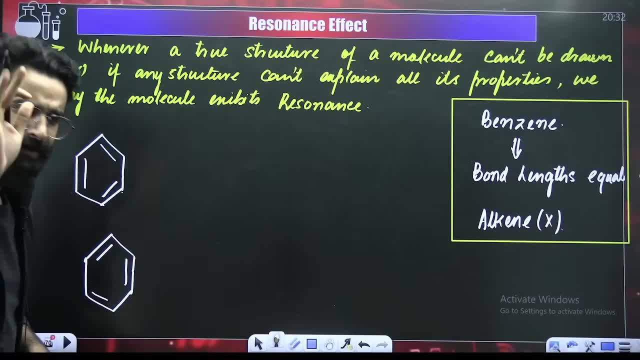 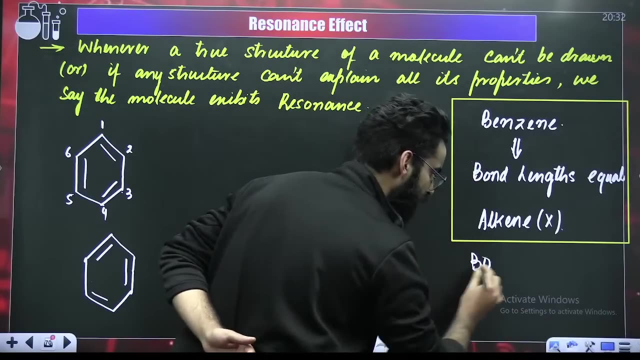 of benzene, and some of you will say: this is the structure of benzene. Now, my dear students, let me call this as carbon number one. let me call this is carbon number two. this is 4,, this is 5,, this is 6, right? Do you know one thing? That bond order is directly. 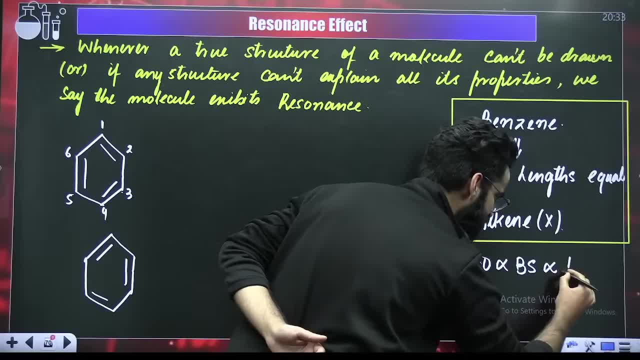 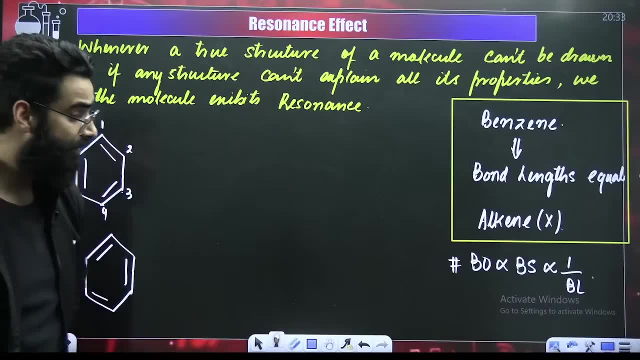 proportional to bond strength right, Which is inversely proportional to bond length. I believe every one of you will be knowing this Bond order is directly proportional to bond strength, which is inversely proportional to bond length. right Now, guys try to understand If you look. 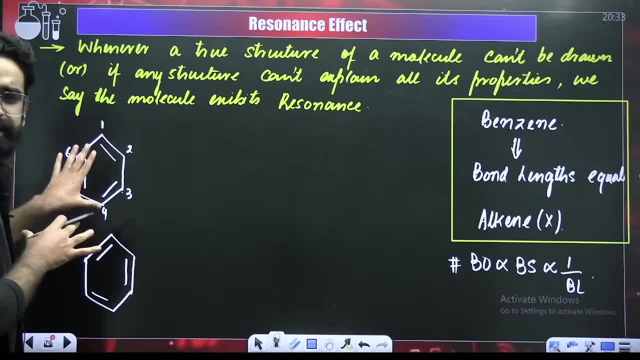 at this particular structure. this is the structure which you gave me about benzene, right? Some of you said this is the structure of benzene and some of you said this is the structure of benzene. If you look at the first structure, in the first structure there is a 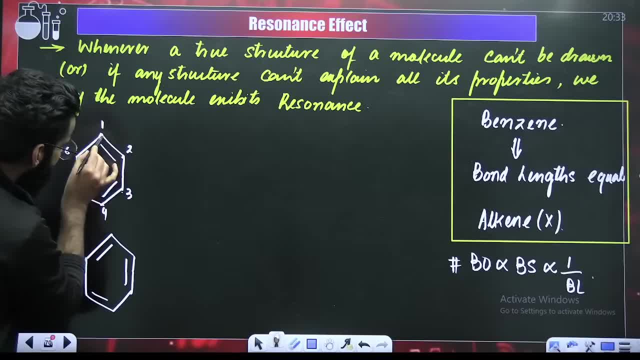 double bond between this carbon and this carbon. There is a double bond between this carbon and this carbon. So between carbon number 1 and carbon number 2, there is a double bond as per this particular structure. right Between carbon number 2 and carbon number 3, there is a single. 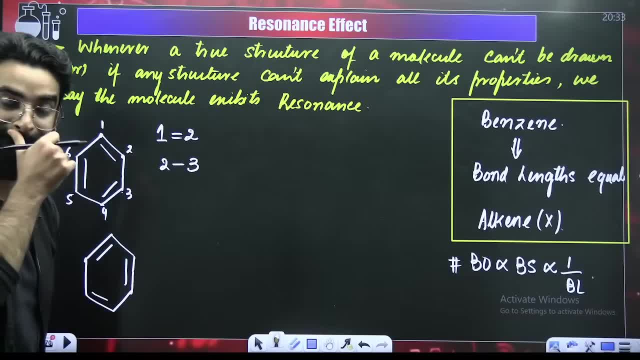 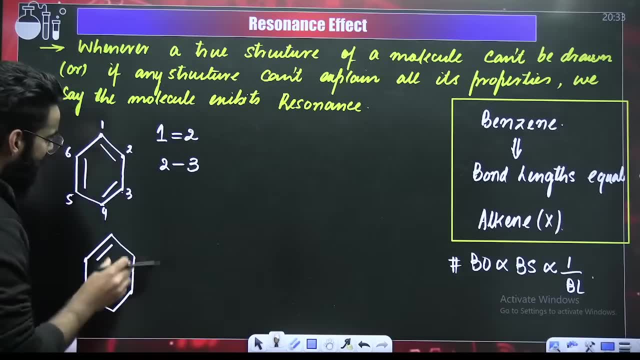 bond Between carbon number 2 and carbon number 3, there is a single bond. Now if I ask you, as per this particular structure, there is a double bond between these two. there is a single bond between these two. As per this structure, will this particular bond length and this particular bond 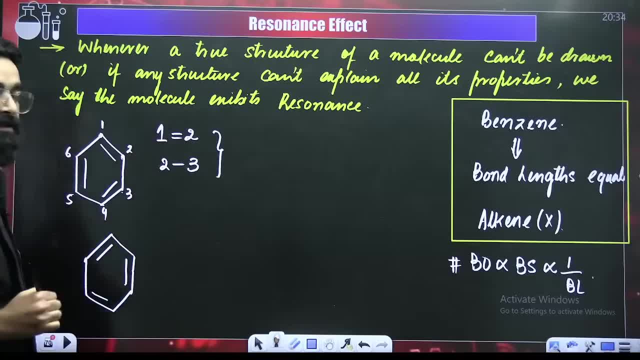 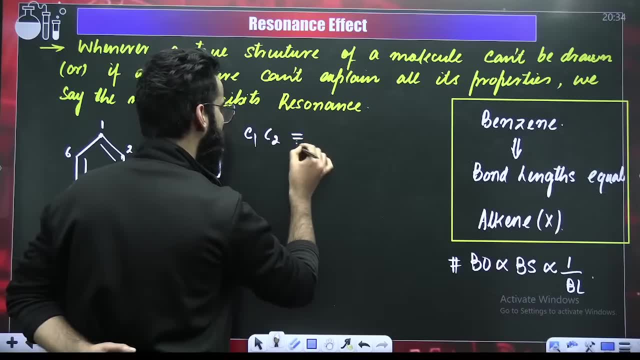 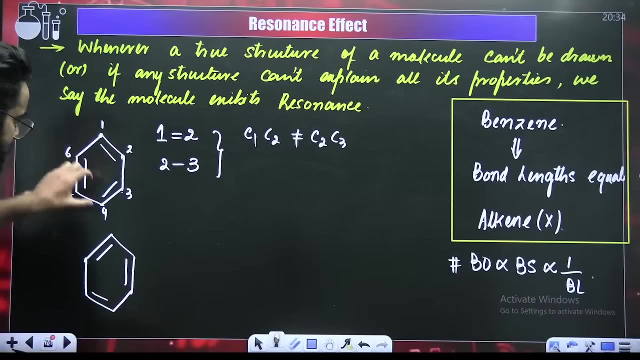 length. will these bond lengths be same or different? as per this structure, I'll say C1, C2.. C1, C2 bond length won't be equal to C2, C3 bond length. correct, Very simple, See, if you look at this particular structure. as per this structure, there is a double bond between 1 and 2, there is a single bond between 2 and 3.. 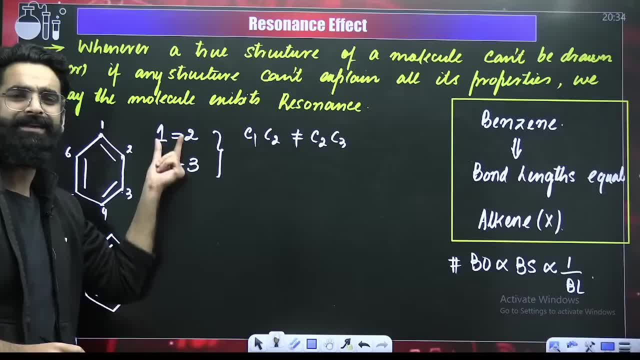 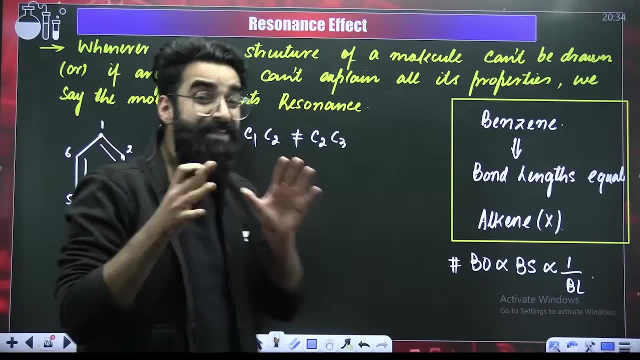 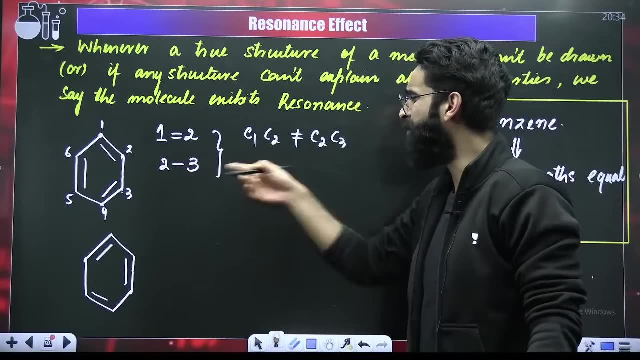 If there is a double bond and a single bond, definitely their bond lengths won't be equal, right? But my dear students, my dear students, already we know something about benzene. We know, in case of benzene, all the C-C bond lengths are equal. But as per this structure, C-C bond lengths are not coming out to be equal. 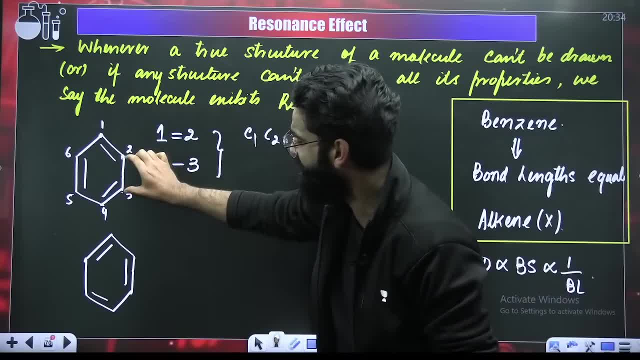 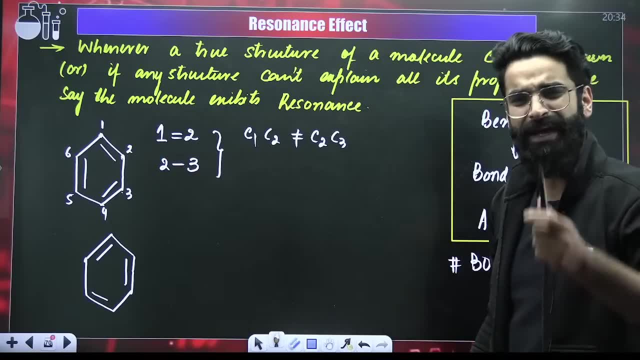 This bond length, as per this structure, will be less than C-C bond length, And this bond length, as per this structure, will be more right. So, as per this structure, the C-C bond lengths are not equal. So if I ask you, is this structure able to explain all the 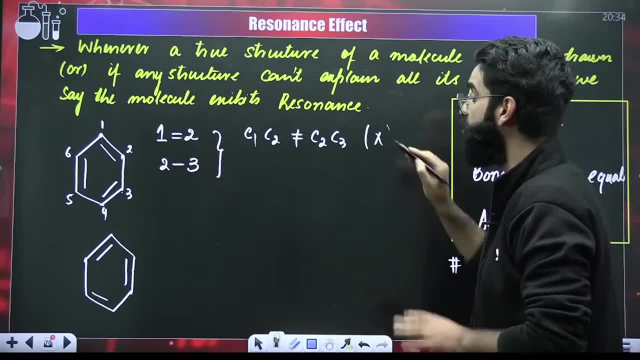 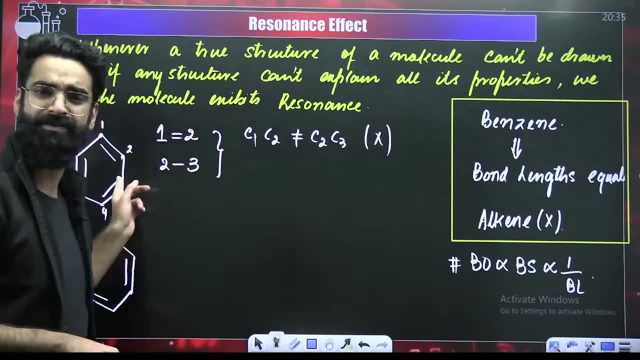 properties of benzene, You'll directly say no, This structure is not able to explain all the properties of benzene, Because we know, in case of benzene, all the C-C bond lengths are equal, But, as per this structure, C-C bond lengths are coming out to be different Because somewhere, 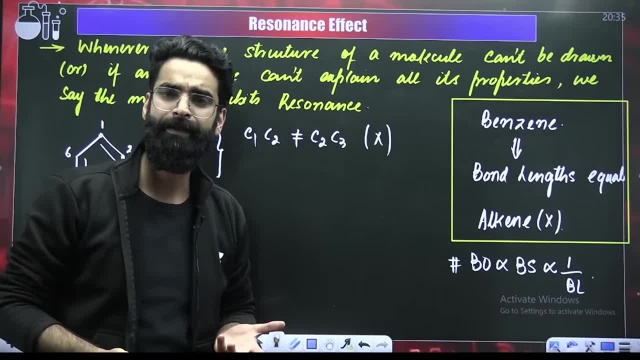 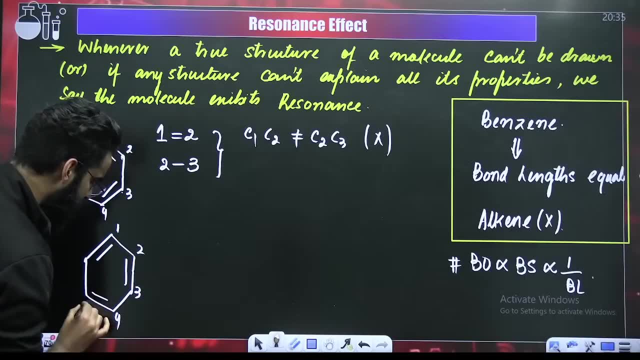 there is a double bond somewhere. there is a single bond right. Similarly, if you look at this particular structure, if you look at this particular structure, let me call this as 1,, let me call this as 2,, this is 3,, this is 4,, this is 5,, this is 6.. 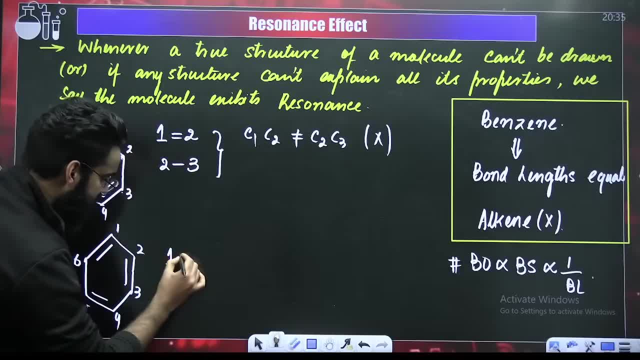 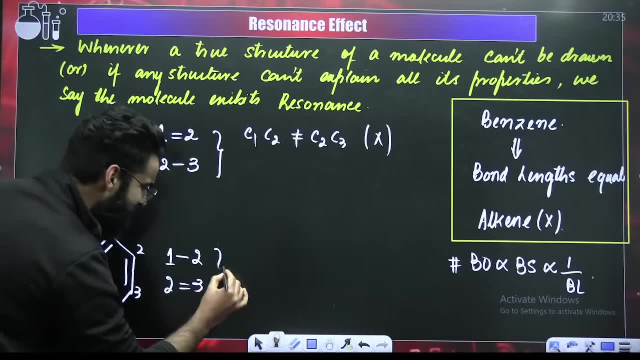 As per this structure, between 1 and 2,, between 1 and 2, there is a single bond right, And between 2 and 3, there is a double bond, perfect. So if I ask you, as per this, 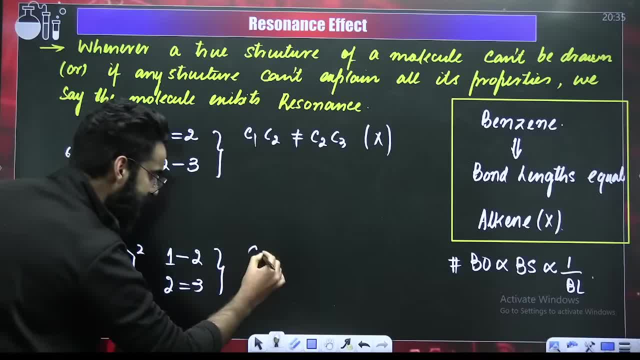 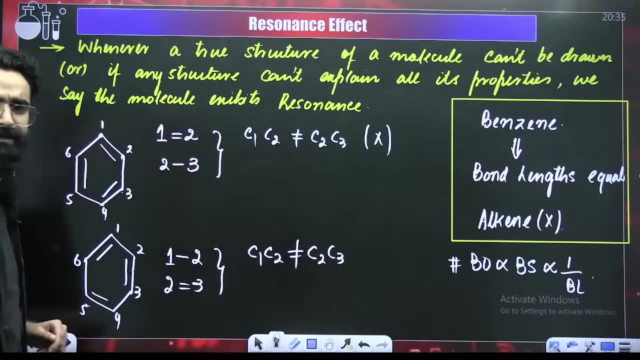 particular structure of benzene, will C1-C2 bond length? will C1-C2 bond length be same as that of C2-C3?? You'll say: no right, They won't be equal As per this particular structure. they won't be equal. 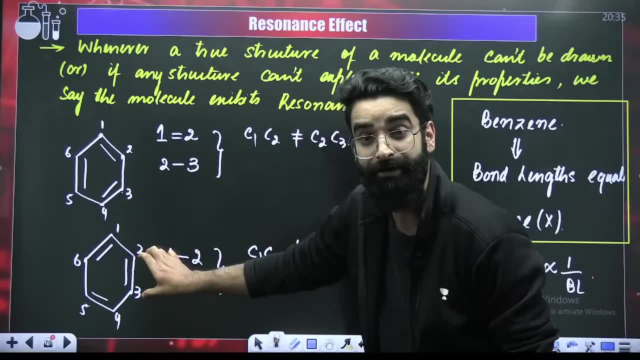 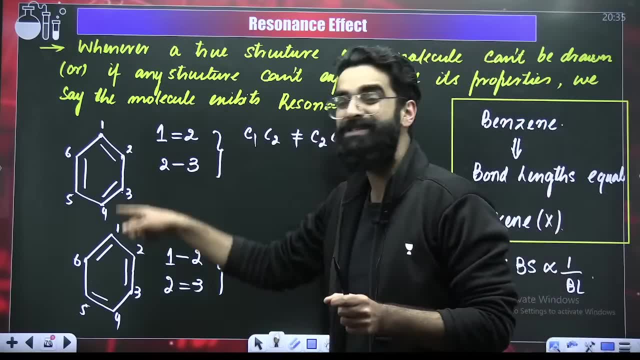 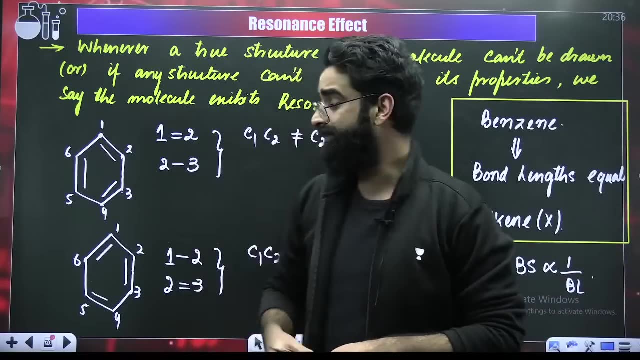 Perfect, Because, as per this structure, there is a single bond here, there is a double bond here. perfect, Right. So if I ask you, are these two structures able to explain all the properties of benzene? These structures are not able to explain all the properties of benzene, This particular structure. 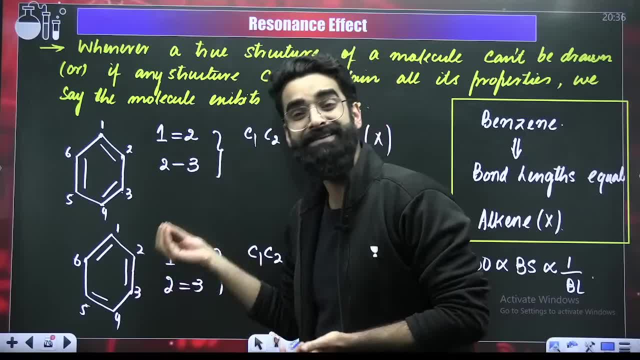 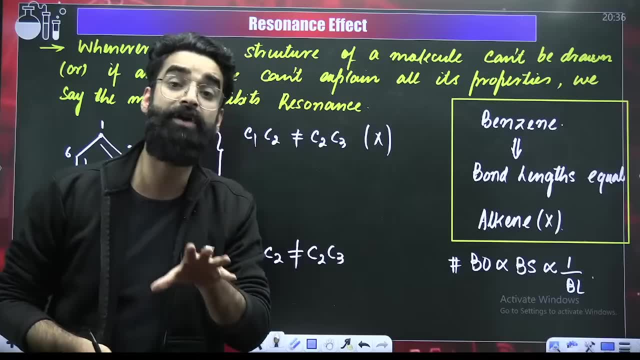 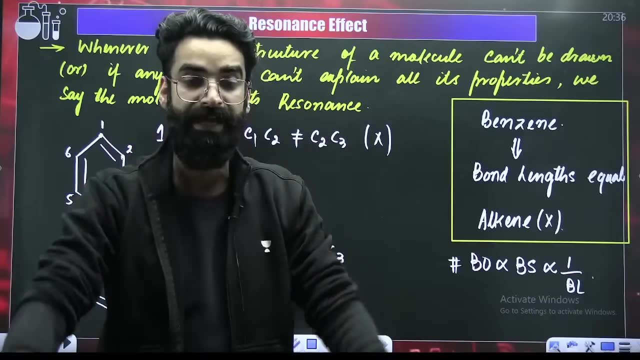 is not unable to explain all the properties. Even this particular structure is unable to explain all the properties of benzene. Whenever you cannot draw the true structure of the molecule, or if any structure will be unable to explain all the properties of the molecule, at that point of time we say the 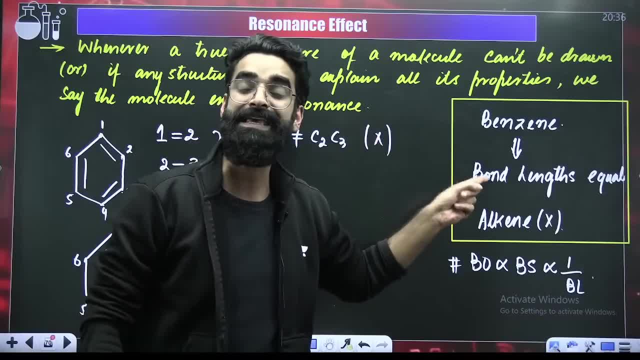 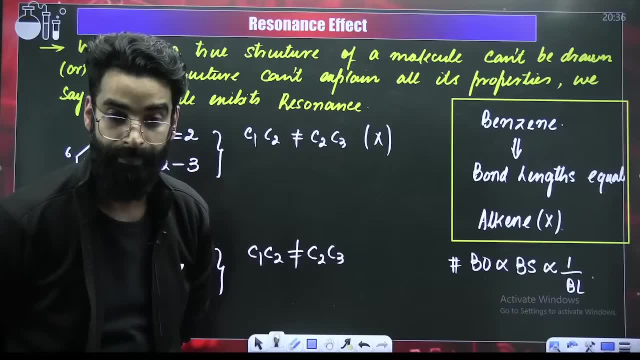 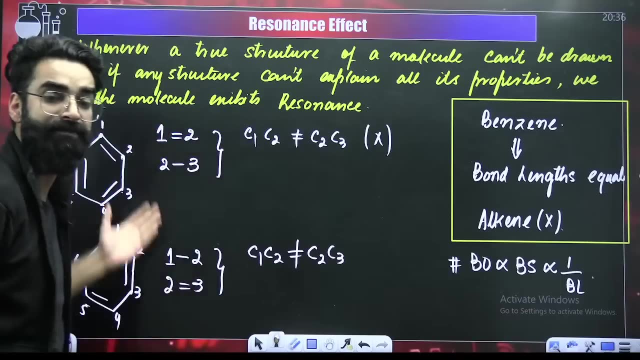 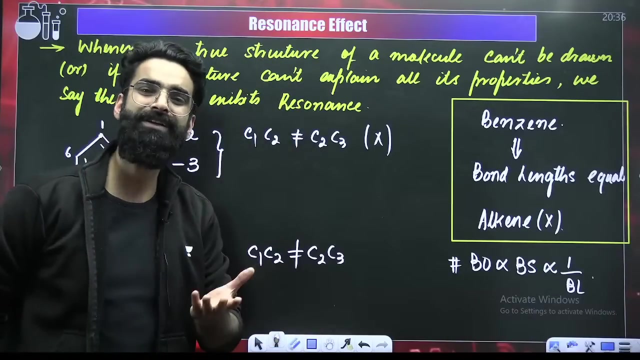 molecule exhibits resonance. So can I say: benzene will be exhibiting resonance Absolutely. benzene will be exhibiting resonance Absolutely. benzene will be exhibiting resonance Because none of the structures of benzene are able to explain all its properties. and any such molecule whose structure cannot explain all its properties, we say that molecule exhibits. 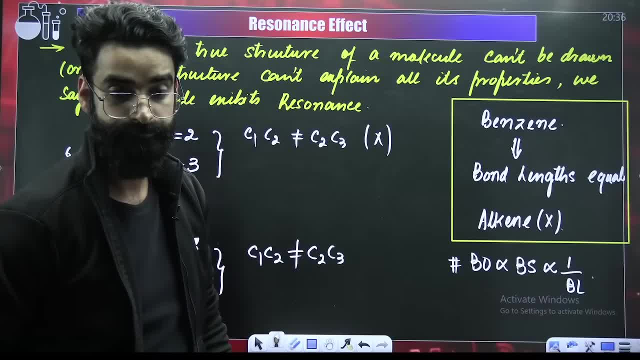 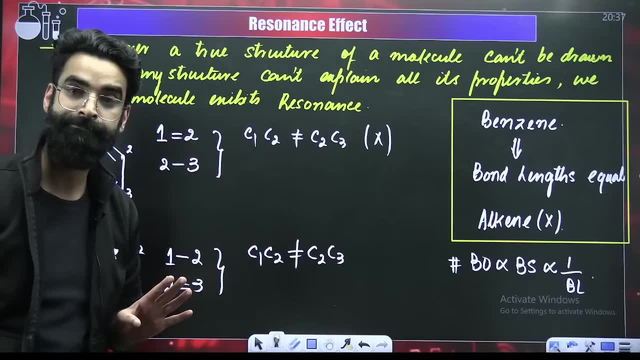 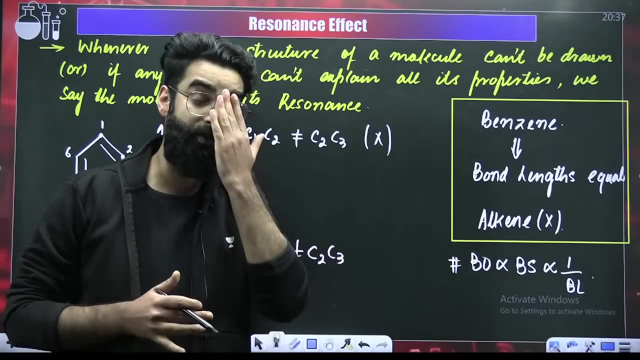 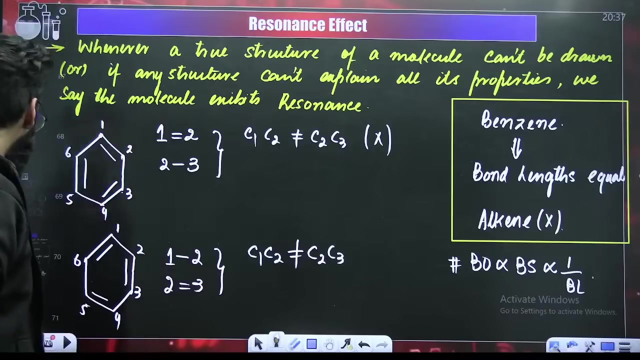 resonance. Okay, Clear guys. So benzene is the molecule which exhibits resonance. Perfect, Now, what this resonance exactly is all about. Before talking about resonance, There are few points which you need to know Before understanding what this resonance is. there are few things which you need to know. 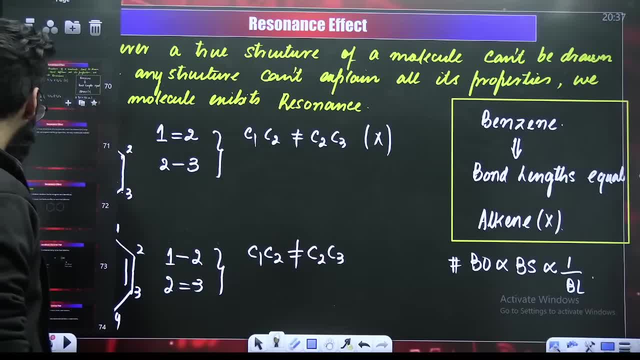 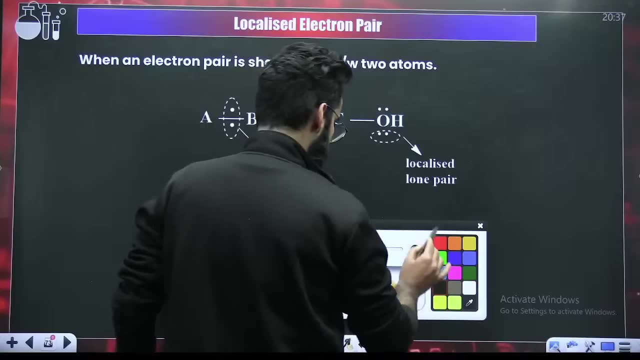 my dear students, Have a look exactly what those things exactly are. Have a look exactly what those things exactly are. Have a look, people. Just a second. Let me create a space over here. Let me create a space over here, Okay. 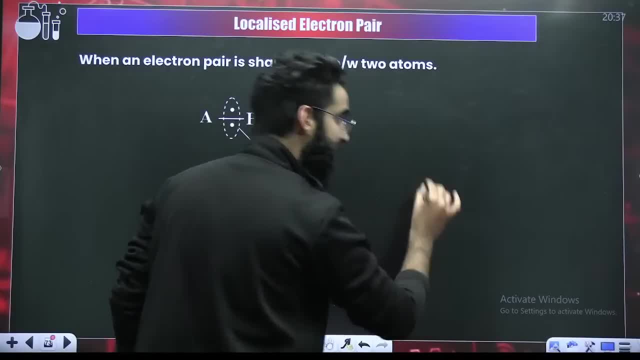 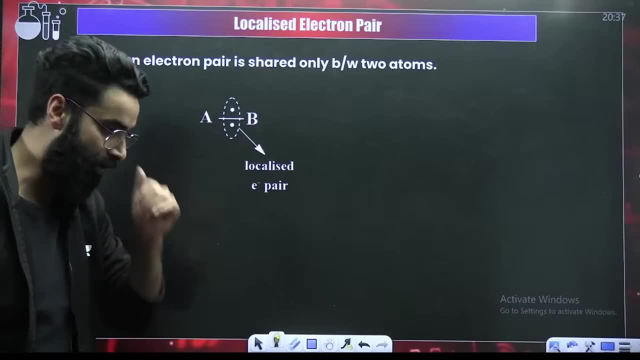 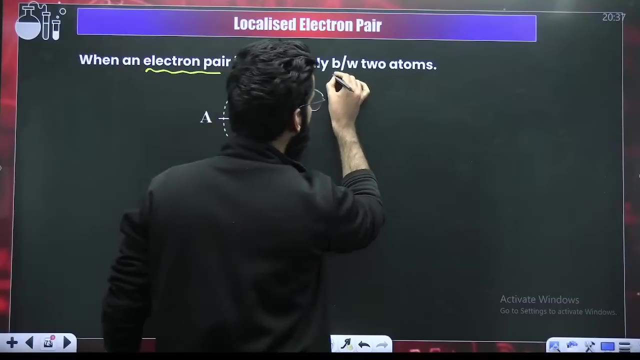 My dear students, in order to understand the term resonance, you should know first of all what is a localized electron pair. You should know first of all what is a localized electron pair And how do we define the localized electron pair When an electron pair is shared only between two atoms. 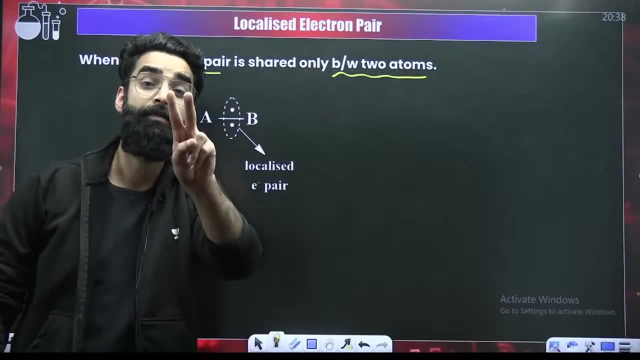 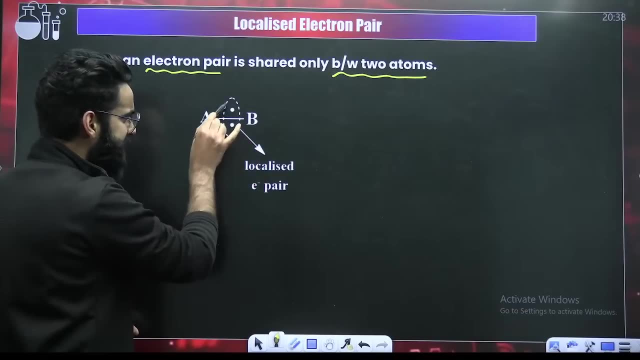 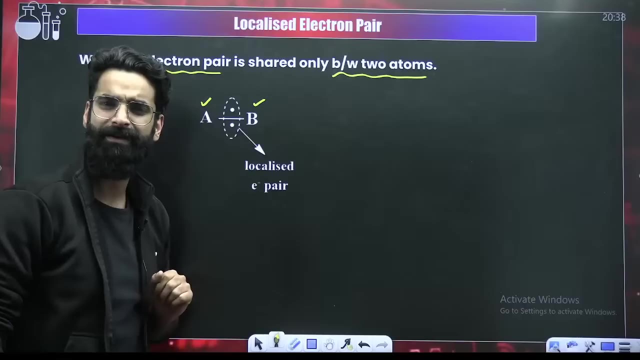 If an electron pair is just shared between two atoms, we call that particular electron pair as a localized electron pair. For example, This electron pair: It is just shared between A and B. This particular electron pair, It is just shared between A and B, Right. 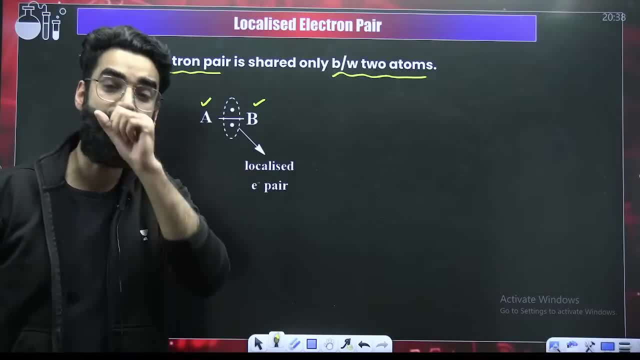 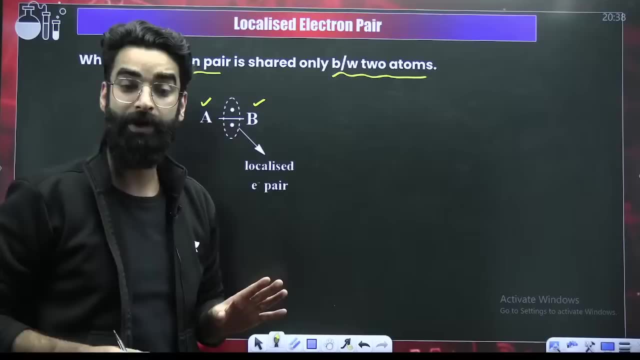 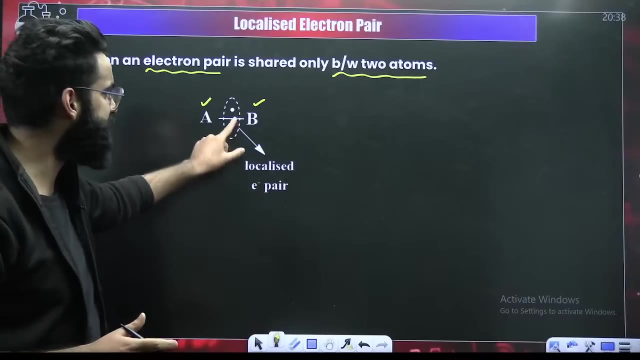 Any such electron pair which will be just shared between two atoms, you call that particular electron pair as the localized electron pair. You will be calling that as the localized electron pair. When the electron pair is shared by just two atoms, you will be calling that as the localized 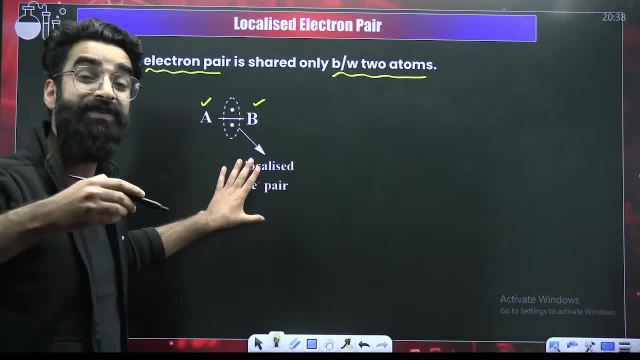 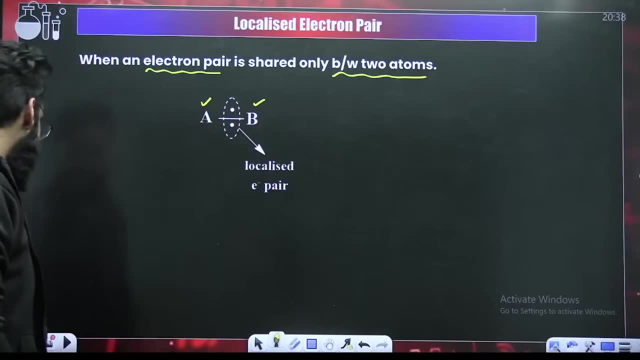 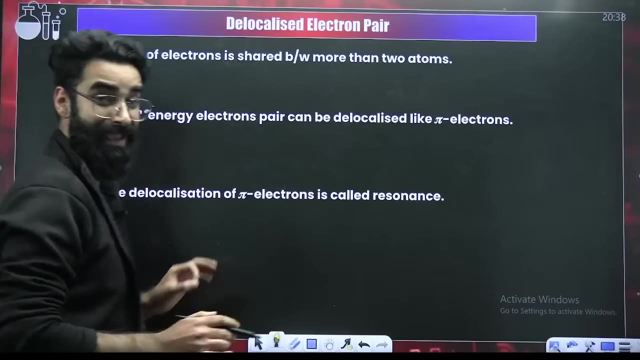 electron pair. Now, Right, What will be the meaning of delocalized electron pair? then, What will be the meaning of the localized electron pair, My dear students, any electron pair, Any electron pair which will be shared, any electron pair which will be shared between 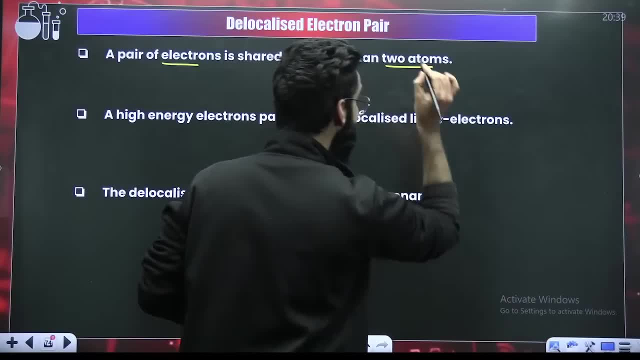 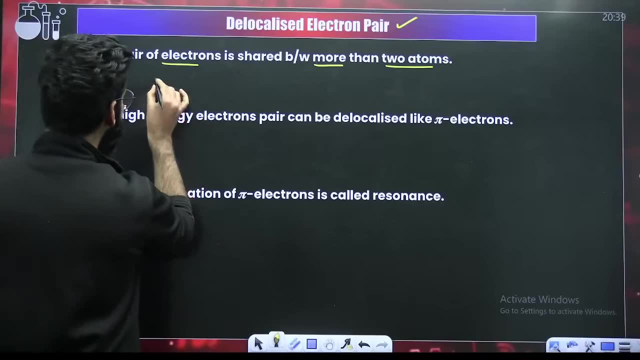 more than two atoms, any electron pair which will be shared between more than two atoms. That is what you will be calling as delocalized electron pair. For example, Let's say I've got a molecule, This is the molecule. Let's say: this is one more electron pair which I'm keeping between A and B. 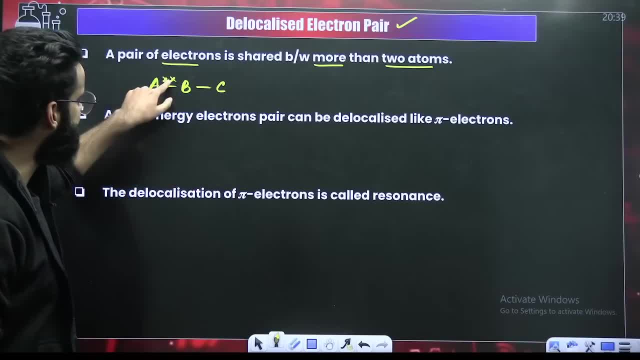 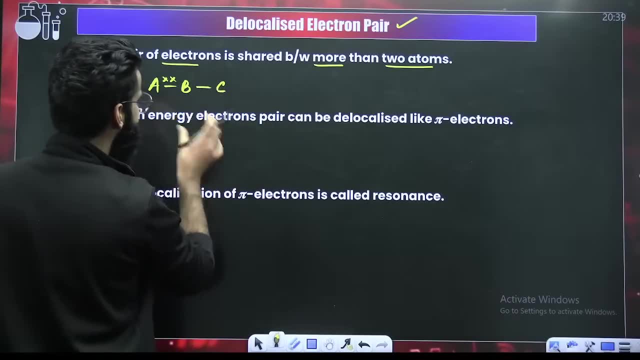 This is one molecule, right? This is one electron pair which I've kept between A and B, correct? Now, my dear students, for example, if I draw the structure of this molecule again, If I draw the structure of this molecule again, 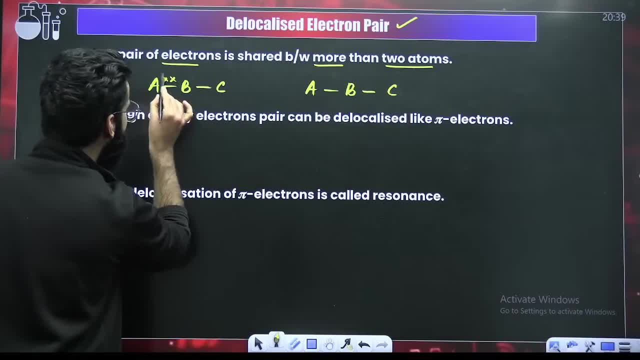 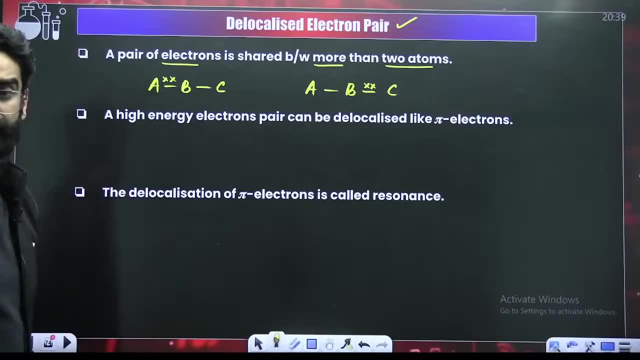 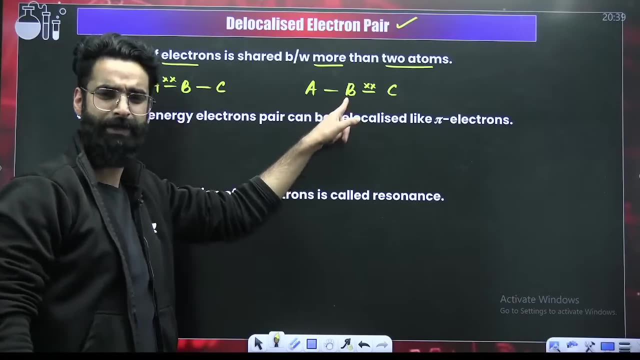 And by chance, if the same electron pair which was earlier between A and B, Now if the same electron pair is between B and C. Earlier this electron pair, which I'm representing by cross, it was between A and B. Now in one more structure of the same molecule, 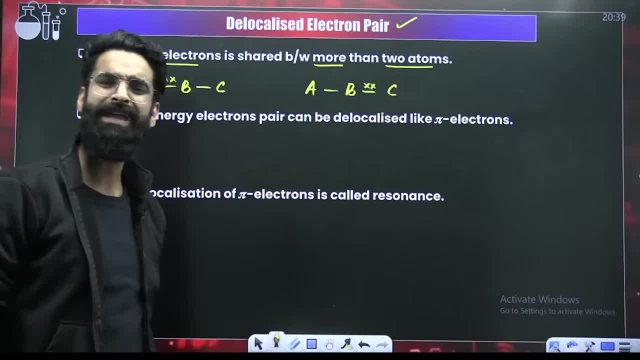 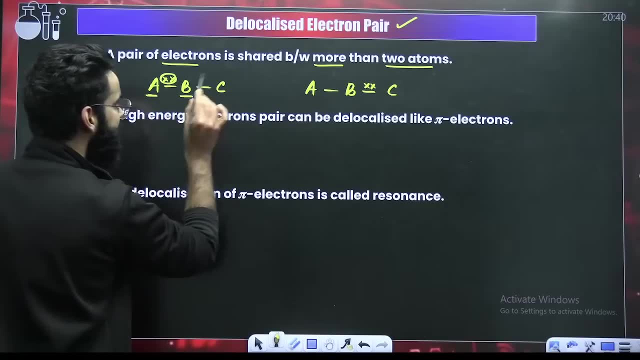 In one more structure of the same molecule, the same electron pair is between B and C. So the first structure is telling you that this particular electron pair is shared between A and B. The second structure is telling you That the same electron pair is shared between B and C. 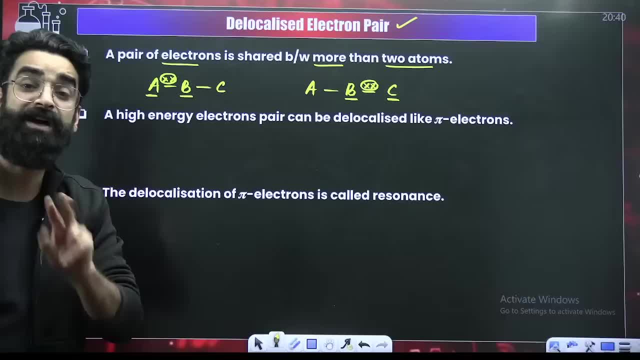 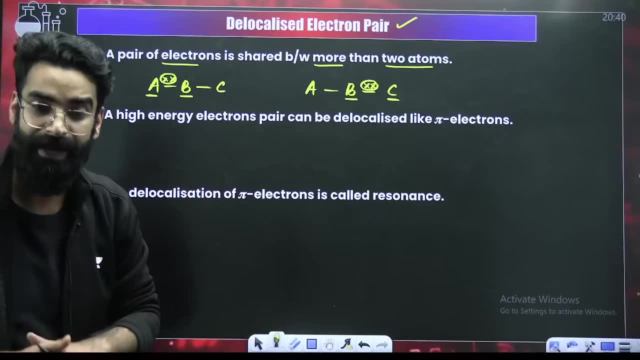 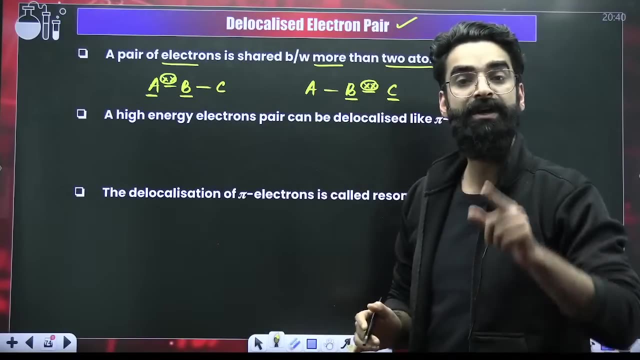 Now tell me whether this electron pair is shared by two atoms or three atoms. I'll say this particular electron pair is shared among three atoms. Any such electron pair which will be shared, which will be shared by more than two atoms, You call that particular electron pair as delocalized electron pair. 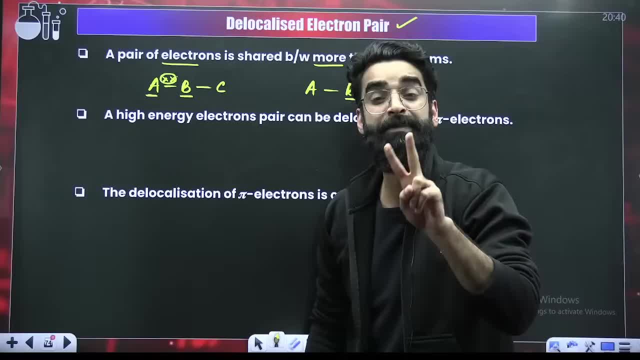 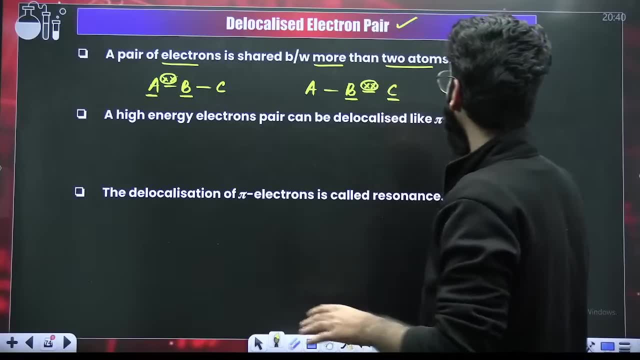 So this particular electron pair which we have, it is not shared only between two atoms, It is shared between three atoms. And any such electron pair which will be shared by more than two atoms, You call that electron pair as the delocalized electron pair. 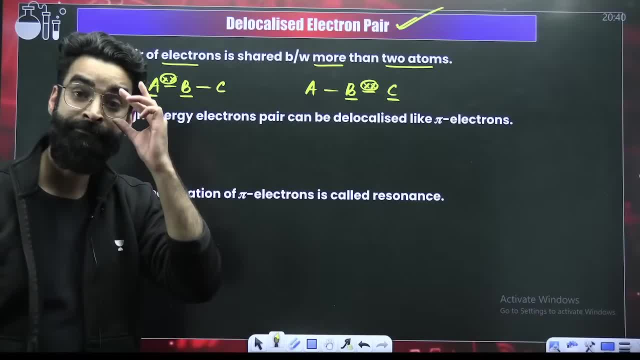 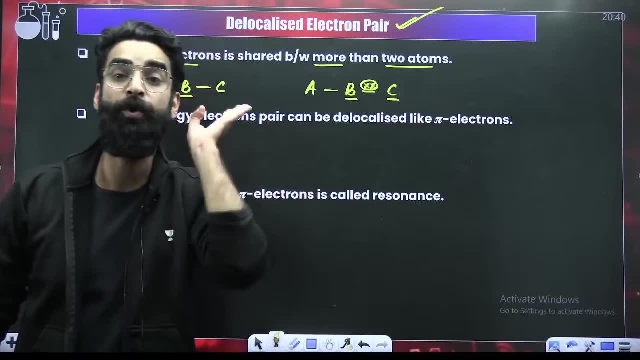 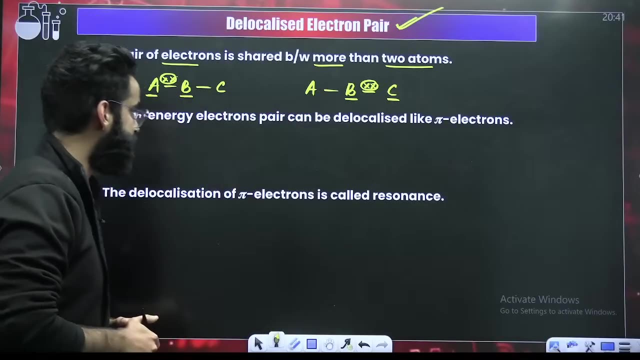 Correct Right Now. my dear students, the point is Which electron pair will be called as delocalized electron pair. The point is Which electron pair will be called as delocalized electron pair. A simple and basic question. Simple and basic statement. 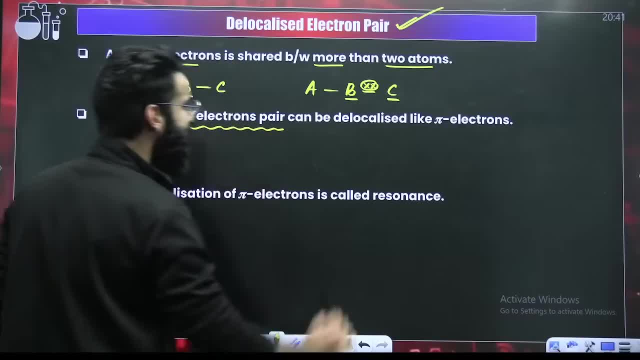 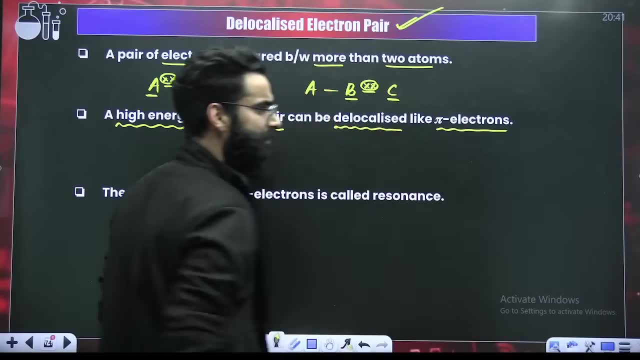 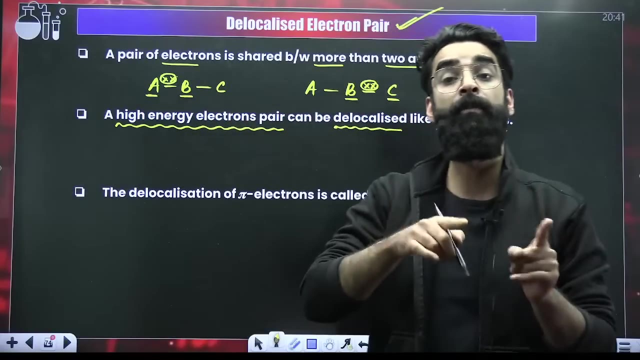 A high energy electron. A high energy electron pair can be considered as delocalized, like your pi electrons. Now, what is meant by this statement? Since I told you, delocalized electron pair is that electron pair which is shared between more than two atoms. 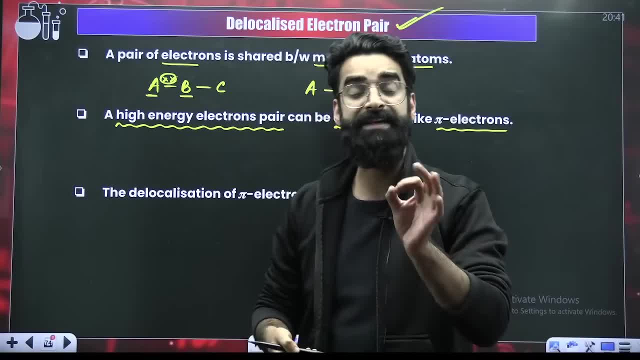 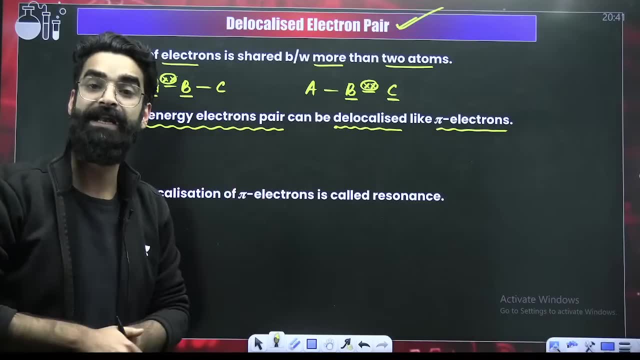 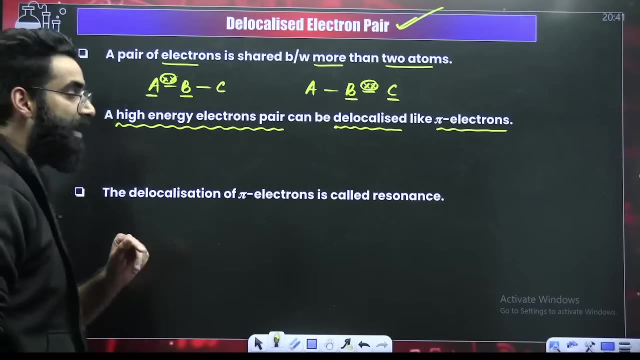 Now which electron pair can be delocalized. My dear students, over here it is mentioned High energy electron pair can be delocalized. Now, what is high energy electron pair? You must be thinking what is high energy electron pair? Let me tell you first of all what is high energy electron pair. 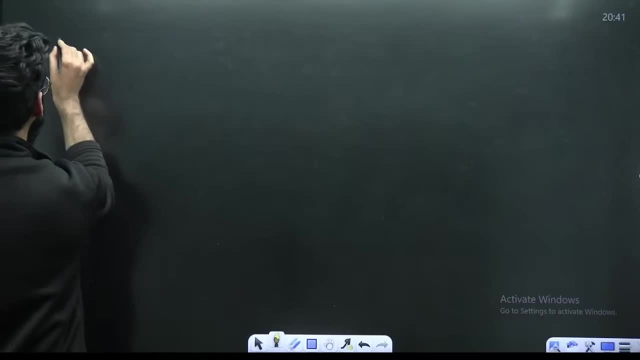 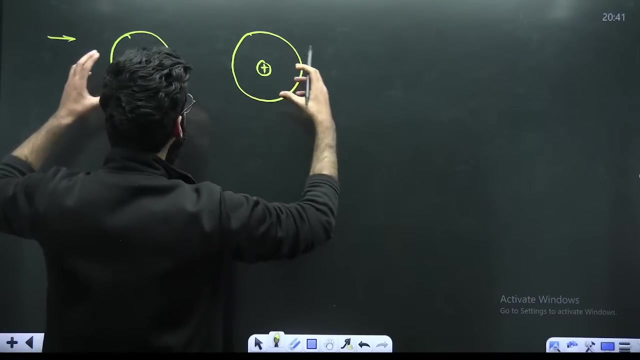 Try to understand exactly what is high energy electron pair. Have a look, For example. imagine This is an s orbital of one atom. Imagine this is s orbital of one more atom. Right Now, my dear students, when these atomic orbitals will approach each other? 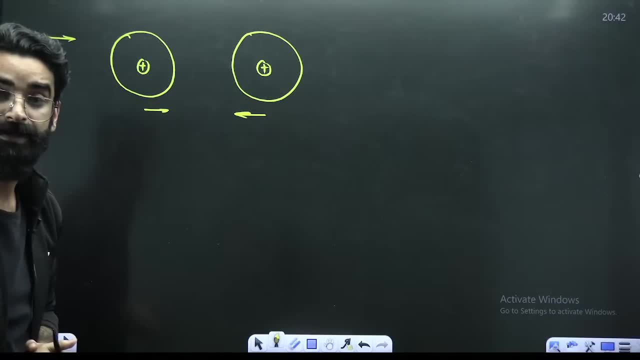 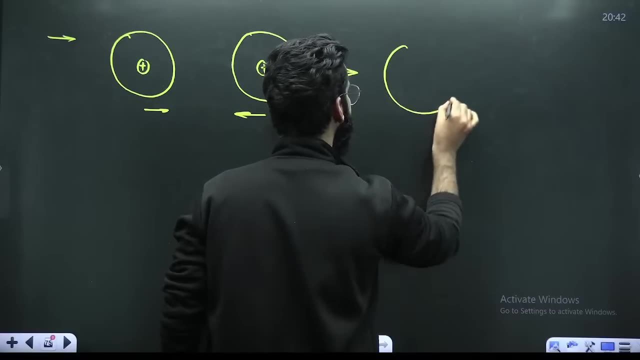 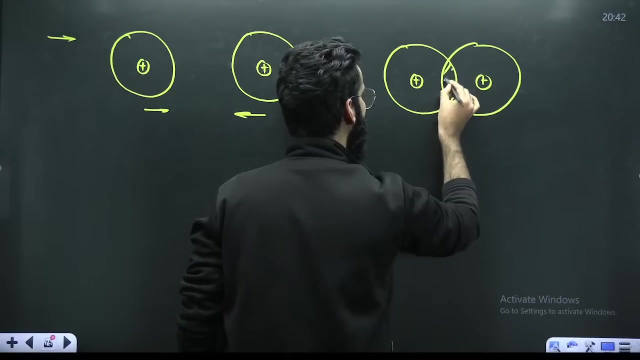 When these atomic orbitals will approach each other, what will happen? Will there be axial overlapping? Will there be head-on overlapping? Absolutely there will be head-on overlapping. Absolutely there will be head-on overlapping Right. And due to head-on overlapping, which bond is formed? 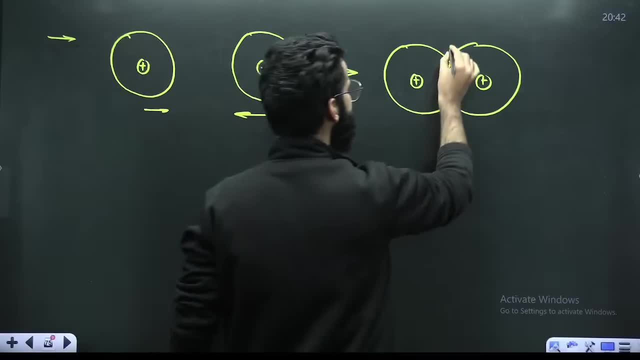 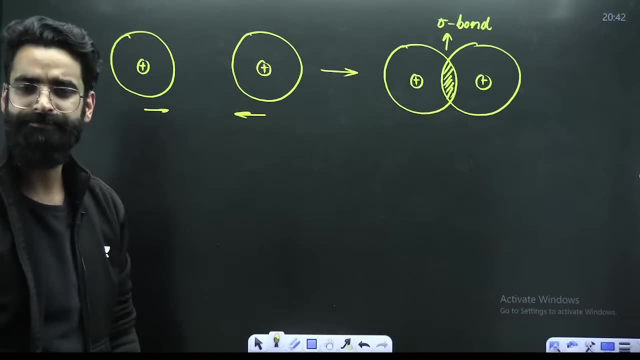 It is the sigma bond which gets formed due to head-on overlapping. So this particular bond which got formed here by the axial overlapping, this particular bond I am calling as sigma bond. Correct, That's something which I call as sigma bond. Now you tell me one thing. 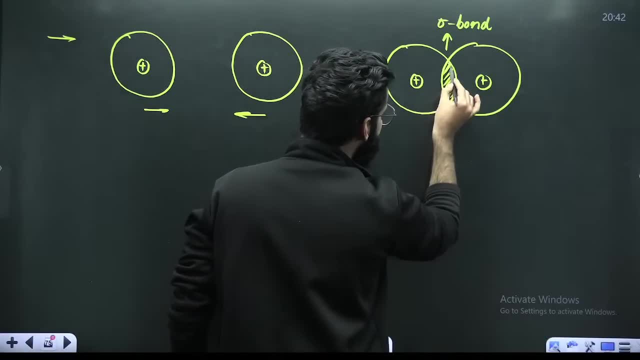 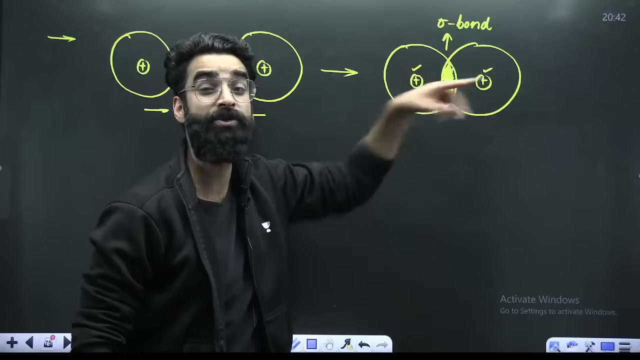 The sigma bond which gets formed over here, right? This particular common electron density, can I say this particular common electron density? it is under the influence of both these nuclei directly. This particular electron density is under the influence of both these nuclei directly. 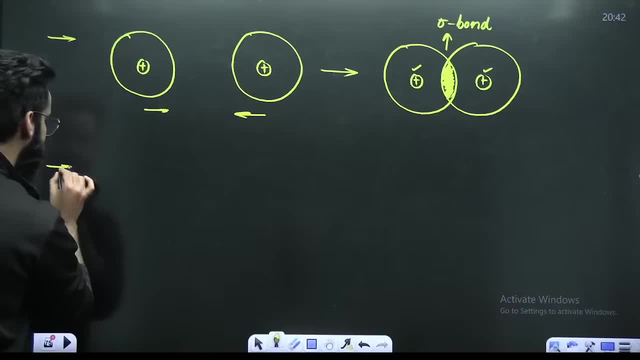 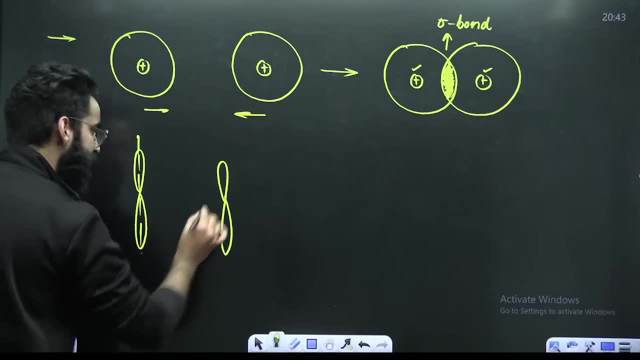 Right Now. now try to understand one more thing. Let's say: this is your p-orbital, This is one more p-orbital. I am keeping their axes parallel. If I keep their axes parallel, tell me, will there be axial overlapping or parallel overlapping? 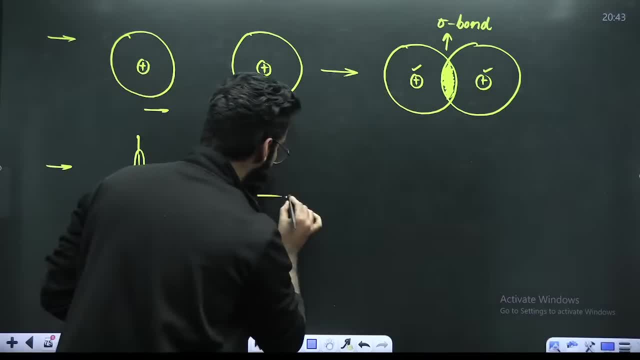 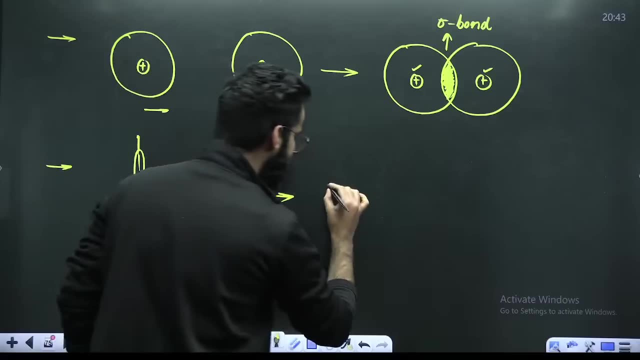 There will be parallel overlapping And, due to parallel overlapping, which bond gets formed? Pi bond gets formed. So what will happen, These lobes? they will bend towards each other and there will be parallel overlapping, Right? So this is your p-orbital and this is your one more p-orbital. 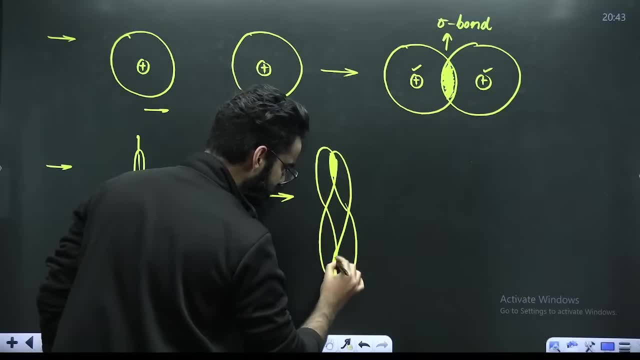 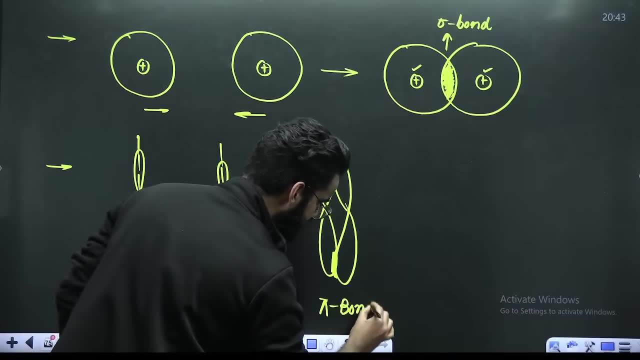 And this particular electron density, right, This common electron density. it results in the formation of what It results in, the formation of pi bond. Perfect. Now how do I make it at the end? Try to understand. This is the nucleus. 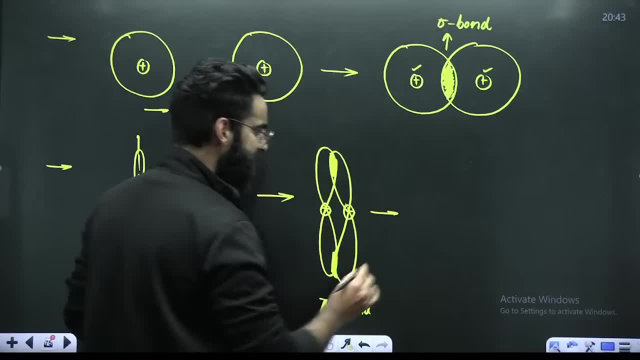 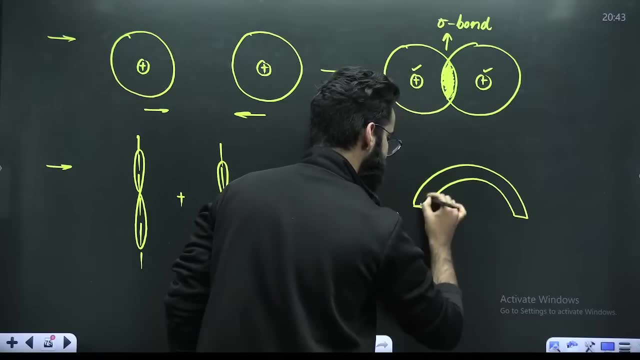 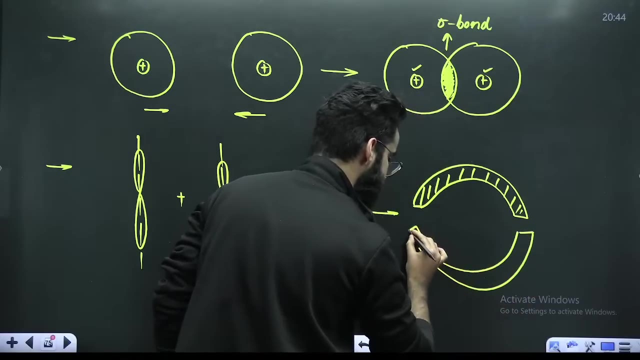 Even here you have got the nucleus Perfect. So let me make it like this. Let me make it like this: This is the common electron density at the top. This is the common electron density at the bottom. This is the electron density here. 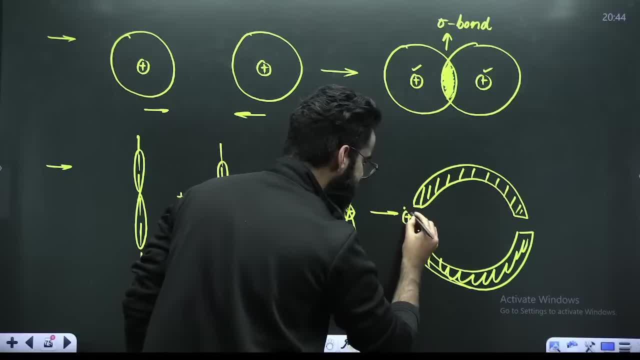 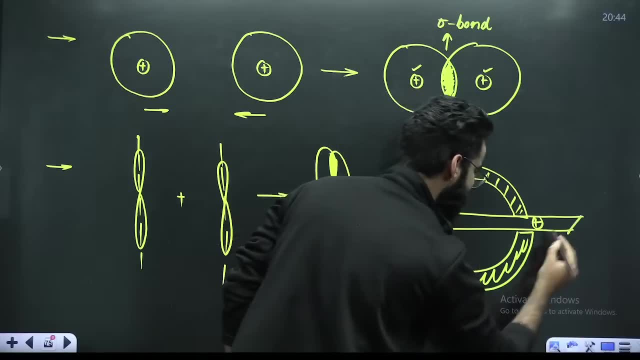 Right, This is the nucleus, This is the nucleus. So in between, I would say, over here there will be a plane, Over here there will be a plane on which electron density won't exist, and you call this particular plane as nodal plane. 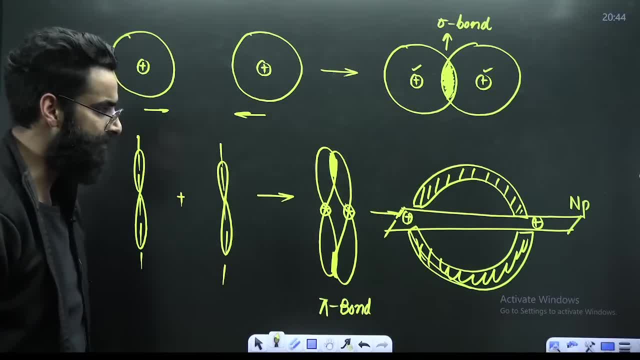 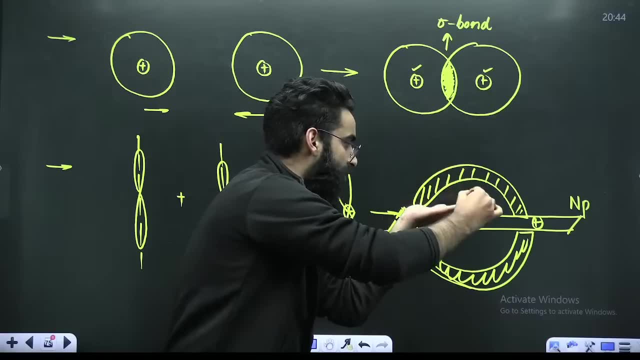 I hope you know that Right Now, my dear students, just tell me: just compare these two. Just compare these two. This is a plane on which no electron density lies. Electron density lies on the top and below the plane. Electron density lies above the plane and below the plane. 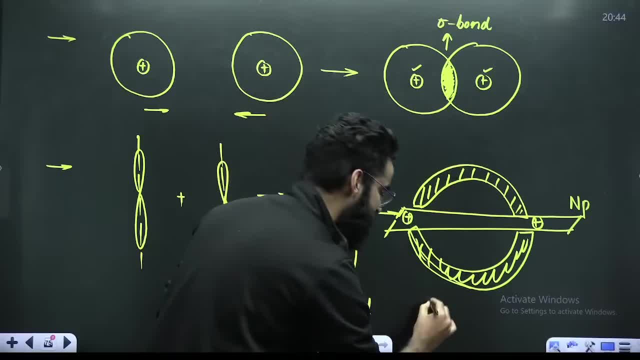 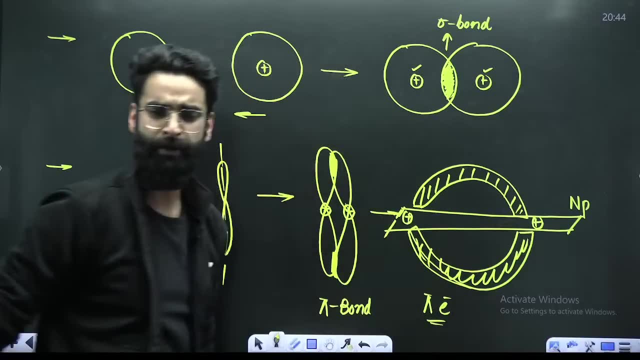 Correct. Now tell me whether this electron density, which you call as pi electron density, Right, Whether this electron density, whether this electron density, is under the direct influence of nucleus. Here, the electron density is not under the direct influence of the nucleus. 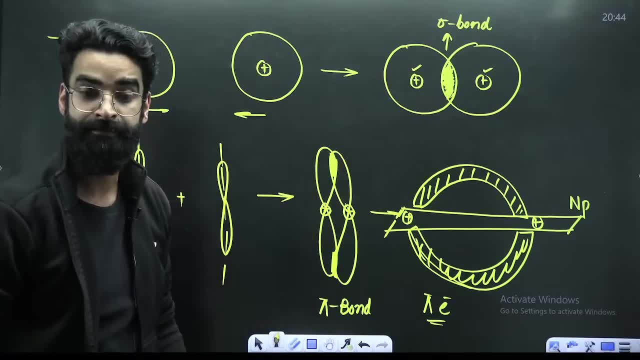 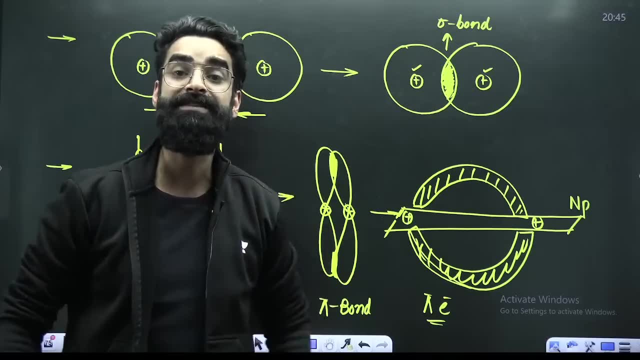 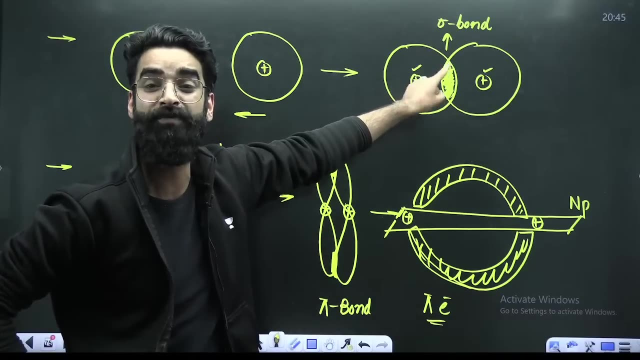 Here the electron density was under the direct influence of the nucleus. Now tell me which electron density among these two, Sigma electron density or pi electron density- Which electron density will be experiencing more force of attraction by the nucleus. Can I say this electron density will be experiencing more force of attraction. 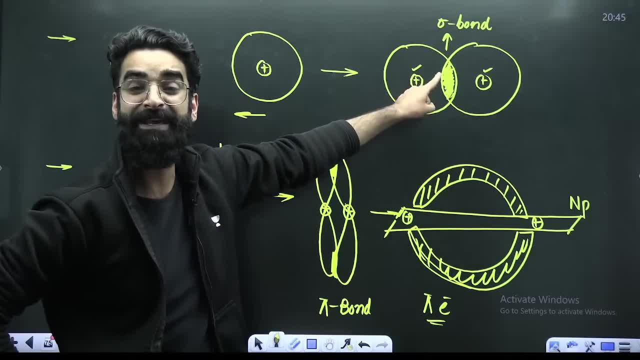 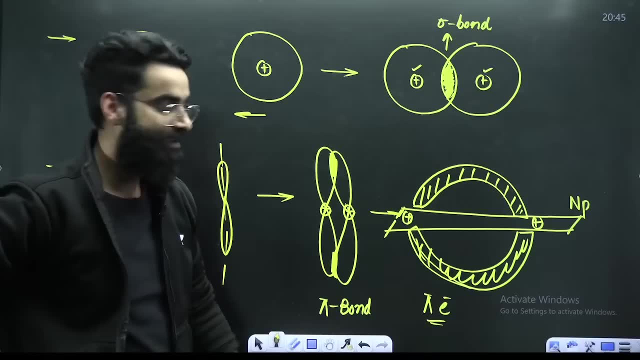 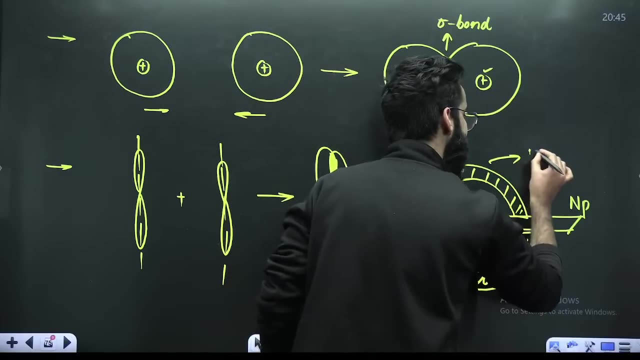 Can I say this particular electron density will be experiencing more force of attraction by the nucleus because it is under the direct influence of these nucleus. Right, Can I say this electron density, This pi electron density, it is under less force of attraction, It is subjugated to less force of attraction. 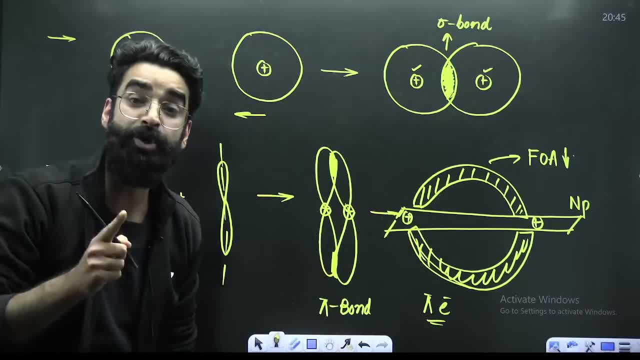 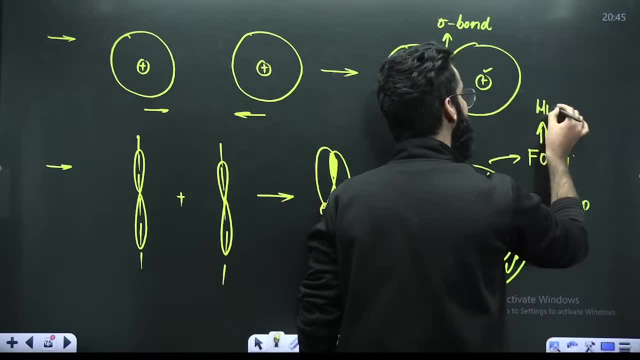 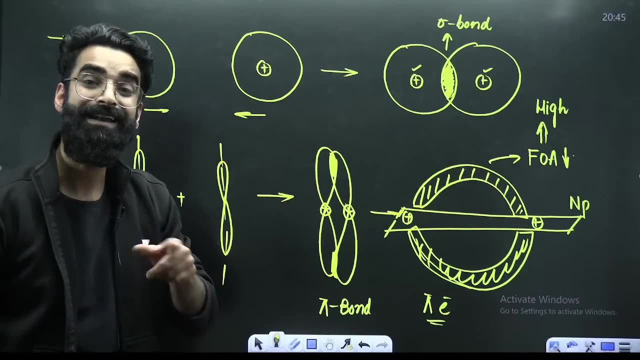 That electron density which is subjugated to less force of attraction. that electron density is something which you call as high Right. That electrons, those electrons which are under less force of attraction by the nucleus, which are subjected to less force of attraction by the nucleus, 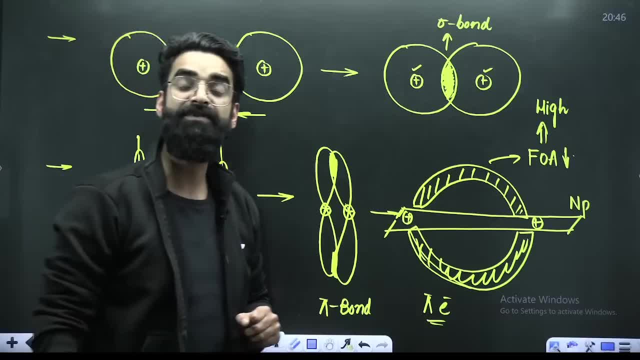 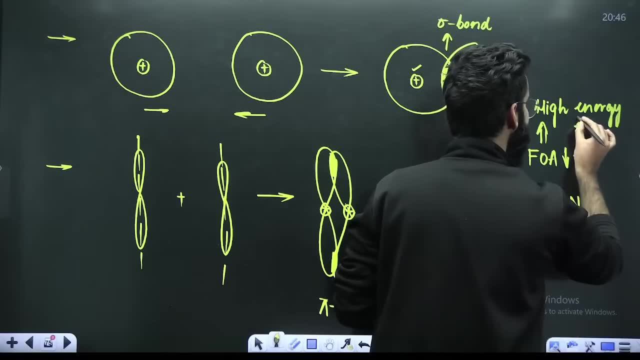 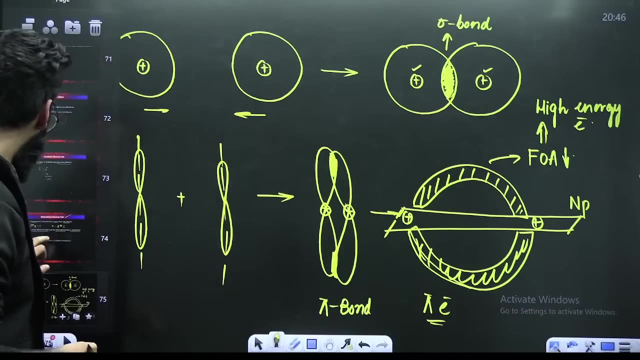 That is something which you call as high energy electron density. That is something which you call as high energy electron density. So what is the high energy electron density? Why did I tell you all this? Because the point was very simple Initially. I told you first of all what is a delocalized pair. 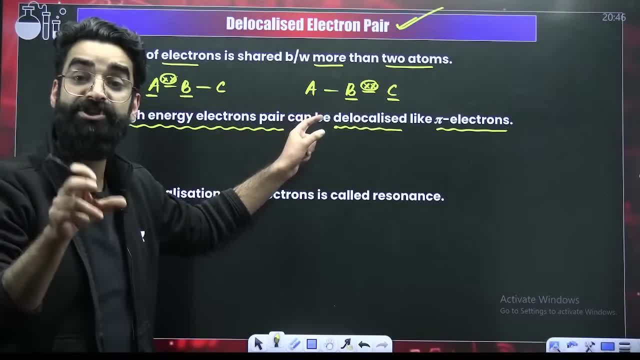 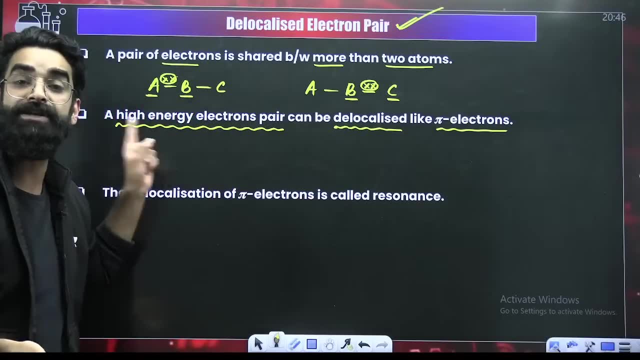 Delocalized electron pair is that electron pair which is shared by more than two atoms. Now the point was: which electron pair can be shared by more than two atoms, Which electron pair can be delocalized? I told you high energy electron pair can be delocalized. 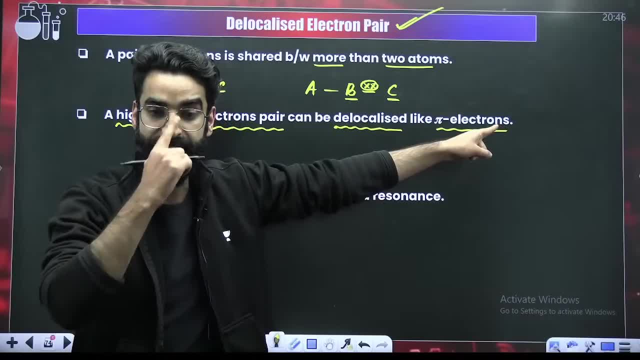 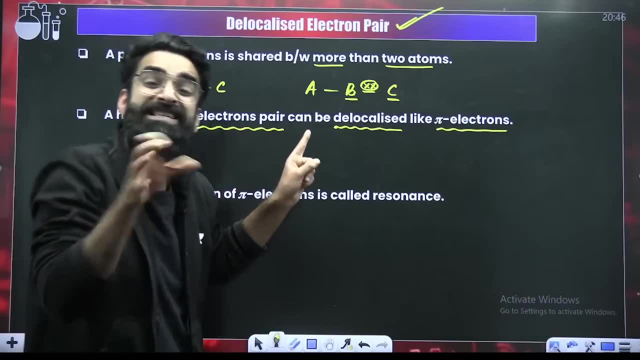 Like your pi electrons, Right, Like your pi electrons? Is this clear High energy electron pair, That electron pair which will be subjugated to less force of attraction by the nucleus? That is something which you call as high energy electron pair. 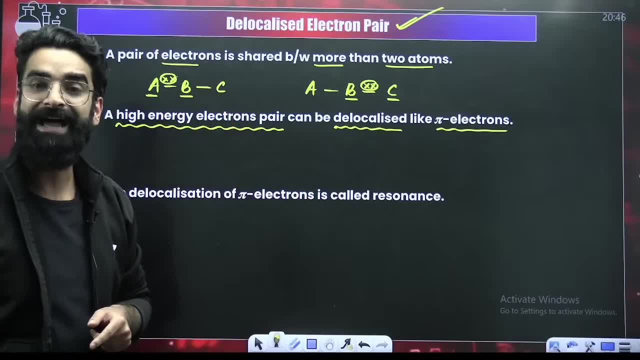 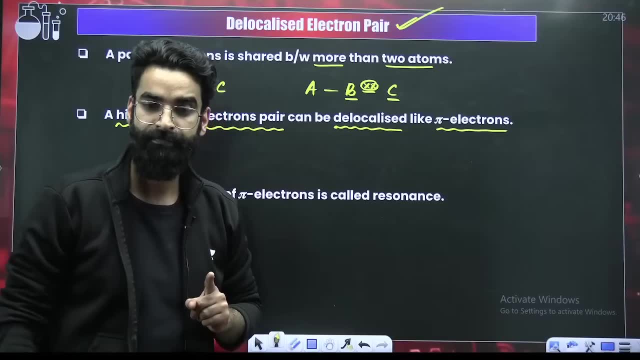 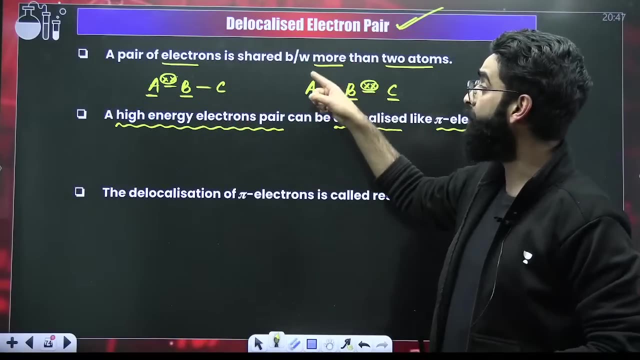 And that high energy electron pair, that high energy electron pair, can be delocalized. Yes, Is this point clear? Is this point clear? Guys, try to understand carefully what I am saying. First, I made you clear what is delocalized electron pair. 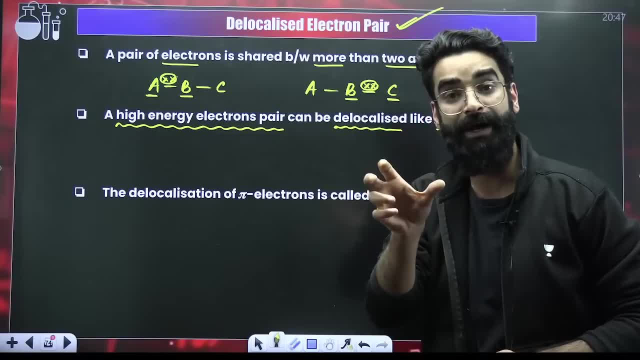 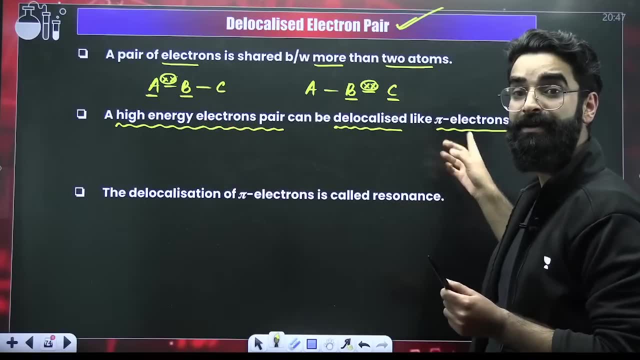 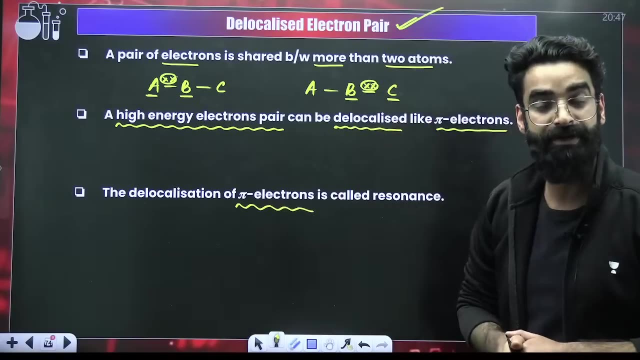 It is that electron pair which is shared by more than two atoms. Now the point was which electron pair can be delocalized. It is the high energy electron pair, like your pi electron pair, which can be delocalized. And delocalization- delocalization of high energy electron pairs. 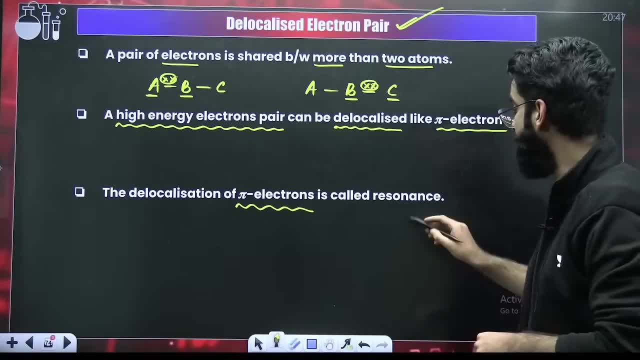 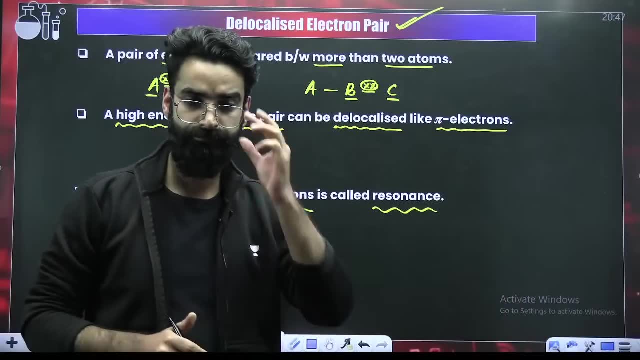 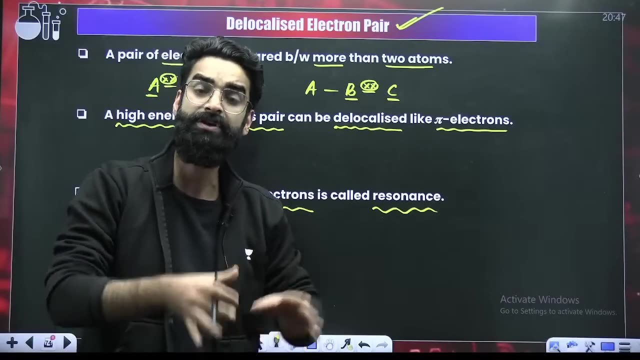 Delocalization of high energy electron pairs is something which is what you call as resonance. Did you get the idea of what this resonance is all about? Did you get the idea of what resonance is all about? So resonance is just defined as the delocalization of high energy electron pairs, like your pi electron. 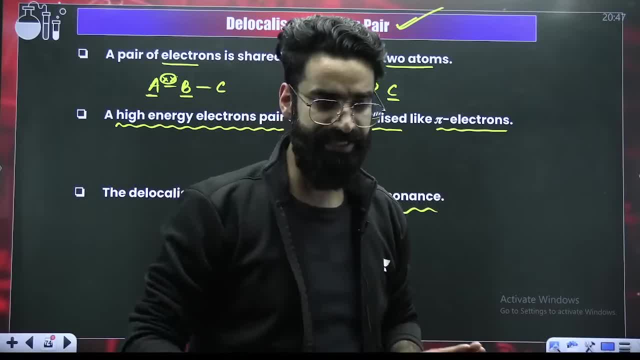 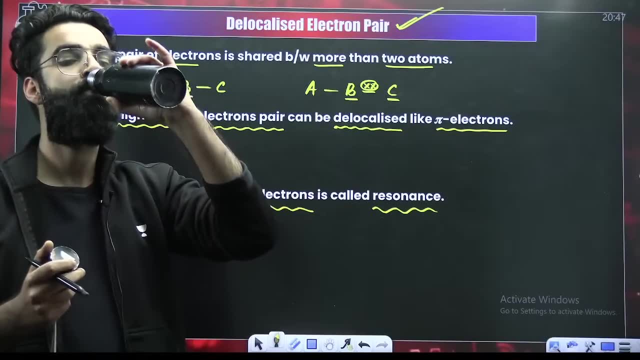 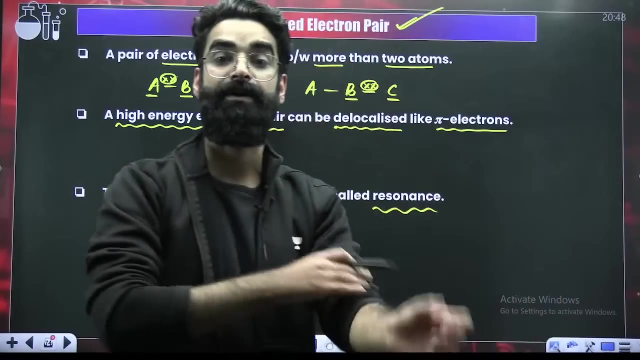 Right, Let me know once in the chats if it is clear. Let me know once in the chats if it is clear. The delocalization of high energy electron pairs like your pi electrons: Right, That is something which is what you call as resonance. 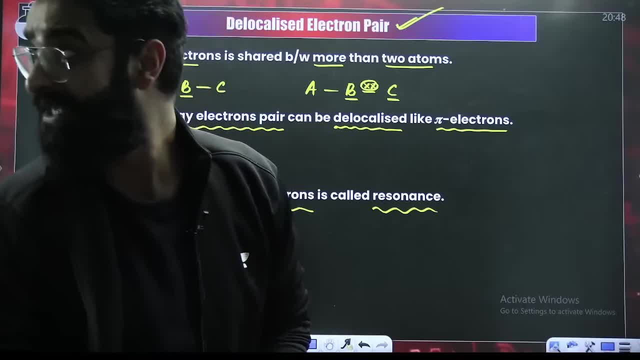 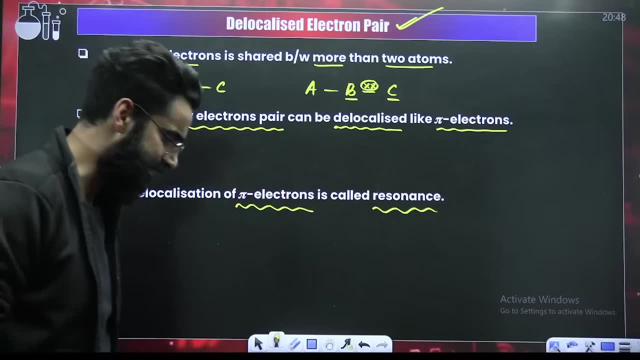 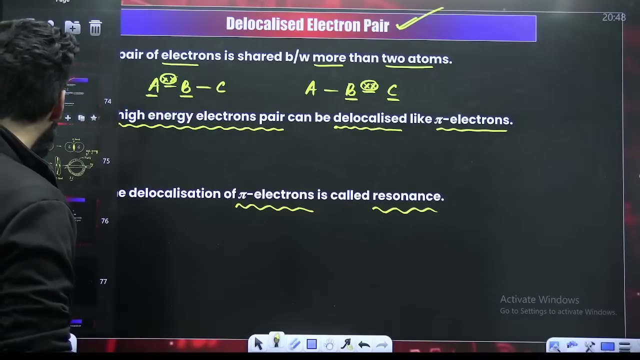 Perfect. Now, guys, before making you understand, before showing you how do we draw the resonating structures, etc. etc. There is one approach which you need to learn, Right, There is one approach which you need to learn That is something which you call as orbital approach of resonance. 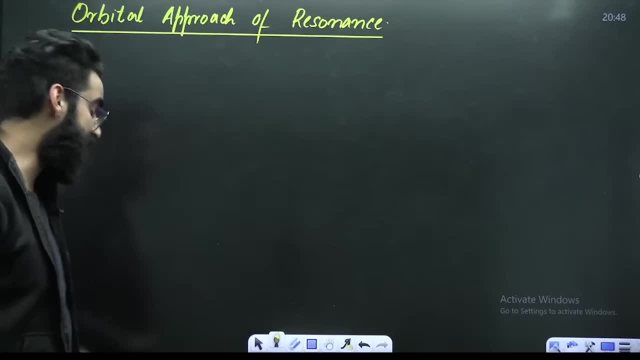 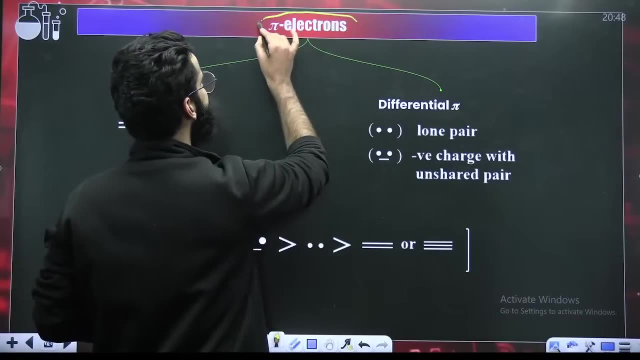 But, but again, before making you understand the orbital approach of resonance, there is one more thing which I want to let you know: Your pi electrons, which are your high energy electrons, right, They can be delocalized. These pi electrons are exactly of two types. 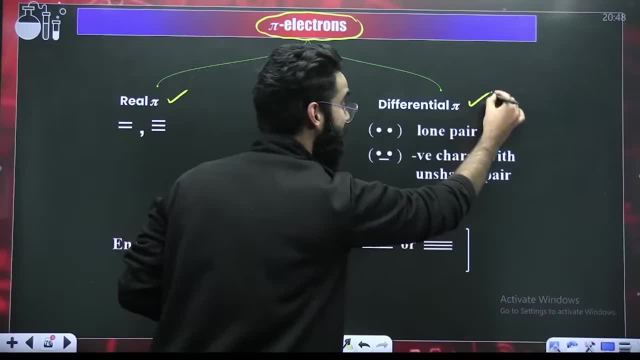 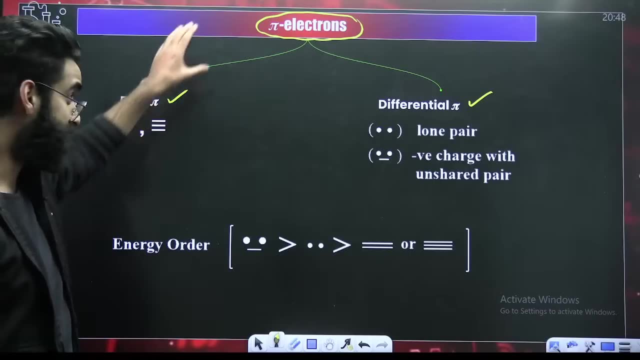 One you call as the real pi electrons, Another one you call as differential pi electrons. If I talk about your pi electrons, Pi electrons are of two types. basically, Right Pi electrons are the ones which are subjugated to less force of attraction by the nuclei. 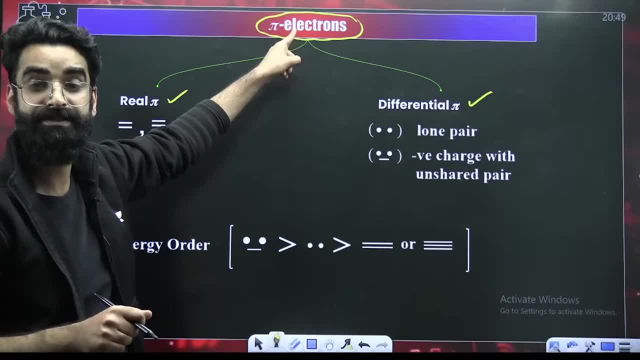 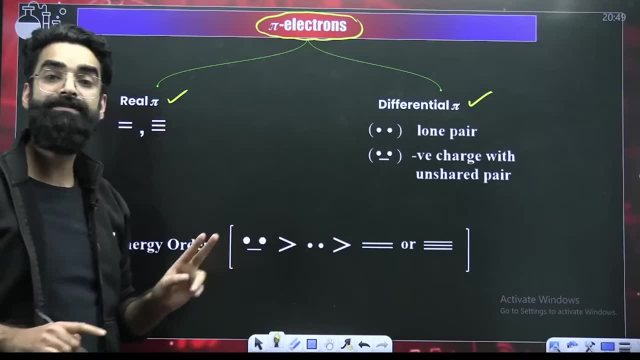 Right, These are high energy electron pairs, Right, And these high energy electron pairs get delocalized. basically, Now these pi electron, these are of two types. One is real pi, one is differential pi. What are real pi electrons? 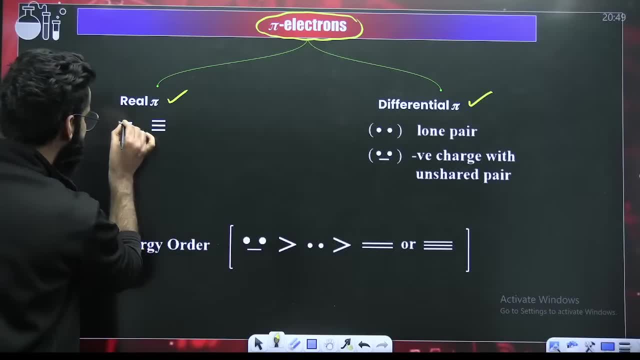 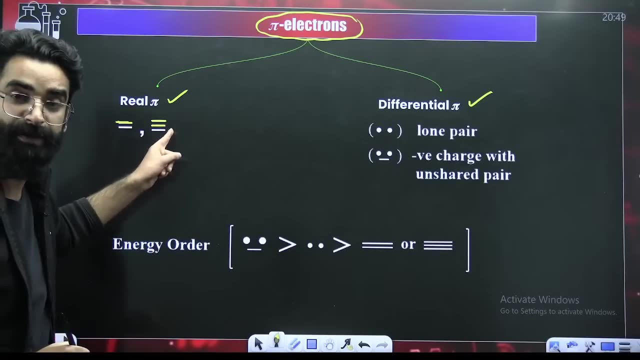 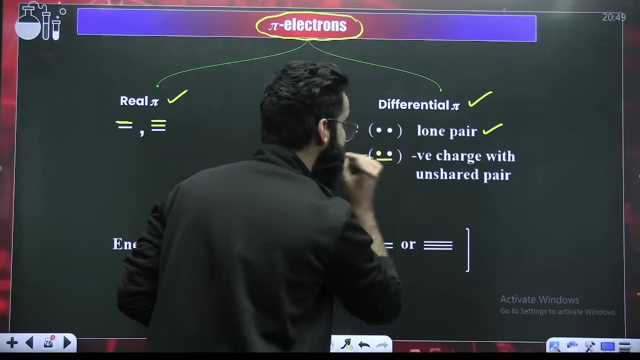 Real pi electrons are the ones which are subjugated, Which are present either in double bond or triple bond. Real pi electrons are the ones which are present in either double bond or triple bond, Whereas your differential pi Lone pair you call as differential pi or negative charge, with an unshared pair of electrons. 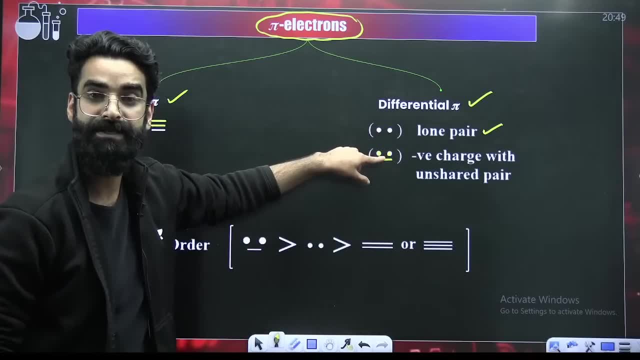 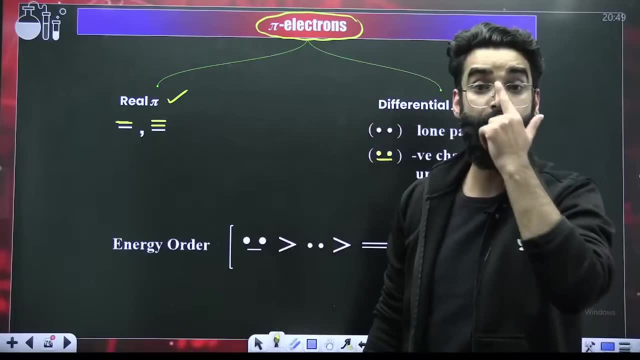 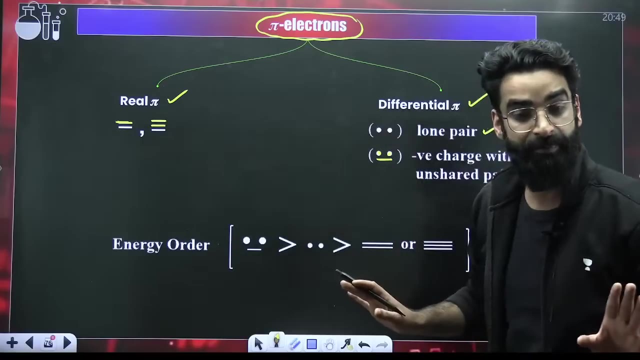 Lone pair and negative charge with unshared pair of electrons. These are what you call as differential pi electrons. These are what you call as differential pi electrons. These are what you call as differential pi electrons. And, my dear students, There is a particular energy order of these real pi and differential pi electrons which you need to remember. 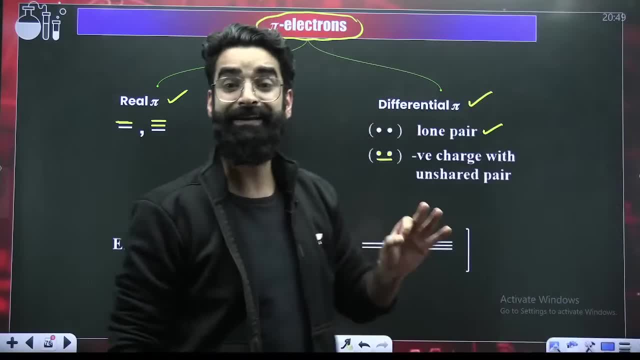 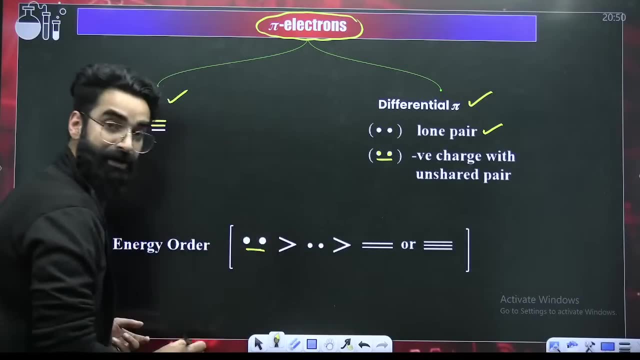 There is one energy order which you need to remember regarding these real pi electrons and differential pi electrons. And what is that energy order? Negative charge. with unshared pair of electrons, This will be always having more energy, Followed by the lone pair. 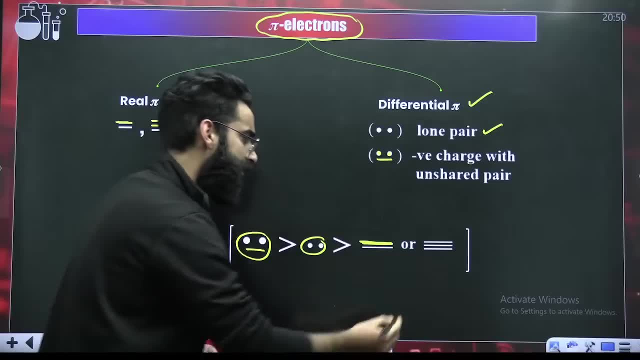 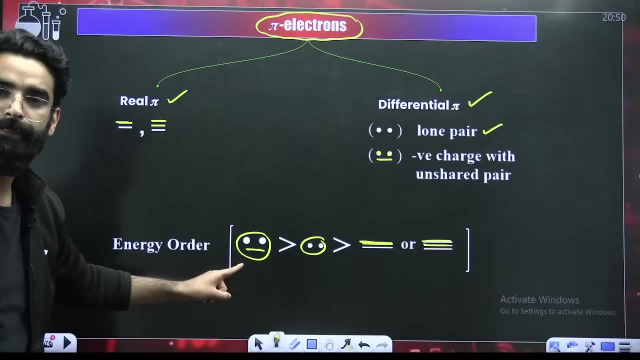 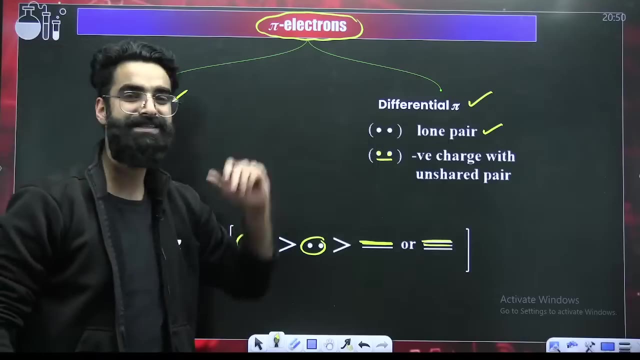 Followed by the pi electron pair of this double bond, Followed by these two pi electron pairs of these triple bonds. Just remember this directly: First of all, what are these electron pairs? What are these electron pairs? What this real pi is all about? 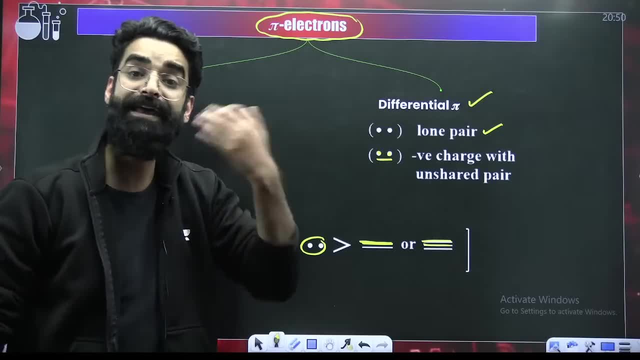 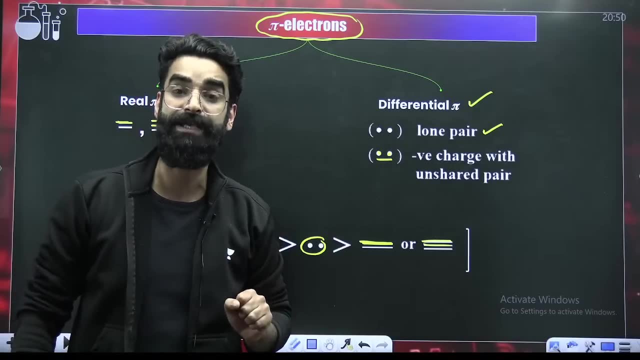 What this differential pi is all about. These are the types of pi electrons. Pi electrons are high energy electrons, And only high energy electrons. they get delocalized. I mean your high energy electrons. they get delocalized, They show delocalization. 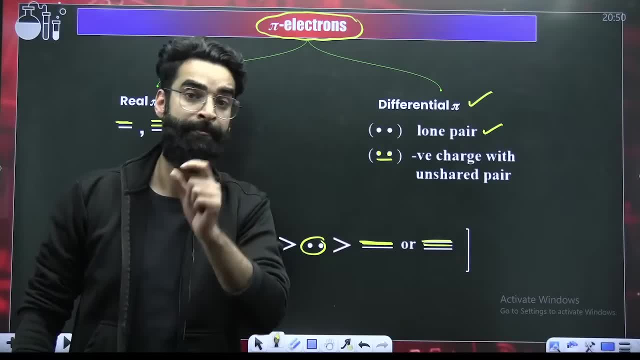 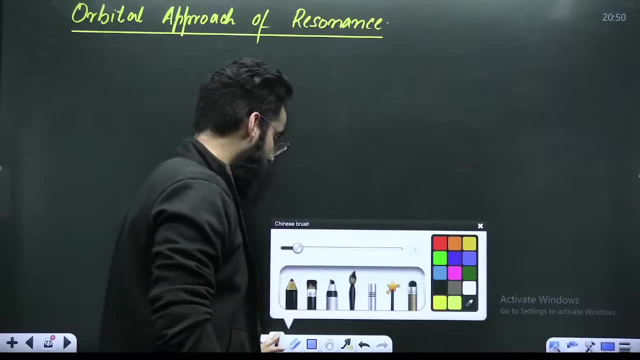 Right, They show delocalization, Now people. now let me make you understand the actual concept of resonance. Now let me make you understand the actual concept of resonance. Try to understand First of all. if I ask you, what is the structure of benzene? 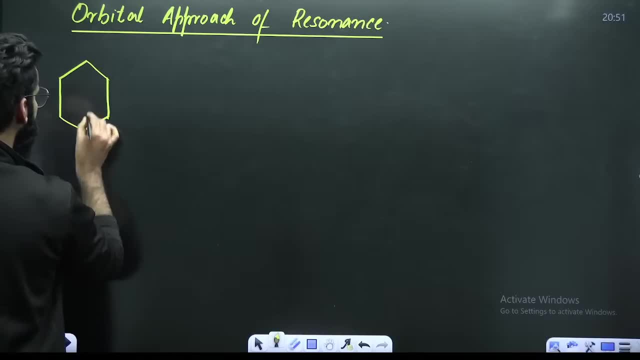 Some of you will come up with this structure. Some of you will come up with this structure Right Now if you exactly have a look on how this structure is formed- actually How this structure is formed, actually, If you have a look on how this particular structure is formed. 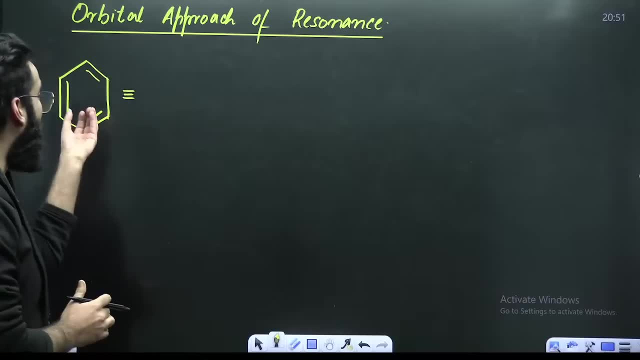 Can you do that? Can you make the orbital diagram of this particular benzene? Can you make the orbital diagram of this particular benzene? Or I will do one thing. I will make it comparatively simple. Let me make it like this. Let me make it like this: 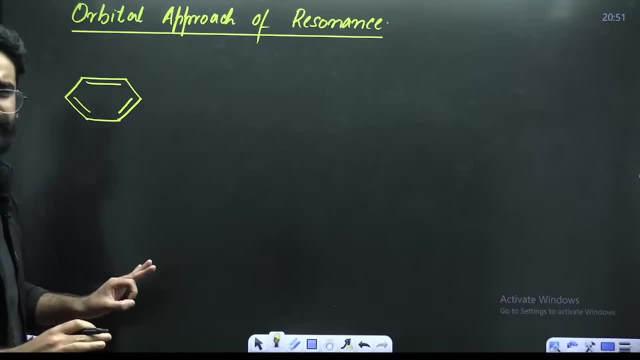 Right. I asked you: what is the structure of benzene? Some of you told me this is the structure of benzene. Now I am going to explain how this structure was formed, basically How this structure was formed. First of all, my dear students, 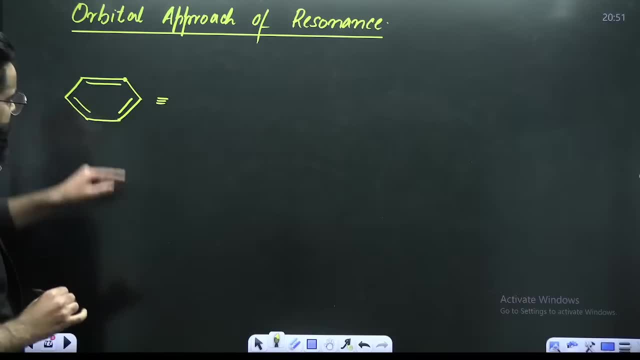 if you look at this particular carbon, can you let me know its hybridization, This particular carbon, its hybridization? See one sigma, two sigma and one more sigma with hydrogen. So it is sp2 hybridized. Even this is sp2,, this is sp2, this is sp2.. 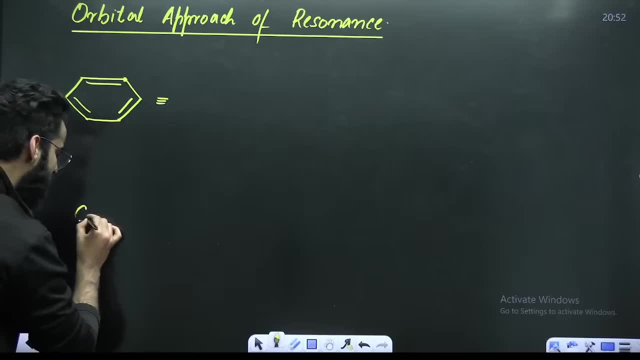 Every carbon here is sp2.. Now, my dear students, what is the outermost configuration of carbon? It is 2s2, 2p2.. How do you know that? This is your 2s orbital and this is your 2p? 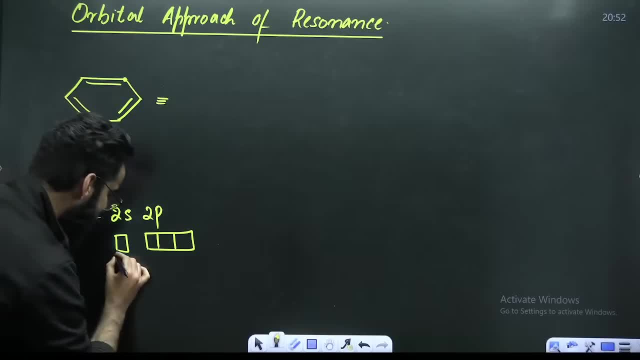 These are your three 2p orbitals. Now, every carbon is sp2 hybridized. Every carbon is sp2 hybridized. Every carbon is sp2 hybridized. Can I say every carbon will contain one pure p orbital as well. Absolutely every carbon will contain. 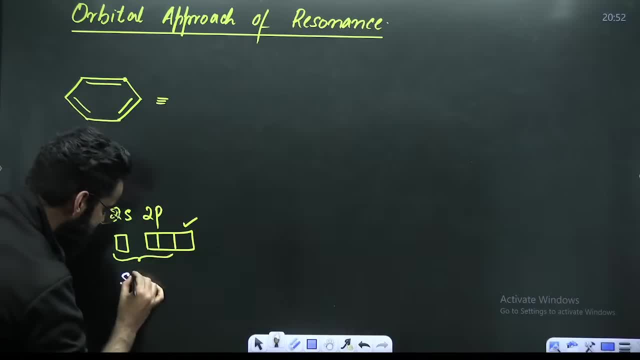 one pure p orbital as well. So, basically, the hybridization involved here is sp2.. Right, The hybridization involved here is sp2.. One pure p orbital present at every carbon. And, my dear students, let me tell you, in case of sp2,, 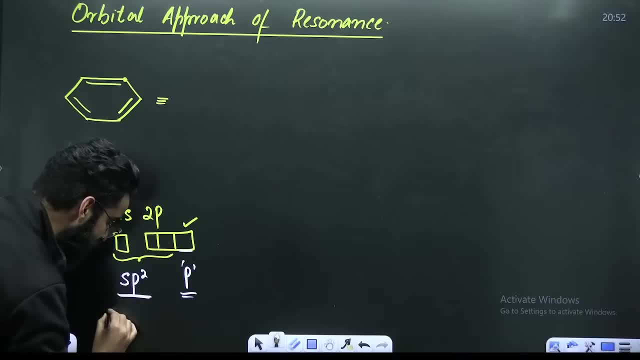 in case of sp2 hybridization, what is the geometry as per sp2 hybridization? It is trigonal planar, It is trigonal planar, Right, You must be knowing this. This is trigonal planar. What is meant by trigonal planar geometry? 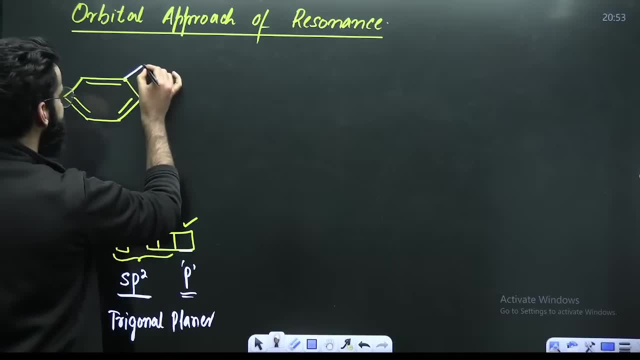 What is meant by trigonal planar geometry. See, if I talk about this particular carbon, it is attached with hydrogen as well. on this side, First of all, the carbon has undergone sp2 hybridization Right, Which leads to the formation of three hybrid orbitals. 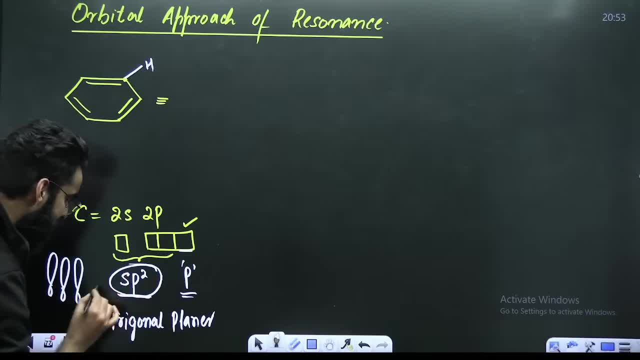 So there will be three sp2 hybrid orbitals, And apart from that, there will be one pure p orbital as well. Perfect Now, my dear students, these sp2 hybrid orbitals, what they have done, One of the sp2 hybrid orbital has done the overlap. 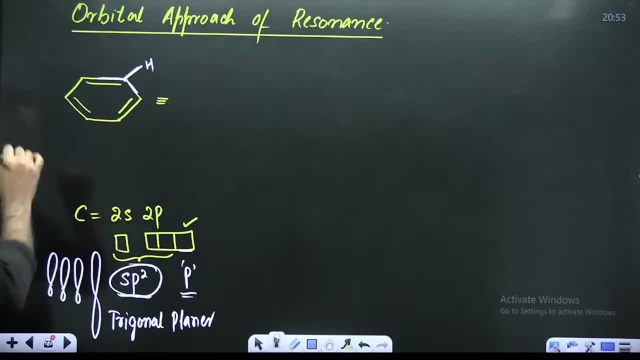 Formed the sigma bond. One more has formed one more sigma bond- Right, Perfect, And this particular carbon. it has got p orbital as well. It has got p orbital as well, And that p orbital will be perpendicular to the plane containing these bonds. 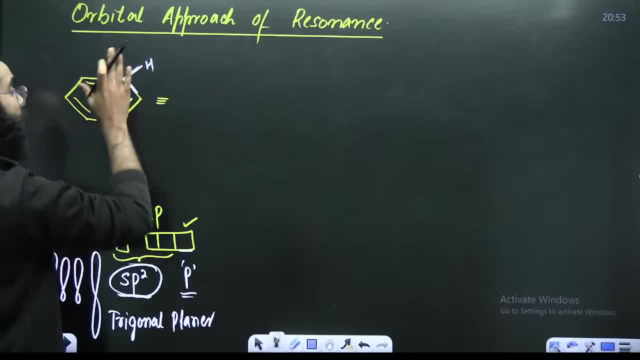 See, first of all, this bond, this bond, this bond. They are present on the same plane, They are present on board. Now, perpendicular to the board, there will be a p orbital. Perpendicular to the board, there will be a p orbital. 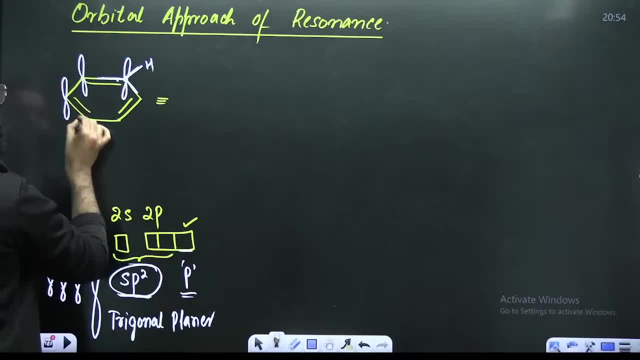 So this is a p orbital here. Even this has got its p orbital. This has got its p orbital. Even this has got its p orbital. You know it now, Right guys? So if I talk about benzene, all the carbon atoms are sp2 hybridized. 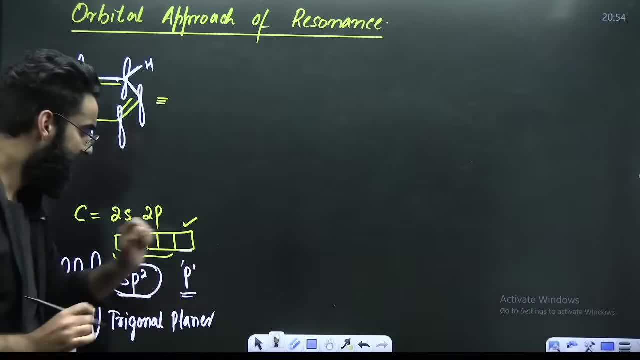 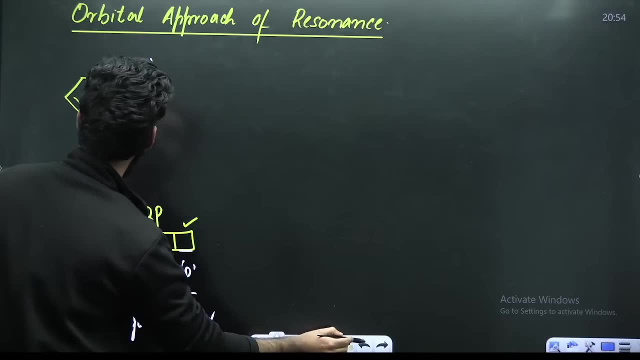 and every carbon has got one pure p orbital as well. Perfect. Now, guys, try to understand If I exactly want to make the orbital diagram. how exactly am I going to make it? Try to understand it carefully. Try to understand it carefully. 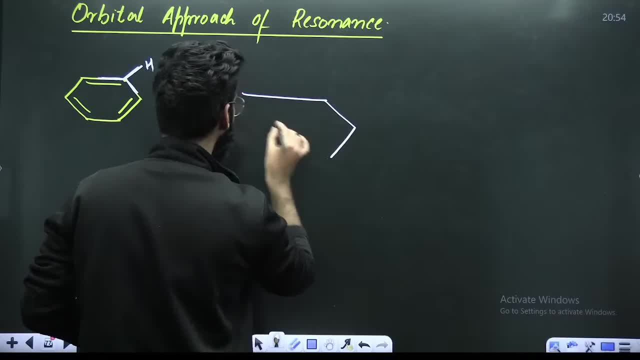 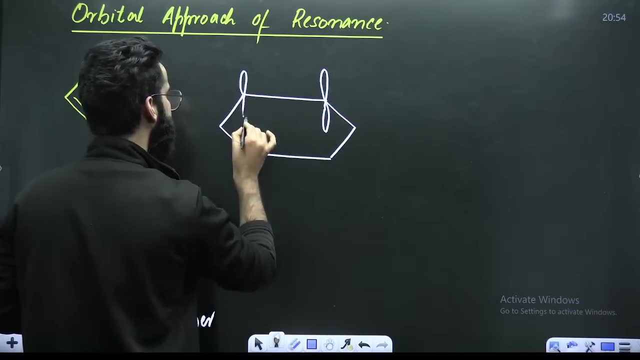 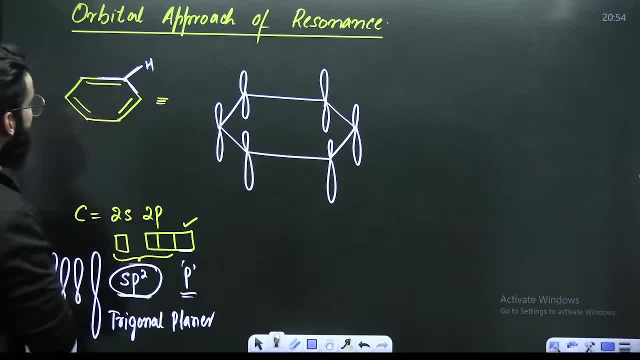 there is a π bond between these two carbons. There is a π bond between these two carbon atoms. How this π bond is formed? It gets formed by the parallel overlapping of the orbitals. Can we say as per particular structure, As per this particular structure, these two orbitals have parallely overlapped. 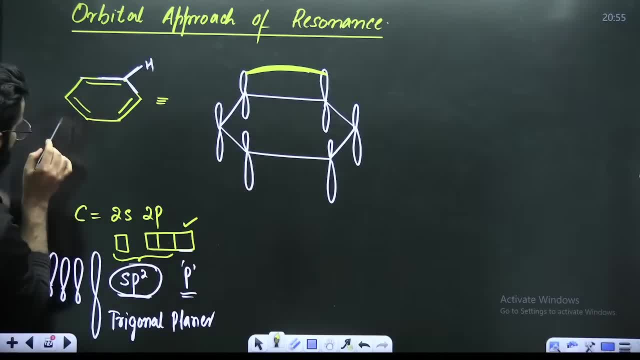 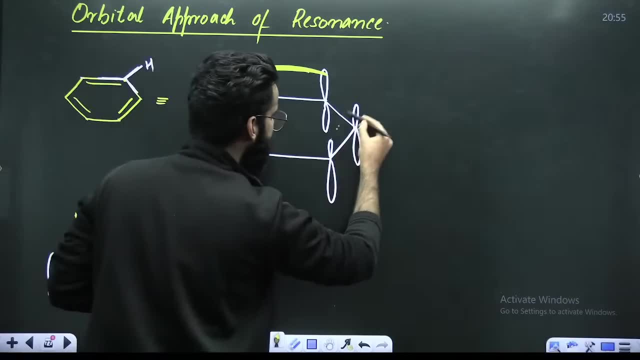 They have parallely overlapped and formed a pi bond here. Similarly, p orbital of this and p orbital of this, they have parallely overlapped and formed a pi bond Right. Similarly, these two have parallely overlapped and formed a pi bond. 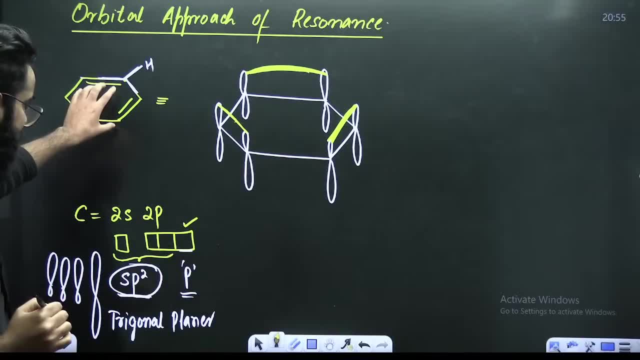 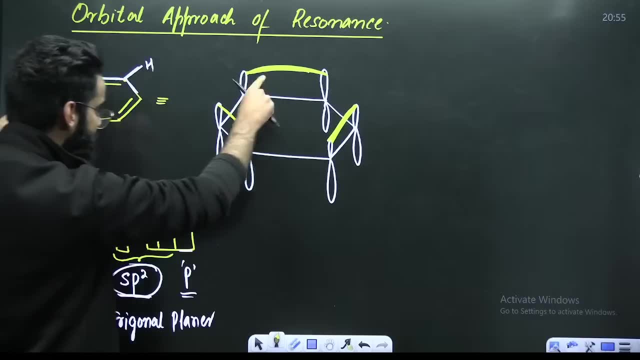 Right, As per this structure. as per this structure, there is a pi bond here. There is a pi bond here. That means the p orbital of these two carbon atoms would have parallely overlapped and formed a pi bond. There is a pi bond. 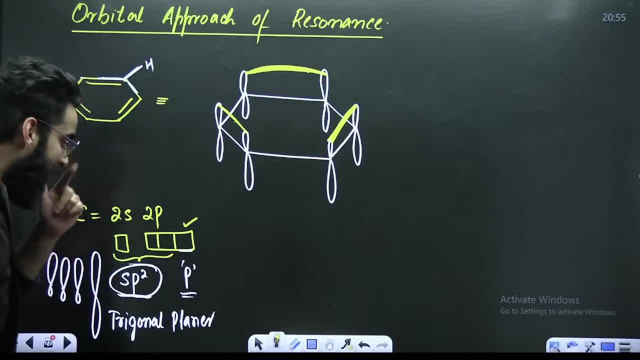 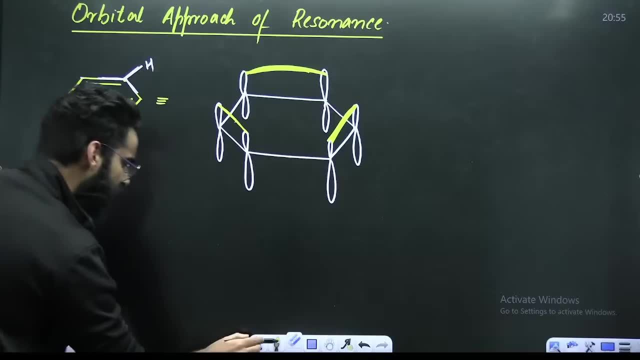 There is a pi bond, Correct? Now, my dear students, one more thing, One more thing, One more thing. If I ask you what is the structure of benzene, A lot of you told me this is the structure of benzene. 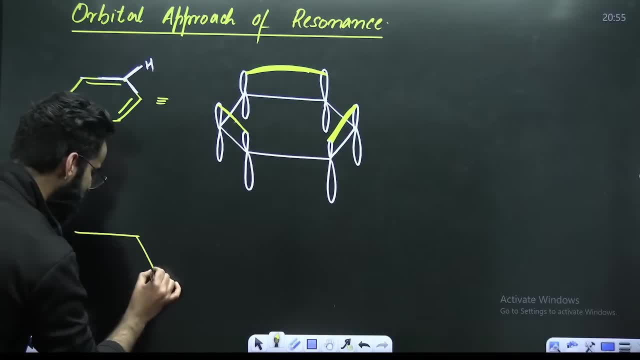 But there will be few students who will tell me that this is not the structure of benzene. This one is the structure of benzene. A lot among you will tell me this is the structure of benzene. Now can you tell me how this structure would have got formed? 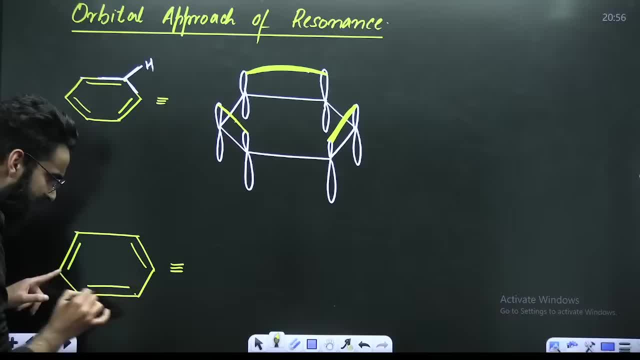 If you look at its orbital approach, See, every carbon will come. Every carbon is sp2 hybridized, Right, And there is a pure p orbital with every carbon here, Right. So if you make its structure, Or let me make its structure over here, 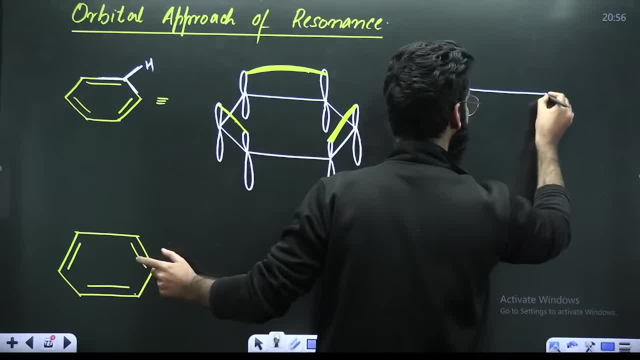 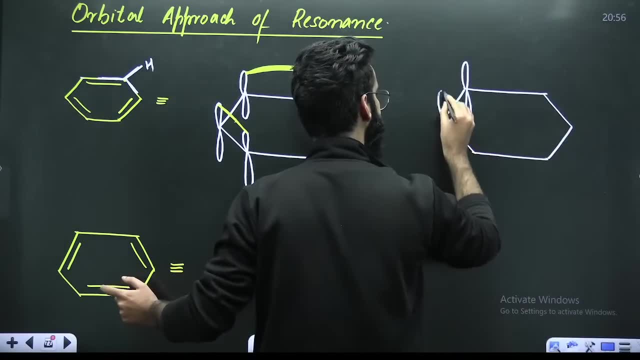 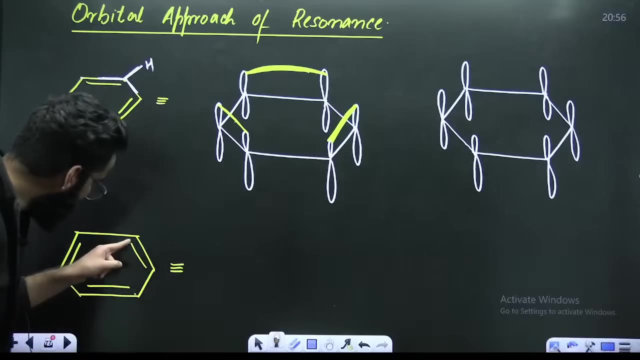 Let me make its structure over here. Let me make its orbital diagram over here. Every carbon has got a pure p orbital. Every carbon has got a pure p orbital. Now people look at this particular structure. There is a pi bond. 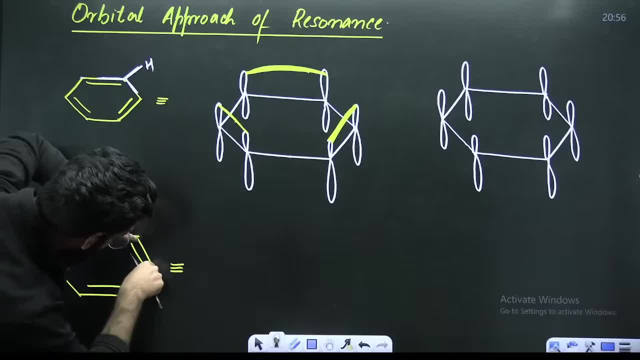 There are piittä in the undulations. There is a pi dot in the Planck domain. There is a right and wrong between these two. There is a correlation between these two. What does that mean? That means the dirt orbital of this and the corto mapa of this they will have. 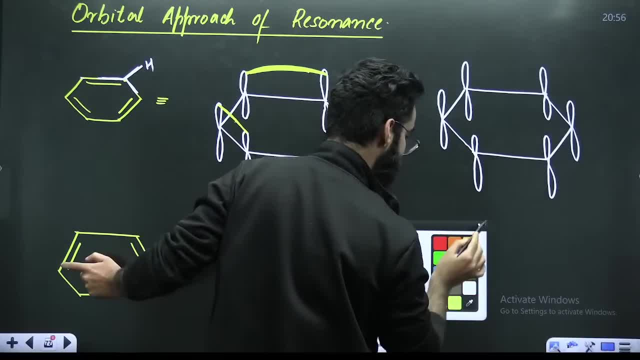 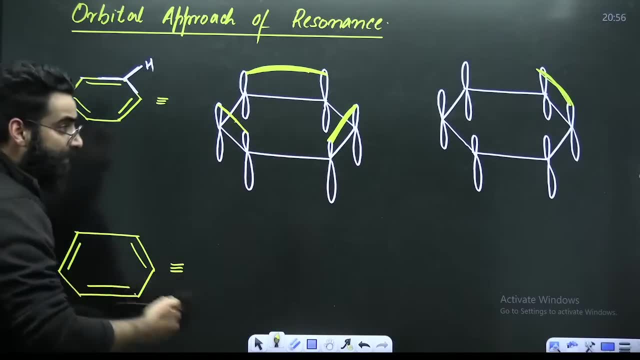 not only overlapped, and from the pi bond I don't see words. So I would say: as for this particular structure, This orbital will, they are badly overlapped right. similarly, the partable of these two they will apparently overlap. that means these two parallel or not. 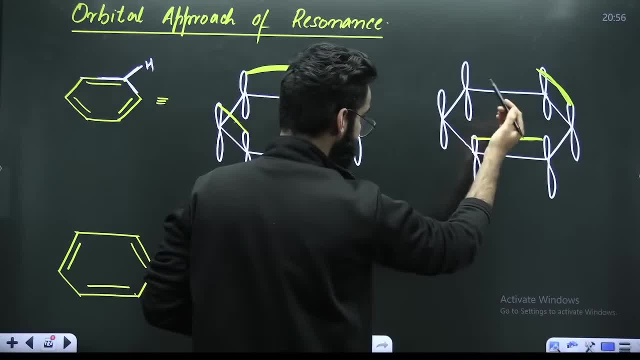 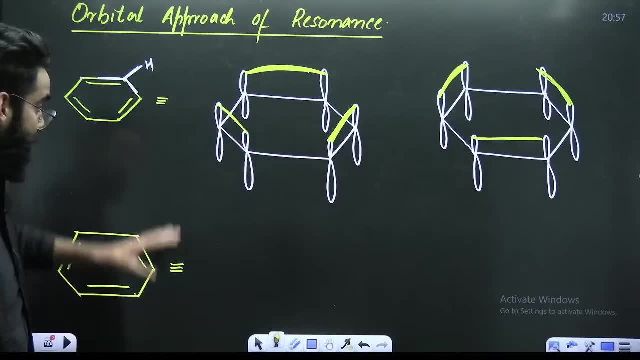 Right. Some balancing these two are partly or not All right, these two are partly overlapped, Correct. Not only you are to change the structure of a building, you just, or, since you are correct, So I give you two structures of benzene. 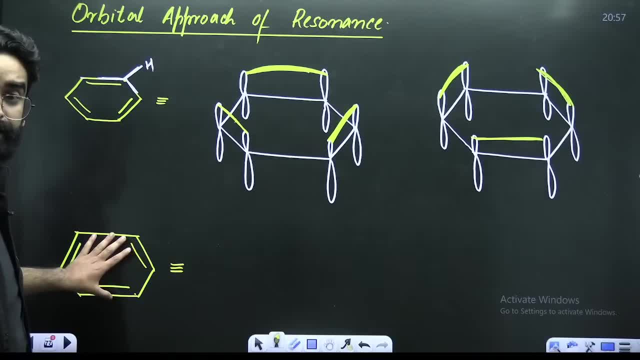 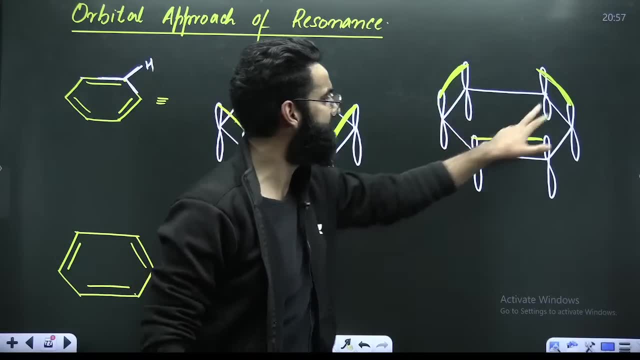 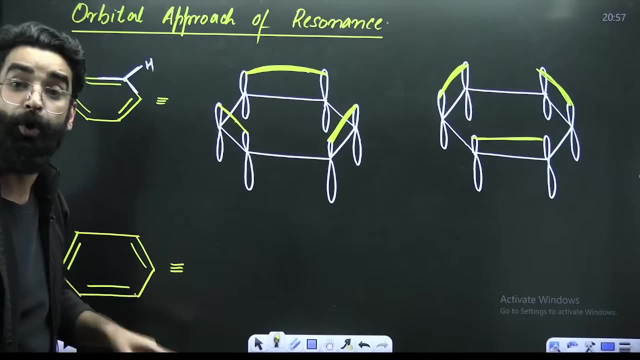 One structure of benzene is this. one structure of benzene is this: This particular structure of benzene is formed when these orbitals overlap. and this particular structure of benzene is formed when these orbitals overlap, But is this structure able to explain all the properties of benzene? 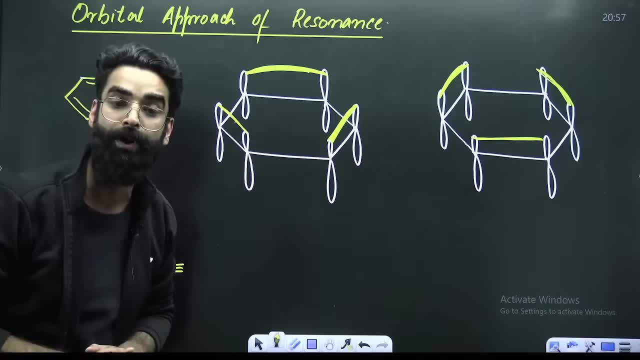 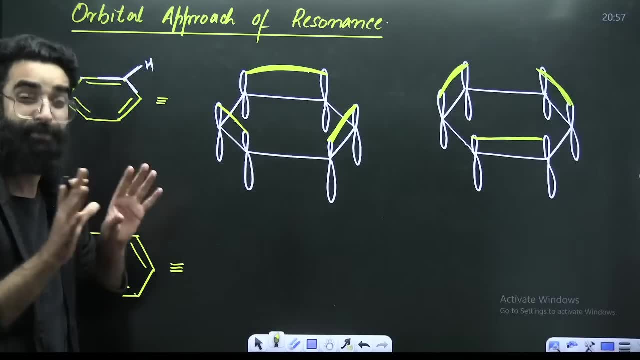 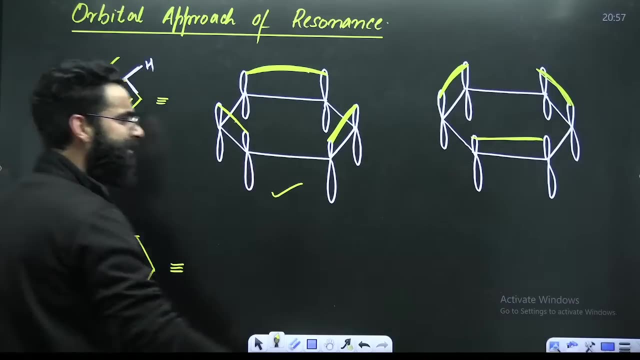 No, Is this particular structure able to explain all the properties of benzene? No, But I would say, but I would say some of the properties of benzene, some of the properties of benzene this structure will be explaining. That means this structure will be explaining and some of the properties of benzene. this 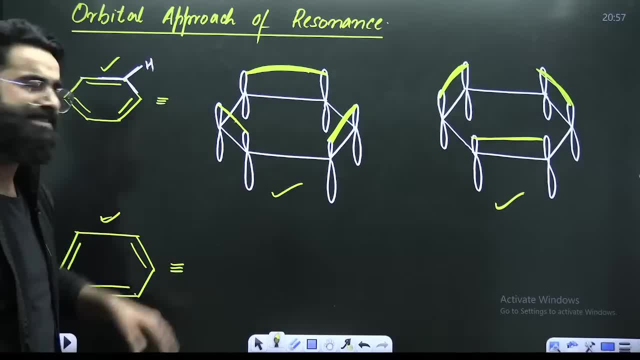 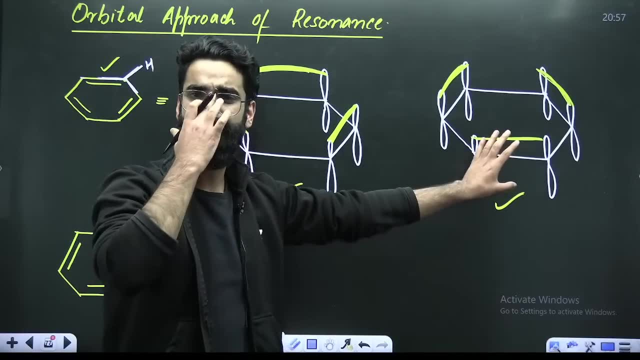 particular structure will be explaining Some of the properties of benzene. this structure will be explaining and some of the properties of benzene this particular structure will be explaining. So basically related to benzene, some of the information you are getting from this particular structure. 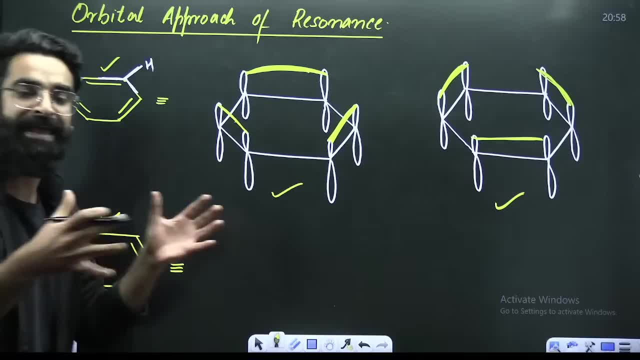 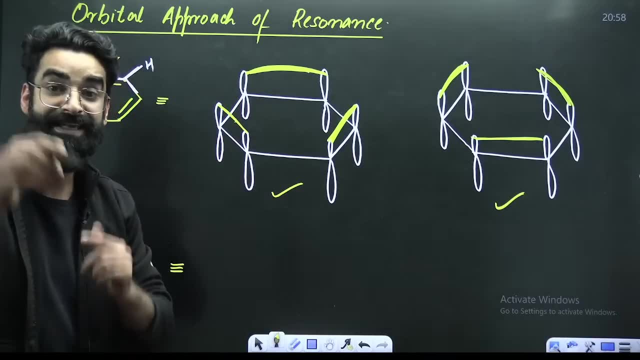 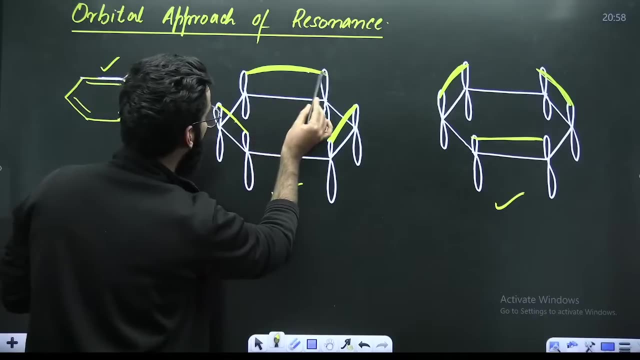 Some of the information you are getting from this particular structure. If you combine the information, if you combine the information, what do you get? See, guys, this particular structure is telling you, this particular structure is telling you that these two orbitals have parallel overlap. but this particular structure is telling: 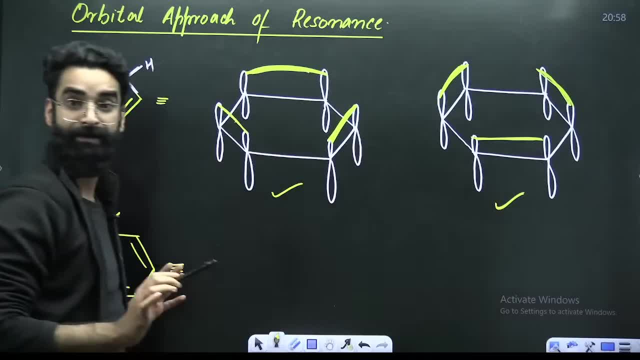 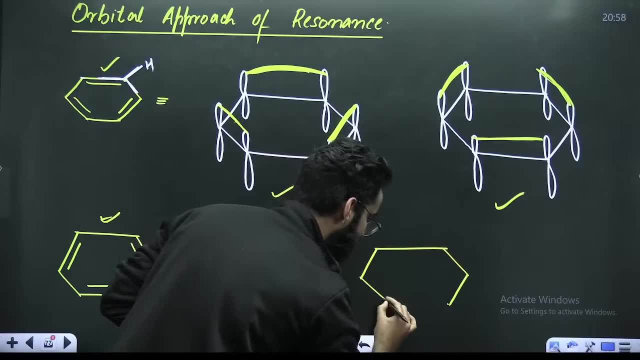 you, these two have not overlapped. these two have overlapped right. So in the actual structure of benzene, what would have happened In the actual structure of benzene, what would have happened? I told you guys, I told you some of the information. this is giving us some of the information. 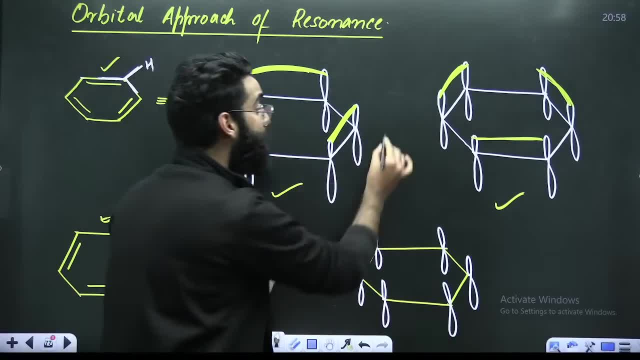 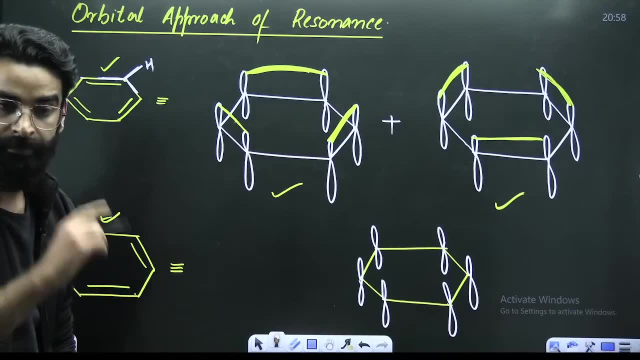 this is giving us. we have to compile both the information. we have to compile both the information. we have to compile both the informations. right, we have to compile both the information. Now, try to understand. Try to understand As per this particular structureISS. 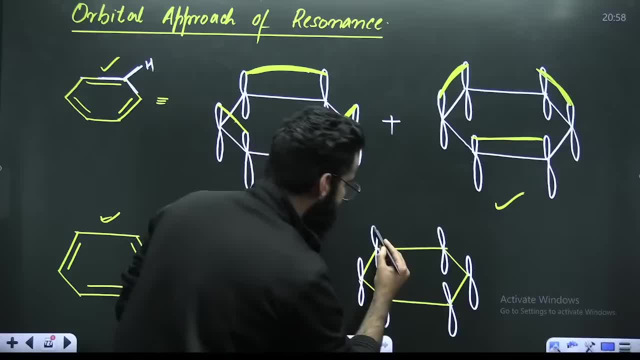 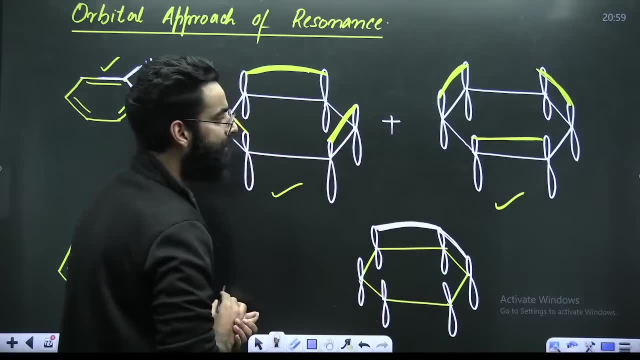 Right, See, Okay, Okay, See, Right See. overlap is between these two. Overlap is between these two, But, as per this structure, overlap is between this and this Right. As per this structure, overlap is between this and this. 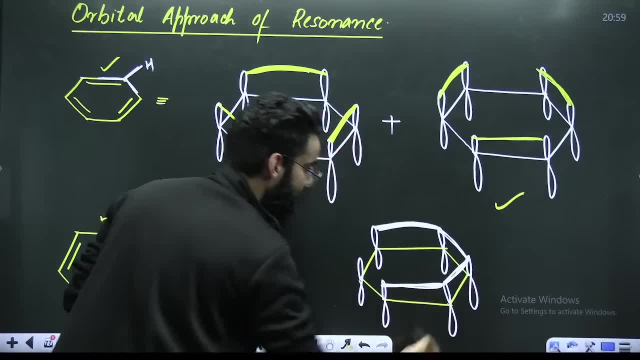 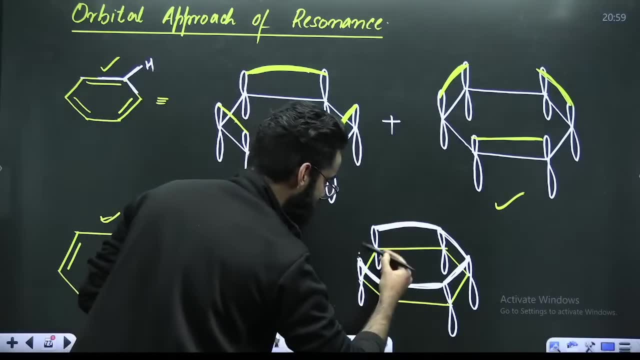 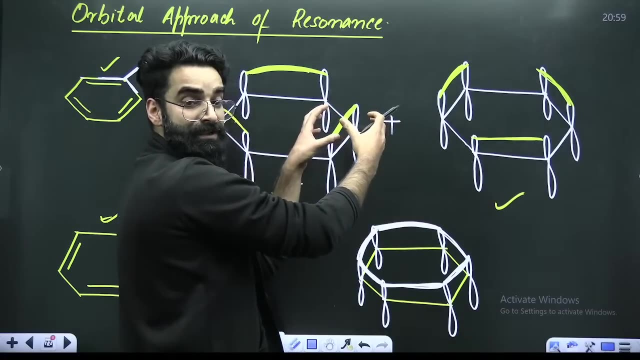 But, as per this structure, overlap is between this and this: Right: As per this particular structure, overlap is between this and this. Parallel overlap: As per this particular structure, overlap is between this and this. So we compiled all the information from these two structures. 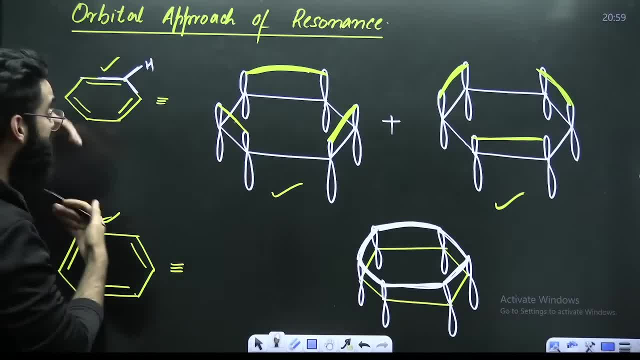 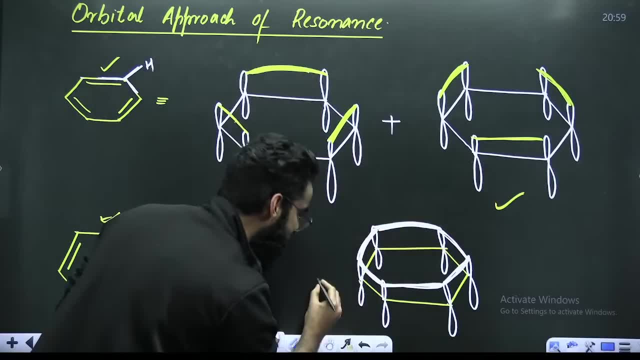 These are the proposed structures of benzene. These are the proposed structures of benzene which we gave And, after giving the proposed structures of benzene, we compiled all the information. We are merging the information and we got something like this. We got something like this: 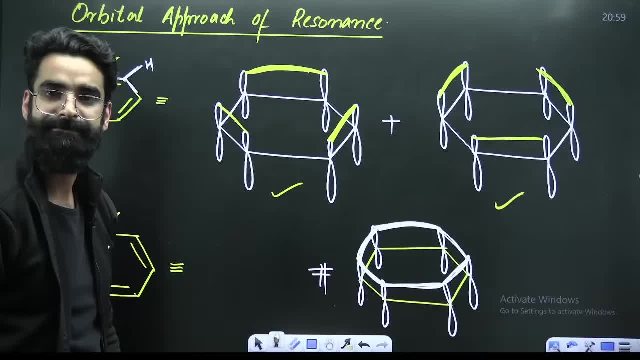 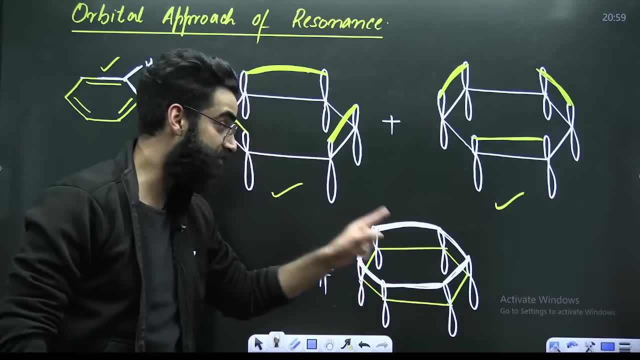 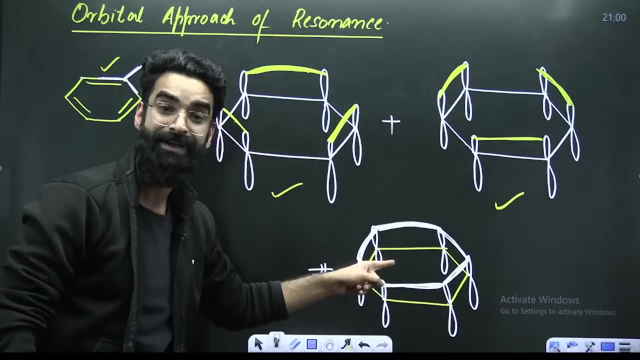 Right, We got something like this. So, this particular structure, try to understand In this particular type of structure, if you see, if you see this particular type, if you see this particular structure, this particular structure is telling you that, in case of benzene. 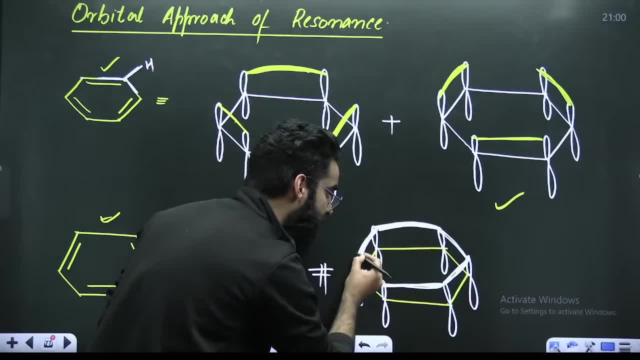 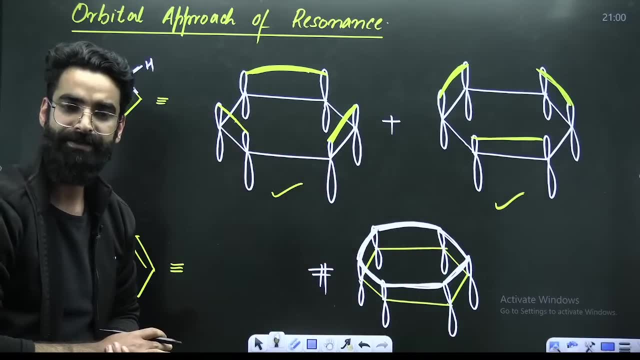 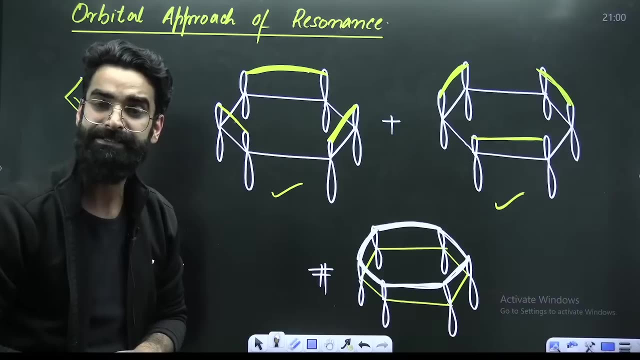 there is the simultaneous overlap, There is a simultaneous parallel overlap of these p orbitals. Right, This particular structure is telling you: there is a simultaneous parallel overlap, There is a simultaneous parallel overlap of p orbitals. Perfect, Please, students, let me tell you. 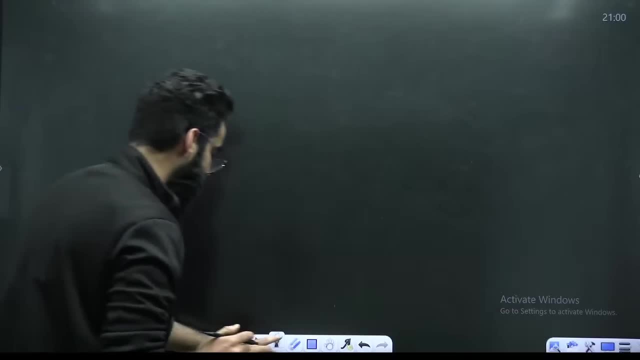 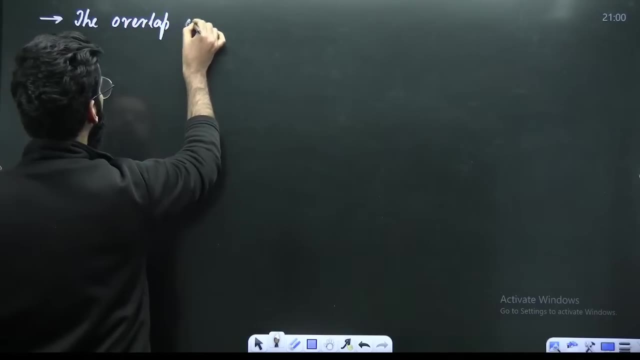 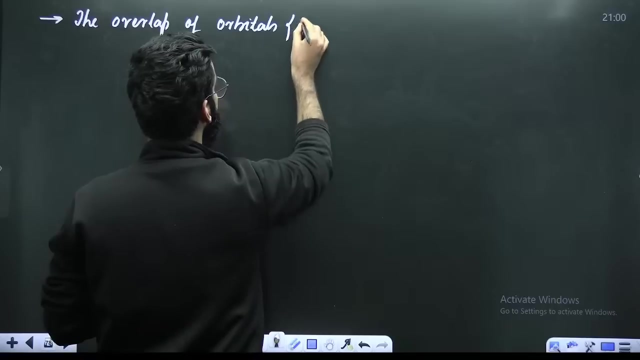 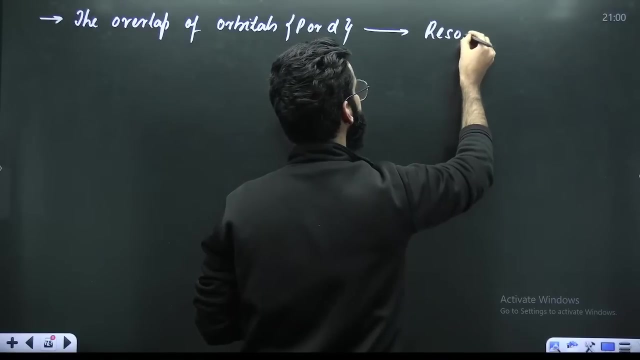 let me tell you one simple thing. Let me tell you one simple thing: The overlap, the overlap of orbitals, the parallel overlap of orbitals- orbitals can be p or d- is something which is called as resonance, basically The parallel overlap of here. 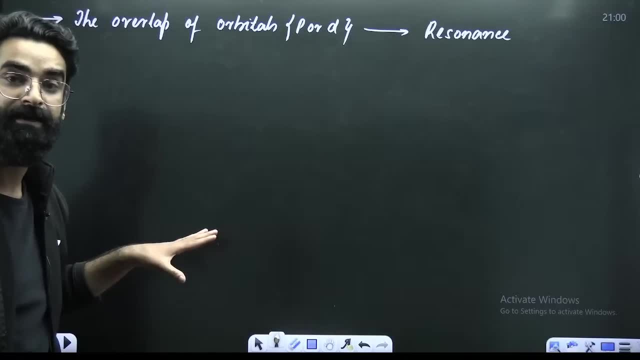 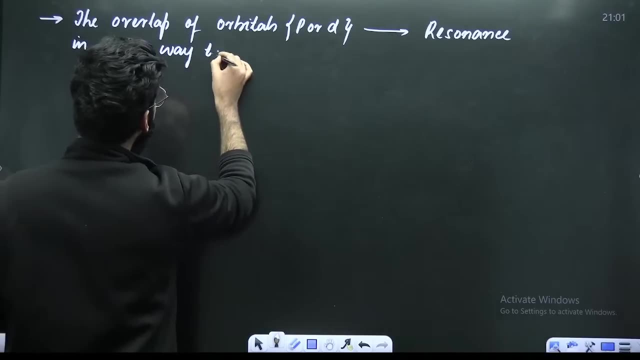 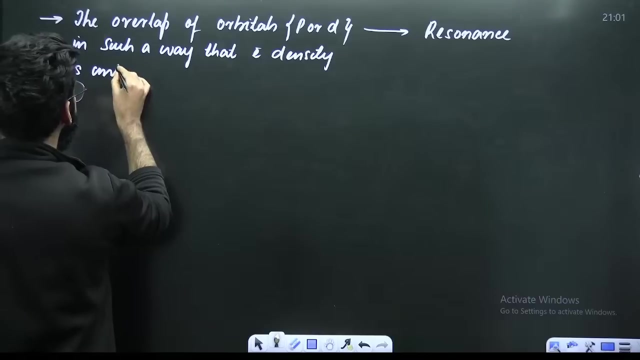 as in case of benzene, the parallel overlap of your p orbitals Right In such a way, in such a way, in such a way that electron density is uniform throughout, is uniform throughout, That the electron density is uniform throughout. 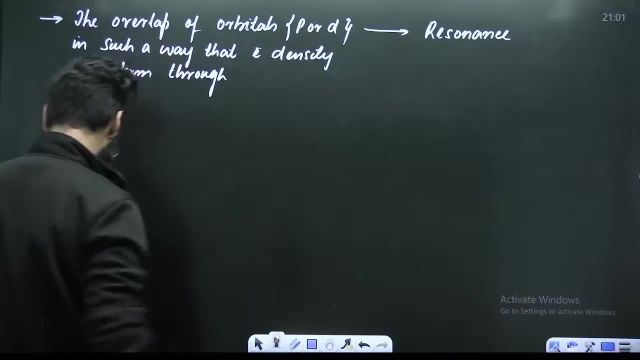 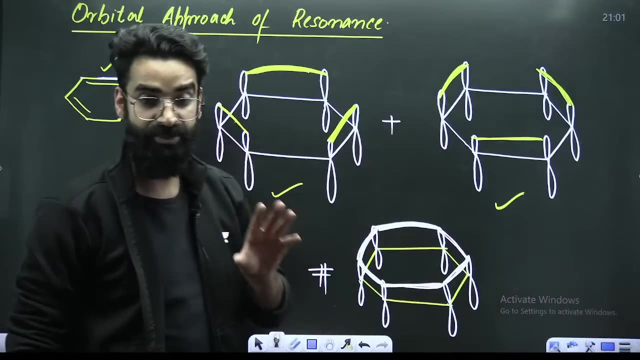 That the electron density is uniform throughout. It is something which you call as benzene. It is something which you call as resonance Perfect. Did you get the idea of what I said? Did you actually get the idea of what I said? Did you actually get the idea of what I said? 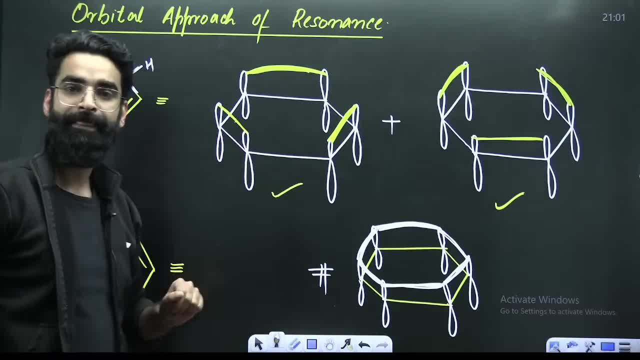 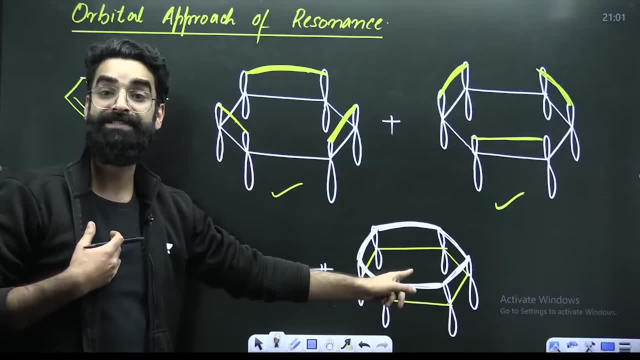 Did you actually get the idea of what I said? Now we will try to understand. This is the structure which we proposed about benzene. This is the structure which we proposed about benzene. We compiled the information. We got the actual structure of benzene. 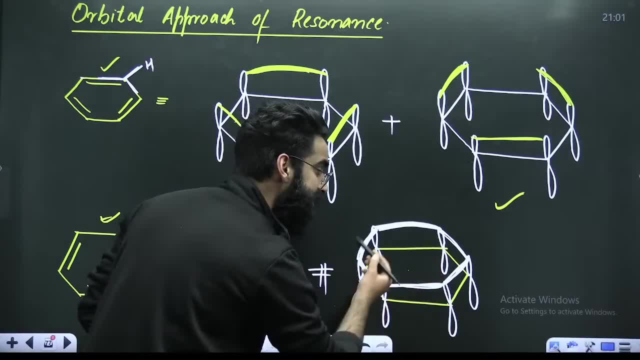 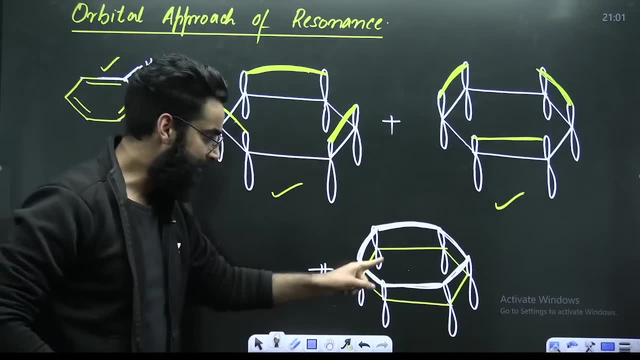 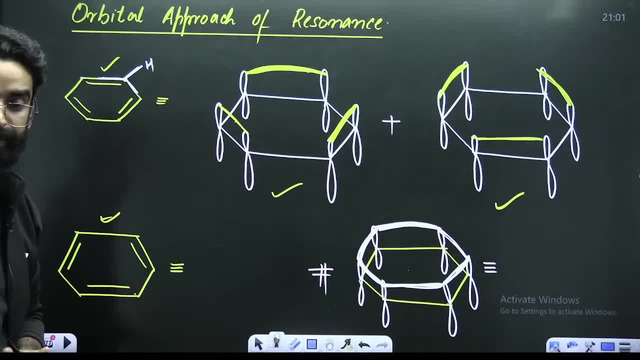 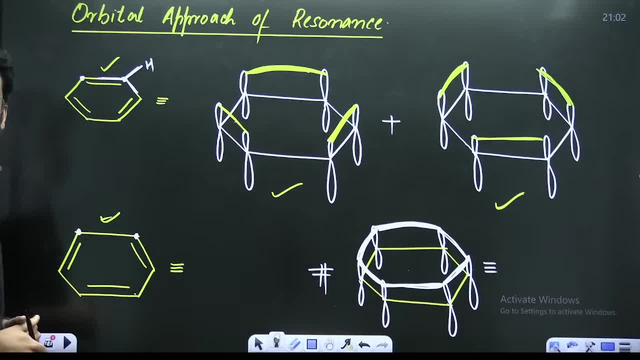 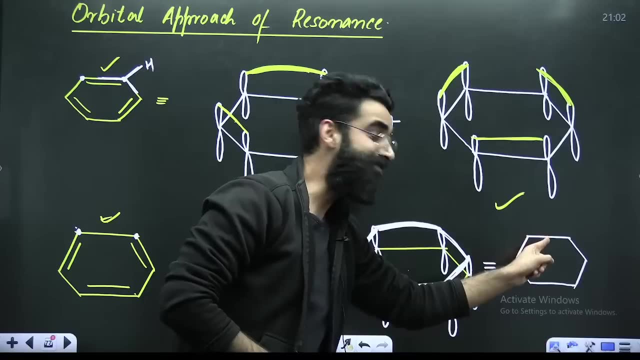 As per this structure, there should be single bond between these two atoms. So, merge the information, Merge the information, Merge the information. This structure is telling you there should be a double bond between these two. This structure is telling you there should be a single bond between these two. 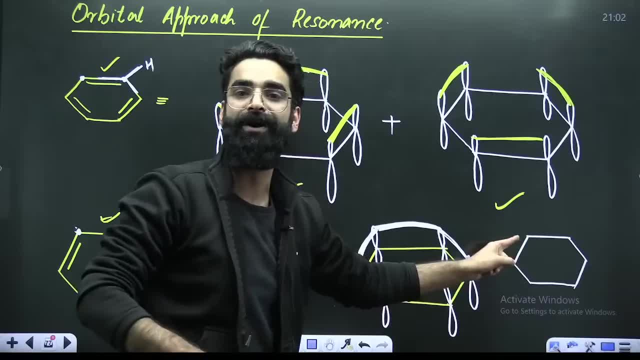 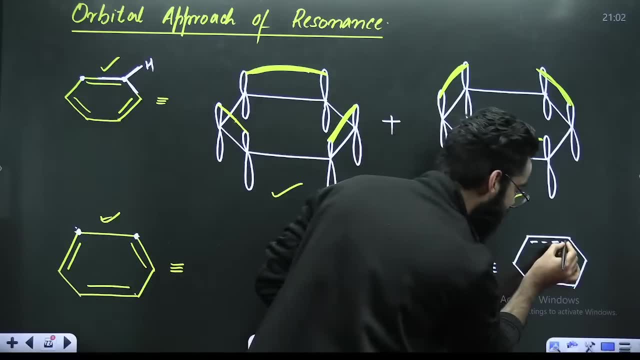 But in the actual structure it will be neither pure single bond nor it will be pure double bond. It will be partial double bond here. It will be a partial double bond here. Similarly, in the actual structure it will be partial double bond here. 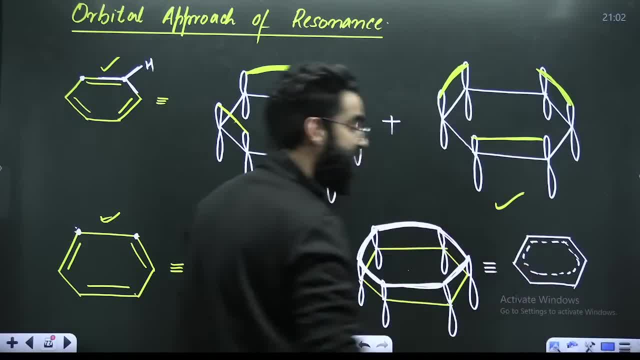 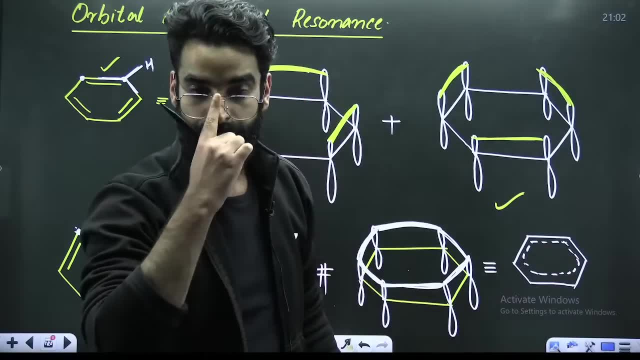 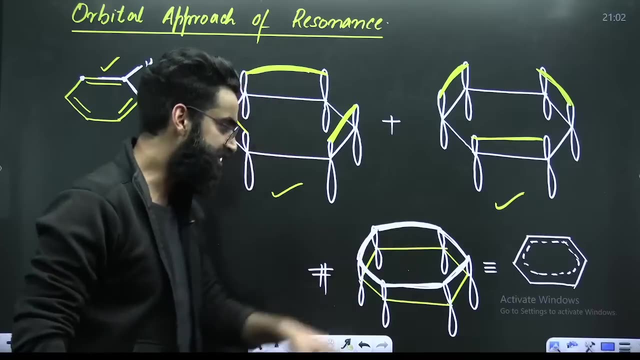 In the actual structure. it will be partial double bond everywhere. It will be partial double bond everywhere. That is the reason why in benzene bond lengths are equal. That is the reason why in benzene all the bond lengths are equal. Got it, My dear students? this particular structure is what you call as the actual structure. 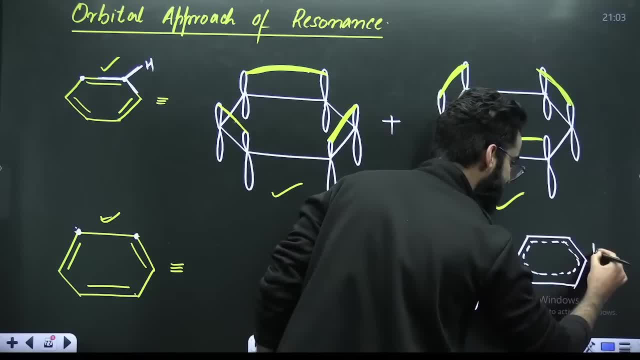 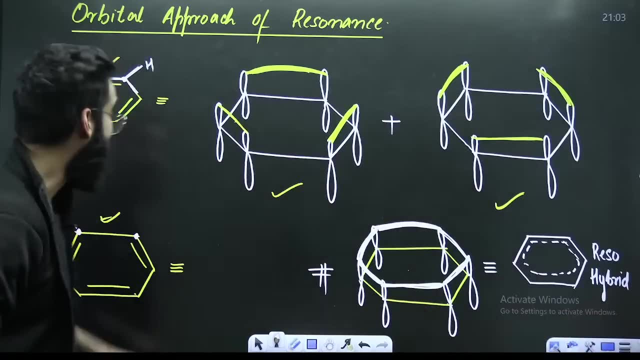 of benzene, or you can call it as the resonance hybrid as well. This actual structure of benzene is something which you call as a resonance hybrid, Resonance hybrid And these particular structures, these are the proposed structures which we have about benzene. right, This is. 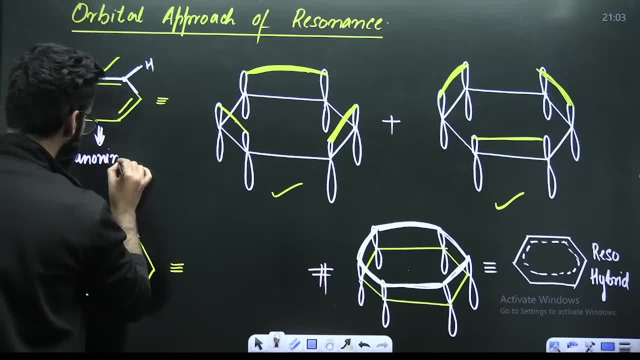 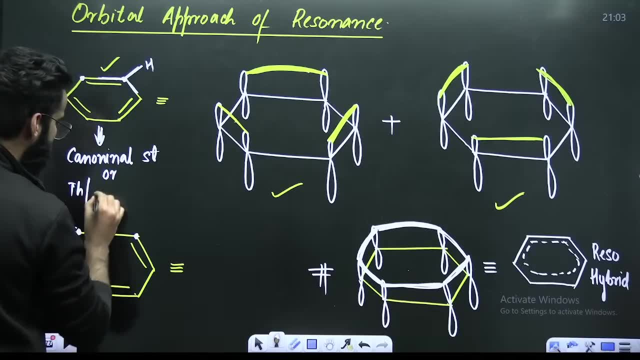 something which we call as canonical structures. This is one of the canonical structure, of benzene, or you can call it as the theoretical structure, or you can call it as the resonating structure, Perfect. Similarly, this one, This either you will be calling as canonical structure. 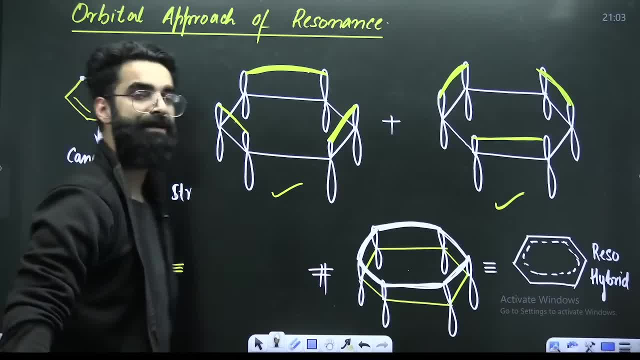 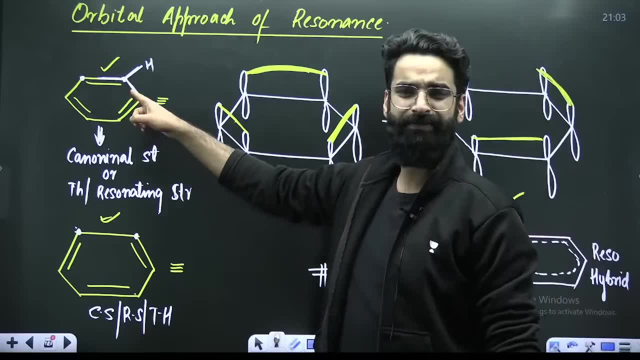 or resonating structure, or theoretical structure. Now you tell me one thing which is very important here, One thing which is very important. Why did you say this, students, in this canonical form? if i ask you, if i ask you whether the bonding is localized or 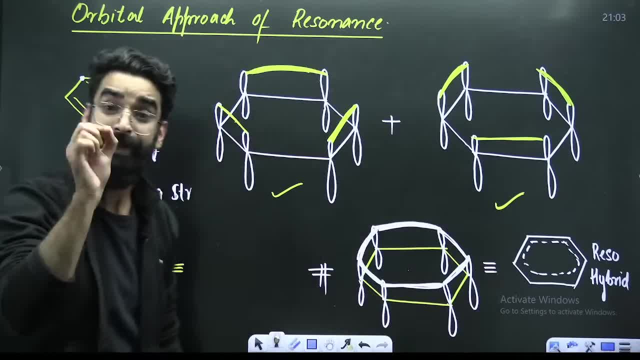 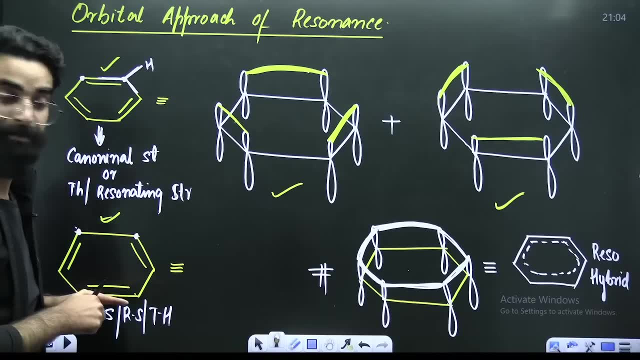 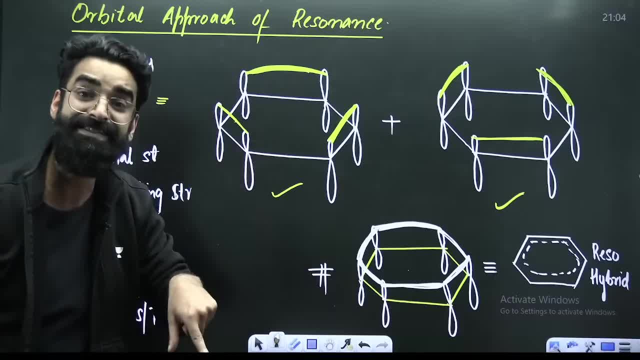 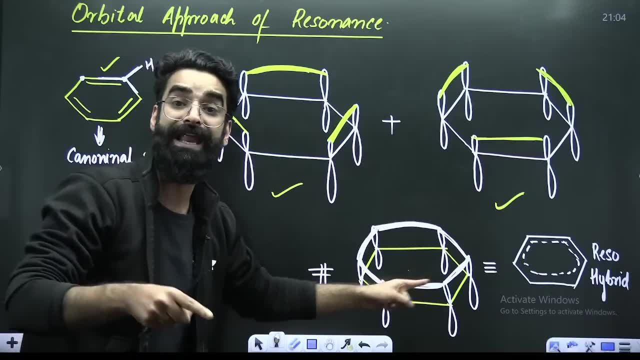 it can be here. so where is the delocalization actually present? is the delocalization present in the canonical form or is the delocalization present in the hybrid? delocalization is present in the hybrid right. delocalization is the present in the hybrid. 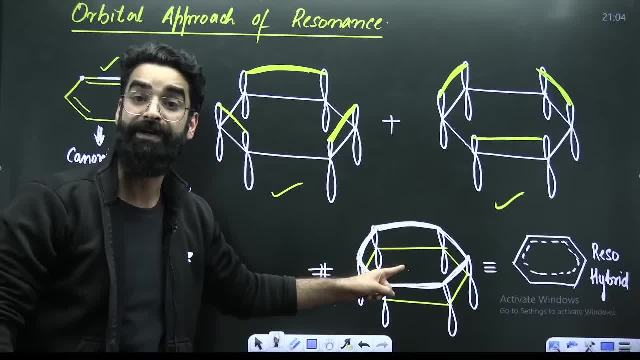 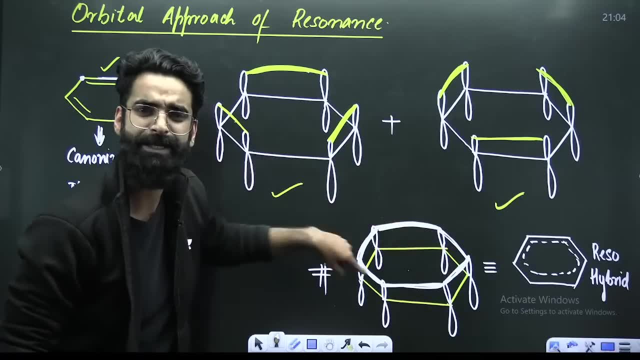 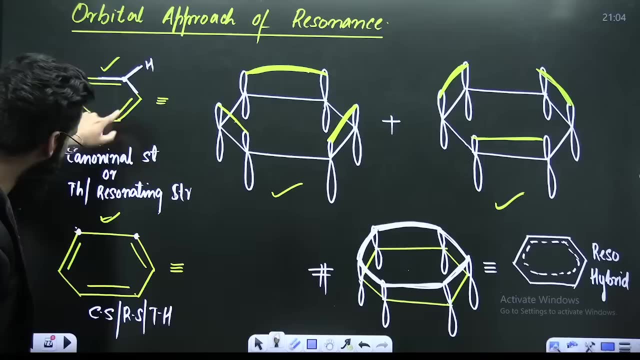 got it. delocalization is present in hybrid. you cannot say with 100 probability that your pi electron pair is here or here, or here or here, it is delocalized, it is delocalized. but here, in this proposed structure, in this canonical form, you can categorically say: your pi bond is here, pi bond is a pi bond is similarly here. 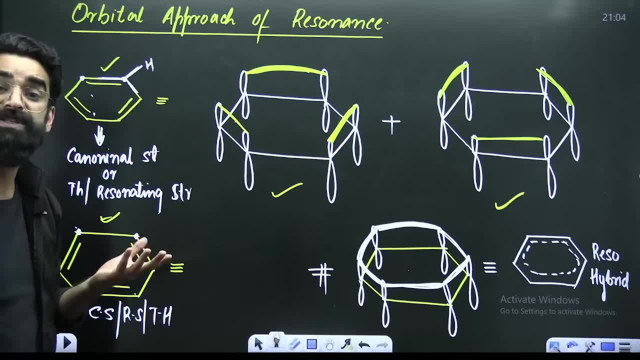 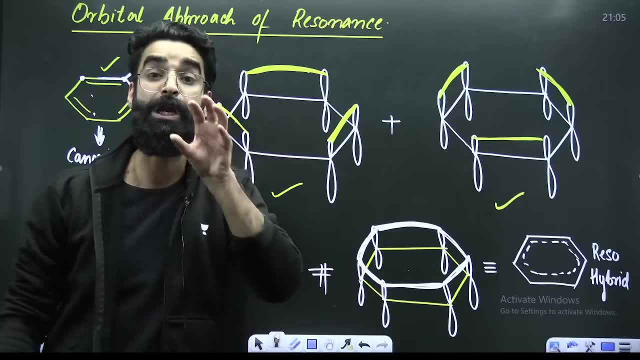 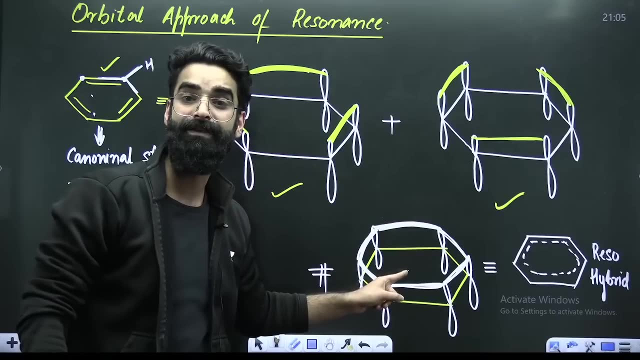 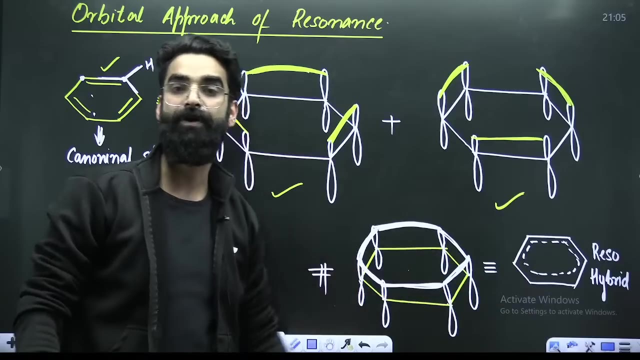 pi bond is here, pi bond is a pi bond is here. so those proposed structures, those proposed structures which give you, which give you the idea about the localized bonding, those proposed structures are what we call as canonical structures. but this particular structure, this particular structure, what does it contain? it contains delocalization of pi electrons, and this is something which we call us. 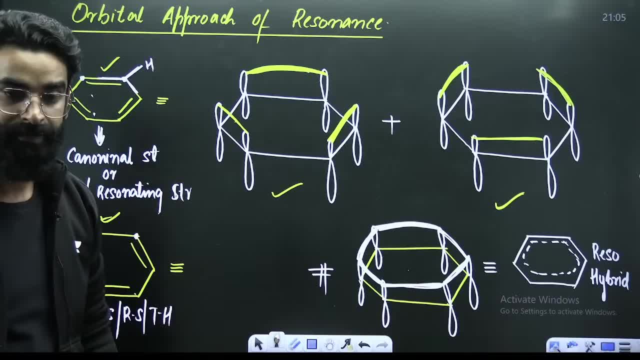 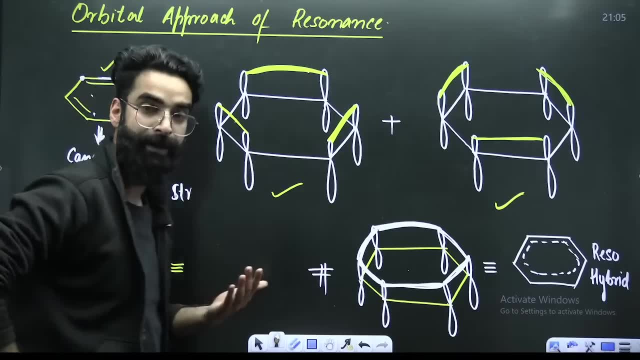 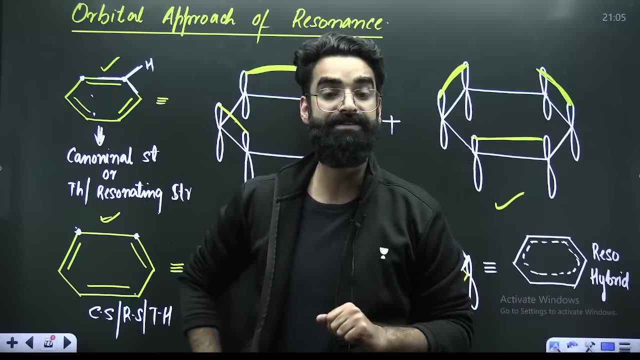 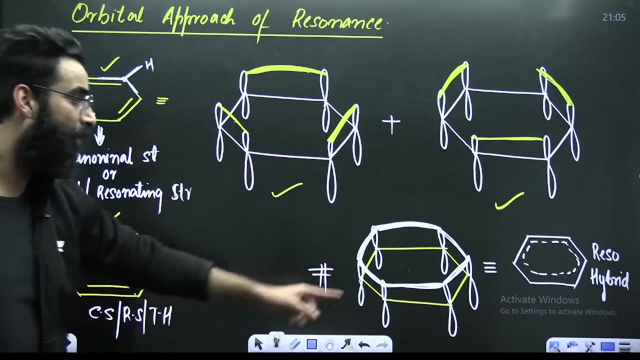 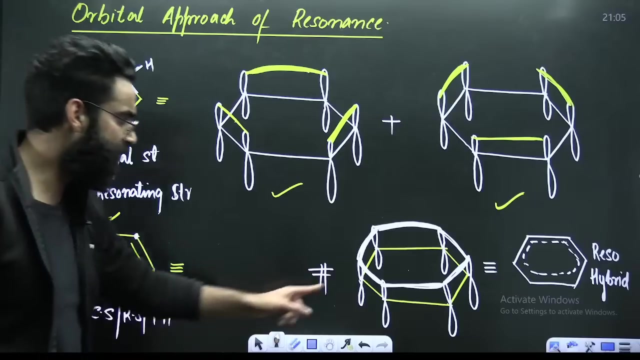 some一下. is this clear? is this clear? people say yes or no in the charts if you've got to know this. so, from now onwards, if i ask you, is delocalization present in the hybrid or delocalization is present in the canonical structure, Right? So, my dear students, the partial overlap of these p orbitals, the partial overlap of these, 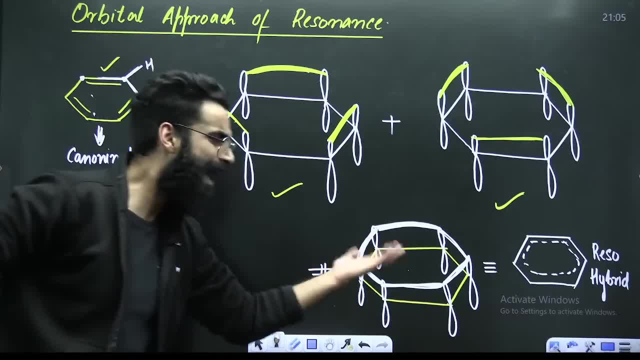 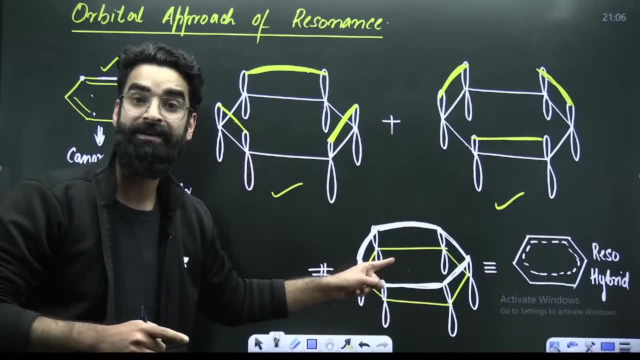 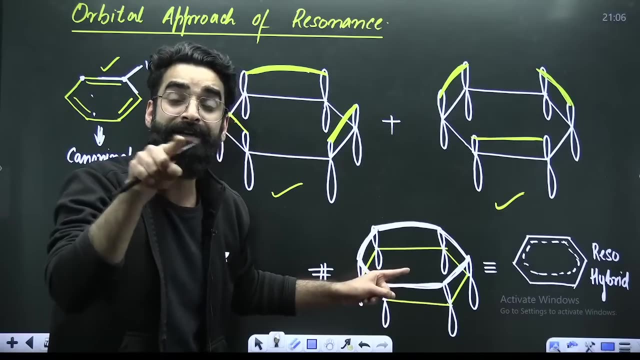 p orbitals is something which we call as resonance. Now, what happens due to resonance? if I ask you What happens, What is the consequence of resonance, My dear students? due to resonance, what is the resonance? Delocalization. Due to delocalization, will the pi electron density 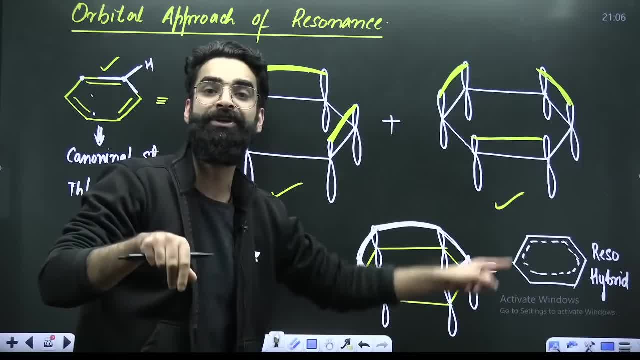 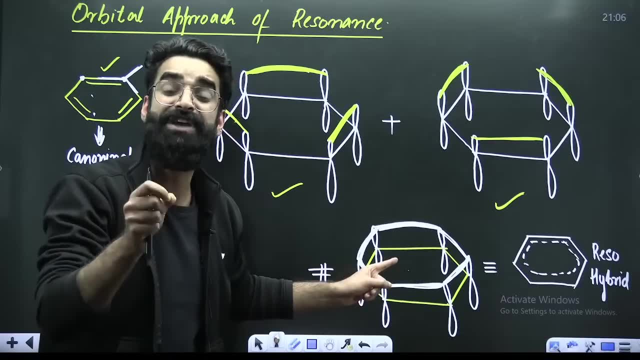 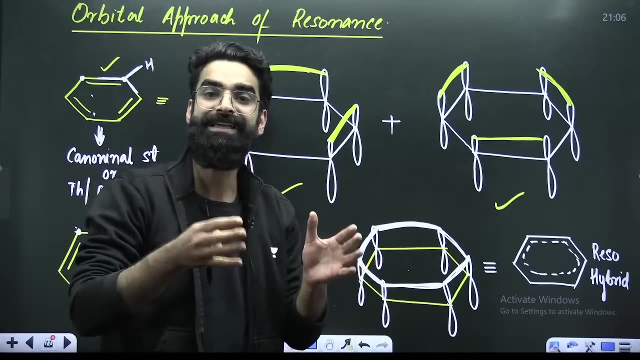 be subjugated to only two nuclei or more than two nuclei. I will say, due to delocalization, pi electron density it will be subjected to, it will be subjected under the influence of more than two nuclei If the pi electron density is subjected, is subjected to more than two nuclei. 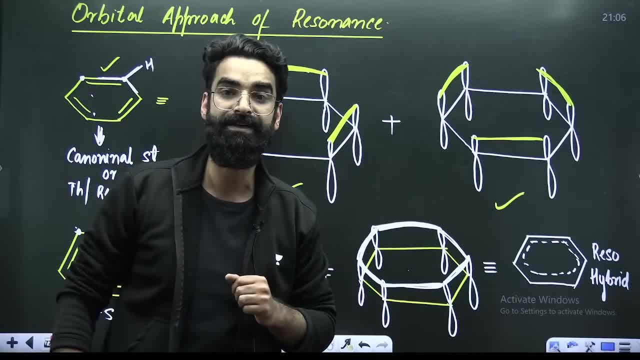 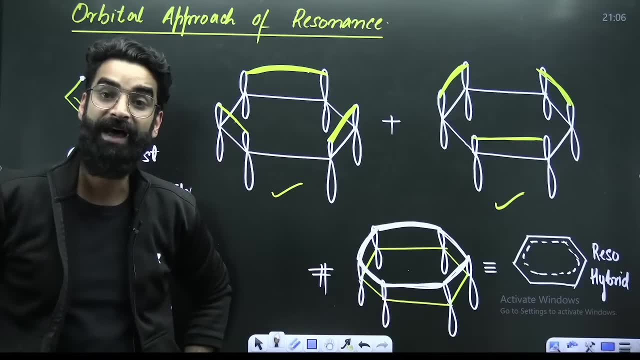 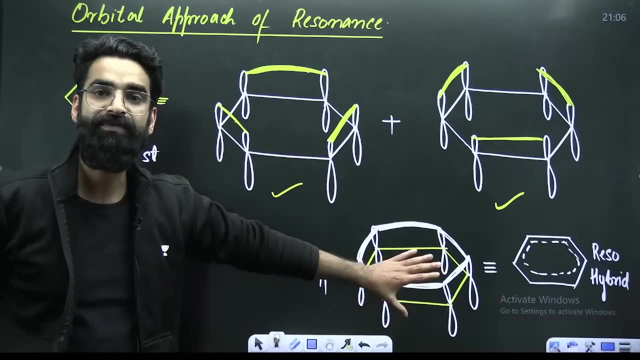 what will happen? Force of attraction on the electron density will increase If force of attraction increases. if force of attraction increases, if force of attraction increases, what will happen? Will stability increase or decrease? Force of attraction increases means energy decreases. Energy decreases means stability. 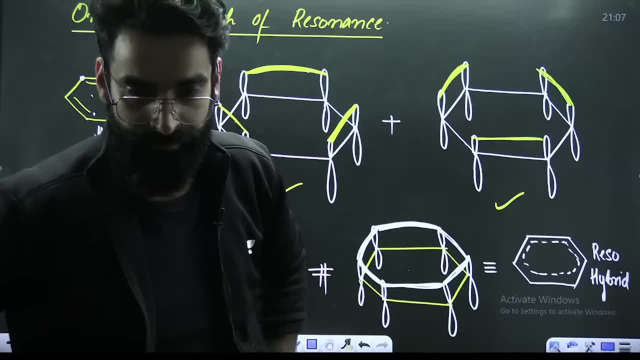 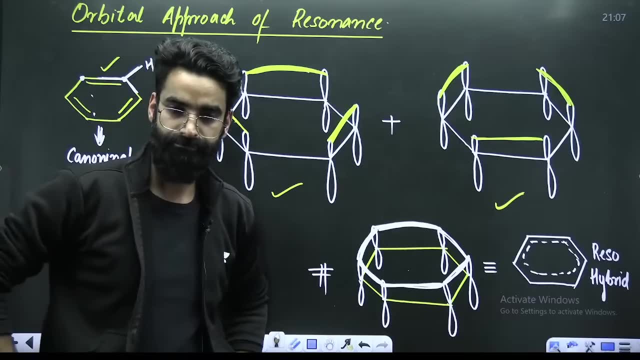 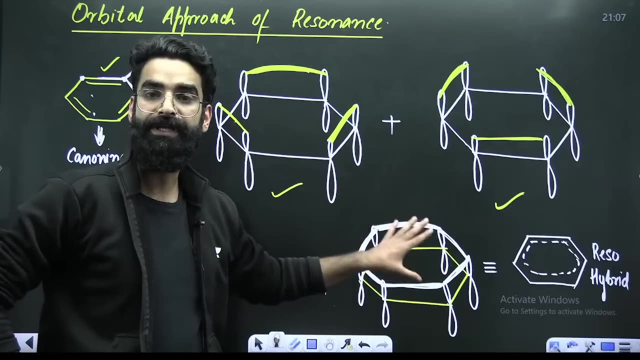 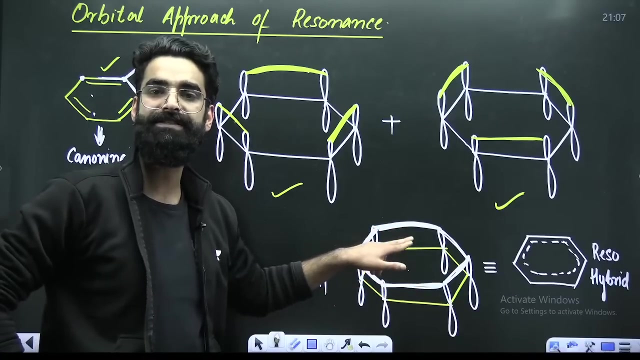 increases. Do you remember this? Yeah, Okay, guys. So, in short, what happens when the energy decreases Due to delocalization, Due to delocalization of these pi energy electrons, due to delocalization of these pi electrons, due to the delocalization of this pi electron density? I would say this: 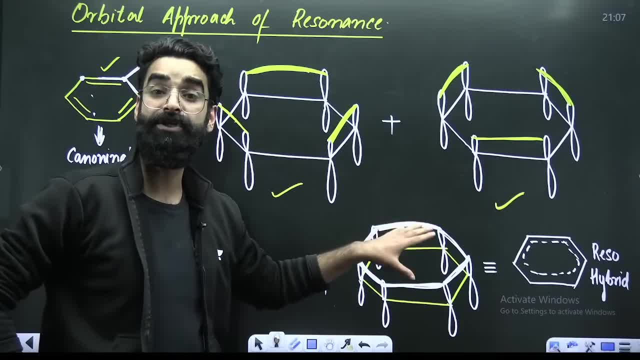 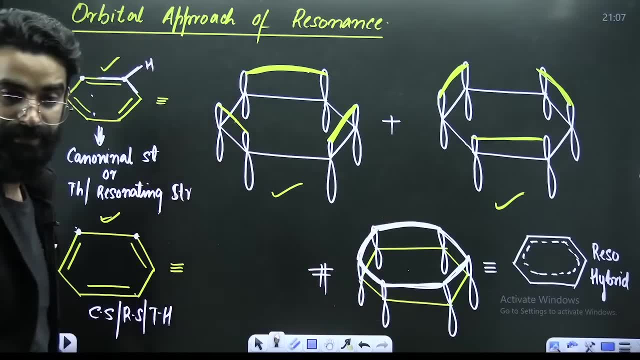 pi electron density. it comes under the influence of more than two nuclei, due to which force of attraction increases. If force of attraction increases, energy decreases and stability increases, Right, Perfect. That is the reason if delocalization is in this particular hybrid. 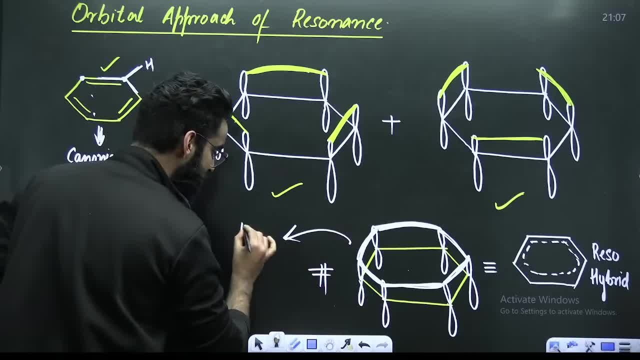 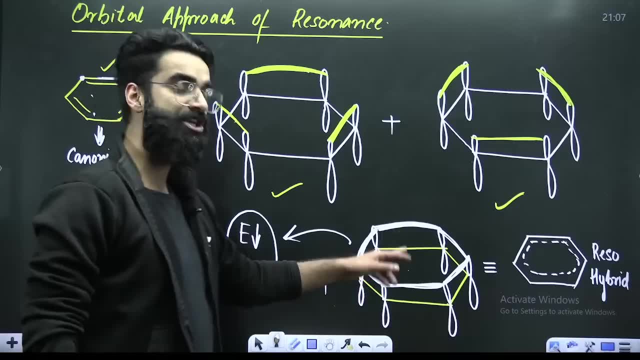 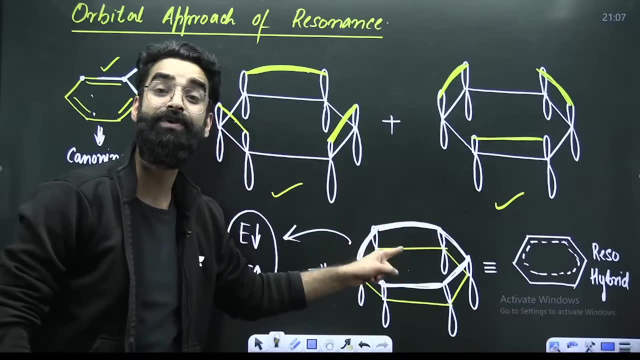 if delocalization is here, that means its energy will be the least and its stability will be the maximum, Right? So do remember: energy of the resonance, hybrid, is the least and its stability will be maximum, because over here resonance is present, Over here delocalization is present. Among these two, 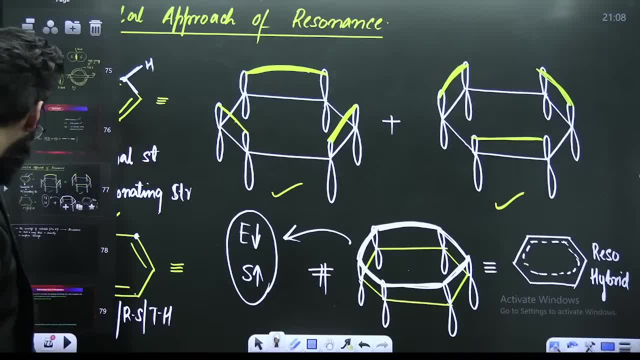 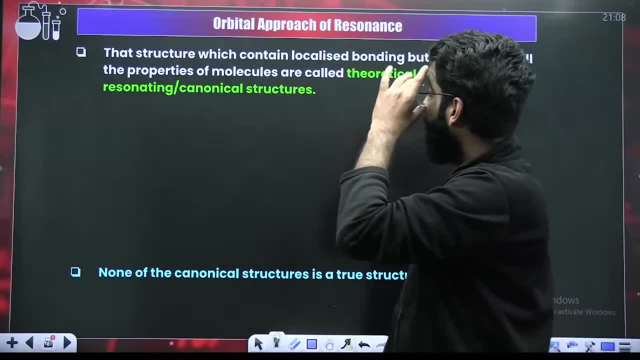 resonance is not present, Delocalization is not present. I hope this is clear. I hope this is clear. So so, guys, in nutshell, in nutshell, have a look. That structure which contains localized bonding, that structure which contains localized bonding. 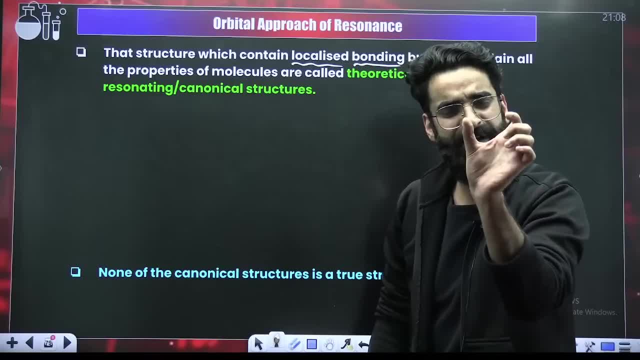 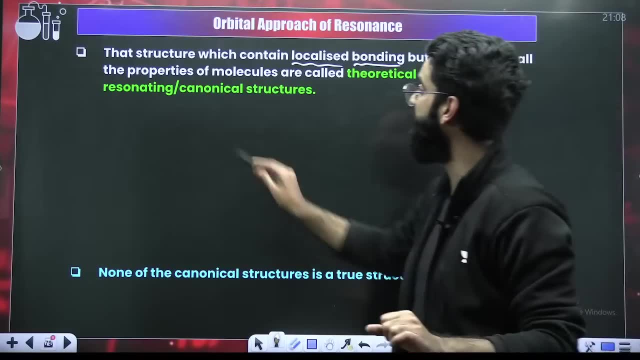 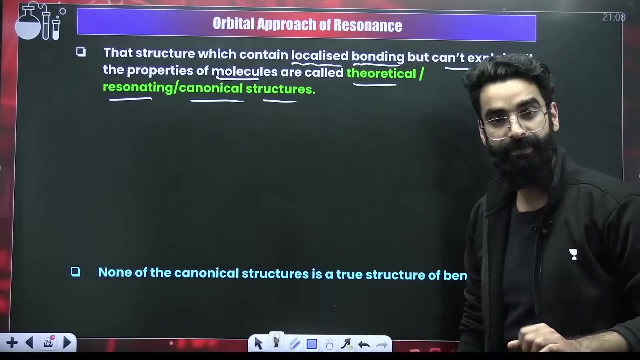 wherein you can clearly say that pi electron is between these two carbons. Pi electron is between these two carbons, So that structure which contains localized bonding but cannot explain all the properties of the molecule. that's what you call as theoretical structure, or resonating structure, or canonical form. Or canonical form, Okay, Or canonical form. 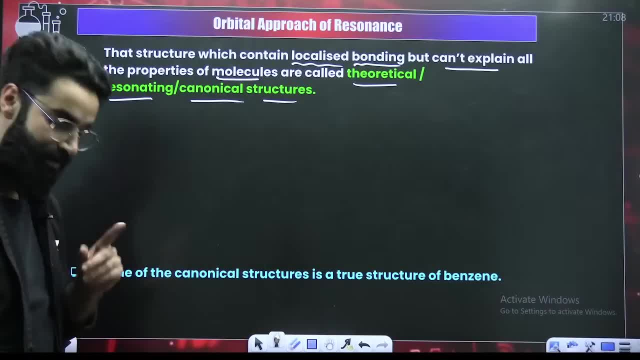 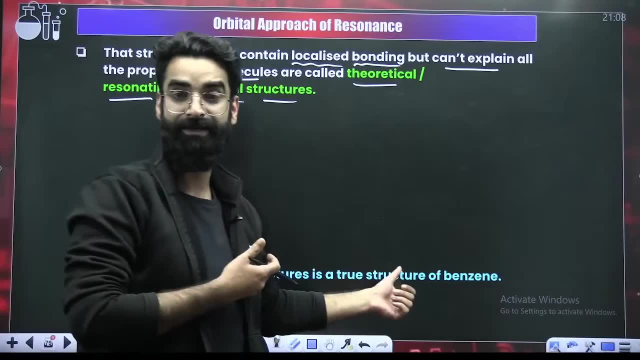 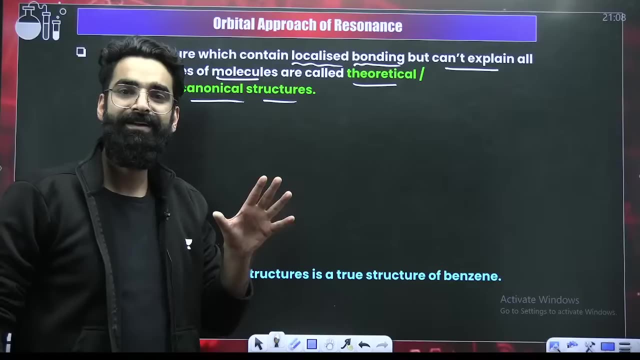 Perfect, Right. Okay, One more thing. Look at this particular statement. None of the canonical structures is the true structure of the molecule. You saw it. None of the canonical structure is the actual structure of the molecule. Perfect, It is just. it is just from the canonical structures We get. 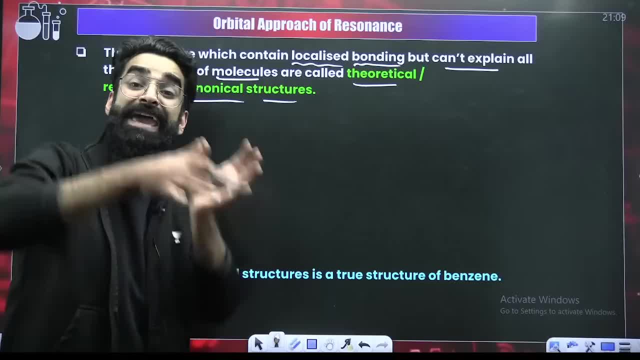 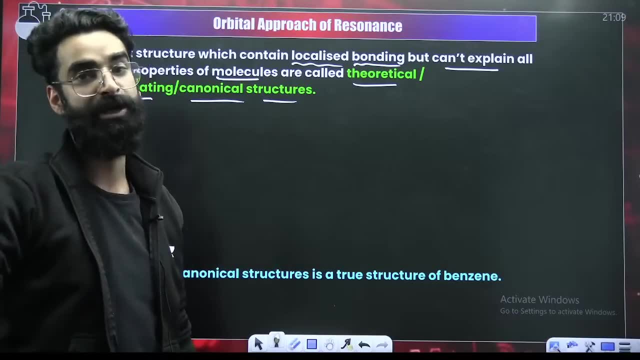 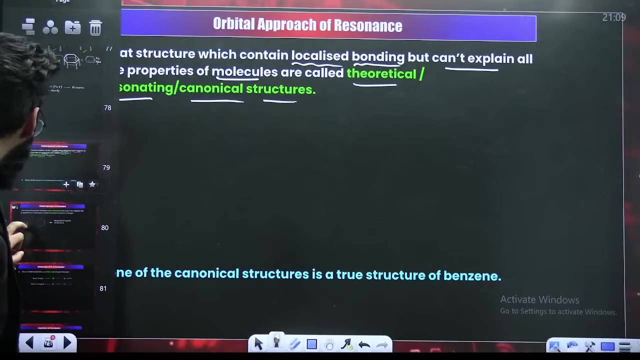 some, some information. We compile that information and make the actual structure of the molecule, which is something you call as a resonance hybrid. And in that resonance hybrid, basically, your delocalization is present, Your resonance, the bond is present. And due to delocalization, due to delocalization, as I told you, due 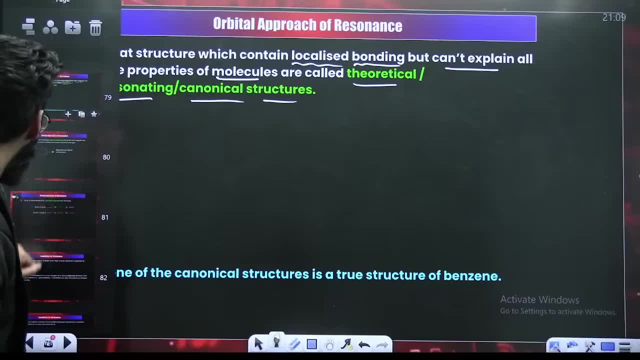 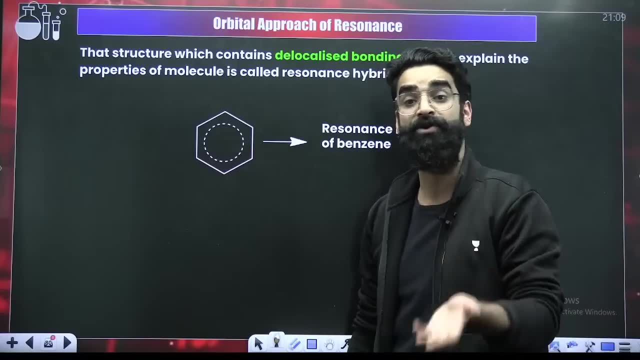 to delocalization. what happens Due to delocalization? what happens? The high energy electrons. they come under the influence of more than two nucleol, due to which force of attraction increases, Energy decreases, stability increases. As simple as that, Right. 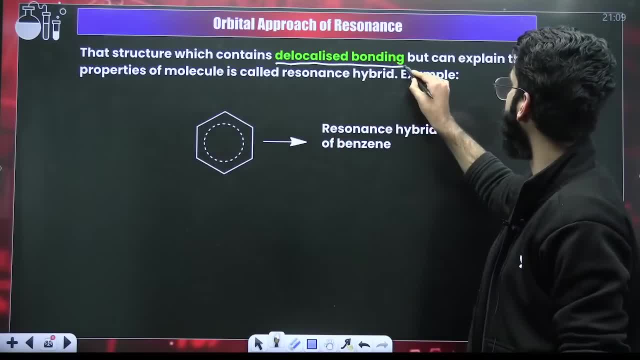 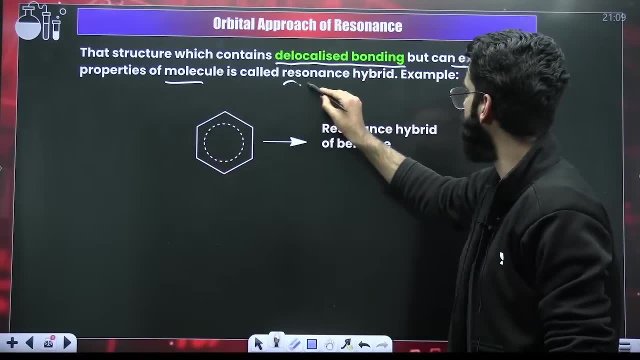 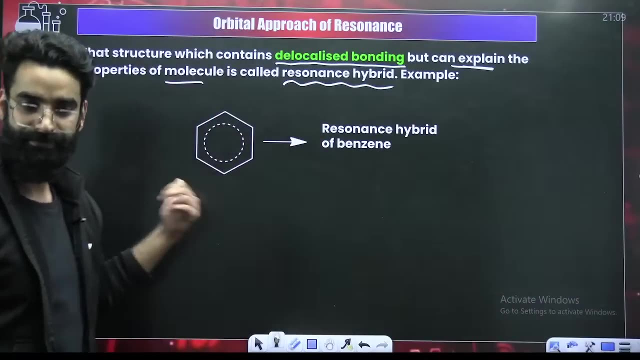 So the structure which contains delocalized bonding but can explain The structure which contains delocalized bonding can explain the properties of the molecule- is something which you call as a resonance hybrid. so this is basically your resonance hybrid of benzene. this is the hybrid of benzene. 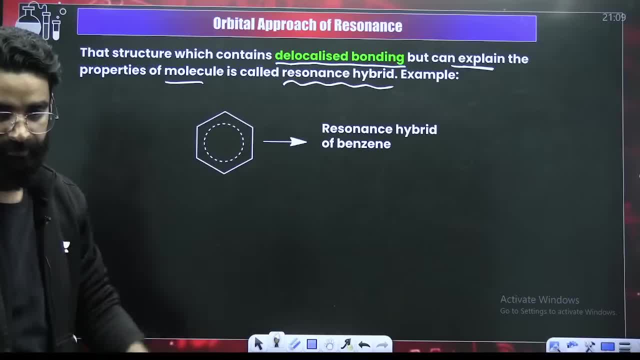 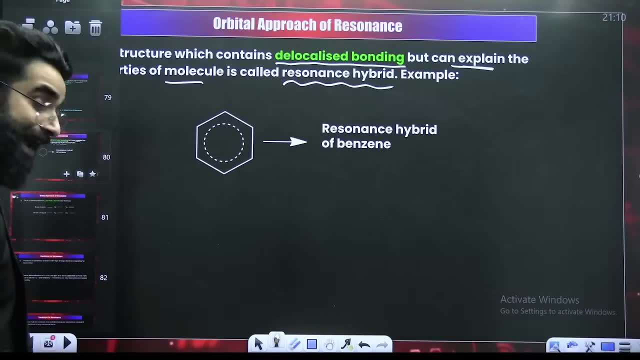 this is the hybrid of benzene. I believe this is clear to everyone. I believe this is clear to everyone. I believe this is clear to everyone. right, perfect. and due to delocalization, what happens? due to delocalization, what happens, can I say? partial pi bonds are formed due. 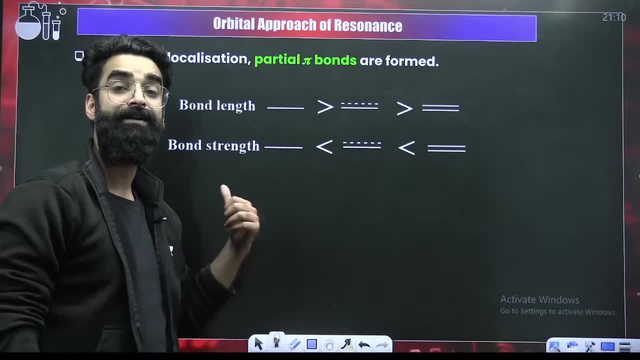 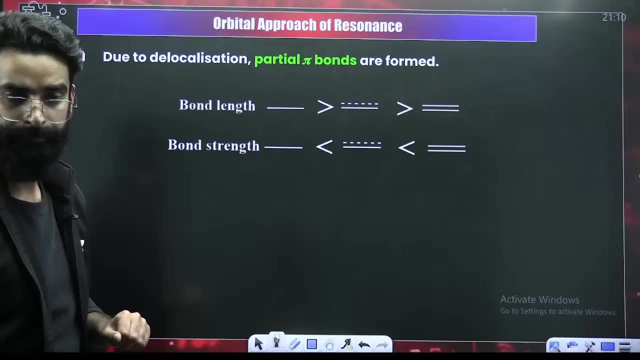 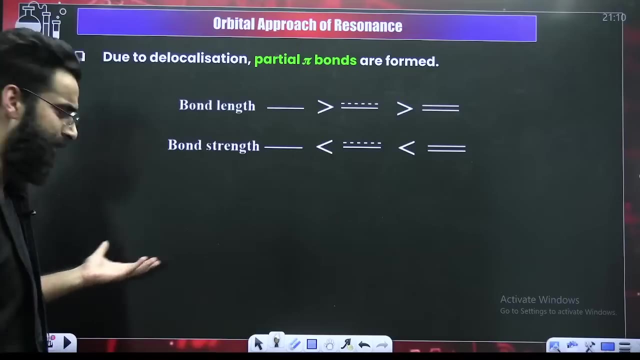 to delocalization. what did you see? what did you see? due to delocalization. what happened? partial pi bonds are formed. right, you saw that. you saw that. okay, partial pi bonds are formed now. my dear students, this is something which is which all of you must be knowing. 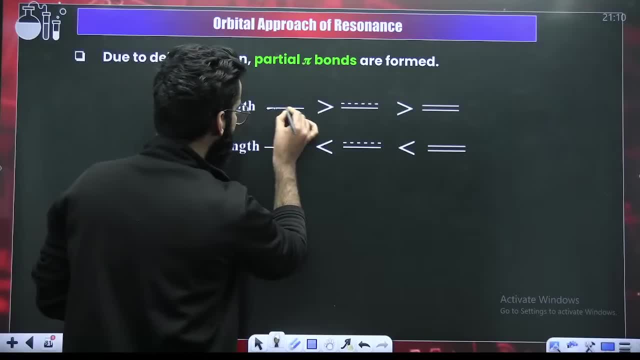 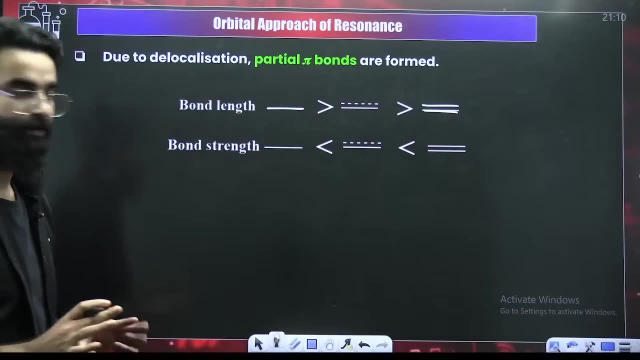 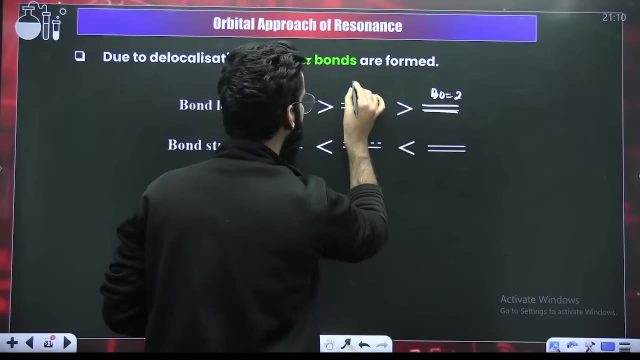 see over here, there is a single bond. it is a pure single bond. it is a pure double bond and it is a partial double bond. it is a partial double bond. I will say: bond is a single bond, so the bond order here will be one. I will say bond order here will be 2 and a bond order. 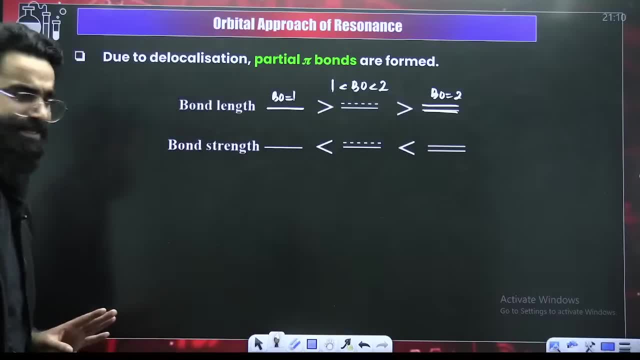 here will be greater than 1 and less than 2, correct? yes, and you know your bond order. it is inversely proportional to bond length, right, perfect. so bond length in case of single bond will maximum, followed by partial double bond, followed by pure double bond, correct? 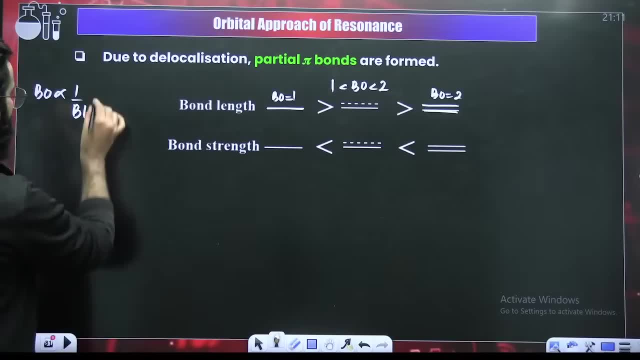 yes, and you know your bond order. it is quickly proportional to bond strength. I will say it will be short creed, correct. but when I will say ituwont, then the pure double bond will abate. want how little. I had to say yes. now you see, the remaining bonds will be 3 by 3, such 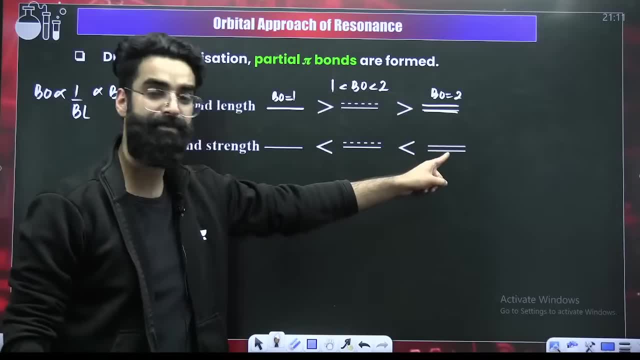 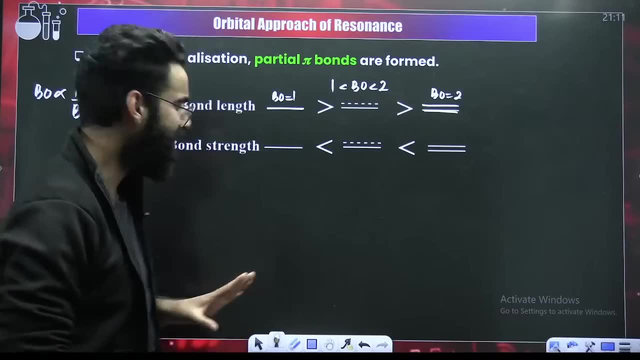 Wherever is the bond order? maximum bond order is maximum here: 2, pure 2.. Its bond strength will be maximum, followed by partial double bond, followed by your single bond Right. All these things will be utilized. All these things will be used in the equations. 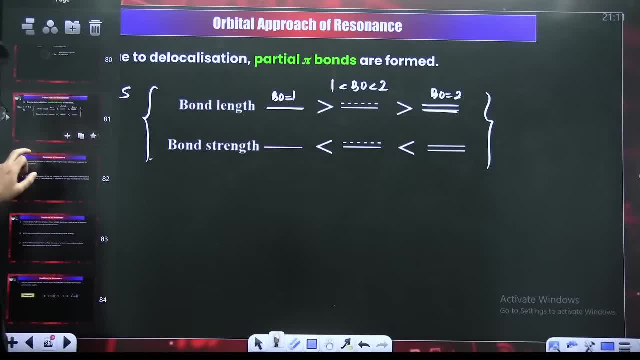 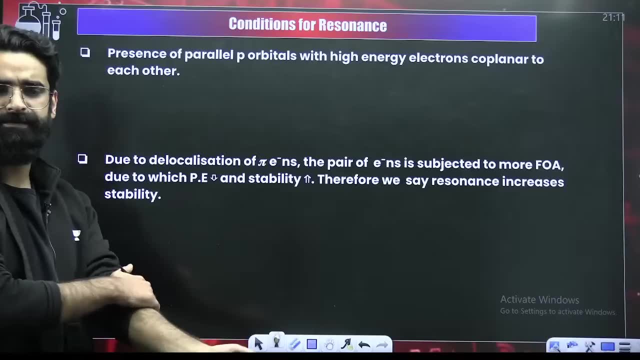 But before doing the equations, there are few more things which I need to tell you related to resonance. If you ask me: what are the conditions? what are the conditions for resonance? What are the conditions for resonance? This is again one more important point. 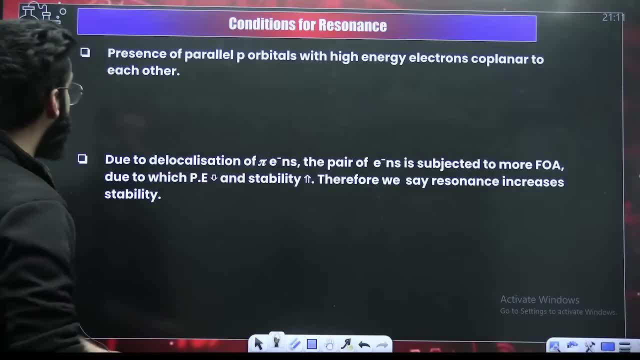 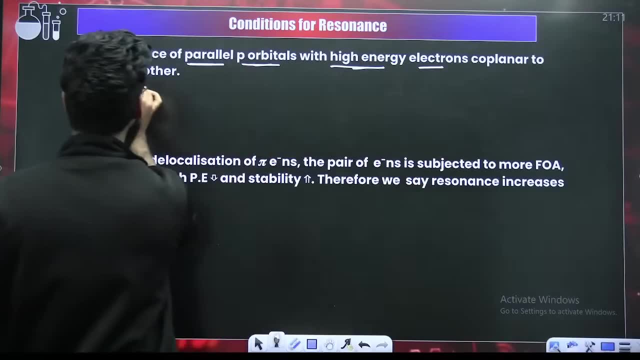 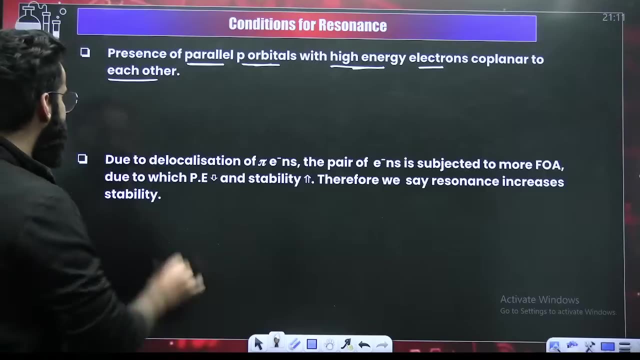 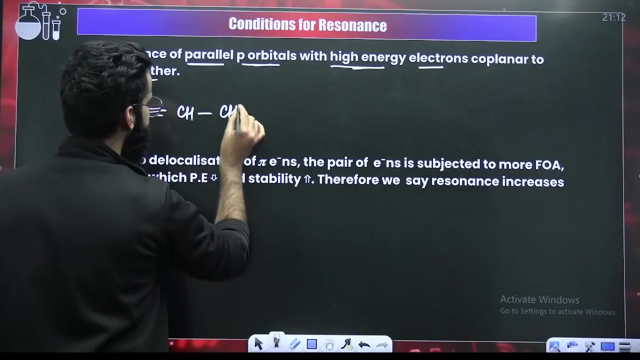 What are the conditions for resonance, My dear students? for resonance, there should be presence of parallel p orbitals with high energy electrons, co-planet to each other, Co-planet to each other, Co-planet to each other. For example, this is CH2, this is double bond, this is CH, this is double single bond, this is CH2 and this is positive. 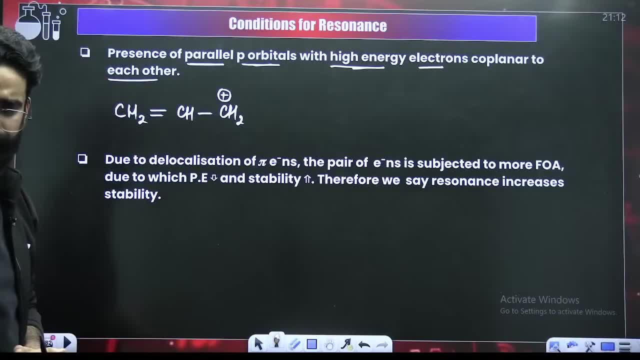 Okay, This is the molecule which I made over here. My dear students, let's try to understand. if you ask me what is the hybridization of this particular carbon? This carbon it's forming how many sigma bonds? 2 with hydrogen, 1 with carbon. 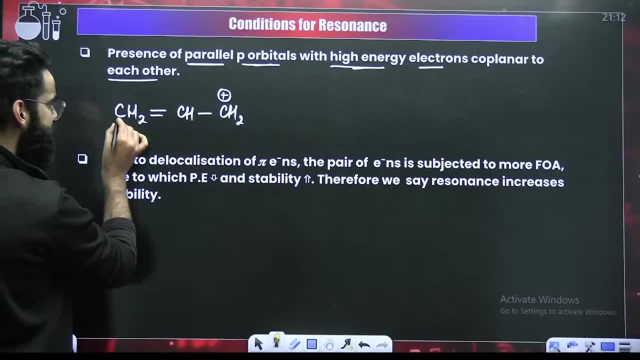 2 with hydrogen, 1 with carbon, 3 sigma bonds. So it is sp2 hybridized. If it is sp2 hybridized, there will be a p orbital. There will be a p orbital, This one. it is also forming 3 sigma bonds, this carbon. 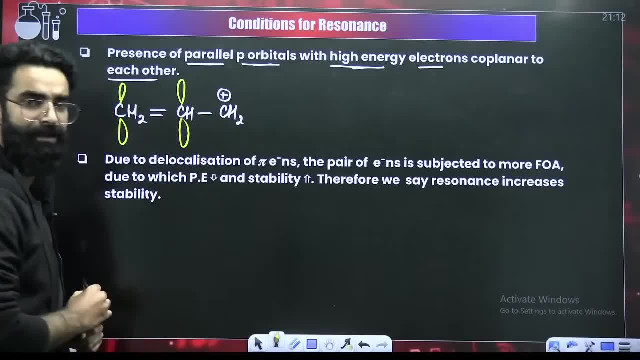 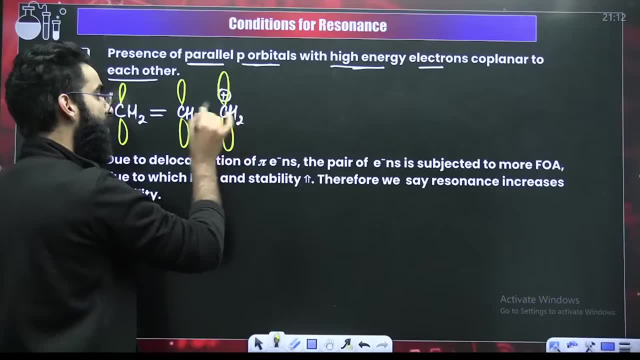 Again, there will be p orbital Right. Perfect. Now look at this particular carbon. It's again forming what It's again forming: 3 sigma bonds. There will be a p orbital here. There will be a p orbital here. 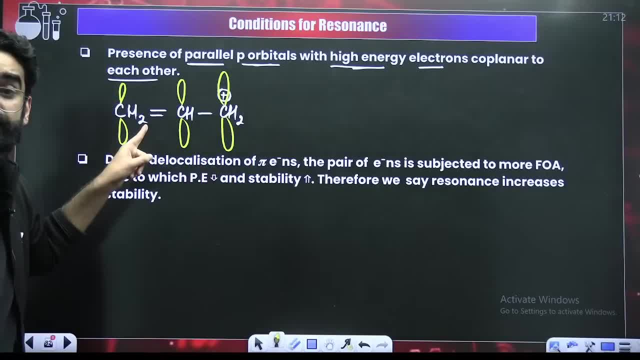 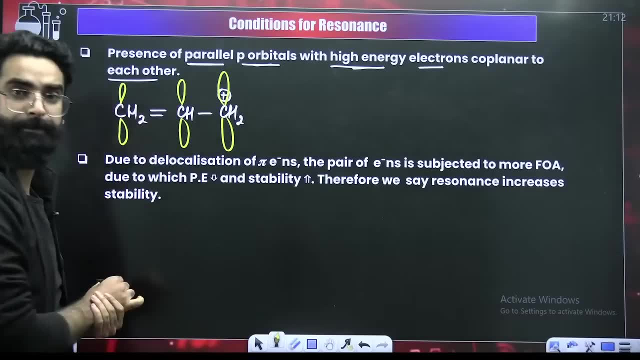 And as for this particular structure, as for this particular structure, which two parallel p orbitals have overlapped, These two parallel p orbitals have overlapped and they have formed a pi bond. They have formed a pi bond. Right, Can you draw? it's one more structure. 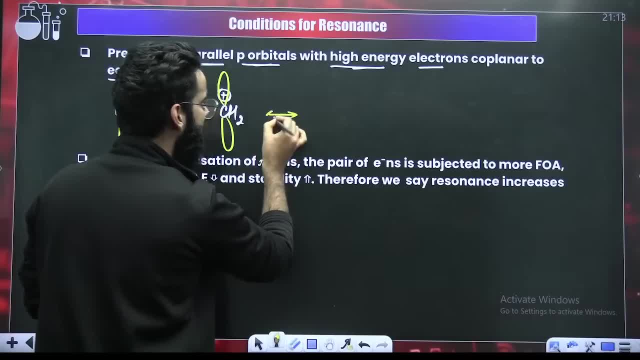 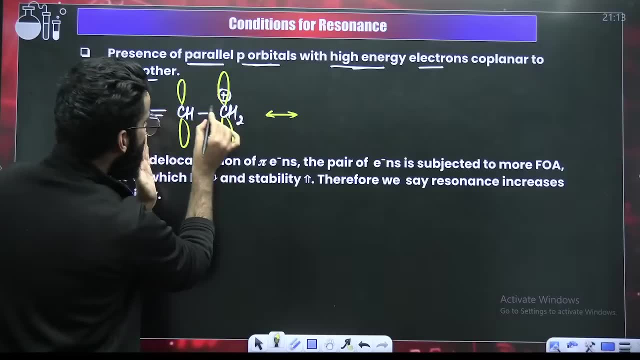 In it. see, this is one of the canonical forms, It's one more canonical form. How will it look like In one more canonical form? I would say, these two p orbitals would have overlapped, So the pi bond would have been shifted over here. 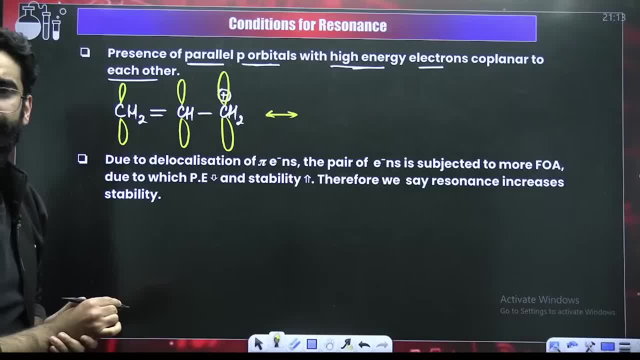 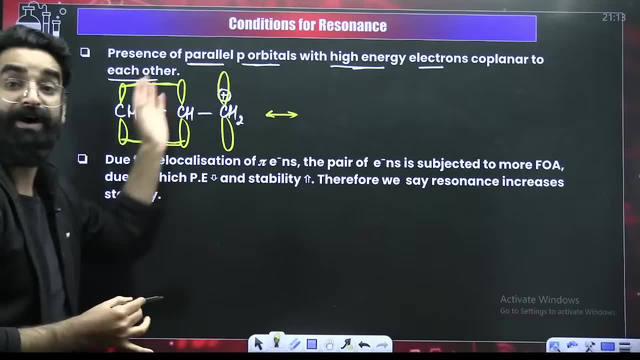 Pi bond would have shifted over here, Correct, Over here. as for this particular canonical form, these two orbitals have parallel overlapped, But in one more canonical form there would have been one more possibility that these two would have overlapped. 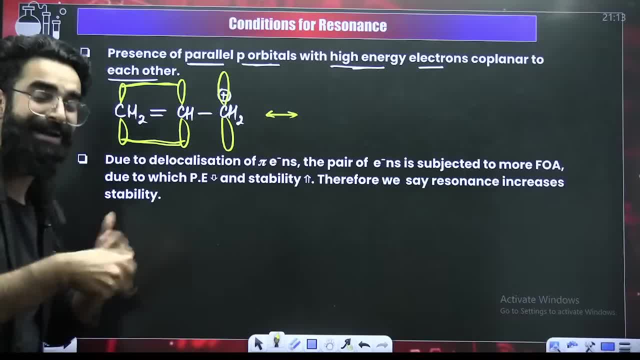 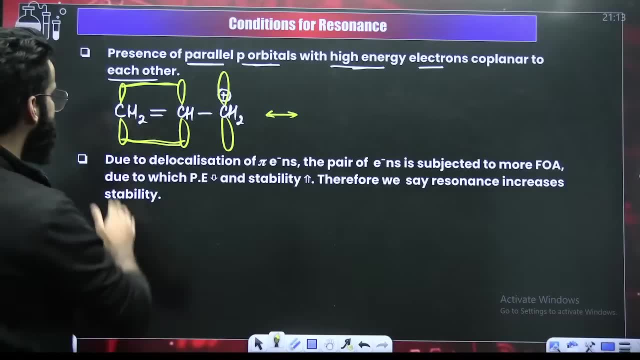 These two would have overlapped, Correct. So what is the condition? basically, Condition is there should be presence of parallel p orbitals with high energy electrons. Correct, Correct. Condition is there should be. Condition is there should be presence of what? 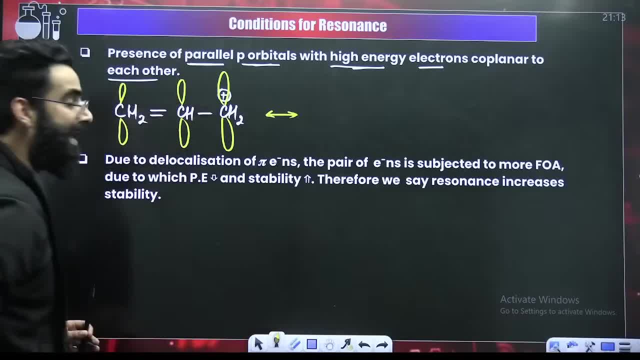 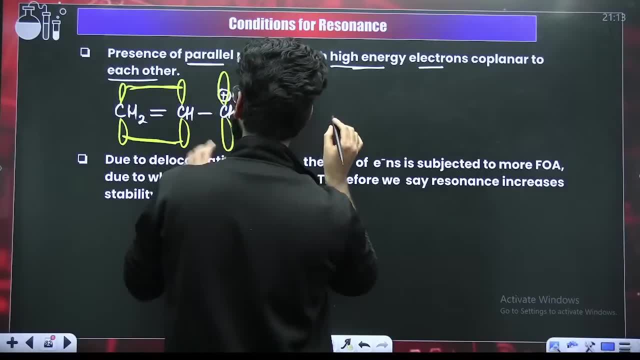 There should be presence of parallel p orbitals with high energy electrons. Like you saw here, these two orbitals have parallel overlapped and formed a pi bond. In one more canonical form I would say these two would have This is CH2.. 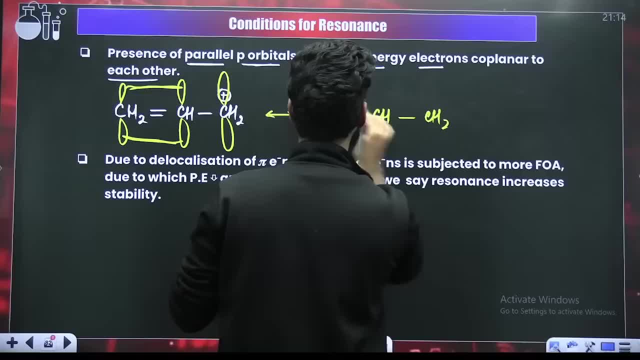 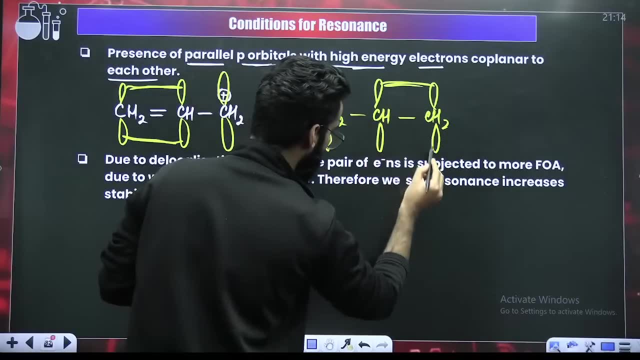 This is CH and this is your CH2.. For example, try to understand what I am going to say. These are the pure p orbitals. So, in one more canonical form, these two would have overlapped parallel. These two would have overlapped parallel. 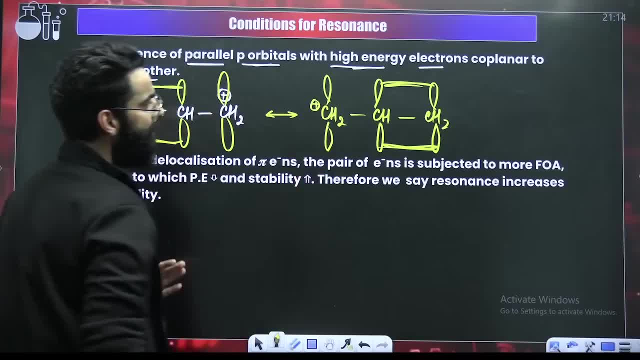 These two would have overlapped: parallel. Perfect, And your pi bond should have been here as per this particular canonical form: Perfect. Now, if I ask you, is this the true structure? Is this the hybrid? This is not the true structure. 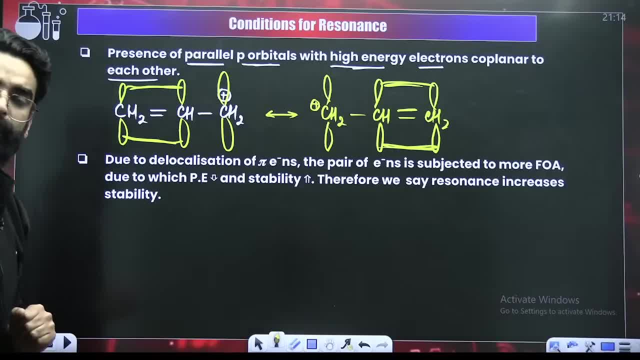 This is not the actual structure of the molecule. Even this is not the actual structure of the molecule. This is giving me some of the information. This is giving me some of the information. If I compile the information, I will get. If I compile the information, I will get the actual structure of the molecule. 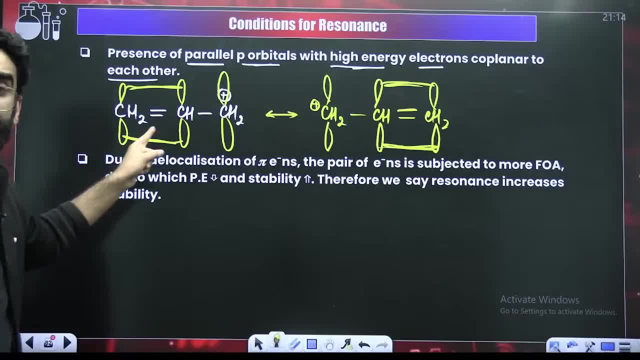 This is giving me some of the information. This is giving me some of the information. If I compile the information, I will get. If I compile the information, I will get the actual structure of the molecule. This is giving me some of the information. 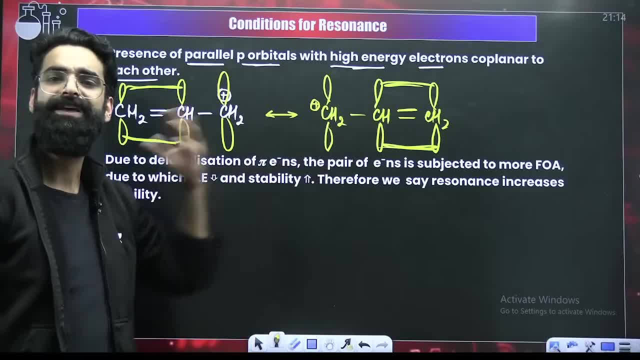 This is giving me some of the information. This is giving me some of the information. If I compile the information, I will get. If I compile the information, I will get the actual structure of the molecule. This is giving me some of the information. 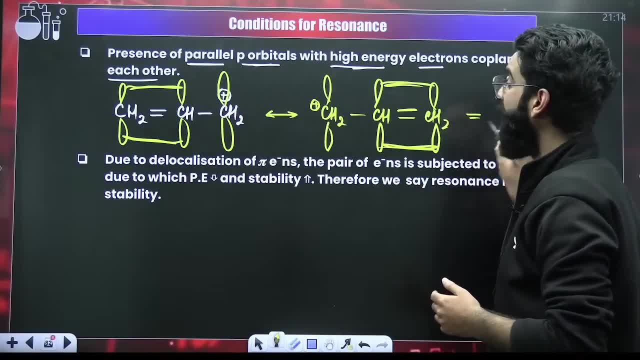 This is giving me some of the information. If I compile the information, I will get. If I compile the information, I will get the actual structure of the molecule. This is giving me some of the information. This is giving me some of the information. 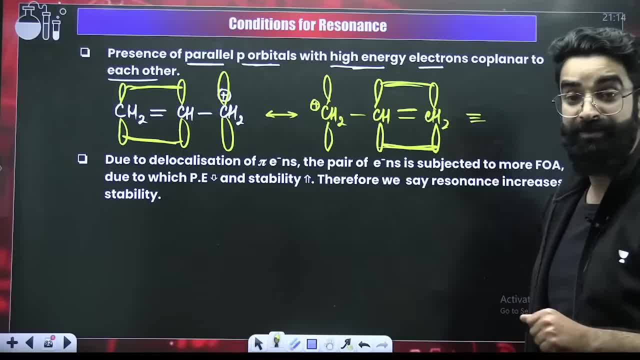 If I compile the information, I will get. If I compile the information, I will get the actual structure of the molecule. This is giving me some of the information. This is giving me some of the information. This is giving me some of the information. 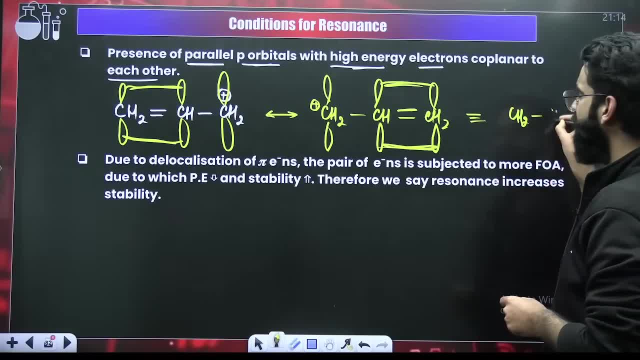 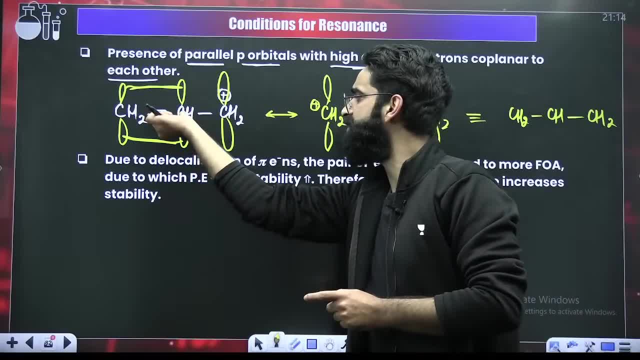 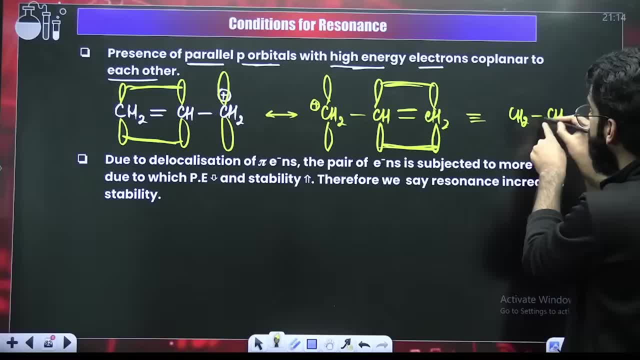 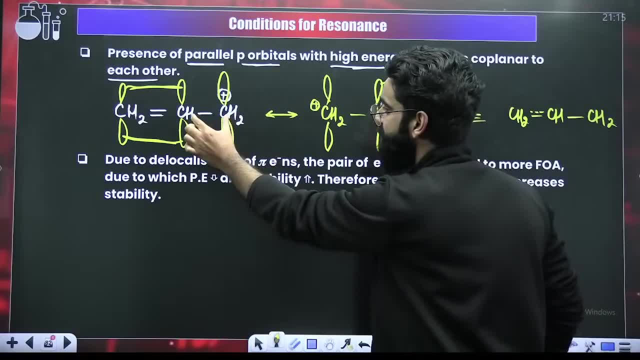 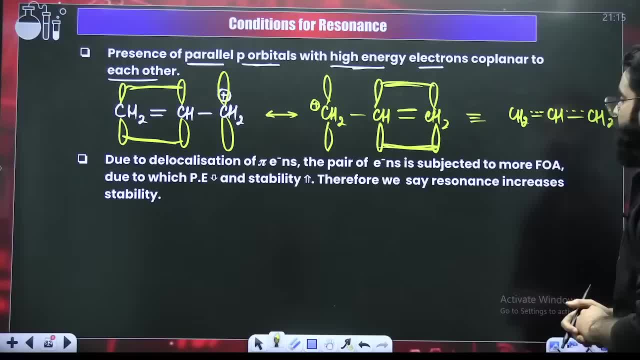 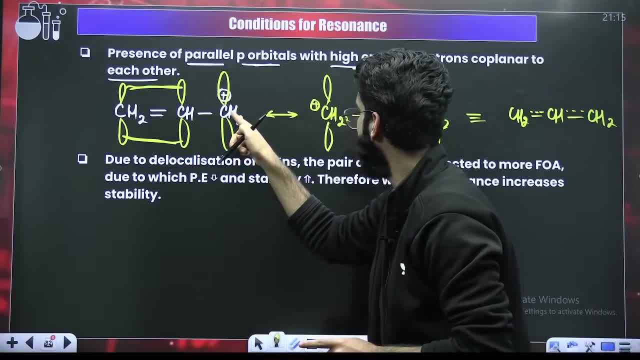 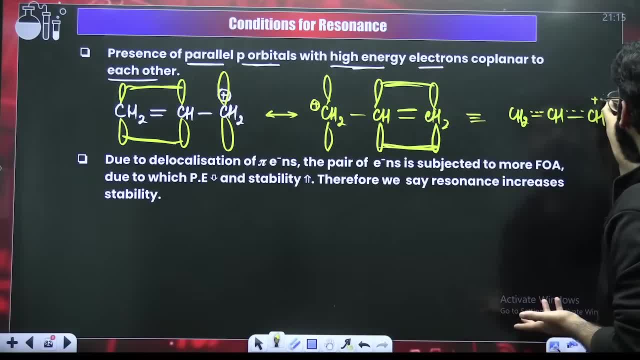 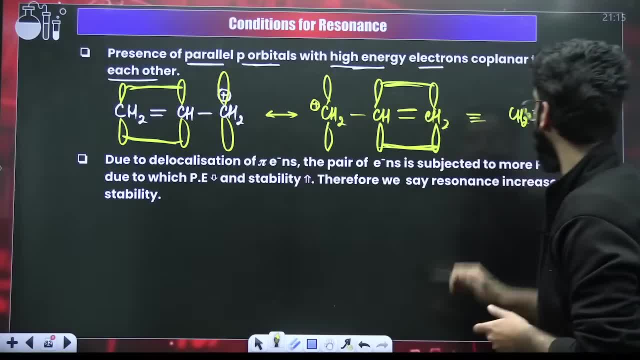 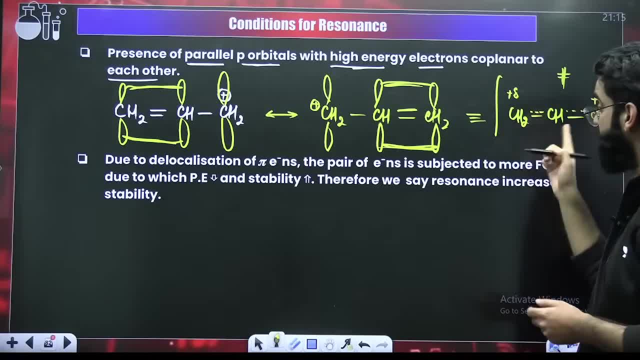 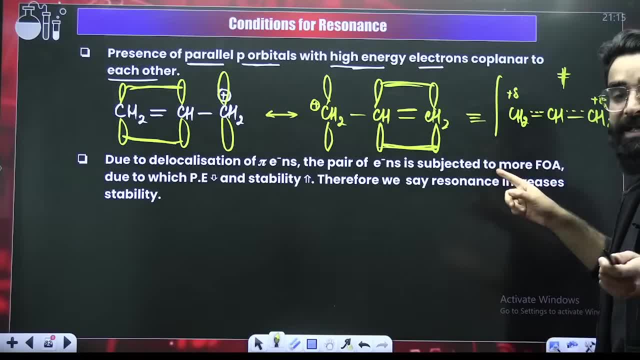 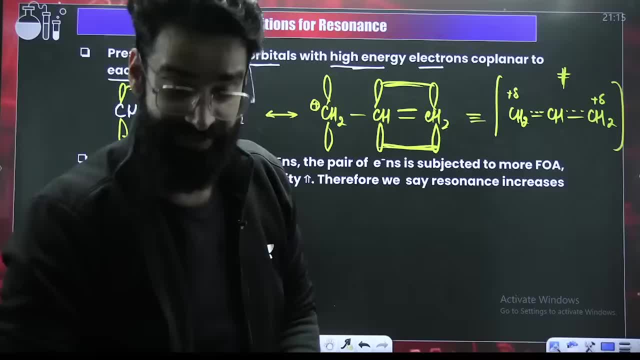 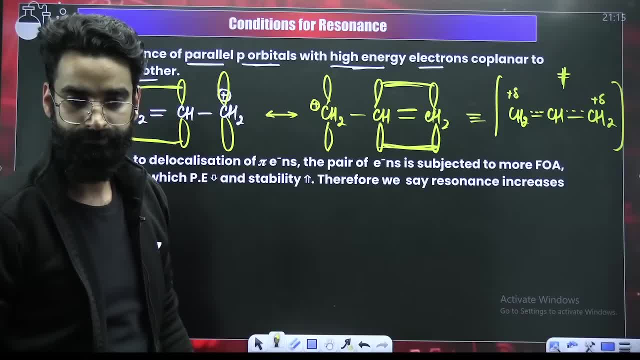 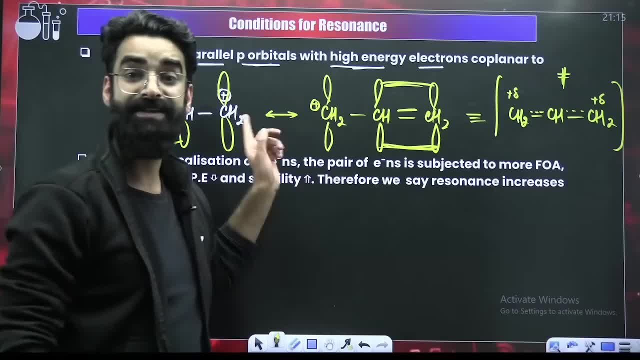 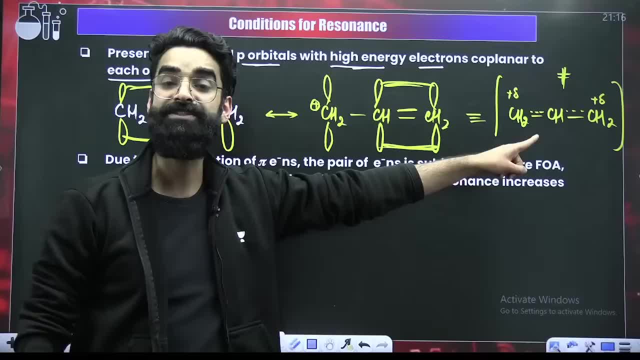 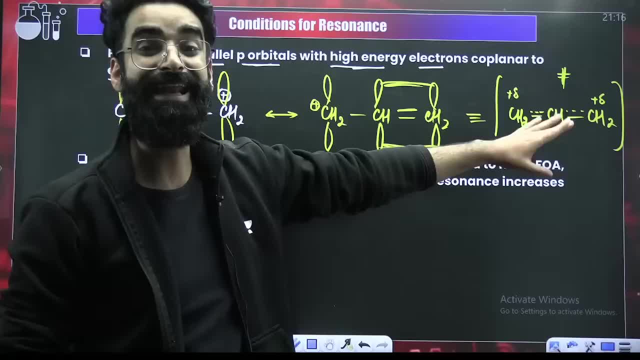 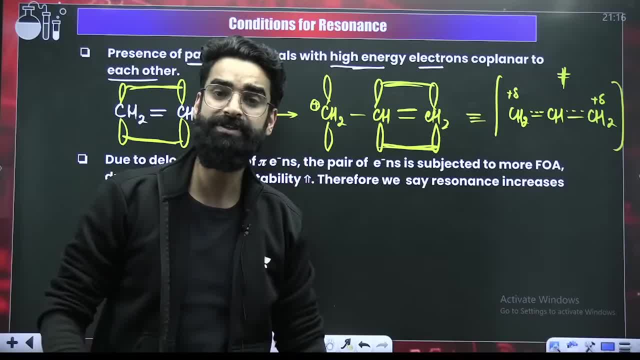 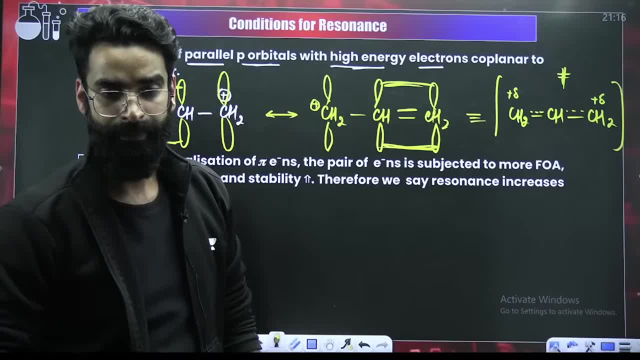 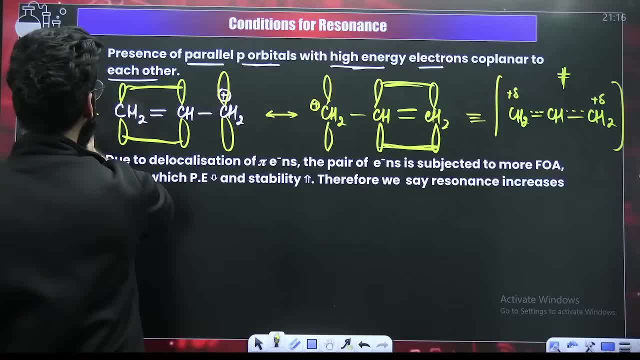 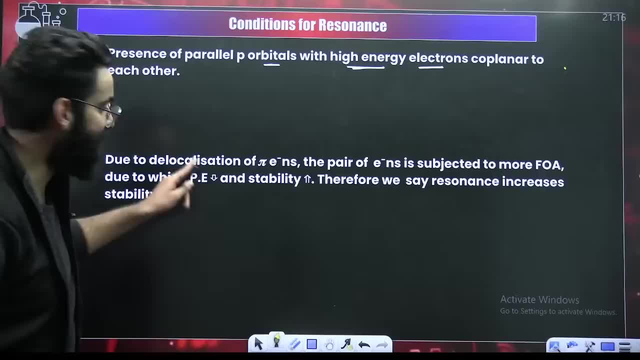 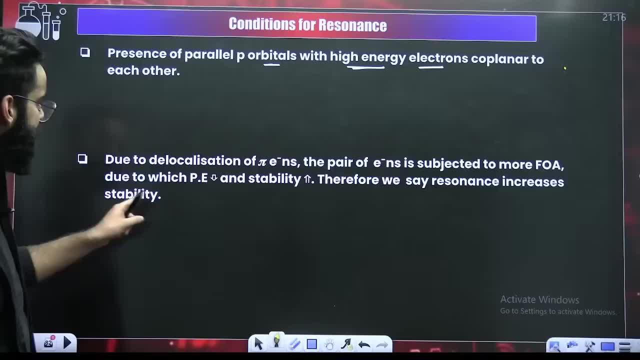 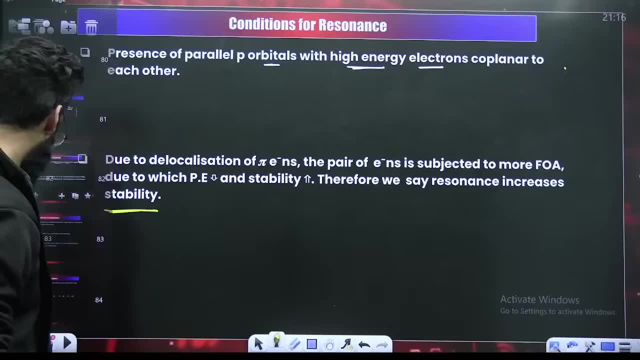 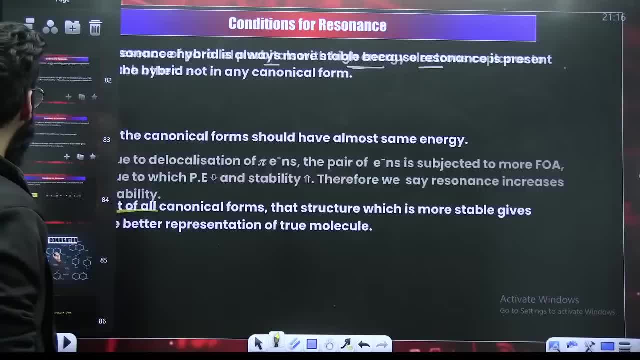 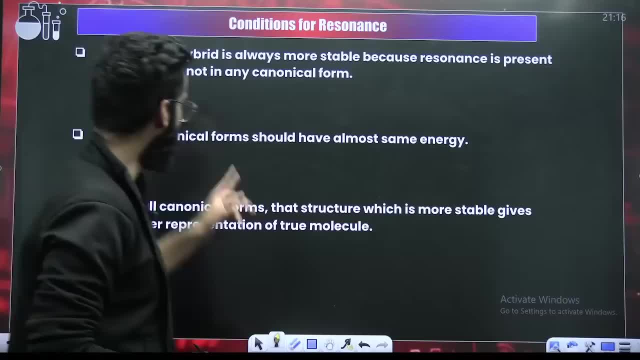 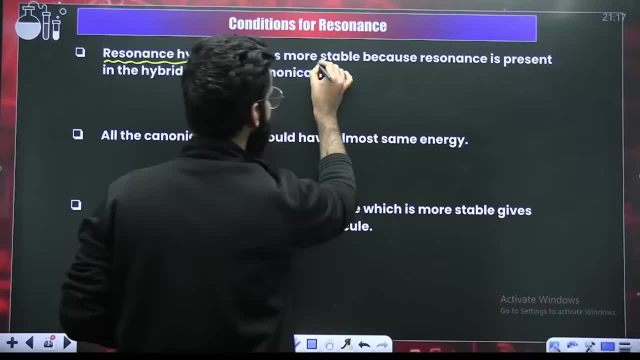 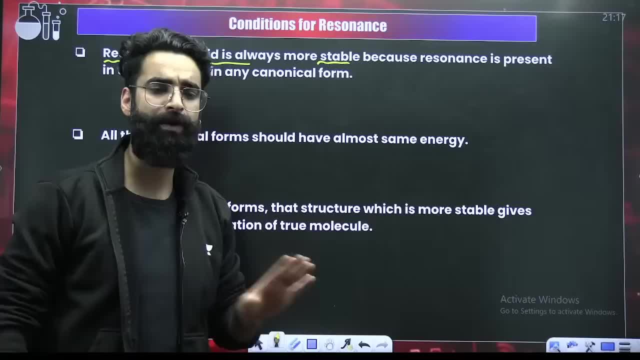 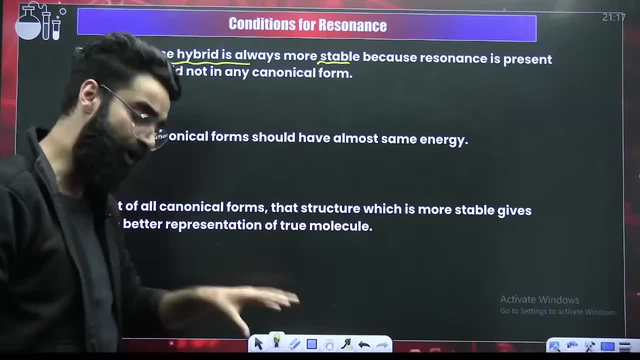 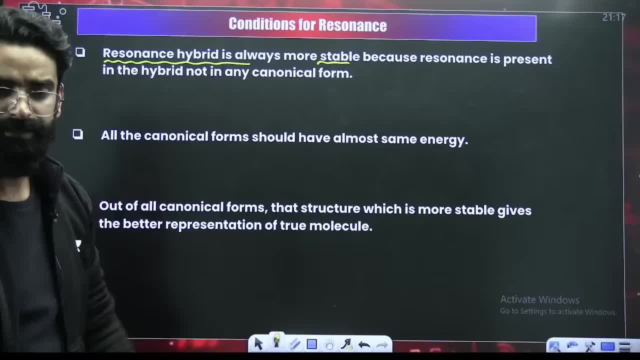 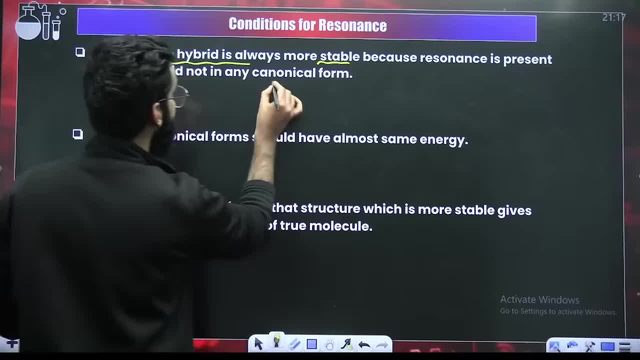 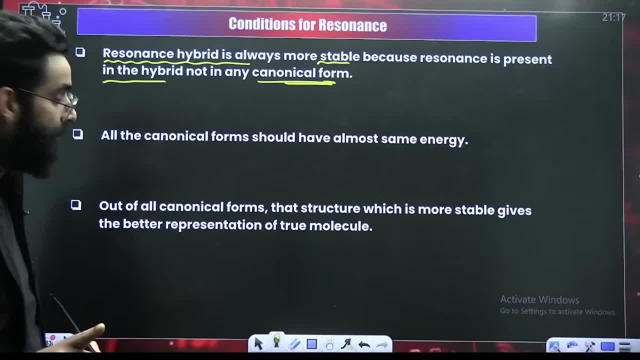 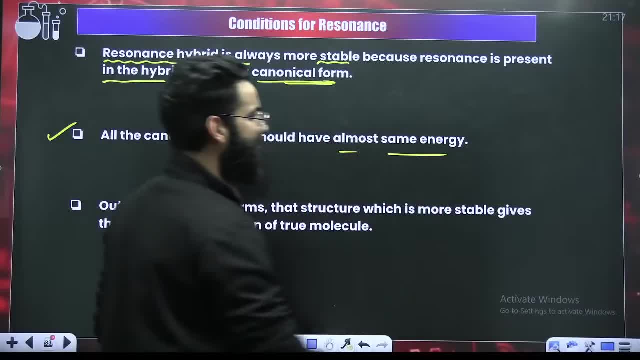 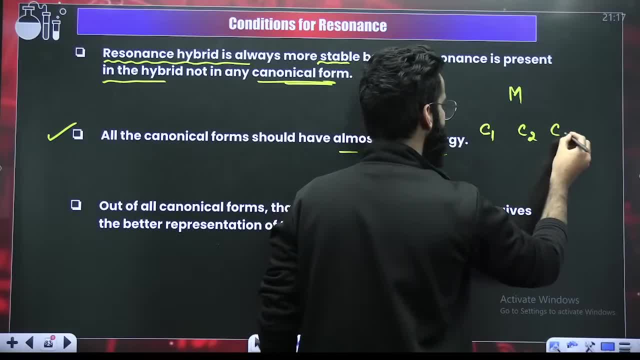 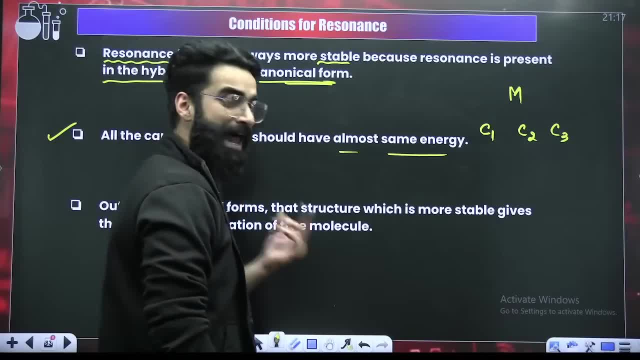 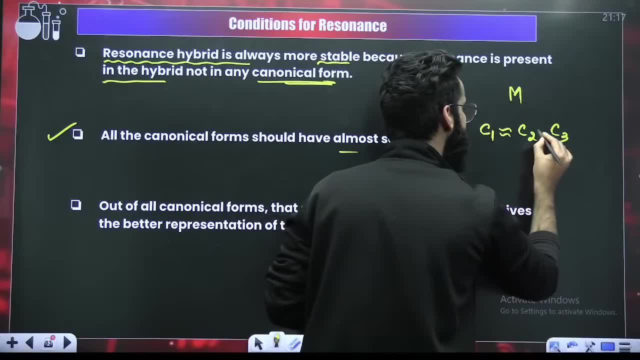 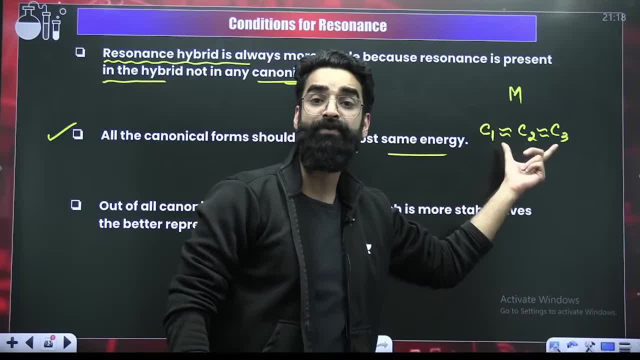 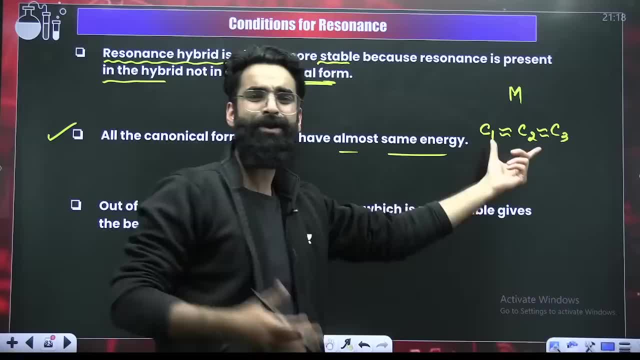 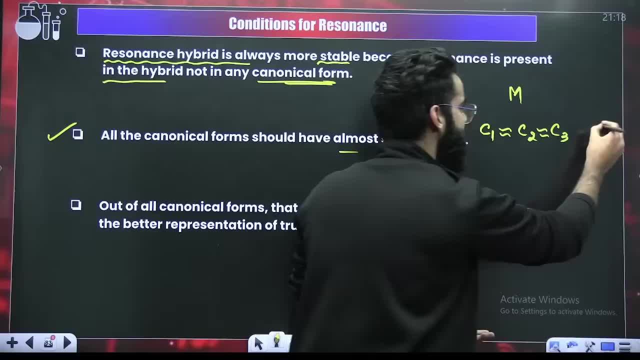 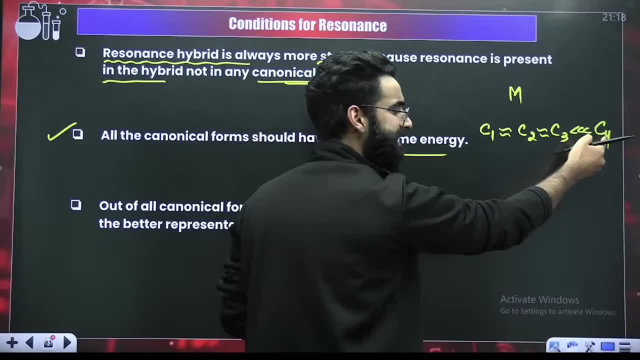 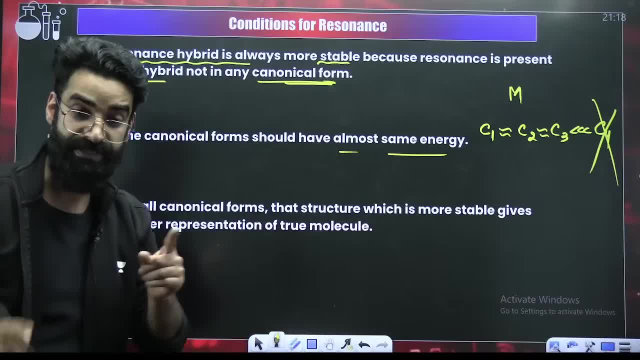 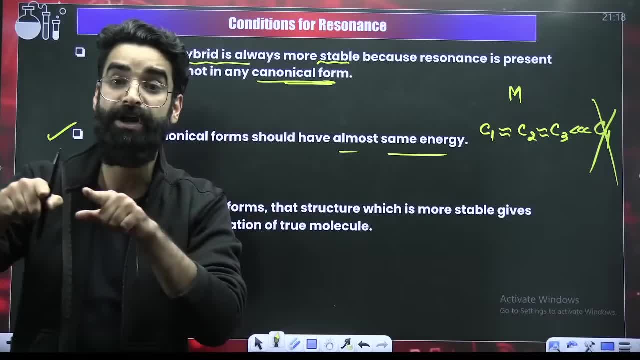 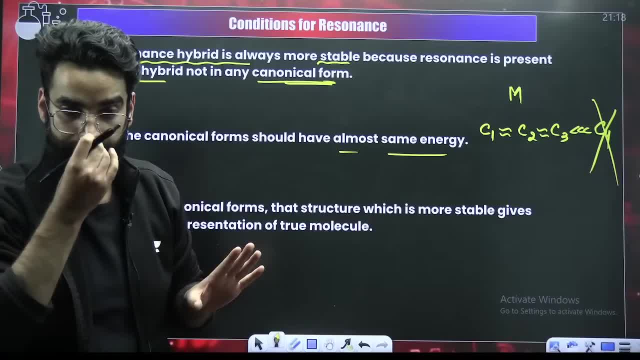 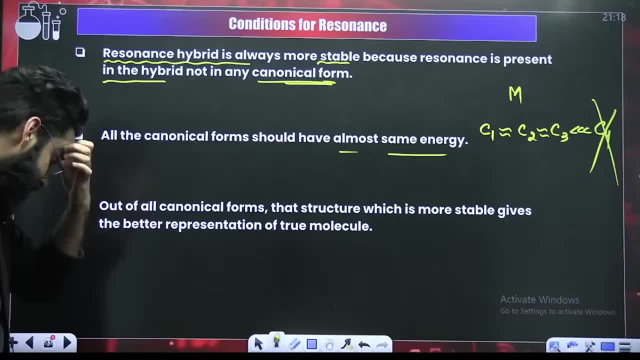 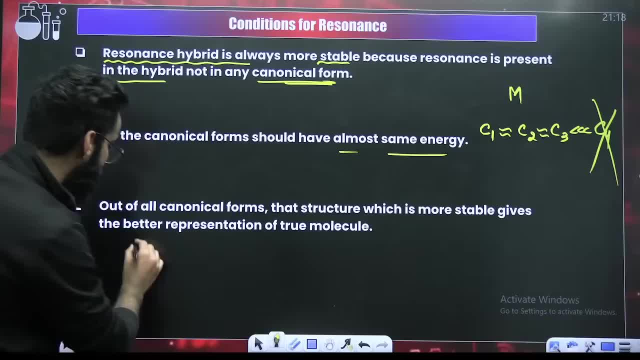 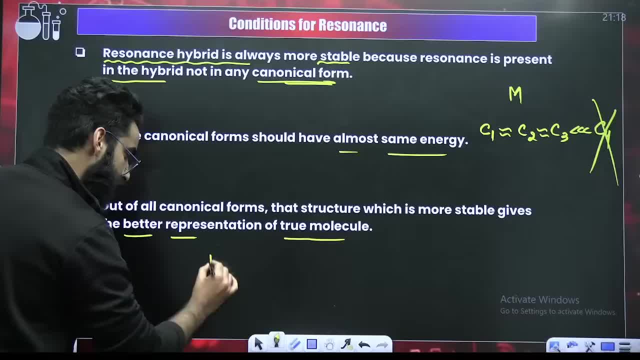 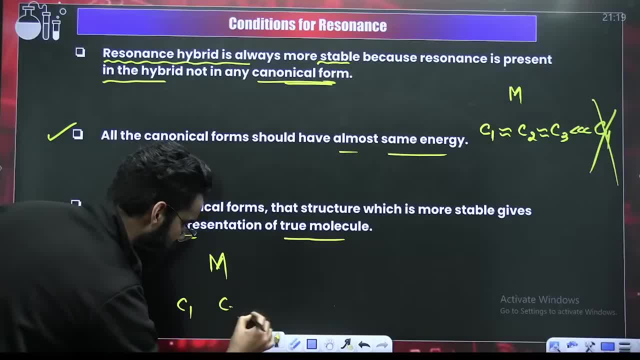 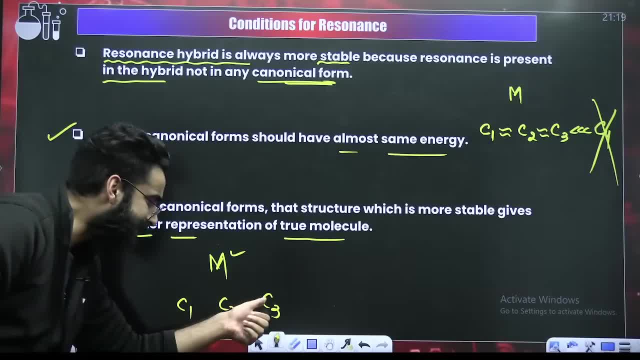 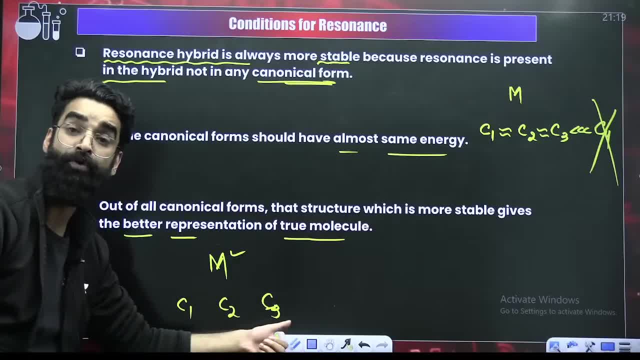 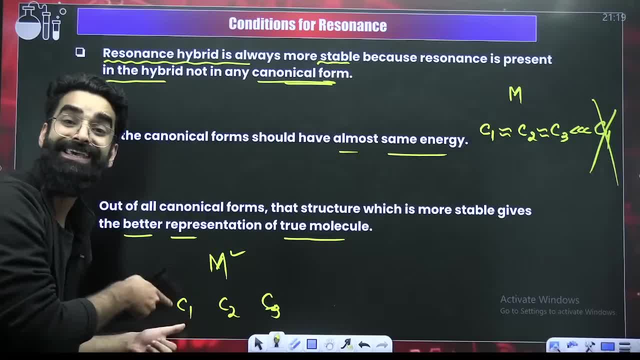 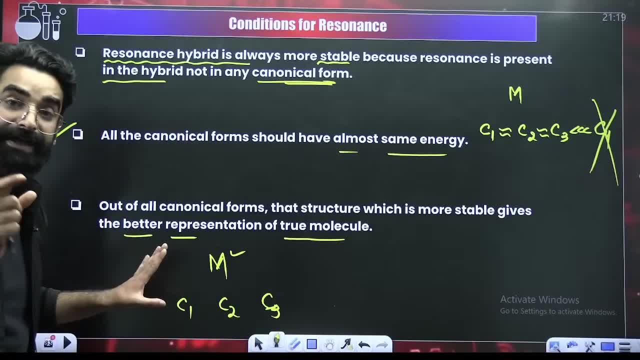 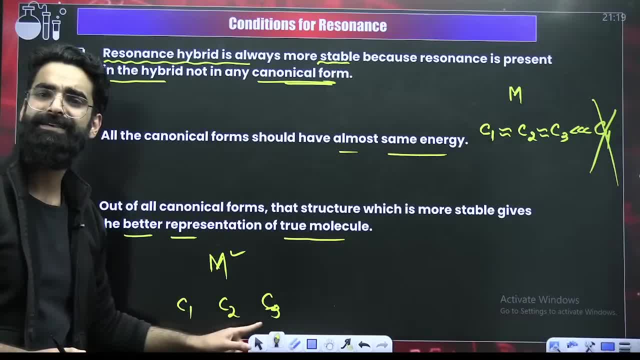 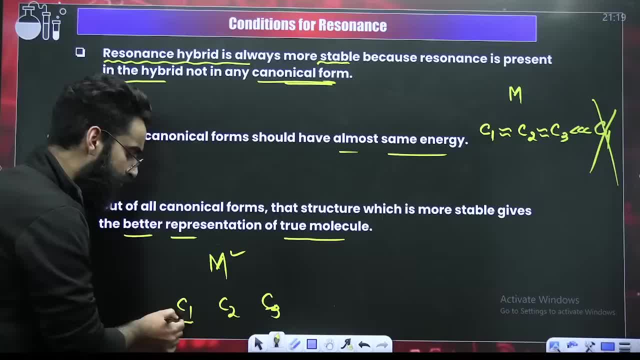 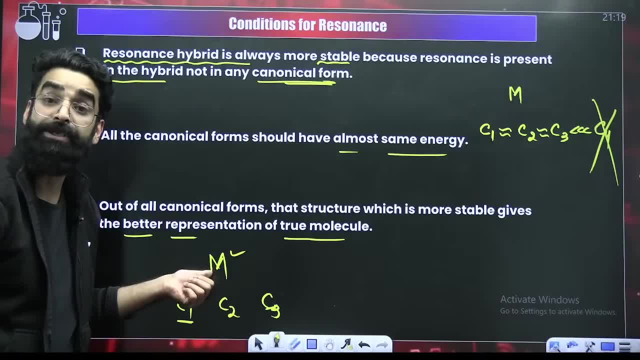 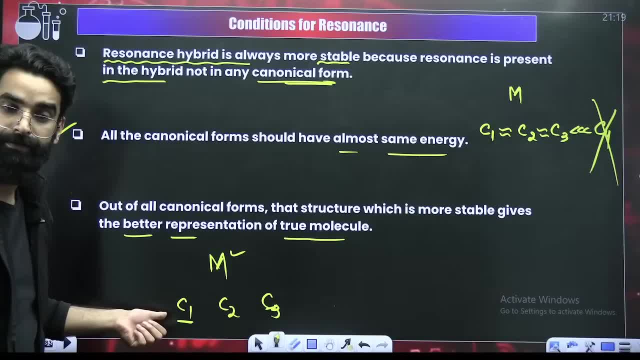 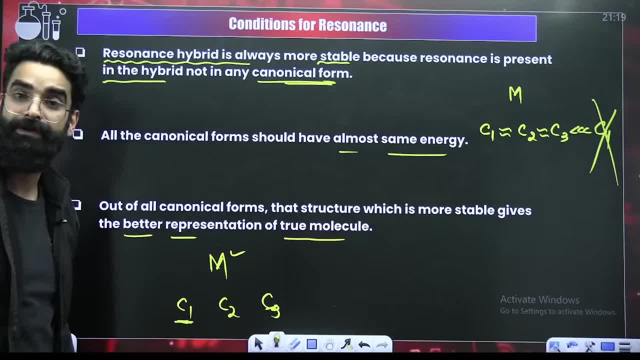 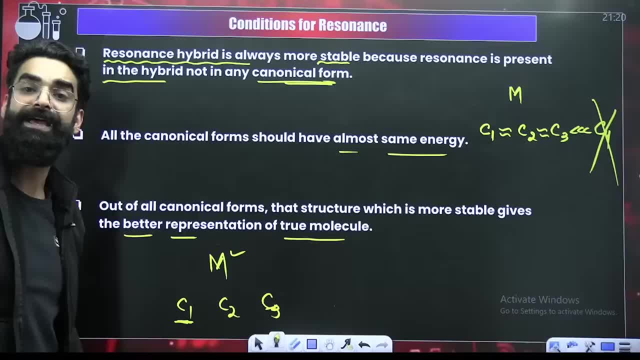 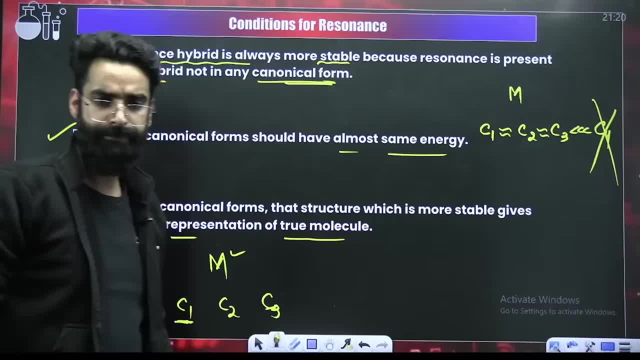 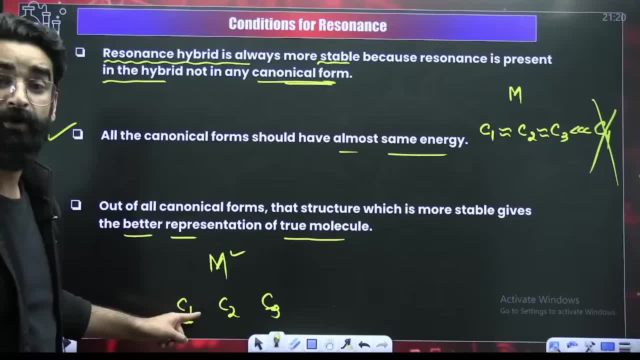 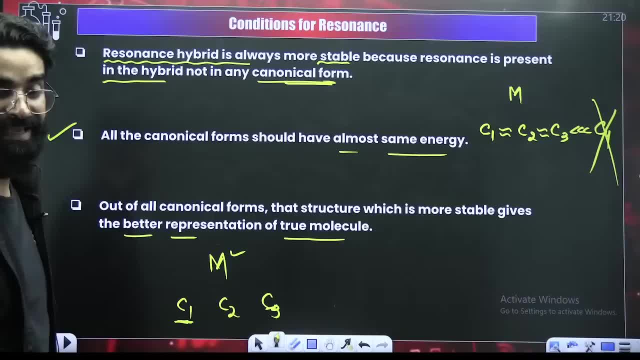 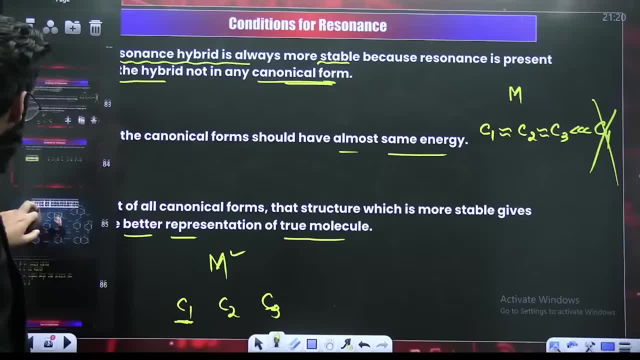 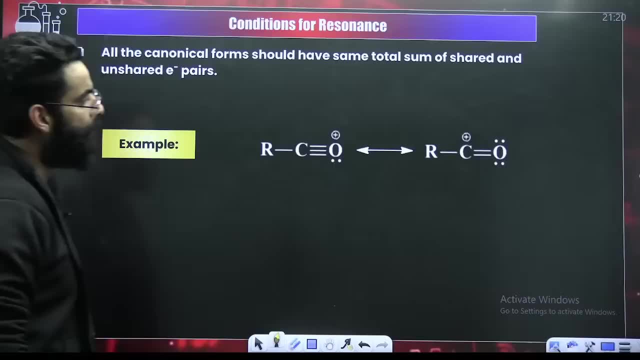 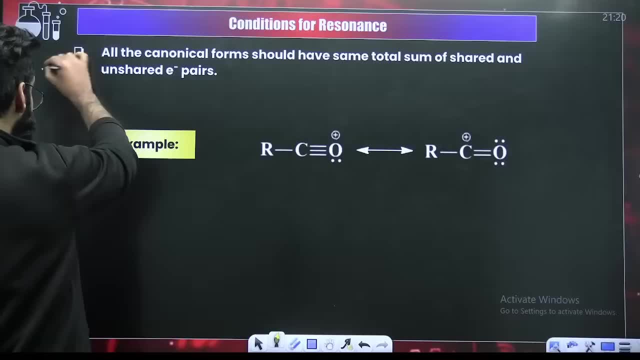 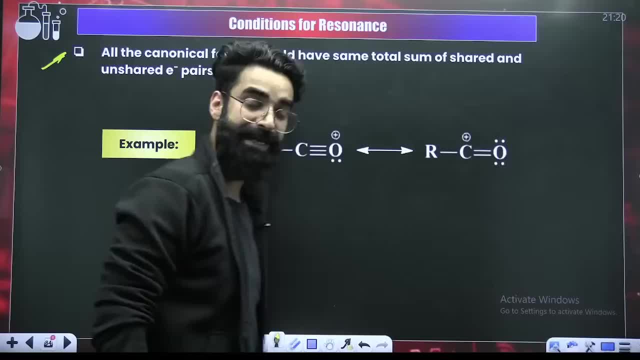 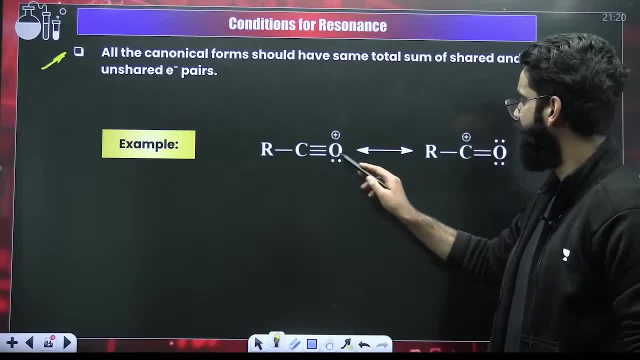 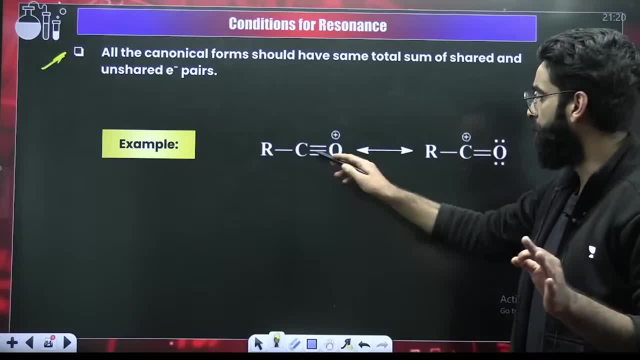 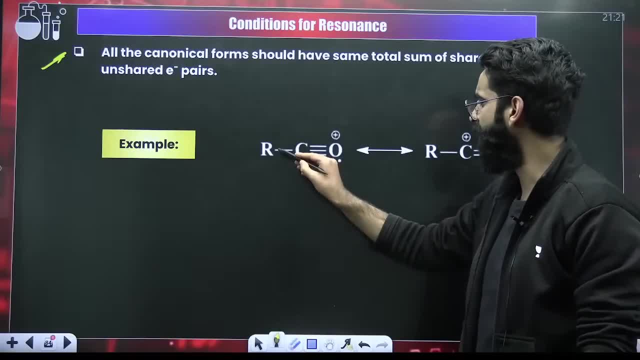 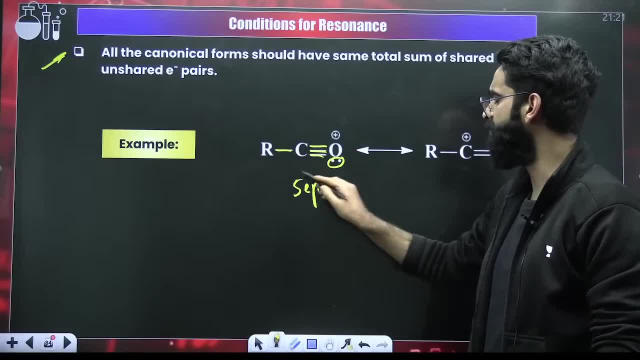 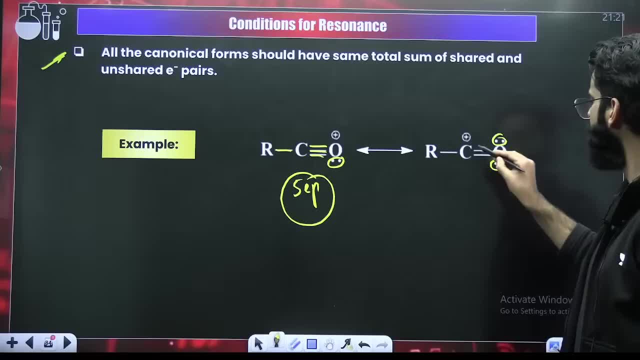 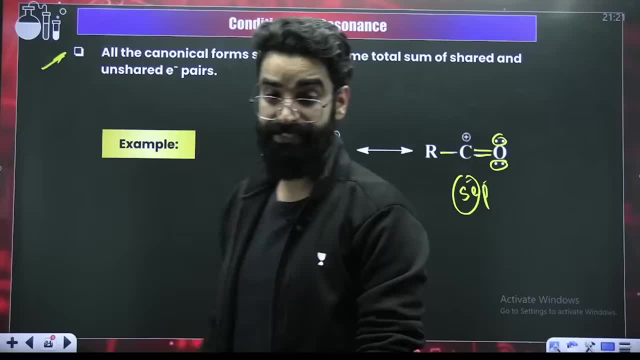 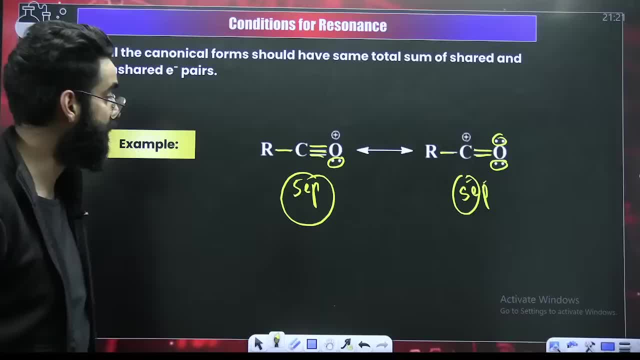 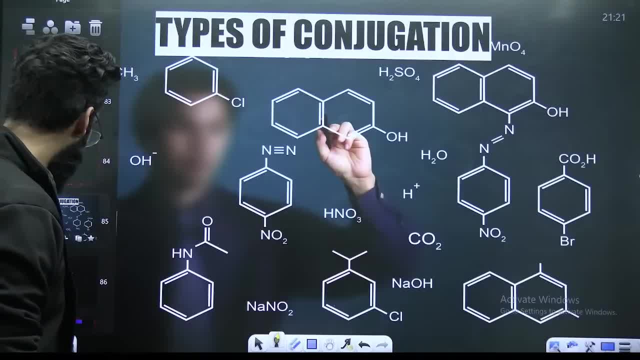 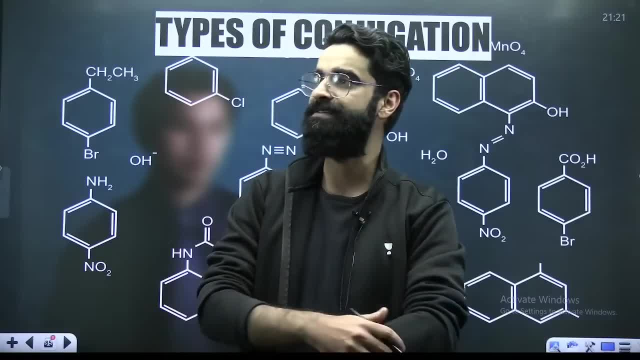 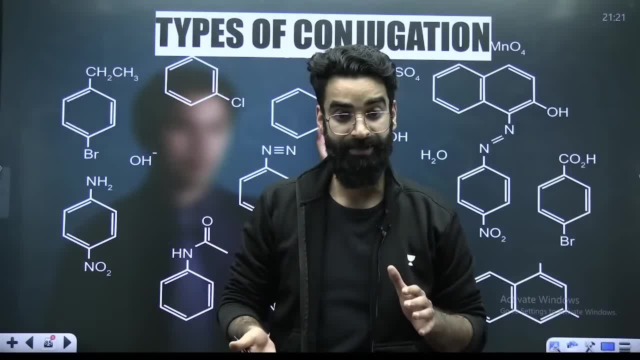 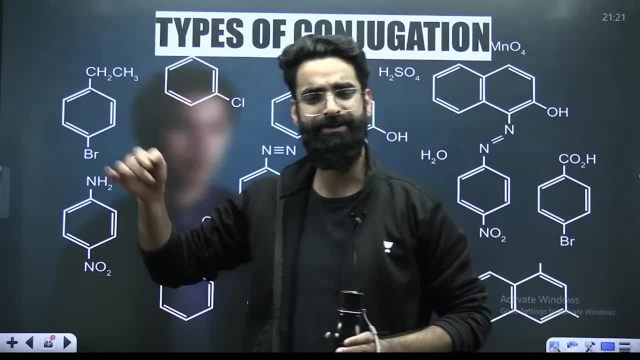 Resonance is considered as the most difficult topic, if it is taught actually, If it is taught in real sense, basically. otherwise it's easy. You know the conjugation, do this, that, give the bonds, that is easy. But the actual meaning of resonance is basically: 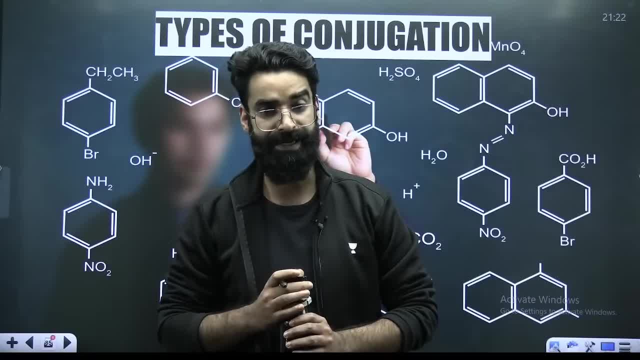 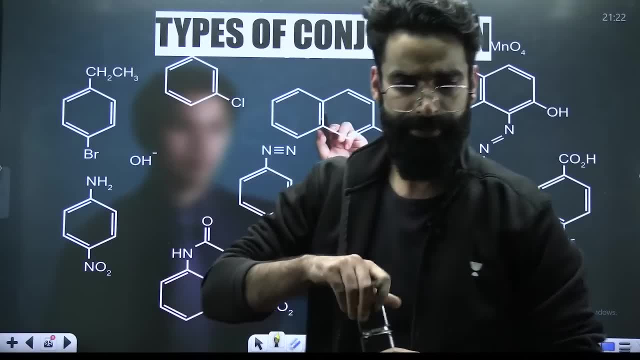 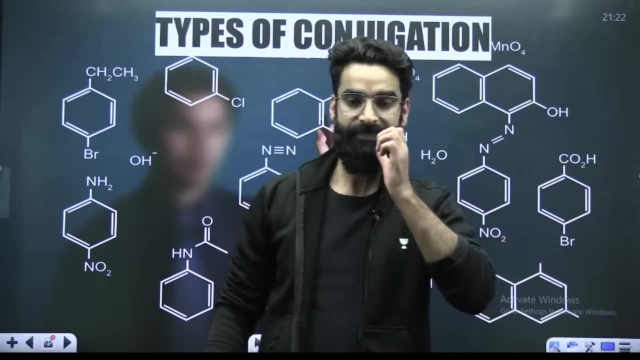 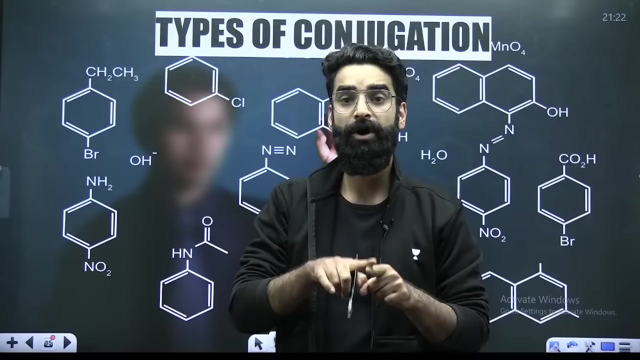 It is difficult to understand And I hope it is clear to everybody. Can you quickly let me know if it is clear? So quickly summarize it. whenever a true structure of the molecule cannot be formed, or if any structure of the molecule cannot explain all the properties of it, you will say that the 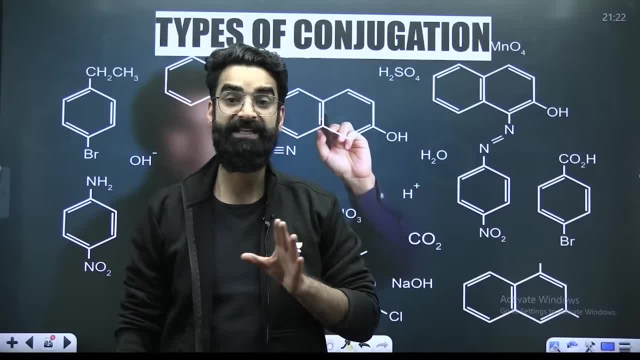 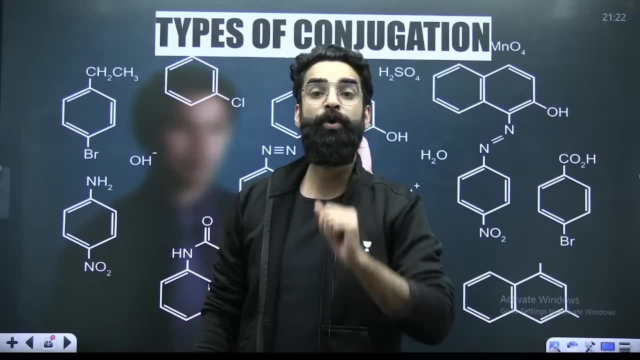 molecule will exhibit resonance. right, You will say that the molecule will exhibit resonance, perfect. What are the conditions? What is the meaning of, first of all, localized and delocalized electron pair? Localized electron pair is that electron pair which is shared between two atoms. delocalized, 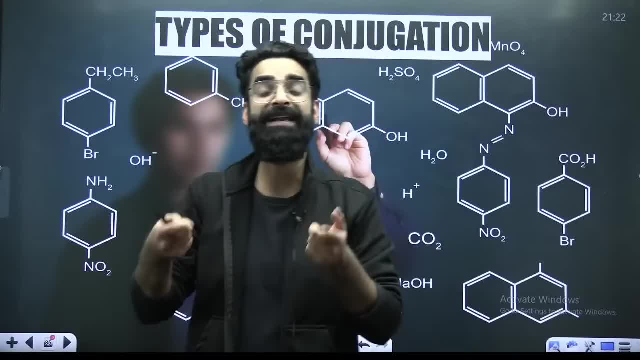 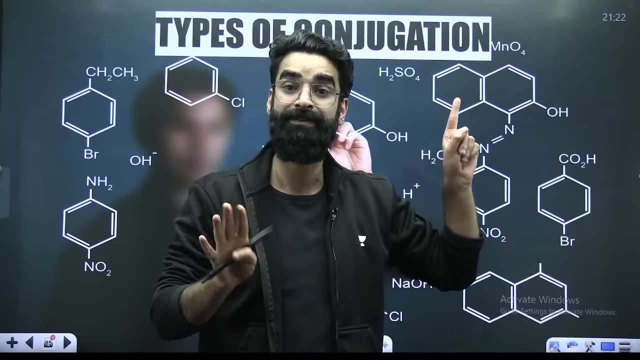 shared by more than two atoms. right Now, which electron pairs can be delocalized? High energy electron pairs can be delocalized, like your pi electrons, which are subjugated to less force of attraction. they can be delocalized. and the delocalization of high energy electrons. 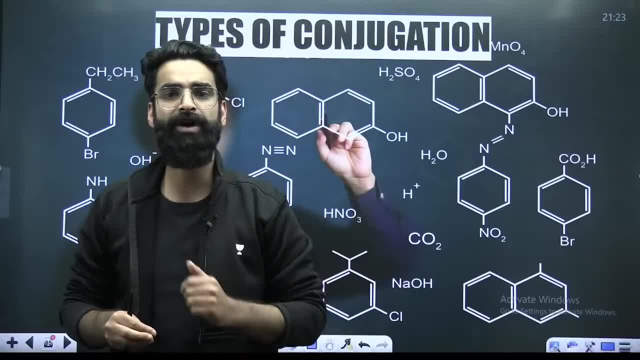 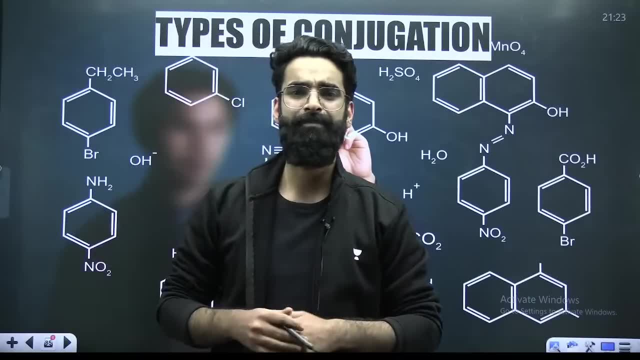 like pi electrons, is something which we call as resonance. If you look at the orbital approach as per orbital approach, what is the resonance? It is the partial overlap of p or d orbitals which are parallel and coplanar to each other. 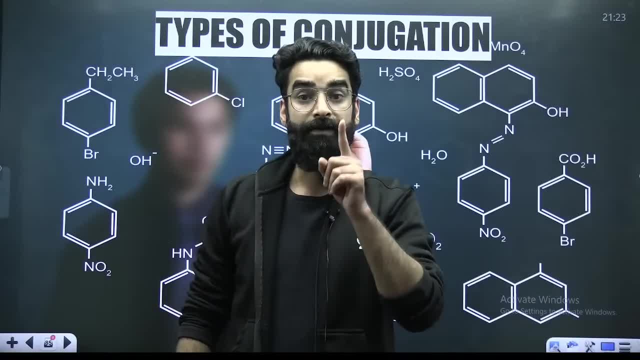 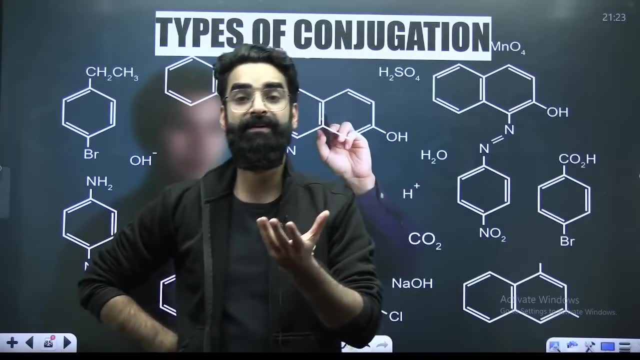 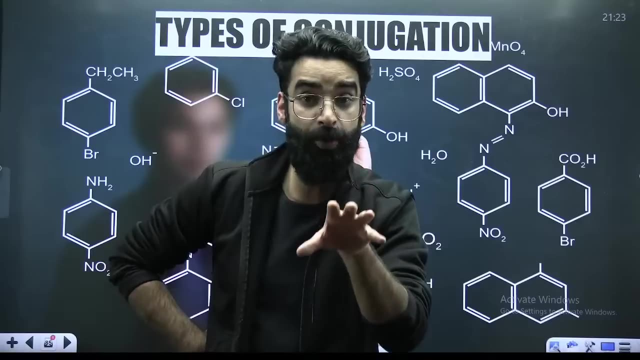 right, Perfect. Now one more thing. one more thing. how do you define the canonical structures? Canonical structures are the ones in which bonding is localized. in which bonding is localized, Delocalization is not present in the canonical form. Delocalization is not present in the canonical form. 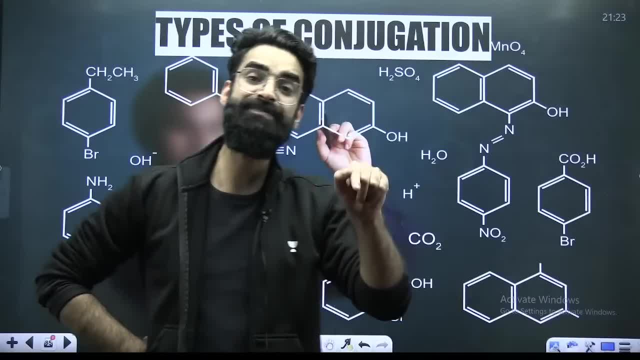 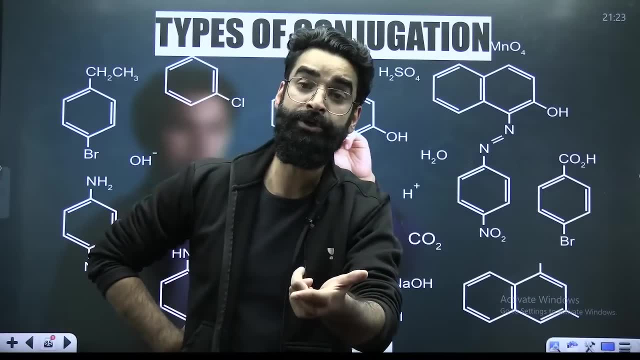 What is the reason why delocalization is present in The hybrid? If delocalization is present in the hybrid, that is the reason why in the hybrid, your pi electron density comes under the influence of more than two nuclei, due to which force of attraction increases right. 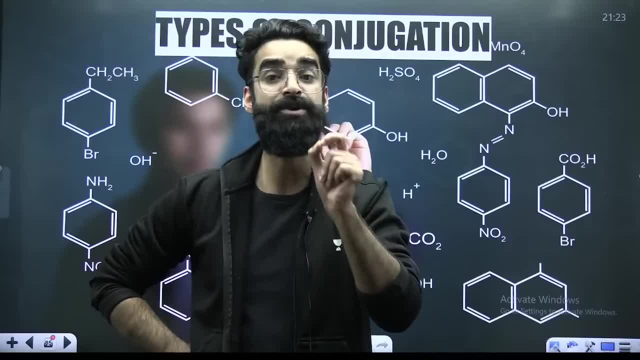 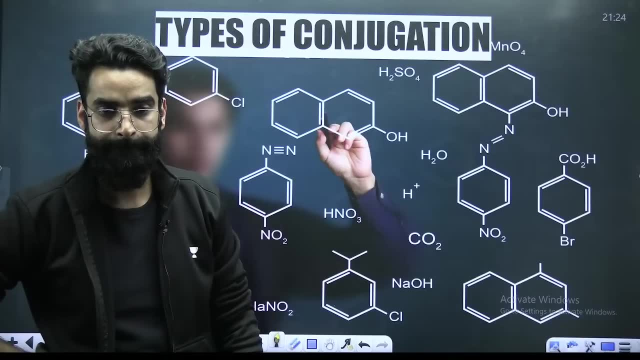 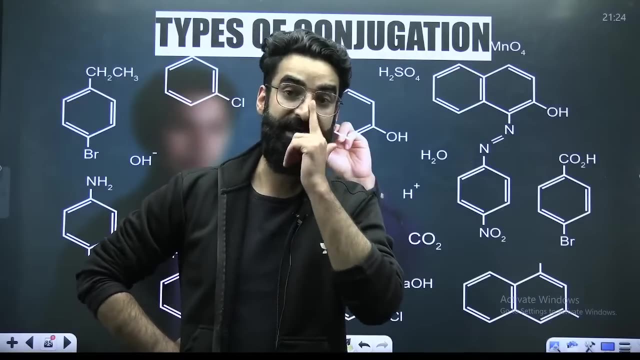 Energy potential. energy decreases, stability increases. That is the reason why your hybrid is more stable. That is the reason why the hybrid is more stable. Yeah, That is the reason why hybrid is more stable, Perfect And at the same time. at the same time, condition for resonance: there should be a presence. 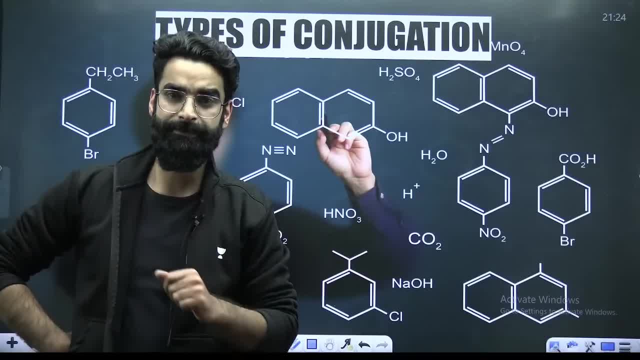 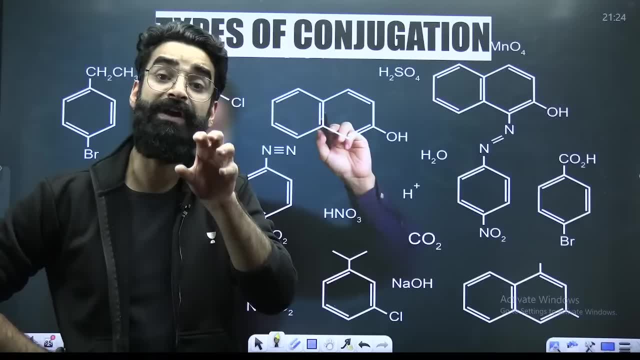 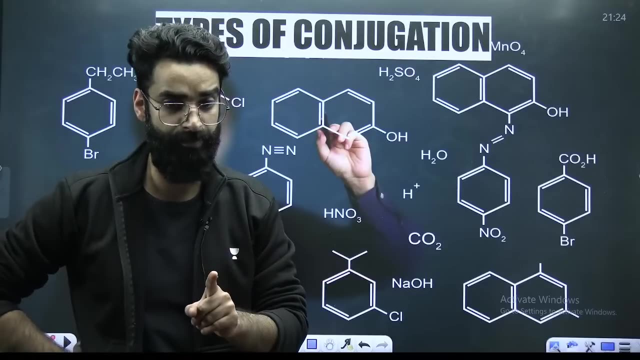 of parallel p orbitals which should be coplanar to each other. perfect, right. Your true structure will look more like that canonical form which is highest stable among all the canonical forms. This is one more important point which we have discussed, okay. 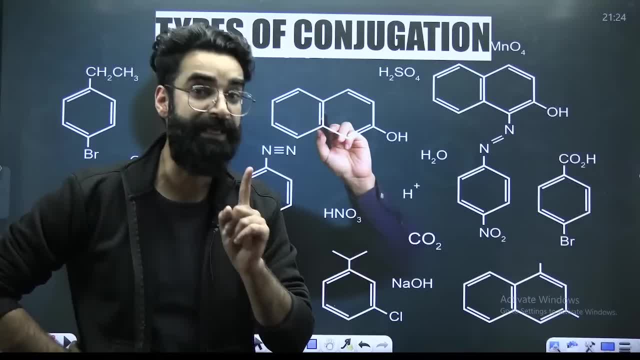 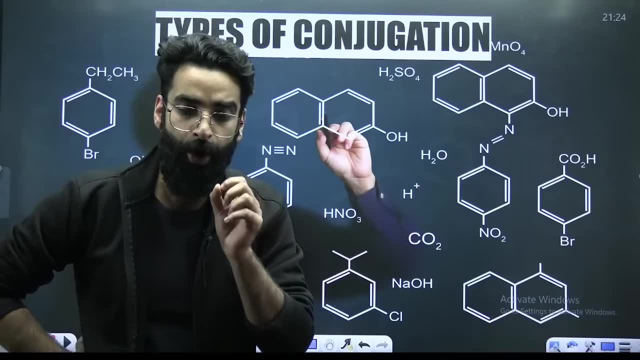 In all the canonical forms, In all the canonical forms, The total number of electron pairs should be equal. One more important point, right. One more important point: perfect. And all the canonical forms should have similar energy. All the canonical forms should have similar energy. 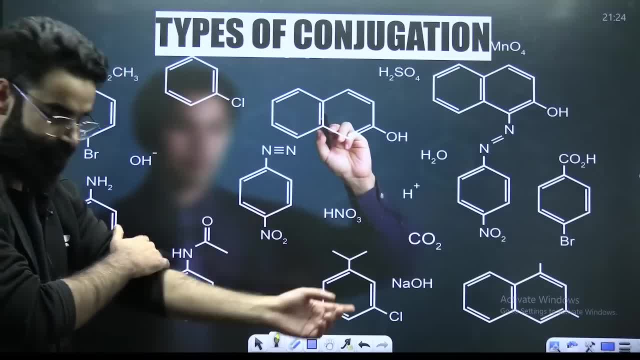 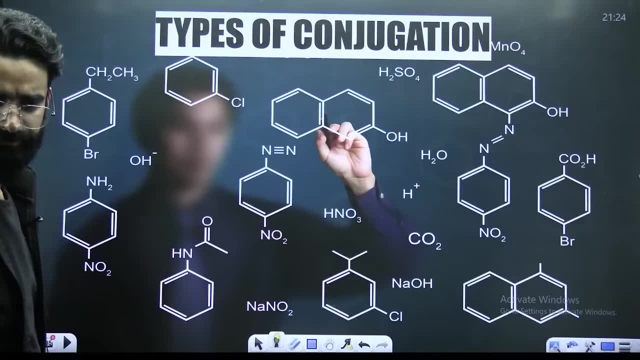 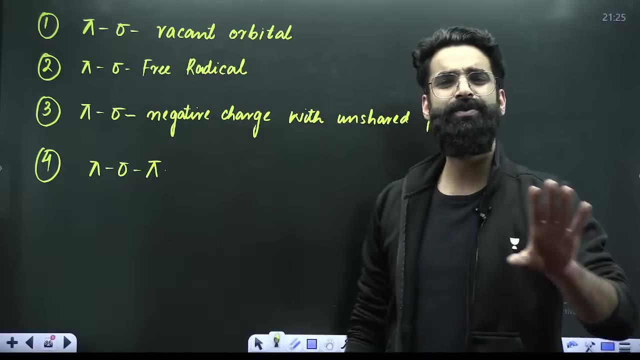 Now, now, now. Now we are going to move into conjugation. Now you will easily do the resonance, etc. etc. Now, this is the easy part, right Now, this is the easy part. See, guys, Basically, Wherever there is conjugation, wherever there is conjugation, resonance will be there. 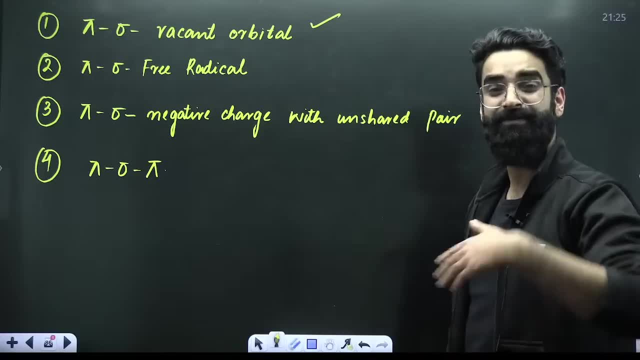 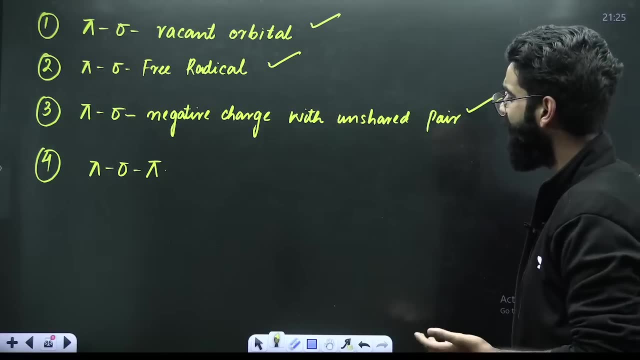 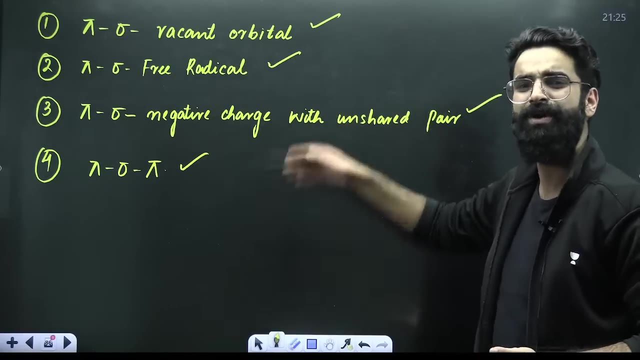 Conjugation can be of many a types: Pi sigma- vacant, orbital conjugation, something which we have to discuss in detail. Pi sigma- free radical conjugation. Pi sigma negative charge with un-shared pair of electron right. Pi sigma- pi conjugation- wherever you see pi sigma, I mean these sort of conjugations. 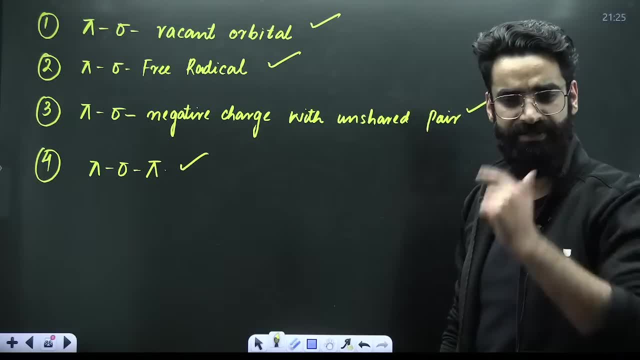 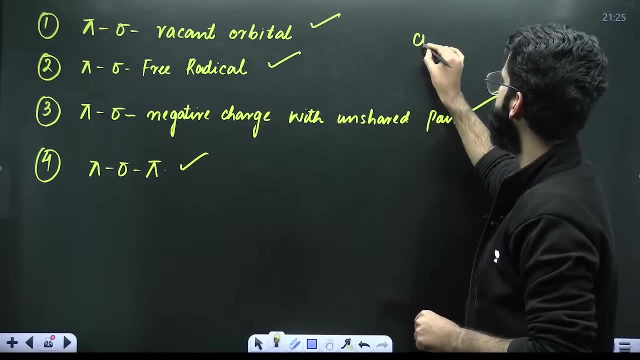 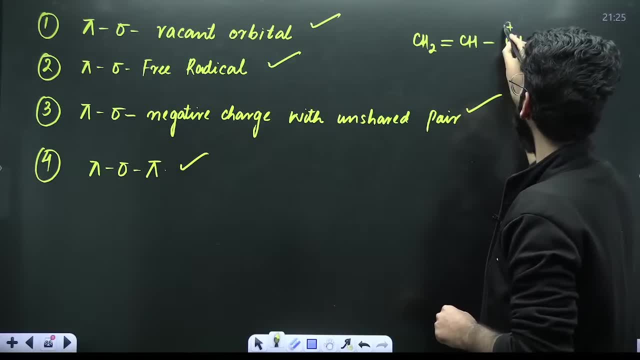 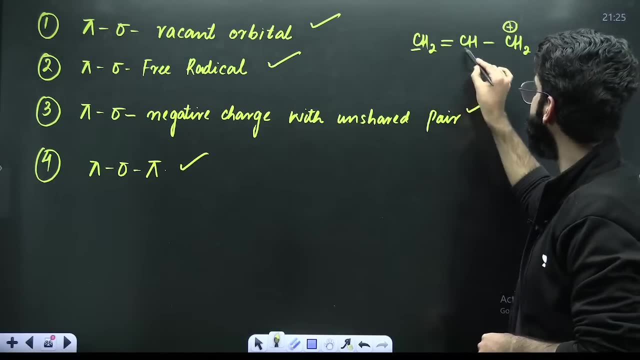 This is double bond. This is CH. This is single bond. This is CH2 positive, For example. Just an example, Just an example. Just an example: First of all, Sp2.. This is also Sp2.. This is also Sp2.. 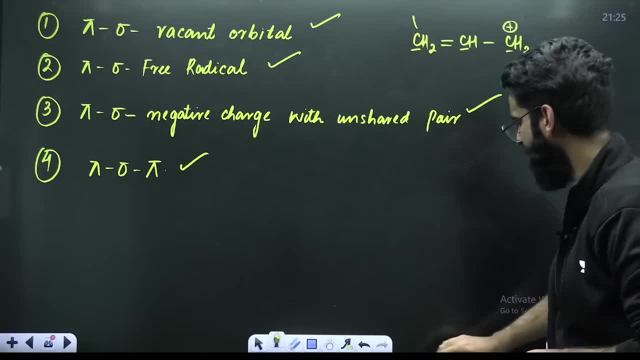 Everywhere, Or let me just make it like this. Let me make it like this: See, guys, Over here, there is a pi bond. As you can see, it is pi, And after pi you have got pi here, Pi, Pi. 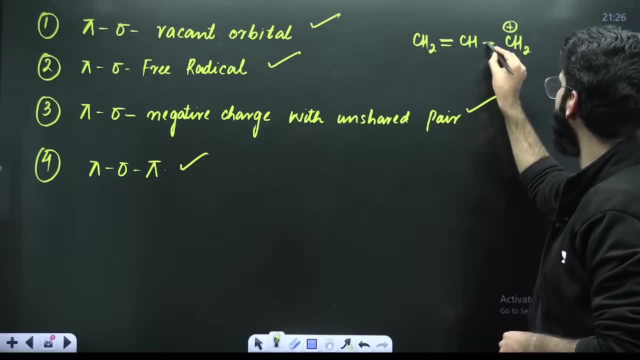 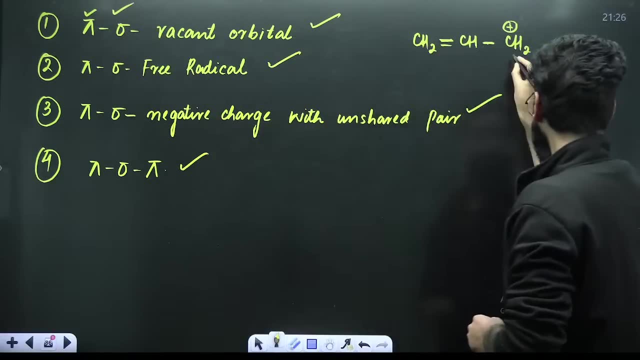 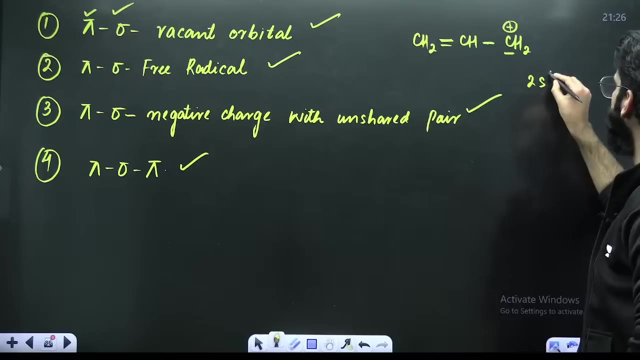 Pi, Pi, Pi, sigma after pi you have got sigma, after pi you have got sigma. so first you have pi, then you have sigma. if you look at this particular carbon, if you look at this particular carbon, if you look particularly at this carbon, what about the outermost configuration of carbon? it's 2s2, 2p2. 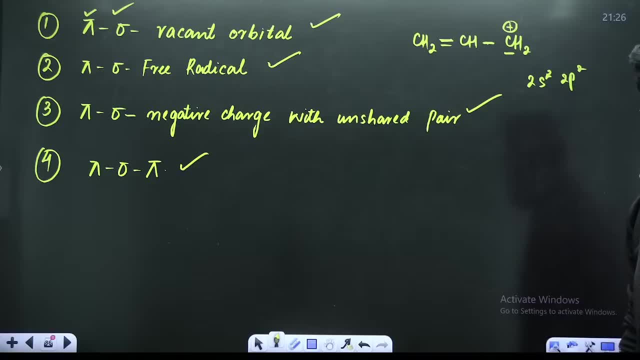 right, 2s2 2p2, correct: 2s2 2p2. so this is 2s containing two electrons, 2p containing two electrons. perfect, now, after excitation is done, 2s will be containing one electron and 2p will. 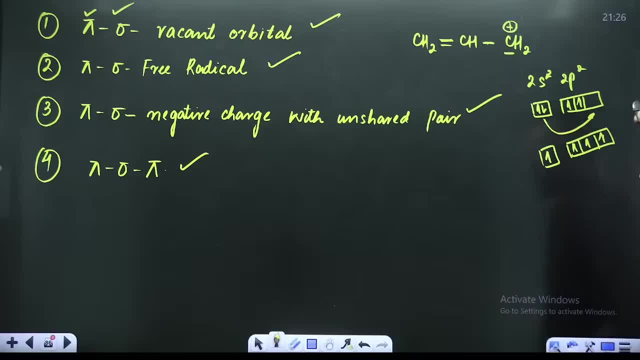 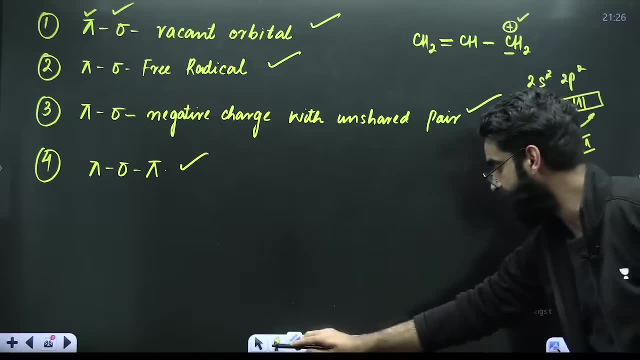 be containing three electrons. 2p will be containing three electrons. now there is a positive charge here. positive charge here means take one electron out. positive charge means take one electron out. let's say one electron is here. let's say that one electron is taken out from here. now this: 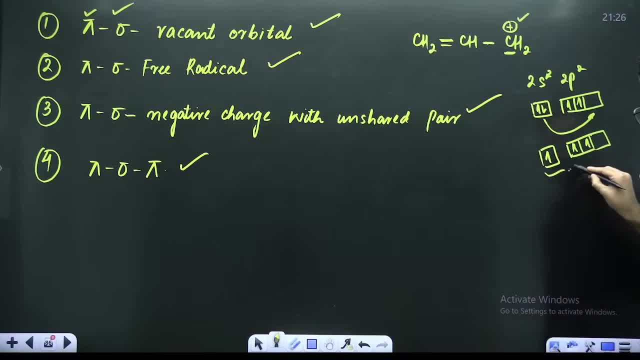 particular carbon, how many sigma it's forming, three sigma. three sigma means sp2, hybridization, this sp2, and there is one vacant orbital, one vacant orbital and there is one vacant orbital, and there is one vacant orbital and there is one vacant orbital, one vacant p orbital. so this carbon, it has got a vacant p orbital over here, right. so in this, 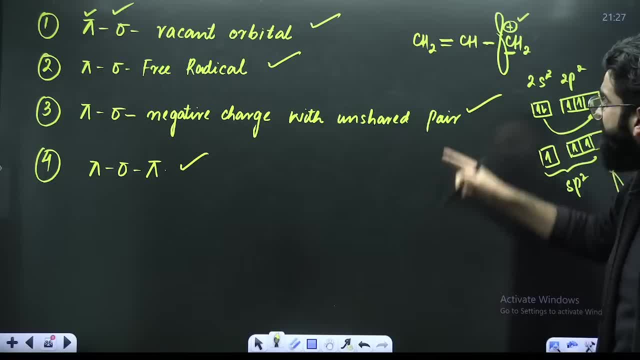 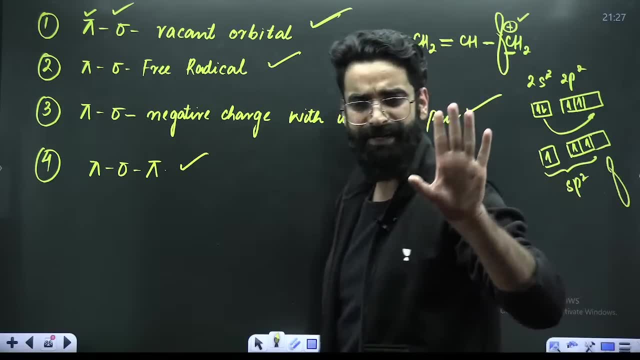 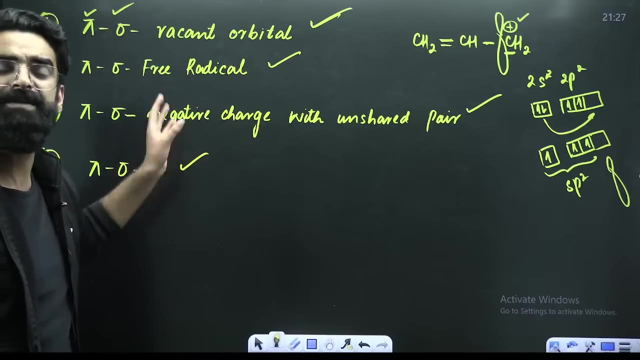 molecule. do you see pi sigma and vacant orbital present? absolutely, here we have pi sigma and vacant orbital. wherever in a molecule you see pi sigma, vacant orbital, understand resonance will happen in that molecule. understand resonance will happen in that molecule. similarly, pi sigma free radical resonance will happen. pi sigma negative charge with unshared pair of electron. 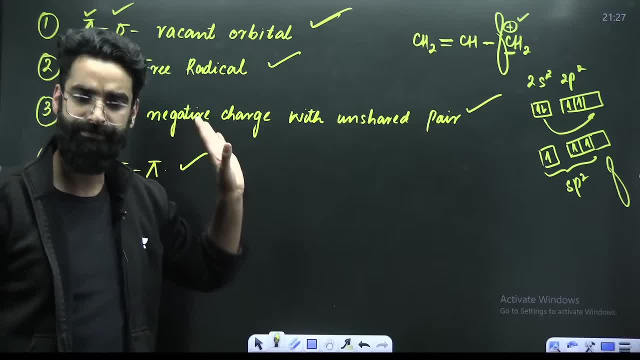 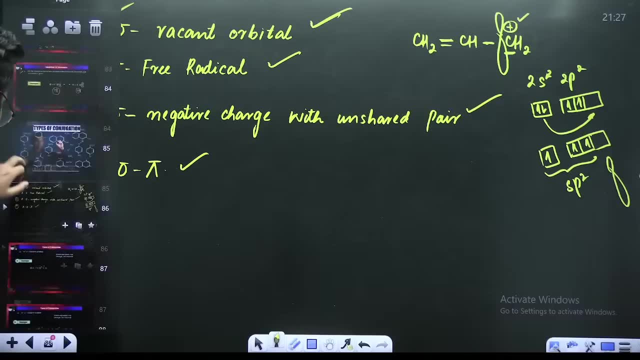 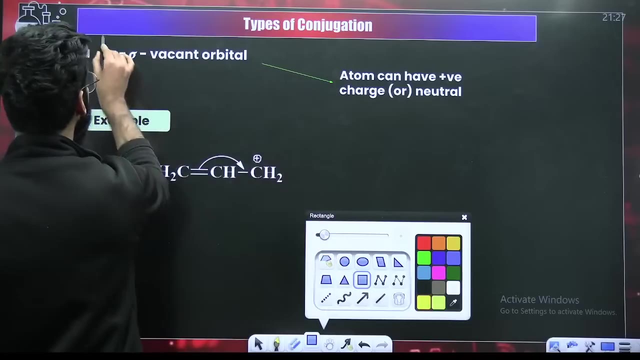 resonance will happen. pi sigma, pi conjugation, resonance will happen. okay, perfect. now, people, one by one, we are going to discuss this conjugation. the first type of conjugation is your pi sigma vacant orbital conjugation. your pi sigma vacant orbital conjugation. your pi sigma vacant orbital conjugation. 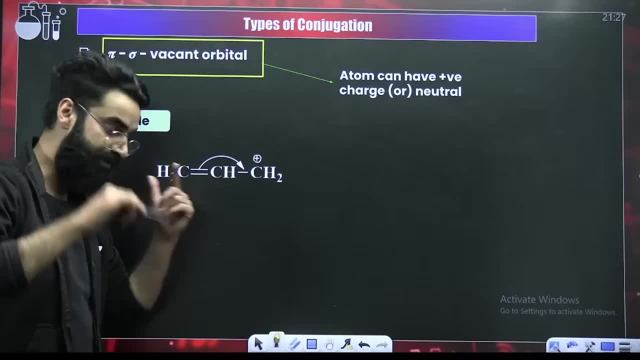 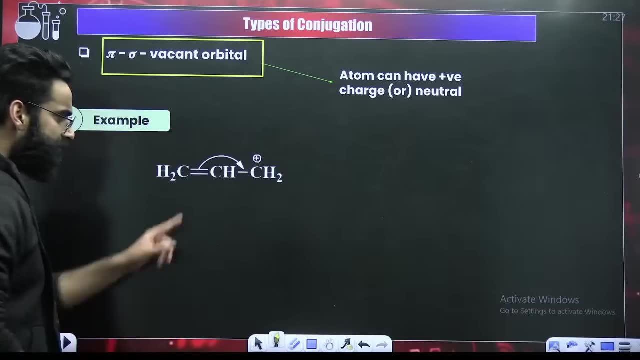 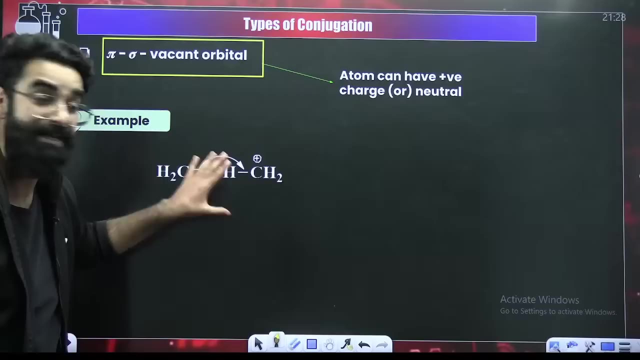 now, guys, firstly, i'll make you understand this particular thing. after that, i'll show you how to draw the structures exactly. see, first of all, okay, This is your sp2,. okay, if you look at this structure, this is one of the canonical forms which is given to me. this is one of the canonical forms which is given to me. 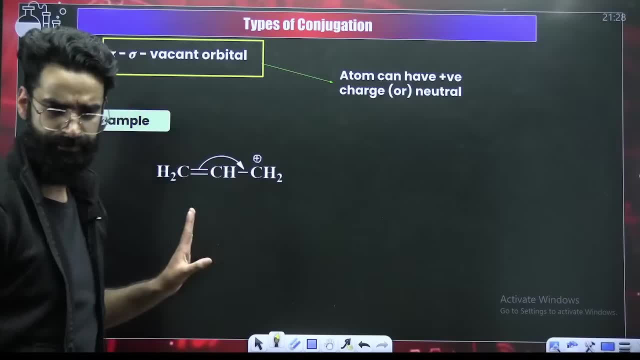 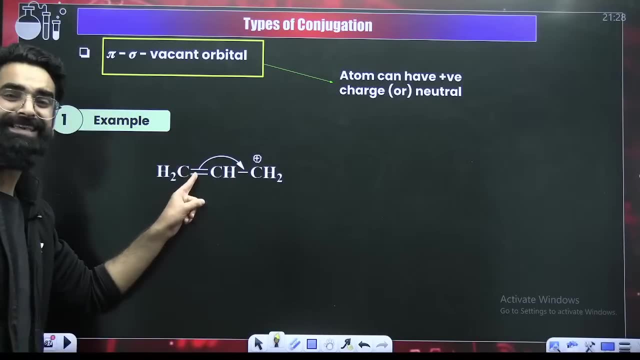 Now, after looking at this canonical form, I will have to make more canonical forms. After looking at this particular canonical form, I will have to make more canonical forms, But before that I will look exactly whether any type of conjugation is present here or 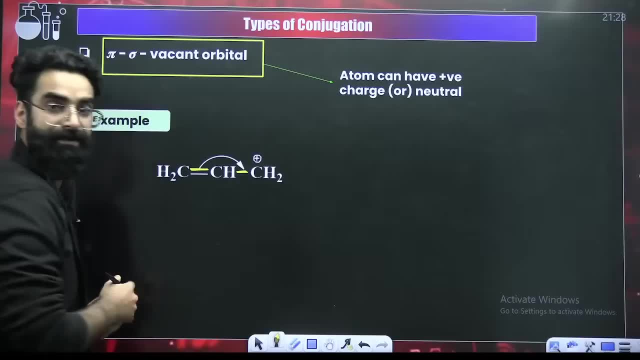 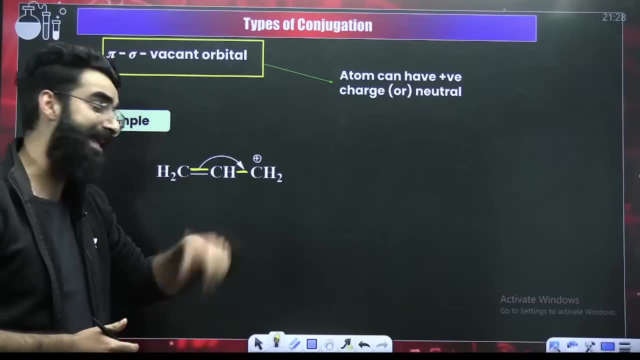 not See. I can see this is a pi bond. I can see, here you have got sigma, Now it has to be pi sigma, vacant, orbital. then only I will say there is conjugation, and then only I will show, I will say that this molecule will undergo resonance. 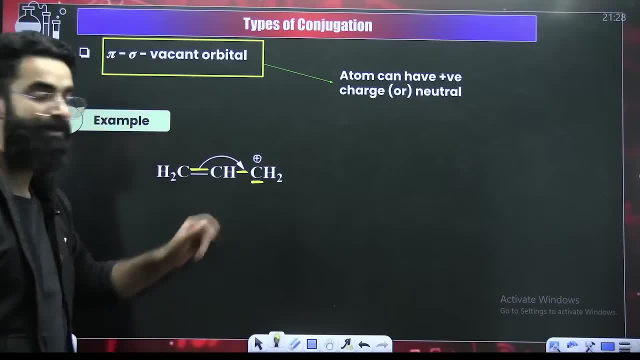 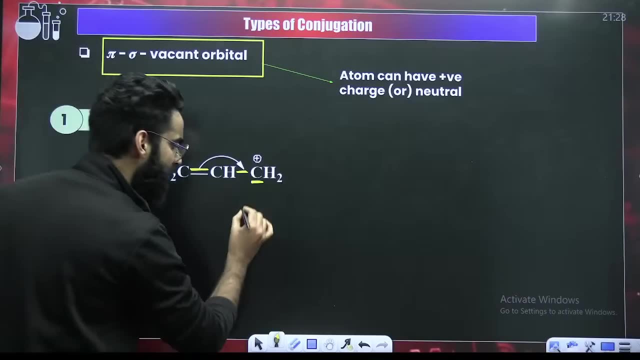 Now, how do you check whether you have got a vacant orbital here or not? The same approach which I showed you 5 minutes back. same approach which I showed you 5 minutes back, right? Tell me: outermost configuration of carbon is 2s2- 2p2, is 2s2- 2p2, right? 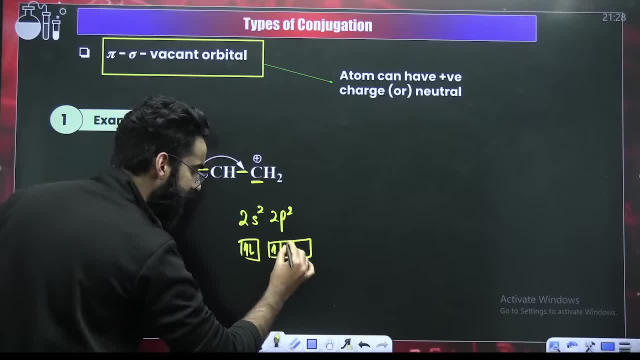 This is 2s containing 2 electrons and 2p containing 2 electrons, One here, one here. After the excitation is done, 1 electron will be here and 3 electrons will be here: 1, 2 and 3.. 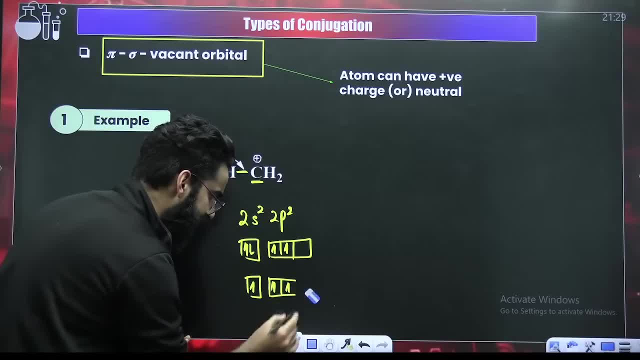 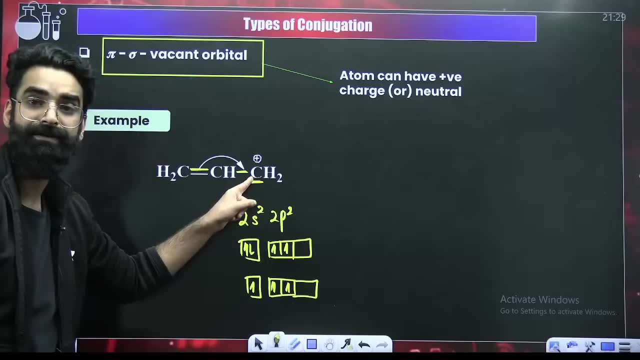 Now there is a positive charge here, so take one of the electrons out. if you take one of the electrons out, there is the structure now. there is the structure now. okay, Now, what is the hybridization of this carbon? It is forming 3 sigma, right, so it is sp2 hybridization. 3 sigma means sp2, so this: 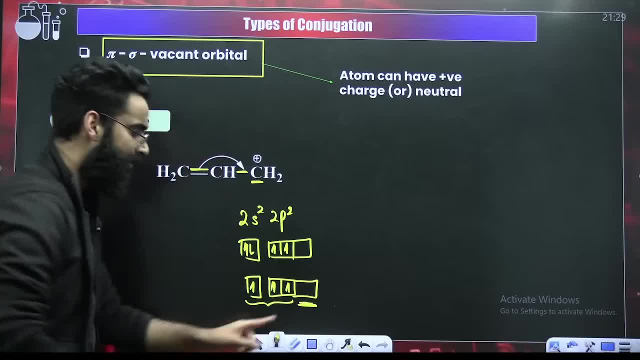 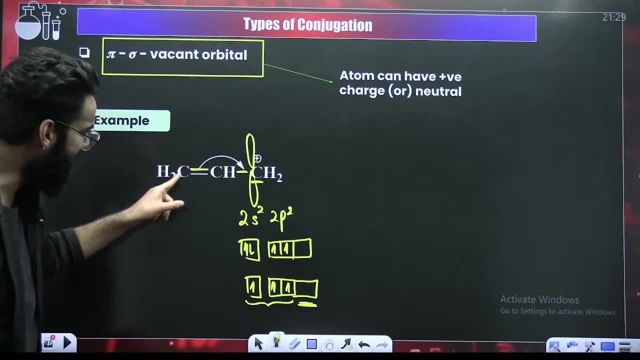 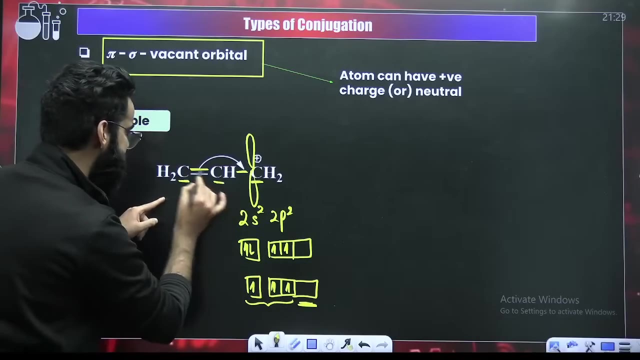 sp2 hybridization, perfect. and there is a presence of a vacant p orbital here. so this particular carbon, It has the vacant p orbital, it has the vacant p orbital. Even this is sp2,, this is sp2, right, If you exactly have a look on the orbital approach, if this is sp2, this is sp2, that. 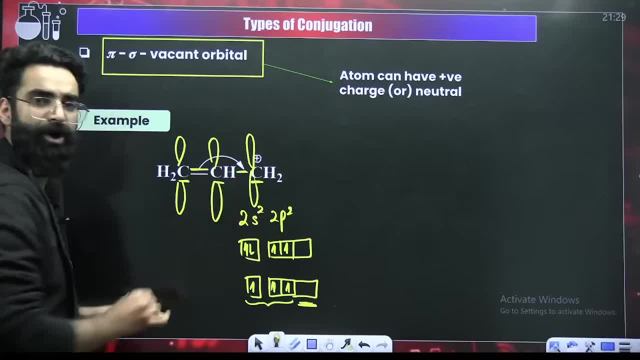 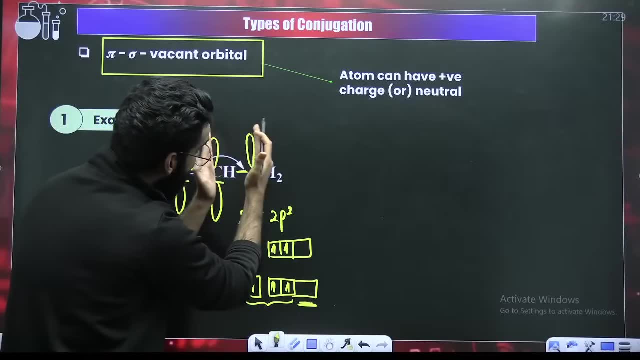 means it will be having one p orbital and here one p orbital, and this structure is telling you that these two p orbitals have overlapped apparently. Now other structure will tell you that these two can also overlap, apparently, right, perfect. Now, I am not going into the details of that. 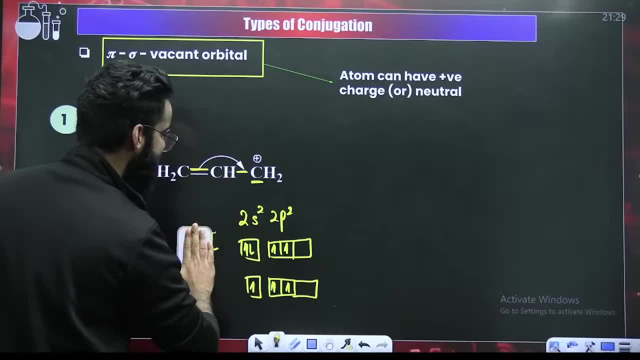 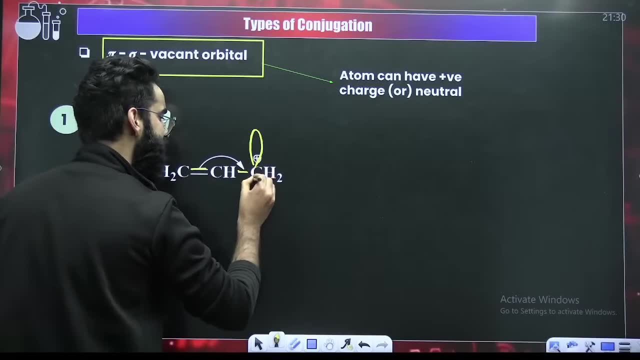 Since over here I got to know that we have got the pi sigma, pi sigma, we have got the pi sigma, vacant orbital conjugation. So I will directly say that resonance will happen here. and how do we make its other structures, other structures? 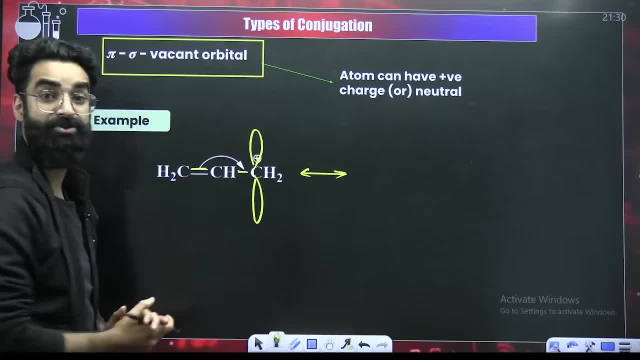 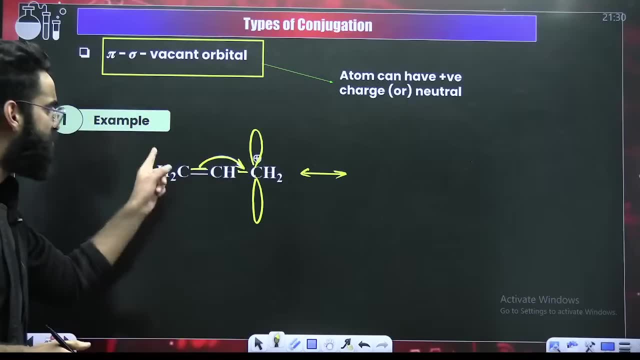 In this structure these two p orbitals have overlapped. in the other structure these two will overlap. So what does that mean? In short, shift this pi bond here. when you shift this pi bond here, it will become CH2. 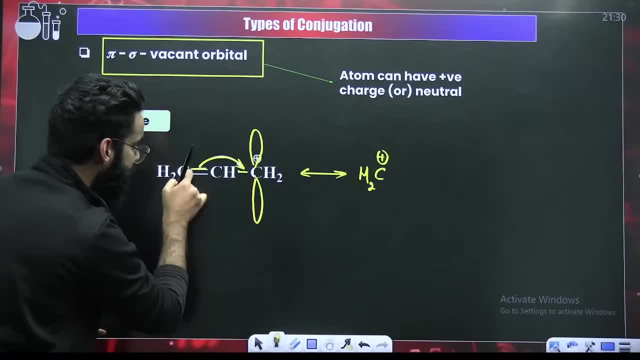 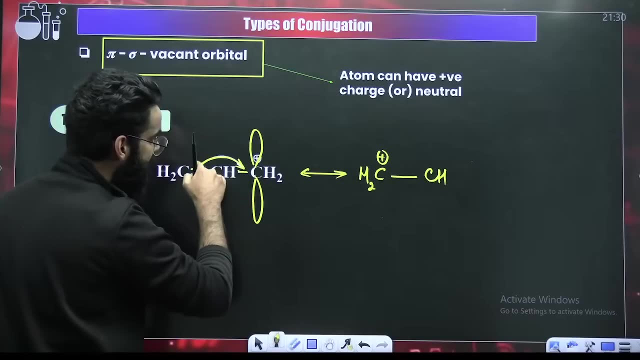 positive, It will become CH2 positive. There was a double bond here. there was a double bond here. now there will be a single bond. This CH you are writing as such. Initially there was a single bond here. now it is going to be a double bond. 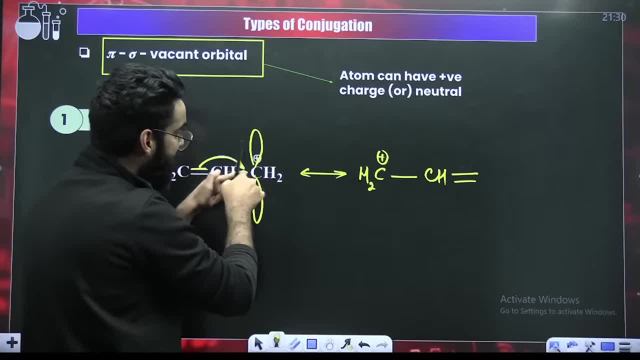 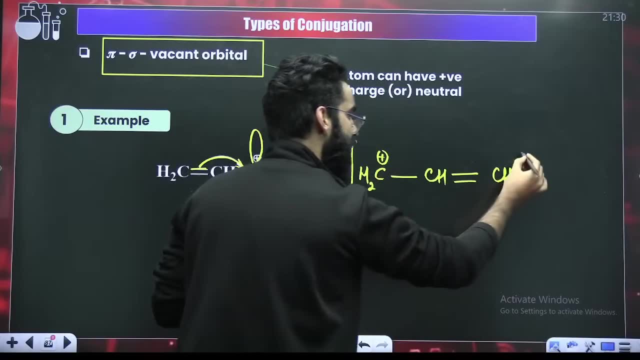 Now it is going to be a double bond. Initially this was CH2 positive but due to the double bond, it is not that positive will be compensated, nullified. this will be CH2 now. So this is one more resonating structure, one more canonical form, and this canonical 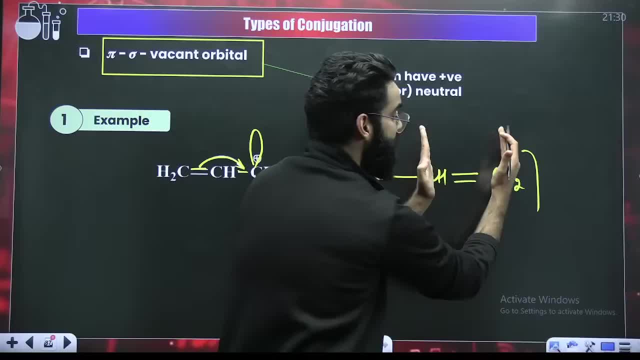 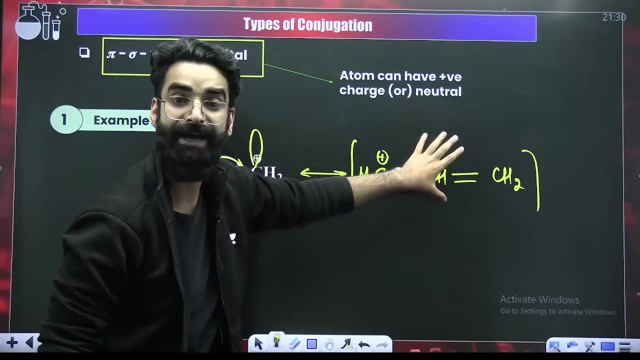 form is telling you, this canonical form is telling you the p orbital of this and the p orbital of this. they have overlapped. Now, some information about the actual molecule, this is given. some information about the actual molecule. this is given, and if you compile the information, you will get the resonance. 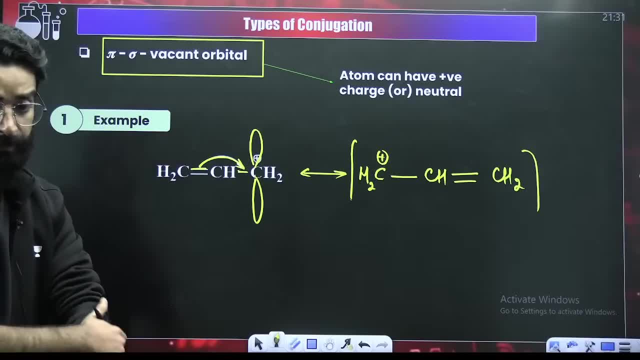 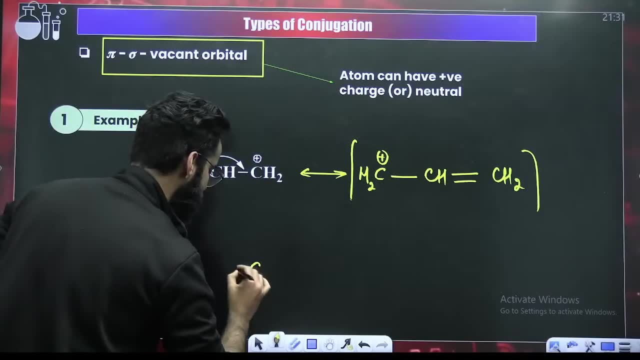 hybrid, You will get the resonance hybrid. so make the hybrid guys, make the hybrid, make the hybrid here, make the hybrid here. try to understand The hybrid looks like this: First of all, I will write CH2, I will put single bond. everywhere I will put single. 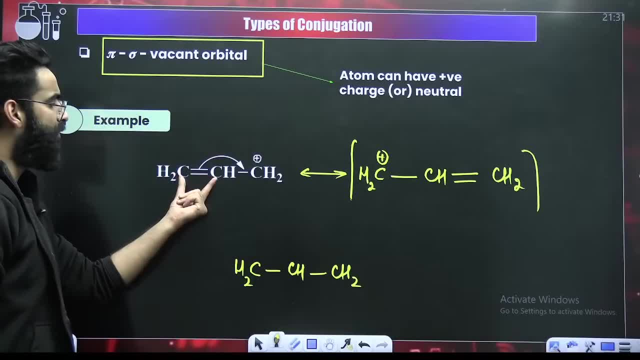 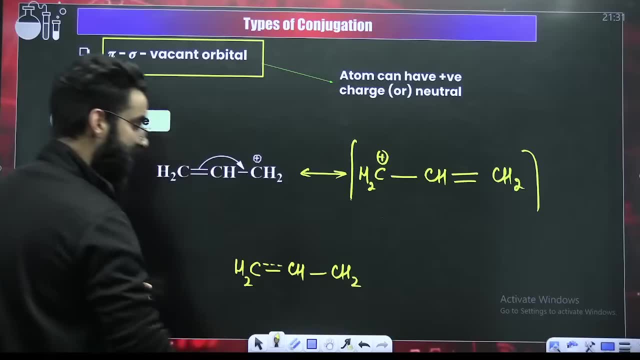 bond everywhere. Correct. Now, as per this structure, there should be double bond between these two. but this structure is saying single bond. In the actual molecule it is neither going to be pure single nor pure double. it will be partial double. Similarly, this is single, this is saying double. so in the actual one it is partial. 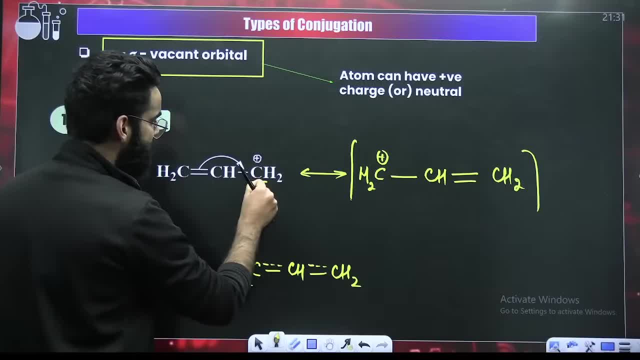 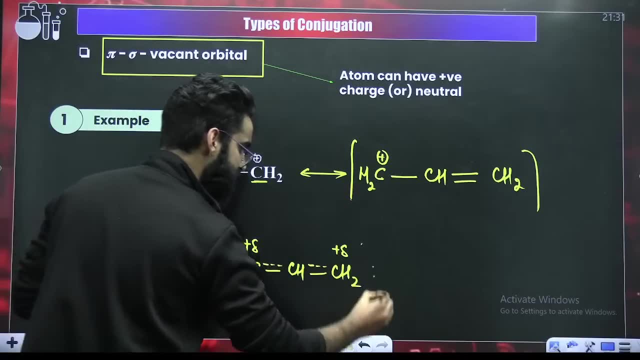 double Right. This structure is telling you that this carbon should have positive, so make delta positive over here. This structure is telling you: no, this carbon has to be positive, so keep delta positive over here. So this is something which I will be calling as the hybrid. 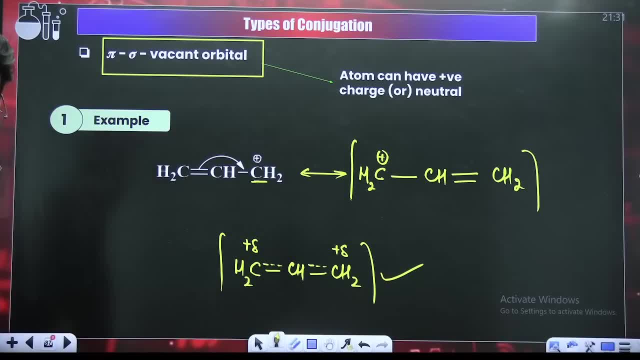 This is the resonance. hybrid people, I hope you got to know how to make it Right. I hope you got to know how to make it Perfect. Okay, Perfect. I hope you got to know how to make it. Now look at this one. 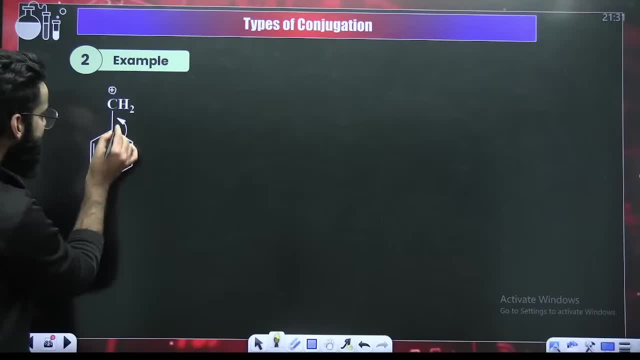 Look at this one, Look at this one Again. you can see. this is pi, this is pi sigma. and over here you will find a vacant orbital. You will find a vacant orbital. This is sp2 hybridized. this is sp2 hybridized. even this is sp2 hybridized, right. 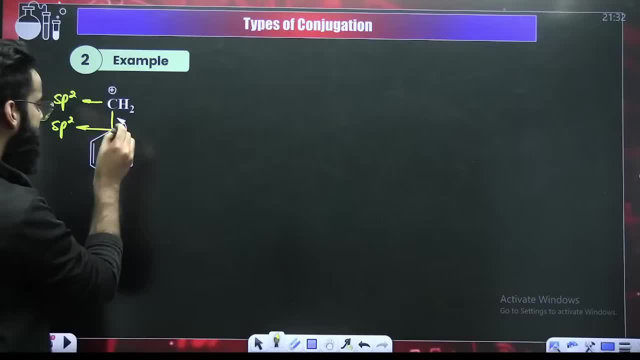 Every carbon here is sp2 hybridized, so every carbon will be having a p orbital, p orbital and those p orbitals will be parallel to each other, Right? So the partial overlap of the parallel p orbitals is something which you call as resonance. 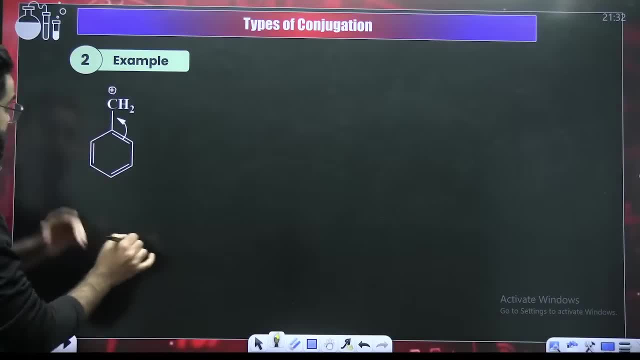 Right Now guys try to understand. This is pi, this is sigma, and here you have got the vacant orbital. Here you have got the vacant orbital, So there is a conjugation. If there is a conjugation, so you will be making its resonant structures. so shift this. 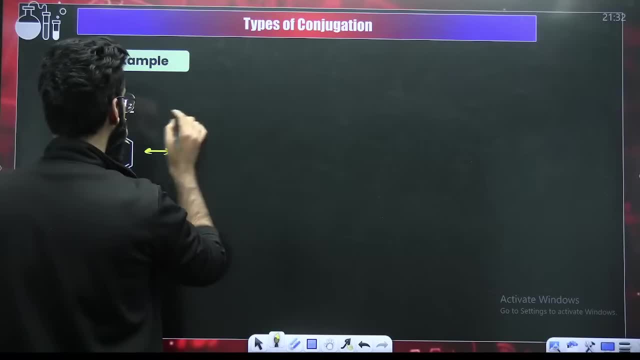 pi bond here first. Right, When you shift this pi bond here, this was CH2 positive in the beginning. now it is going to be CH2, positive charge compensated. Now there will be a double bond here. Right, There will be a double bond here. 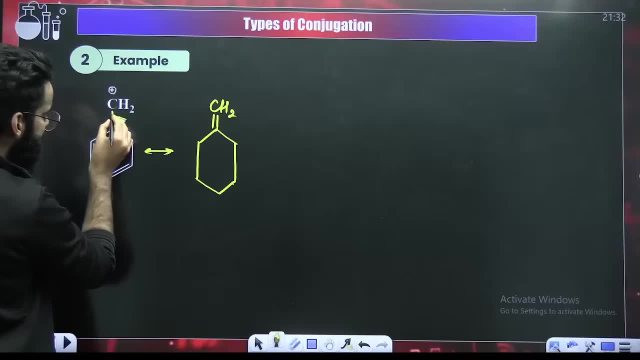 Since you have shifted this pi bond here. this was CH2 positive in the beginning. now it is going to be CH2 positive Since you have shifted this pi bond towards this Right. So I would say this particular carbon will be getting positive. 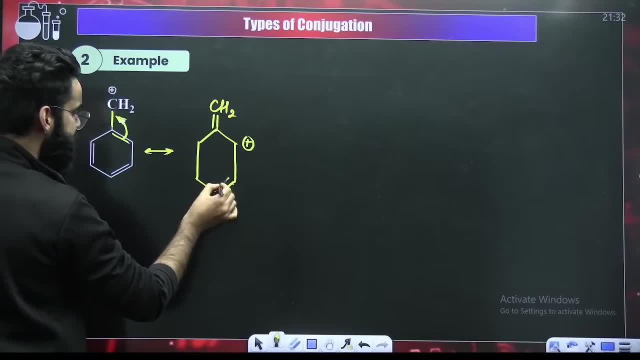 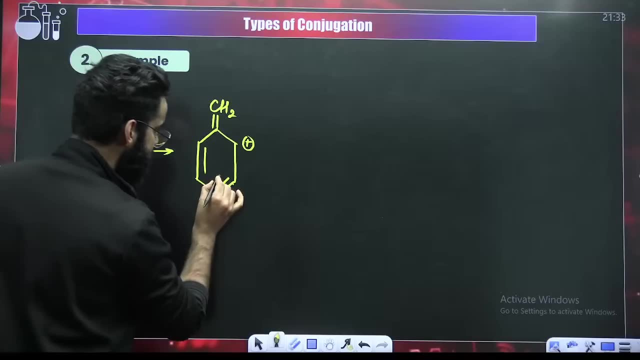 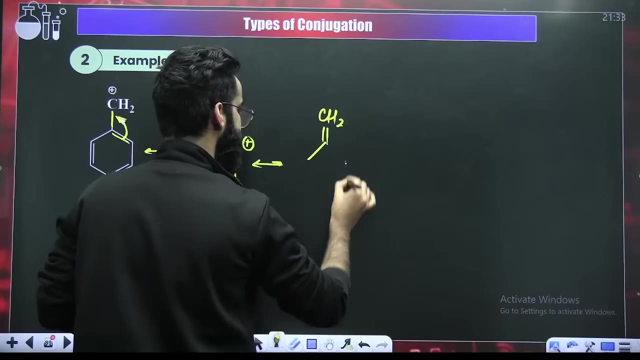 Right, It will be getting positive. Rest, everything is same. Now again, if you see, this is pi sigma vacant orbital, pi sigma positive, pi sigma vacant orbital. So again resonance. So this pi bond will shift here. When this pi bond shifts here, the other resonant structure will be like this: 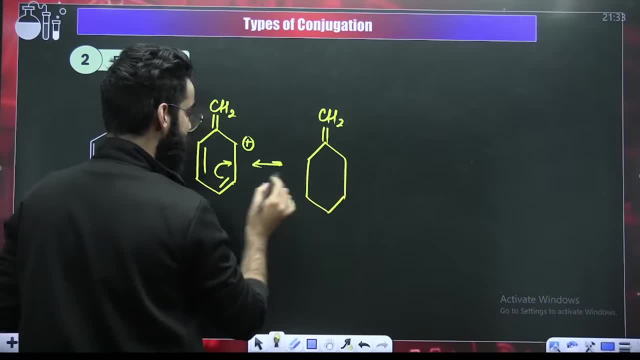 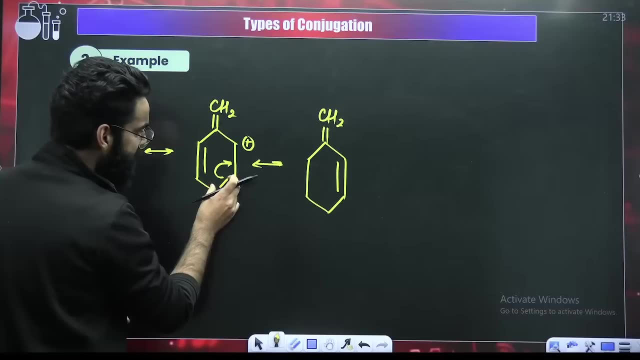 Guys, see exactly how do we make the resonant structures. See, there was a positive here. now pi bond is shifting Right From which carbon pi bond is shifting In this structure. In this structure, your pi bond was between these two. 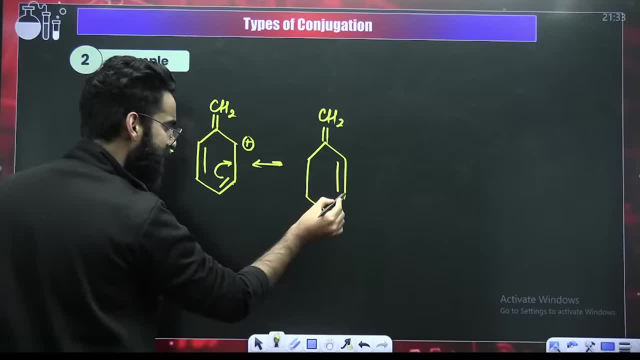 In this structure. your pi bond is between these two. So basically, this is the carbon at which pi bond is present, But pi bond is shifting from this carbon That carbon from which pi bond is shifting. that will get the positive charge Rest. everything is same. 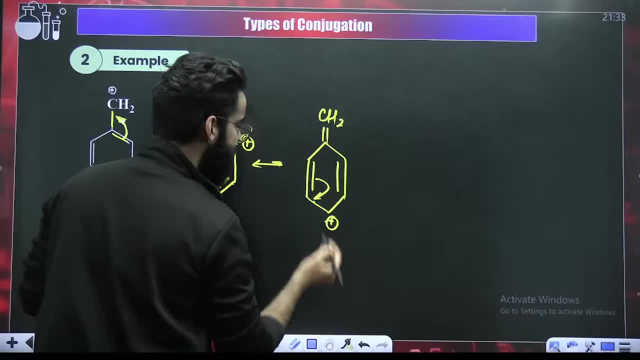 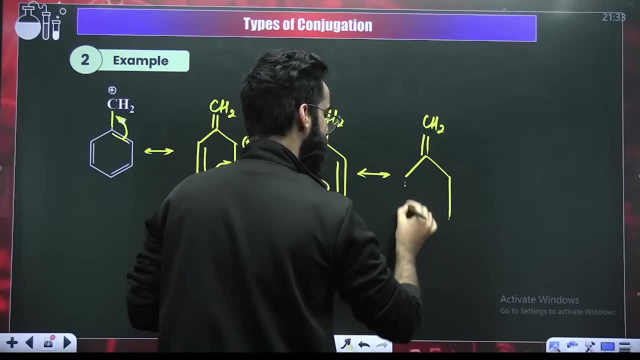 Again, if you see pi sigma positive, pi sigma positive, that means shifted in this direction, When you shift it in this direction, so what is one more conjugating structure which you will get? This is CH2.. And others: This is CH2.. 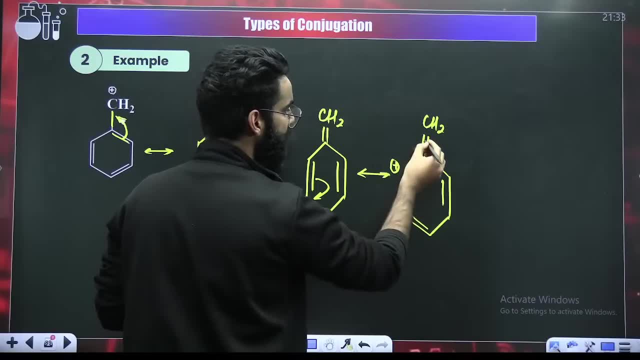 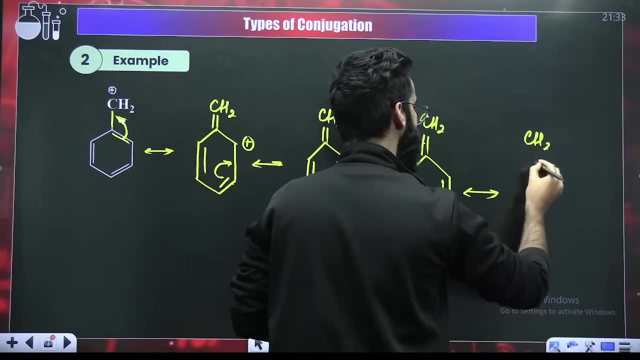 This is this Right, And this will get the positive. Now again, pi sigma positive. Pi sigma positive means shift in this direction. So what do we get at the end? This is CH2.. This is double bond. Sorry, not the double bond. 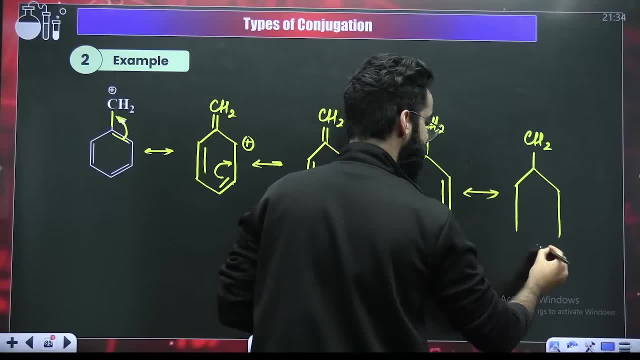 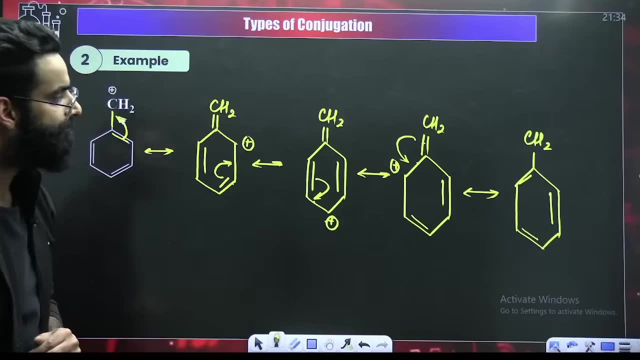 This is CH2.. This is single bond And rest, Rest, have a look, There will be a double bond here. There will be a double bond here. There will be a double bond here. Perfect Right, guys. Now, if you categorically look at one more important thing here, 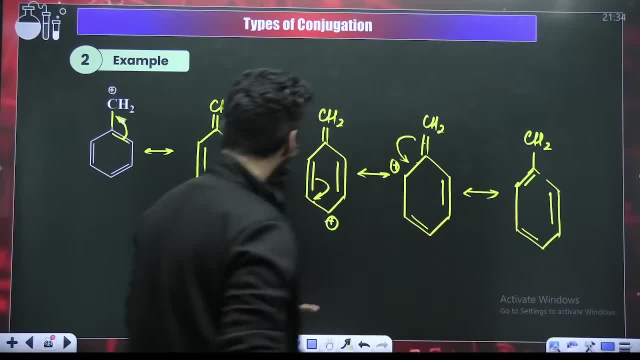 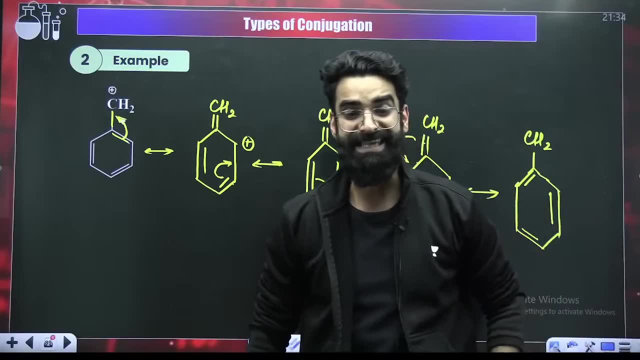 One more important thing, One more important thing, One more important thing here. Guys, look at the first canonical form and the last canonical form. If I ask you, are these same or different canonical forms? Are these same or different? First one and last one: are these same or different? 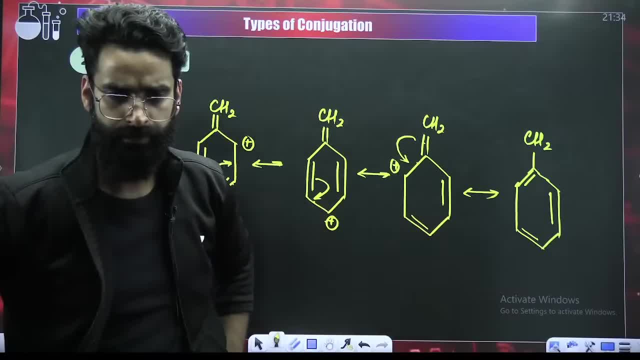 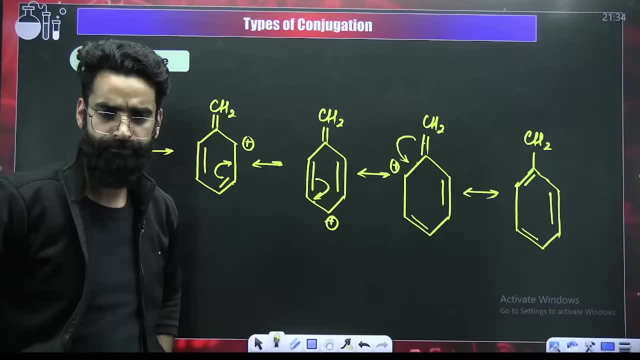 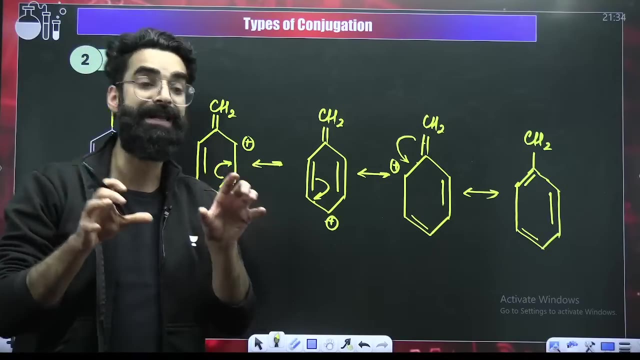 Are these same or different? Are these same or different? Quickly, First and the last: are these same canonical forms or different? See These canonical forms. they contain localized bonding. This canonical form is telling you there is a pi bond between these two. 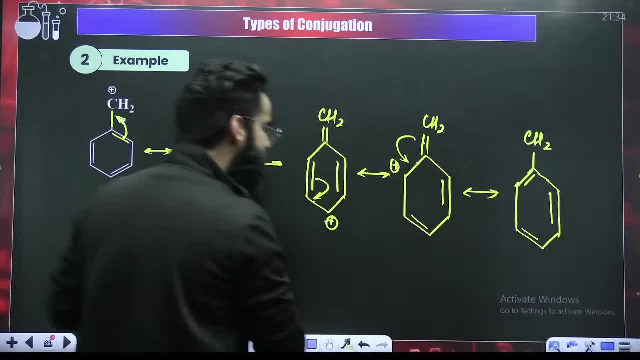 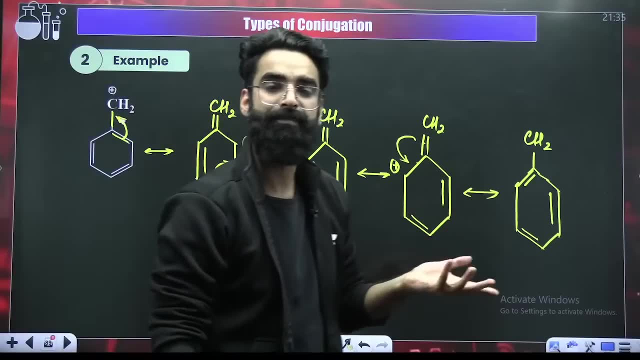 But the last one is telling you there is a single bond between these two, Right? So these two canonical forms, they are different, Right? No doubt they are different, but but, but, first and last, no doubt they are different. 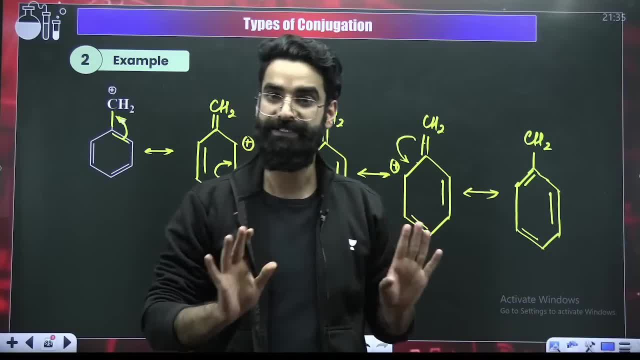 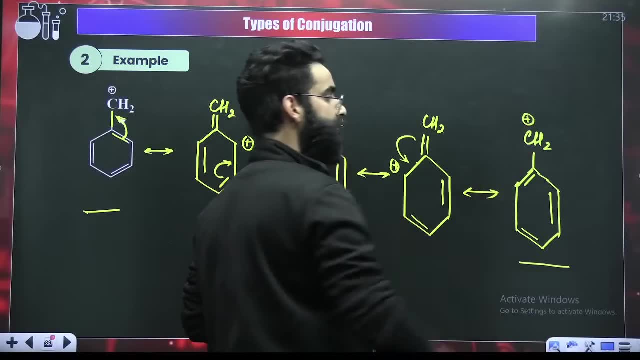 canonical forms, but let me tell you, their energy and stability will be the same. Look at both of them. Look at both of them. Look at both of them. This is a charge here. Look at both of them. Look at both of them. 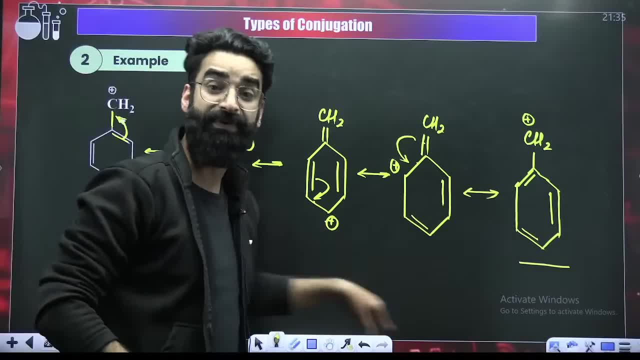 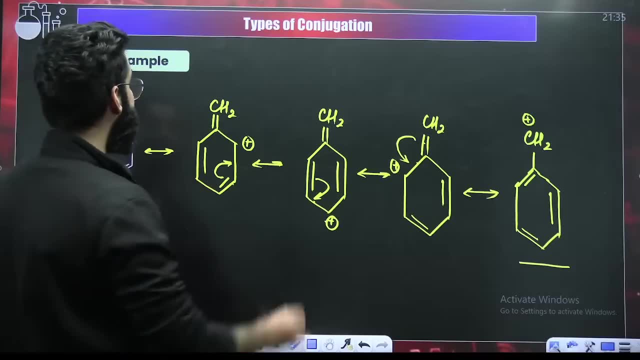 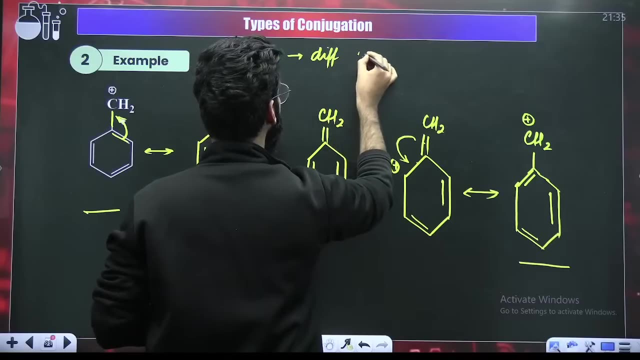 Right. So they are basically different canonical forms, but their- but their- energy and stability will be the same. Okay, So, first and last, Let me write it here. First and the last: They are actually different canonical forms. They are actually different canonical forms, but their energy and stability is same. 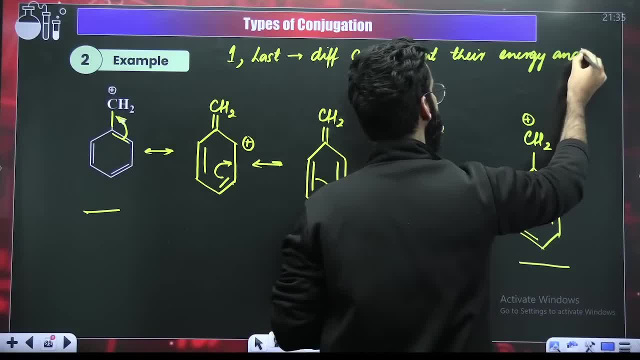 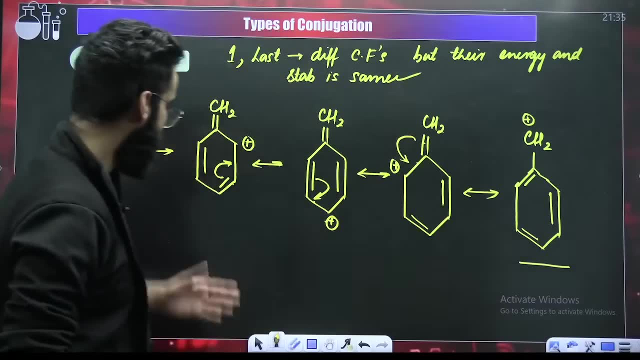 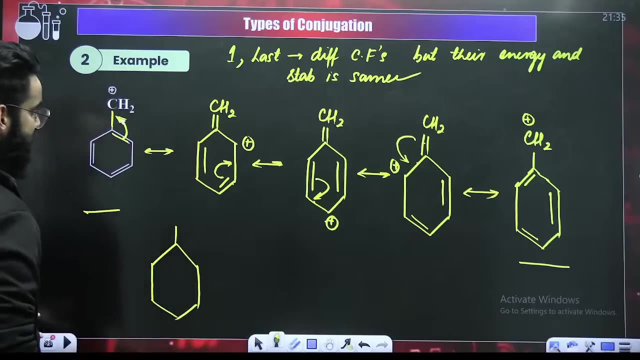 But their energy and stability are same, Right? Okay, energy and stability is the same, is the same, right. so, finally, if i want you guys to make the hybrid, you can easily make the hybrid. let's make the hybrid, people. let's make the hybrid. see, every bond here is getting the partial double bond character. this is getting 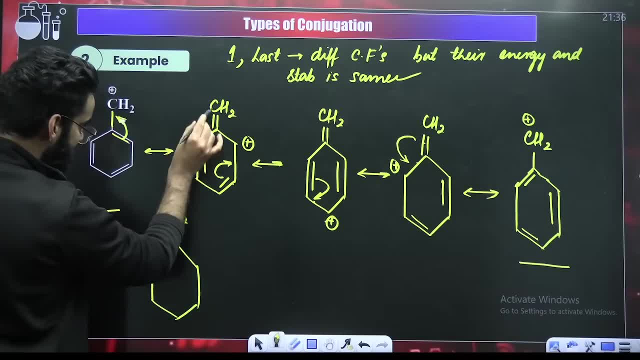 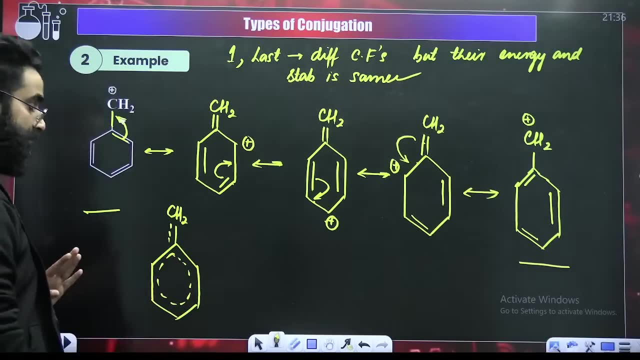 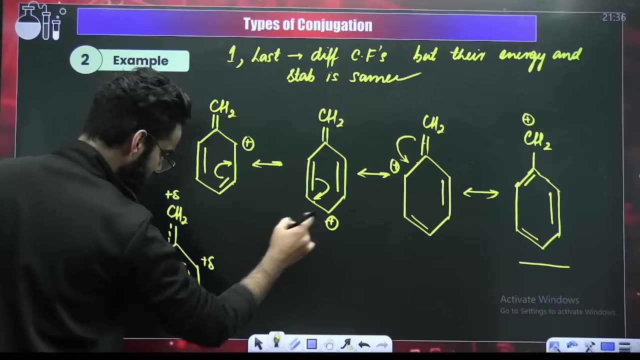 partial double bond. why? because here it was supposed to be single, but here it is double, so it will be partial double. right every bond there will be partial double bond character. there will be partial double bond character. number one: as per the first structure. this should have positive. as per this structure. this should have positive as per this structure. 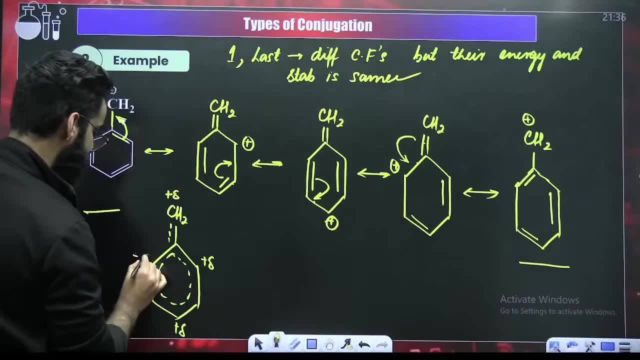 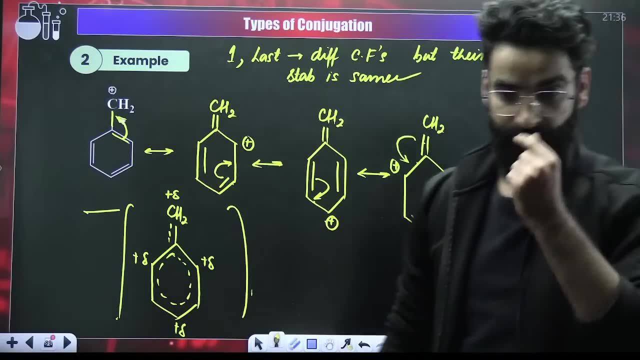 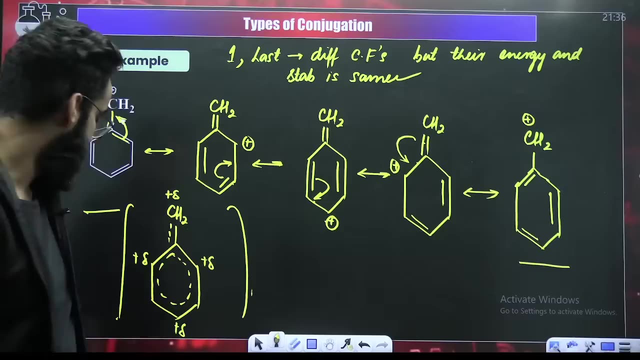 this should have positive and, as for this structure, this should have positive, perfect. so this is something which you will be calling as a hybrid right. this is something which is what you'll be calling as the hybrid perfect. is it clear, people, is it people? is it clear? 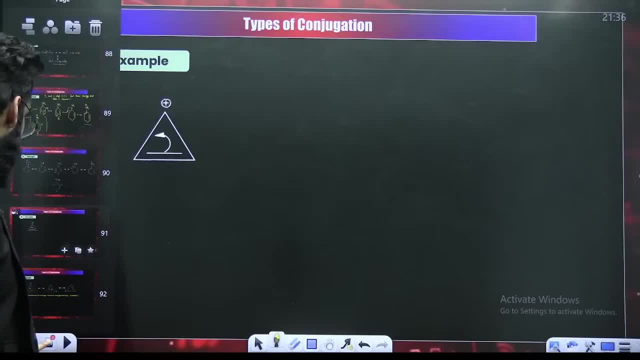 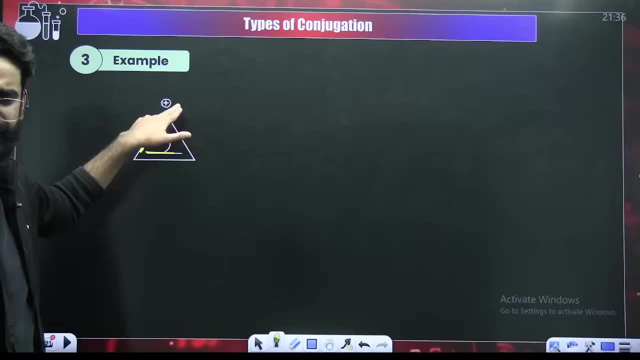 people quickly have a look, you've got again pi sigma, and here you've got positive pi sigma, vacant orbital. basically right, pi sigma, vacant orbital. if you see, every carbon here is sp2 hybridized. every carbon here is sp2 hybridized. so it's again pi sigma, vacant orbital. if it is pi. 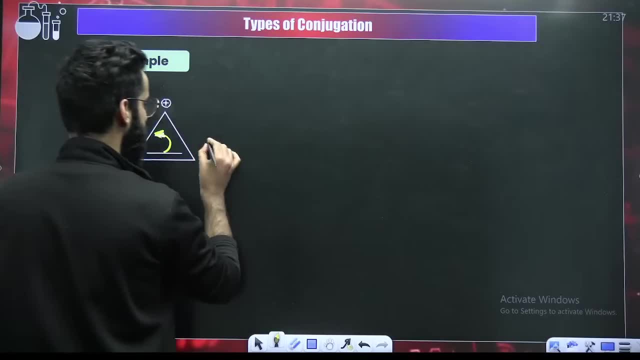 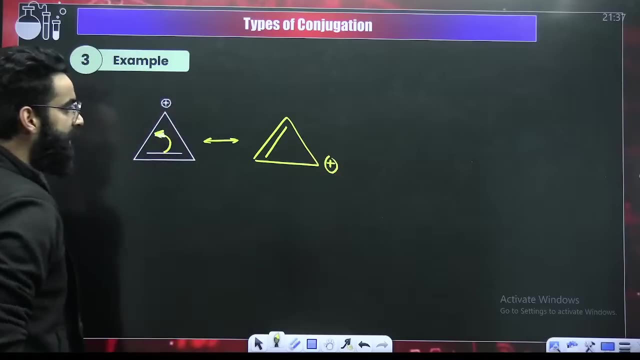 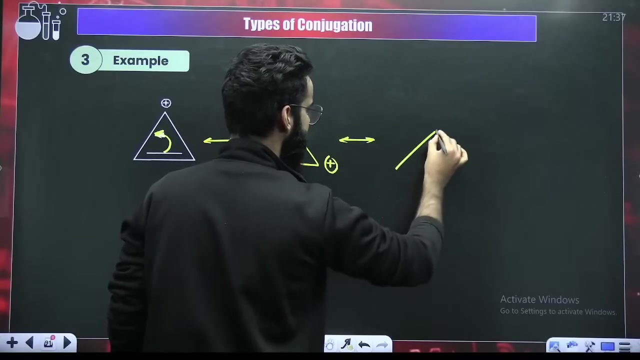 sigma vacant, orbital right, draw its structures. so it's one of the structure will be like this. so pi bond got shifted and now this gets the positive right. now again you've got pi sigma positive. Let me shift it here. When you shift it here, there will be a structure. 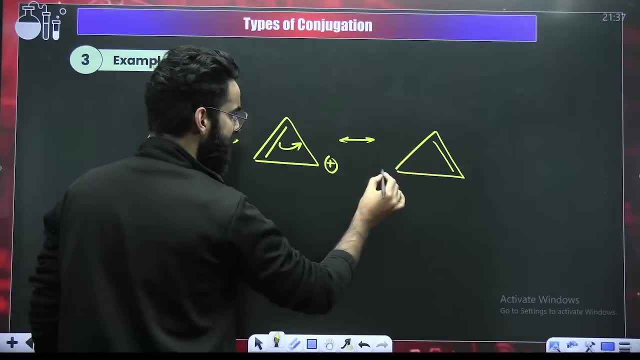 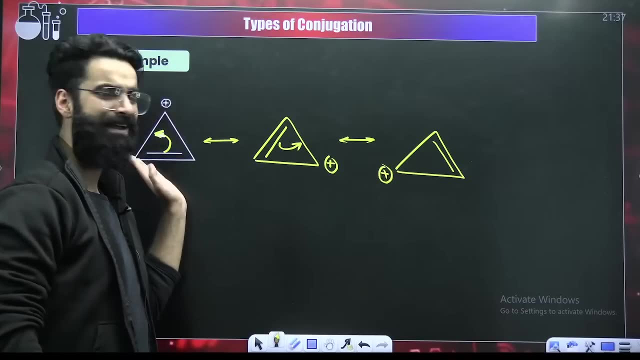 like this: Now there is a pi bond here and this particular carbon will be getting the positive Perfect. Now do you see First one and last one. First one and last one. Are they same or different? They are different, but their energy and stability will be same. 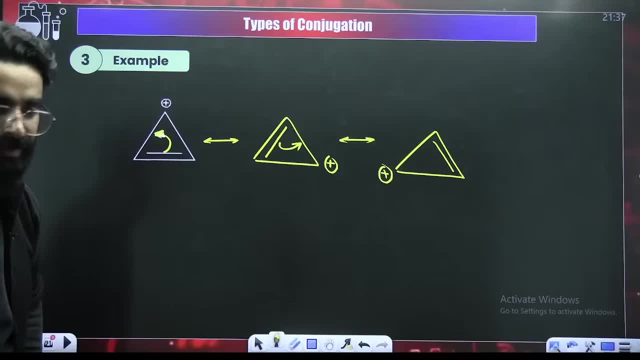 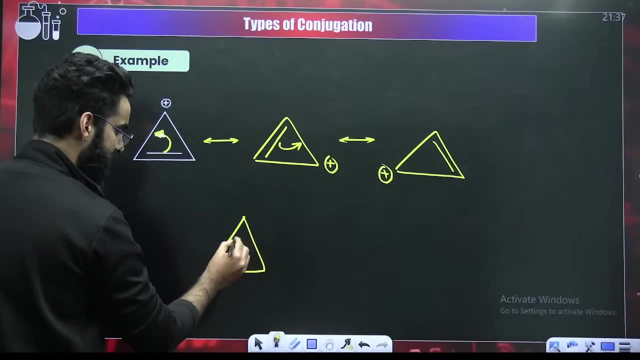 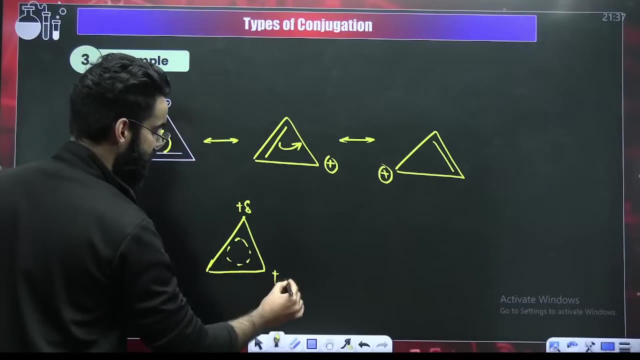 Okay, tell me one thing: How do we make the hybrid here? How do we make the hybrid? Every bond is getting partial double bond, right, Every bond is getting partial double bond As per the first structure- delta positive here. As per the second structure- delta positive. 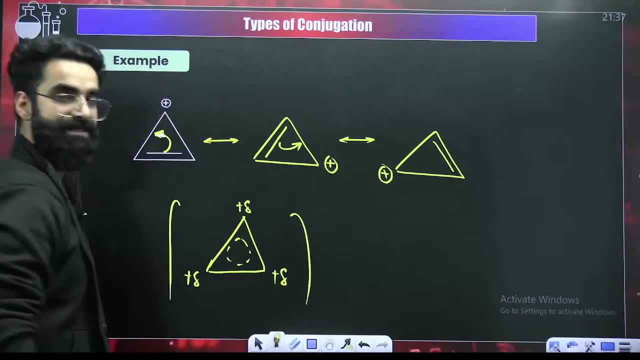 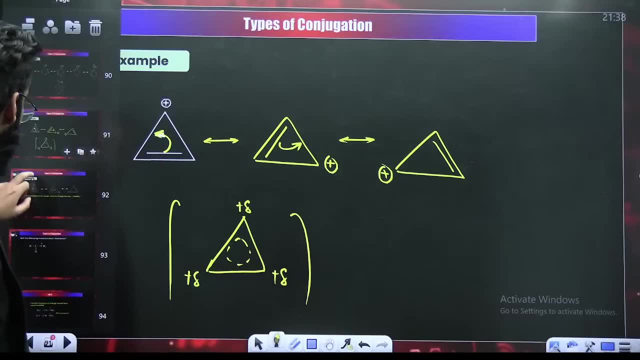 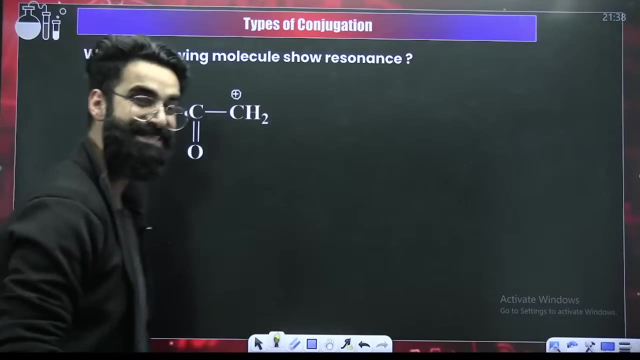 here. As per the third structure, delta positive here. So this, what you will be calling as hybrid and hybrid, will be maximum stable as per all these structures here. Okay, so this was your, this was your, This was your. pi sigma, vacant orbital conjugation. right Now, tell me one thing: Will the molecule 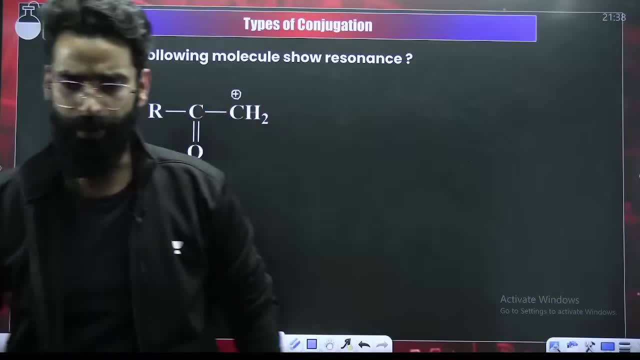 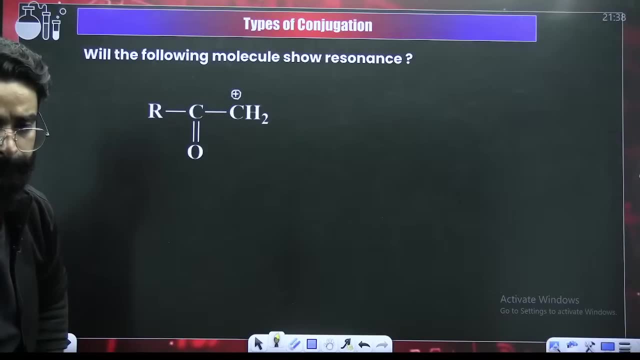 show resonance or not. What do you think? Will the molecule show resonance or not? Will there be resonance in this molecule You are going to tell me? Will there be resonance in this molecule? What do you think? What do you think I am asking you? It is a simple. 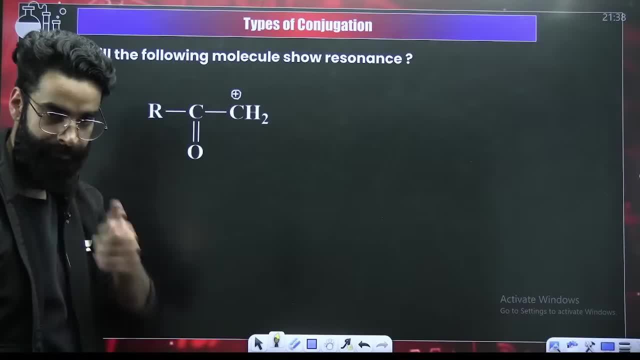 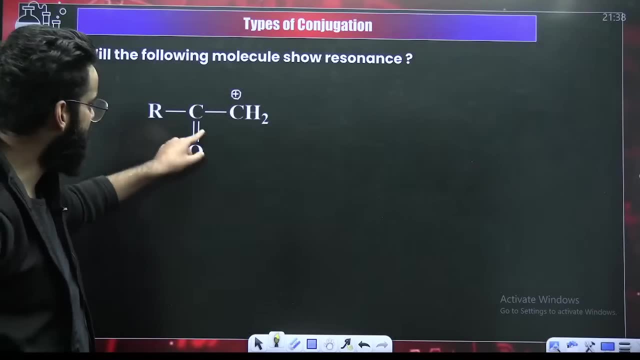 question I am asking you, It is a simple question. I am asking you, It is a simple question: Is there conjugation, Yes or no? See what you are saying here. You are saying: pi sigma positive, pi sigma vacant, orbital right. So there is conjugation, right? So 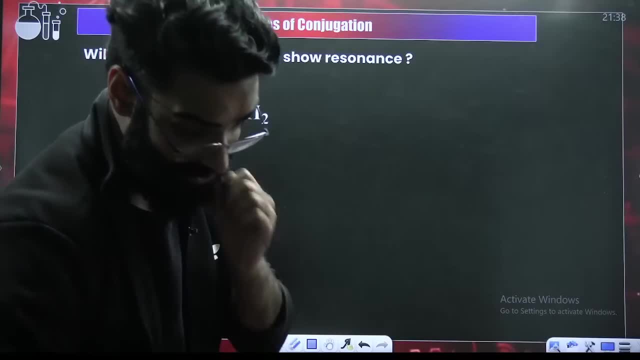 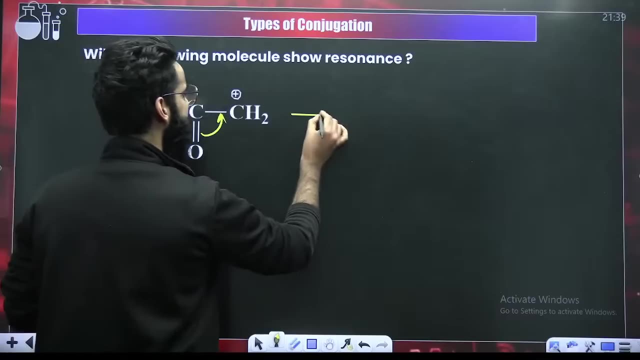 majority is saying: there is conjugation, Nice Good. If there is conjugation, that means it should undergo resonance. Most people just tried to understand. if it undergoes the resonance, this bond will shift here. Right, If this bond shifts here, what do we get? We got. 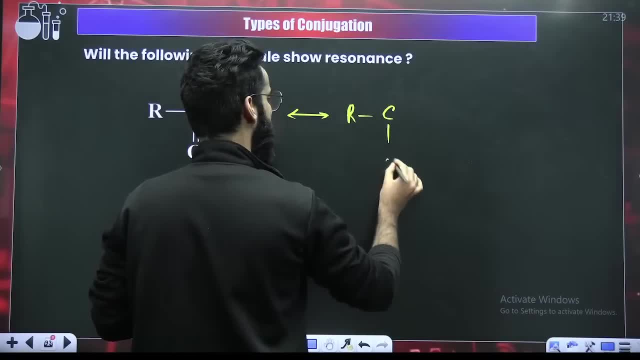 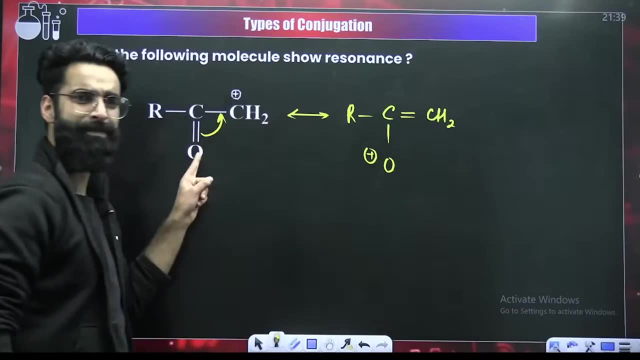 There is a bond length here. If there is a bond length here, what is this bond? Vouvel و R C. this is oxygen, since a bond is getting shifted from oxygen. so oxygen carries positive now and there'll be a double bond here. this will be CH2. if resonance happens here, this has to be its. 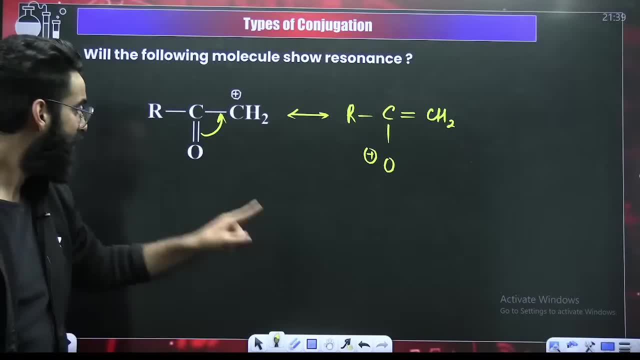 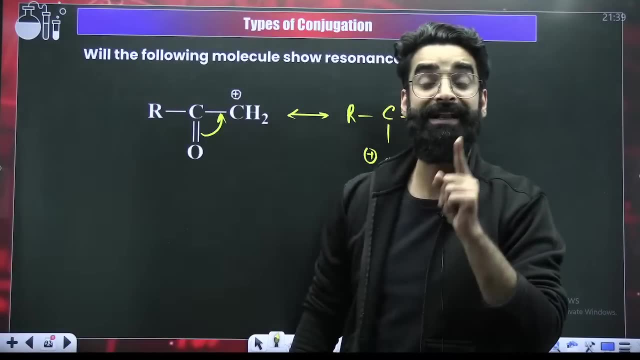 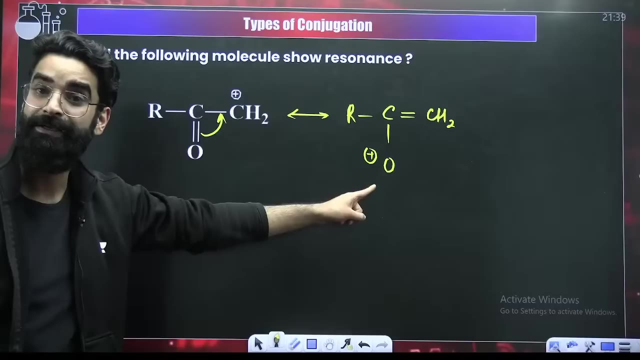 canonical form. but if you look at this form, oxygen was not carrying any charge. where oxygen is carrying positive charge, if you remember, positive charge on an electronegative element makes it highly unstable. positive charge on an electronegative element makes it highly unstable. so i would say, if this is i'm calling as canonical form one, this i'm calling as canonical form two. 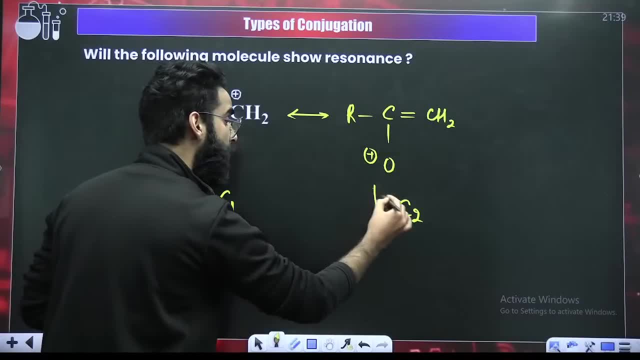 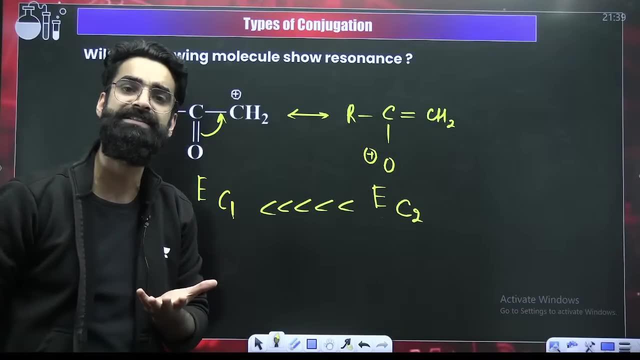 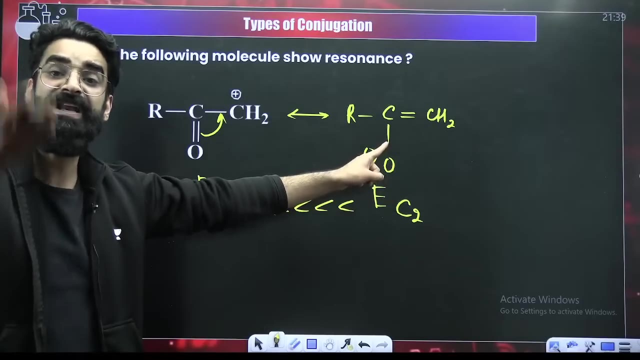 i would say energy of canonical form two will be will be higher than that of canonical form one. but we know, as for the property of canonical forms is concerned, canonical forms, they show same energy, similar energy, similar energy, but its energy is very, very, very high. so this cannot be its canonical form. so this molecule won't undergo resonance, understood. 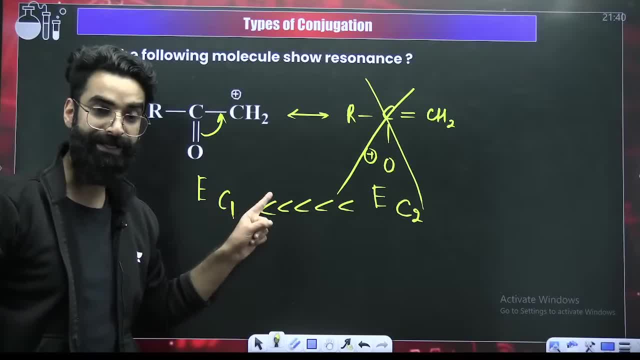 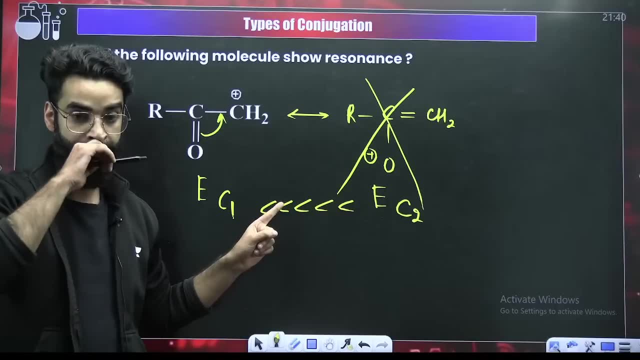 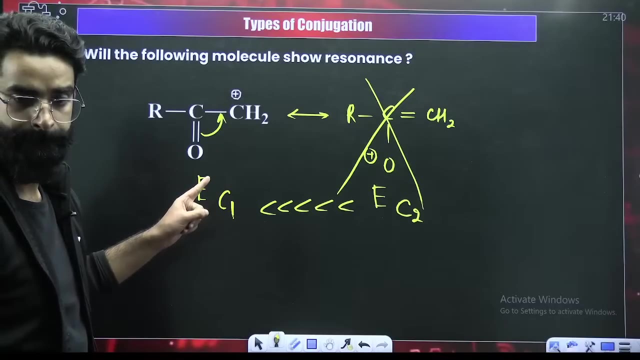 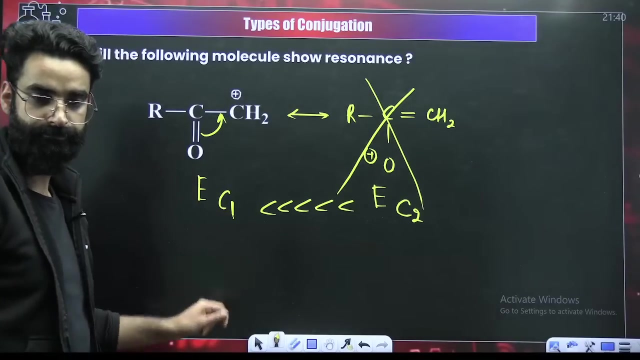 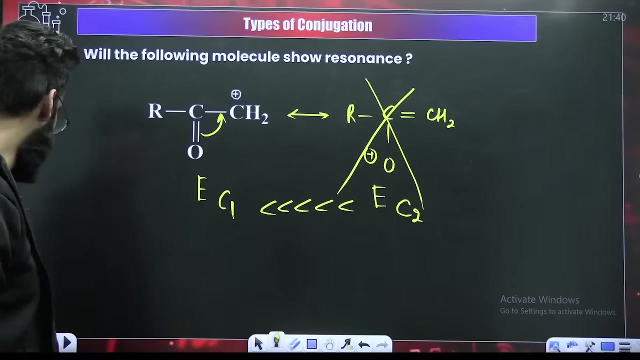 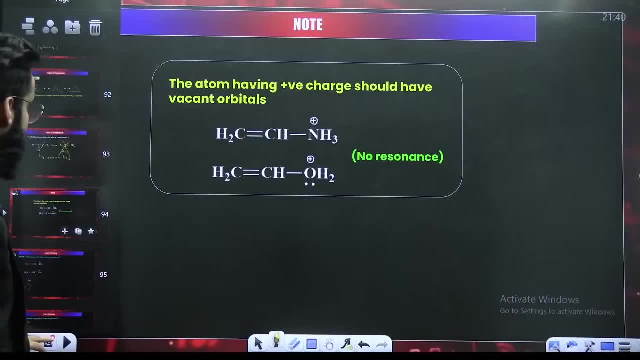 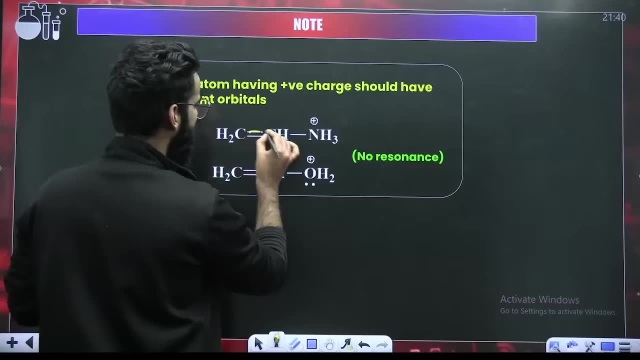 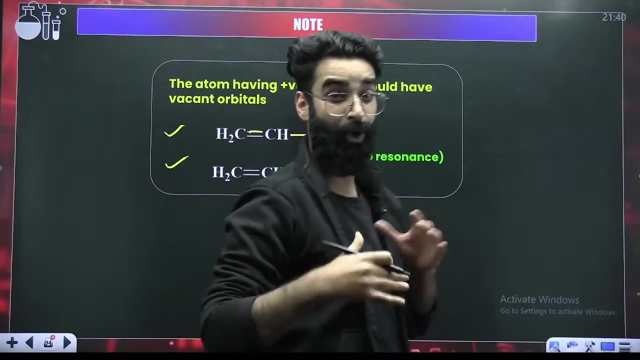 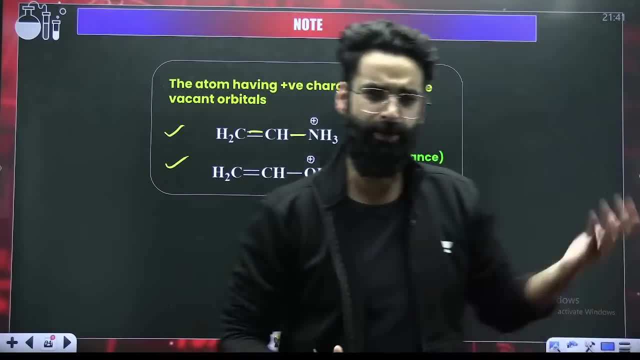 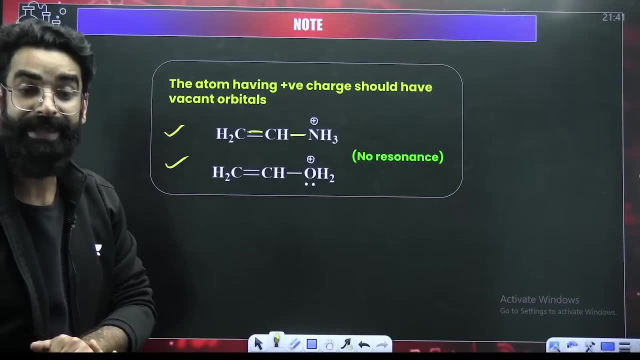 undergo resonance, right? if the concept of resonance is not clear, if you would have superficially, you will clearly say there is a conjugation: pi sigma positive, pi sigma positive, so it will undergo resonance. but I will say this will not undergo resonance. why? what is the reason? 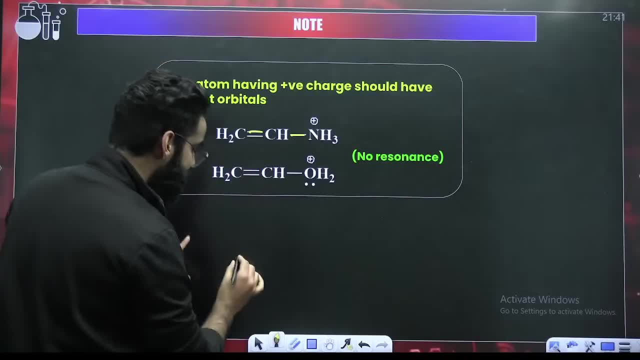 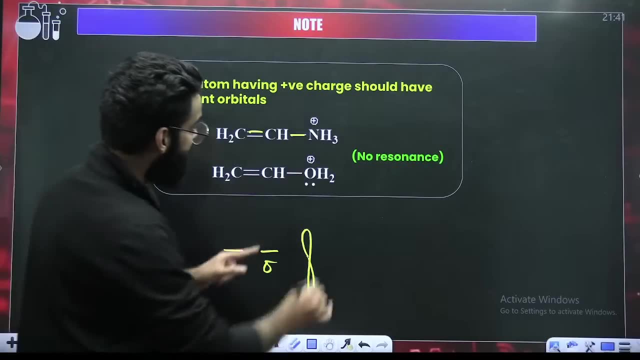 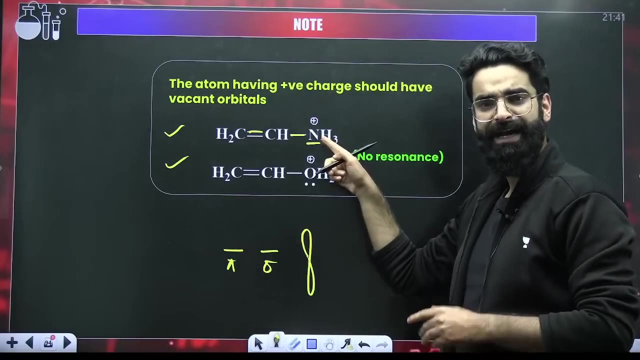 my dear students, conjugation is basically like this: this is pi, then there should be sigma, then there should be a vacant orbital. but look at this particular nitrogen. how many bonds it is forming. it is forming 4 bonds. if it is forming 4 bonds, its octet is complete. 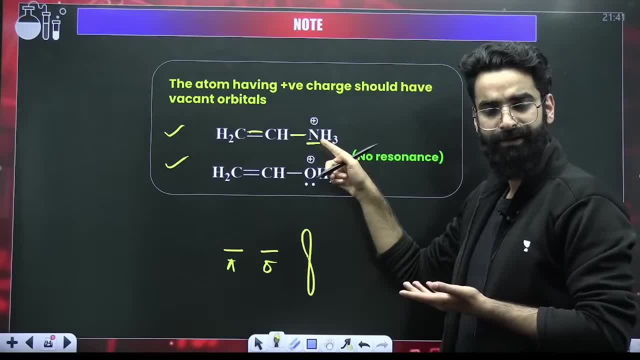 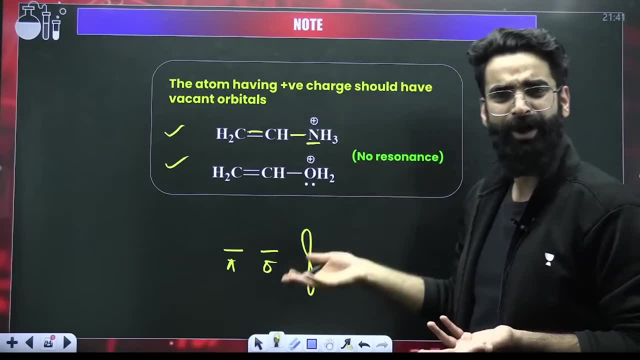 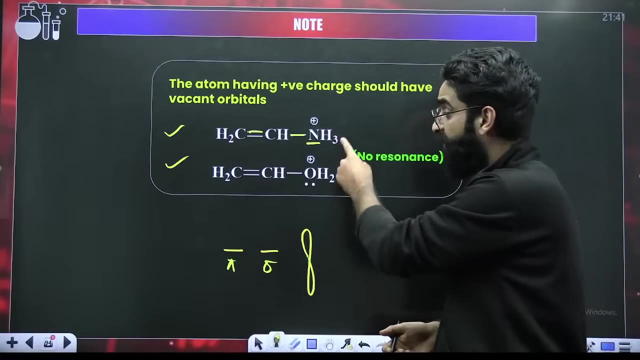 right, its octet is complete. if its octet is complete, will there be any vacant pi orbital? will there be any vacant pi orbital with this nitrogen? it is forming 4 bonds. this nitrogen is forming 4 bonds, so its octet is complete, so will there be. 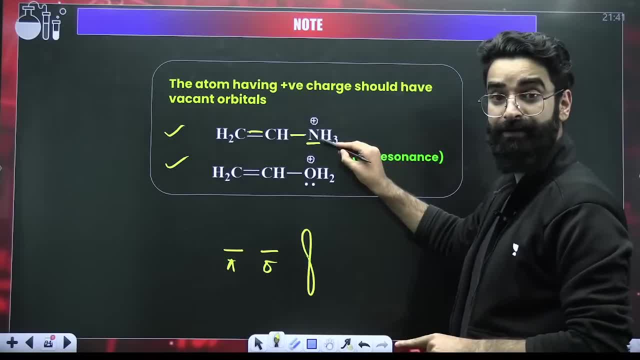 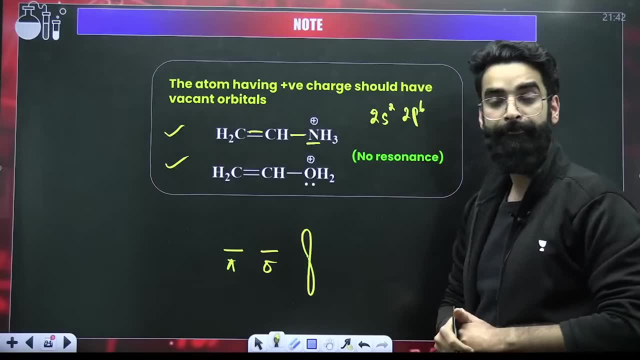 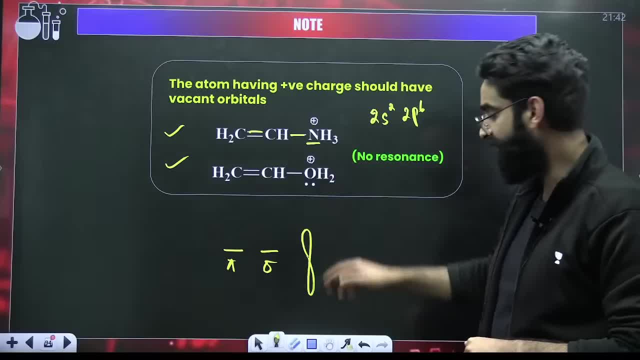 2s2, 2p6, 2s2, 2p6, 2s2, 2p6. right, so do you see any vacant orbital with nitrogen? do you see any vacant orbital with nitrogen? nitrogen does not have the vacant pi orbital here. 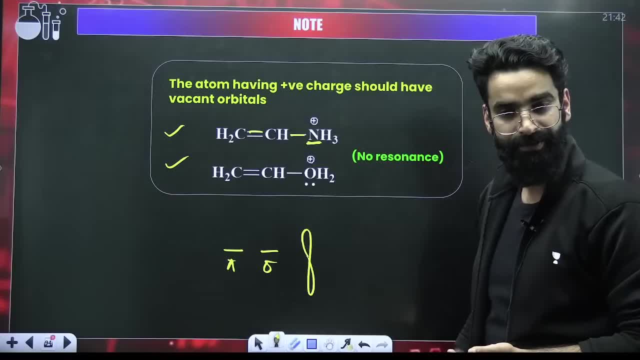 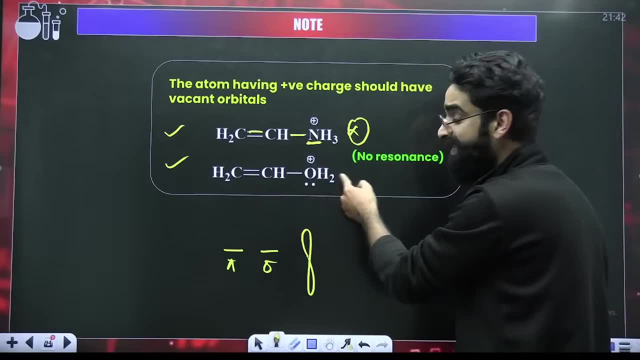 right, because all its pi orbitals are carrying the electrons now, so it is not going to show resonance. look at this one pi sigma vacant orbital should be present here. it is forming 3 sigma bonds, so 3- 2s are 6 and 2 electrons here. 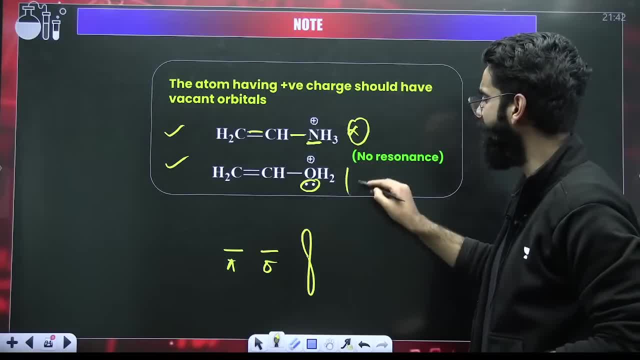 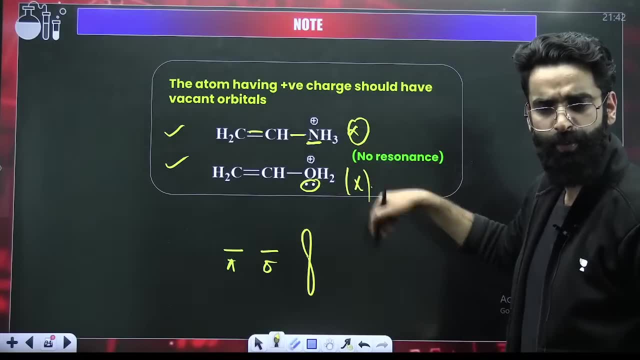 6 plus 2, 8. Its octet is also complete. If its octet is complete, it is not going to have any vacant p orbital. If there is no vacant p orbital- if there is no vacant p orbital- it is not going to. 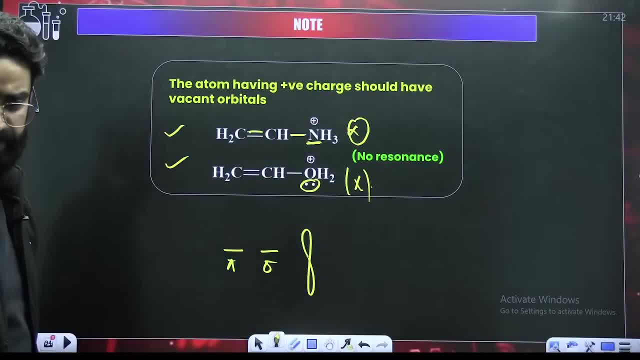 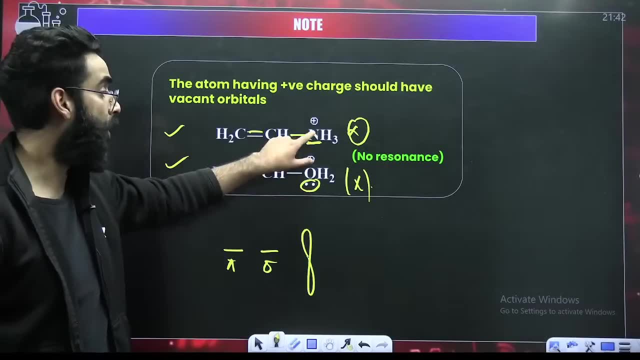 show any resonance here. Got this point. So these two are not going to show any resonance, Because there is no vacant p orbital here. The octet of this nitrogen and oxygen is complete. If the octet of nitrogen and oxygen is complete, there will be no vacant p orbital with them. 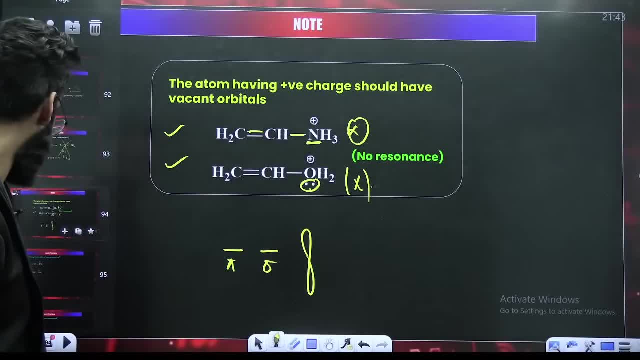 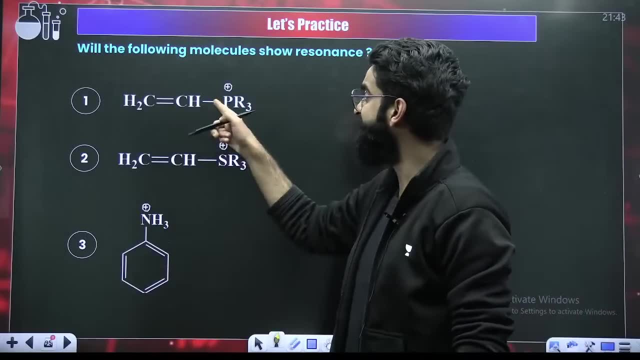 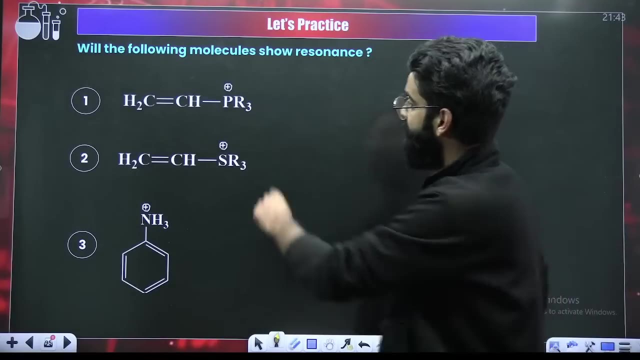 Yeah, Alright, Tell me, Tell me whether this molecule will show resonance or not. This is pi sigma positive, Whether they will show resonance or not. See, phosphorus is forming 3 plus 1.. 4 bonds, So its octet is complete. 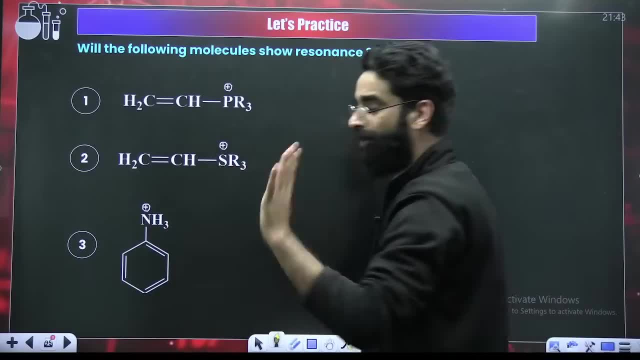 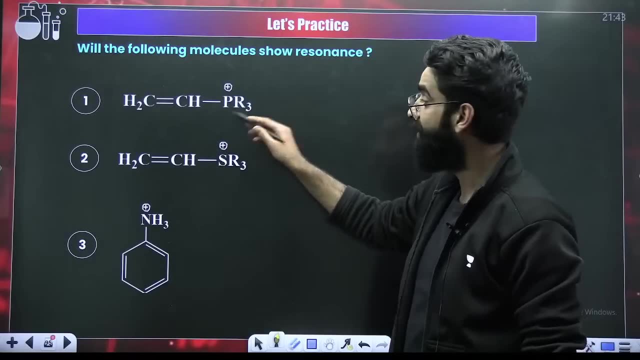 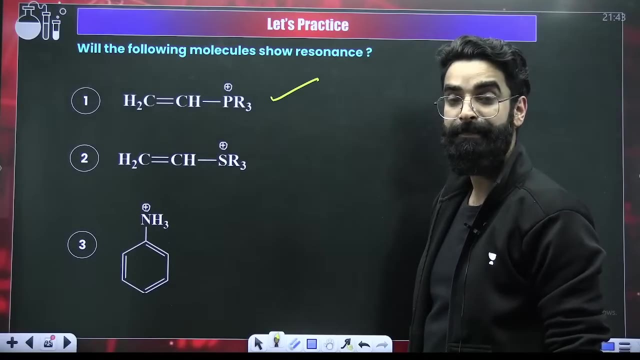 Right. Sulfur, its octet is complete. Nitrogen: its octet is complete, Right. Will this show resonance? This will show resonance. This will show resonance In phosphorus, say: nitrogen, phosphorus, Nitrogen, phosphorus. 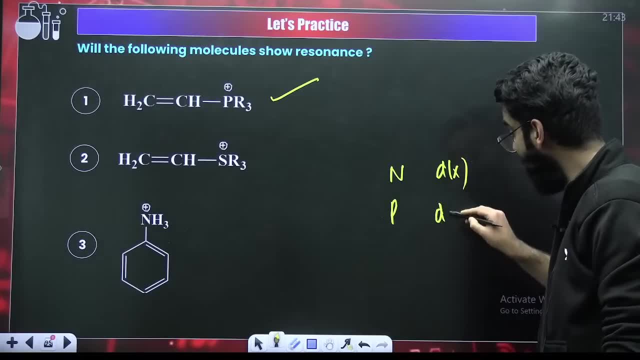 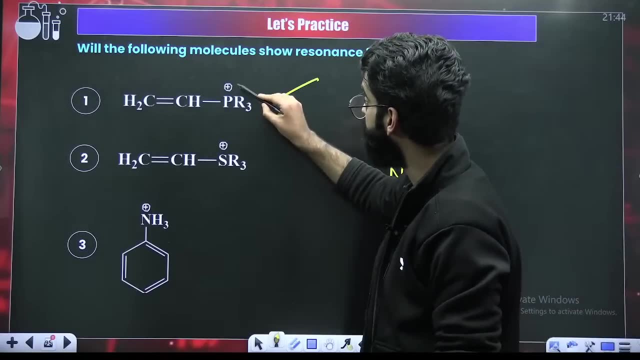 Nitrogen does not have any d orbital, but phosphorus has vacant d orbital. Phosphorus has vacant d orbital. Right Phosphorus has vacant d orbital. So I would say: phosphorus, over here, it has vacant d orbital. 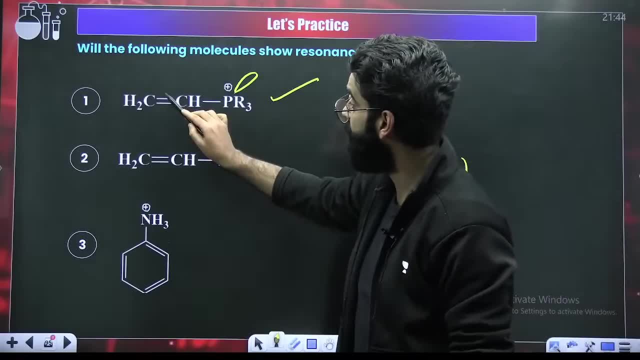 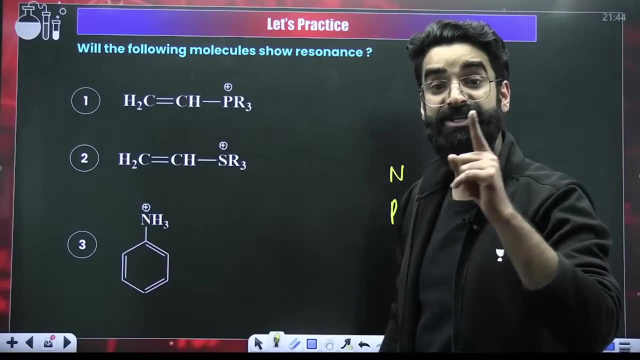 It has vacant d orbital. So the conjugation would be pi sigma vacant orbital, Pi sigma vacant orbital. Right I had categorically mentioned in the first case It has to be pi sigma vacant orbital. That vacant orbital can be p or d. 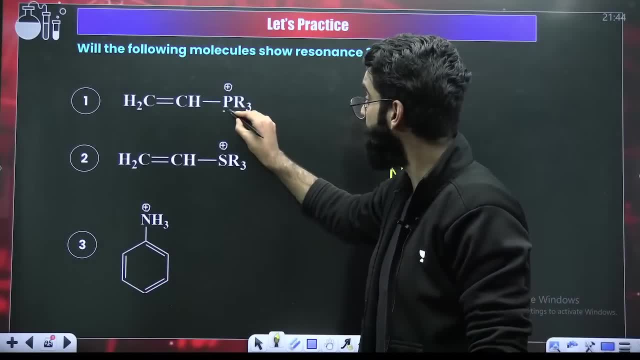 That vacant orbital can be p or d, Right, No doubt? It looks like it's forming 4 bonds. Its octet should be complete, But it has got vacant d orbital guys. Right, If there is a vacant d orbital. 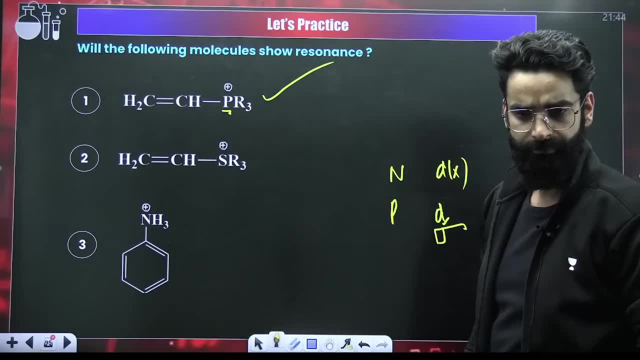 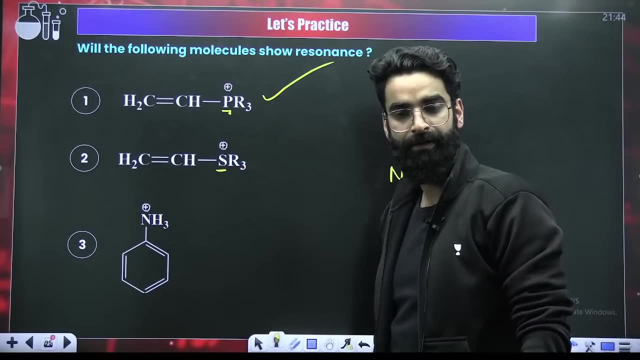 that means it will show resonance. Look at this one: Sulfur. Sulfur, 4 bonds. it's forming Octet complete. Now tell me Sulfur, Does it have vacant d orbitals? Sulfur has d orbitals Right. 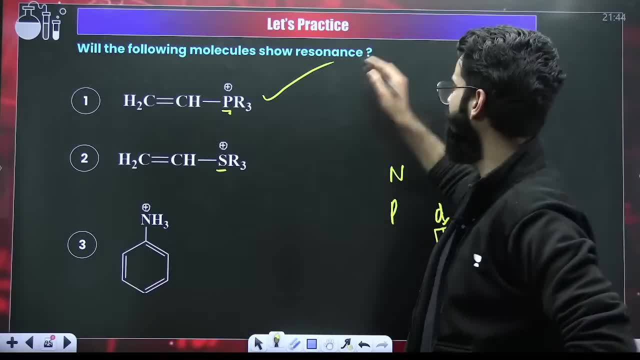 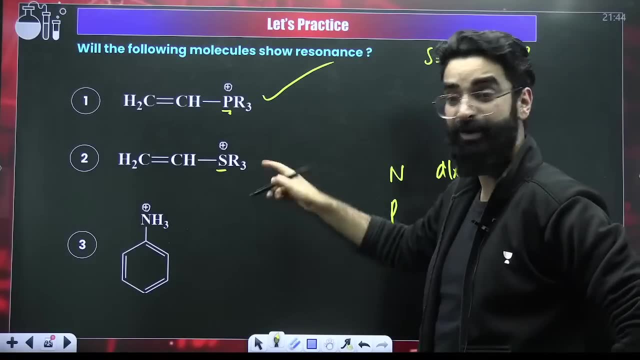 There is a vacant d orbital with sulfur. What is the electronic configuration of sulfur outermost? It is 3s2.. It is 3p4.. There is 3d as well, which contains 0 electrons. So it has vacant d orbitals. If it has vacant d orbital, 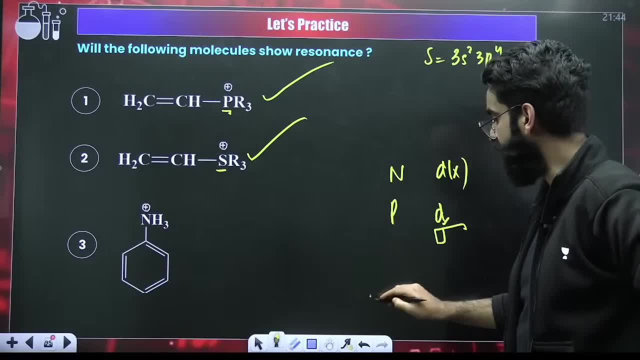 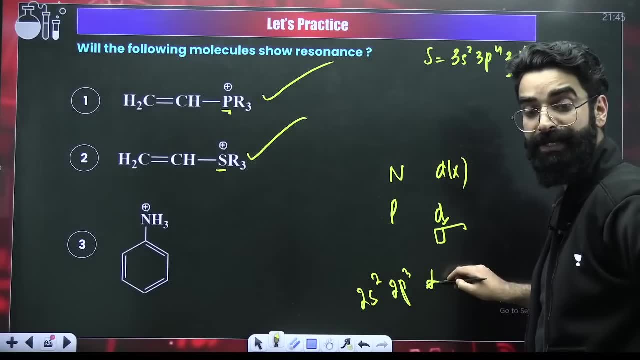 it will show resonance. But nitrogen, Nitrogen, Nitrogen. If you look at the configuration of nitrogen 2s2, 2p3.. Is there a any d? There is no d in nitrogen. There is no d in nitrogen. 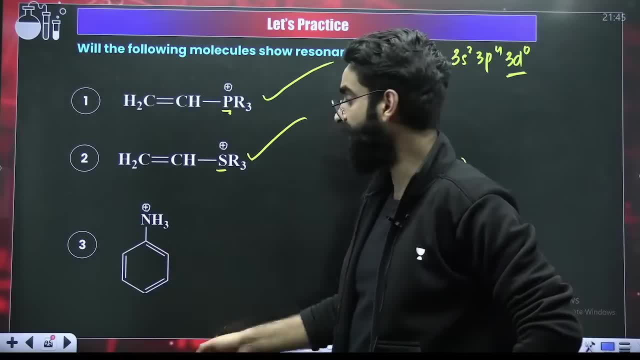 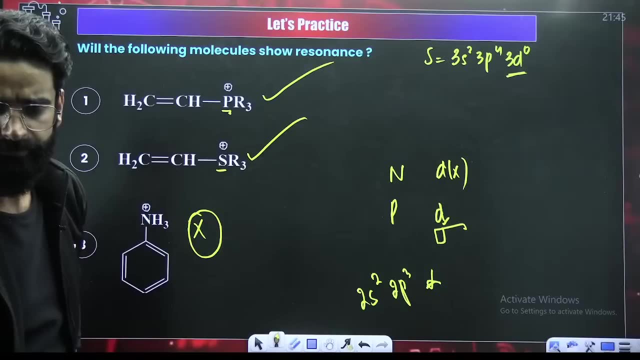 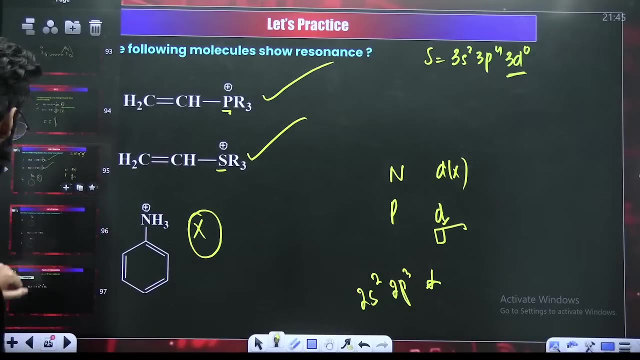 Right, There is no d in nitrogen. If there is no d in nitrogen, this will not show resonance. Is it clear? Is it clear? Is it clear, guys? I hope you can analyze from now onwards which one can show resonance, which one cannot. 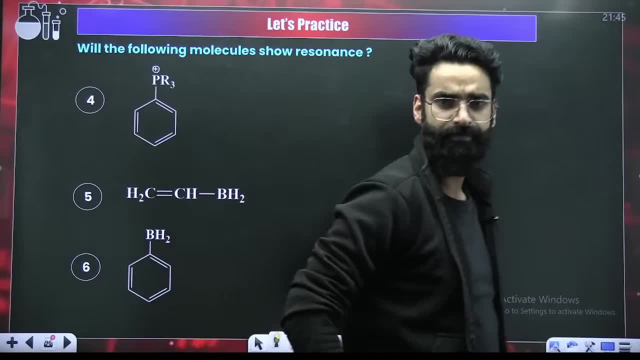 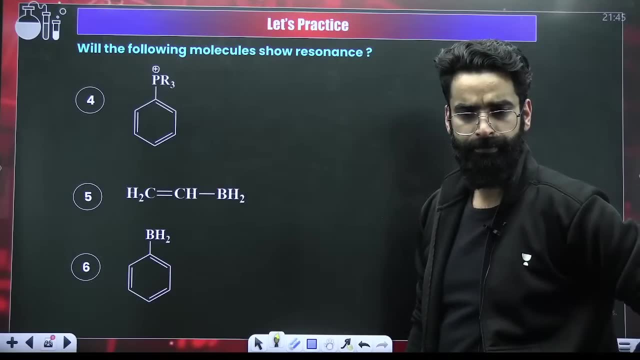 Okay, Among these 3.. Among these 3.. Quickly, Among these 3.. Is the first one going to show resonance? Is the first one going to show resonance, Yes or no? Every one Is the first one going to show resonance. 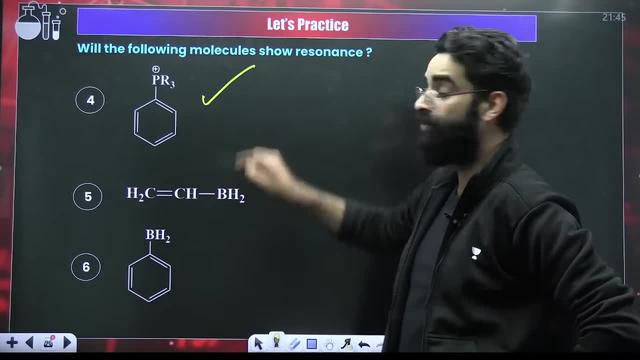 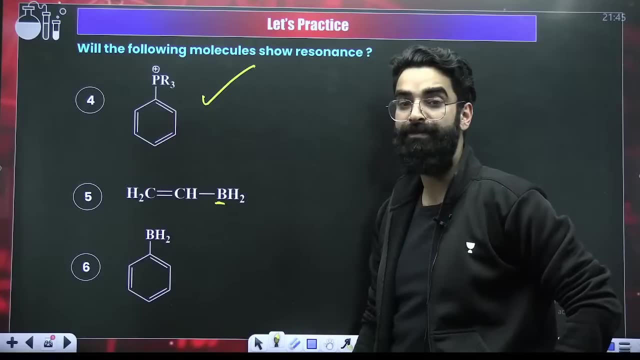 This is pi sigma and it will have this. phosphorus will have vacant d orbital. It will show resonance, right? What about the second one, Pi sigma? Look at this boron, It's forming. how many bonds? 3 bonds. 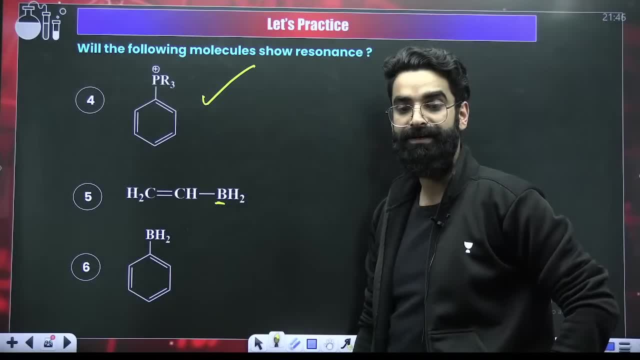 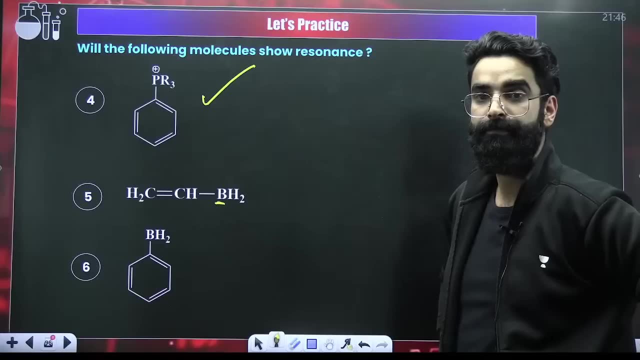 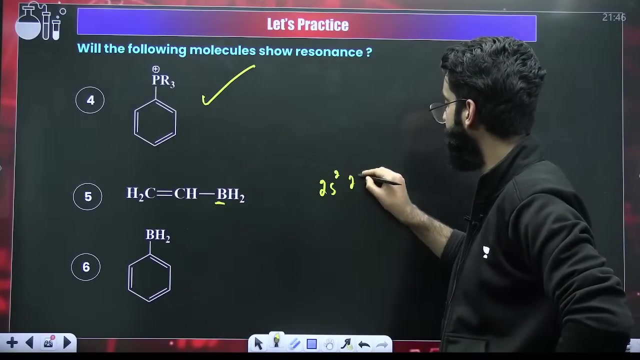 It's forming 3 bonds. right, it's forming three bonds. quickly tell me, is this particular molecule going to show resonance or not? quickly tell me, is it going to show resonance or not. if you look at boron guys, what is the outermost configuration of boron? it is 2s2, 2p1, correct, this is 2s carrying two electrons. 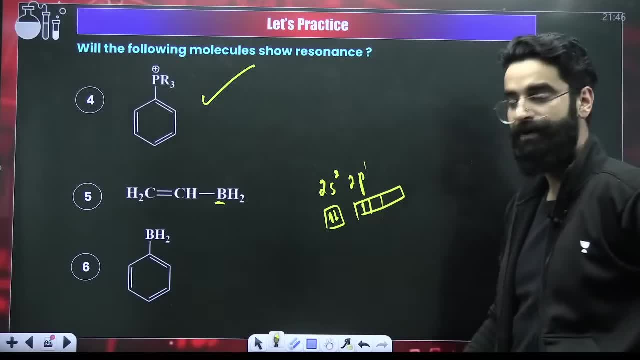 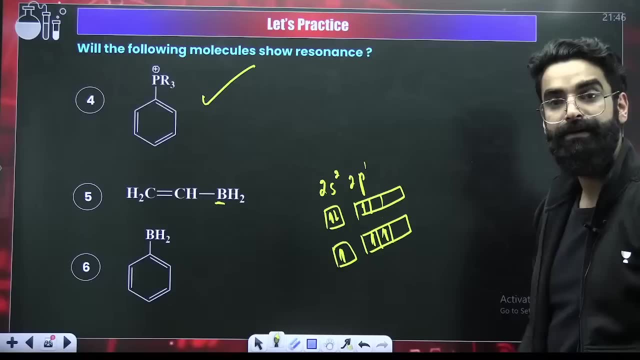 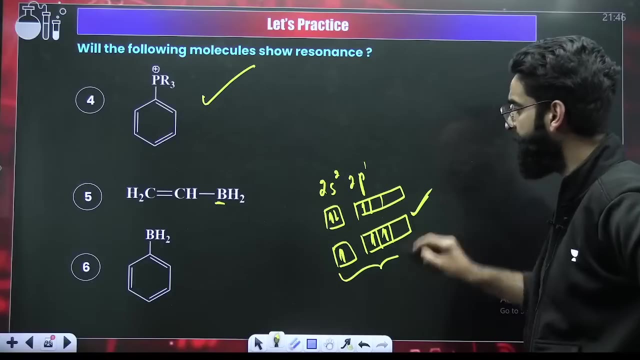 and 2p carrying one electron. 2p carrying one electron now, after the excitation is done. after the excitation is done, one electron here, one electron here, right, okay, how many bonds it's forming? it's forming three sigma bonds. three sigma bonds means sp2. this sp2 is there, the vacant p? 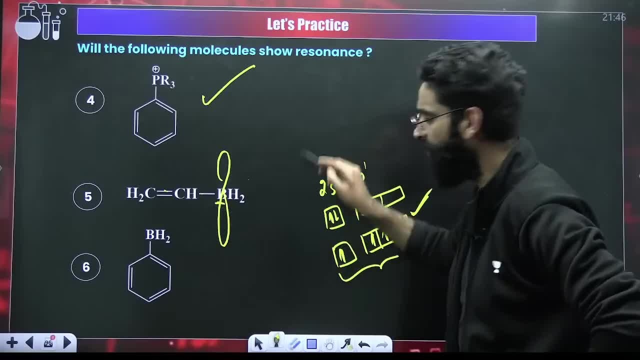 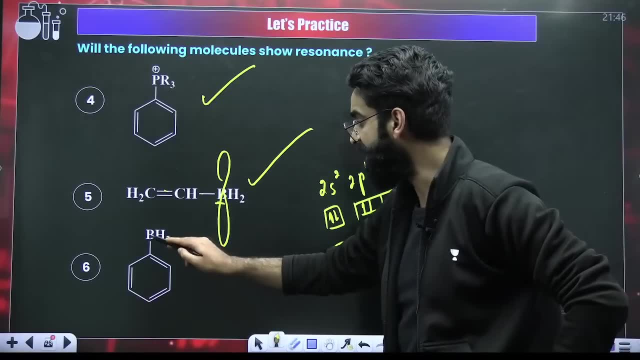 orbital. yes, this boron has vacant p orbital. so pi sigma, vacant p orbital absolutely will show resonance. right, look at this one, look at this one, is it going to show resonance? pi sigma, again the similar scenario. this will show resonance. so all these three will show resonance. 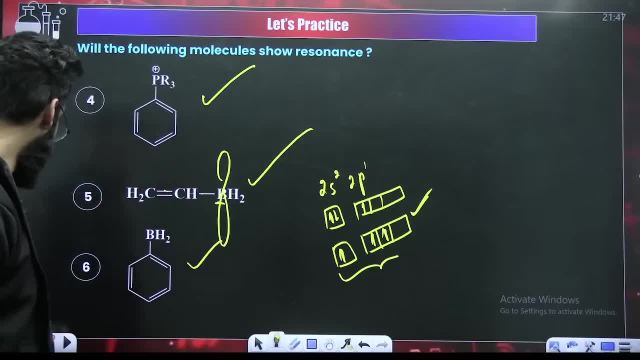 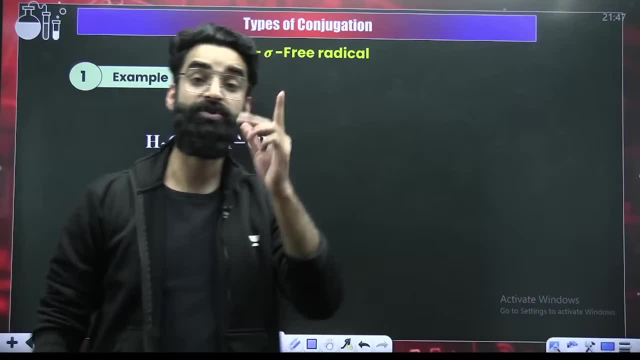 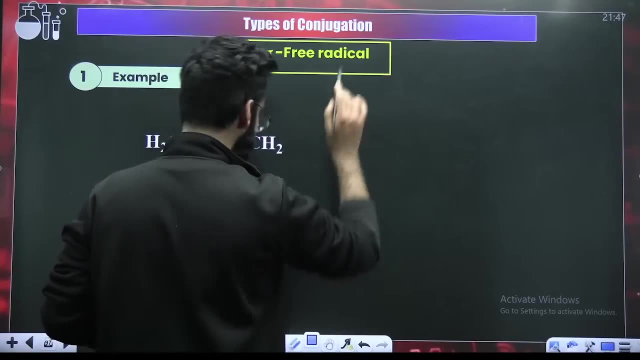 right, all these three will show resonance. i hope this is again clear to everyone. now there is one more conjugation. so till now i showed you one conjugation. what is that? what is that? that is your pi sigma vacant, orbital conjugation. the second one is pi sigma free radical conjugation. pi sigma free radical conjugation. right, have a look. 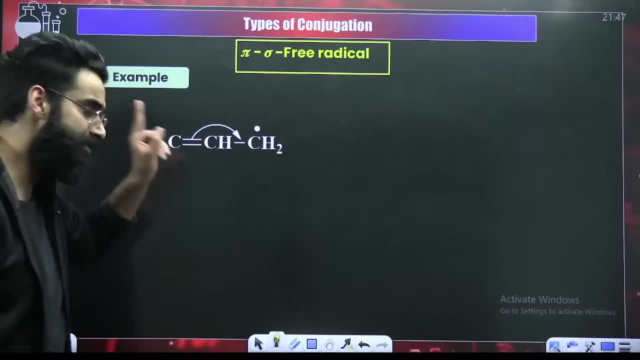 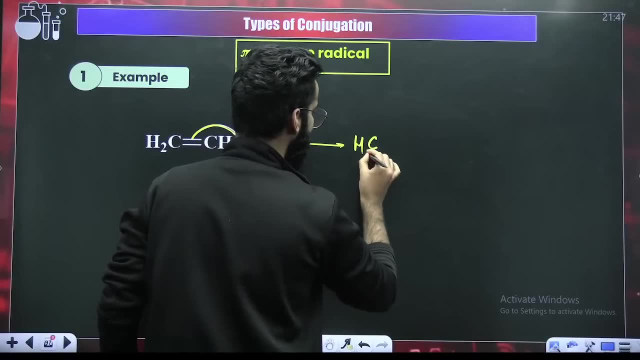 pi sigma radical, pi sigma radical conjugation is there, so it will undergo resonance right. so when you shift the pi bond on this side, when you shift the pi bond on this side, the ch2 will get a radical right. and this was a double bond here, now it's going to be a single bond. this is ch now. now. 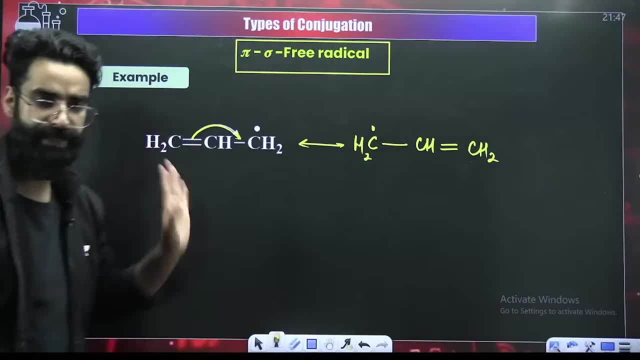 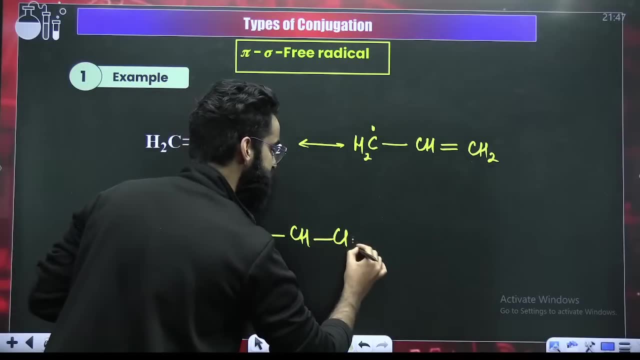 it's going to be double one, so it's going to be ch2 like this. so this is one more canonical form of it. now, if you want to make its hybrid, so make it simple: ch2 everywhere, keep a single bond for ch. this is ch2 right now. there's a double bond here, but this structure is telling single bond. so 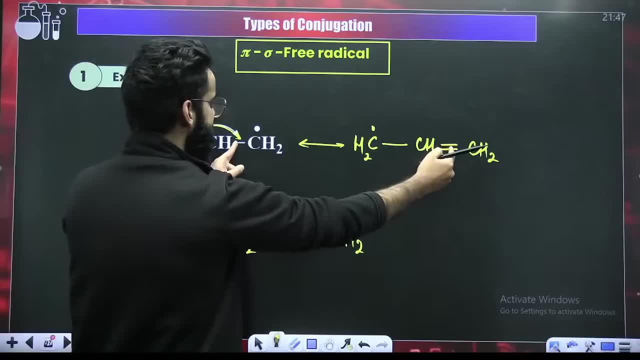 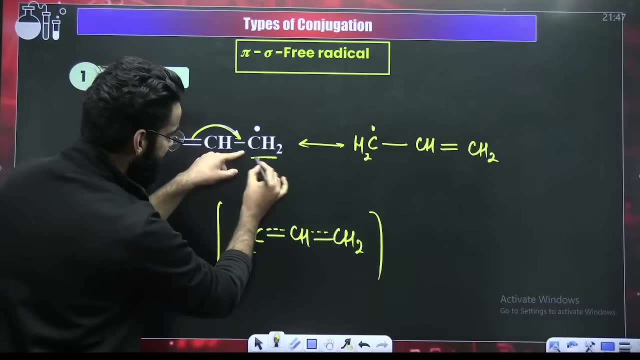 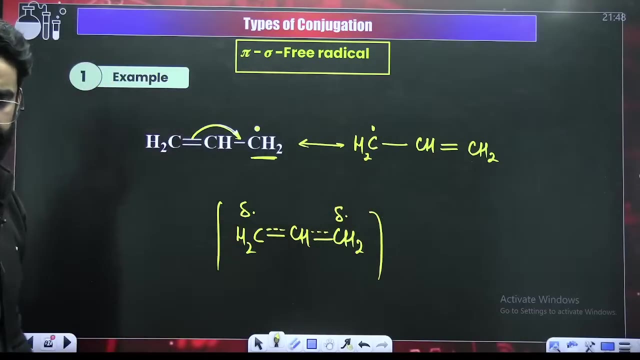 neither single nor double, partial double. single, but this is saying double. neither single nor double, partial double. now look at this particular resonance, hybrid, see, as per this particular structure is concerned, this having a radical, so have a radical here. as for this structure, this having a radical, so have a radical here. delta radical, right, so this is the hybrid, this is the 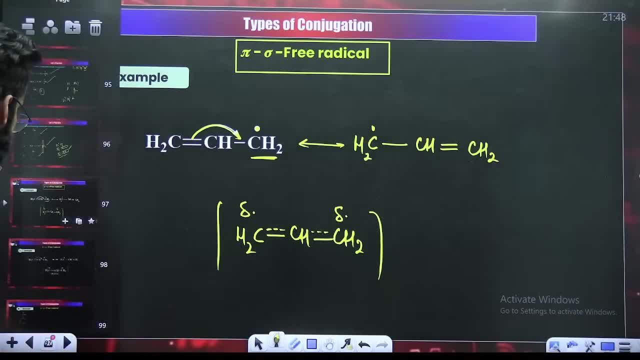 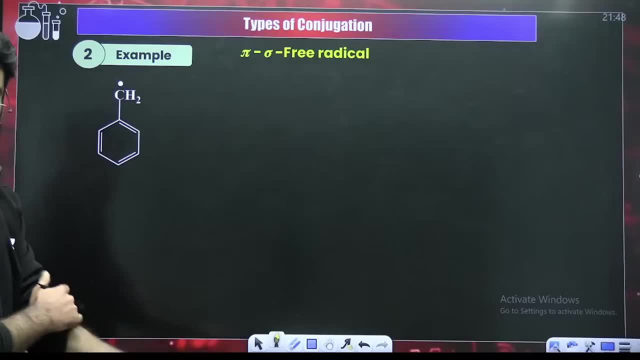 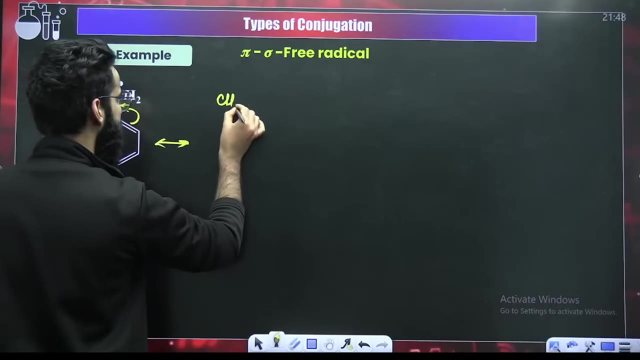 hybrid people clear: this is the hybrid. make its resonating structures. how will you make its resonating structure? see pi sigma radical. so shift this pi bond in this direction. when you shift the pi bond in the direction, this is ch2. now it's going to be a double bond, right. 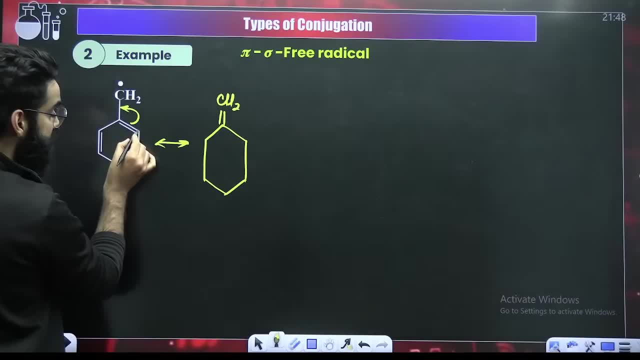 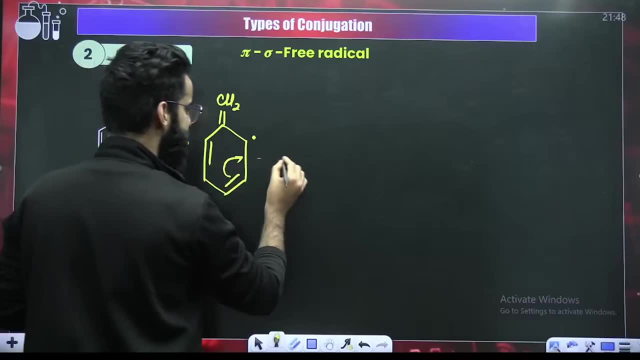 that carbon from which the bond has been shifted, from this carbon bond has been shifted. i'll put a radical here. rest. everything is same. now it's again pi sigma radical. if it's pi sigma radical shifted in this direction. when you shift in this direction, what do we get? 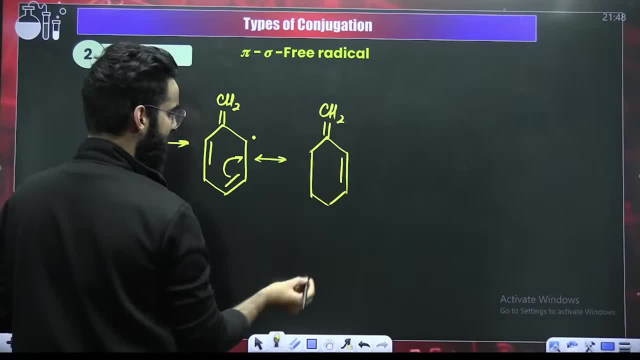 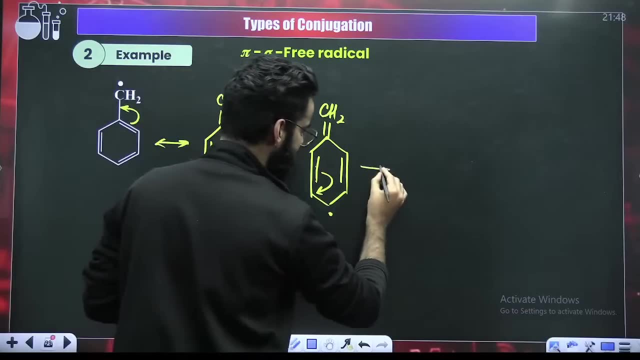 try to understand. what do we get exactly? this is your pi, here you will be getting the radical, and here is a double bond. perfect, now again, this is pi sigma radical, right. so shift in this particular direction. so what do we get again? this is ch2, this is double bond and rest, i believe. 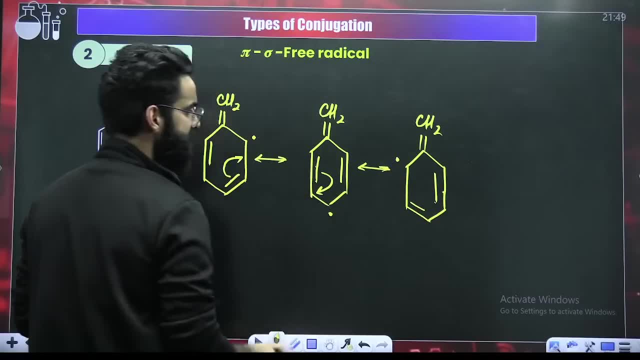 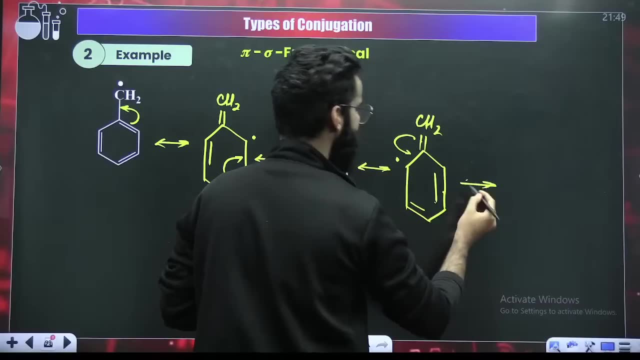 everything is similar. only right now this particular carbon gets the radical because the bond has been shifted from this particular carbon. now have a look, this pi sigma radical, pi sigma radical. shift this bond here. when you shift the bond, it is going to be, at the end, ch2 radical. 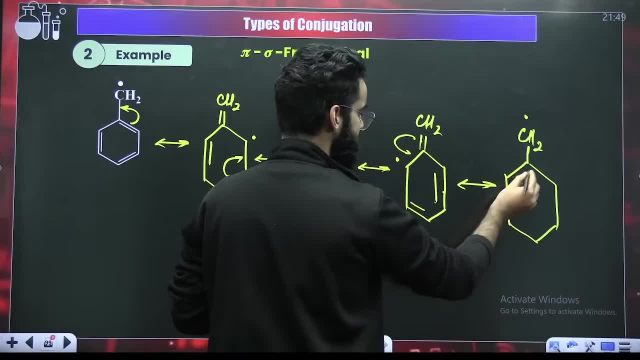 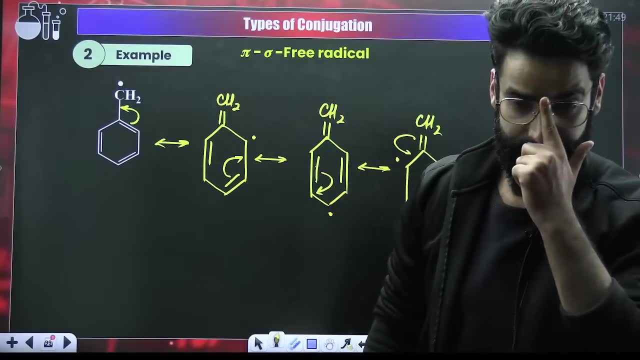 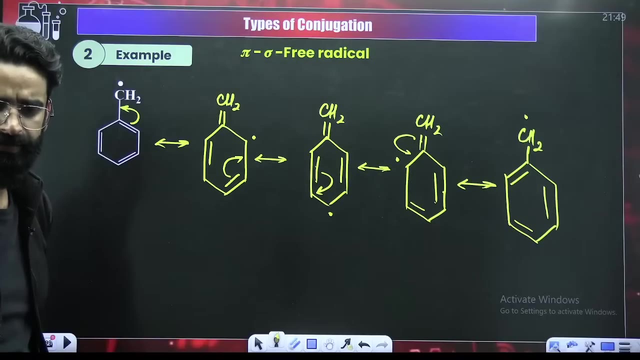 it is a single bond. rest all the things. this is like this. now tell me one thing, first and the last: these same or different resonating structures, first and last, same or different, same or different. quickly, first and last, same or different. first and last, same or different. 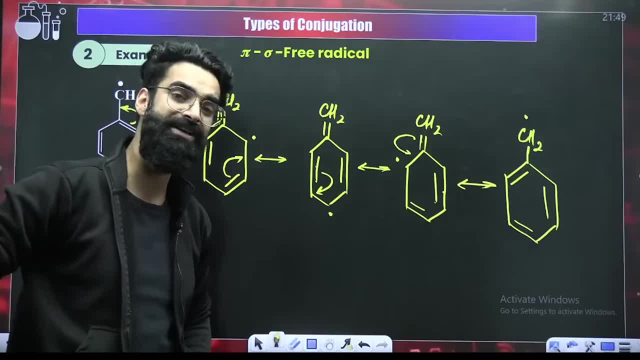 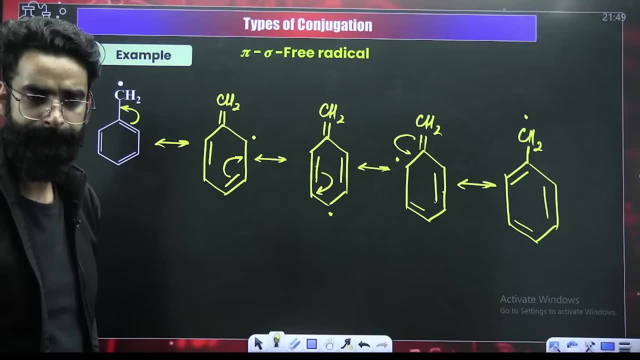 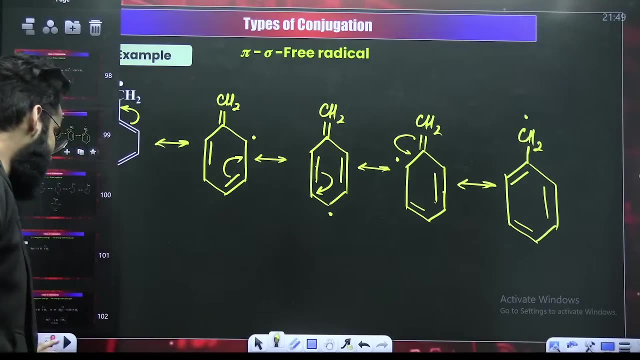 they are different resonating structures, but their stability and energy that is same. that's equal. yeah, so i hope this particular conjugation is also clear. now, guys, there is one more conjugation. what is that? first one was pi sigma- vacant, orbital. second one is pi sigma- free radical. third one is pi sigma. 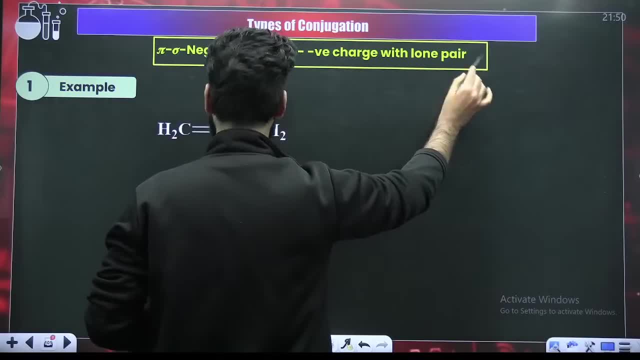 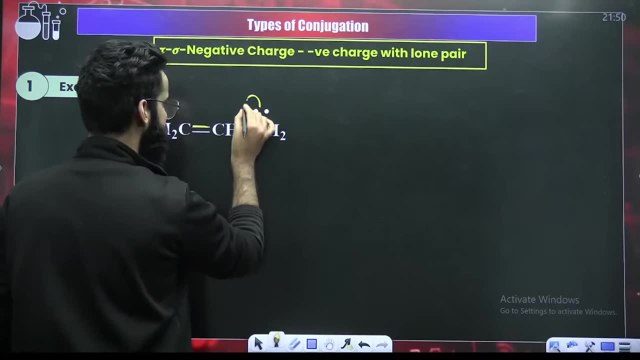 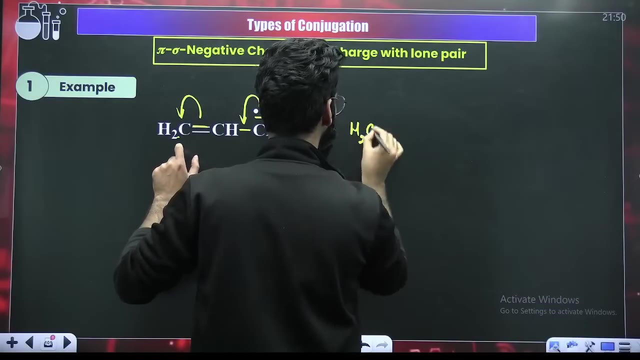 negative charge with unshared pair of electron. negative charge with unshared pair of electron. have a look, this is your pi, this is sigma. this is negative charge with unshared pair of electron. so shift it, just shift it. after shifting, what do we get? this will be your ch2 negative. 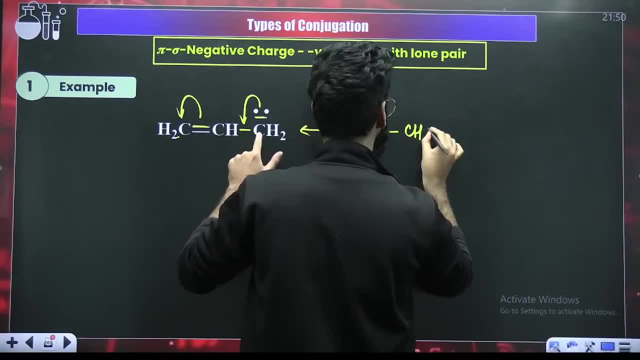 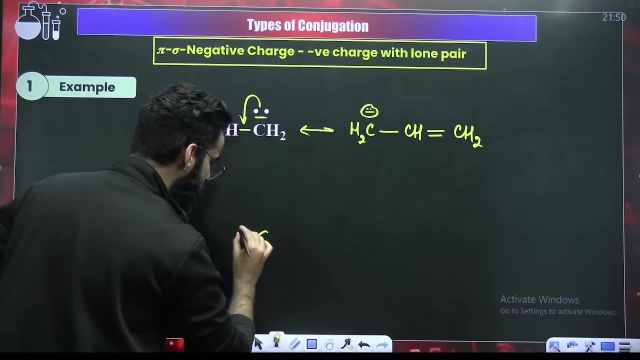 this is your ch2. there will be a single bond here. this is ch right, there'll be a double bond here, and this will be your ch2. perfect, simple. now make the hybrid. how will you make the hybrid? first, put a single one everywere. first, put a single one everywhere. 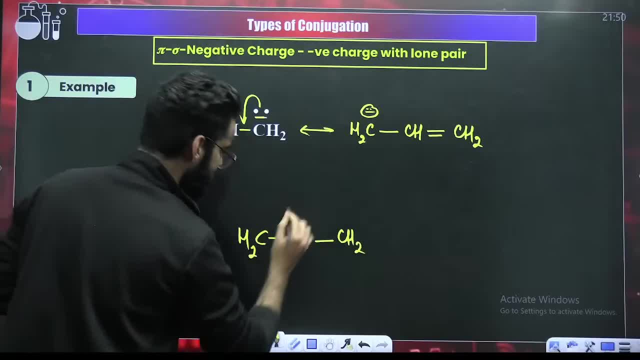 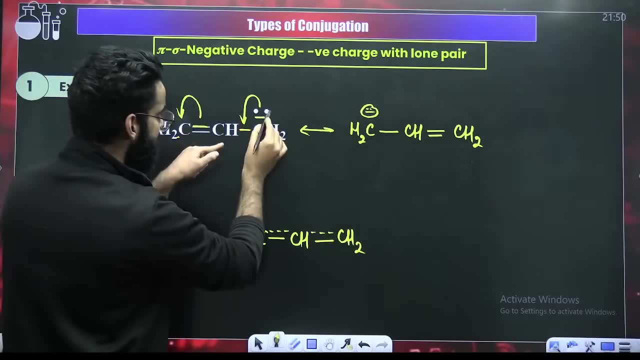 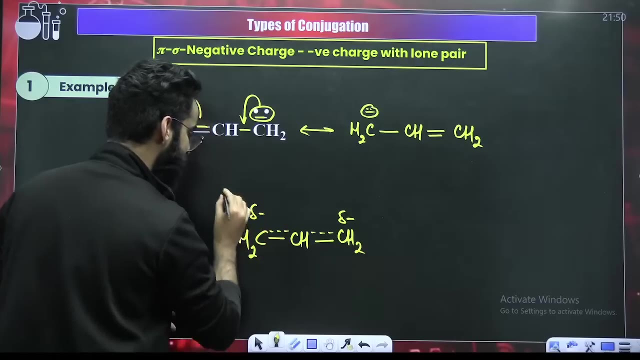 after putting the single one everywhere. now, this is double hair, this is single, so hybrid will contain partial double. single. this is double, hybrid will contain partial double. now, as for this particular structure, this one carries negri charge, right, so this is delta negative. As per this one, the other carbon carries a negative charge, so delta negative. 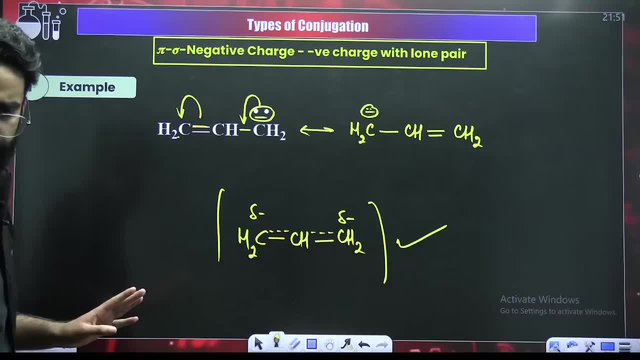 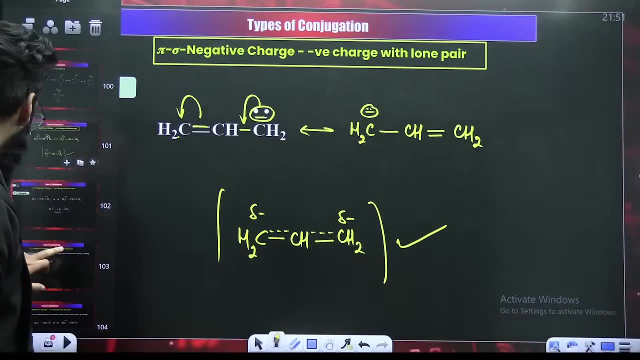 So this is your hybrid. This is your hybrid. I believe this is also clear. I believe this is also clear right Now. similarly, guys, there is one more conjugation. There is pi sigma lone pair conjugation. Okay, 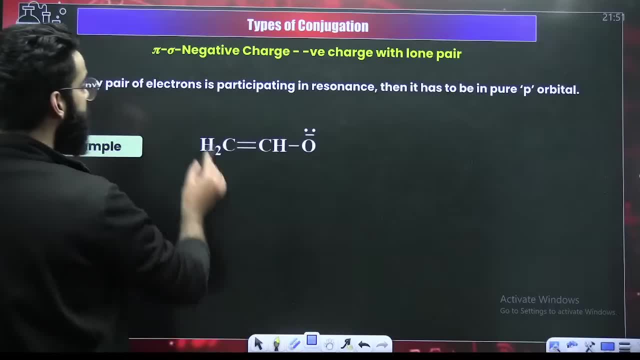 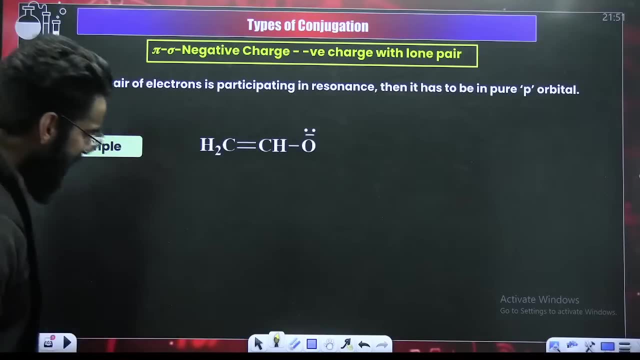 One more example we have here. One more example we have here Right. One more example we have here. Have a look guys. Look at this one. This is pi, This is sigma, This is negative Right With an unshared pair of electrons. 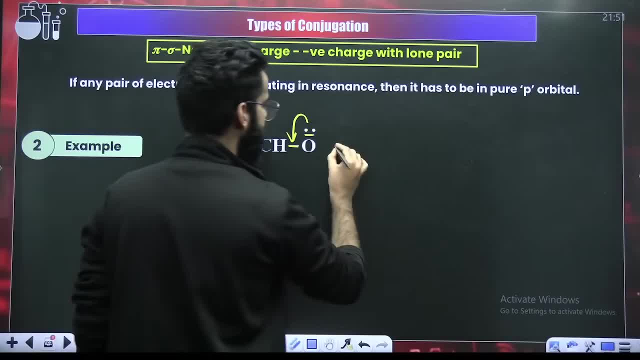 So again, conjugation, Shift it Right. When you shift it, what do we get at the end? This is CH2.. There is a single bond here, This is CH. There is a double bond here And this is O. 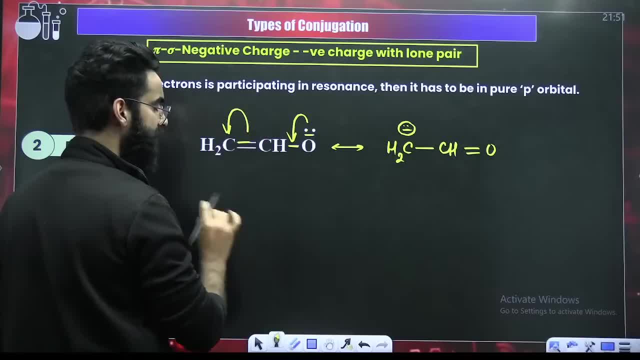 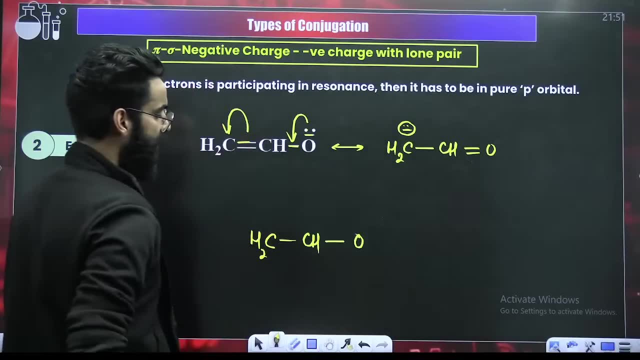 Now, this will carry the negative because this bond has been shifted. Now, if I ask you, what is the hybrid? how the hybrid looks like, this is CH2.. Single bond: CH Right, This is O Perfect. Now, as per this particular structure, there is a double bond. 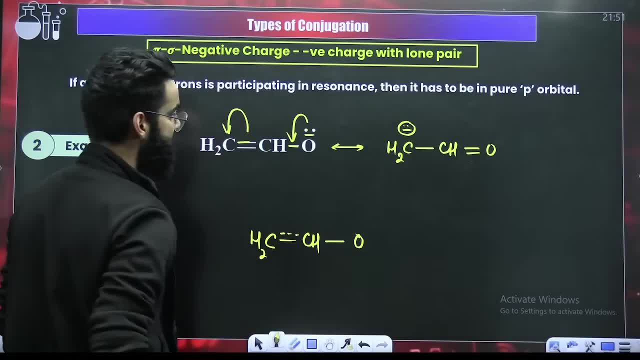 As per this structure, there is a single bond, So in the hybrid it will be partial double. In the hybrid it will be partial double Right. This is going to be delta negative And this is also going to be delta negative. 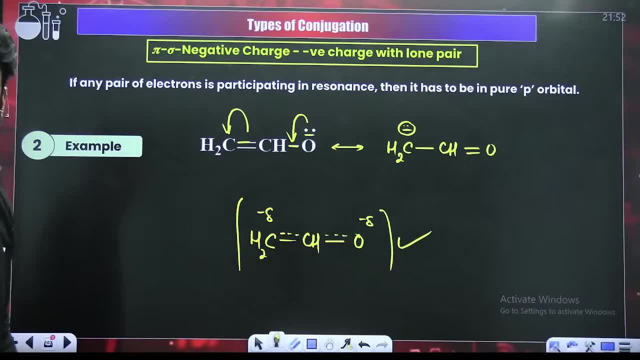 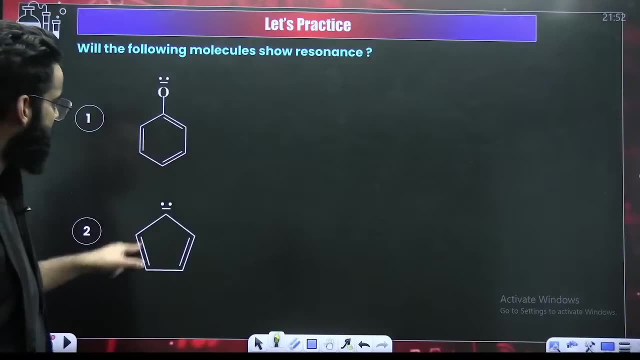 So this is your hybrid overhead. Yes, I hope you can easily do all these sort of things. Right, I hope you can easily do all these sort of things. Okay, Can you make the resonating structures of these two? You should be in a position to make the resonating structures of these two. 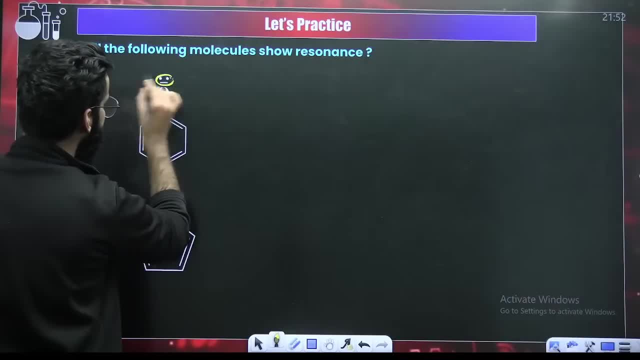 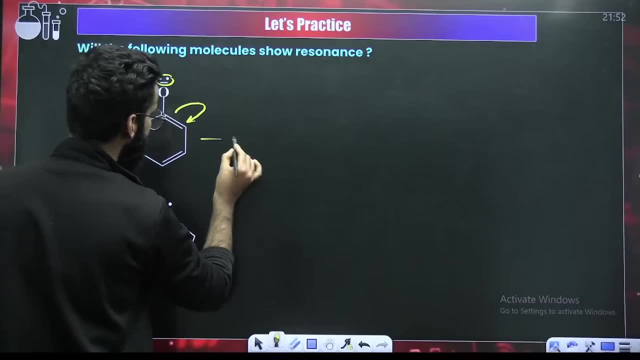 Have a look. This is pi sigma negative charge with an unshared pair. Right Pi sigma negative charge with unshared pair. What will happen? Shift this negative charge here, Shift this pi bond here. So what do we get? This is O. 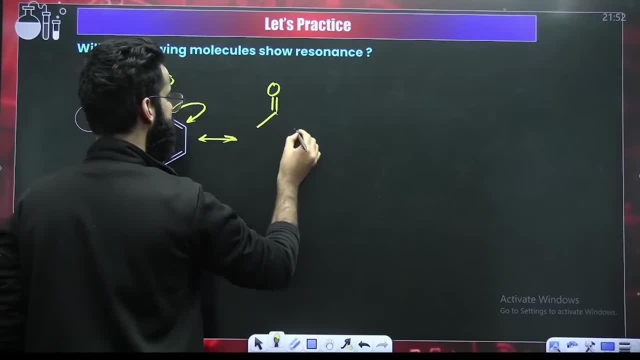 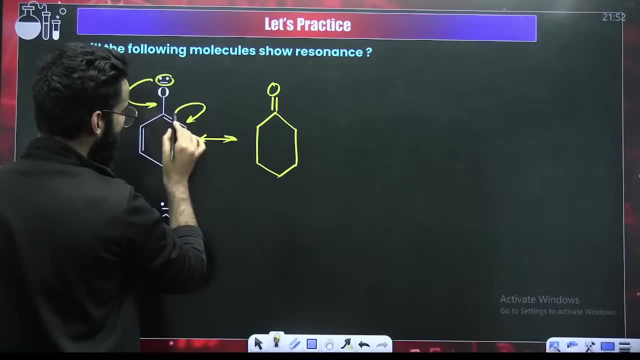 So what do we get? This is O. Now there is a double bond here. Perfect. Now see what all shifting would have happened Now, since this is a double bond, Right, This pi bond has shifted in this direction. 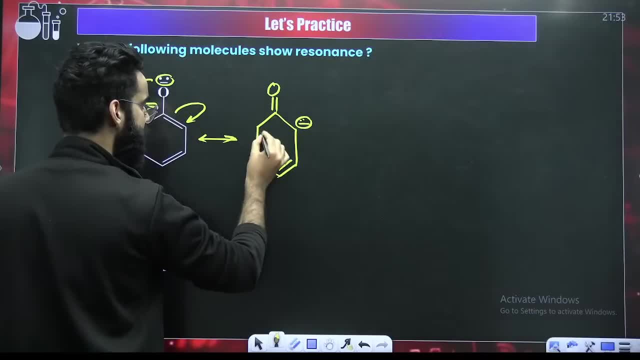 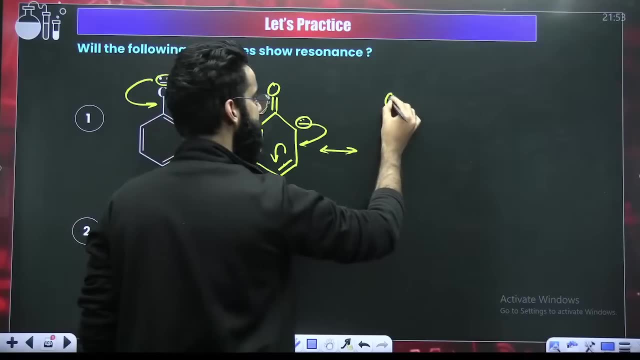 So now this carries the negative charge. Rest everything, keep it as such. Now, this is pi sigma negative, So shift it here, Shift this one here. What do I get? This is oxygen, This is double bond And all the things. 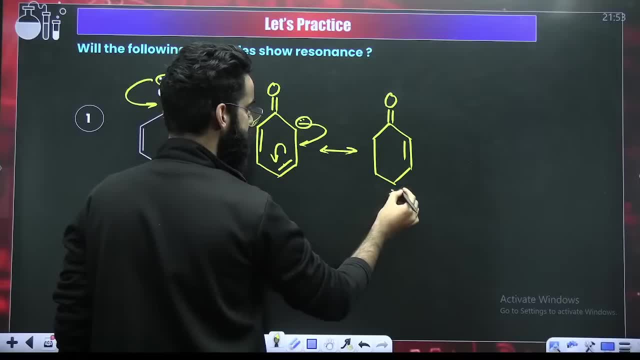 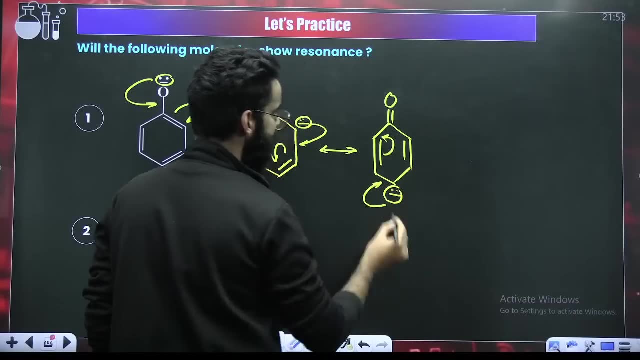 All the things Rest. This is double. This is negative. Perfect In this particular direction. Now again, this is pi sigma negative. Shift this in this direction, Shift it in this direction. What do I get? I get oxygen. 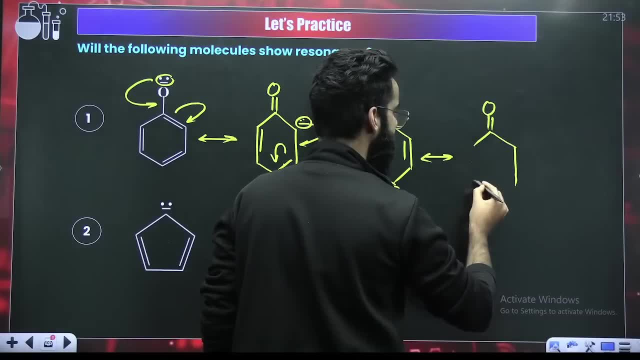 This is O, This is double bond. Right, And see all the things. This is now negative, Right, There is a double bond here. There is double bond here. Perfect. Now again this pi sigma negative, Shift it and shift it. 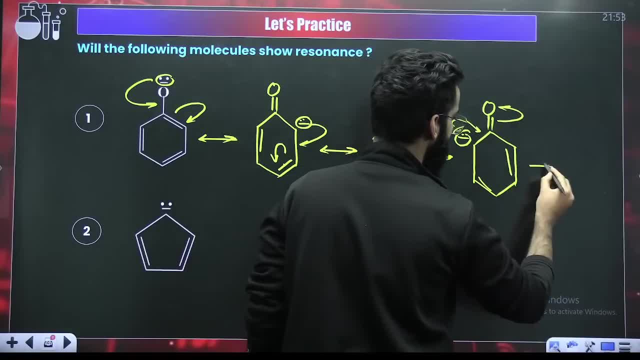 So what do I get at the end? I got something like this: Perfect. So these are all the resonating structures which we have here. Now people tell me, first and last, are these the more different? They are different, But which one is the most different? 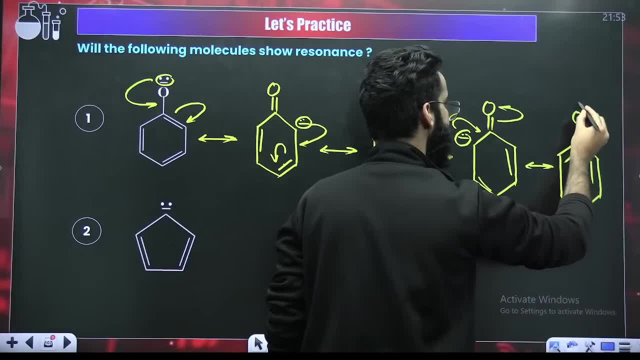 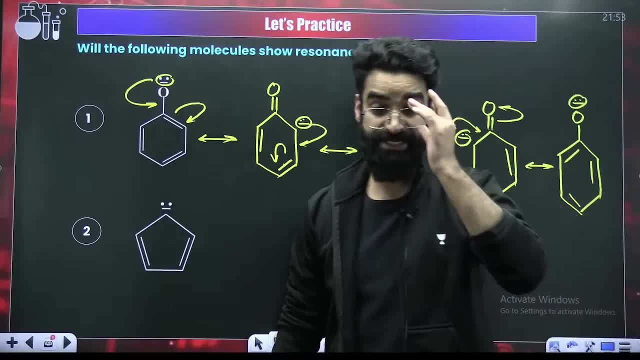 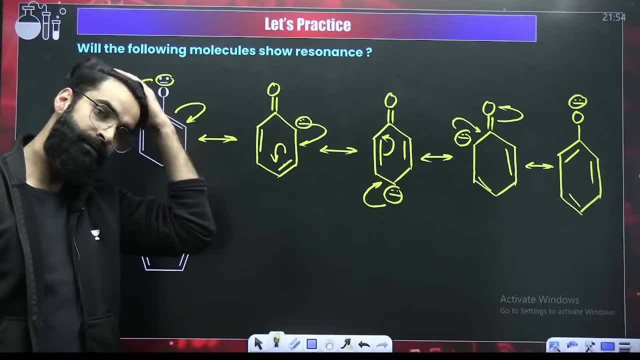 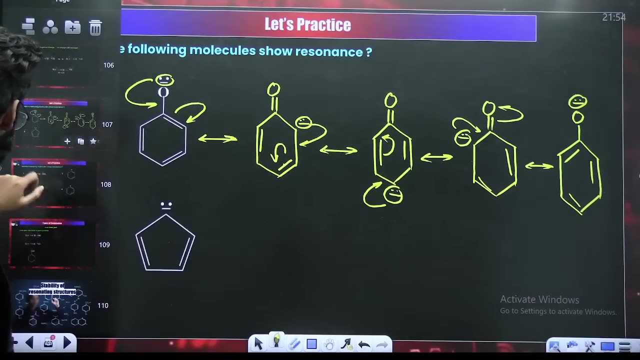 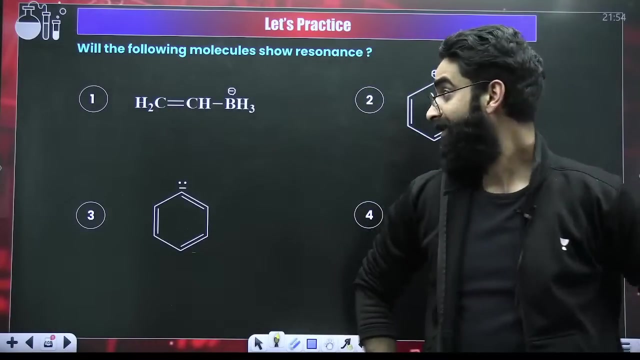 This is a two. are they more different? they are different, but their energy stability both is same. yeah, perfect. now i think this one you can easily do on your own. this one you can easily do on your own. now here is a duck for you. this is your chuck meat. will the following molecules show resonance or not? 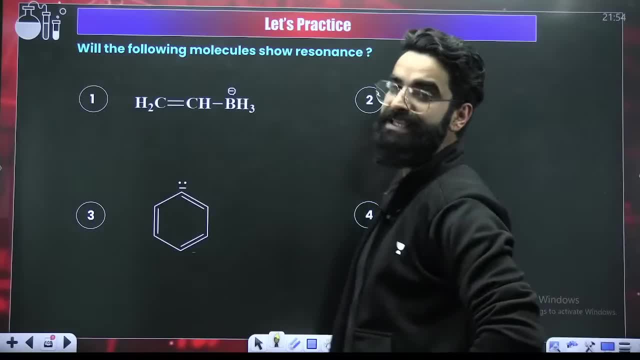 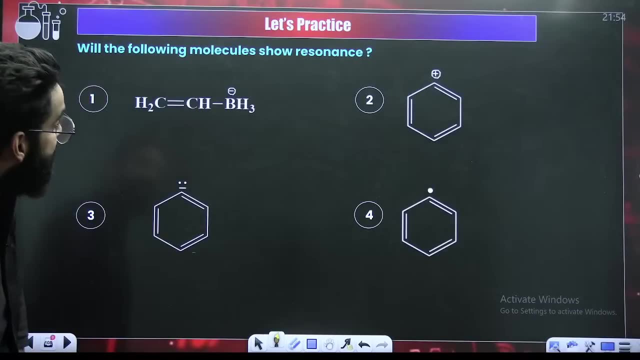 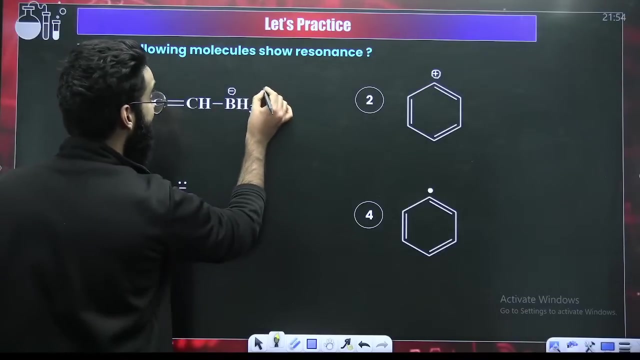 i've got four molecules here. among these four molecules, which one will show resonance, which one will show resonance among these four? among these four, which one will show resonance? among these four will first one show resonance? this is part of the process, pi sigma negative, but it has to. 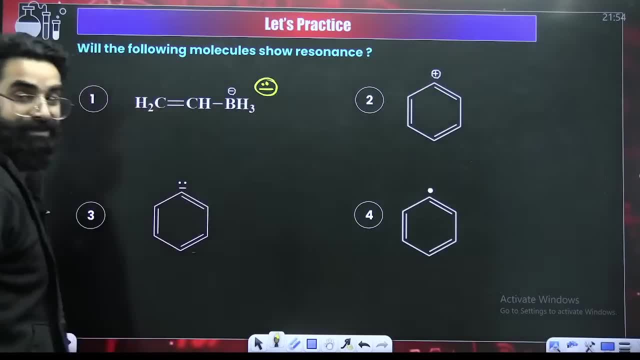 be pi sigma negative with unshared pair. this has to be the actual scenario. i'm just mentioning pi sigma negative, but it has to be pi sigma negative with unshared, negative with unshared. so is this going to show resonance? no way, tune in music, music. look at the second option. look at the 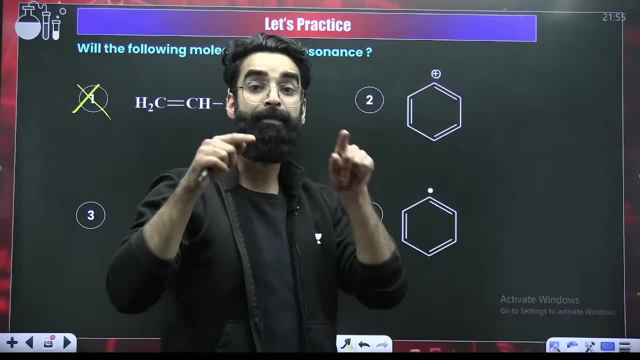 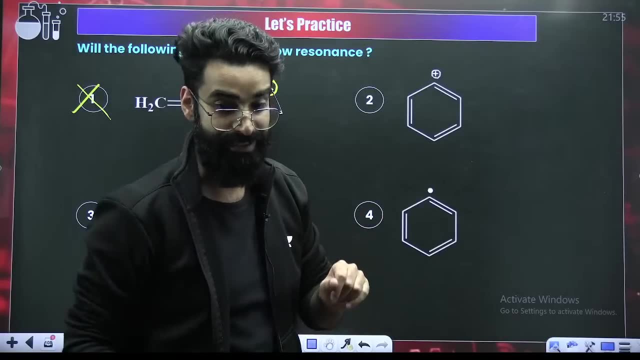 second option: tell me one thing: what is the resouance? the partial overlap of p orbitals, right, the partial overlap of orbitals which can be p or d, correct. now, guys, try to understand. try to understand if you look at this particular carbon, if you look at this. 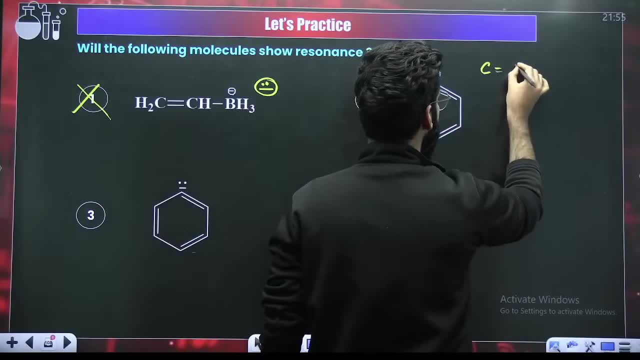 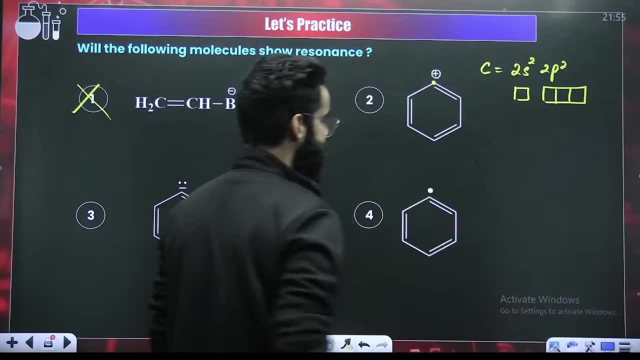 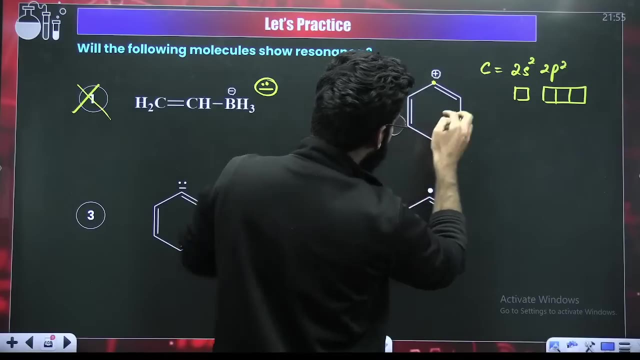 particular carbon. what is the? if you talk about carbon, it is 2s2, 2p2, right, so this is s and these are 3p orbitals of carbon. okay, first of all. first of all, there's a pi bond here. if there's a pi bond, 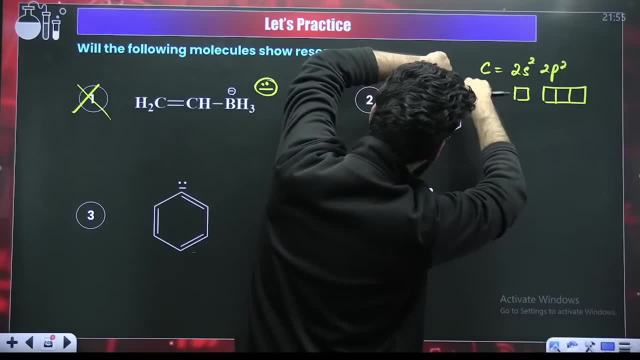 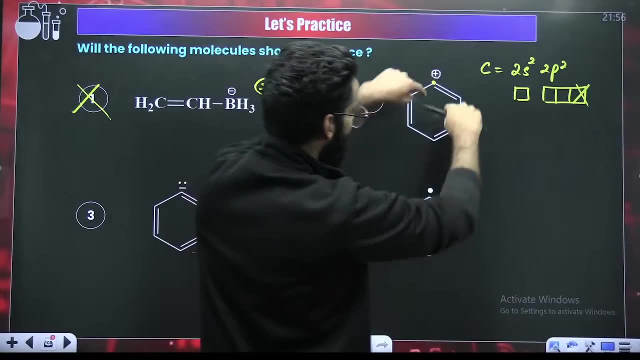 that means p orbital of this and p orbital of this. they have fairly overlapped, so one of the p orbital is consumed. it is consumed right, one of the p. i mean this p orbital and this p orbital. they are partially overlapped right, so this p orbital is gone. now how many orbitals are left? 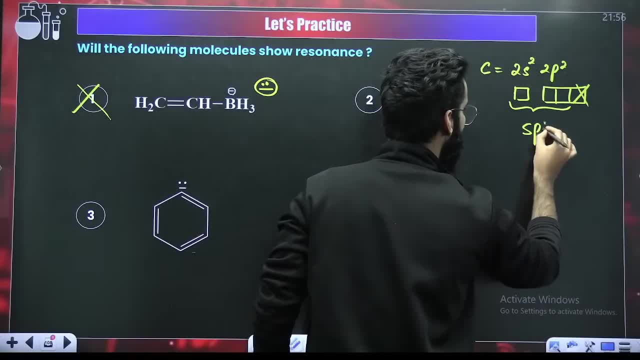 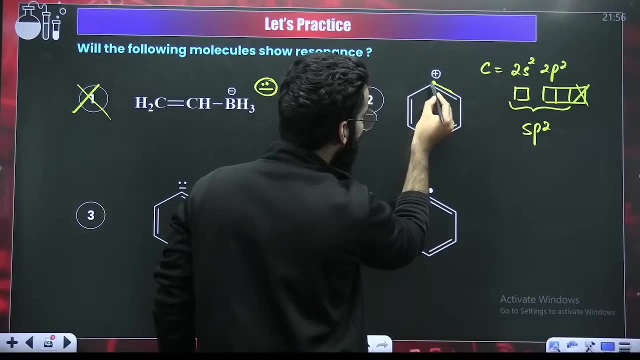 s and 2p, so this will undergo sp2 hybridization. sp2 hybridization means: how many hybrid orbitals? three hybrid orbitals? one of the hybrid orbital would have formed this sigma bond, one of the hybrid orbital would have formed this sigma bond, and one hybrid orbital will be carrying this positive charge. 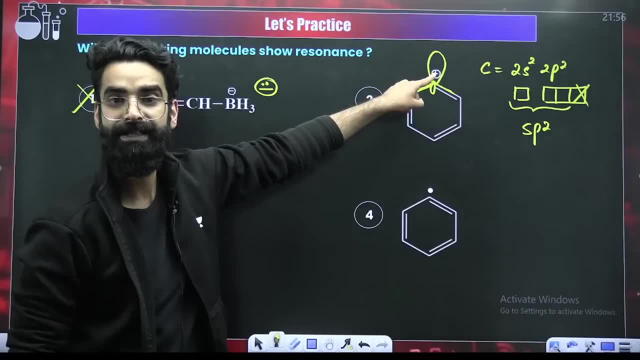 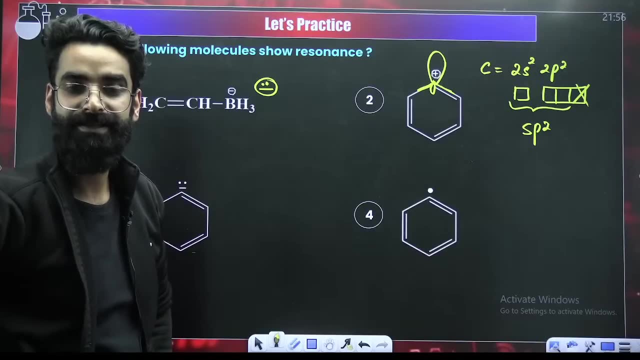 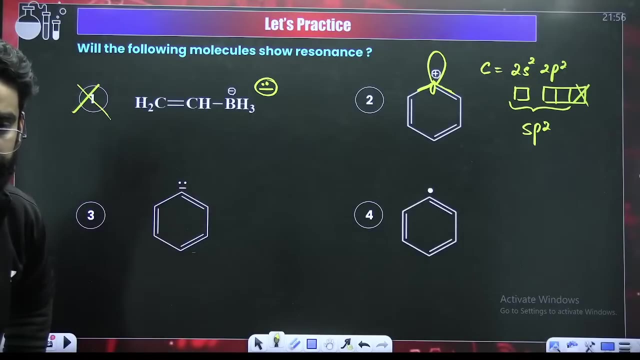 one hybrid orbital will be carrying this positive charge right now for resonance, for resonance, for resonance. now you tell me: will this molecule show resonance or not? will it show resonance? what is the resonance? will it show resonance, yes or no? quickly, quickly, so that positive charge is basically present in what sp2 orbital? 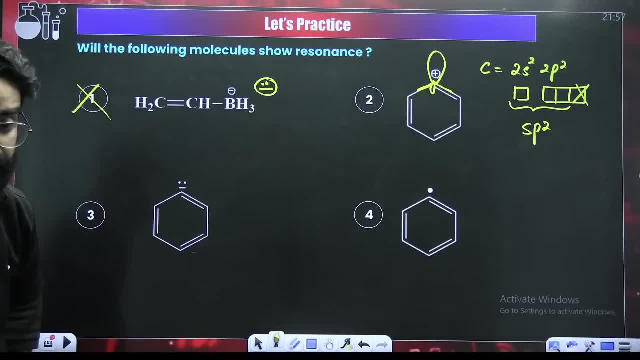 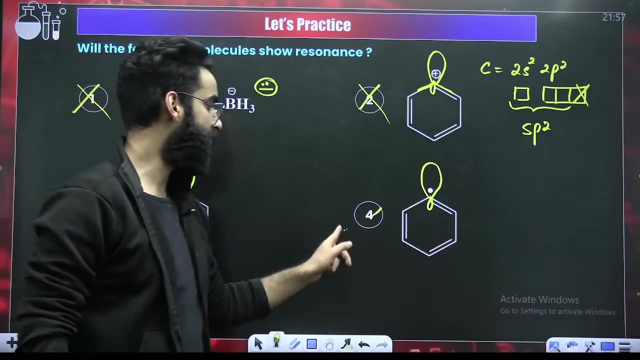 it should have been in s, it should have been pure p, orbital right. so it is not going to show resonance. look at this one again here. it is present in sp2. this radical is also present in sp2, so none of the molecule will show resonance among these four. 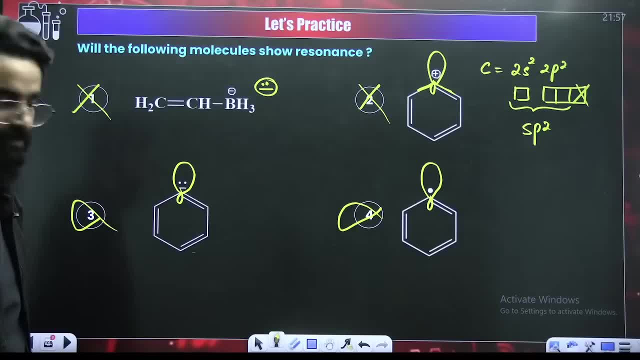 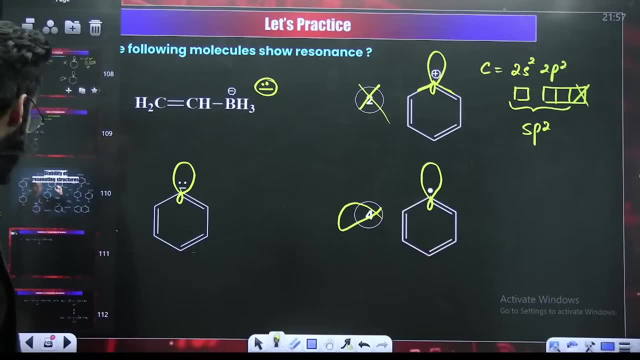 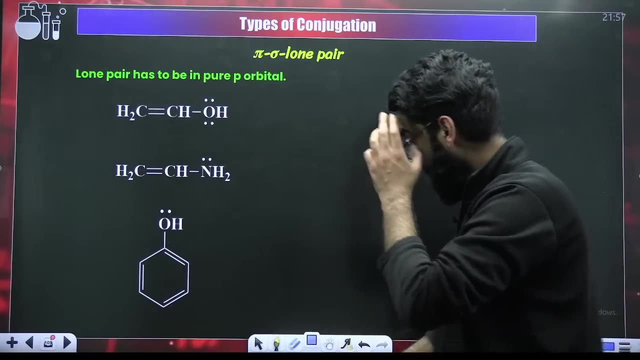 none of the molecule will show resonance among these four. none of the molecule will show resonance among these four. okay, none of the molecules will show resonance among these four. these are some typical cases, guys, which i'm showing you. okay, this is one important statement. lone pair has to be present in the pure p orbital when you talk. 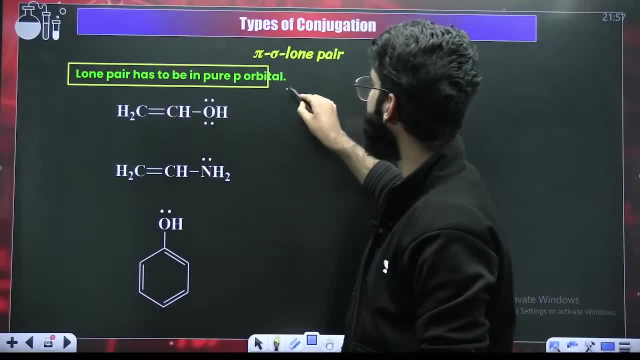 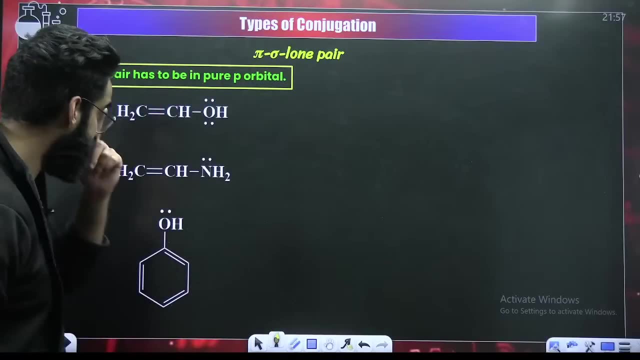 about pi- sigma lone pair conjugation. when you talk about pi- sigma lone pair conjugation, the lone pair has to be present in pure p orbital. there is one important thing which i'm going to tell you now. first of all, have a look. have a look, guys. this is pi, this is sigma, this is a lone pair. 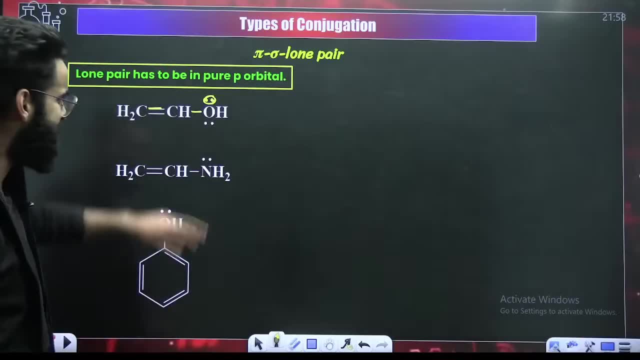 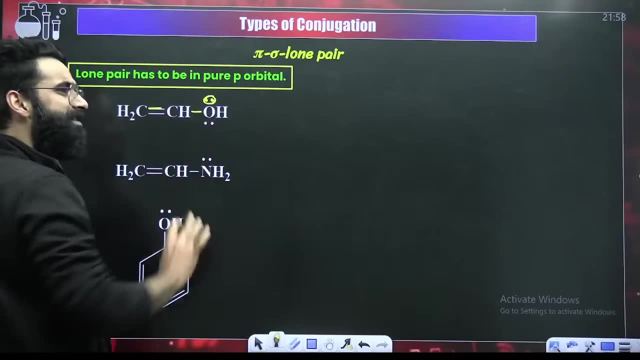 is this lone pair over here conjugated? yes, this conjugate. so basically, oxygen has two lone pairs. oxygen has two lone pairs. out of the two lone pairs, one lone pair will participate in the resonance. that lone pair, which is participated in the resonance, that is not con. 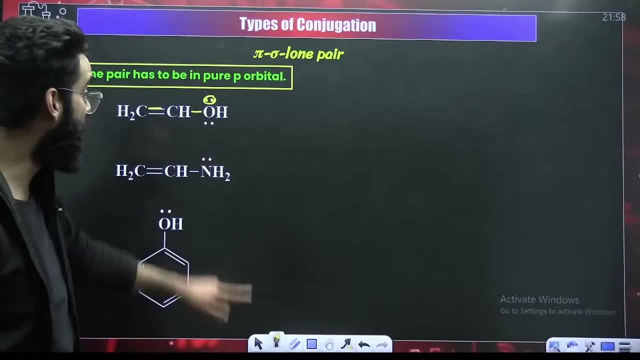 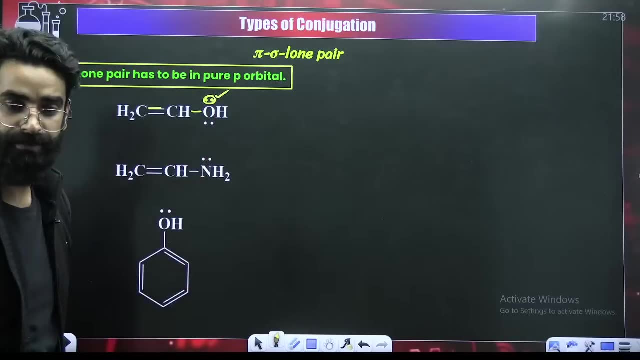 going to be considered and what that is, what that is not considered while calculating the hybridization, that lone pair which participates in the resonance, that is not considered for hybridization. so one of the lone pair you don't have to consider for hybridization. now if i ask you, what is the 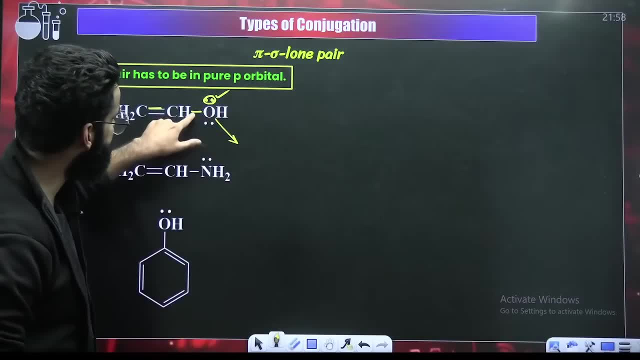 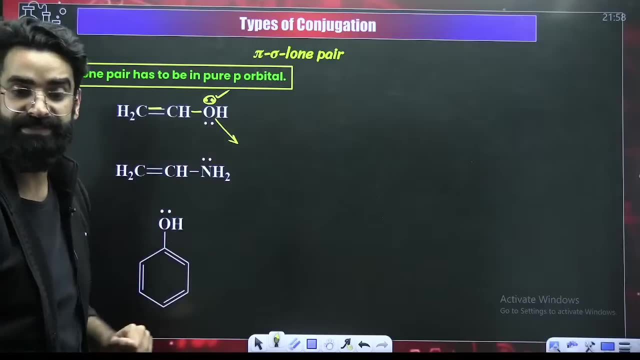 hybridization of this oxygen. quickly see it's forming one sigma, two sigma. so two sigma and one loan period. you have to consider, you don't have to consider two, you have to consider one. so two sigma, one lone pair. steric number three: if steric number is three, so it is sp2. 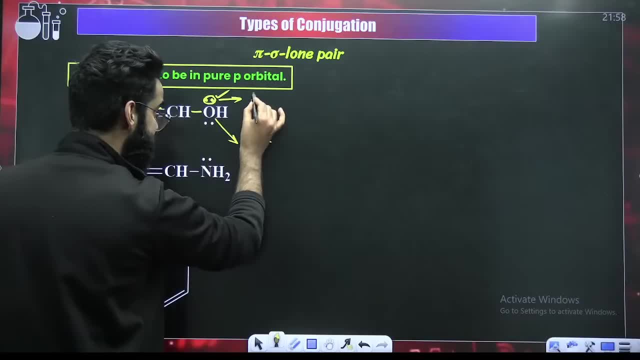 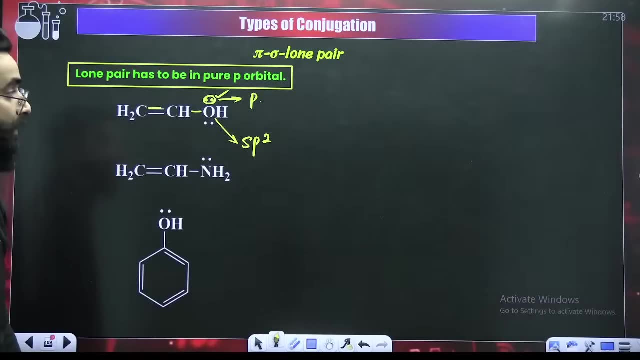 it is sp2. it is sp2. that means this: of this lone pair, it is present in pure p orbital. that's what i mentioned over here. lone pair has to be present in the pure p orbital. lone pair has to be present in the pure p orbital. perfect right. so make its resonating structures. 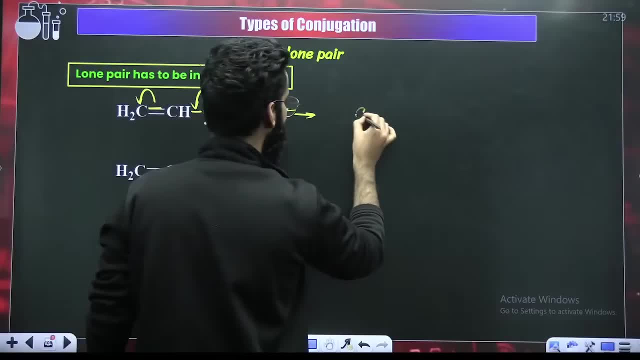 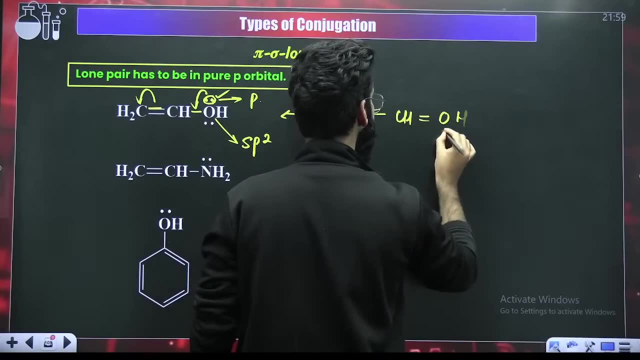 so shift this load pair in this direction, shift this bond in this direction. what do you get? you get ch2 negative. you get ch2 negative. there is a single bond, this is ch. this double bond, this is, oh, carrying only one lone pair and there'll be a positive charge here, perfect. so this is its one more. 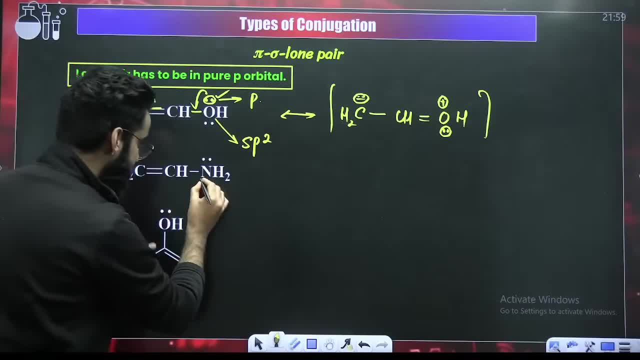 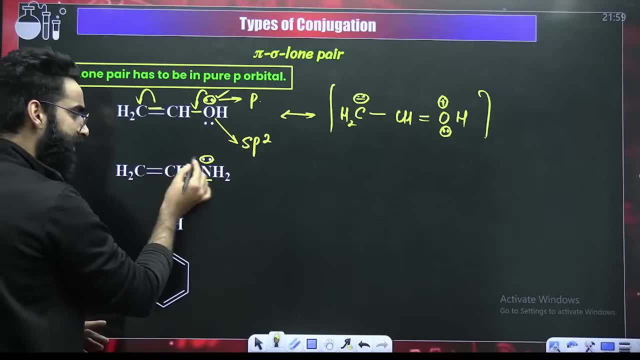 canonical form. look at this particular nitrogen. this nitrogen, it's forming three sigma bonds. it's forming three sigma bonds and this lone pair is conjugated. this is pi sigma lone pair. it is conjugated, perfect. now, this nitrogen, if i ask you, it's hybrid region, it's sp2. 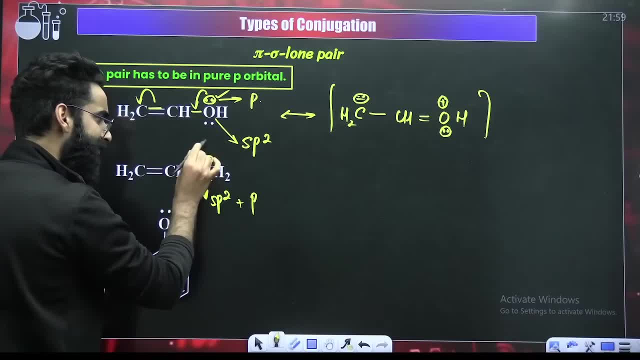 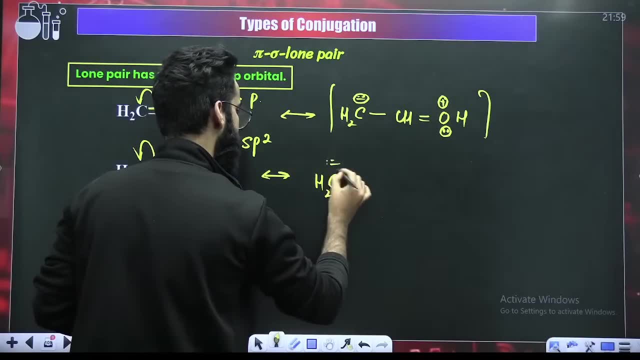 if it is sp2, there will be a p orbital and that p orbital will be carrying this lone pair right. so shift it. when you shift it, it's going to be ch2 negative, stage two negative. there is a single bond. this is ch. there's a double bond. 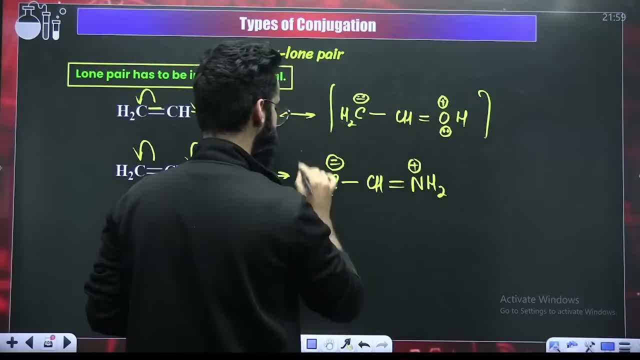 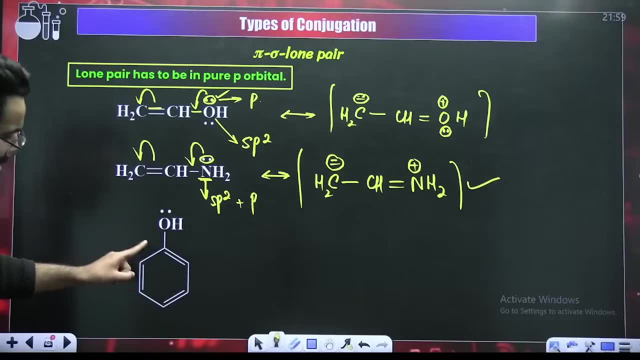 this is going to be your nh2 positive here. perfect, so this is going to be its canonical form. similarly, can you make the canonical forms for this one? can you make canonical forms for this one? this is: pi sigma lone pair, pi sigma lone pair. this oxygen, it has got two lone pairs. basically, it has got two lone. 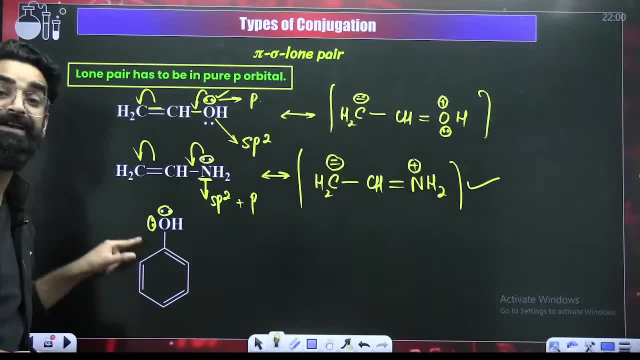 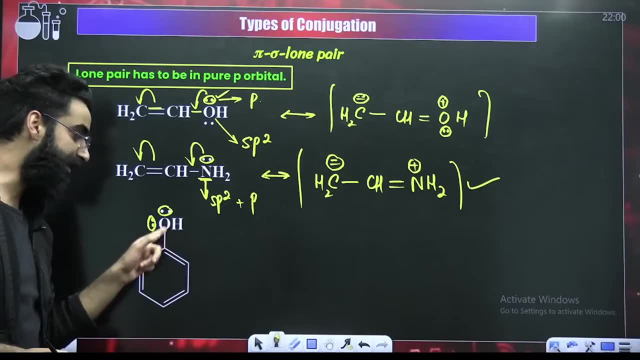 pairs, basically. but out of the two lone pairs, one lone pair will participate in resonance, so you do not have to count that lone pair for hybridization. now tell me the hybridization of this oxygen. it's forming two sigma and one lone pair. two sigma, one lone pair, that means steric number three, so it's sp2. 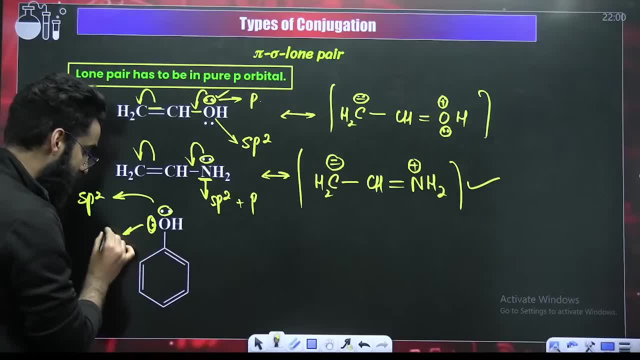 that means this particular lone pair. it is present in pure p orbital and that is the criteria. lone pair has to be present in the pure p orbital, correct? now you can do all the wonders right. shift it in this direction. shift it here. there'll be a negative charge when there. 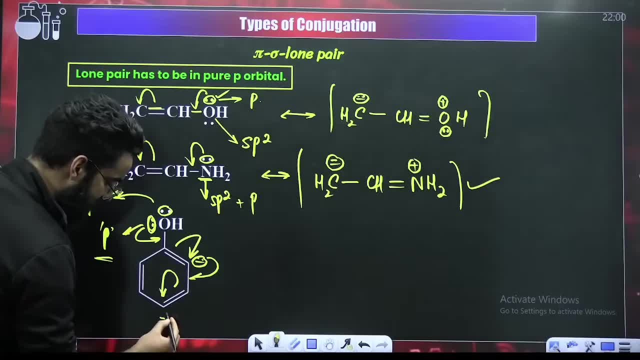 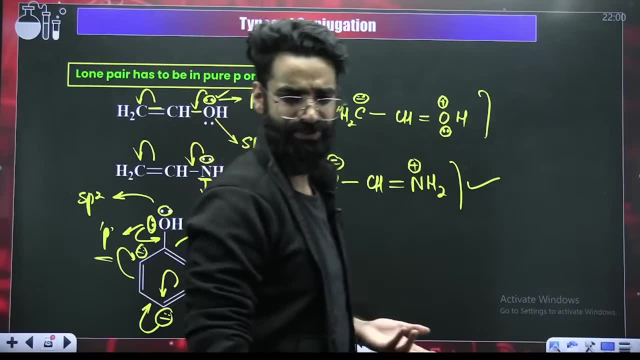 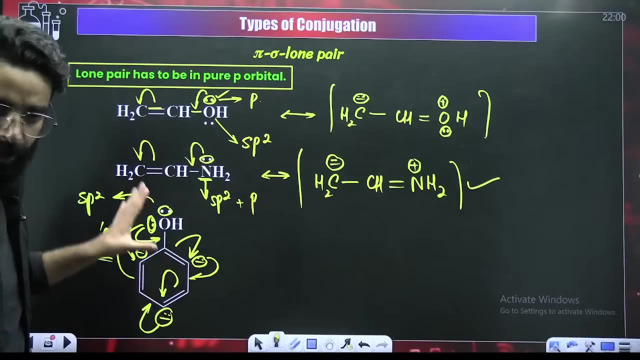 is a negative charge here. shift it in this direction. this will shift in this direction. there'll be negative charge. then shift this in this direction and shift it here. I mean, you can easily make these structures, you can easily make these resonating structures now, okay, is it clear? now, my dear students, once you are 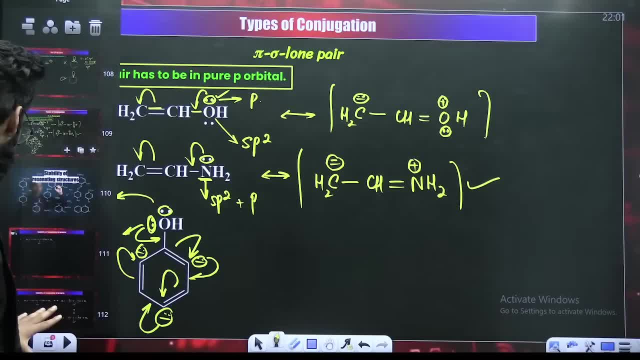 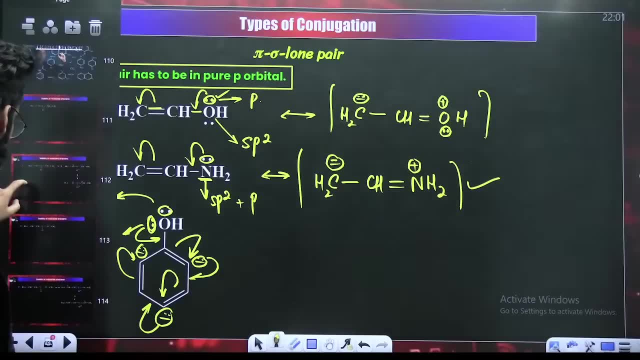 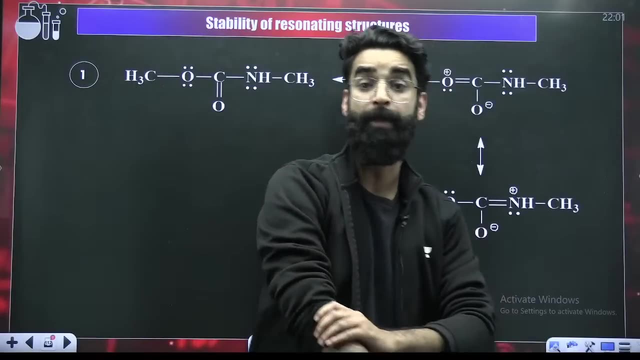 familiar with how to draw the resonating structures. how to draw the resonating structures. now it is the time to compare. it is the time to compare the stability of the resonating structures. it is the time to time to compare the stability of resonating structures. This is the question which is 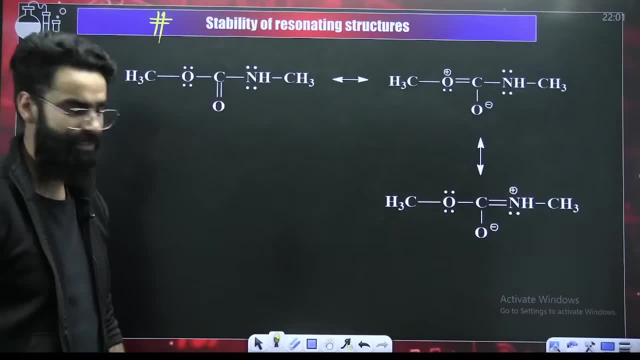 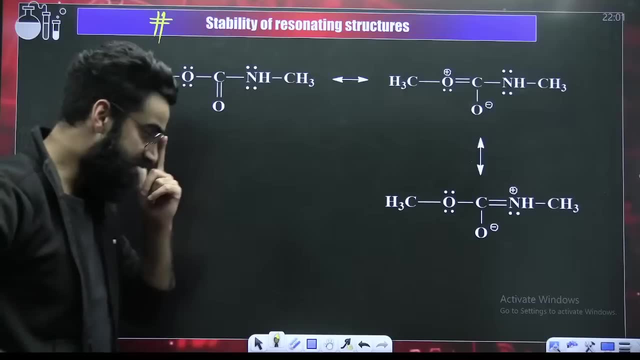 frequently asked: How do you check the stability of the resonating structures? These are the three resonating structures which are given to us. We need to compare their stabilities. My dear students, the first and the most important point. First and the most important point. 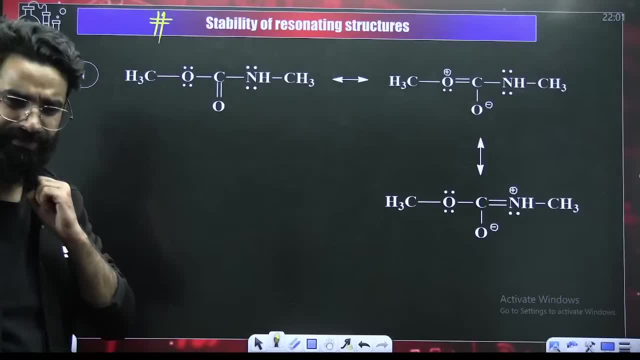 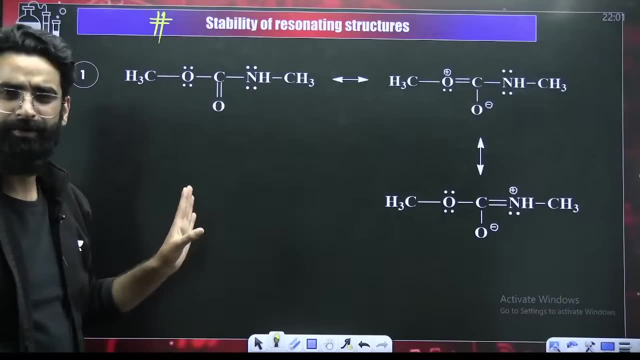 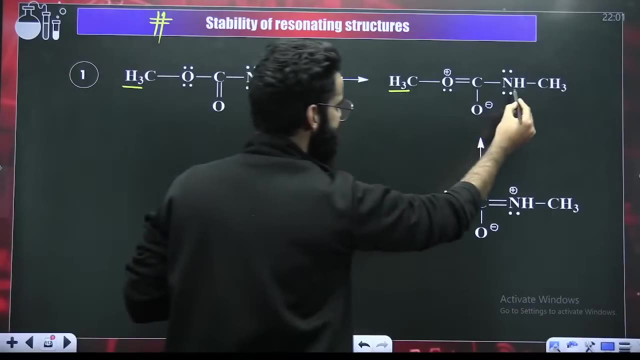 If you need to compare the stability of these resonating structures, what you should do, What you should do, first of all, Try to calculate the number of covalent bonds. See, first of all, this is CH3 here, CH3 here, CH3 here. right, This is NH, this is NH here. this is. 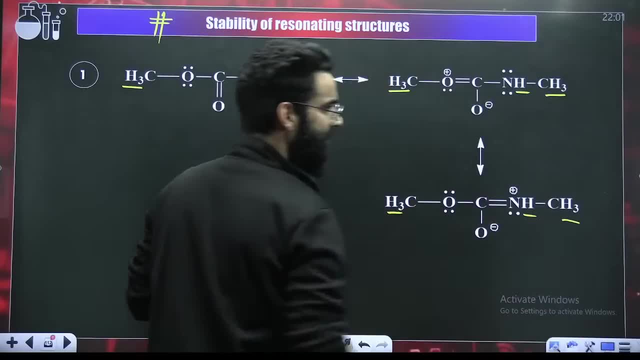 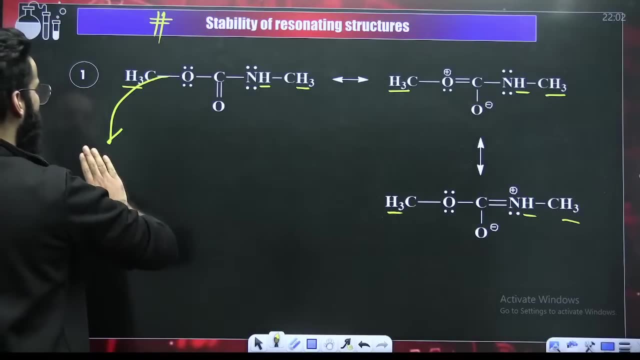 NH. here, This is CH3, here, this is CH3, this is CH3.. So all these things are same everywhere. All these things are same everywhere. So, what I will be doing, I won't be counting the exterior bonds, I will be counting the interior bonds, I will be counting the interior. 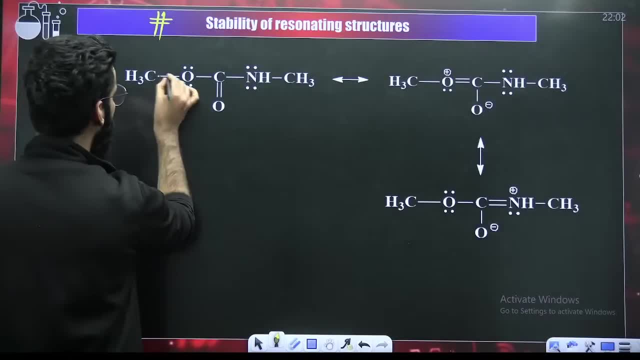 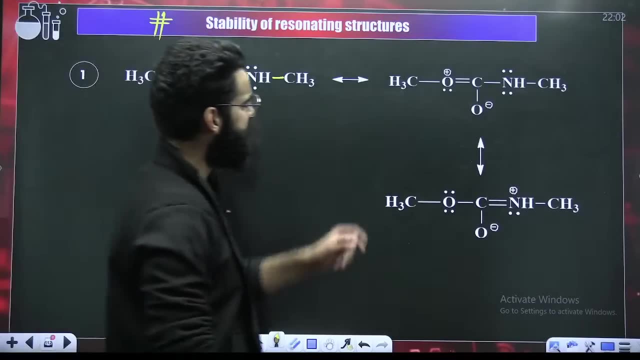 covalent bonds. Tell me how many interior covalent bonds do we have here? 1,, 2,, 3,, 4,, 5 and 6.. 6 interior covalent bonds. right, Look at this one: 1,, 2,, 3,, 4,, 5,, 6.. 6 interior covalent. 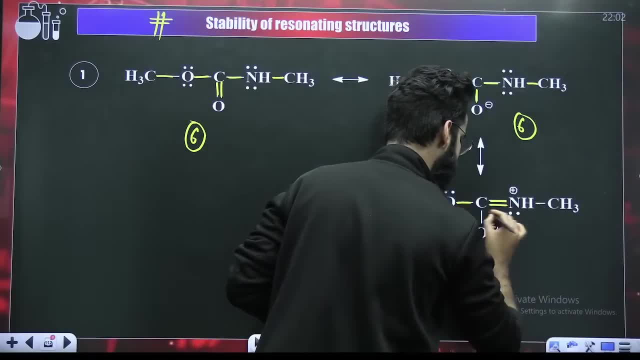 bonds here. Absolutely, How many here? 1,, 2,, 3,, 4,, 5,, 6. 6 interior covalent bonds here, My dear students, whenever you need to compare the stability of the resonating structures, 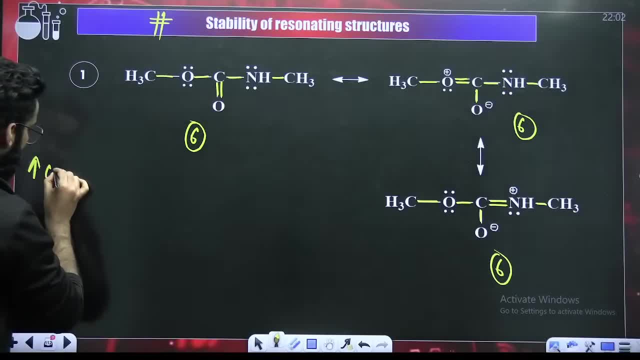 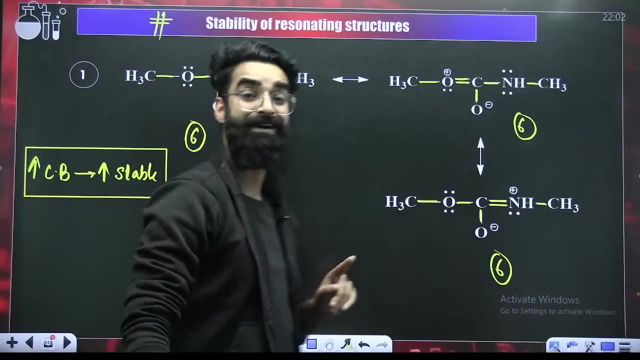 the first point is you have to count the covalent bonds, interior covalent bonds, That structure wherein covalent bonds are maximum, that will be maximum stable. This is the first point, which we will be checking all the time: Calculate the maximum, calculate. 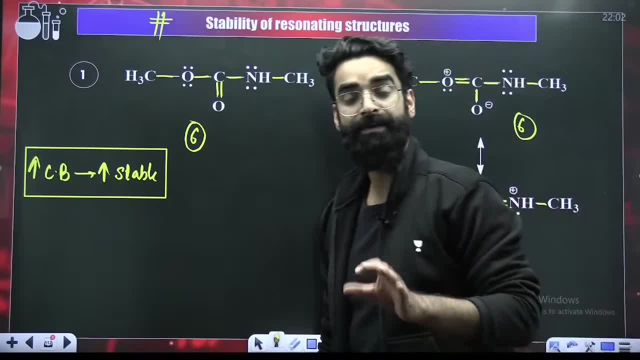 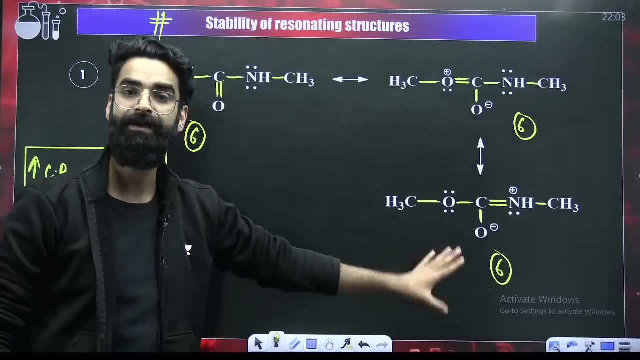 the interior covalent bonds. That resonating structure, that resonating structure, which will be containing maximum interior covalent bonds, will be maximum stable. But here, in these three, the interior covalent bonds are same. So you can not decide on. 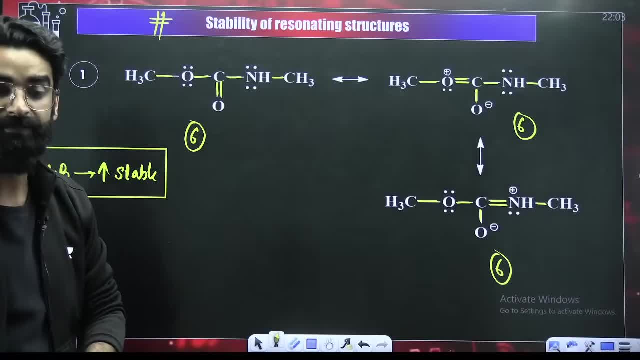 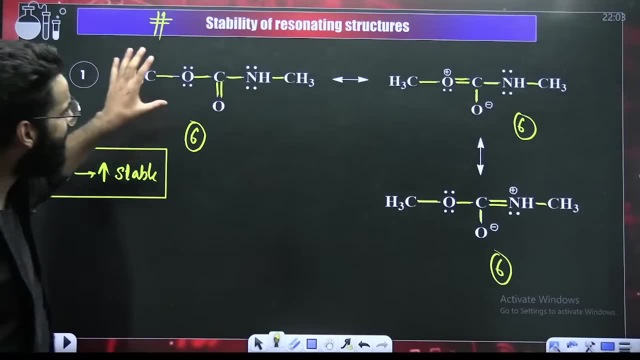 the base of interior covalent bonds. You can not decide on the base of interior covalent bonds, right, But your priority is always covalent bonds No 2,, no 2.. No 2. Look at that resonating structure. look at that. find that resonating structure in which. 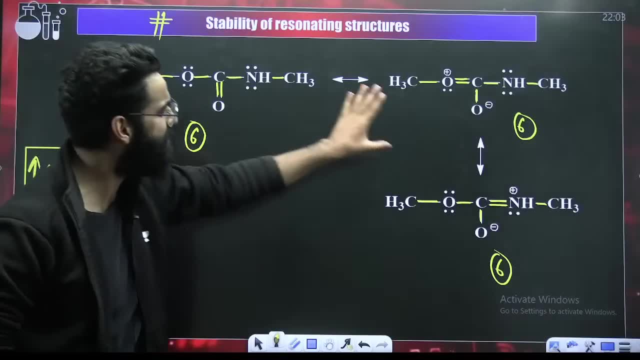 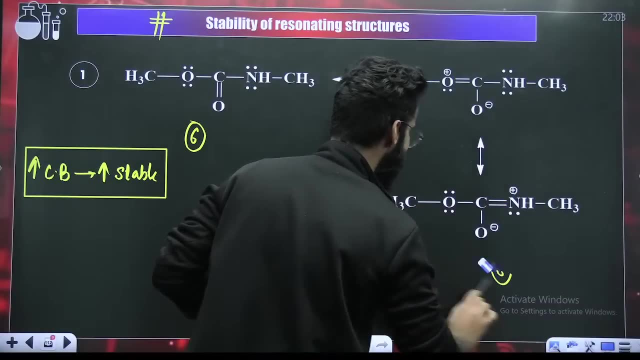 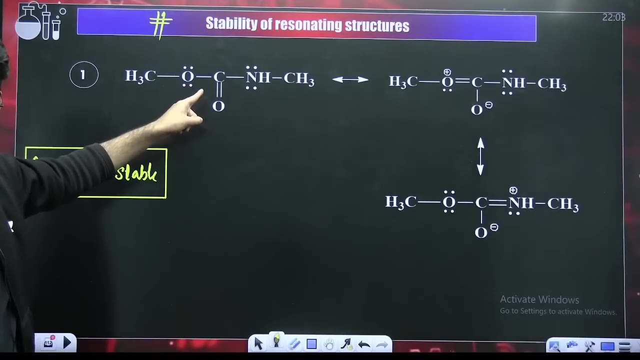 atoms do not contain any charge. Is there any resonating structure like that in which atoms do not contain any charge? Is there any resonating structure like that in which atoms do not contain any charge? I can directly say first one. right, I can say first one. 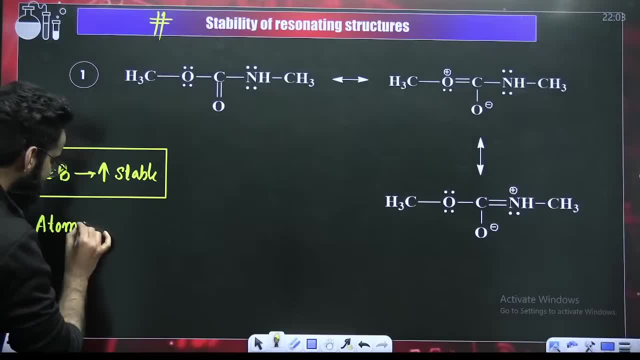 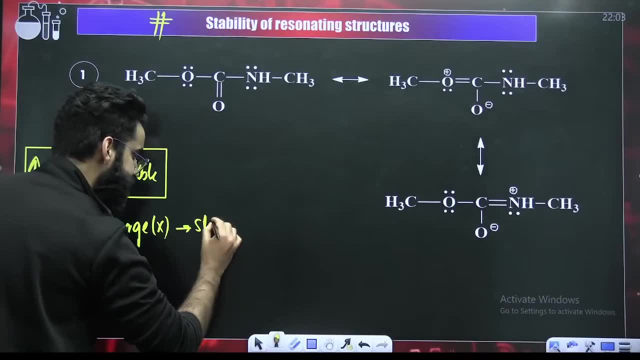 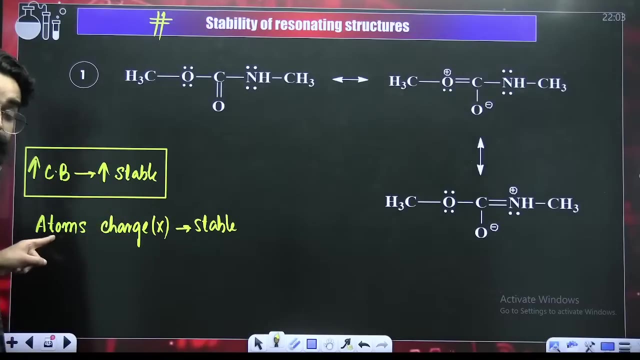 That resonating structure, that resonating structure in which atoms do not contain any charge. atoms do not contain any charge. that is going to be stable. that is going to be stable. First you are going to check what, First you are going to check number of bonds, then you are going to see that resonating. 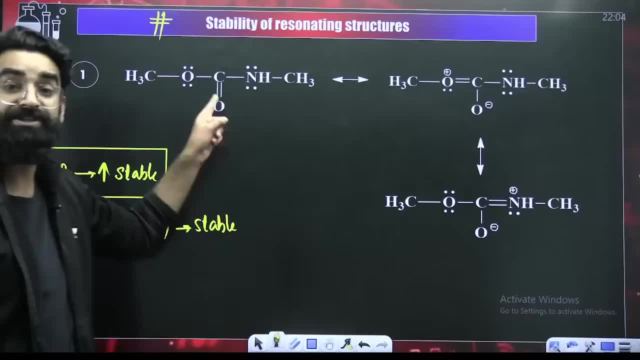 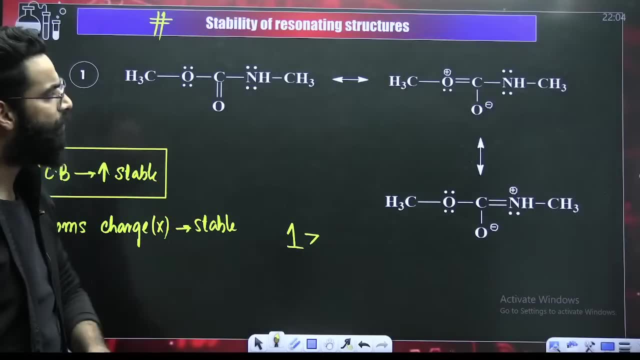 structure in which the atoms do not contain any charge. this is the structure in which atoms do not contain any charge. so first one is maximum stable. first one is maximum stable Now, among 2 and 3, among 2 and 3, have a look properly. 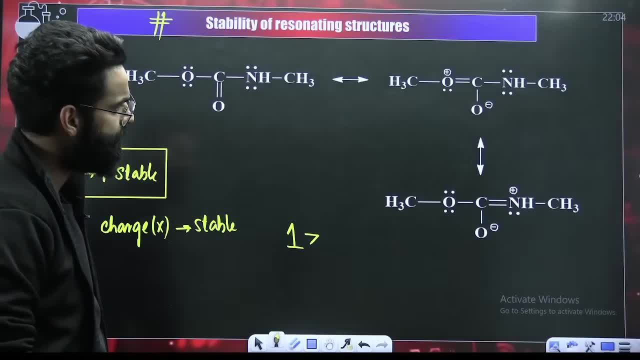 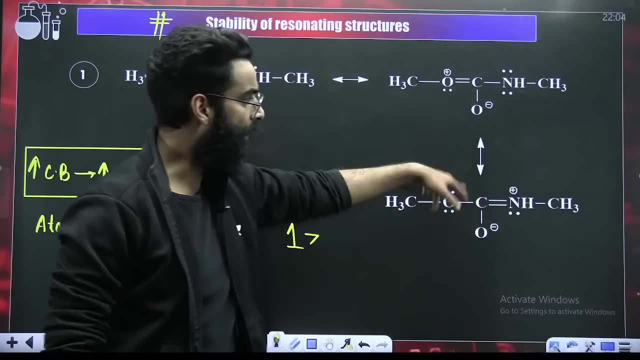 What exactly we are going to say. have a look, My dear students. what do you think? 1,, 2,, 3,, 4,, 5,, 6, ok, What do you think Among 2 and 3, which one? 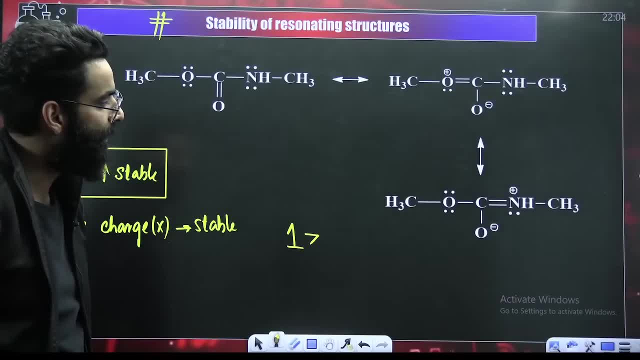 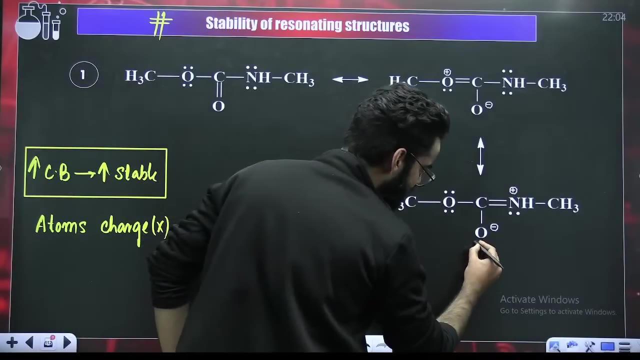 Among 2 and 3, which one, Quickly, Quickly, among 2 and 3, which one, which one is more stable? What do you think? What do you think, See, See, Look at these two structures carefully. 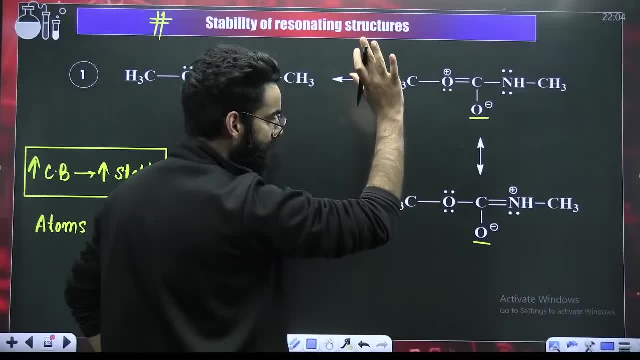 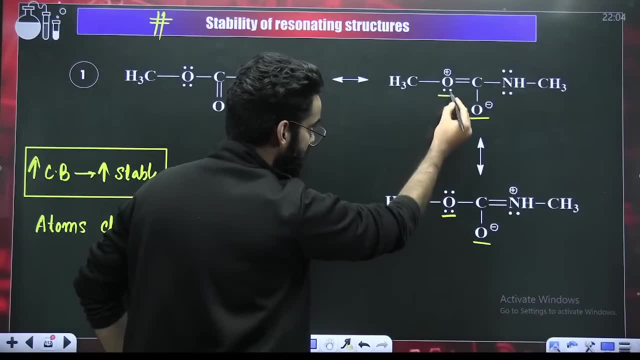 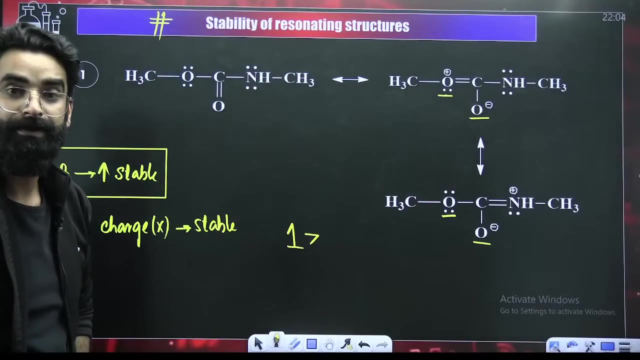 This oxygen carrying negative oxygen carrying negative. same right, same perfect. Look at this particular oxygen. look at this particular oxygen. oxygen is carrying positive here. oxygen is carrying positive. here, oxygen is carrying positive. positive charge on an electronegative element makes it highly unstable. right so, among 2 and 3, among 2. 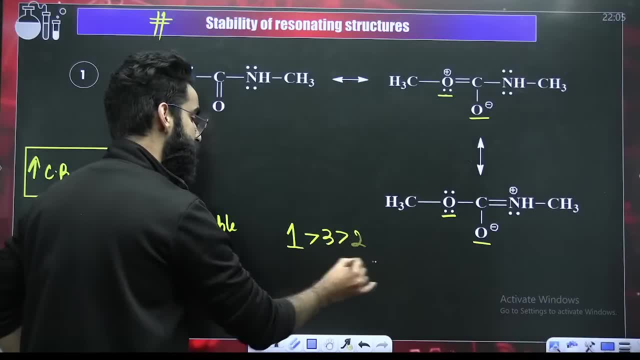 and 3, which one is more stable? I will say 3 is more stable, followed by 2.. So is this the order? Ok, This is going to be the order here. Right, This is going to be the order here. 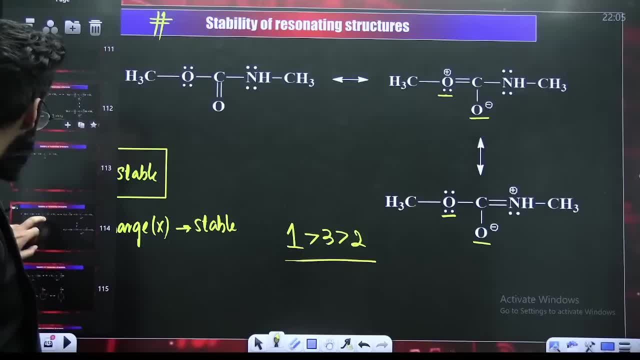 Let's have a look on one more question. Have a look on one more question. Check the order of the stability of these resonating structures. Check the order of the stability of these resonating structures. Have a look, guys. First of all, calculate the total number of internal covalent bonds. 1,, 2,, 3,, 4,, 5,, 6,, 7, 8.. 8 covalent bonds: 1,, 2,, 3,, 4,, 5,, 6, 7.. 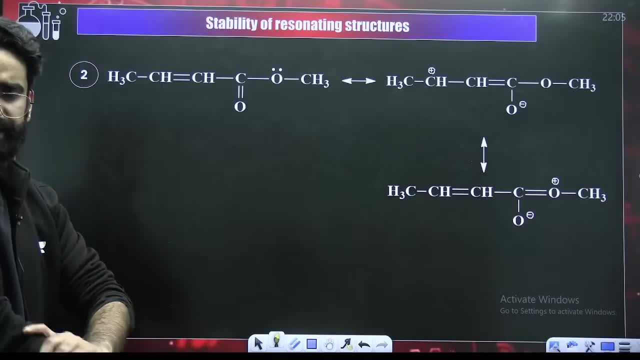 7 covalent bonds: 1,, 2,, 3,, 4,, 5,, 6, 7.. 7 covalent bonds: 1,, 2,, 3,, 4,, 5,, 6, 7.. 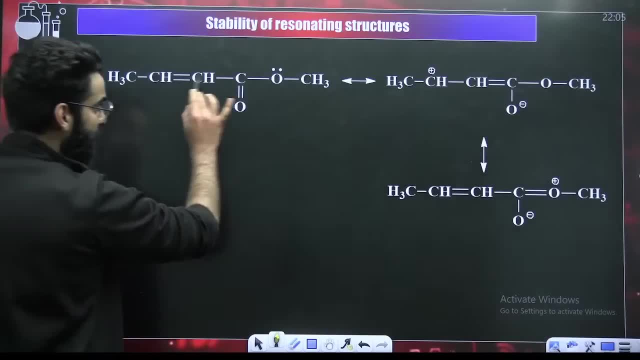 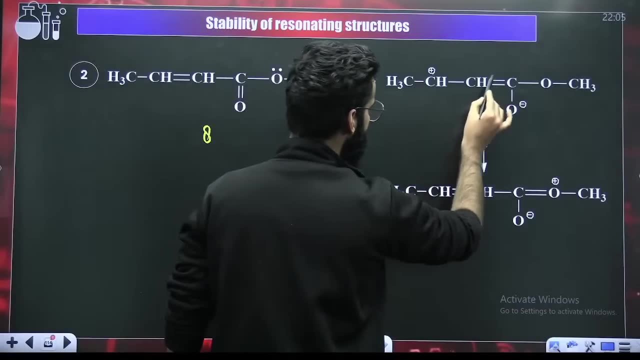 8 covalent bonds: 1,, 2,, 3,, 4,, 5,, 6, 7.. 8 covalent bonds: 1,, 2,, 3,, 4,, 5,, 6,, 7, 8.. 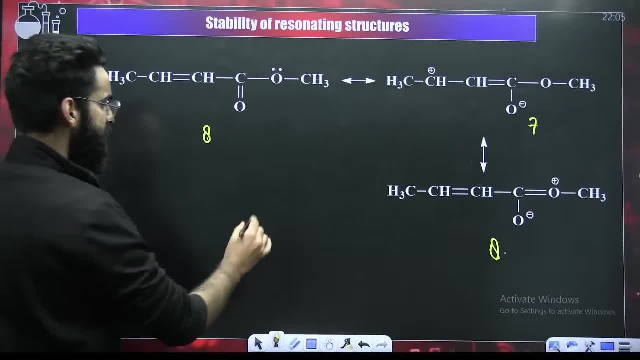 8 covalent bonds. Wherever bonds are minimum, that is least stable. So 1, 2, 3.. 2 is least stable. 2 is least stable Now among 1 and 3.. This is the resonating structure in which atoms do not contain any charge. 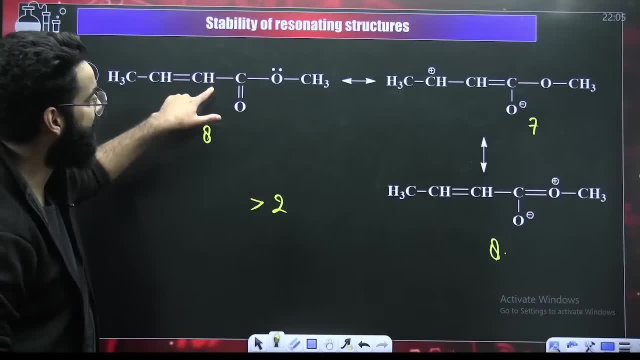 So 1 is maximum stable, Followed by 3.. Followed by 2.. All of you got this order: 1,, 3, 2.. All of you got this order: 1,, 3, 2.. 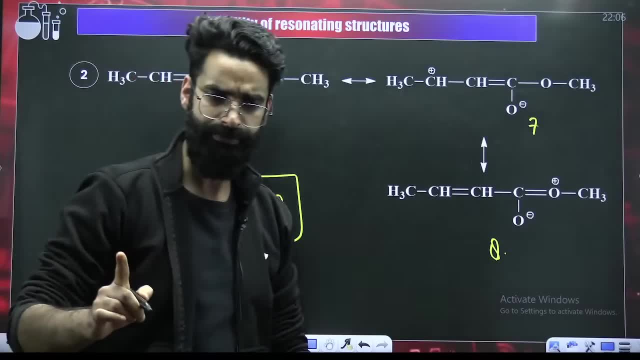 Perfectly done. Now let's have a look at the order of the covalent bonds. 1, 2, 3, 4,, 5,, 6,, 7, 8.. 8 covalent bonds. 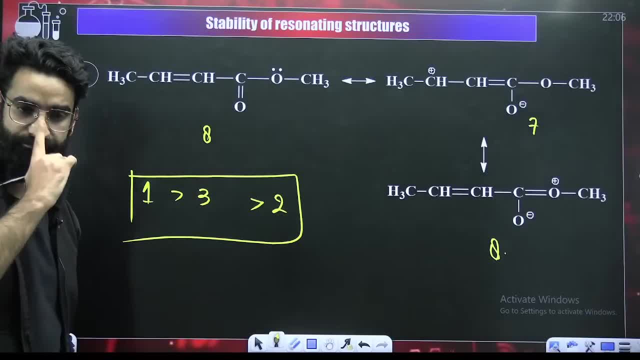 1,, 2,, 3,, 4,, 5,, 6,, 7, 8.. 8 covalent bonds: Perfectly done, Perfectly done, Wonderful. Okay, Tell me the answer of this question. 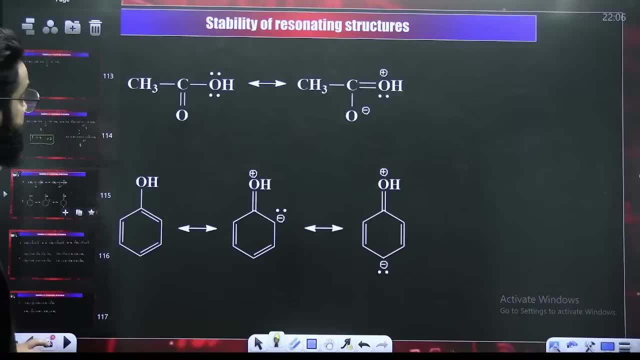 Among these two, which one is more stable? First calculate the bonds 1,, 2,, 3, 4.. 1,, 2, 3, 4.. Bonds are same. Bonds are same. Now, this one does not carry any charge on atoms. 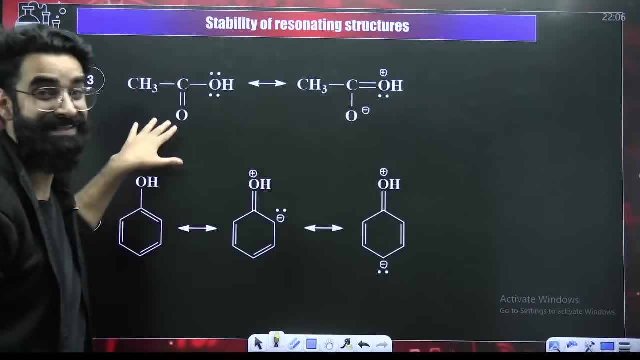 So this one will be more stable. 1,, 2, 3.. Calculate the bonds. Calculate the bonds 1. These are 6 plus 1, 7.. 1, 2, 3.. 1, 2, 3.. 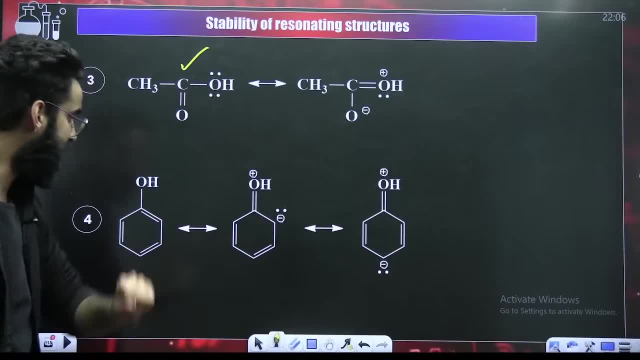 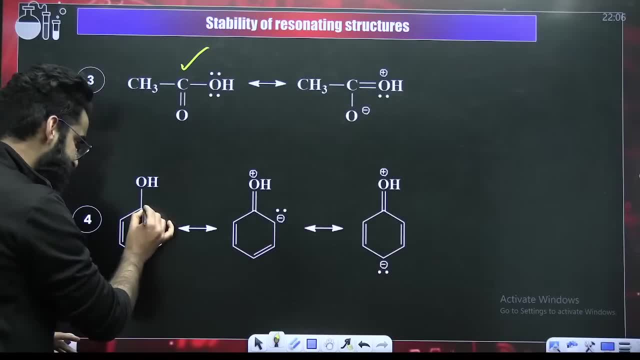 1, 2, 3.. 1. These are 6 plus 1,, 7.. 8,, 9, 10.. 10 internal bonds: 2. 2 plus 6 is 8. 8 plus 2 is 10.. 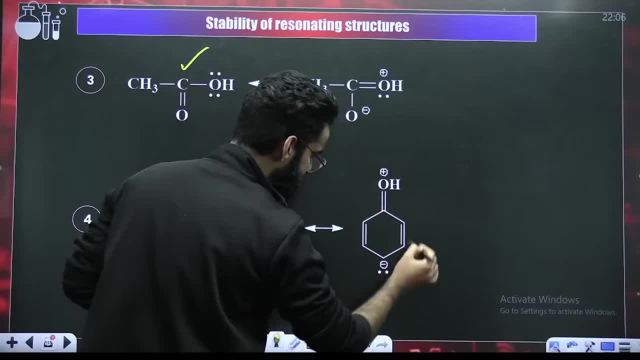 10. 2.. 2 plus 6 is 8.. 8 plus 2 is 10.. So bonds are same. Bonds are same. So I am not going to talk in terms of bonds. Now, what is the next thing? 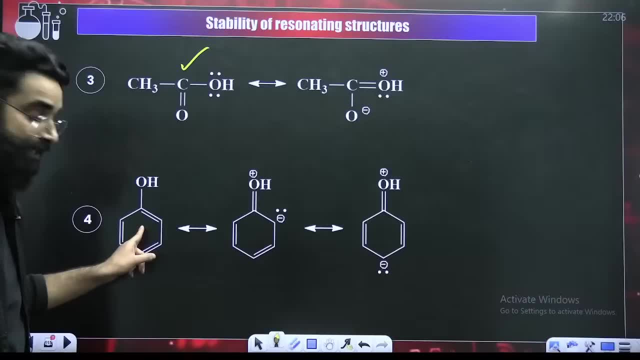 This particular resonant structure. its atoms do not contain any charge. It is maximum stable Now among 2 and 3.. Among 2 and 3.. See Oxygen carrying positive. Here also oxygen is carrying positive, Carbon carrying positive. 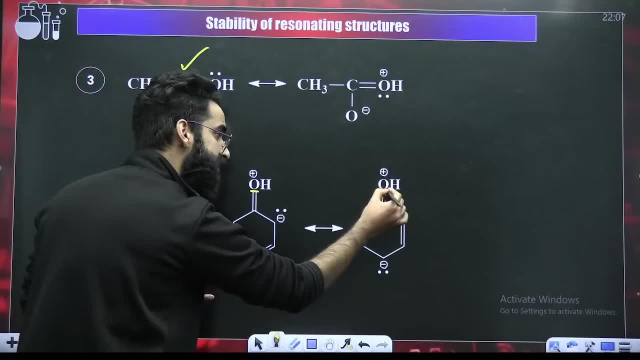 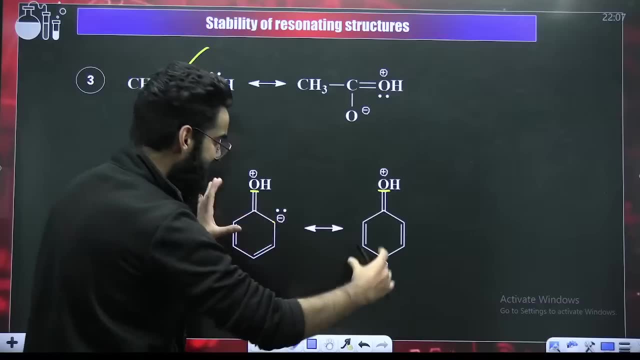 Carbon carrying positive, Oxygen carrying positive, Carbon carrying positive- Here also oxygen is carrying positive, Carbon carrying positive- Here also carbon is carrying negative. So these are the 2 resonant structures wherein same atoms carry similar charge: Oxygen positive, Oxygen positive. 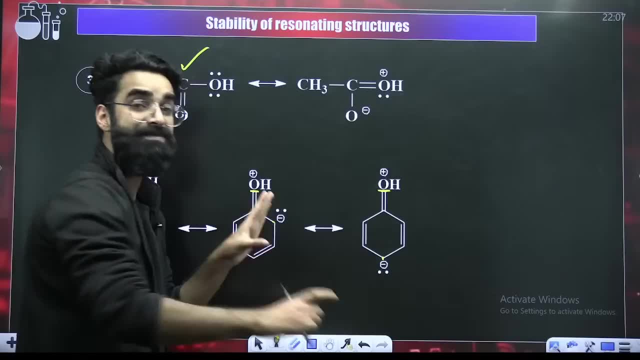 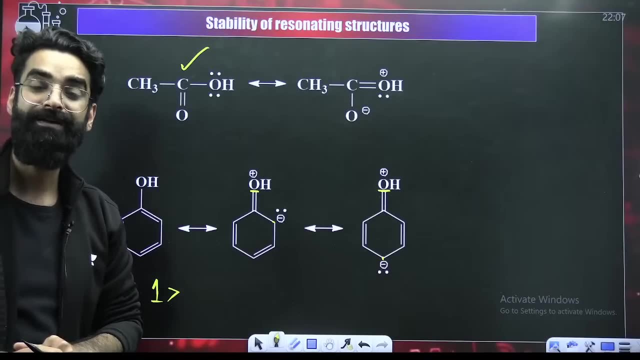 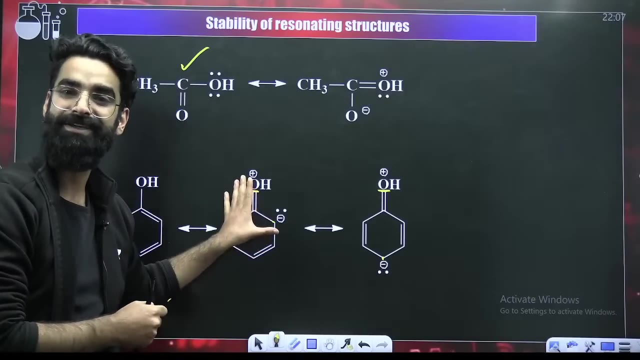 Carbon negative, Carbon negative, And when same atoms carry similar charge. at that point of time, what do we say? At that point of time, how do we distinguish? more stable, less stable? These are like charges or unlike charges. These are unlike charges. 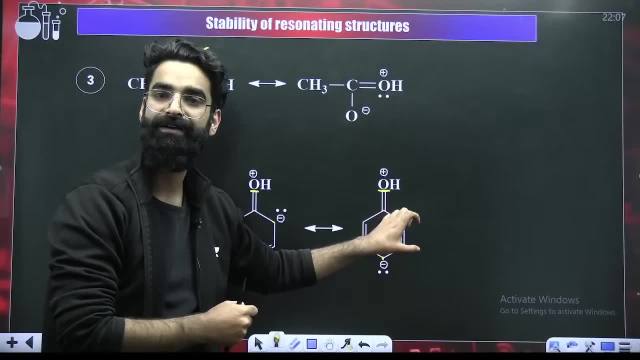 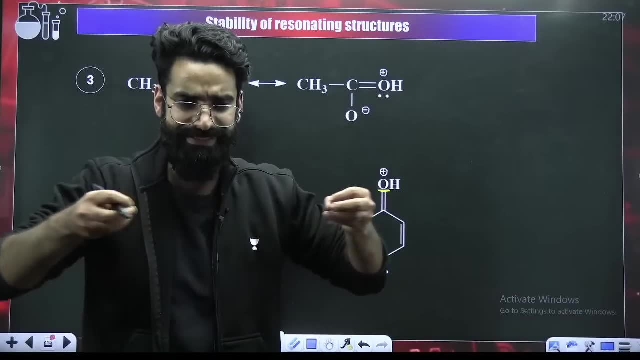 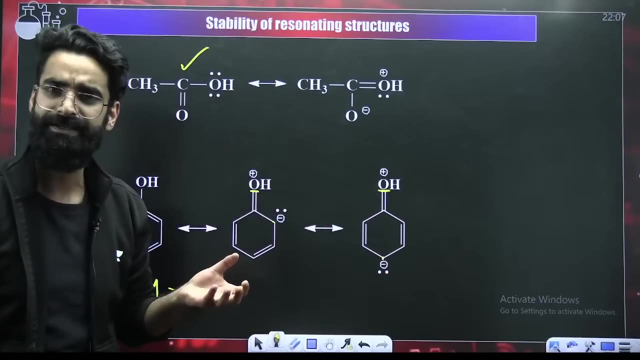 Positive, negative, Unlike Positive, negative, Unlike More. the distance between positive and negative- Can I say more- will be the potential energy of the system. As the distance increases between unlike charges, potential energy of the system increases. And if potential energy of the system increases, stability decreases. 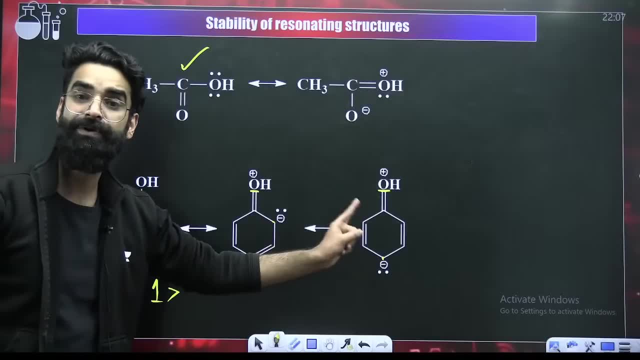 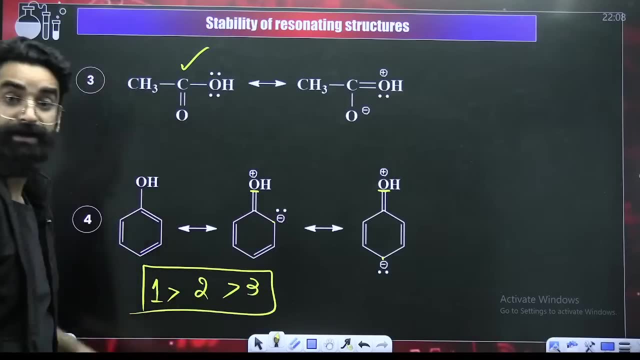 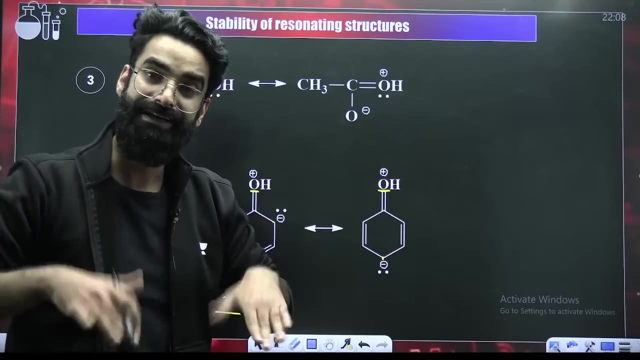 So which molecule will have more potential energy? This resonant structure will have more potential energy, So less stability. So 3 is least stable And here is 2.. I was talking about unlike charges, right? Well, more the distance between unlike charges, more is the potential energy of the system. 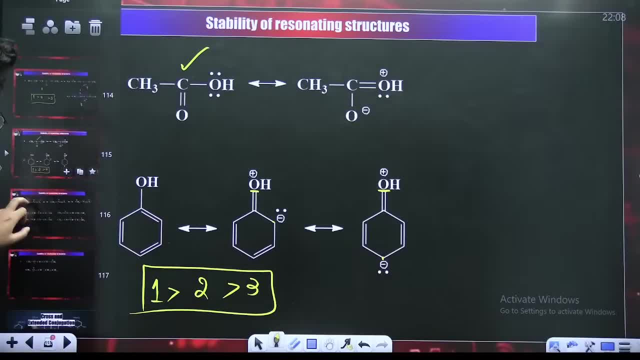 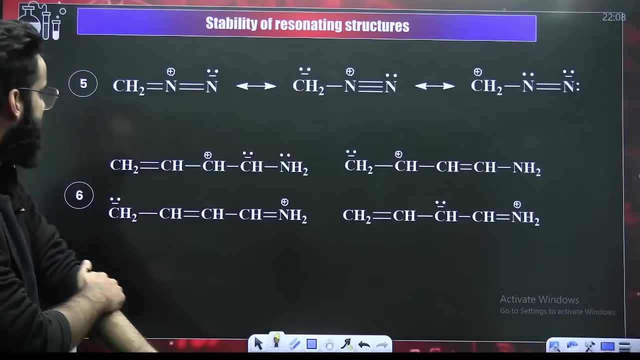 lesser is the stability right. So 1,, 2,, 3 is the order of the stability here. Alright, Among this and this, Okay, these are 3 basically given in the beginning: 2, 4.. 4 sigma bonds. 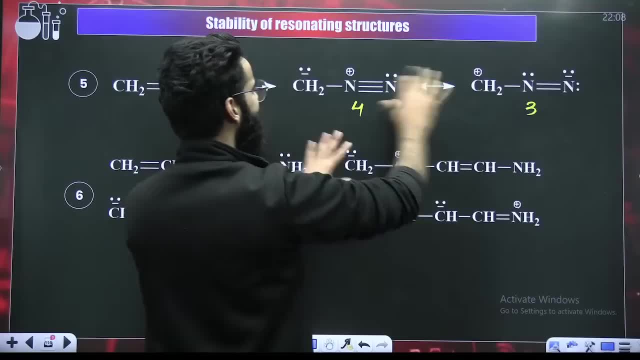 I mean 4 covalent bonds, 4 covalent bonds, 3 covalent bonds. So third one is least stable. Leave that. Third one is least stable Now, among 1 and 2.. Among 1 and 2.. 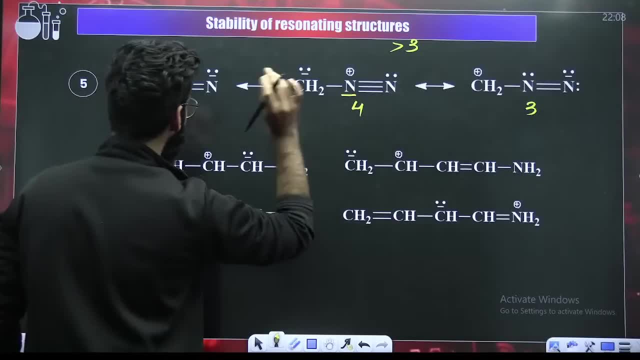 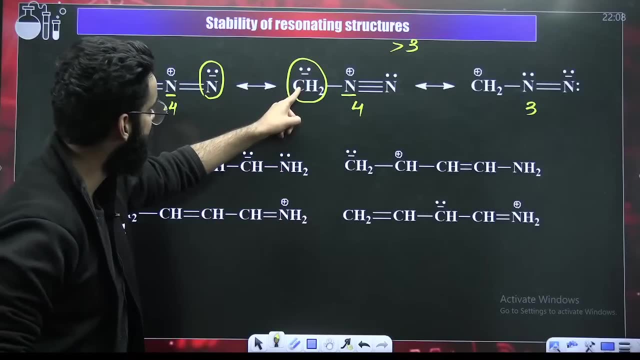 Check it out. See: Nitrogen carrying positive Nitrogen carrying positive: Perfect. This nitrogen is carrying negative And here carbon is carrying negative Nitrogen carrying negative Carbon carrying negative Nitrogen carbon. They belong to same period. 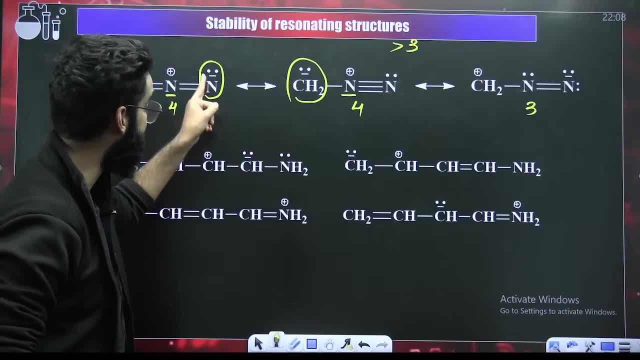 Same period, electronegativity plays a role. Negative charge is more stable and more electronegative, So this particular first one will be maximum stable, Followed by 2.. Followed by 3.. Do you agree with all this? 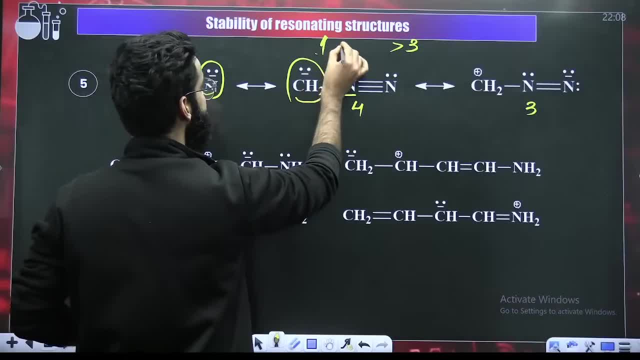 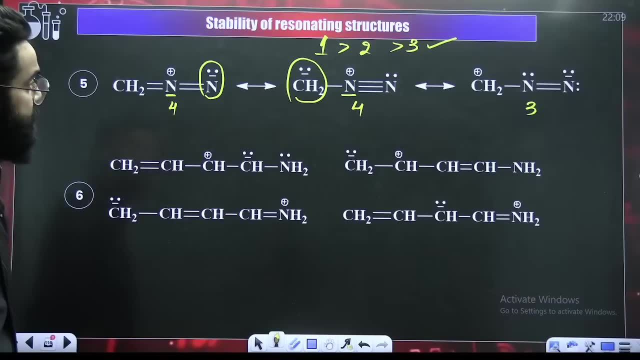 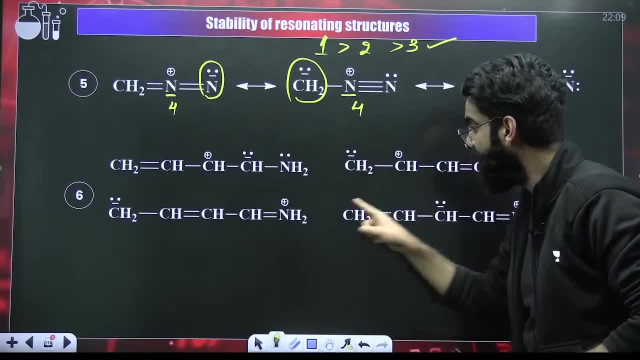 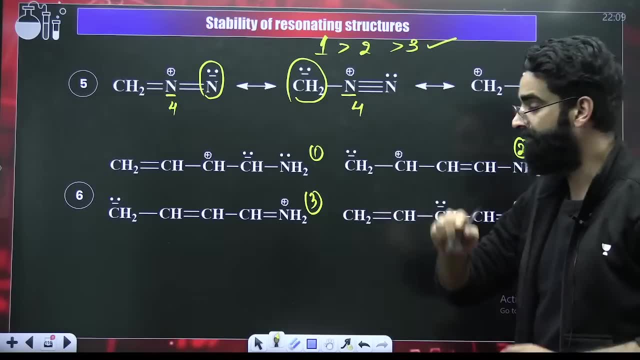 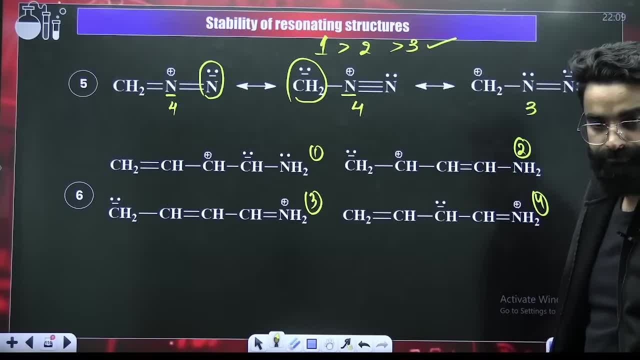 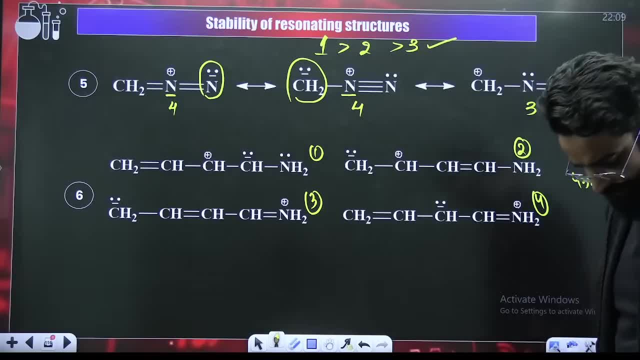 one of the option. i'll be taking four options from you. sweetie is saying the same thing: four, three, two, one. everyone is, i think, saying four three, one, two. i got one more option: four, three, one, two. okay, three, four, one, two. three, four, one, two. now. 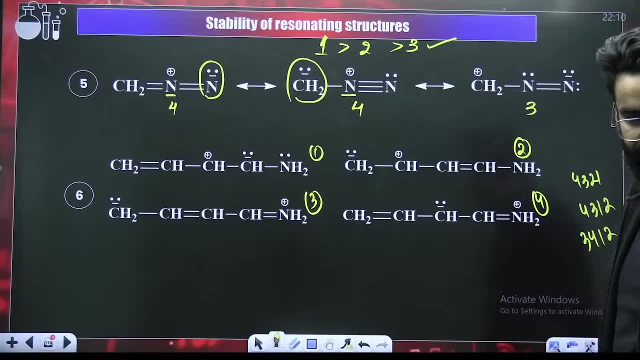 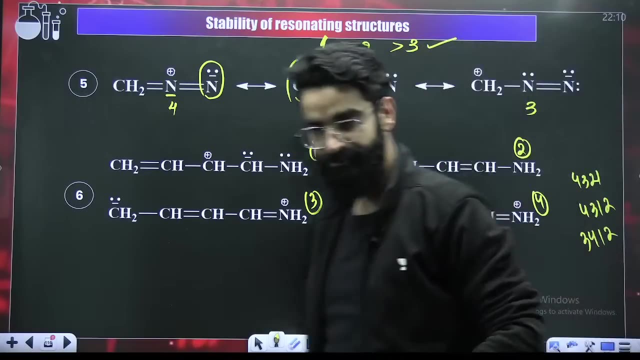 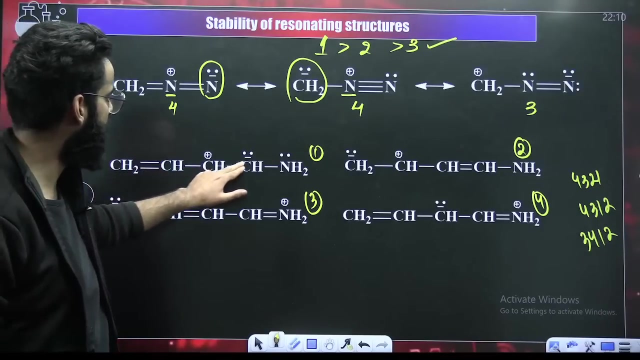 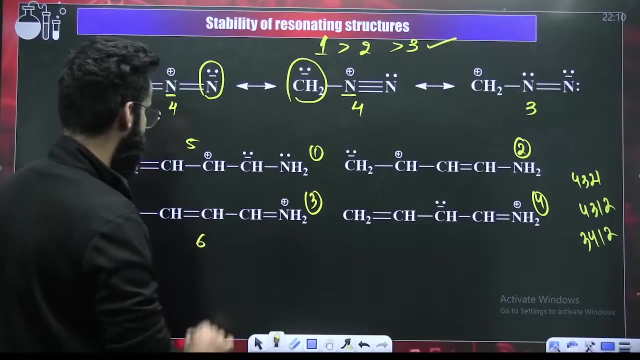 any any other? are you doing some permutation combination here? okay, let's have a look. let's see what is going to be the actual answer. first of all, count the total number of internal coordinates: bonds: two, three, four, five, right five. one, two, three, four, five, six. this is six. right one, two, three, four, five. 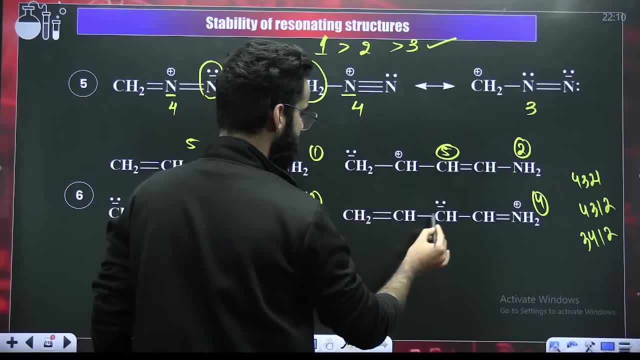 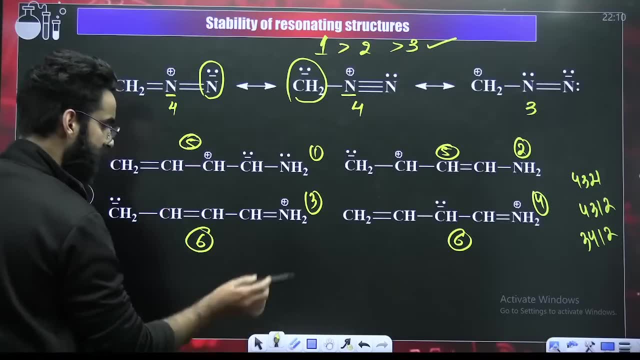 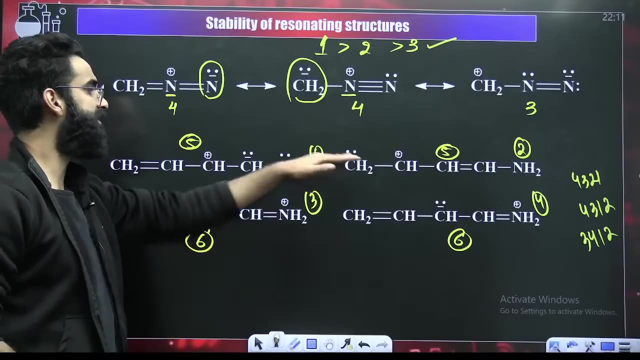 five, perfect. one. two, three, four, five, six. this is six, right? so you calculated. what did you calculate? you calculate the total number of internal coordinate bonds. now you tell me, more the bonds, more the stability. so it is evident that three and four will be more stable than 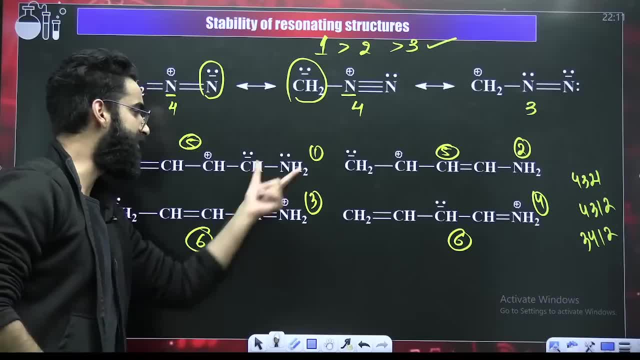 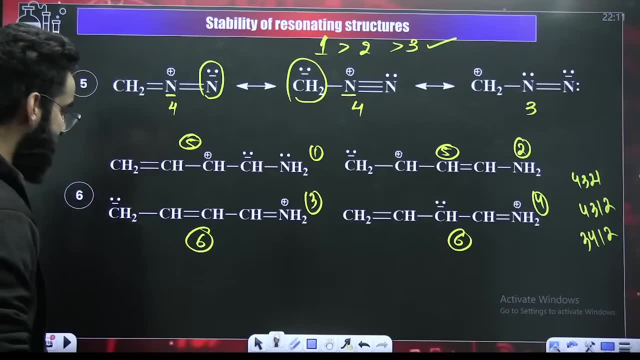 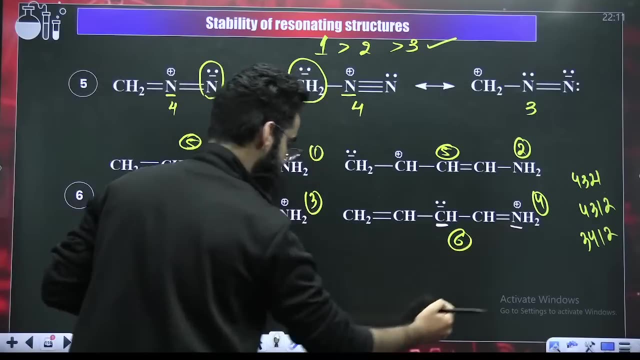 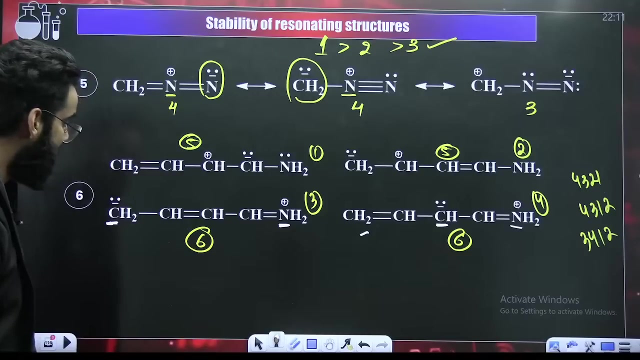 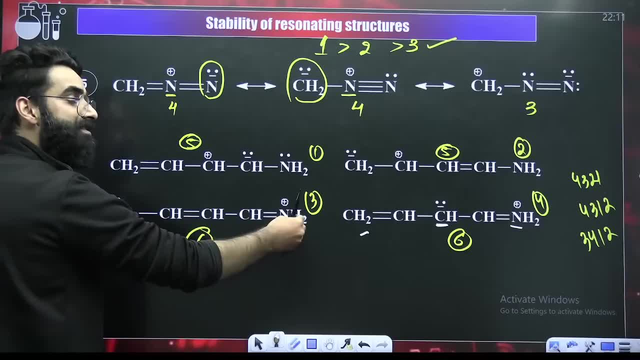 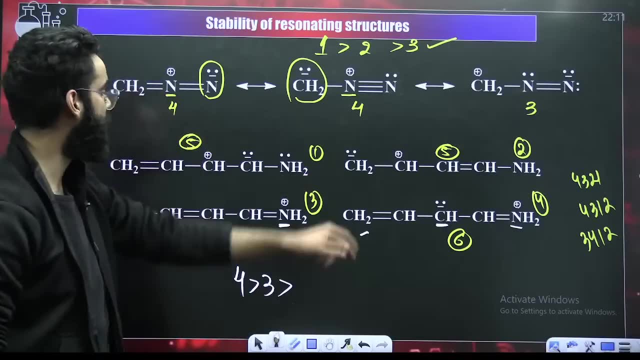 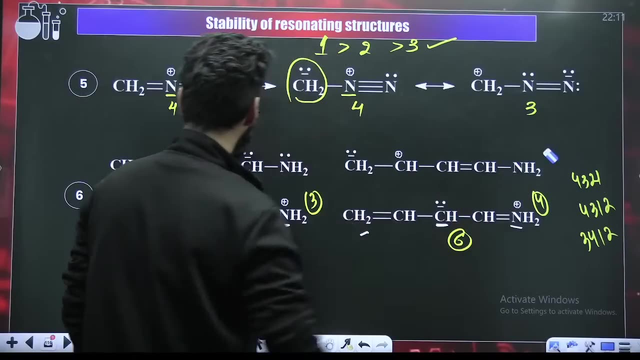 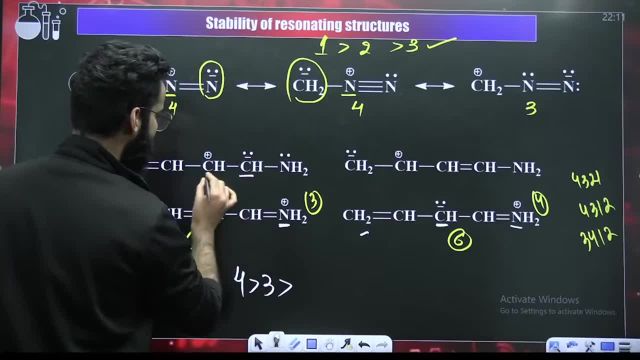 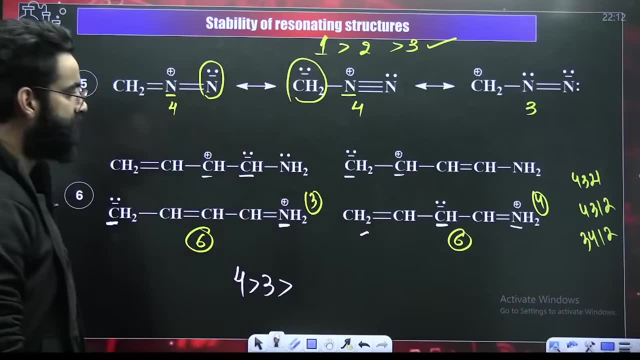 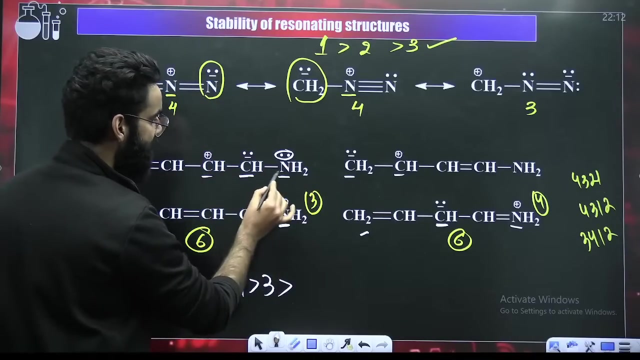 n2 and 1. what do you say? negative 1 carbon. positive one carbon: right. negative one carbon, positive one carbon, perfect. now here will you use the distance, the distance rule between? unlike no, after this carbon, there is nitrogen. nitrogen has got the lone pair. right after this carbon, there is a nitrogen, nitrogen has got a lone pair. so 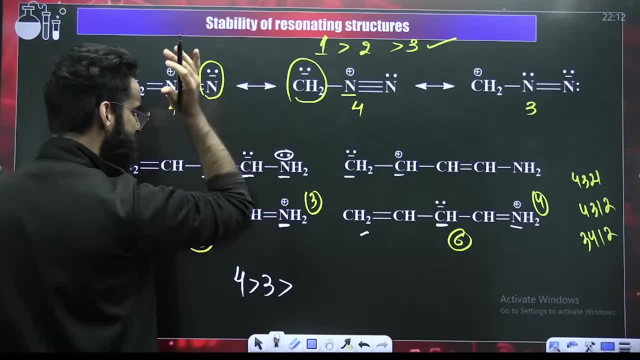 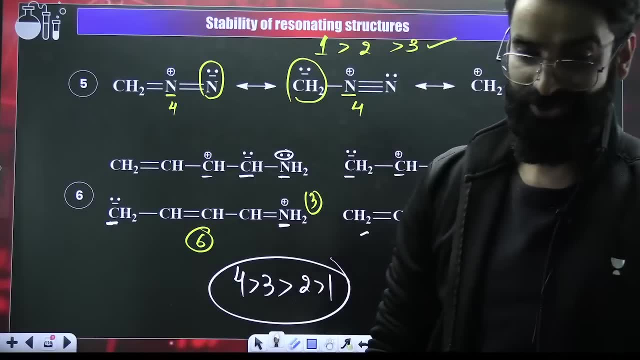 lone pair and negative, they'll ripple. ripple means more will be the energy of the stem, less is the stability, so two will be more stable than that of one. did you get this, guys? you should be able to solve these questions. i'm giving you the typical questions. these are not easy ones. 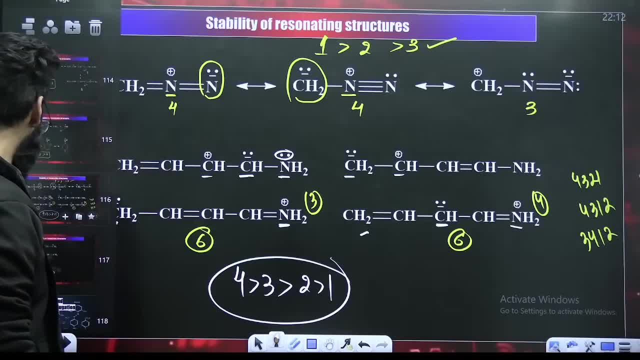 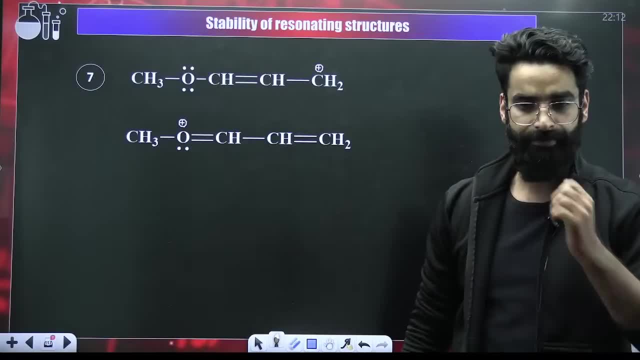 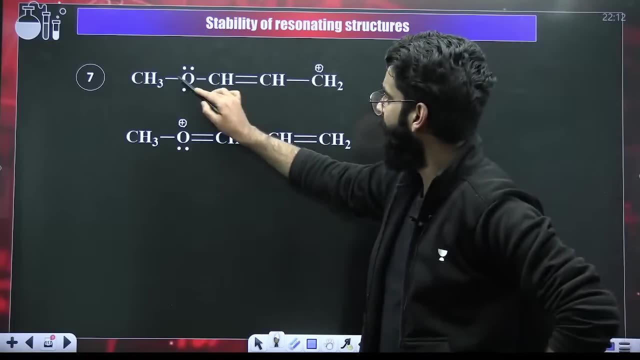 i'm giving you the typical ones wherein you can do a mistake, wherein you can do a mistake. tell me among these two which one will be more stable. this easily you can, this easily you can. one, two, three, four, five. one two, three, four, five, six, right two is more stable. one. 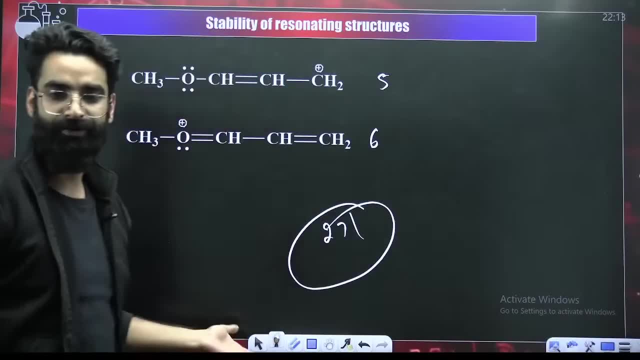 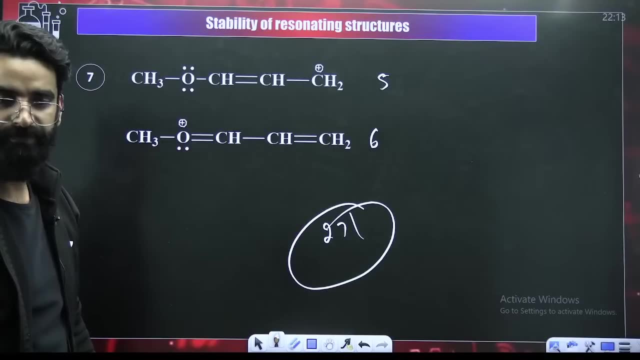 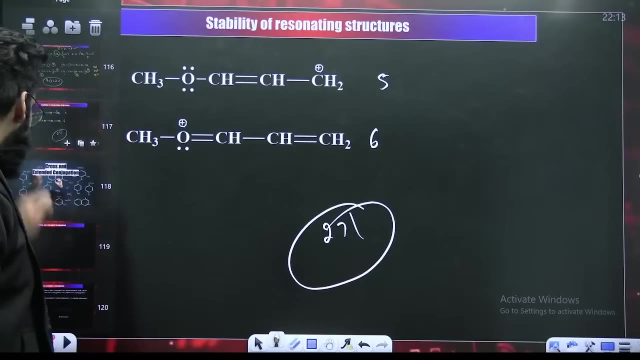 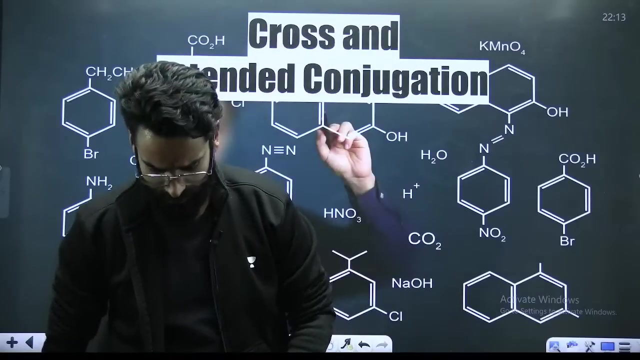 yeah, directly count the bonds from the bonds itself. you got to know everything right from the bonds itself. you got to know everything, every possible thing. i hope this is clear to everyone. now let's move on to one more topic, that is, cross and extended conjugation. have you ever come across this particular topic? cross and extend conjugation. 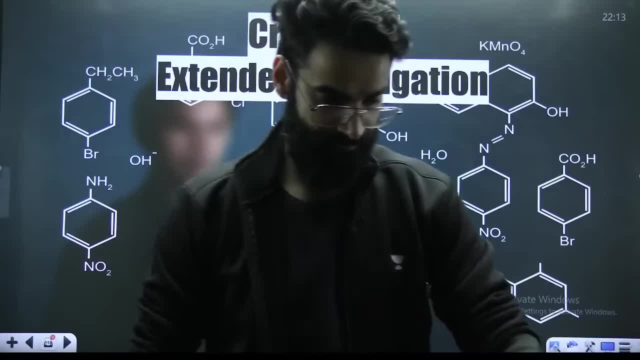 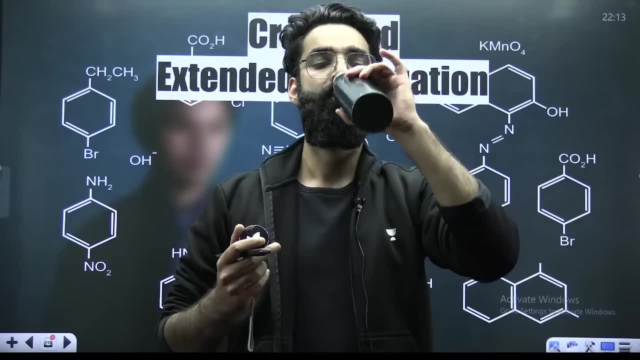 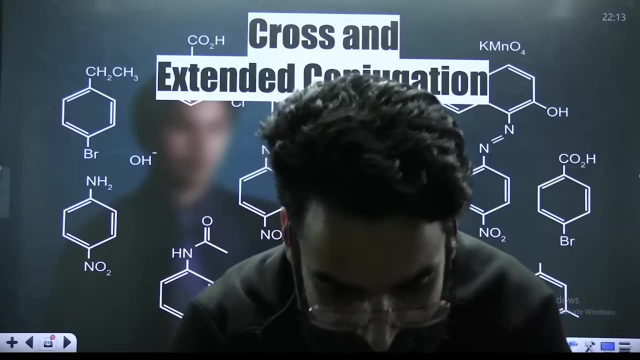 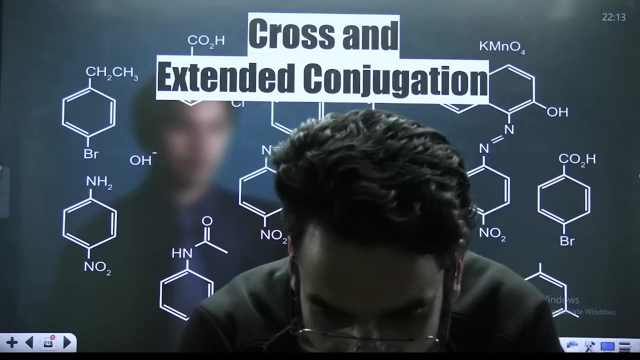 have you ever come across this particular term: cross and extended conjugation. guys, i think the josh is over. is the josh over? do you want me to cancel the class from here? do you want me to cancel the class from here? is josh over, is the josh over? 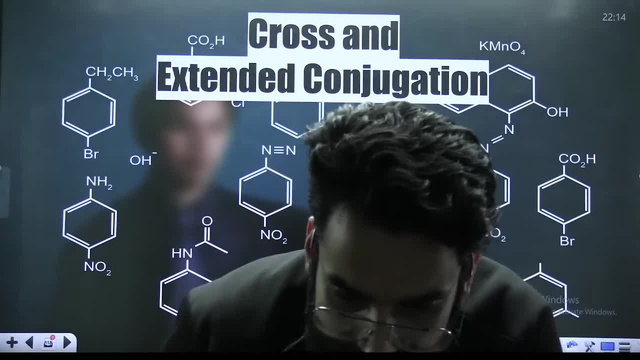 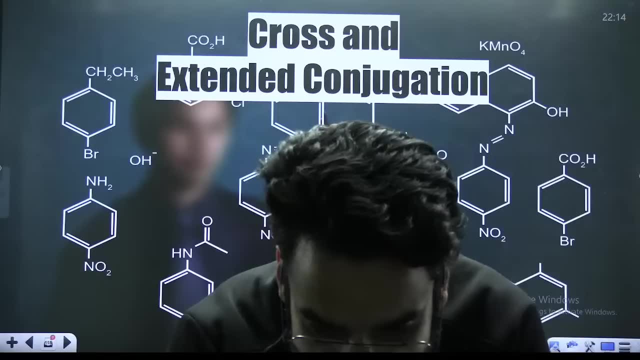 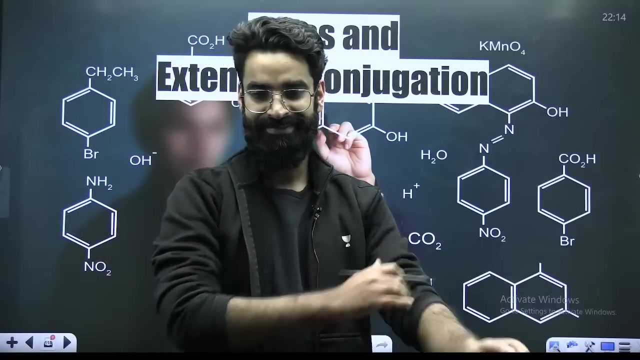 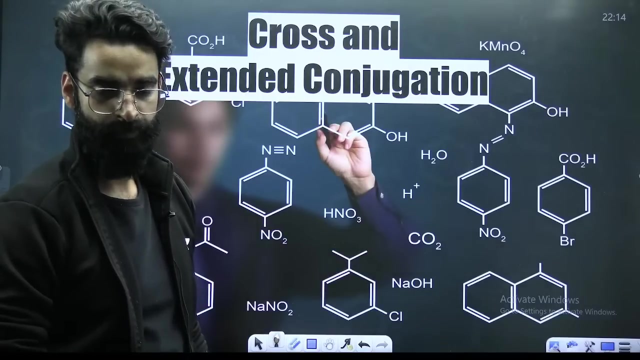 is that. it is that. it are you done, you done. i want everyone to say: it is the josh still high? is the josh still high? no, right now i'm not giving any break. we'll complete this topic, then maybe we'll see: is fire still left or it's over? 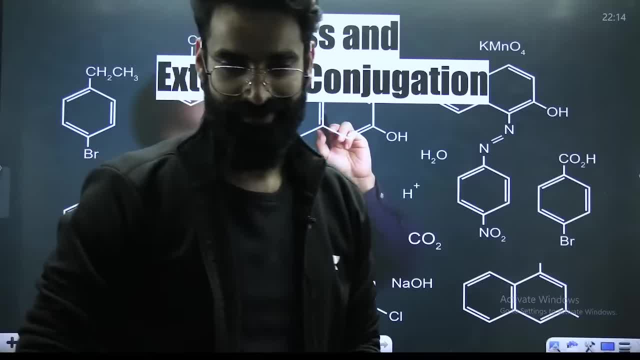 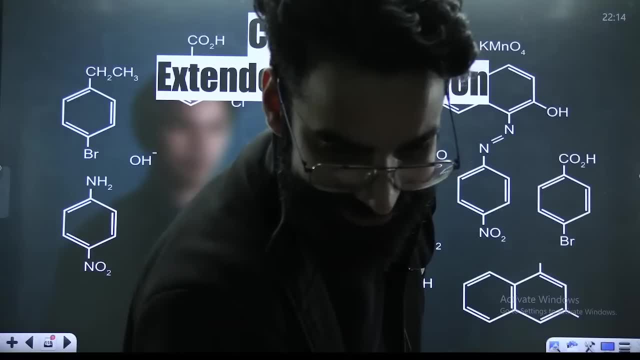 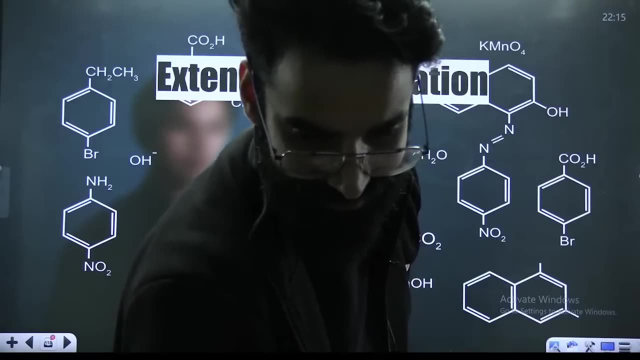 is fire still left or it's over? are you all active, guys? don't do this. don't do this, okay, don't sleep before school for me. I'm not going to be the one who's going to write the exam, okay? and I'm not sure whether you would have solved these sort of questions before or not. I don't. 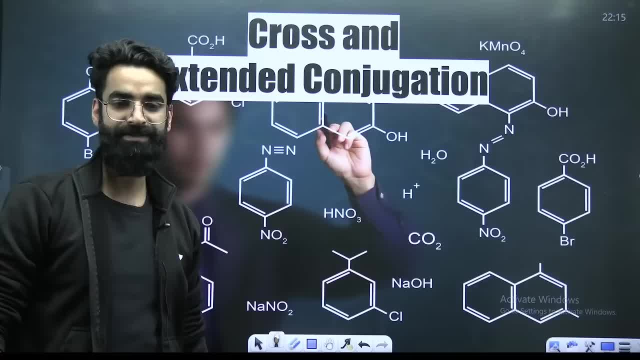 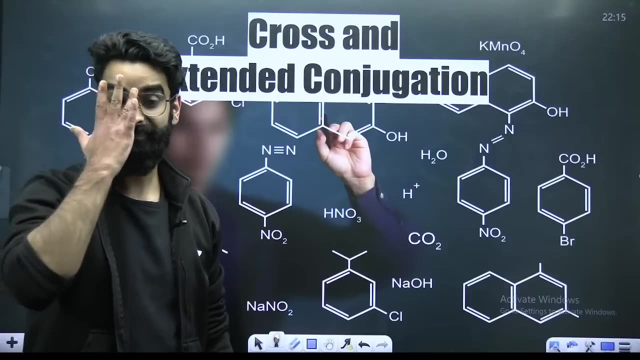 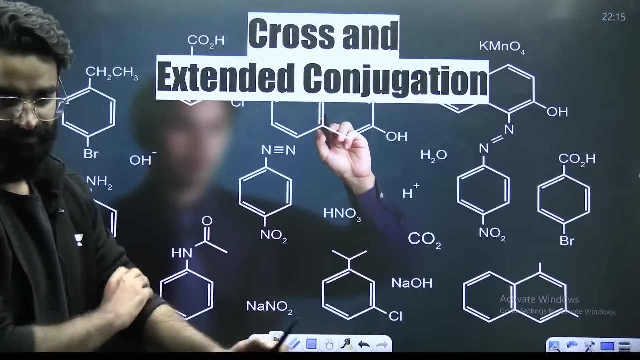 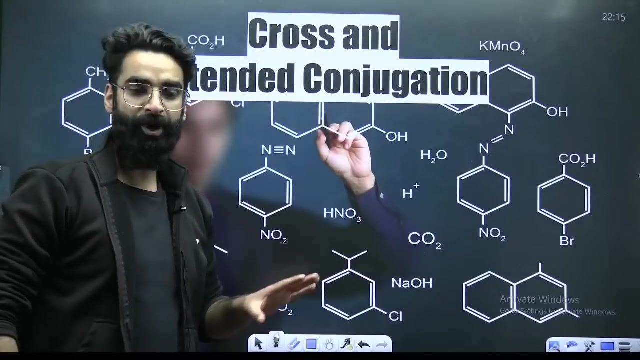 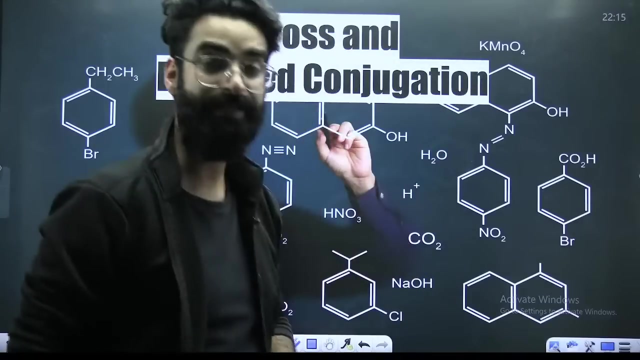 think is a typical example which I'm giving you, typical examples which I'm giving you a you, hmm, okay, yes, sharp magnet JS parent can also watch it. hello, let's have a look on one more topic. this is again important: cross and extended conjugation, right cross and extended cause. now, what is? 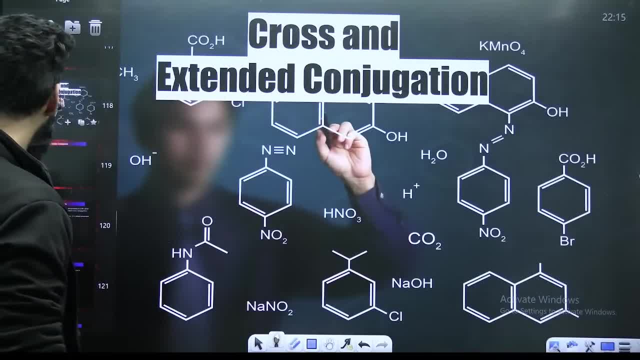 conjugation from one distance to another distance, then now drag into a cross and extended conjugation. all about: See guys, see guys. in just a second, look at this particular slide once. from this particular slide, I will make you understand what is cross. 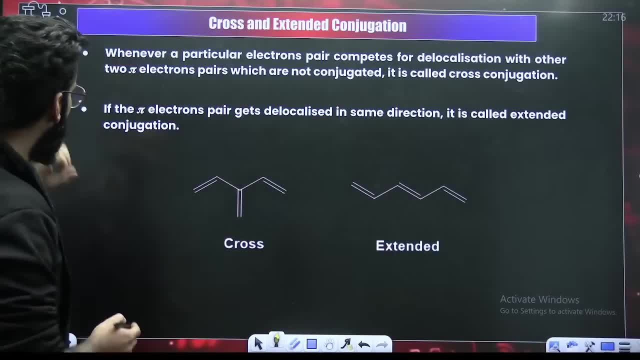 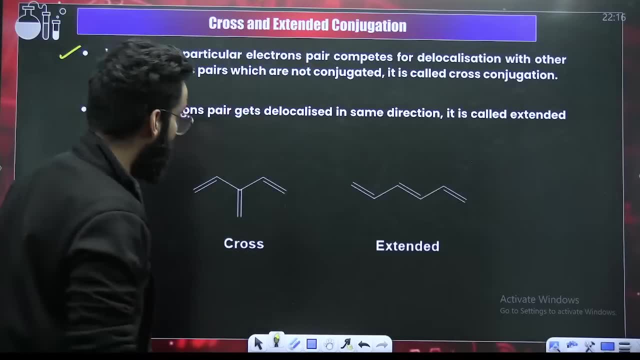 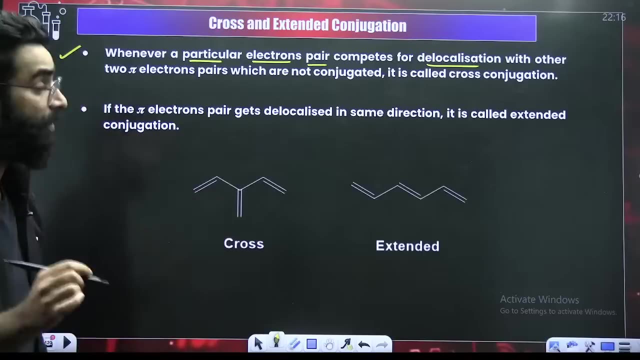 and extended conjugation all about. If you read the first point: whenever the first point says: whenever a particular electron pair, whenever a particular electron pair competes for delocalization, whenever a particular electron pair competes for delocalization with 2 pi electron pairs, with two pi electron pairs which are not conjugated, it is termed 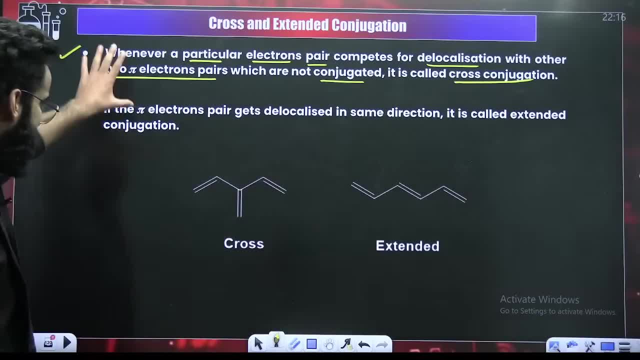 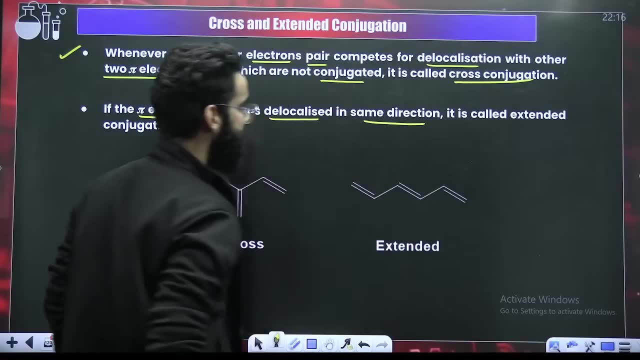 as cross conjugation. it is termed as cross conjugation. What is meant by this? you will get the idea in some time. If the pi electron, if the pi electron pair gets delocalized, localize in the same direction, It's called as extended conjugation. Try to understand. 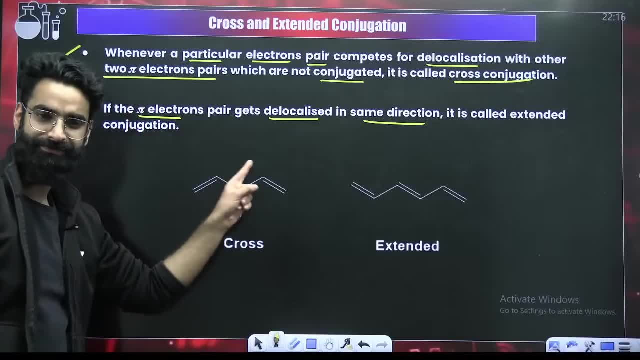 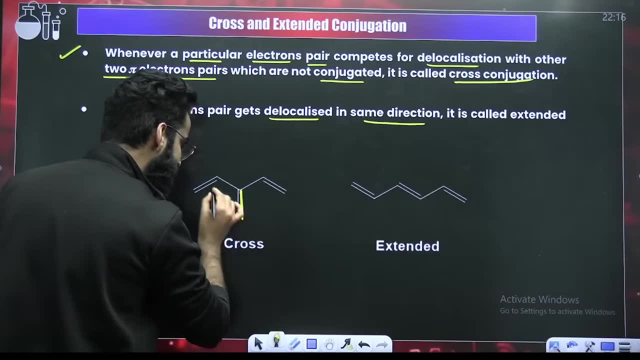 what it means. IDS students, if you look at this particular molecule, look at this particular molecule carefully, Carefully. look at this particular molecule. Here you have got a pi bond. Right Here you have got a pi bond. Here you have got a pi bond. Look at this. 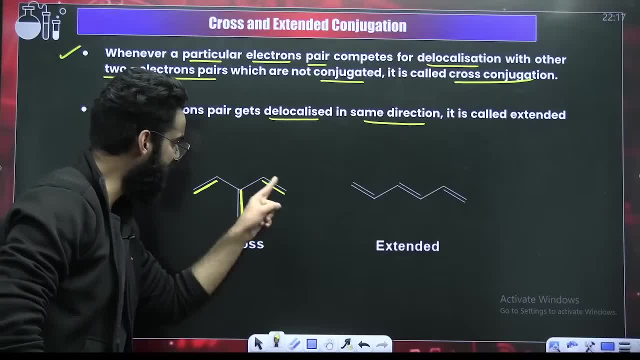 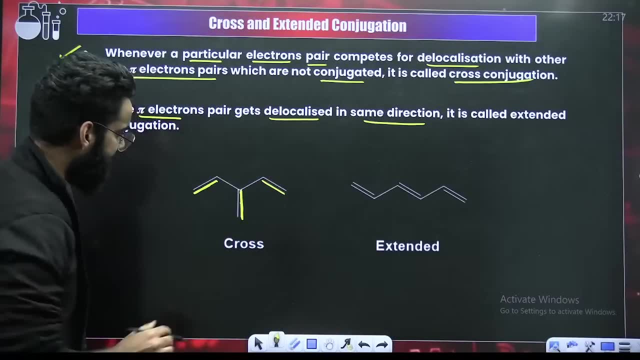 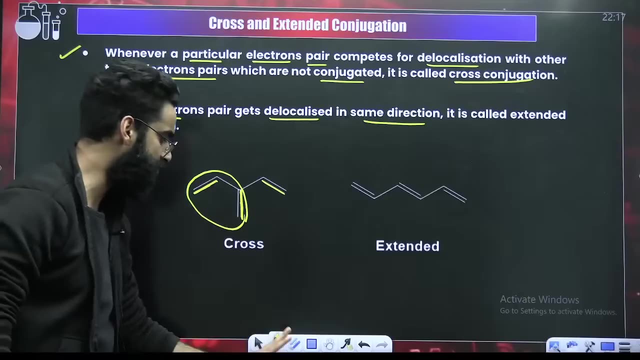 Pi sigma pi. Pi sigma pi. There is conjugation over this particular side. Pi sigma pi Right. Similarly, pi sigma pi. Again there is conjugation. Again there is conjugation On both the sides, there is conjugation Correct. Can I say this particular pi electron pair, this particular. 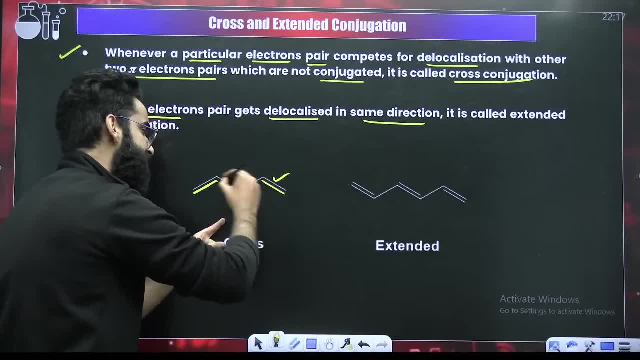 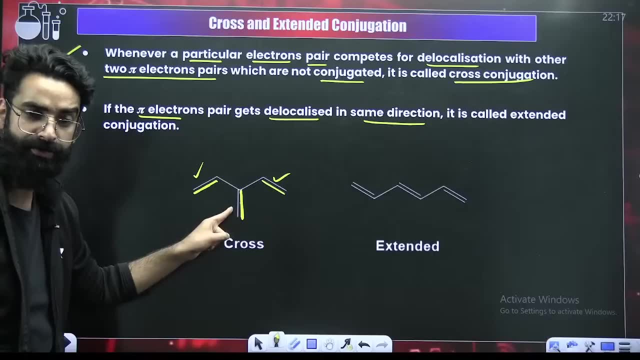 pi bond, it is simultaneously in conjugation with this one as well as this one, This particular electron pair, this particular pi electron pair. it is simultaneously in conjugation with this pi bond, as well as this pi bond, Whereas if I consider these two pi bonds, 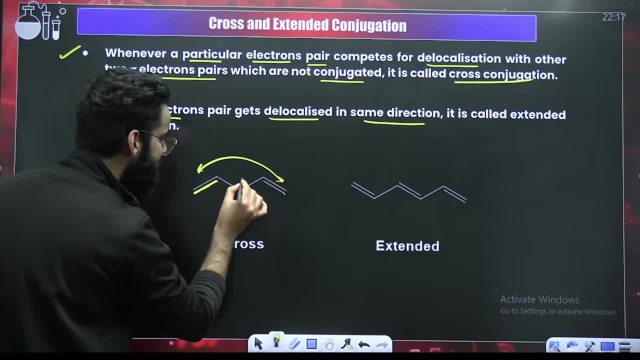 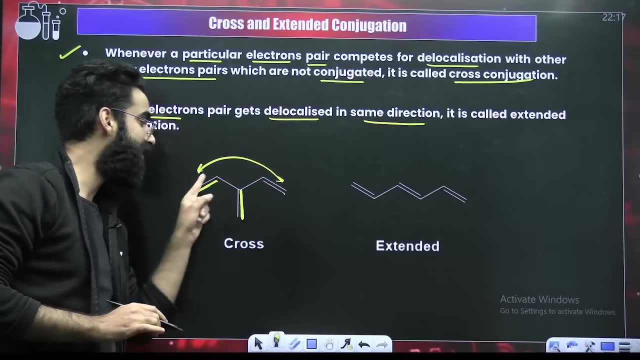 are these two pi bonds conjugated? This is pi sigma, sigma pi. They are not conjugated with each other. They are not conjugated. I will say: this particular pi bond is in conjugation with this one, as well as this one, Whenever you see this kind of the scenario in which a particular electron 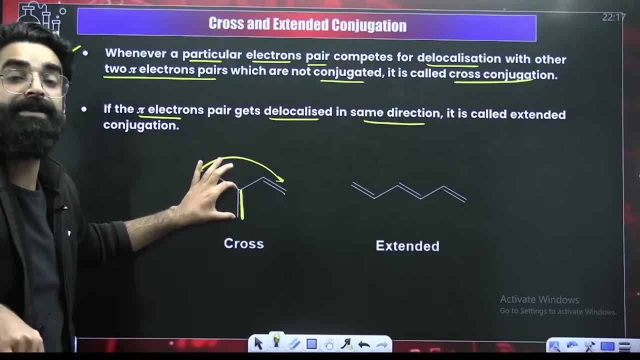 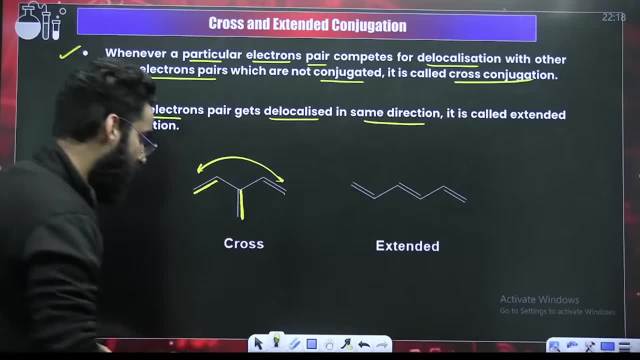 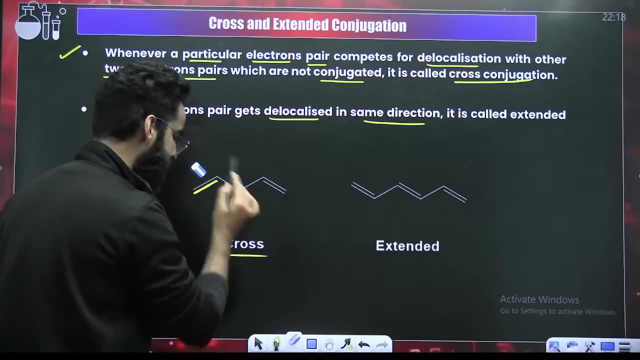 pair simultaneously will be in conjugation with. will be in conjugation with two electron pairs. will be in conjugation with two pi electron pairs. This is something which I call as cross conjugation. Whenever a particular electron pair, whenever a particular electron pair, whenever a particular. 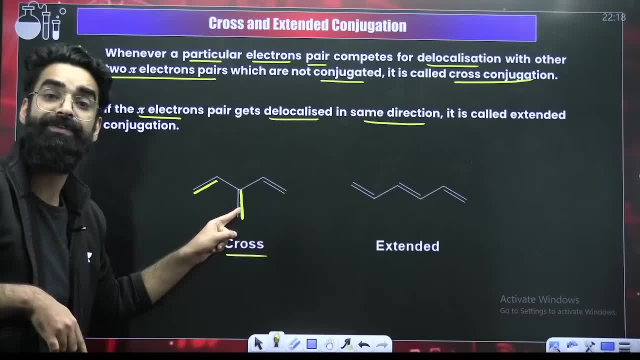 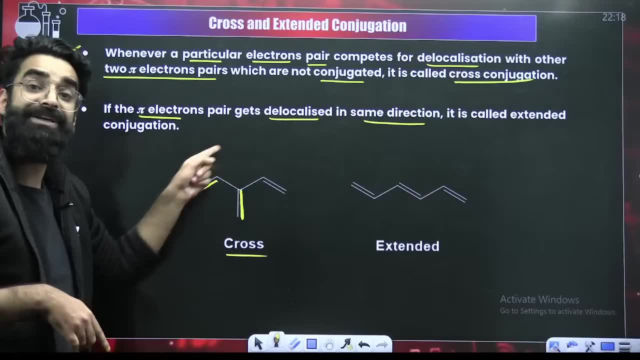 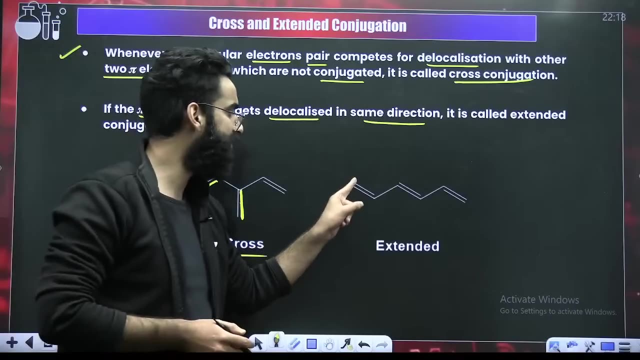 high energy electron pair is simultaneously in conjugation with is simultaneously in conjugation with two other high energy electron pairs, But those two high energy electron pairs are not conjugated. This particular system is what you call as cross conjugation, Whereas if you look here, this is pi sigma, pi, sigma pi. The conjugation is in a single. 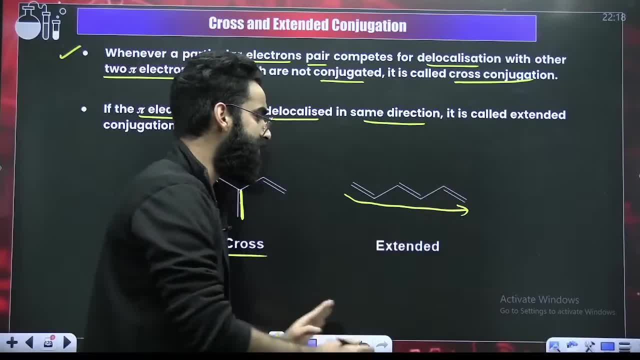 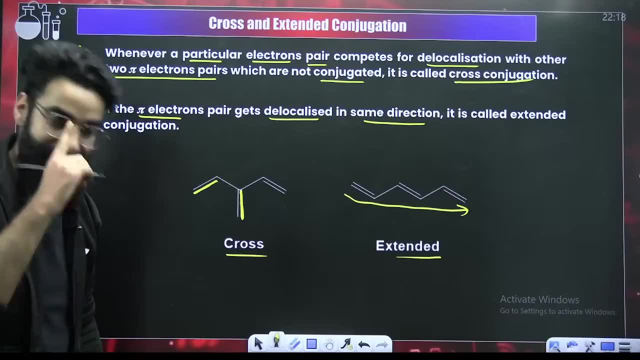 direction, When your conjugation is in single direction. this is something which you will be calling as extended conjugation, You can call it as linear conjugation. You can call it as linear conjugation. Let me tell you, people, extent of resonance. extent of resonance in cross. 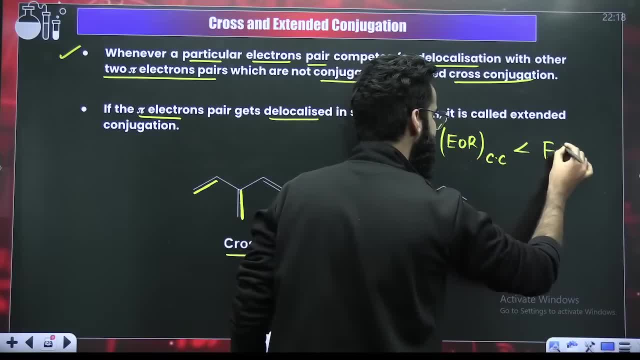 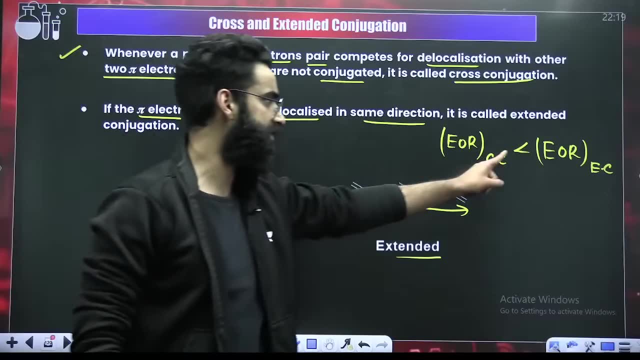 conjugation is always less than that of extent of resonance in extended conjugation. Extent of resonance in cross conjugation is always less than that of extent of resonance in extended conjugation. And do remember, extent of resonance decides the stability More the extent of 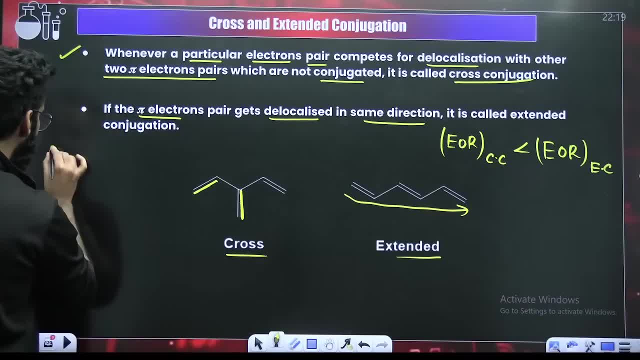 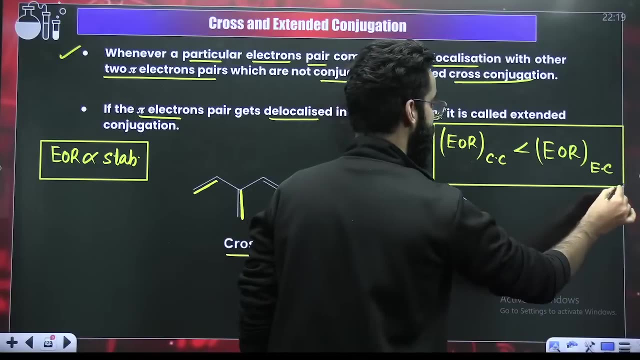 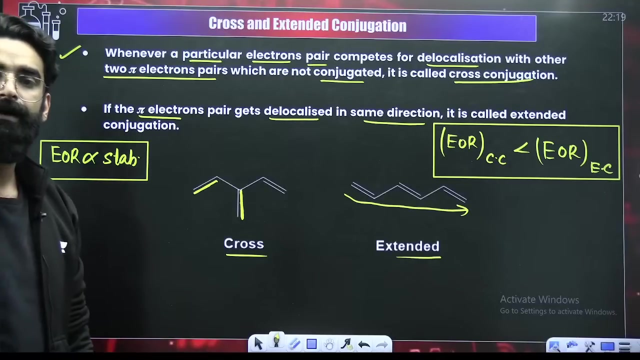 resonance, more the stability, More the extinct of resonance, more the stability. More the extend of resonance, more the stability. So tell me one thing: over here, a pi electron pair represents E1. over here and over here, an j electron pair represents j дополнative. 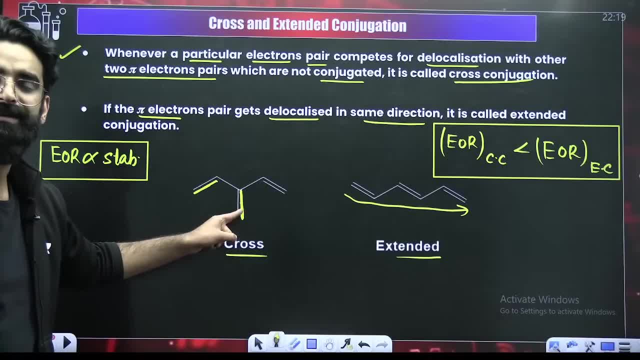 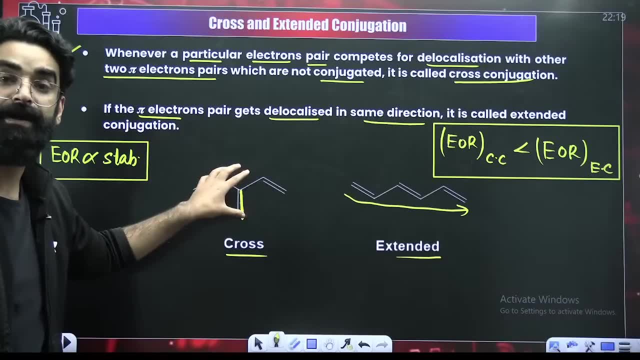 line over here We will see this- Come on. pair is simultaneously in conjugation with these two electron pairs, but these two electron pairs themselves, they are not conjugated. this kind of the system is something which we call as cross conjugation. but here there is a. 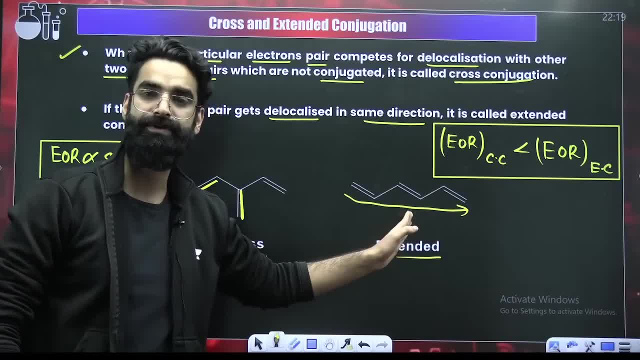 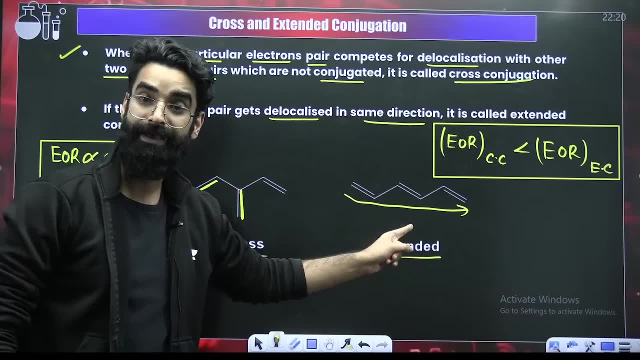 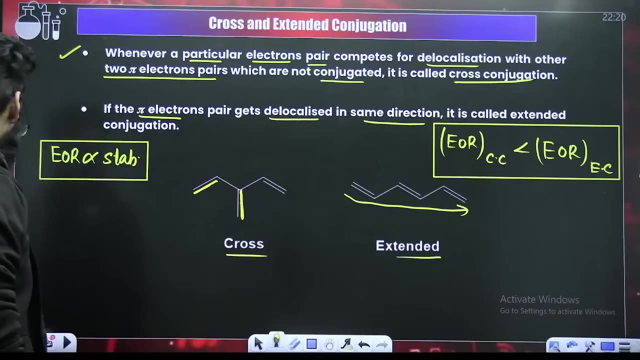 conjugation in one direction. you call it as linear conjugation or extended conjugation. extent of resonance in cross conjugation is the less than that of extent of resonance in extended conjugation. right wherever extent of resonance is more, stability is more just. if you remember two things, you are done. 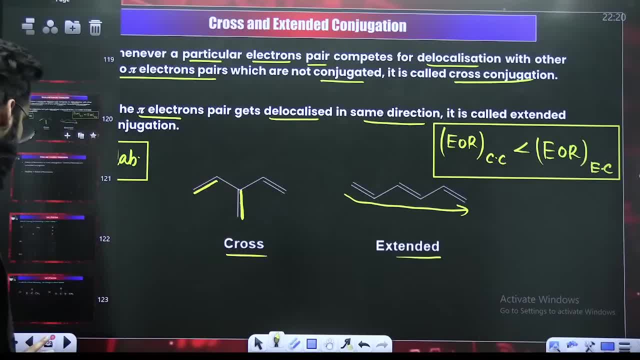 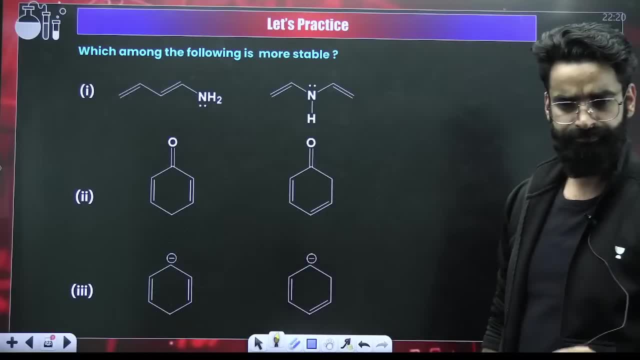 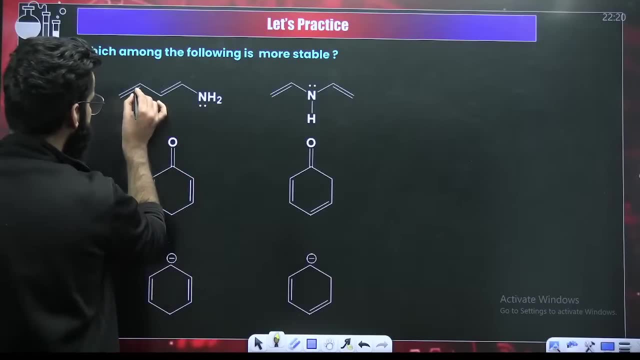 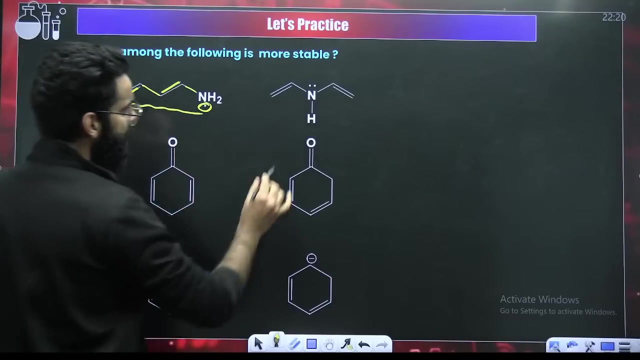 if you just remember these two things, you are done. tell me the answer: which one among these two is more stable? which one among these two is more stable, first or second? more stable first of all, my dear students, if you have a look, this is PI, Sigma, PI Sigma lone pair. the conjugation is throughout, right over. 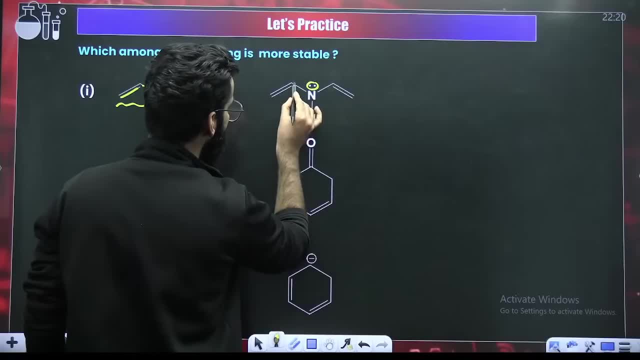 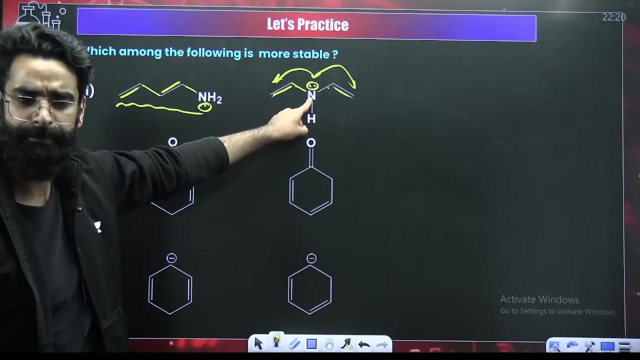 here. this is: this is PI Sigma lone pair. okay, this is PI Sigma lone pair. even this is PI Sigma lone pair. so can I say this lone pair is in conjugation in this direction as well as this direction. so can I call this as the example of cross conjugation? it is the example of cross. 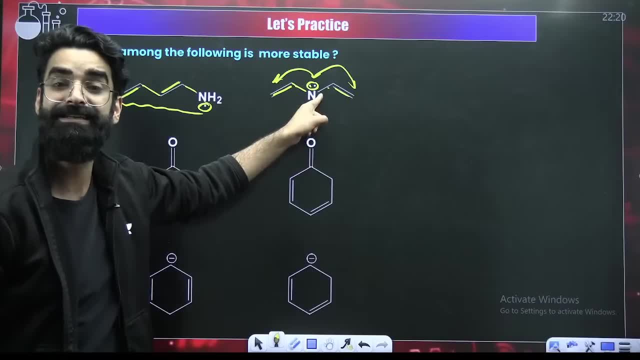 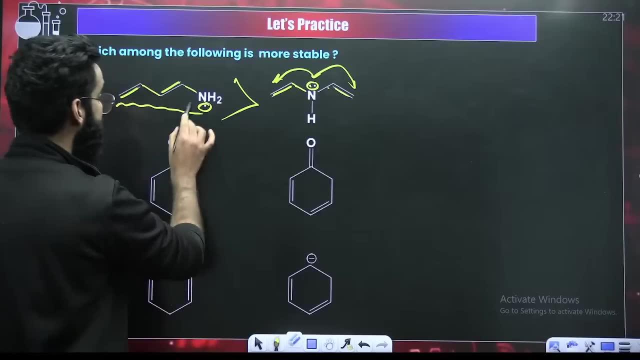 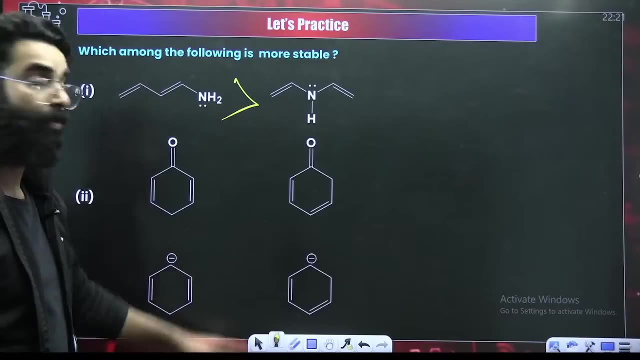 conjugation, extent of resonance in cross is less. if the extent of resonance in cross is less, stability is less. so which one is more stable? I'll say first one is more stable. right, and my dear students, this concept you are going to use, use at the time when both these molecules will have same pi electrons. Have a look. 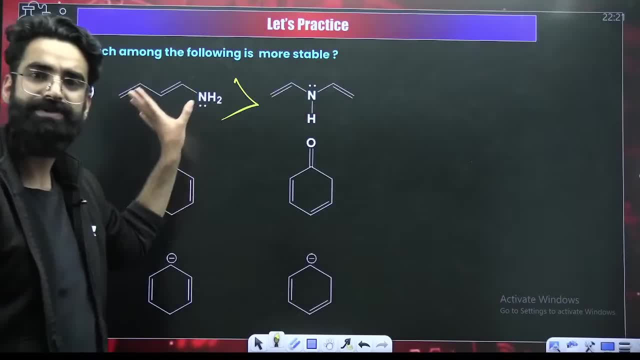 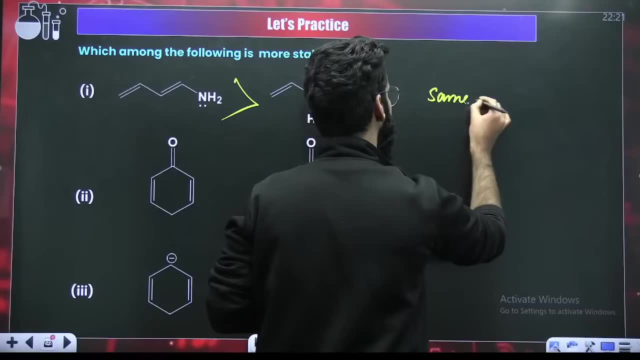 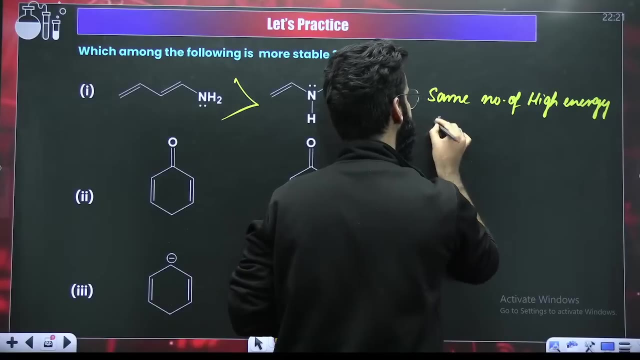 2, 4, 6.. 2, 4, 6.. So same number of high energy electrons are there. Both these molecules are having same number of high energy electrons. So whenever same number of high energy electrons are there, whenever same number of high energy electrons are there at that point of time. 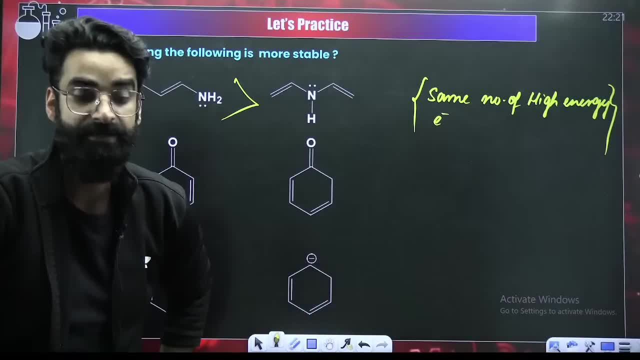 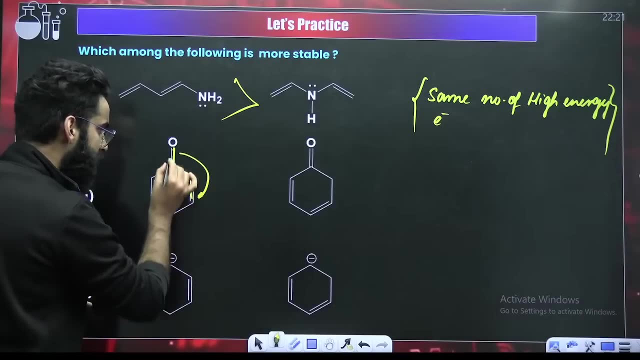 you are going to use the concept of cross and extend conjugation. Otherwise, not, Otherwise, not Tell me. in this case, See, this is pi sigma pi, So conjugation. Now, pi sigma pi, Conjugation. So I will say this: high energy electron pair. I will say this: high energy. 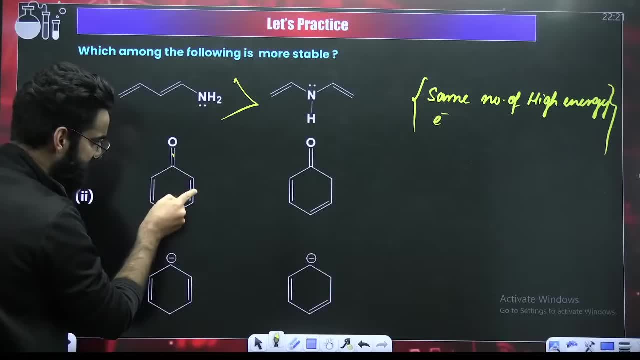 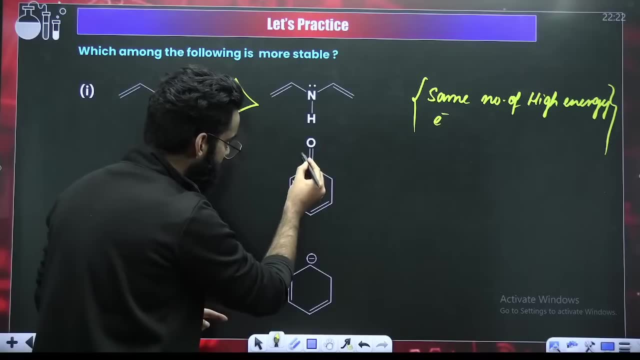 electron pair. This high energy electron pair is simultaneously in conjugation with this one, as well as this one. So this is the example of cross. Look at this one: Pi sigma, pi, sigma, pi. So conjugation is throughout. Conjugation is throughout. 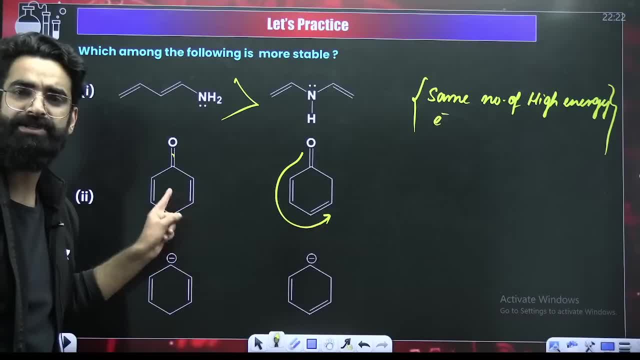 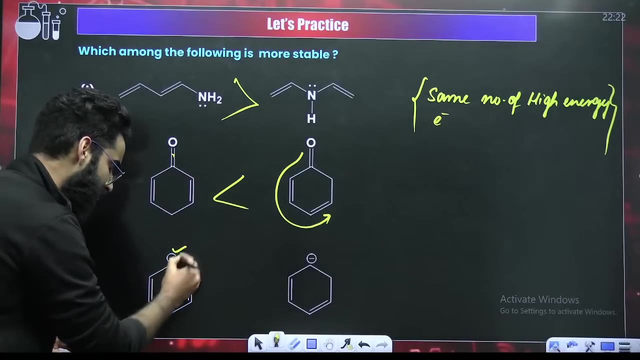 Right. So this is cross conjugation Extent of resonance and cross is less Extent of resonance and cross conjugation is less, So stability is less Right. Look at this one, This negative Pi sigma negative, Pi sigma negative. So this high energy electron pair. 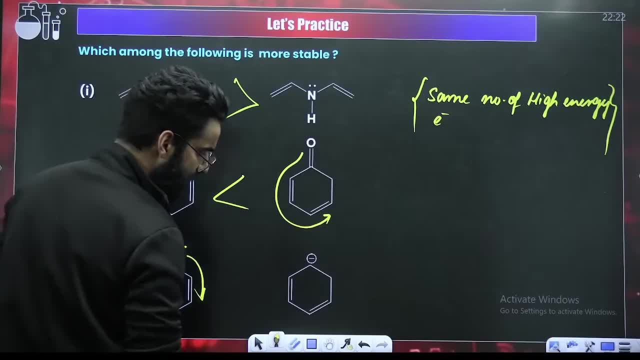 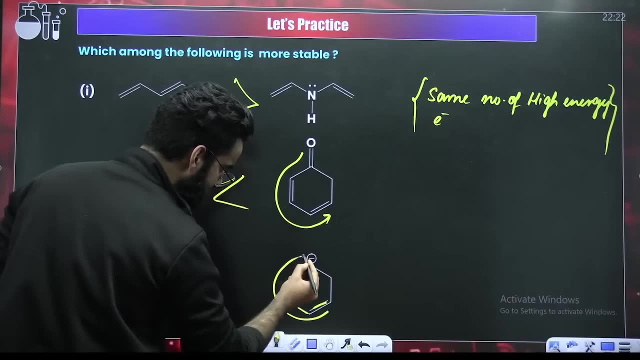 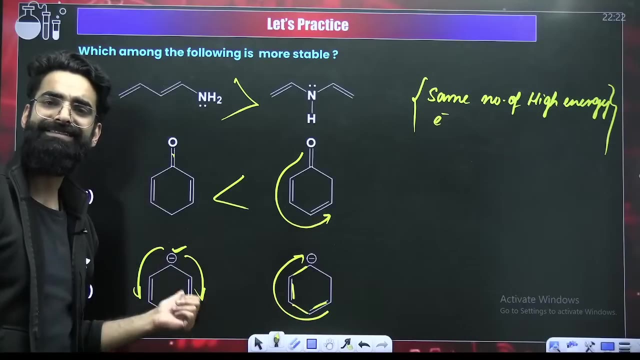 is conjugated on this side as well as this side. Right, Okay, But have a look on this one. This is pi sigma, pi sigma, negative. Here conjugation is cross Conjugation is basically right. this is your cross, this is your extended right. extent of resonance in cross is: 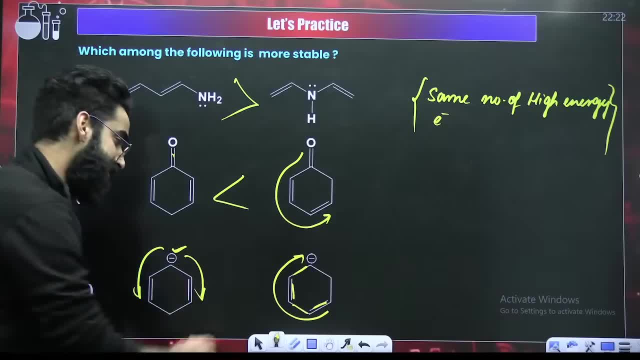 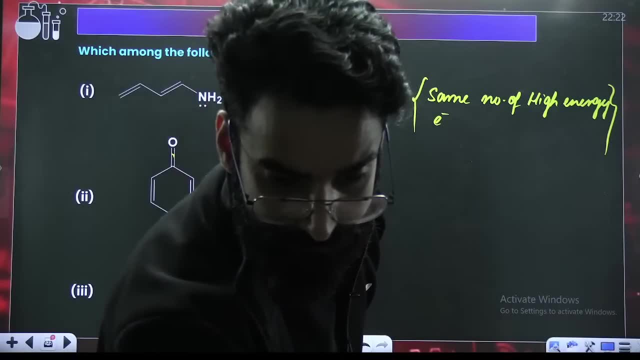 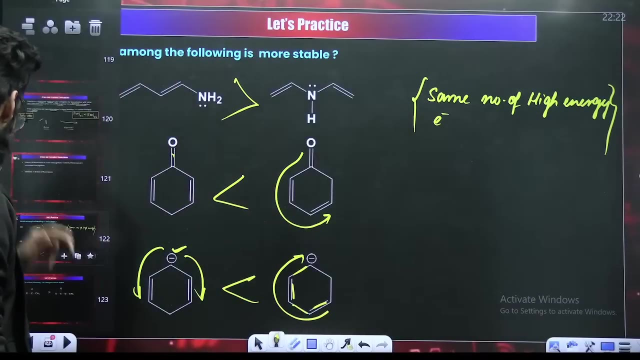 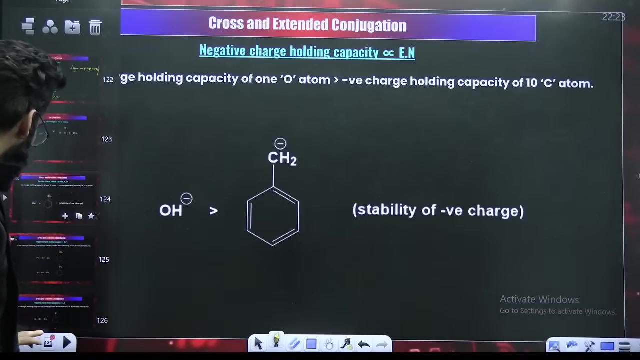 less. if extent of resonance in cross is less, stability is less. so this is the stability order. this is the stability order. is it clear? is that clear, people, quickly, is it clear? i believe this is clear. all right, tell me one more example, just a second. okay, one more. one more thing? from which question comes? 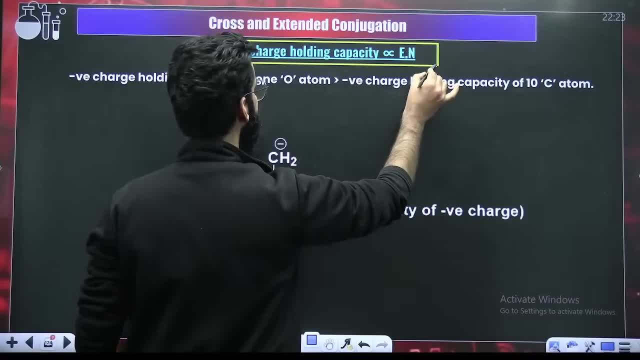 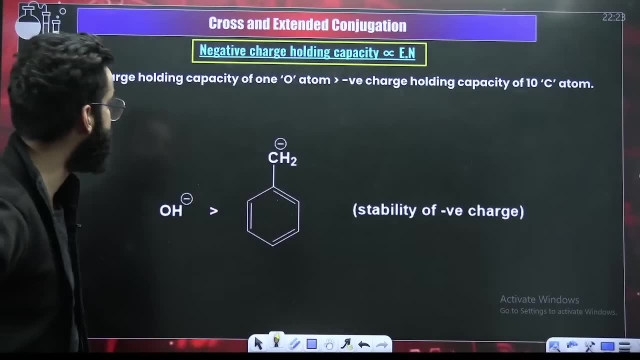 that is, negative charge holding capacity. negative charge holding capacity of an atom. negative charge holding capacity of an atom by these students, as i told you in the starting of the lecture. then, negative charge holding capacity of an atom. negative charge holding capacity of an atom by these students, as i told you in the starting of. 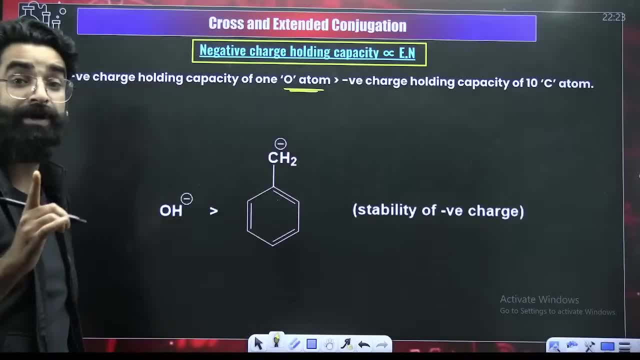 holding capacity of an atom by these students, as i told you in the starting of holding capacity of one oxygen atom, holding capacity of one oxygen atom. holding capacity of one oxygen atom. the negative charge holding capacity of one. the negative charge holding capacity of one. the negative charge holding capacity of one oxygen atom. it is greater than the. 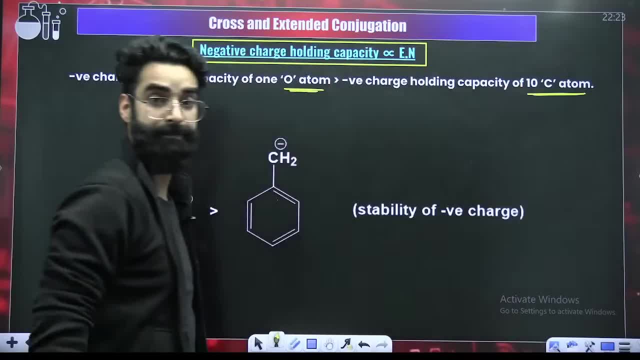 oxygen atom. it is greater than the oxygen atom. it is greater than the negative charge. holding capacity of negative charge. holding capacity of negative charge. holding capacity of 10 carbon atom. 10 carbon atom- 10 carbon atom. the negative charge holding capacity of one. the negative charge holding capacity of one. 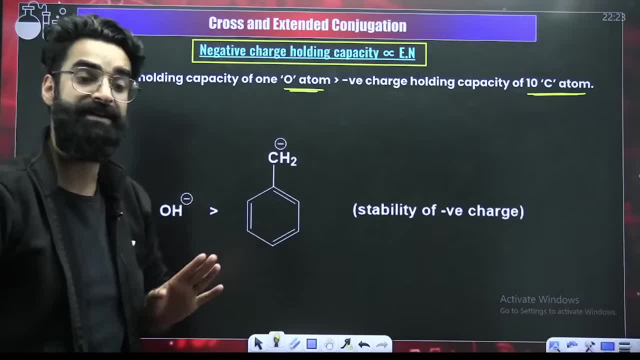 the negative charge holding capacity of one oxygen atom is even greater than the negative oxygen atom, is even greater than the negative oxygen atom, is even greater than the negative charge holding capacity of 10 carbon charge. holding capacity of 10 carbon charge, holding capacity of 10 carbon atoms, for example. oxygen is getting. 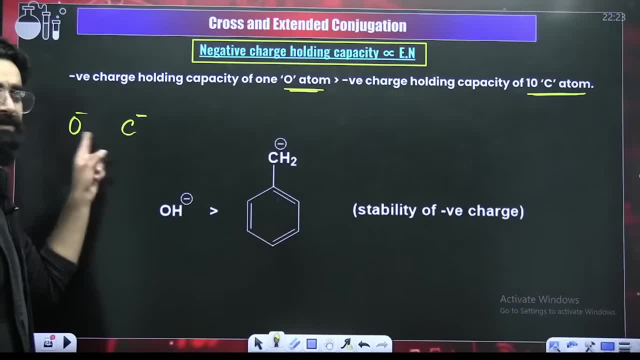 atoms, for example. oxygen is getting atoms. for example, oxygen is getting. negative carbon is getting negative. negative carbon is getting negative. negative carbon is getting negative right oxygen carbon. they belong to same right oxygen carbon. they belong to same right oxygen carbon. they belong to same period, same period. electro negativity. 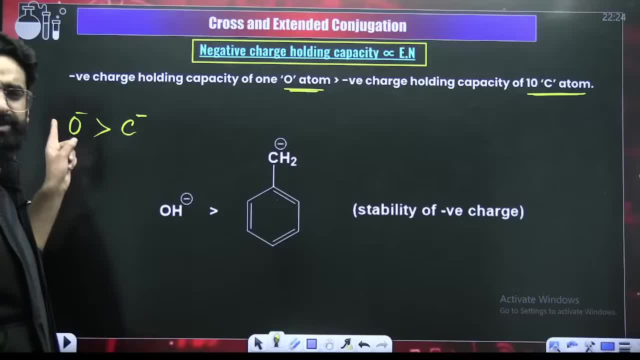 period- same period. electro negativity period: same period. electro negativity: negative charge is more stable and more negative. charge is more stable and more negative. charge is more stable and more electronegative right, so negative charge. electronegative right, so negative charge. electronegative right, so negative charge, of course, will be stable on oxygen. 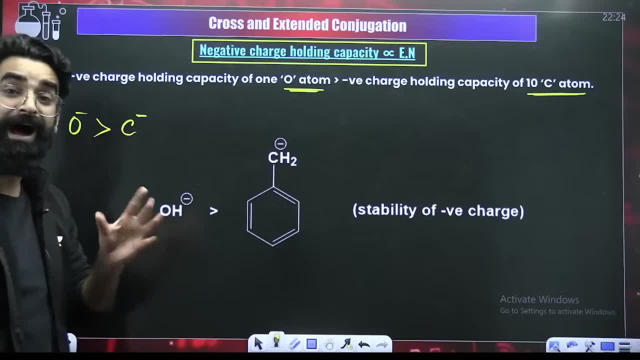 of course will be stable on oxygen. of course will be stable on oxygen. it'll be more stable in oxygen, but it'll be more stable in oxygen, but it'll be more stable in oxygen. but if you want to see how much stable this, if you want to see how much stable this, 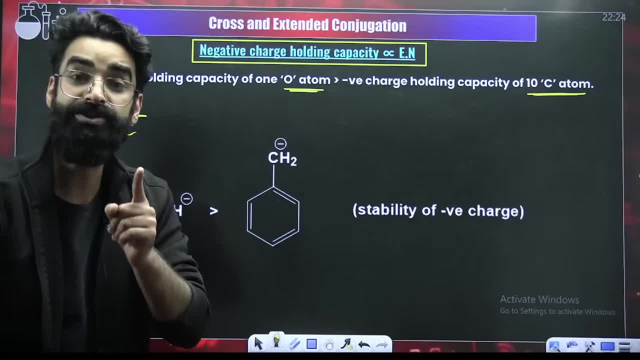 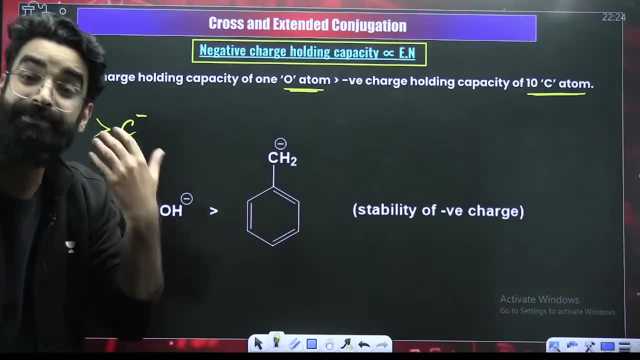 if you want to see how much stable this negative charge and oxygen will be negative charge and oxygen will be negative charge and oxygen will be negative charge will be an oxygen as that negative charge and oxygen will be an oxygen as that negative charge and oxygen will be an oxygen as that of carbon. 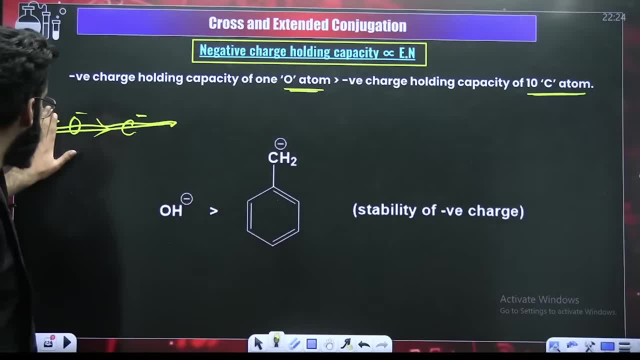 of carbon, of carbon as there of carbon. now you tell me one as there of carbon. now you tell me one as there of carbon. now you tell me one thing now, you just tell me one thing thing now, you just tell me one thing thing. now, you just tell me one thing: look at these two molecules. this is: 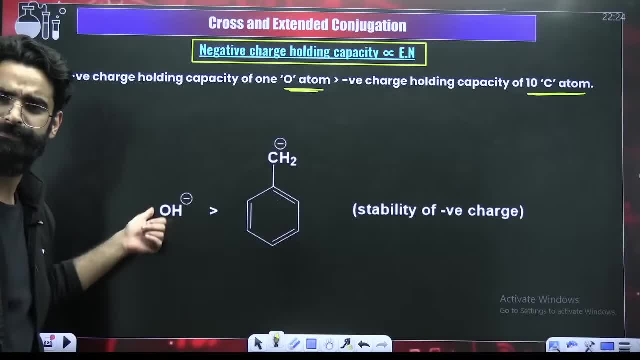 look at these two molecules, this is: look at these two molecules. this is oh negative, oh negative, oh negative. this was negative oxygen carrying, this was negative oxygen carrying, this was negative oxygen carrying, negative, negative, negative. but over here, over here, is there any? but over here, over here, is there any? 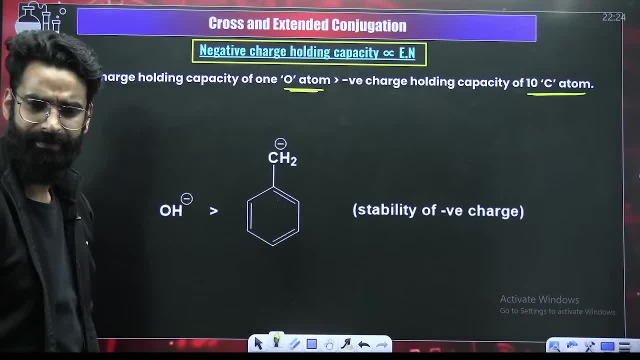 but over here, over here, is there any oxygen, oxygen, oxygen, there's no oxygen, but i would say resonance will be there, but i would say resonance will be there. but i would say resonance will be there. this will come here, this will go here, and this will come here, this will go here and 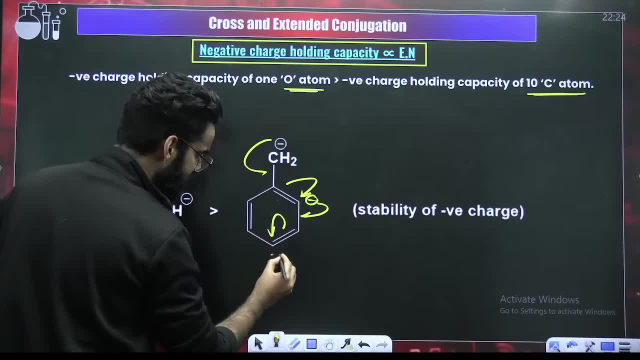 this will come here, this will go here, and there'll be a negative here. then there'll be a negative here, then there'll be a negative here. then negative comes here, this will go on. this negative comes here. this will go on. this negative comes here, this will go on this side. negative comes on here, then this. 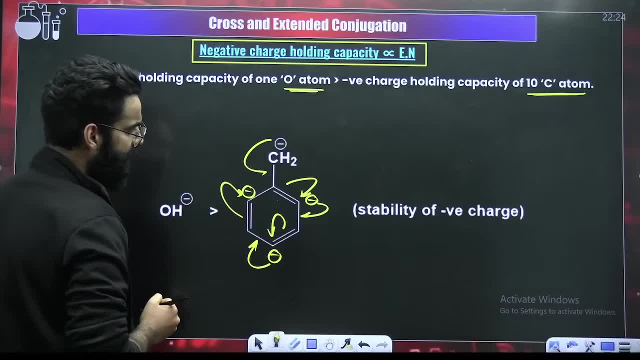 side negative comes on here, then this side negative comes on here, then this will shift here and this will shift here, will shift here and this will shift here, will shift here and this will shift here. negative comes here, perfect. negative comes here. perfect. negative comes here, perfect. that's something which will happen. 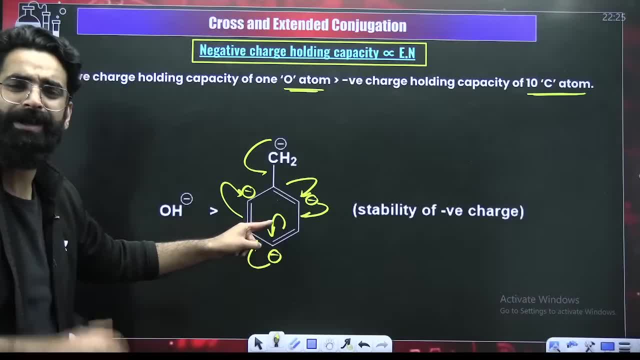 that's something which will happen. that's something which will happen. so, in this particular molecule, where so? in this particular molecule, where? so? in this particular molecule, where all nigiru charge is getting generated, all nigiru charge is getting generated, all nigiru charge is getting generated. it was there. now the nigiru charge is. 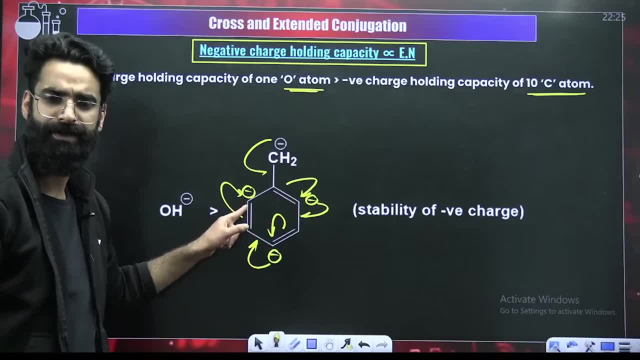 it was there. now the nigiru charge is. it was there. now the nigiru charge is getting generated at this position, at getting generated at this position, at getting generated at this position, at this position, at this position, this position, at this position, this position, at this position, perfect. no doubt there is dispersion of 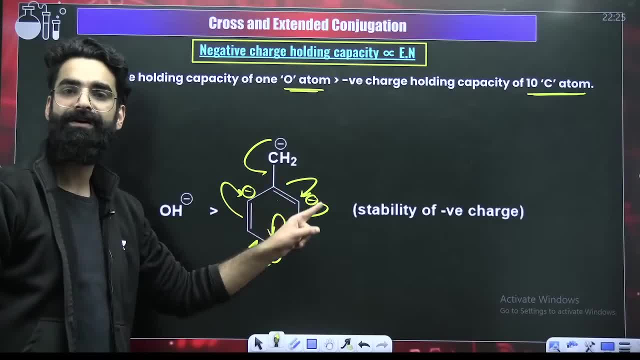 perfect. no doubt there is dispersion of perfect. no doubt there is dispersion of nigiru charge. nigiru charge, nigiru charge. there is dispersion of nigiru charge. there is dispersion of nigiru charge. there is dispersion of nigiru charge. nigiru charge is coming on. one, two, three. 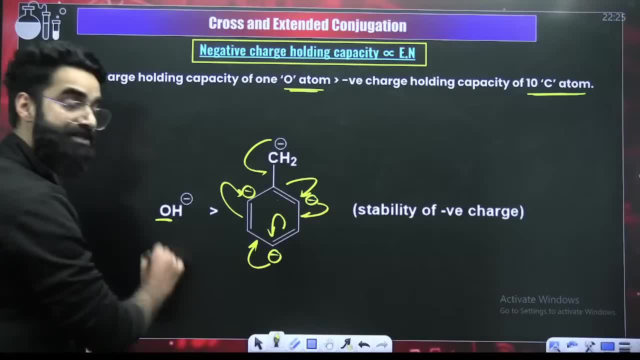 nigiru charge is coming on one, two, three nigiru charge is coming on one, two, three, four, four carbon atoms, four, four carbon atoms, four, four carbon atoms. but here the nigiru charge is in oxygen. but here the nigiru charge is in oxygen. 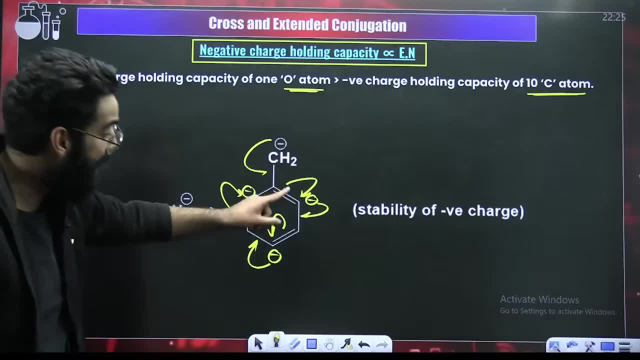 but here the nigiru charge is in oxygen, so can you compare the stability of so? can you compare the stability of so? can you compare the stability of nigiru charge, nigiru charge, nigiru charge. no doubt here nigiru charge is getting. 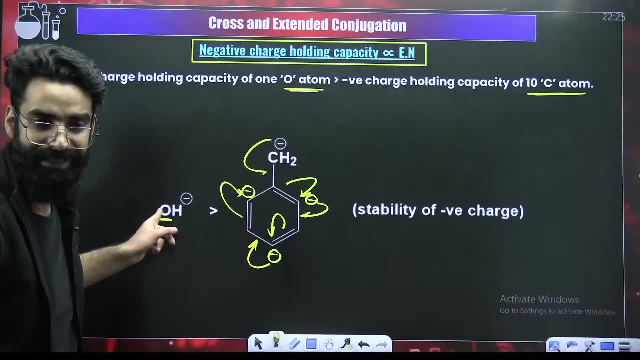 no doubt here nigiru charge is getting, no doubt here nigiru charge is getting dispersed on four oxygen atoms, but dispersed on four oxygen atoms, but dispersed on four oxygen atoms. but in this case, in the first case, in the, in this case, in the first case in the, 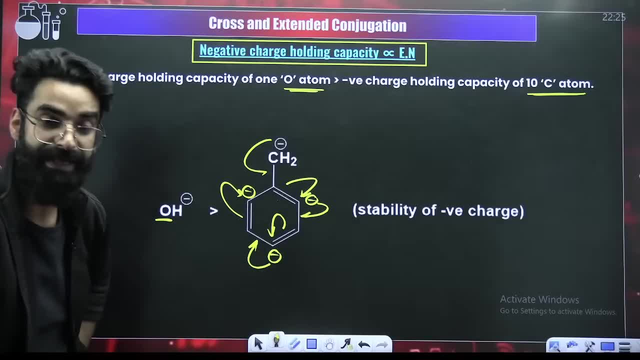 in this case, in the first case, in the first case, in the first case. nigiru charge, first case, in the first case. nigiru charge, first case. nigiru charge is on oxygen, so tell me where is the is on oxygen, so tell me where is the. 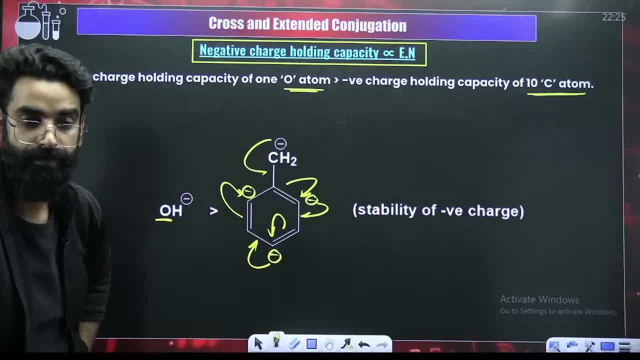 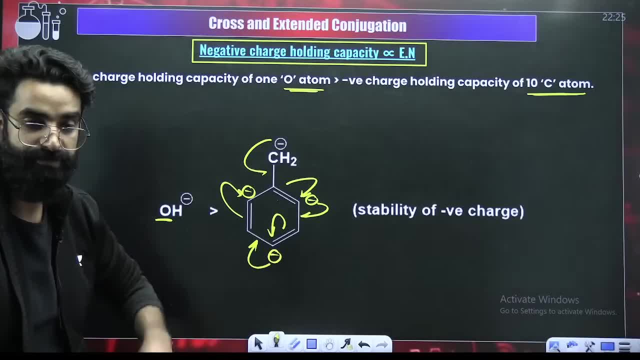 first or second quickly. first or second quickly. first or second quickly. where is the nigiru charge more stable? where is the nigiru charge more stable? where is the nigiru charge more stable, first or second? first or second? first or second? guys, you have to tell me the answers in. 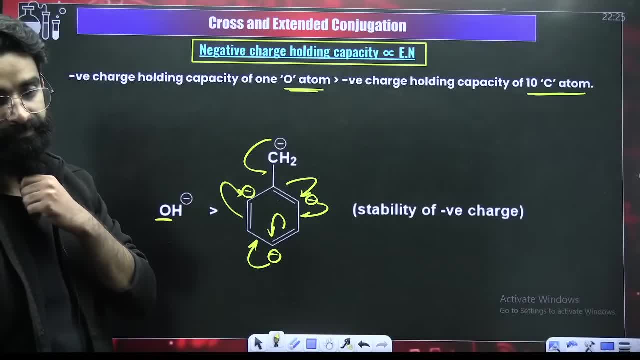 guys, you have to tell me the answers in. guys. you have to tell me the answers in the charts quickly. look at this statement. i told you, nigiru, look at this statement. i told you nigiru, look at this statement. i told you, nigiru, charge holding capacity of oxygen is: 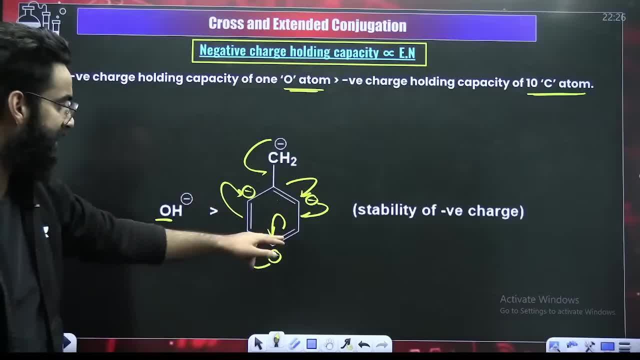 charge. holding capacity of oxygen is charge. holding capacity of oxygen is greater than nigiru charge. holding greater than nigiru charge. holding greater than nigiru charge. holding capacity of 10 carbon atoms here nigiru. capacity of 10 carbon atoms here, nigiru. 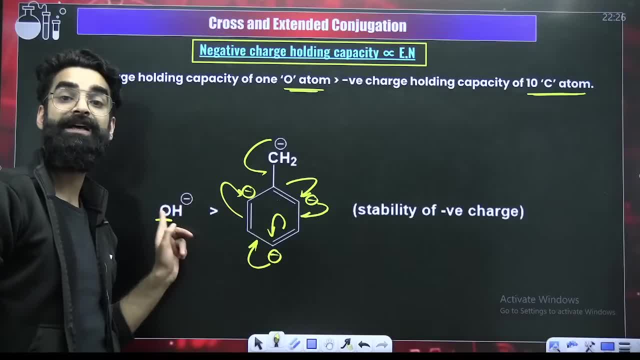 capacity of 10 carbon atoms. here nigiru charge is spread on four carbons charge is spread on four carbons charge is spread on four carbons. here nigiru charge is alone on oxygen. here nigiru charge is alone on oxygen. here nigiru charge is alone on oxygen. but you know, nigiru charge carrying 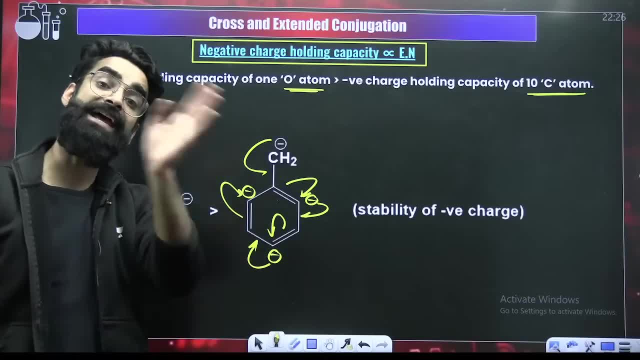 but you know nigiru charge carrying. but you know nigiru charge carrying capacity of oxygen is greater than the capacity of oxygen is greater than the capacity of oxygen is greater than the nigiru charge carrying capacity of 10. nigiru charge carrying capacity of 10. 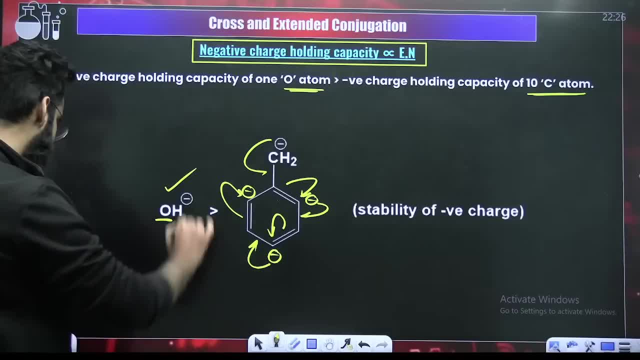 nigiru charge. carrying capacity of 10 carbon atoms: right. so where is the carbon atoms? right? so, where is the carbon atoms right? so where is the nigiru charge? more stable in the first nigiru charge? more stable in the first nigiru charge. more stable in the first case? 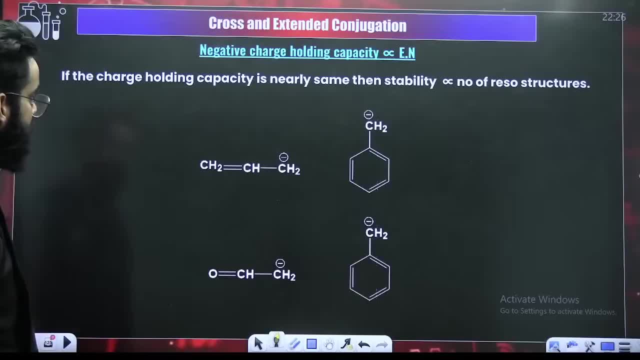 case case in the first case. right, okay, in the first case. right, okay, in the first case, right, okay, tell me among these two, among these two. tell me among these two, among these two. tell me, among these two, among these two, which one is more stable among these two? 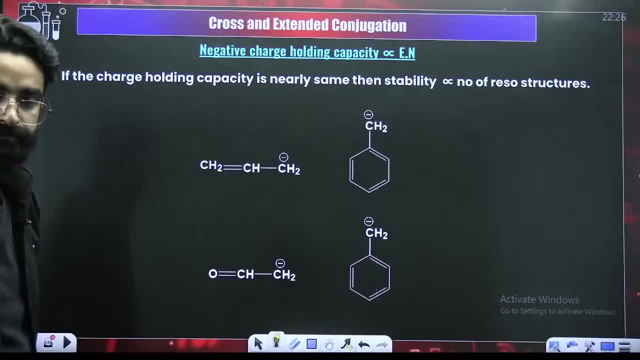 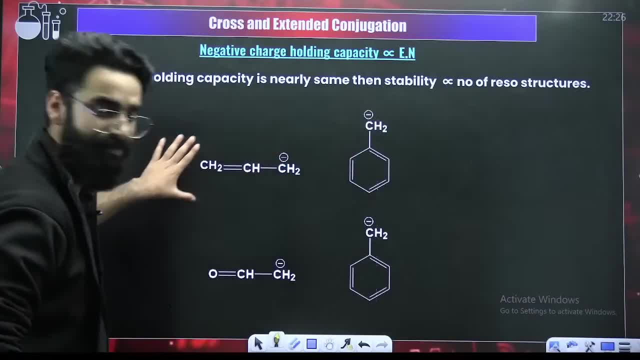 where is the nigiru charge more stable? where is the nigiru charge more stable? so, first of all, no more electronegative. so, first of all, no more electronegative. so, first of all, no more electronegative element. or everywhere there is carbon. 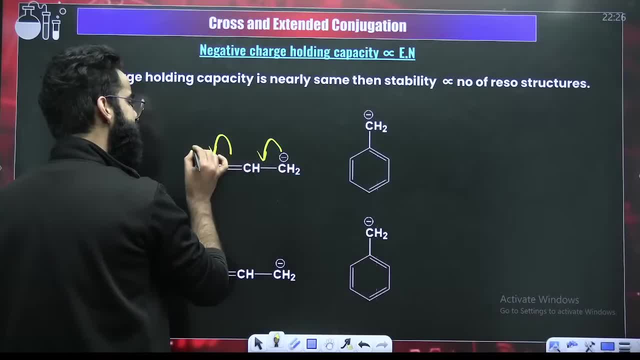 element, or everywhere there is carbon element, or everywhere there is carbon. carbon right, so resonance can happen. carbon right, so resonance can happen. carbon right, so resonance can happen. and due to resonance, this nigiru charge and due to resonance, this nigiru charge and due to resonance, this nigiru charge can come here. similarly, due to resonance. 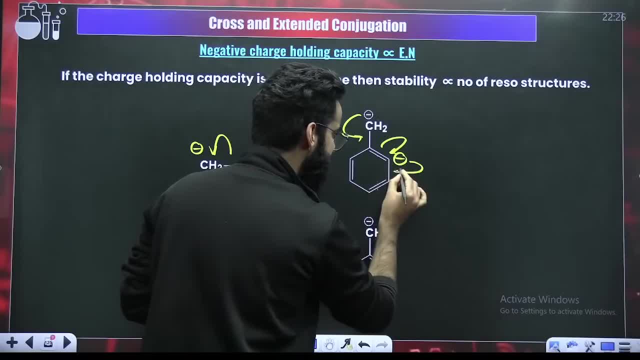 can come here, similarly due to resonance. can come here similarly due to resonance. this nigiru charge can first come here. this nigiru charge can first come here. this nigiru charge can first come here, then the same nigiru charge will come. then the same nigiru charge will come. 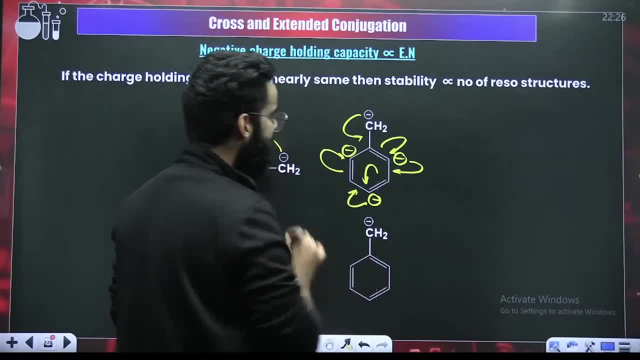 then the same nigiru charge will come here. then the same nigiru charge will come here, then the same nigiru charge will come here, right? so where is the dispersal here? right? so where is the dispersal here? right? so where is the dispersal of nigiru charge? more? 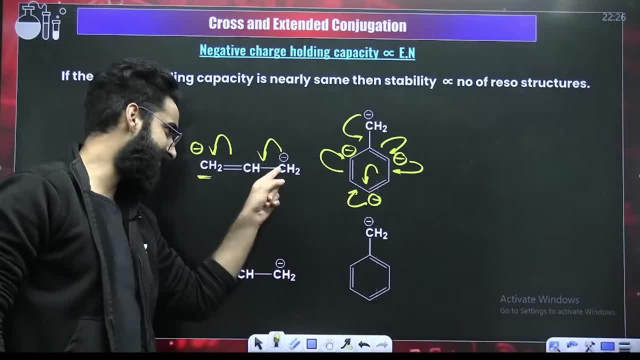 of nigiru. charge more of nigiru. charge more in the second case. in the second case, in the second case. right in this, since everywhere there's right in this, since everywhere there's right in this, since everywhere there's carbon. again, everywhere there's carbon. no, 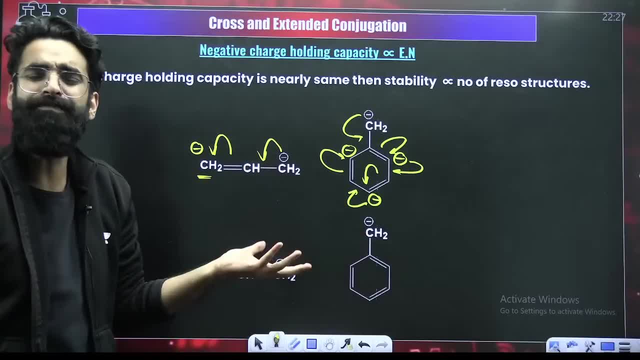 carbon again: everywhere there's carbon. no carbon again: everywhere there's carbon. no electronegative element, nothing right. electronegative element, nothing right. electronegative element, nothing right. so here you'll be simply seeing the. so here you'll be simply seeing the. 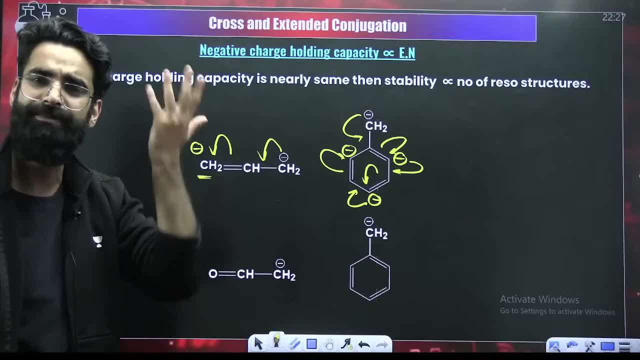 so here you'll be simply seeing the dispersal of charge. wherever dispersal of dispersal of charge, wherever dispersal of dispersal of charge, wherever dispersal of charge is more. stability is more is more stability is more stable, right. so where is the nigiru charge? 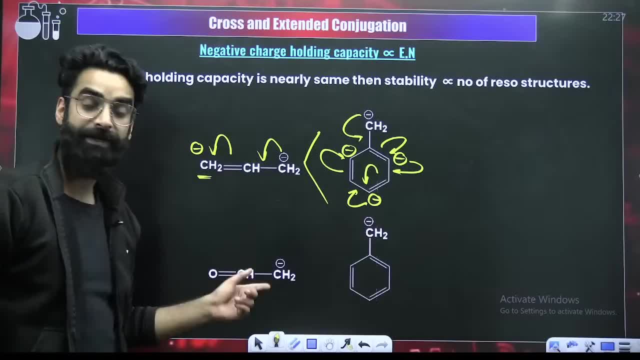 right, so where is the nigiru charge? right, so where is the nigiru charge? more stable, more stable, more stable. okay, look at this one, look at this one. okay, look at this one, look at this one. okay, look at this one, look at this one. here you have got oxygen. no oxygen here. 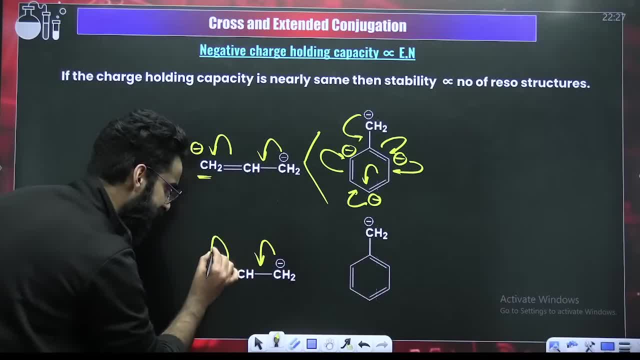 here you have got oxygen. no oxygen here. here you have got oxygen. no oxygen. here, no oxygen. it's evident. if this undergoes no oxygen, it's evident if this undergoes no oxygen, it's evident if this undergoes resonance, nigiru charge will automatically. resonance nigiru charge will automatically. 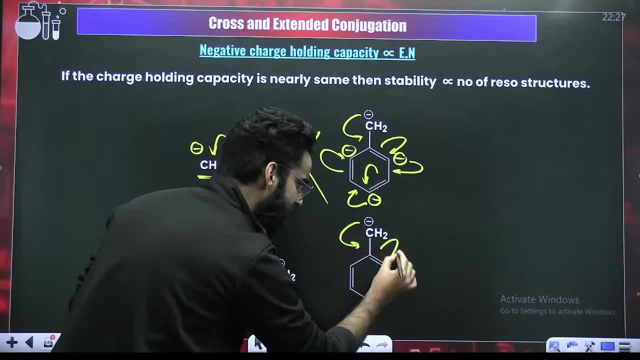 resonance nigiru charge will automatically come on oxygen. come on oxygen. come on oxygen if this undergoes resonance nigiru charge. if this undergoes resonance nigiru charge, if this undergoes resonance nigiru charge, can come here then. can come here then. 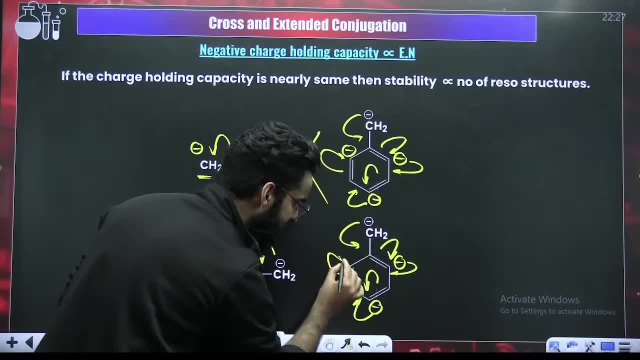 can come here, then then it can go downwards, then it can, then it can go downwards, then it can, then it can go downwards, then it can. come this side right, come this side right, come this side right. nigiru charge is spread on one, two, three. nigiru charge is spread on one, two, three. 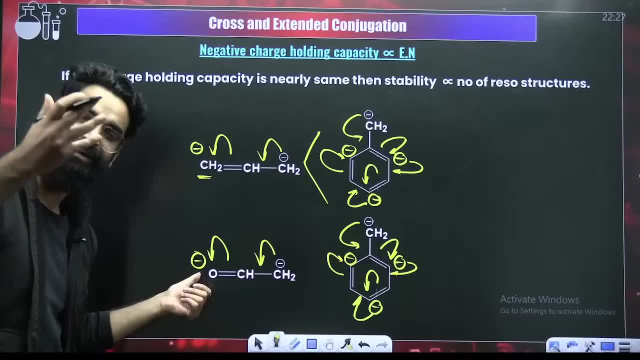 nigiru charge is spread on one, two, three, four, four carbon atoms. but here four, four carbon atoms. but here four, four carbon atoms. but here one oxygen atom alone is enough, right. one oxygen atom alone is enough, right. one oxygen atom alone is enough, right. one oxygen atom alone is enough. 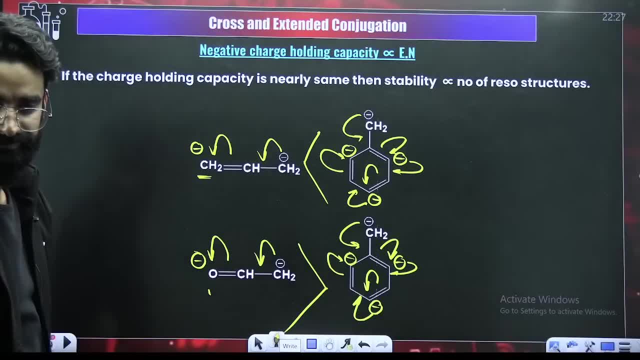 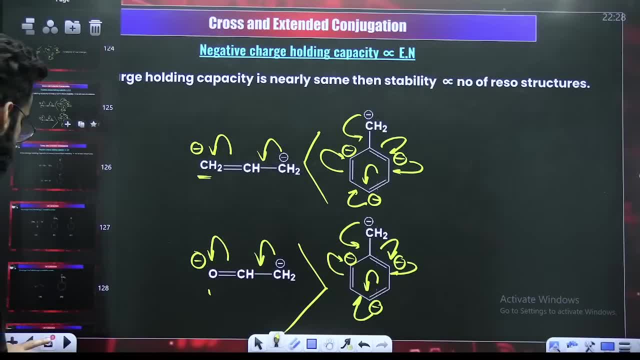 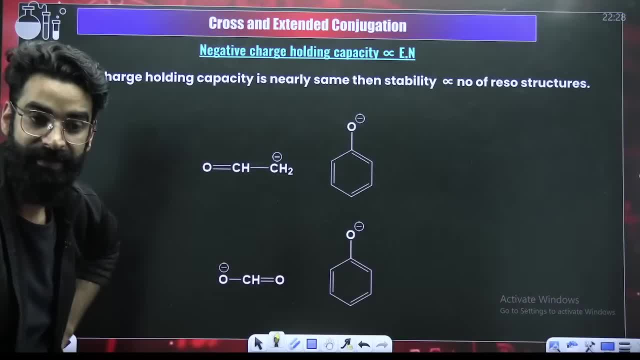 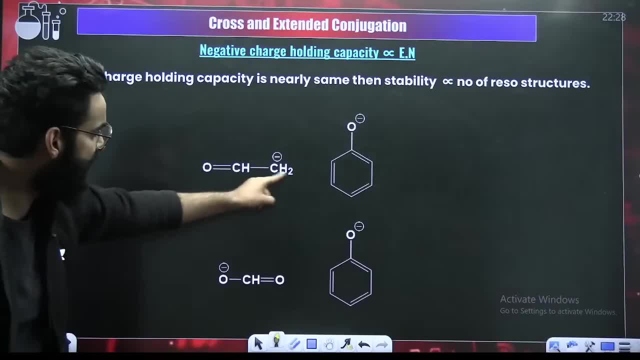 where is the negative charge more stable quickly? you have to answer this question quickly. you have to answer this question quickly. you have to answer this question: where is the negative charge more stable? where is the negative charge more stable? where is the negative charge more stable among these two? 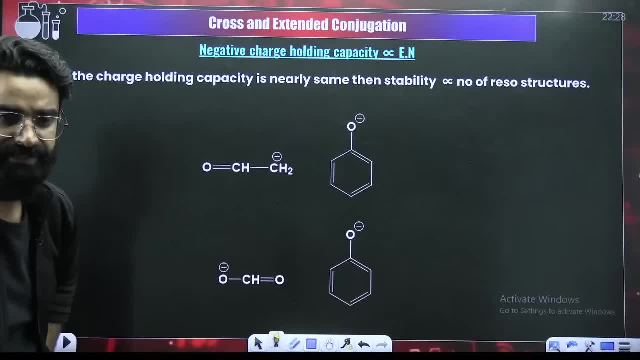 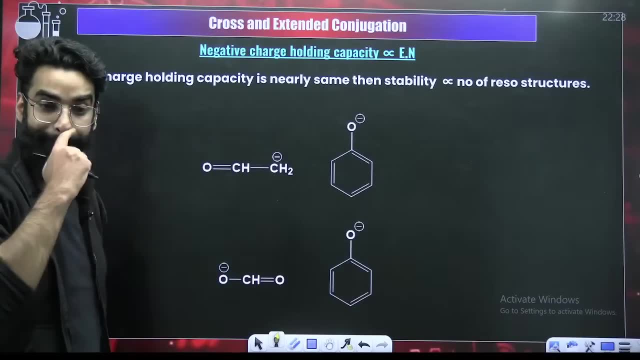 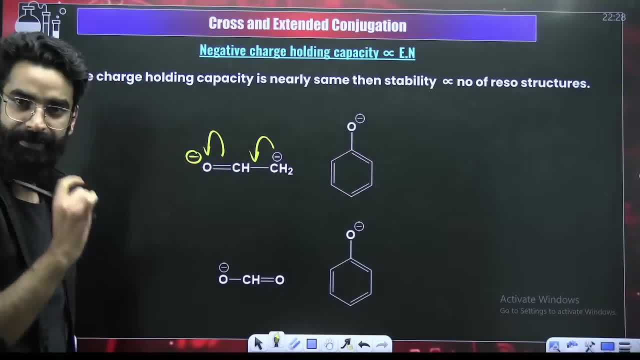 see, this can undergo resonance and this bond will shift in this direction. due to bond will shift in this direction. due to bond will shift in this direction. due to which oxygen will get negative, so negative. which oxygen will get negative, so negative. which oxygen will get negative, so negative. charge is on one carbon and one oxygen. 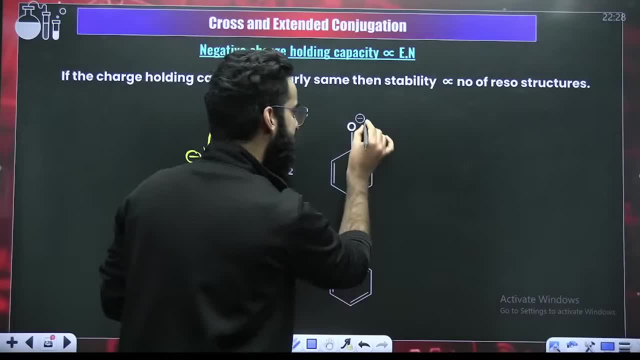 charge is on one carbon and one oxygen charge is on one carbon and one oxygen, but here already the negative charge is, but here already the negative charge is. but here already the negative charge is on oxygen, now when it undergoes on oxygen, now when it undergoes. 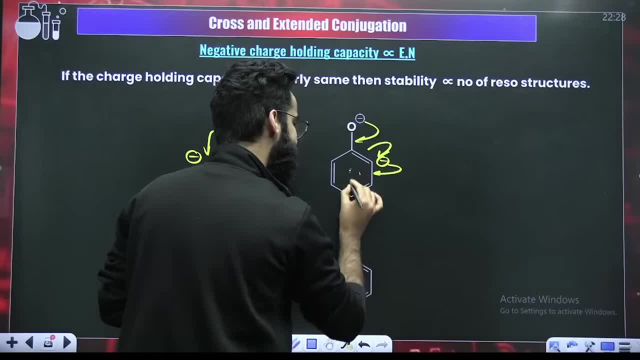 on oxygen. now, when it undergoes resonance, this negative charge can come resonance. this negative charge can come resonance. this negative charge can come here, or the same negative charge can here, or the same negative charge can here, or the same negative charge can come here. here the negative charge was. 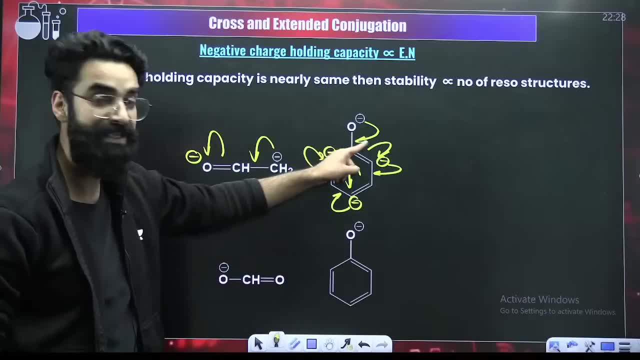 come here here. the negative charge was. come here here. the negative charge was on oxygen. apart from that, due to on oxygen, apart from that, due to on oxygen, apart from that, due to resonance: it is coming on three carbon resonance. it is coming on three carbon resonance. it is coming on three carbon atoms. 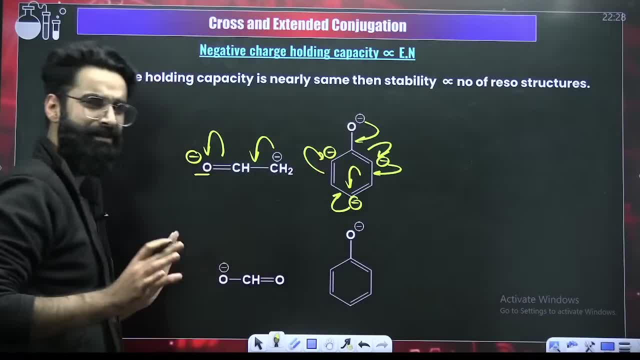 atoms, atoms, so leave. you cannot decide on the base, so leave. you cannot decide on the base, so leave. you cannot decide on the base of oxygen, oxygen oxygen of oxygen, oxygen oxygen. 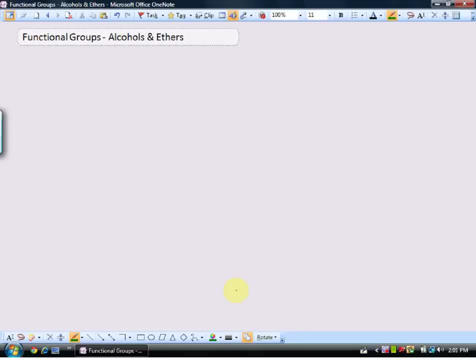 Okay, here we go. We're going to talk today about functional groups in organic chemistry, And functional groups are where we add dip atoms other than carbon and hydrogen to the carbon framework, And these functional groups create special places within the molecule that give it special properties or functions. Therefore, we call them functional groups. 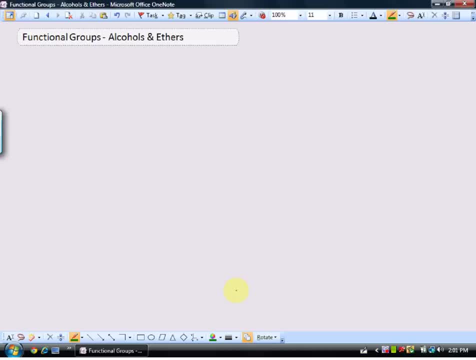 You might think of adding these atoms, and the atoms we're going to talk about are oxygen and nitrogen. Adding these atoms adds a little bit more personality to the basic hydrocarbon. Again, it's the carbon that makes up the bulk of the structure, but it's these other atoms. 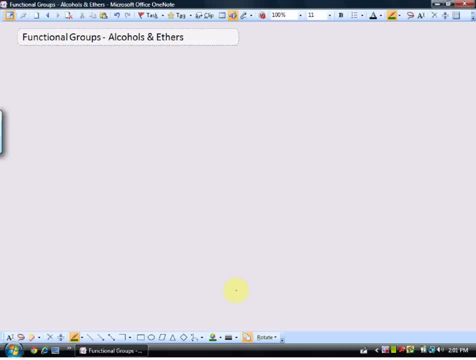